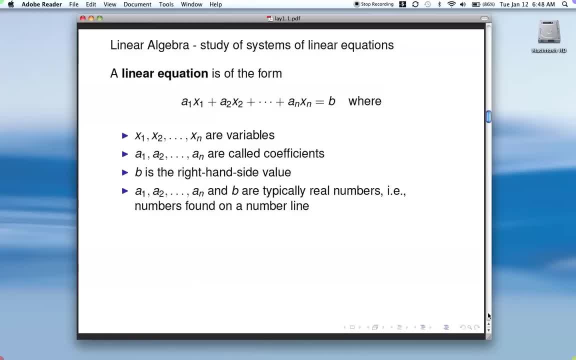 Rational numbers, irrational numbers, negative numbers, positive numbers, zero- Just about any number or any number you can find on a number line is a real number. This is as opposed to complex or imaginary numbers. Those would not be real numbers. So for our purposes we'll not be dealing with complex numbers. 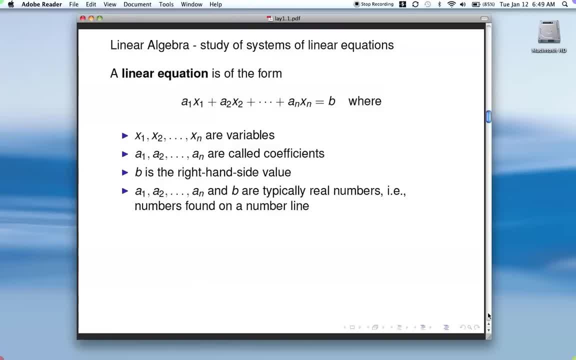 We'll stick to just real numbers In our equations. the linear part means that we don't allow non-linear expressions of the variables, So terms like x1 squared or x1 times x2.. Those type terms are non-linear and so we don't allow those type expressions. 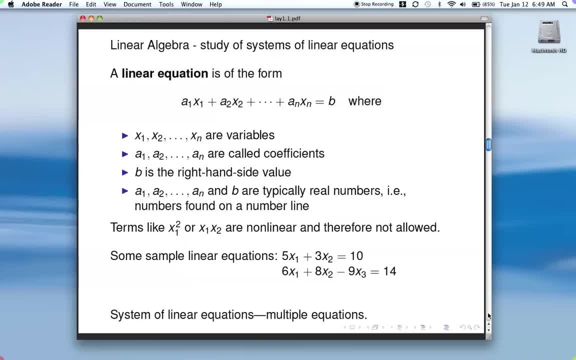 So here's a couple of sample linear terms, A couple of sample linear equations. You know, those are just typical. First one has two variables here, Here's one with three variables. This one, first one, you'll recognize, it's got two variables. 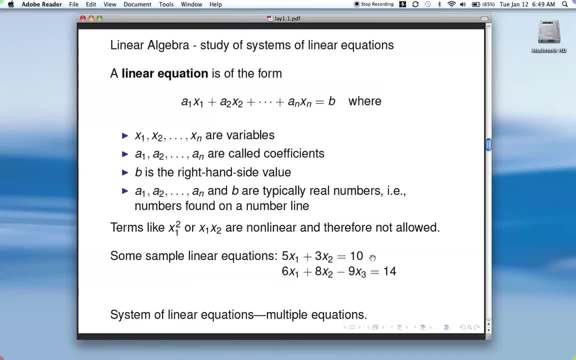 So that just defines a line in the plane. In the xy plane here Got three variables, so that actually defines a plane in three dimensions. So we'll talk more about that as we go along. So we're back to what is linear algebra. 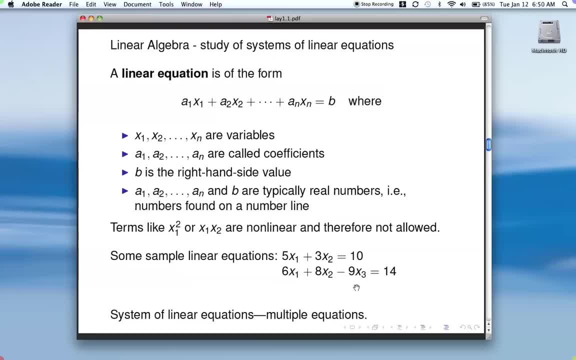 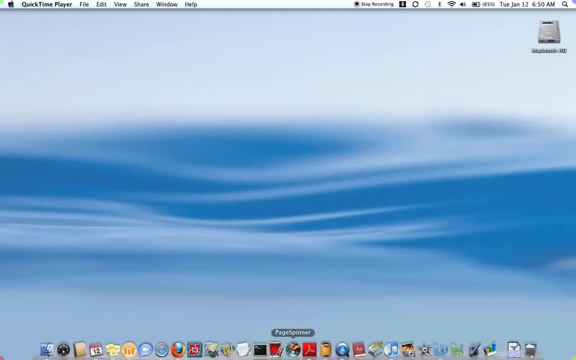 So we've talked about what's a linear equation, And linear algebra is the study of systems of linear equations. So what's a system? That just means you have multiple equations. So, for example, let's go to the drawing board. Here's a system of two equations. 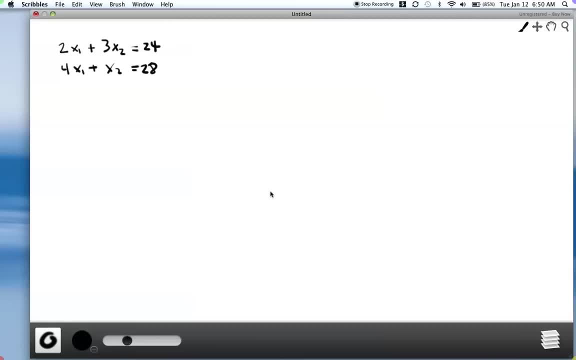 You have two equations and two unknowns, And all of you have had college algebra, So you're familiar with a system of this form And you probably learned a couple of different ways to solve this system when you were in algebra, And so we're just going to talk about that first off here. 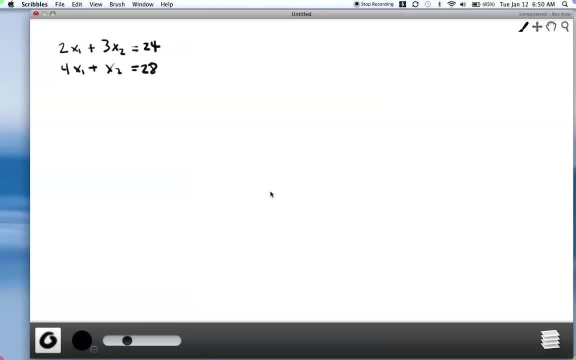 If I asked you how would you solve this system, then you might say: well, I'd use substitution, Because that seems like a way to go. If you look here, you've got the x2 term. You can solve this equation for x2.. 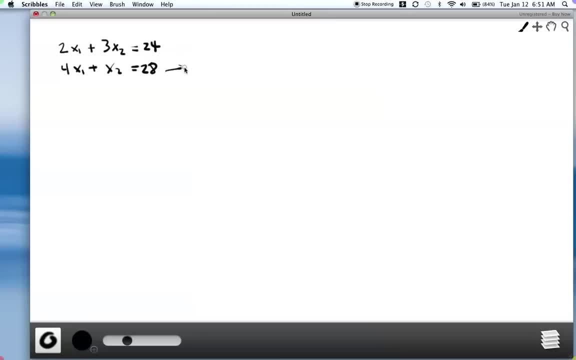 So let's do that, So from this equation I can get: x2 equals 28 minus 4x1. And then I substitute this expression for x2 back into the first equation, So that gives me 2x1 plus 3 times this stuff here. 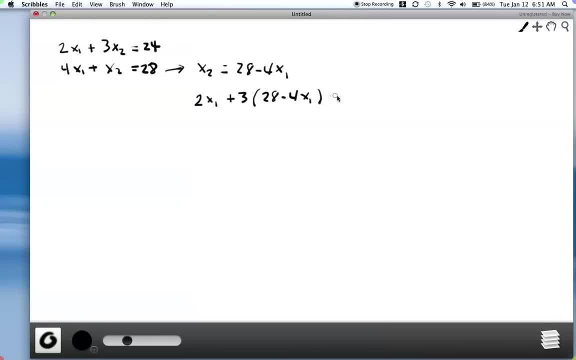 28 minus 4x1.. And that equals 24.. So then I simplify: 2x1 plus 3 times 28 is 84.. Minus 12x1 equals 24.. So that gives me 10x1 equals. 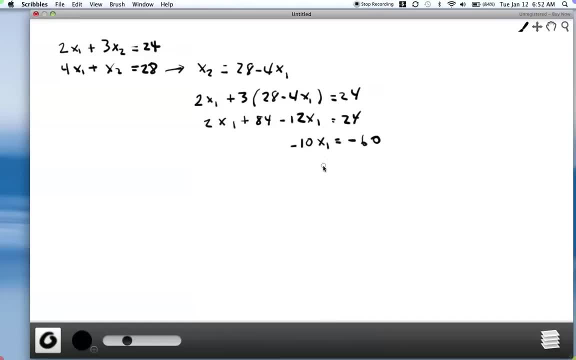 24 minus 84 would be negative 60. So it looks like x1 is equal to 6.. And then if x1 is 6, we can go back and plug in here to figure out what x2 is. So x2 is going to be 28 minus 4 times 6.. 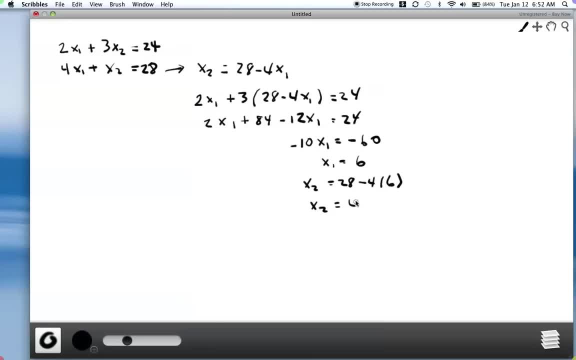 So x2 is equal to 4.. So, oops, Back up there. So x, Ah, do it again, x. There we go. x2 equals 4.. x1 equals 6 is our solution. So that's one way to solve this system. 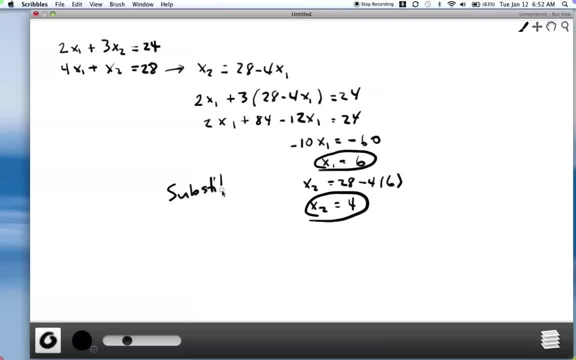 That's using the method of substitution. Another method that's sometimes used is to Go back and look at the system and try to eliminate one of the variables by multiplying one of the equations or maybe even both the equations by a constant and then adding or subtracting one from the other. 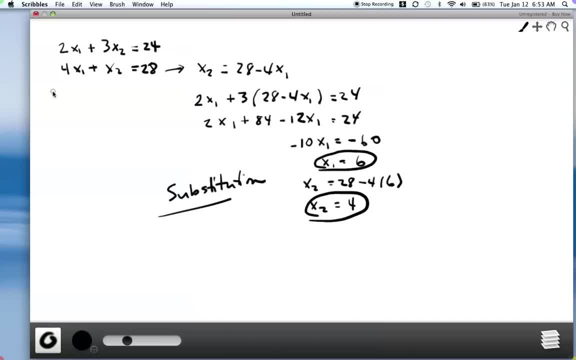 So I'm going to try that method here. So I'm going to multiply this first equation by negative 2.. Okay, and I'll just write what I get down here. So negative 2 times 2x1 gives me negative 4x1.. 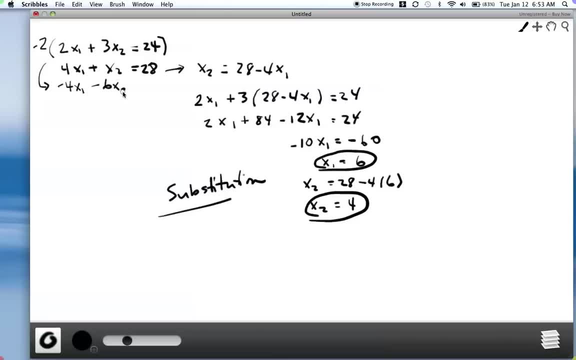 And then negative 6x2.. And then negative 2 times 24 would be negative 48. And then if I add these two together, these two that I have here, then notice that the x1s cancel out. So they're gone. 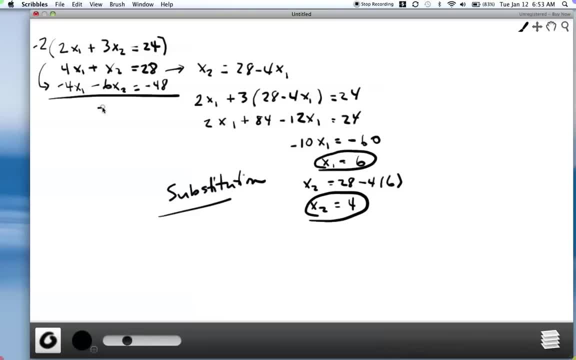 I've eliminated x1 in here. If I add, I get negative. 5x2 equals negative 20. So that says x2 equals 4. And then to get x1, I can substitute that back into either of these equations. 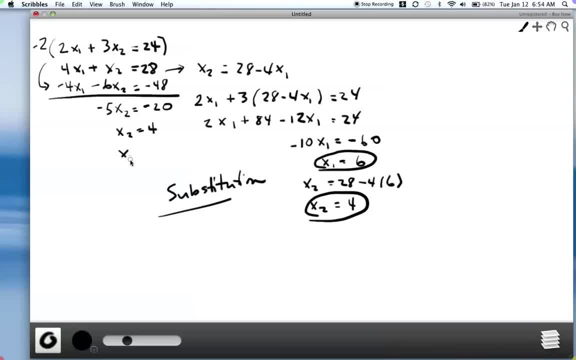 And we already know that x1 is 6, so I won't go through that process. Okay, so there we go. We have our solution, And that's using the method of elimination. Okay, systematically eliminate variables. So those are the two methods that you probably learned back in algebra class for solving this system. 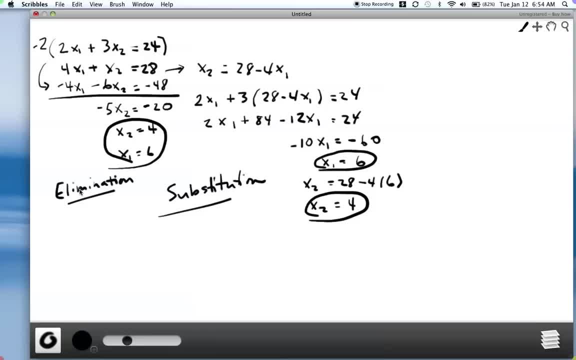 Let's take a look at what we're doing graphically. Let's take a graphical look at it. So I go back to my equations and I draw them on a graph. Let's see if I can come over here, And I'll try to do this. 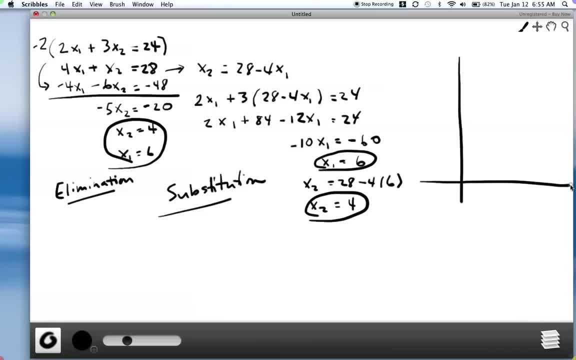 All right. so if I graph my equations where this is going to be my x1 axis, this will be my x2 axis And let's see, If I look at the first equation, if x1 is 0,. well, actually I'm going to start with this one. 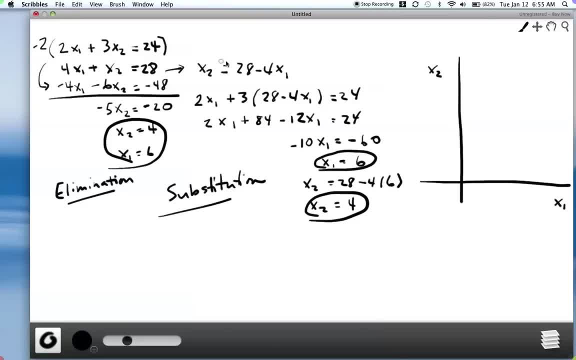 because if x1 is 0 here, then x2 is 28.. So that gets us way up here. So there's 28.. So I've got one point right there at 0, 28.. Then if x2 is 0, we get x1 equals 7.. 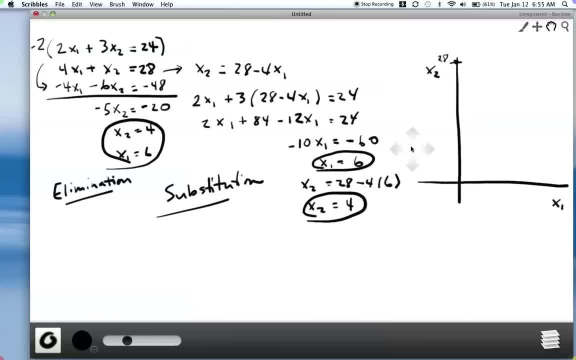 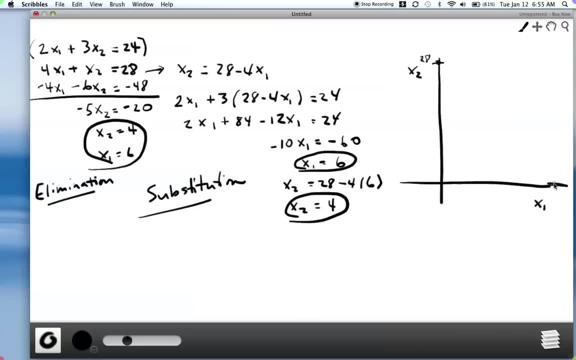 So I'm going to scoot this over just a little bit to give me a little more room here. Look this out. Okay, so it looks like. let me try to get my scale as best I can, So it looks like this would be about 7.. 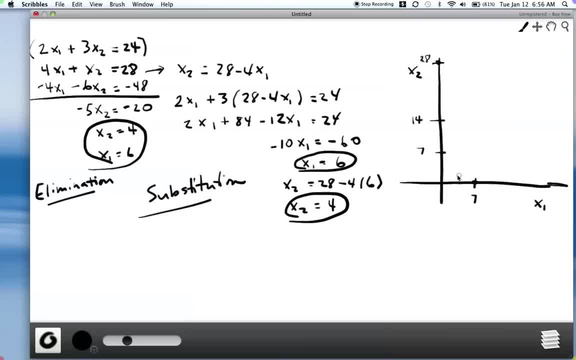 And so my other point is here at 7, 0.. So I've got one line that comes like this, And let me see if I can do a better job drawing that. Apparently I'm not. Let me get a little better angle on that with my computer here. 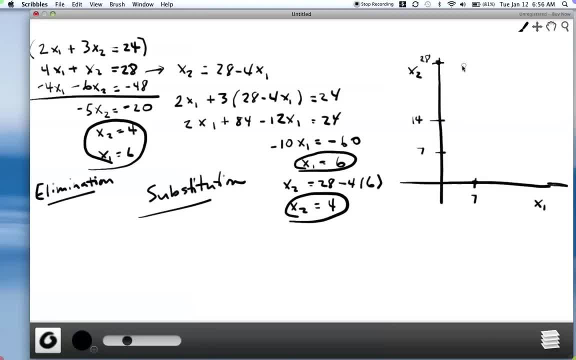 Okay. well, that's not very good either. Let's try one more time. Looks like I am. I'm not going to be able to make this work. Let's see one more time. Okay, I'm going to just call that good. 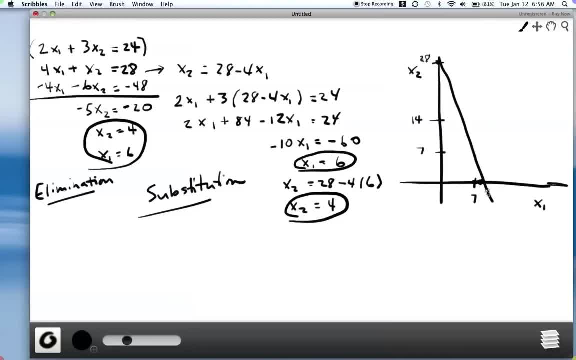 Let's call this 7, right here. All right, so then let's do. let's look at the other one. The other equation is- I've got this one- If x1 is 0, it looks like x2 is 8.. 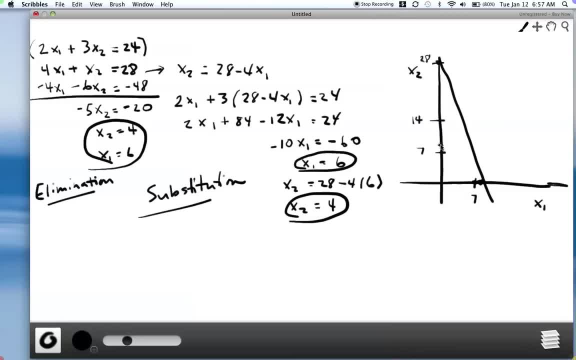 So that's going to be along about right there. And if x2 is 0, it looks like x1 is 12.. So that's going to be somewhere along about right here. Let me try once again see if I can make a line. 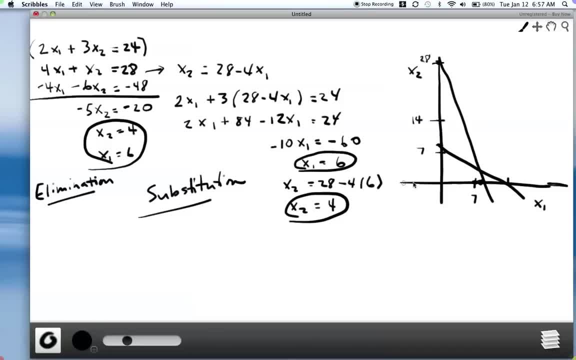 That one's not terrible there, All right. so this is about 7, right there, Let's take that away, All right. so if we look, my scale is better, It would be better to see, But along about there. that's the point where those lines intersect. 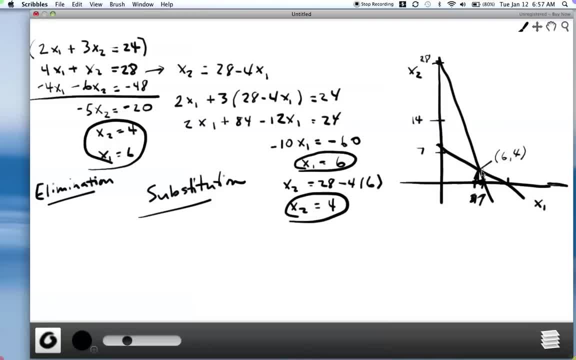 And so that's the point 6, 4.. So my scale is better. It would look better, But you get the general idea. So what we're looking at here is: we've got this system And we want to find x1 and x2 that satisfy both those equations. 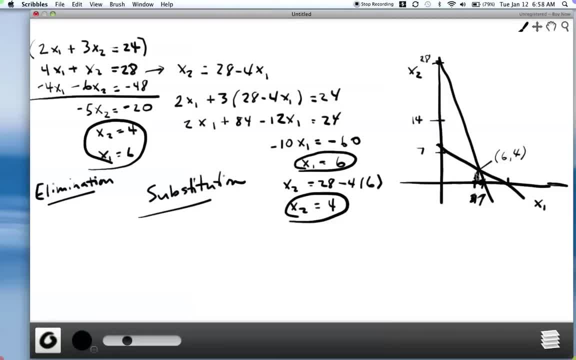 So since each of those equations represents a line, then we're looking for a point that satisfies both, And that means it's a point that's on both lines. So that's the point where the lines intersect. OK, so in this example, we ended up with a unique solution. 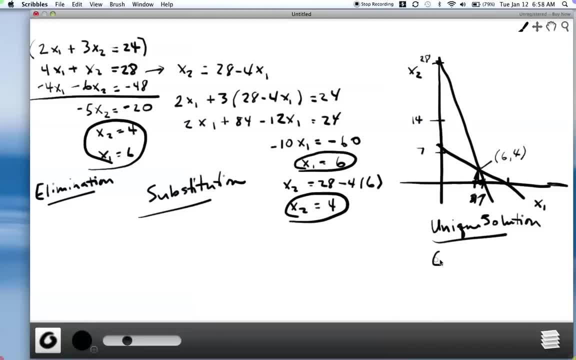 All right, a unique solution. That means exactly one solution. OK, now let's think: Are there any other possibilities? No matter what your system is, you're always going to have exactly one solution. I think you know that that is not the case. 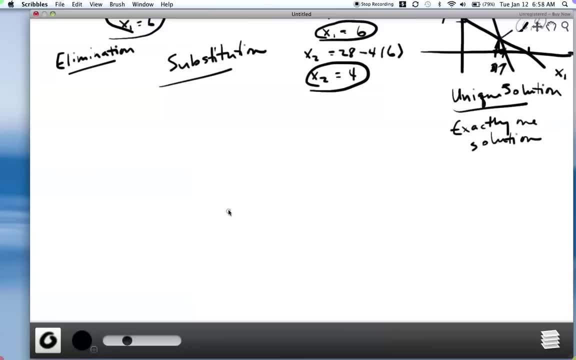 So what are the possibilities? You don't have exactly one solution. How about do you have a solution every time? And you probably know that the answer is no, And that happens when you have a solution. You have a situation like this. There's one line: 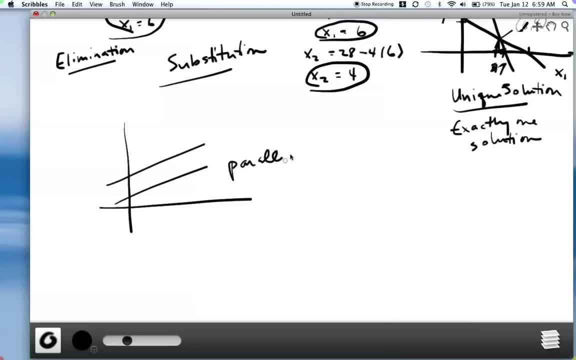 There's another. They're parallel And so they never intersect, And so this case you have no solution. No solution in that case. OK, so we've got zero solutions. You have one solution. How about two? Can you come up with a system where you have two solutions? 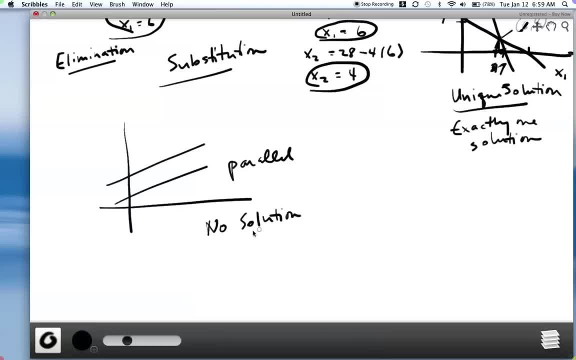 Let's think on that Two solutions Now. in my class one day I had somebody say: well, what if you drew another line here? So you had a line like this: Right, Then you got the intersect there, the intersect there. 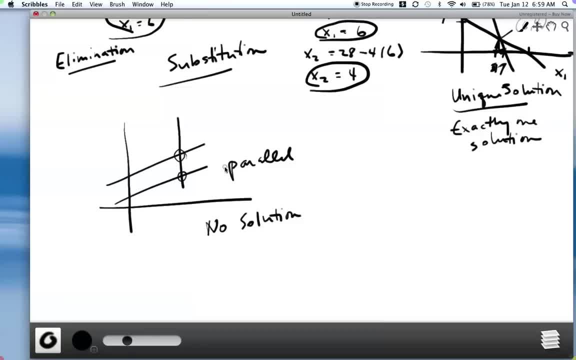 So there's two solutions, right? And the answer is well no, because here you've got three lines, And so if you were trying to solve a system with these three lines, then that means that you need to find a point where all three intersect at the same time. 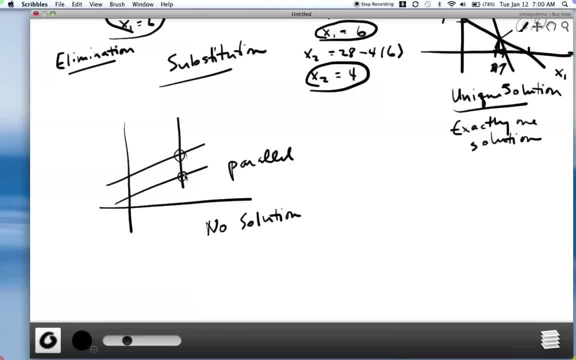 So in this case there's still no solution because there's no point at which all three lines intersect. I've also had students say: well, hey, what if you had a parabola? Say you had a case like this. There's a parabola. 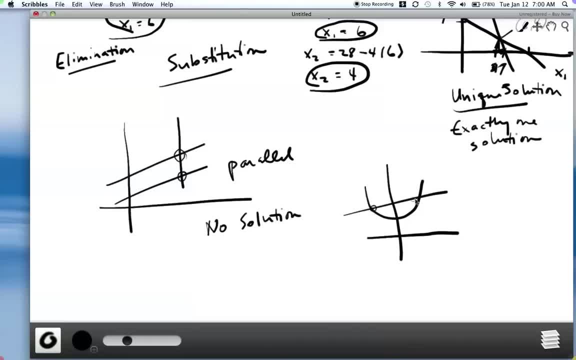 You've got a line going through it. Look there, they intersect right there, intersect right there. So you've got two solutions. Now this is legitimate because you've got two solutions, You've got two functions and they intersect at these two places. 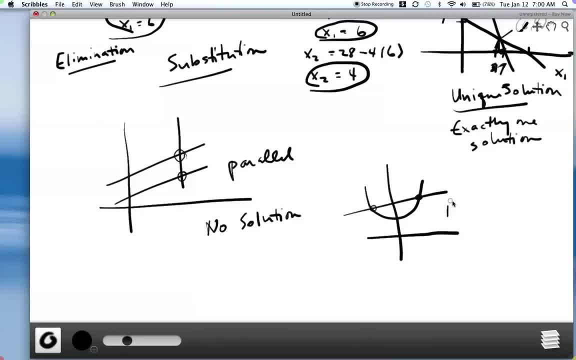 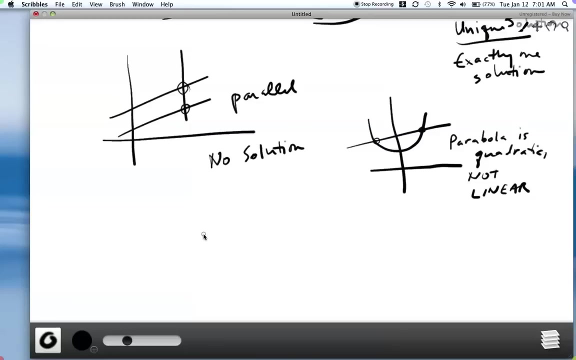 The problem is that this parabola is not a linear function. The parabola is quadratic, not linear, So that case doesn't work either. So it turns out that if you have a system of linear equations and you don't have no solution, 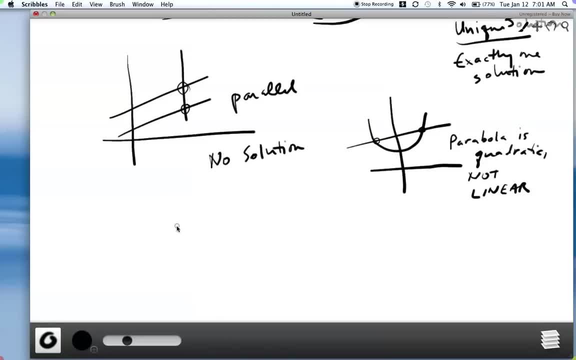 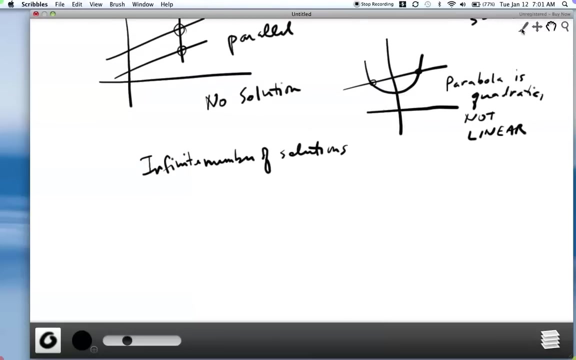 you don't have exactly one solution, then you must have an infinite number of solutions. So infinite number of solutions, And in two dimensions. that's a little bit tough to come up with a good example. The best you can do is two dimensions, is one like this: 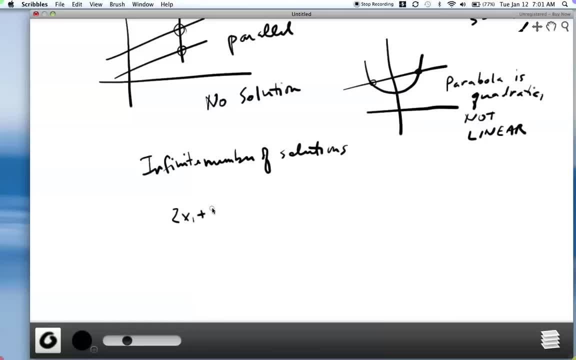 where you have something like 2x1 plus 3x2 equals 10, and then maybe 4x1 plus 6x2 equals 20.. Now on the surface it looks like, yeah, you've got two. 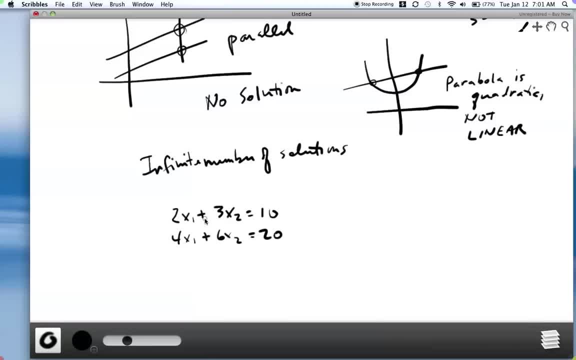 You've got a system of equations, You've got two equations, But when you go to graph this, what do you find? Well, you find that this is actually the same equation, because I wrote it so that the second one was just a multiple of the first. 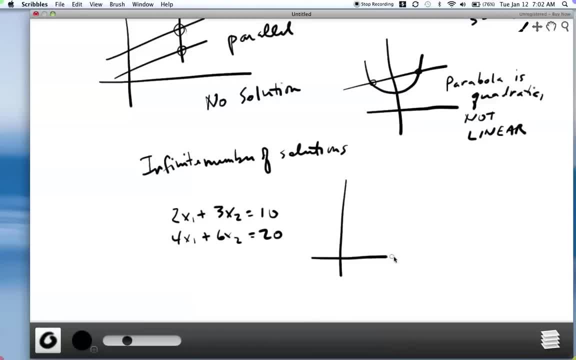 So when you draw it, if you were drawing the graph, whatever it might look like- you graph one of the lines and then you graph the other one and it sits right on top of the first one. So in that case, any point on the line would be a solution. 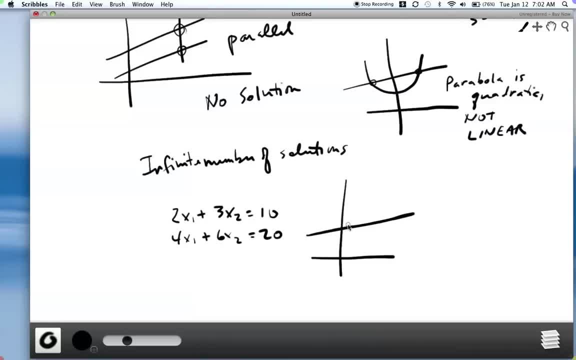 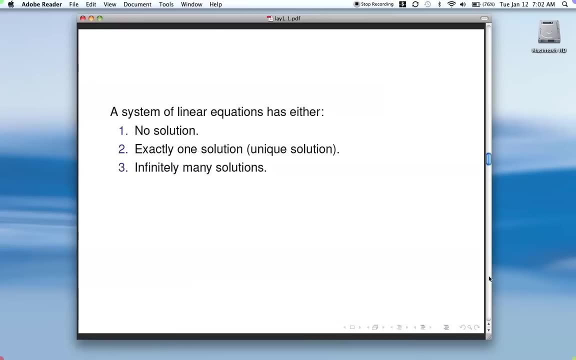 and so there would be an infinite number of solutions. Okay, so just to recap, let's go back to our slide, Let's go to the next one. So these are your possibilities. A system of equations has either no solution, exactly one solution, 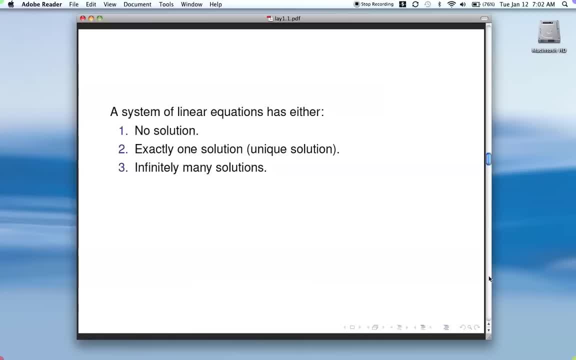 in which case we say it's a unique solution or it has an infinite number of solutions- And a little more terminology for you. We say: a system is consistent. Okay, consistent is a word we'll use a lot, So a system is consistent if it has at least one solution. 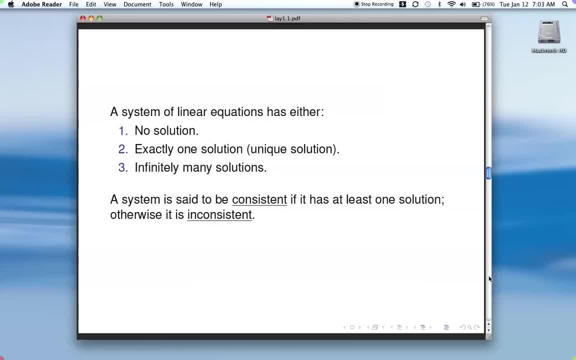 So that means either unique or an infinite number, but it has at least one solution: It's consistent. Otherwise we say it's inconsistent. So inconsistent means that it has no solution at all. Okay, so I think we'll stop there for this one. 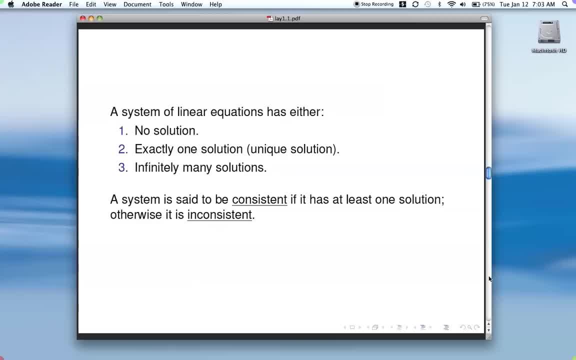 and we'll pick up with this on the next video. Okay, we're back now. We're talking about solving systems of equations And we need a systematic method because probably, as you can recall from your days in college algebra- once you get up to even a three-by-three system, 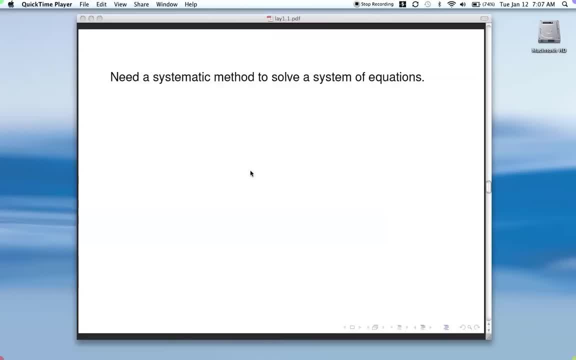 then things start to get a little messy, And so we're going to talk about now, about how- to a systematic method, Okay, a method that will work, no matter what size your system, no matter how many rows, how many columns or how many variables, how many equations. 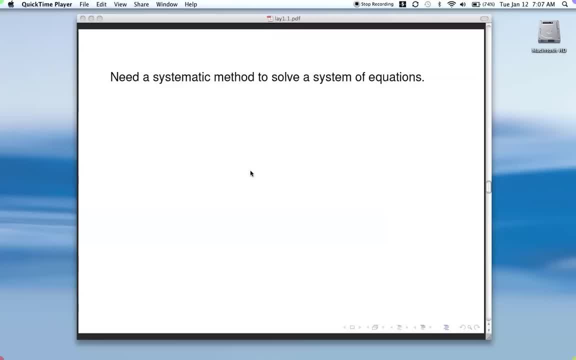 It's an algorithm that will work no matter what. Before we do that, I want to go back and look at that system that we were talking about earlier, which I have on my notepad here, So remember. I just want to refresh your memory. 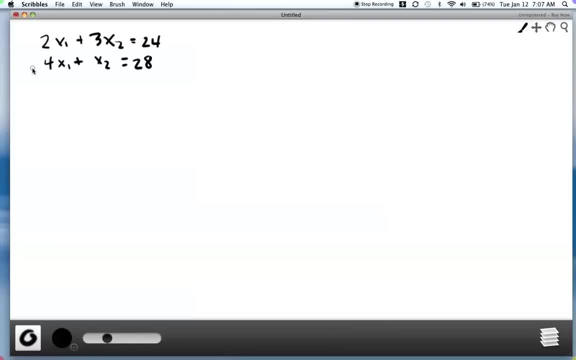 of what we did there. The second way we used to solve this system, if you recall, was we decided to multiply this equation by negative 2, and then we added that to the second equation. So let's just go through that quickly again. 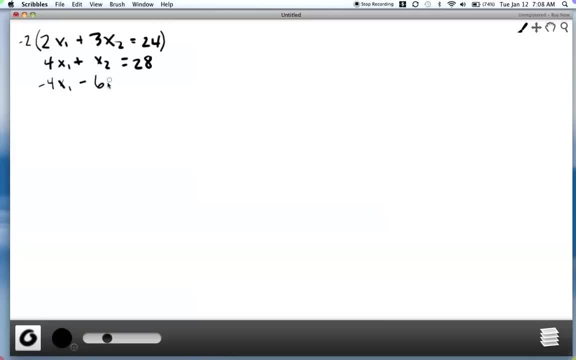 So we end up with negative: 4x1 minus 6x2 equals negative 48, right, And then we added that, So the x1's canceled out. Then we ended up with negative 5x2 here equals negative 20.. 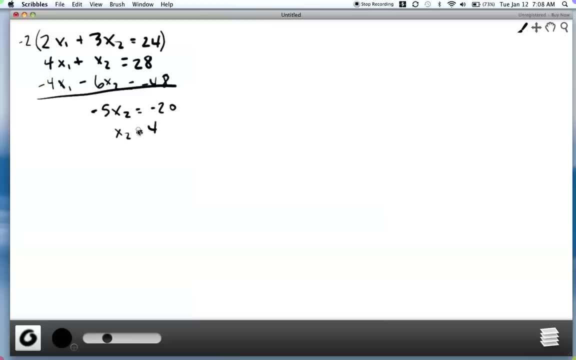 So x2 is equal to 4.. And then we didn't actually do it because we'd done it before, but I'll go through At this point. to find x1, you have to plug back in. You can plug into either one. 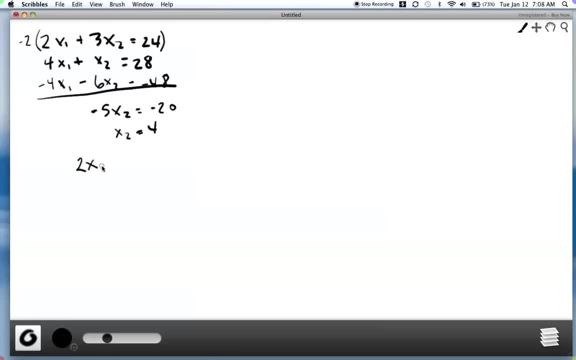 Let's just go back to the first one. First equation: we'll have 2x1 plus 3 times x2.. And we know that x2 is 4, so we plug that in Equals 24.. So we get 2x1 equals looks like 12.. 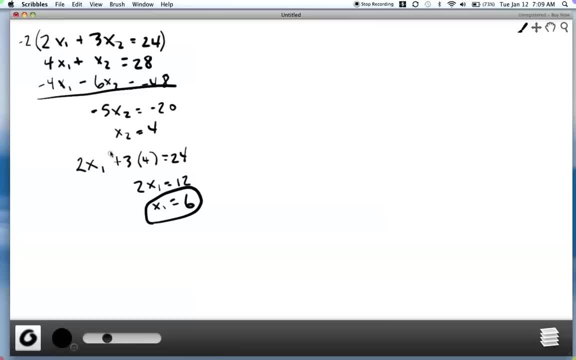 So x1 equals 6.. So there's our solution that we found in the previous video. To do this in a systematic way, we set up a matrix, And a matrix is just a rectangular array of numbers. So in this case, we would be interested in this matrix. 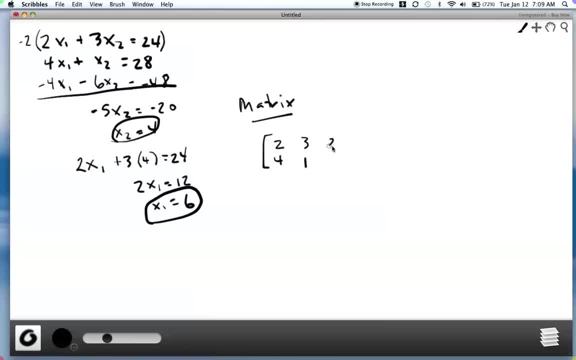 where I take the coefficients, And so I just write it like that. First row here represents the first equation. Second row represents the second equation. This matrix is called an augmented matrix, And it's called augmented because it has this right-hand side column included. 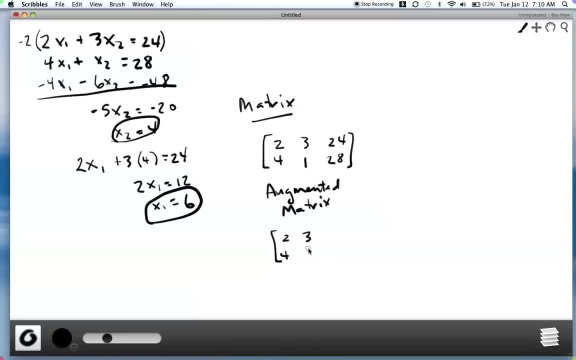 A lot of times we're only interested in this matrix, which we call the coefficient matrix, since it includes only the coefficients of the variables. So that's coefficient matrix. If we augment or add on the right-hand side, then we get the augmented matrix. 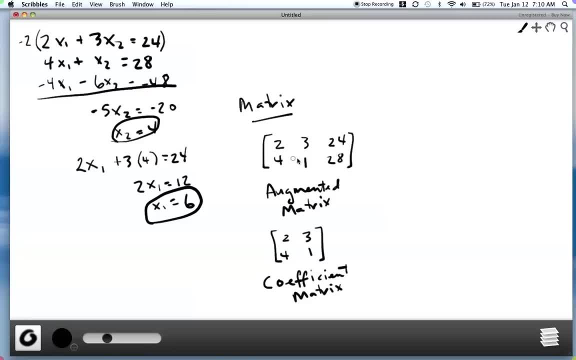 which is this one, And this is actually the one that we'll work on most of the time when we're solving. If we want to solve a particular system, we can work with the augmented matrix. Now, what do we do with the augmented matrix? 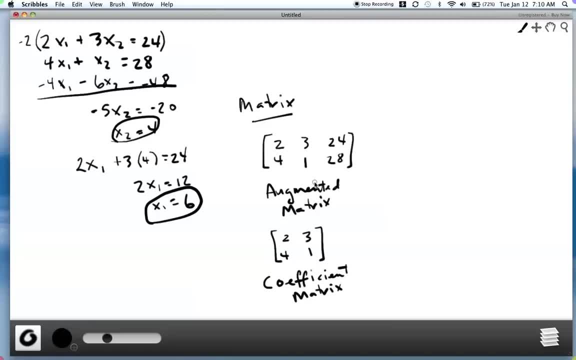 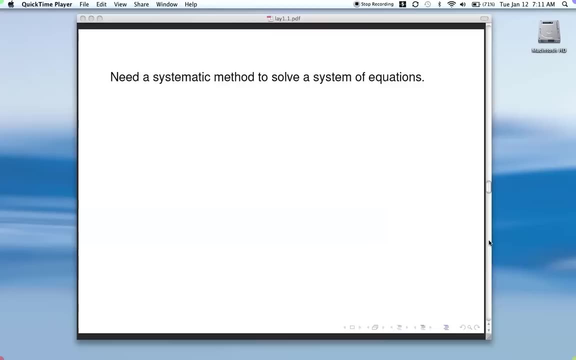 Well, it turns out that there are three row operations, three operations in our toolbox that we can perform on this matrix in order to solve the system. So to do that, let's go back to our slides here, And here we'll talk about our elementary row operations. 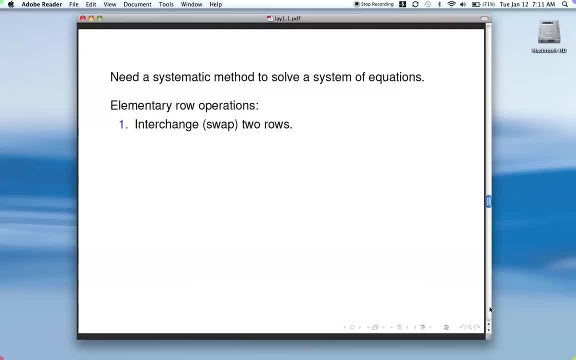 So number one is to interchange or swap two rows. So, since a row in a matrix represents an equation, that just means we're reordering the equations, which, as you know, has no effect on the solution. We could also multiply all the entries in a particular row. 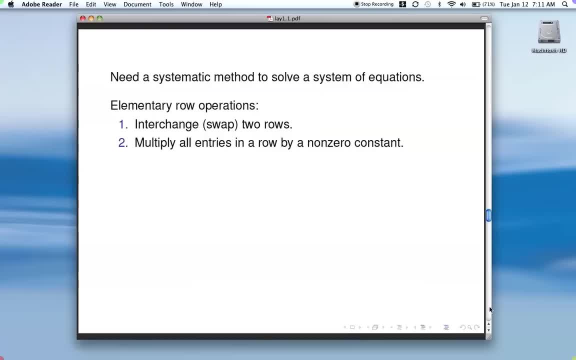 by a non-zero constant. Now, you can't multiply by zero because that would be essentially throwing out an equation and that wouldn't work. But you can multiply by any non-zero constant And the other is. sounds kind of complicated. 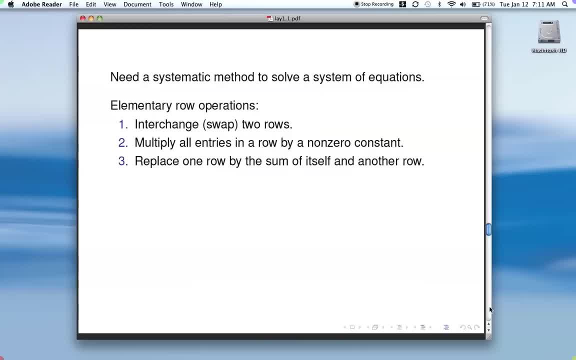 but it's really not. And really, this third one is the one that you'll do 99% of the time, okay, And it is the replacement operation. It's where you replace one row by the sum of itself, and that should be a multiple of another row. 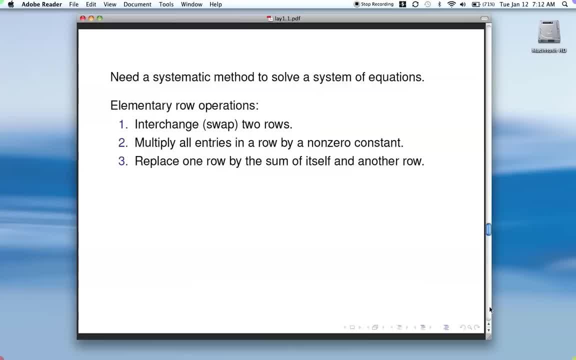 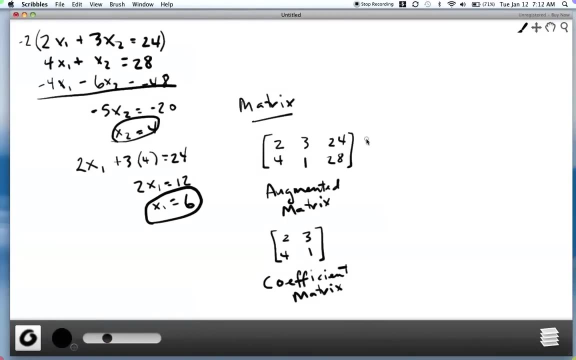 So you replace one row by the sum of itself and a multiple of another row. It's an error right there. So let's talk about how you do that. Let's go back to our example. okay, And that operation is actually what we did here. 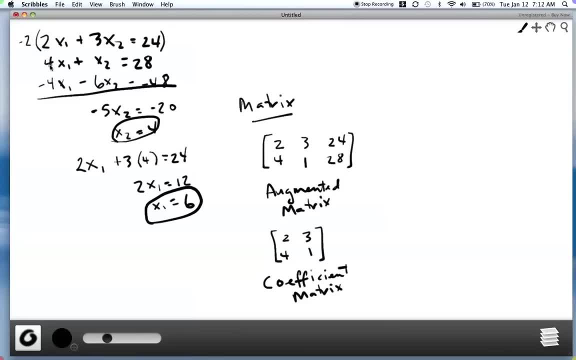 If you go back and look, we replaced- you can think of it as we were replacing- the second equation by the sum of itself and a multiple of the first row. okay, So we multiplied the first row, took a multiple of the first row. 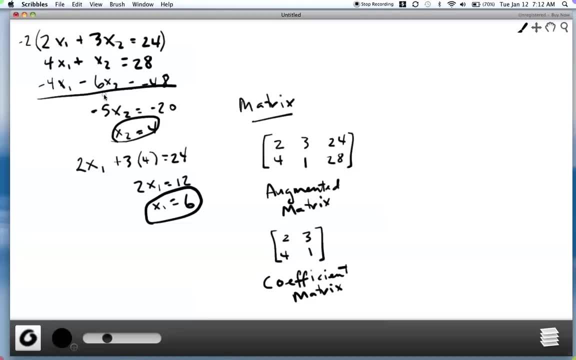 added it to the second, And so we ended up with this new equation right here, okay, So we're going to do the same thing, except in matrix form, okay, And I like to use a shorthand when I'm doing these operations. 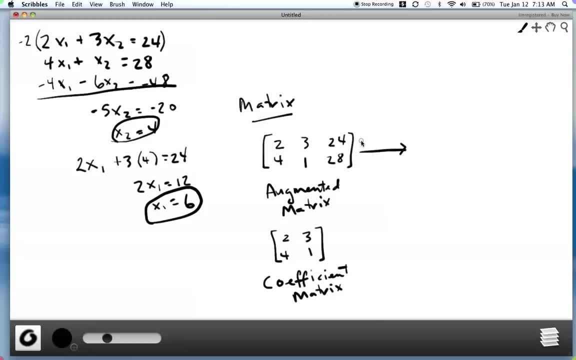 And so for the replacement operation, I write it like this: I'm going to multiply negative 2 times row 1 and add that to row 2.. Okay, so negative 2 times row 1, add it to row 2.. 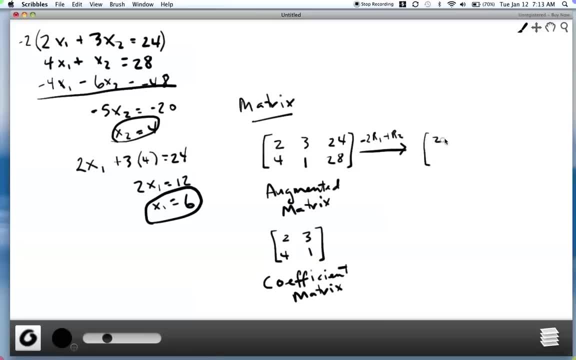 Now, this doesn't change row 1, so I'm just going to write that, just as I normally would. No change there, But row 2 is going to change, So I'm going to multiply each entry in row 1 by negative 2 and add it to the corresponding entry in row 2.. 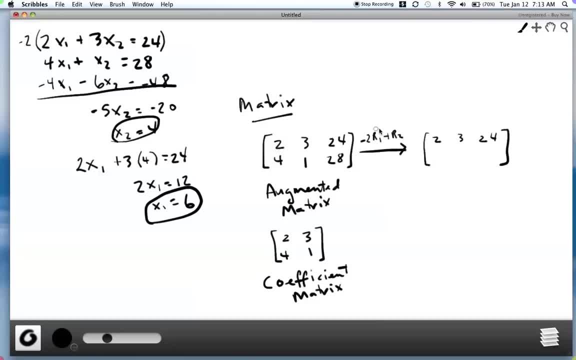 So I got negative 2 times 2, is negative 4 plus 4.. That gives me 0.. So I've eliminated x1 from this row. Then negative 2 times 3 is negative 6, plus 1 is negative 5.. 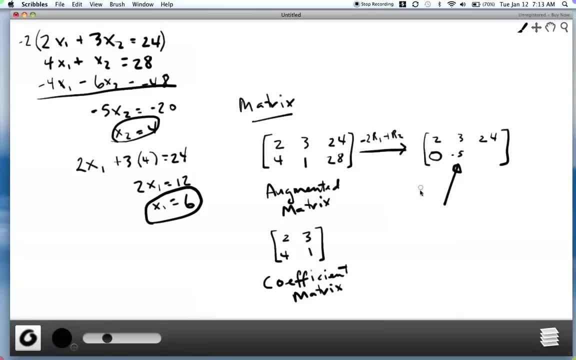 Okay, so just a reminder there. How did I get that? I multiplied negative 2 times 3 and added it to 1. So negative 2 times this entry plus 1.. Then I did the same thing in the third column. 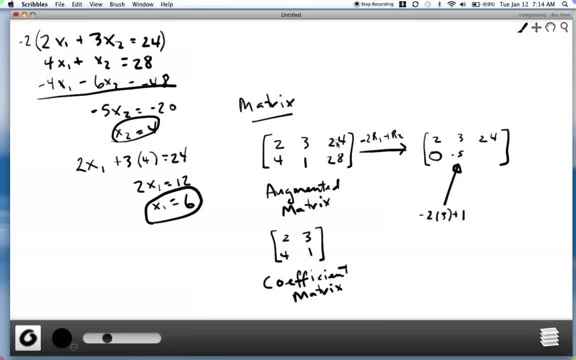 So I got negative 2 times negative. 24 is negative 48, plus 28 is negative 20.. So here I'll get negative 20.. And just to make that clear, that's negative 2 times 24 plus 28.. 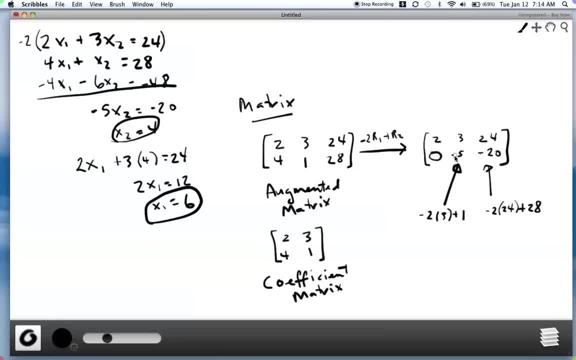 Okay, And so you can see if you wrote out the equation that corresponded to this row. it looks exactly like this equation here that we ended up with Right, And so at this point now I have in my second row only one variable, and so I can solve. 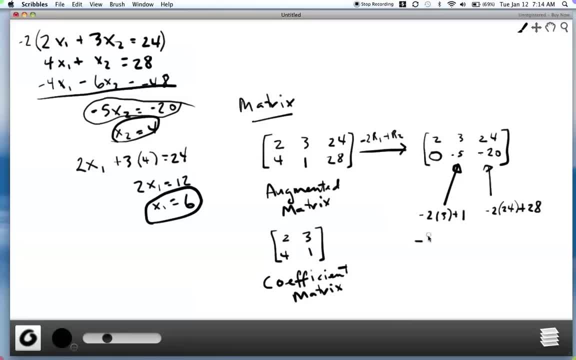 So I would say: okay, from row 2, I get negative. 5x2 equals negative 20.. So that means x2 equals 4.. Okay, just like I did before, And then we do something. Let me get a little more space here. 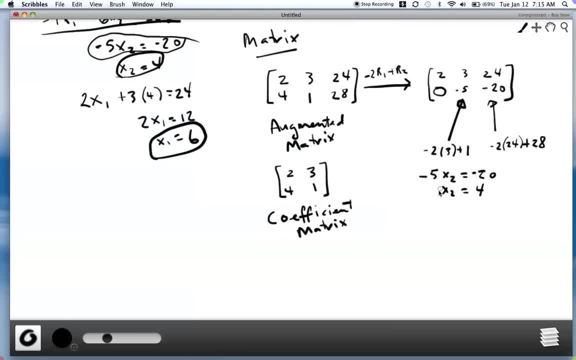 Then we do a process called back substitution. Okay, And that just means you back up to the next row and you substitute. So if we back up to the next row, then that would be backing up to the first row, And there I've got 2x1 plus 3x2.. 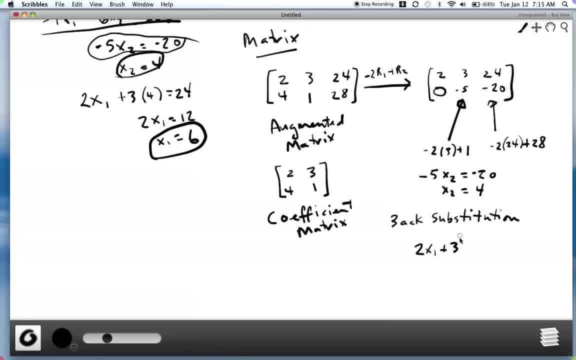 But now I know what x2 is: It's 4.. So that's the substitution part, Okay. So I plug that in Equals 24.. And we know that we end up with x1 equals 6 at this point, Okay. 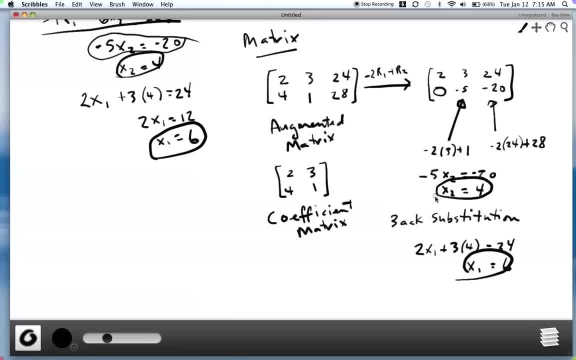 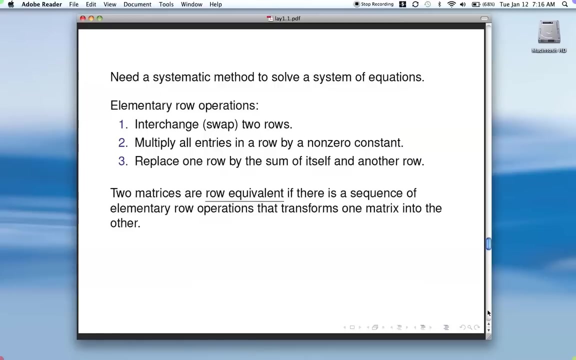 So here we've solved the system using elementary row operations and then using back substitution. Let's see Just one more note on why this is okay to do this. Let's go back to our slides. A little more terminology for you. We say two matrices are row equivalent. 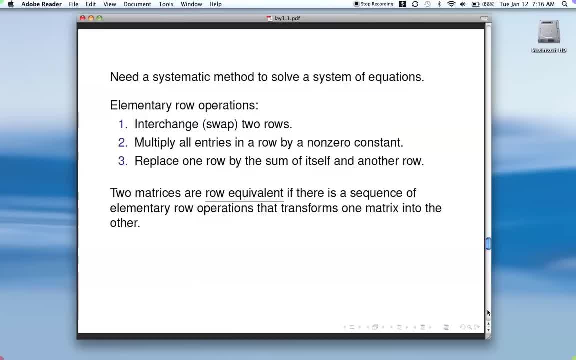 if there is a sequence of elementary row operations that transforms one matrix into the other. So the way I usually say that is they're row equivalent. if you can get from one to the other by doing elementary row operations, Okay Doesn't mean they're equal. 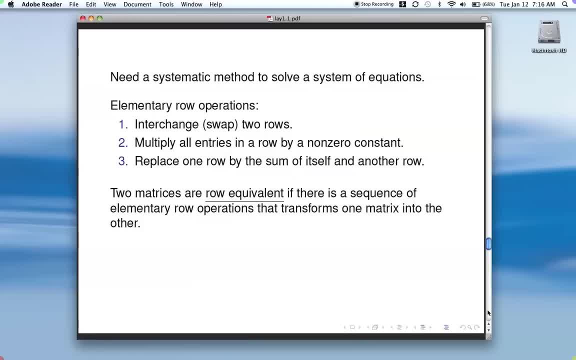 Row equivalent does not mean the matrices are equal. It just means that you can get from one to the other by doing elementary row operations, Okay, And then here's the clincher. That's why this works Okay. So remember, our goal is to solve a system. 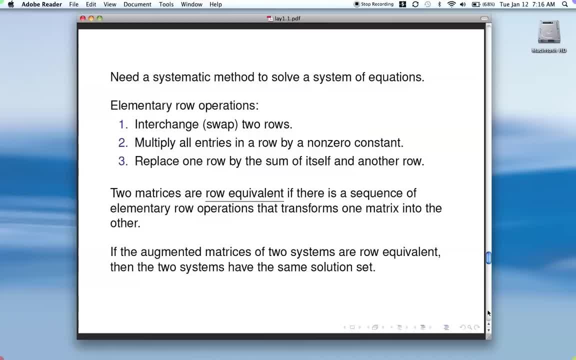 And so we need to know that when we do these row operations, we're not changing the solution or the solution set. Okay, And so this statement gives us that assurance. It says if the augmented matrices of two systems are row equivalent, then the two systems have the same solution set. 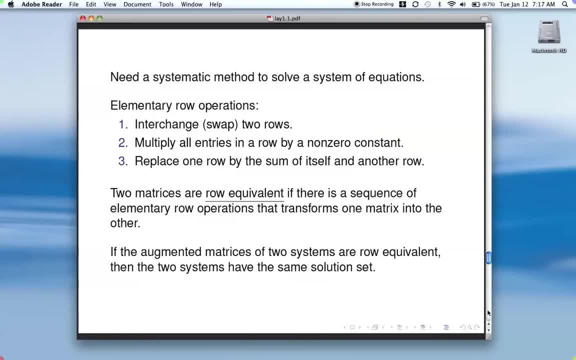 So that means we can start off with one matrix, We can do row operations and get to another one that we can solve easily and know that the solution that we get based on the last matrix will be the same for the first one. So that's why we can do these row operations. 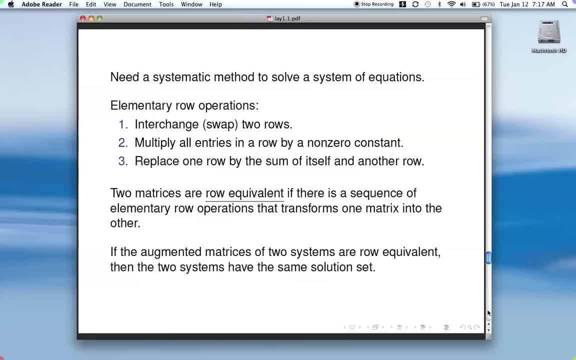 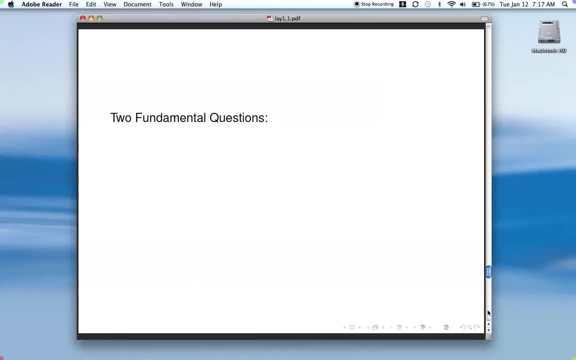 in order to solve a system of equations. This leads us to two questions. The first one is: is the system consistent? Does it have at least one solution? And if that's so, if it's consistent, then is that solution unique, or are there an infinite number of solutions? 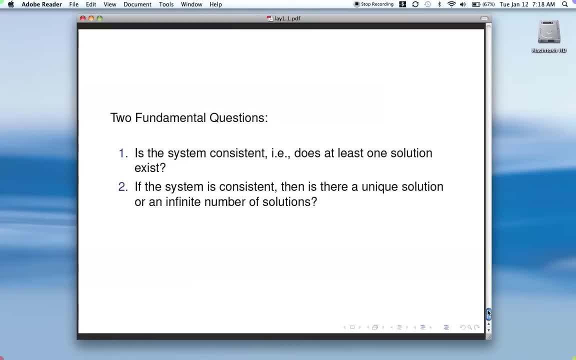 So we'll talk about how to determine. Number one: is the system consistent? Number two: if it is, then how do you know if there's a unique solution or an infinite number of solutions? Okay, we're going to stop here and I'll do one more video. 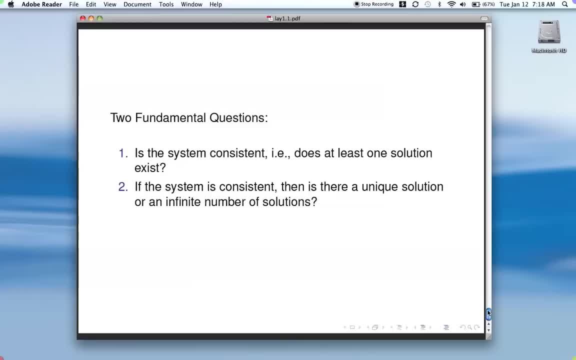 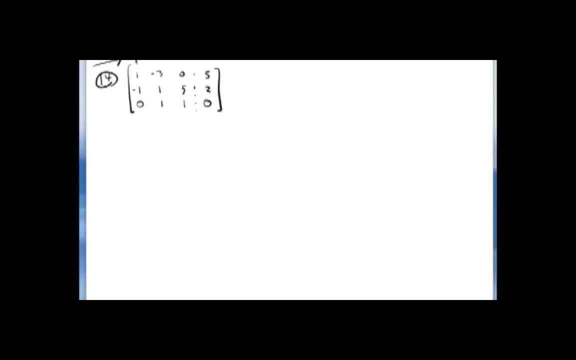 that has some problems worked out for you, So that'll be next. Okay, now I want to do a few sample problems from section 1.1 of the textbook. So first let's look at number 14.. So in the problem, 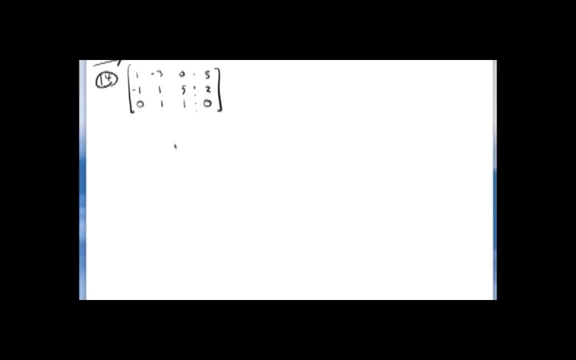 they're giving you a system of equations and asking you to solve it. So I've already got it here in the augmented matrix form, And so we just need to do elementary row operations in order to try to solve the system. So the first thing we want to do, 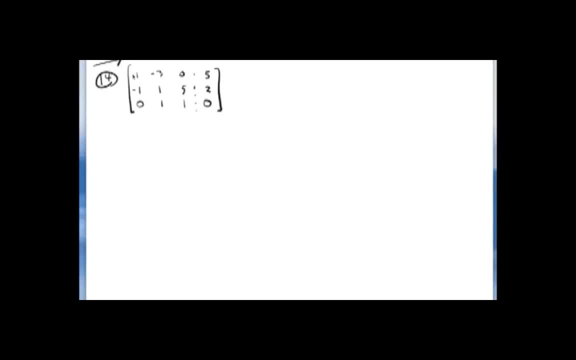 is: make sure that up here in the 1,1 position- that's the first row, first column- we've got a non-zero value, if possible. Well, it's already non-zero, so we don't need to do anything. 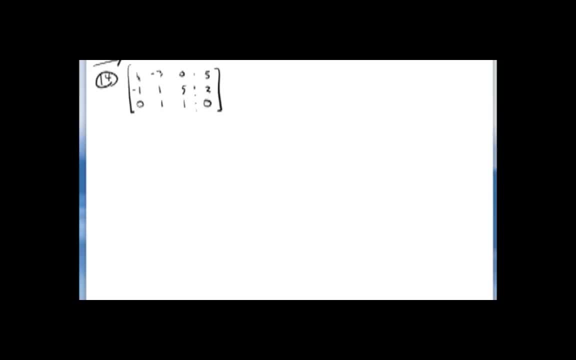 If this had been a zero, we would want to swap rows in order to get a non-zero value here. Okay, we already have one, so then we can next turn our attention to creating zeros in the column below this leading entry. Okay, a leading entry. 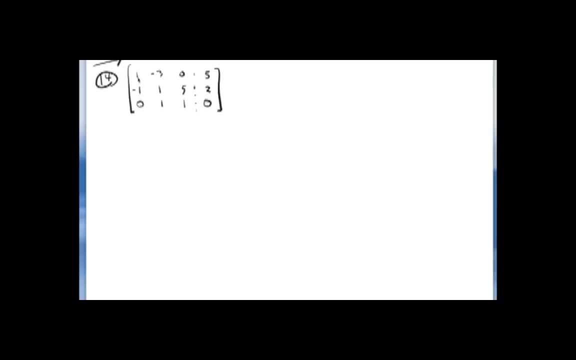 is the first non-zero value in a row, So we want to create zeros below it. So we need to create a zero in this position here. So we need to figure out what do we multiply by this one and add to negative one to get zero. 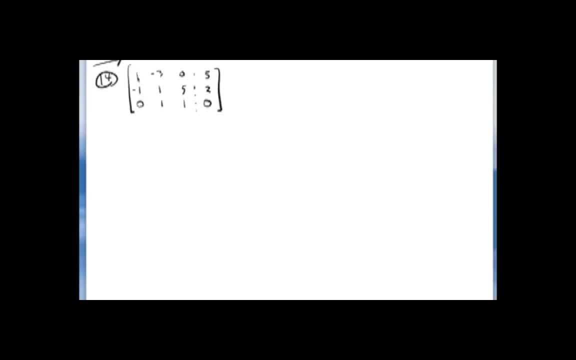 And clearly, to multiply by one or don't multiply by anything, we really just need to add the first row to the second, and that will give us a zero here. So I'm going to add row one to row two Now. that does not change row one. 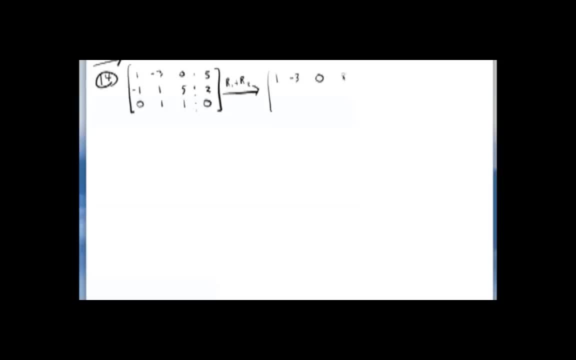 so I'm just going to repeat it here, And it doesn't change. row three: Okay, so now row two. we've got our zero there. Then we'll have negative. three plus one gives us negative two. Zero plus five is five. 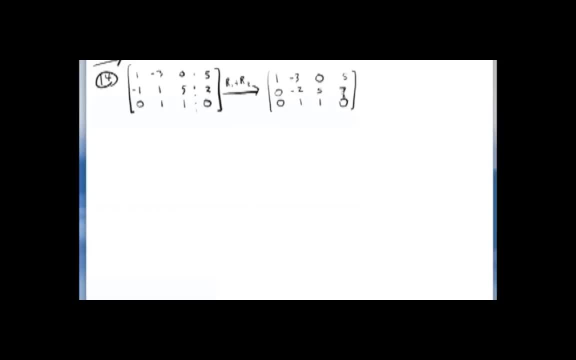 And five plus two gives us seven here. All right, So now we've got our leading entry, Zero's below it. We're done with that column, so we move on to the next column and down a row. So we want a non-zero element here. 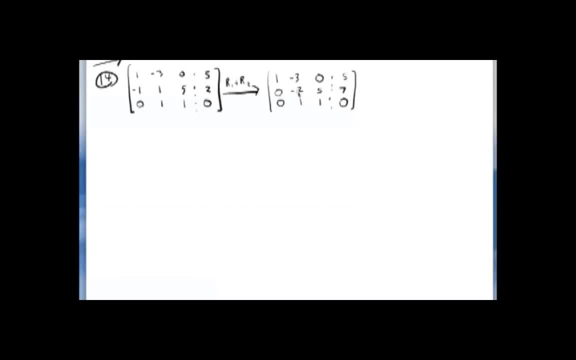 which we already have, And normally we would just want to zero out below it, But given that we have a one here, that's kind of a nicer number to work with. So I'm going to actually swap rows two and three at this point. 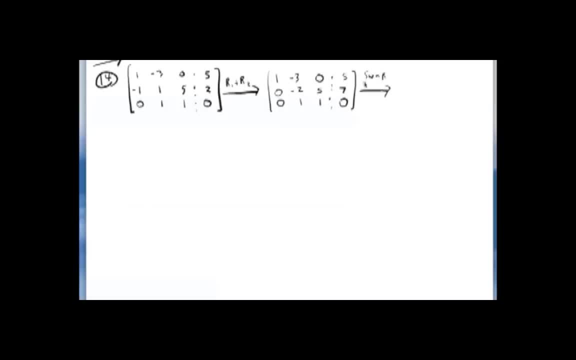 Swap row two and row three, And so row one doesn't change And row knee row two is the old row three And the knee row three is the old row two. All right, So I've got that, Now this. the reason I did that was because I 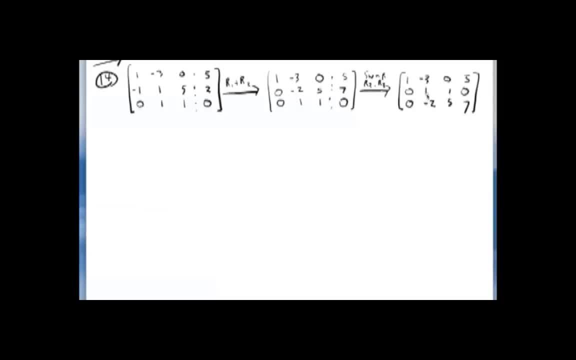 this just makes the arithmetic easier and I don't have to deal with fractions. Otherwise, if I left a negative two there, I'd have to figure out. you know what do I multiply by this to add to one to get zero. 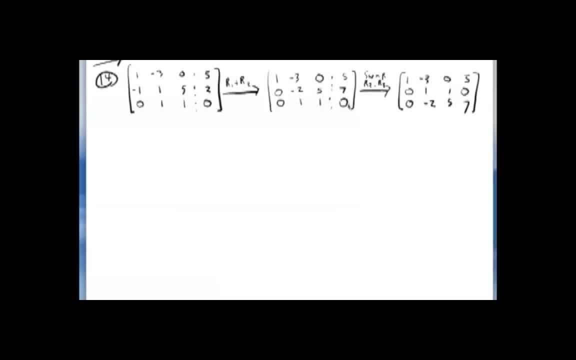 And I would have to carry that out through the rest of that row. So this is just easier arithmetic-wise. So now I've got a one here and I need to zero out underneath it, So I need to multiply by two and add a negative two to get a zero here. 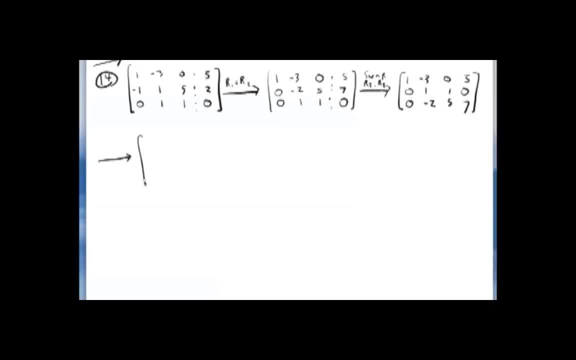 So my next operation is two times row two added to row three. Okay, so row one again doesn't change, Row two doesn't change And row three: just get my zero there and I'll get two over here. 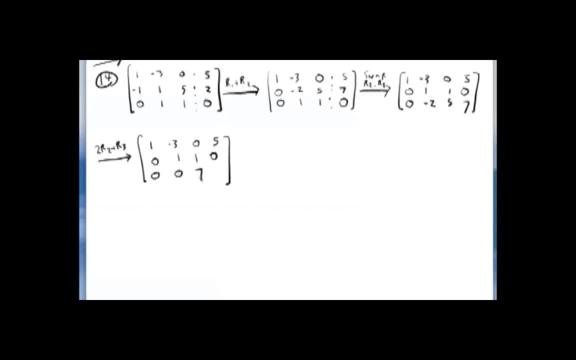 Two times one plus five is seven. Then I've got two times zero plus seven is seven. Okay, now at this point I'm done with the second column and I move over and I'm done with the matrix, because now in the third row, 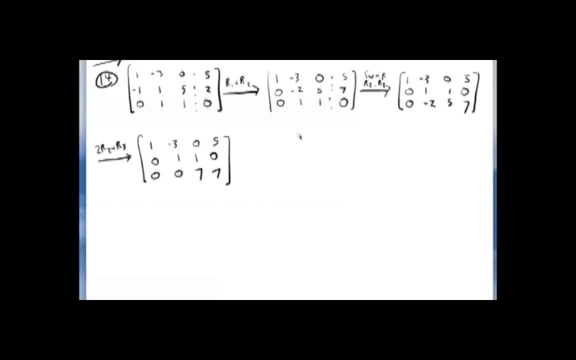 I've eliminated all the variables except for one, So from the third row I get seven. x three equals seven, So I can solve for x three. It's gonna be one. And then I do the back row, Back substitution. All right, so that means back up. 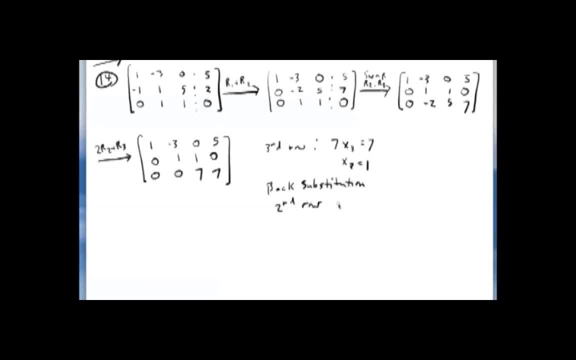 So I back up to the second row, which looks like, if I write down the equation corresponding to the second row, be x two plus x three equals zero. But I know what x three is, so I plug that in And I've got x two equals negative one. 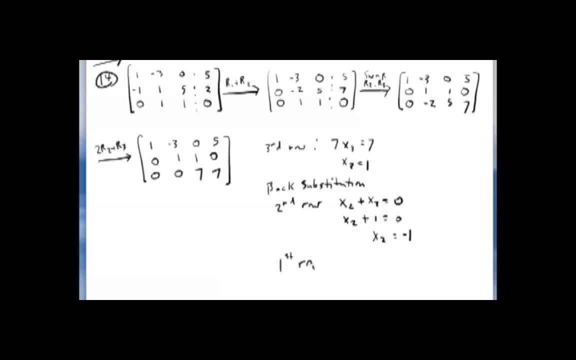 Okay, then I back up again to the first row, The first row. that equation looks like: x one minus three, x two equals five. I know what x two is. Plug that in So a little more room here, And so I get: x one is equal to. 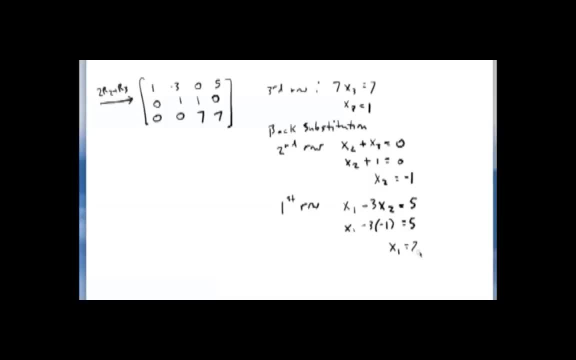 let's see that's a plus three Minus three, so it would be two. So x one equals two, x two equals negative, one x three equals one. There's a solution to my system, Okay, so this system here. 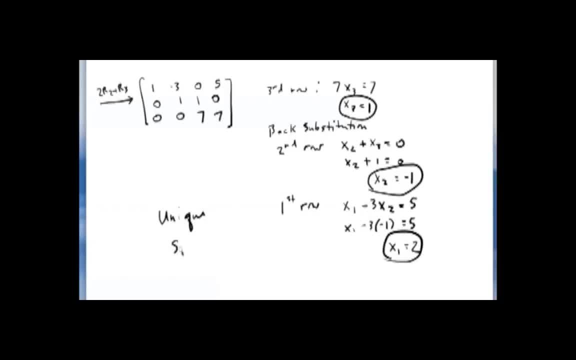 had a unique solution, Just one. All right, let's go on and look at another homework problem. I want to go to number 12.. Okay, so still in section 1.1., Problem number 12. Actually, before we do that, 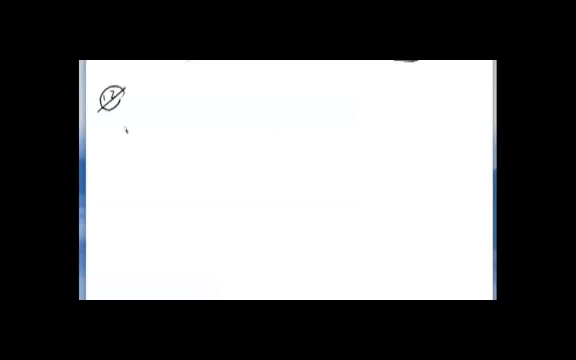 let's look at one thing. Before we do that, let's look at one other thing. Suppose I have a system that looks like this: Two x one plus three x two equals ten. And how about four x one plus six x two equals twelve. 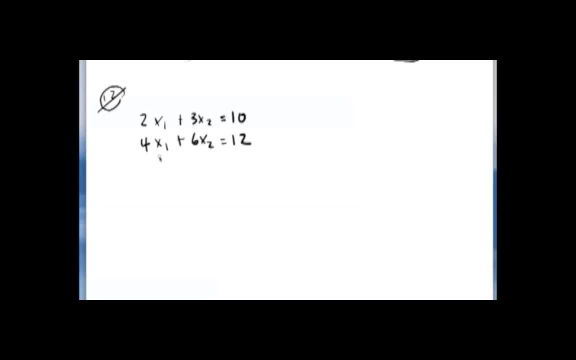 Now, if you examine that a little bit, you're going to see that to get this second equation I just multiply the first one by two, right? So two times two is four, Two times three is six. But then I didn't multiply this by two. 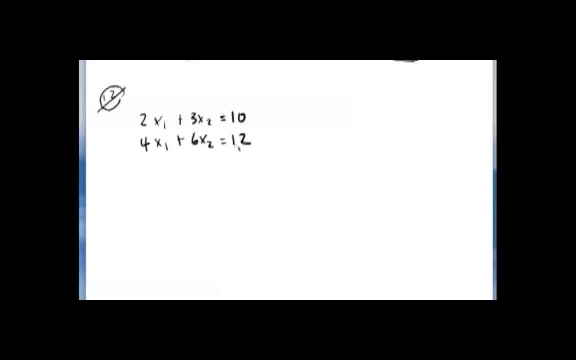 Actually I did, and then I didn't want to get that same value, So I changed it. So just based on that analysis, it seems that this system should have no solution right. And if you were solving it using elimination, say, 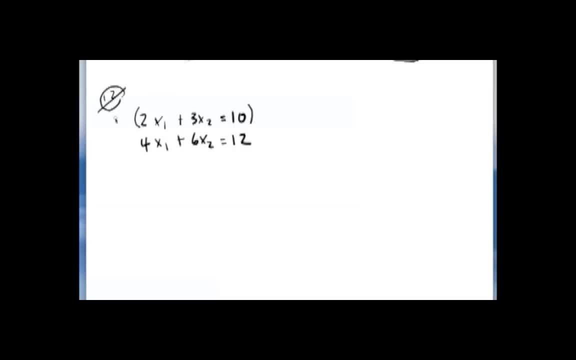 right. maybe you'd multiply. Maybe you didn't notice that it's not going to have a solution, So you're just merely going along your way solving it. So if we multiply through by negative two, we're going to get negative four x one. 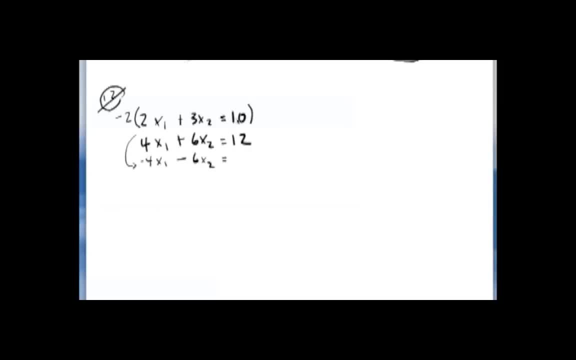 minus six x two equals negative two times ten is negative twenty. Then we'd get add that and here we get zero, Here we get zero. So on the left we've got zero, And on the right what do we have? 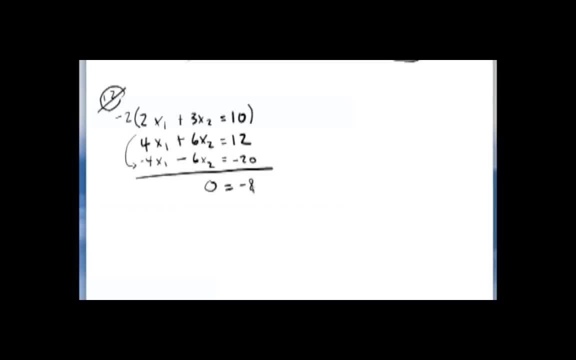 Negative eight. Well, zero can't equal negative eight, right. So this is what tells us that this system has no solution. Okay, we get to this point where we have zero on the left and something not zero on the right. Okay, we've got a non-zero value. 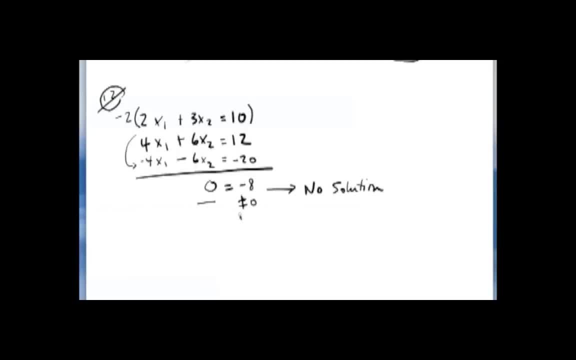 over here on the right. Okay, so if we had thrown that into a matrix it would look like this: All right, so we do one row operation, same one we did up there, negative two: row one plus row two. All right, so row one doesn't change. 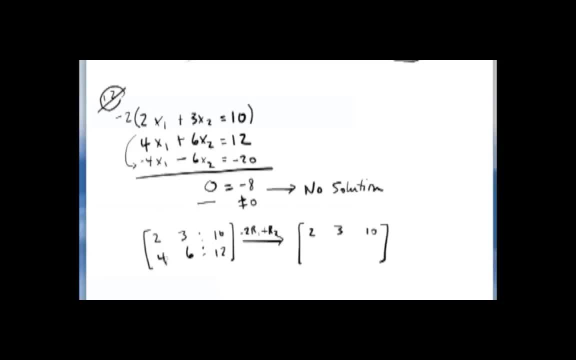 And row two, we get negative. two times two is negative. four plus four gives us zero Negative. two times three is negative. six plus six gives me zero Negative. two times ten is negative. twenty plus twelve is negative eight, All right. so if you look at this, 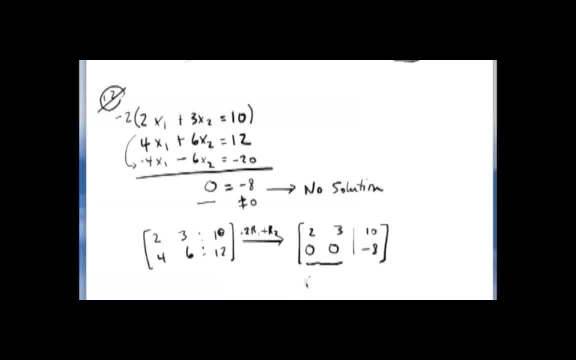 we have the same thing, right, We've got all zeros, And over here on the right, we've got something that's not zero. Okay, this is the marker that you look for to indicate no solution. Okay, all zeros on the left. 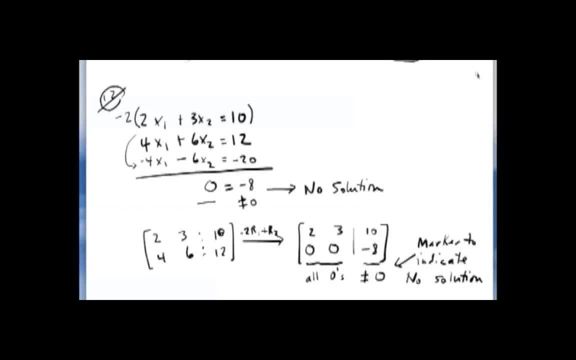 something not zero on the right. Okay, so keep that in mind. We're going to be using that all semester. Okay, so now let's go to number twelve. Okay, still in section 1.1.. So number twelve: one negative three: four negative four. 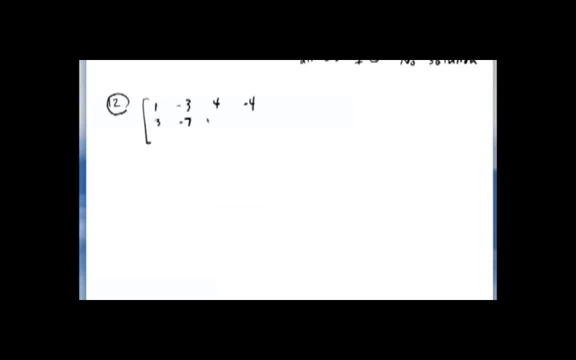 Three negative, seven, seven Negative, eight Negative four, six negative, one And seven. Okay, and this is an augmented matrix. So we start, We do our row operations, So we look We've got a non-zero value here. 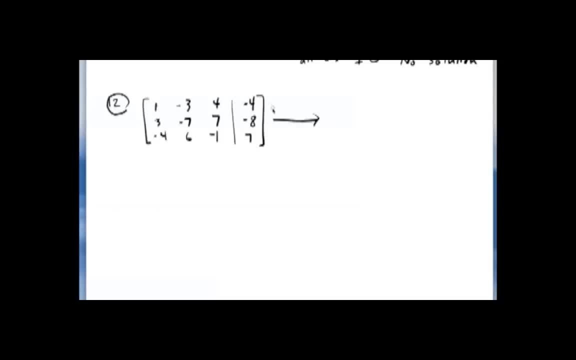 So we want to zero out underneath. So the first thing I'm going to do is negative three, Negative three times row one plus row two, So that I can generate a zero there. So I've got one negative three, four negative four. 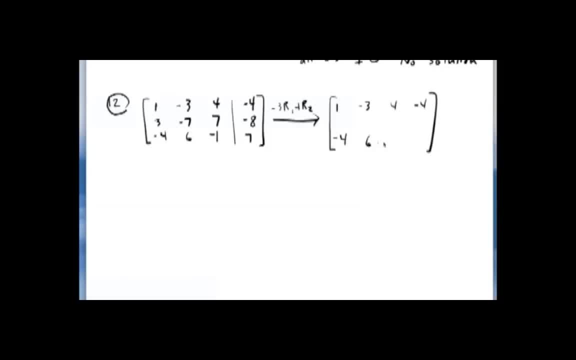 Alright, first row and the third row don't change. And this one, I'm going to get my zero there. And what do I got Negative three times. negative three is nine Minus seven gives me two there. Negative three times four is negative twelve. 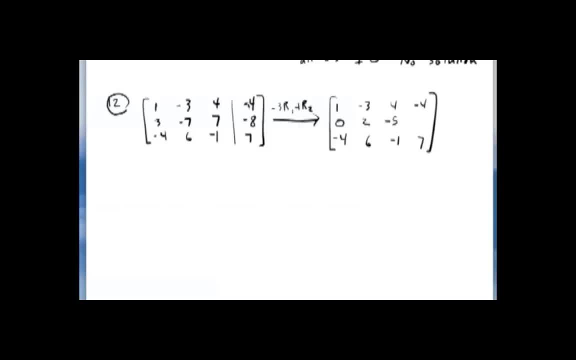 Plus seven is negative. five Negative three times negative four is twelve Minus eight is four. Okay, so I've got my zero there. I need to keep working down, Get a zero in this position. So the next operation I'm going to do: 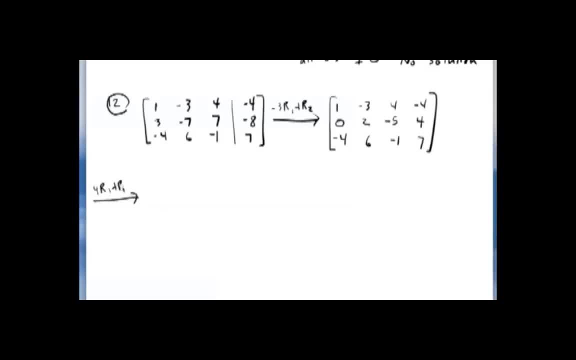 will be four times row one plus row three. So again, row one doesn't change, Row two doesn't change And row three: I get my zero there. So I'm at four Minus four gives me zero. Four times negative. three is negative twelve. 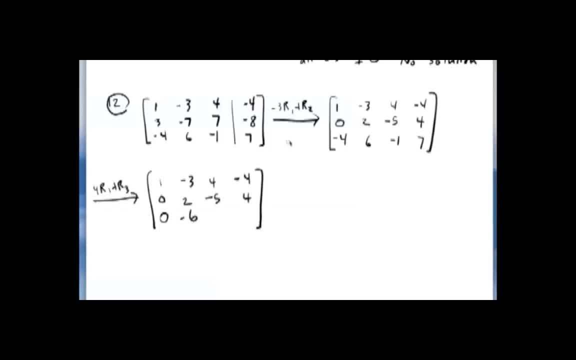 Plus six is negative. six Four times four is sixteen. Minus one is fifteen. Four times negative four is negative. sixteen Plus seven is negative nine. Alright, so that first column is looking good. Then I move over to the second column. 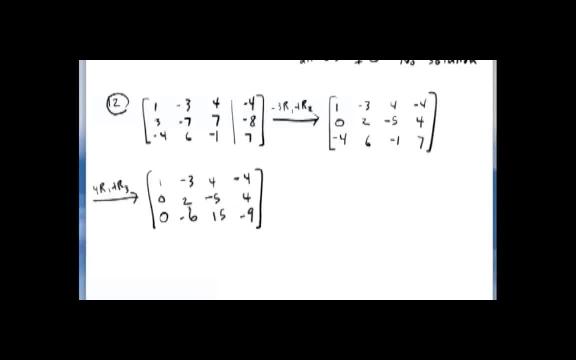 second row. I've got a non-zero value here, So I want to zero out underneath, So I need to work on that six there. Okay, so I'm going to multiply row two by three And add that to row three, Because three times two is six. 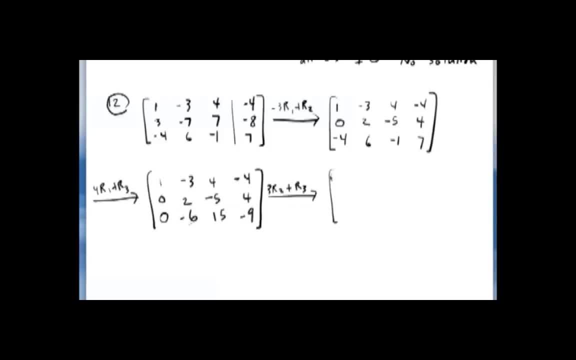 Minus six gives me the zero that I need right here. So one negative three, four negative four, Row two doesn't change, And row three: I get my zero. It's already zero. So three times zero plus zero is zero. 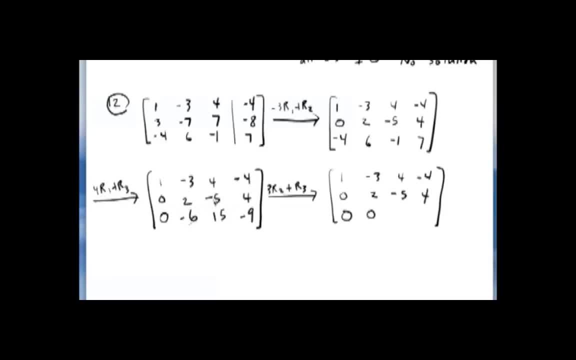 Three times two is six Minus six. There's my new zero. Three times negative. five is negative. fifteen Plus fifteen is zero. Okay, and remember, we're looking At this point. you can see we've got all zeros here, Okay, and then we're ready to get the last position. 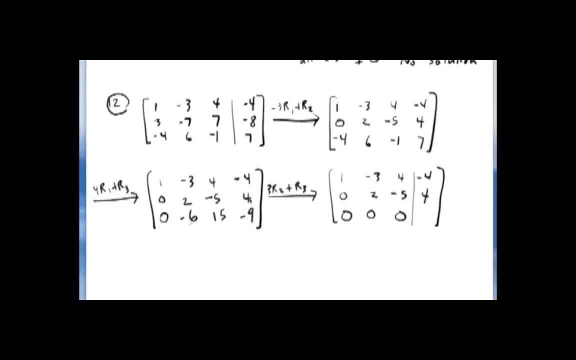 And what do we have here? Three times four is twelve Minus nine gives us three. So what do we have here? We've got all zeros on the left And on the right. we've got a value that's not zero. 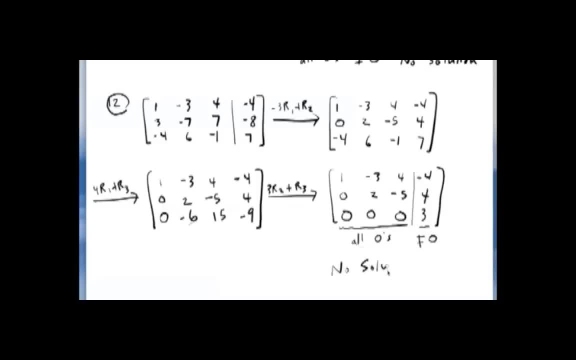 So, as we saw before, that means this system has no solution. Okay, Alright, I want to do one more problem from this section, And this one islet's see, Actually, maybe a couple more Aboutlet's look at number. 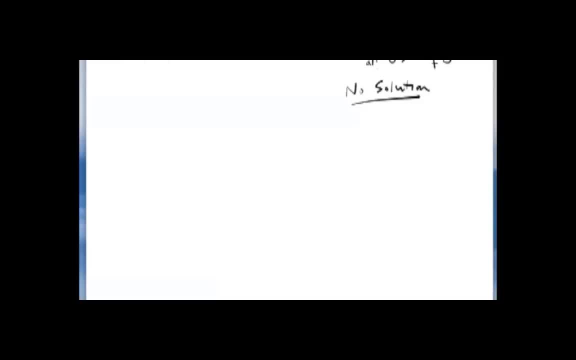 Let's see number twenty-two. Okay, twenty-two, Twenty-two looks like this. Okay, we'll put it in the matrix form. Okay, now the directions ask you to find the values of h. Okay, this parameter For which this system is consistent. 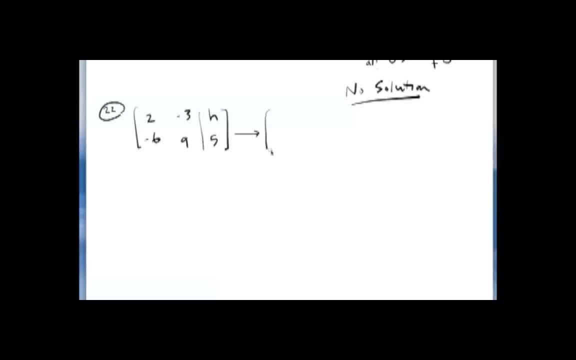 Okay, so to do that, you want to just get an echelon form. Actually, we don't know what echelon form is yet. Let's just do what we've been doing. So we've got our non-zero value here. 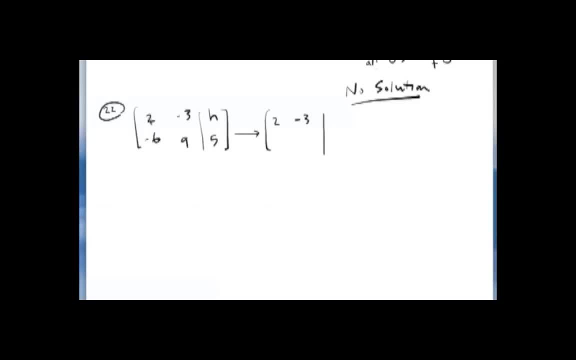 We zero out underneath it. So multiply by three. So I'm going to do three times row one plus row two. So that gives me a zero there. Oops, this doesn't change. Okay, so three times two is six Minus six gives me zero here. 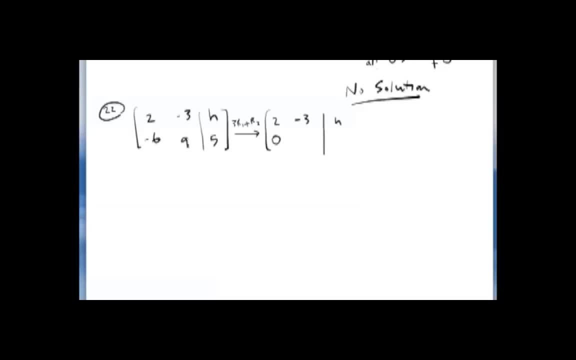 Three times negative. three is negative, nine plus nine Gives me zero here, And three times h plus five is just three times h plus five. Alright, now, at this point, look, It looks just like the one previous right, Like back at the one we were just looking at. 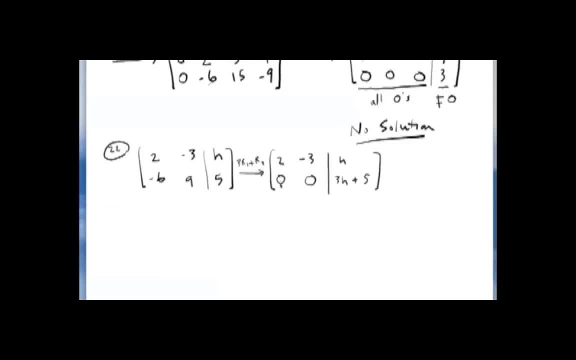 We had all zeros and then something not zero. Well, here we have all zeros, Okay, so that's significant. But over here we don't know what this is, because we're asked to find h so that this system is consistent. So we want this to, we want three h plus five. 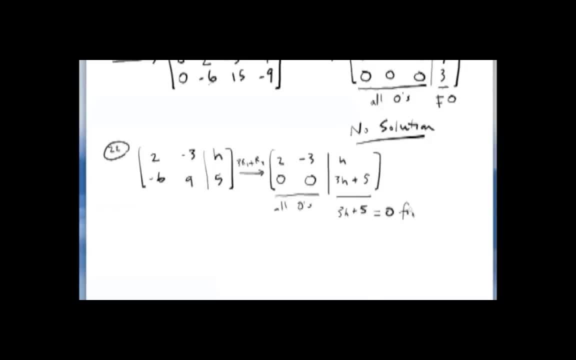 Plus five must equal zero for the system to be consistent. Okay, so that means that three h must equal negative five, So h has to equal negative five thirds. Okay, so that's what we're looking for for this one. Alright, because this has to equal zero for the system to be consistent. 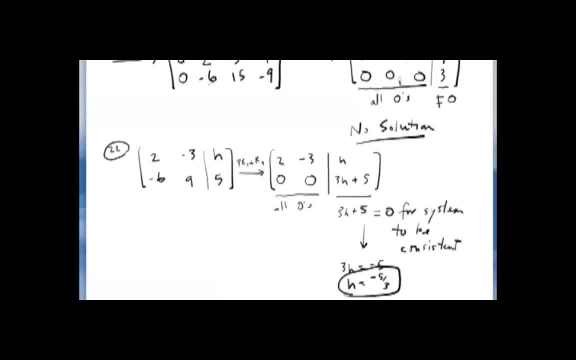 Because if this is not zero, we're like this case up here where there's no solution. Alright, let's look at one more, And I'm kind of going out of order here, just because I like to kind of stick with the same theme. 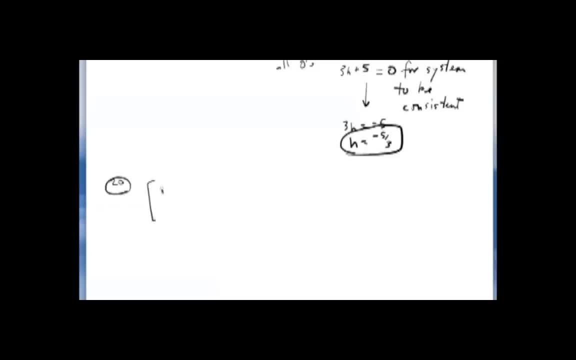 So I'm going to back up to number 20. And it's a similar kind of question as 22. But this time the h is not on the right side, It's part of the coefficient matrix, So it's a little bit different. 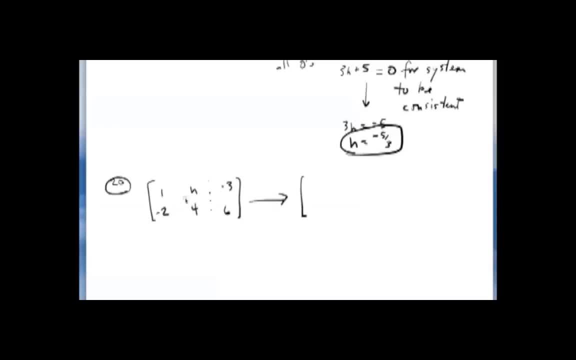 So again, we do our row operations. We got a non-zero here. We want to zero out this position, So we do two times row one plus row two. So I've got one h negative three And I got a zero here. 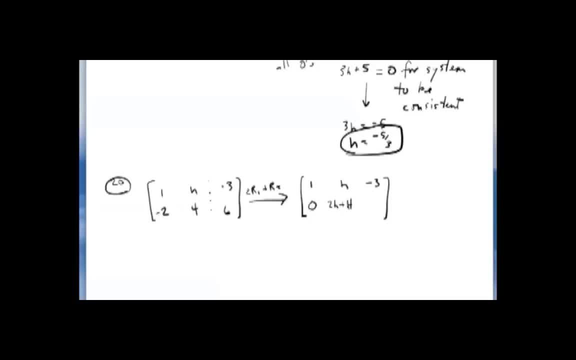 Two times h plus four And two times negative three is negative. six Plus six is zero. Alright, so I've got this situation. Now, remember, the problem is to find h such that the system is consistent. Well, system is consistent, as long as we don't have a case like we had up here. 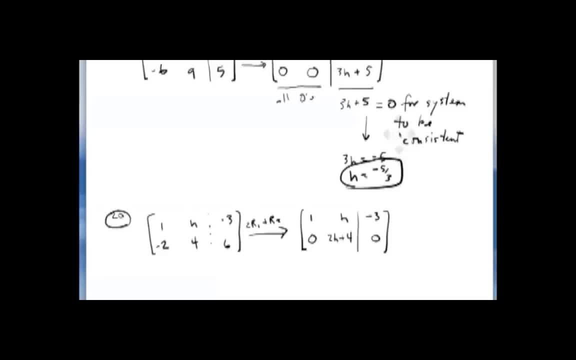 Alright, system is consistent as long as we don't have a row that looks like zero, Zero and then something not zero. Okay, Well, notice that that can never happen. We can never have zero, zero, something not zero, Because the right hand side is already zero. 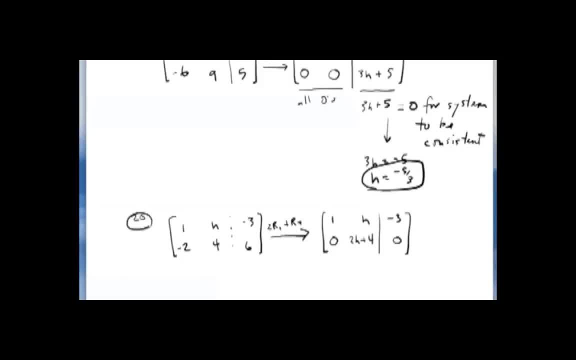 Okay, So that means this system. Let's have a little more room here. This system is always, Always consistent, Alright, Because we can never have a row of the form zero, zero, And then, on the augmented side, something not zero. 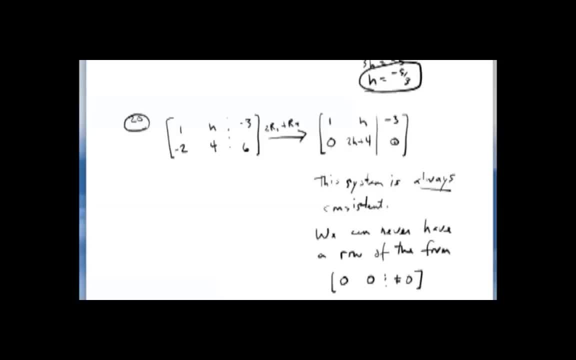 Alright, Can't happen in this case, Because the right hand side is a zero. Okay, So this system is always consistent. Yeah, Irregardless of what h is Alright. So I think that's about it for section 1.1.. 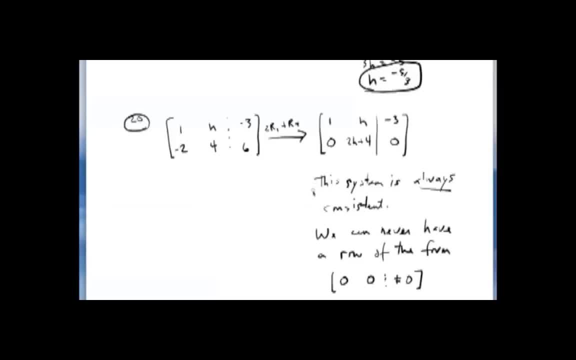 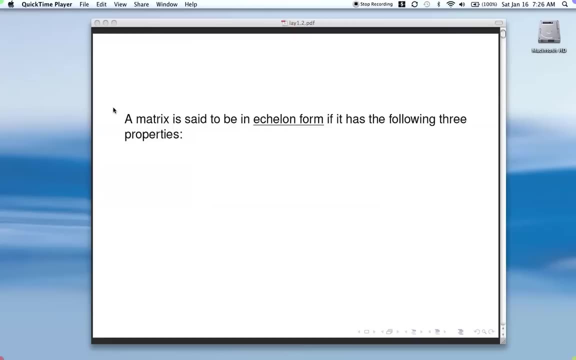 As always, keep in mind that you can call me up, email me any time to let me know if you have any questions. Alright, Good luck with those homework problems. Okay, Today we're going to be talking about section 1.2.. 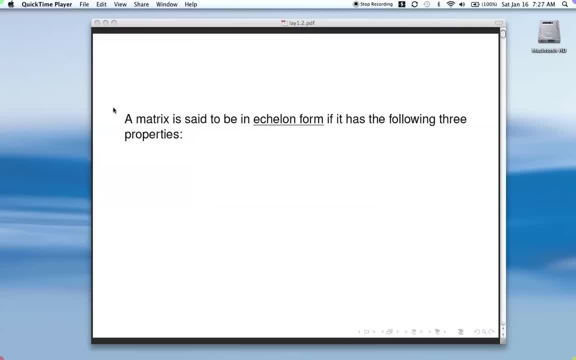 And really the main thing I want to cover today is to talk about a specific form that we want to get a matrix into when we're trying to solve a system. So we've kind of talked about that a little bit up to now, But at this point we're going to get very specific about that. 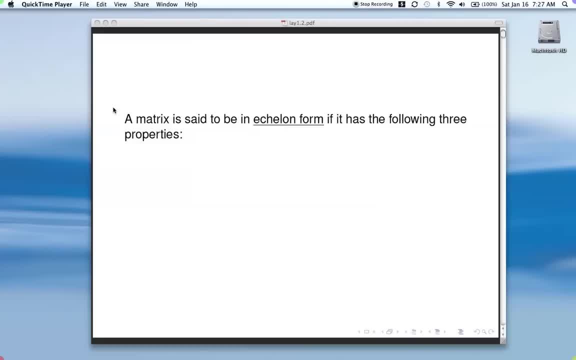 So the form that we're trying to get at is called echelon form. Okay, And echelon form is defined by three properties. So the first one of these is that if there are any rows of all zeros, they're at the bottom of the matrix. 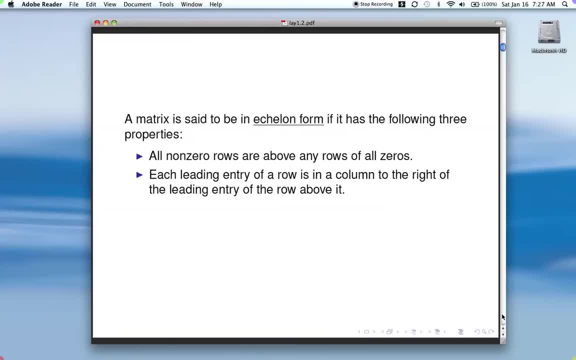 So you swap rows to get those at the bottom, The leading entry. Remember that's the first non-zero entry. So leading entry, The leading entry in each row is in a column to the right of the leading entry in the row above it. 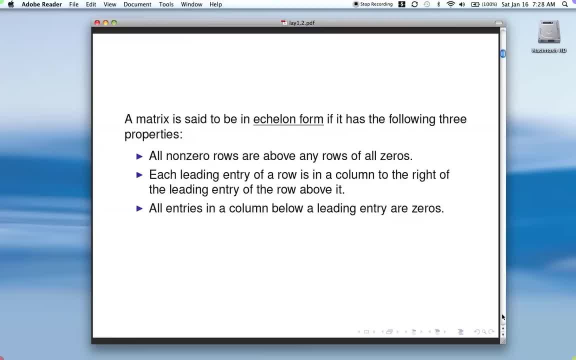 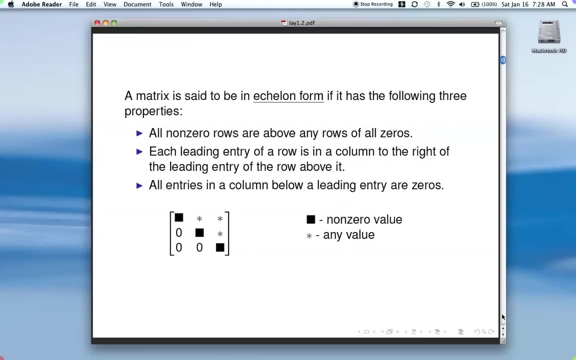 And I'll show you that in just a sec. The third one is that all entries in a column below a leading entry are zeros. So we've done that up to now: We get our leading entry and then we zero out below it. So that's that idea. 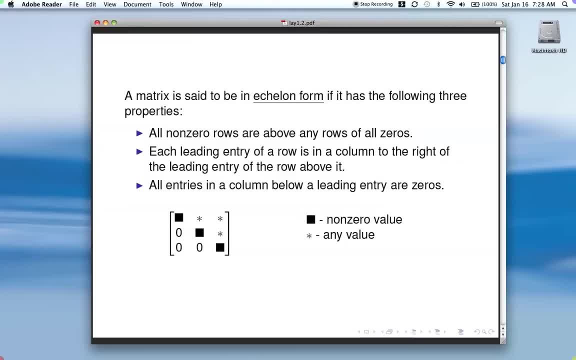 Here's an example: The black squares here represent non-zero entries, Zero values, And they're the leading entries in each of these rows. And so you can see, here we have a leading entry and zeros underneath. Here we have another leading entry, zeros underneath. 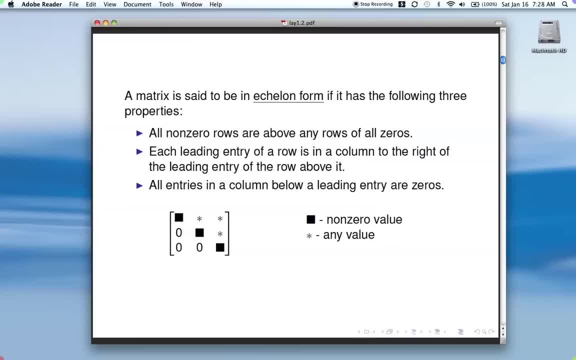 And notice that this leading entry is to the right of the one before it. And here's another leading entry and it's to the right of the one that came before it. Okay, So that second property is basically what gets you this stair step kind of structure. 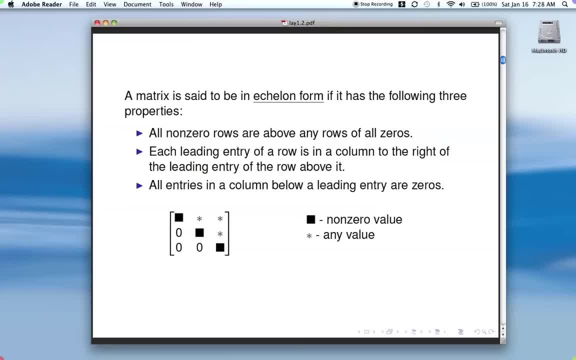 in your matrix. All right, Let's see. Here's another one. This one's also in echelon form. Leading entry here: zeros below it. Another leading entry: zeros below it, And it's to the right of the previous one. 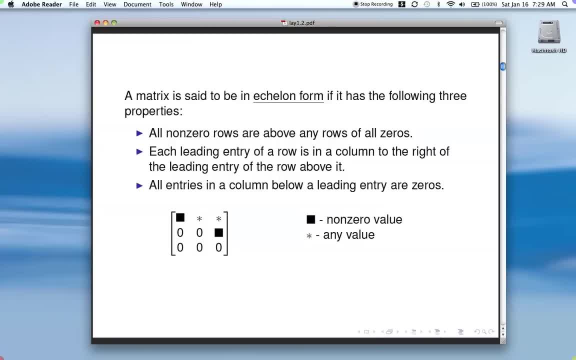 And we have a row of zeros and it's at the bottom, So we satisfy all the criteria. Now, sometimes you want to go a little bit farther and get your matrix in reduced order. Okay, So you want to get your matrix in reduced echelon form. 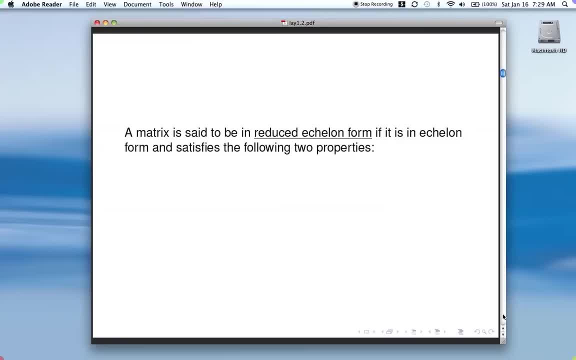 So if it's in reduced echelon form, that means it's in echelon form plus. it satisfies two more properties, Okay, And these properties are that each leading entry is a one, So you scale the rows to make each leading entry equal to one. 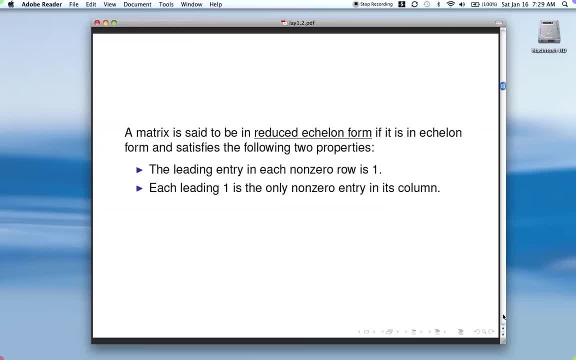 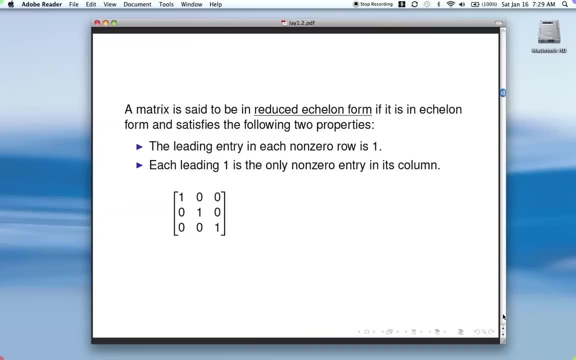 And that one is the only non-zero entry in its column. So you zero out not only below it, but also above it. So here's an example of a matrix that's in reduced echelon form: Each leading entry is a one And it's the only non-zero entry in its column. 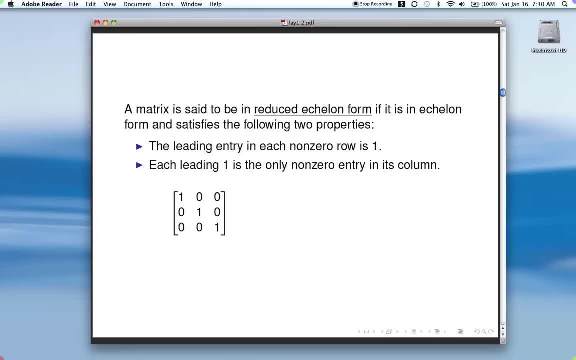 So we zeroed out below here, Zeroed out above and below And zeroed out above in this case. All right, Here's another one. This one's in reduced echelon form, Because each leading entry we've only got two. 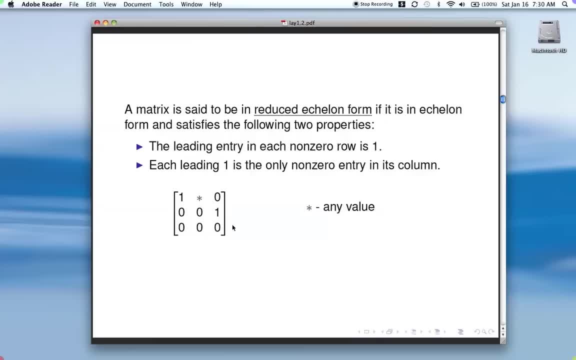 And they're each one, And we've zeroed out above and below each one. The row zero is at the bottom. Okay, So that's in reduced echelon form. Now, for purposes of just solving a system. typically, you just want to get it in echelon form. 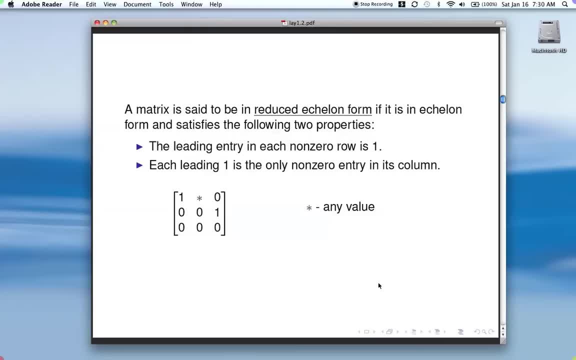 Although there will be one particular case that I'll talk about later in another section coming up where you want to get it in reduced echelon form. Reduced echelon form just makes life easier then, But for the most part, at this point, echelon form is fine. 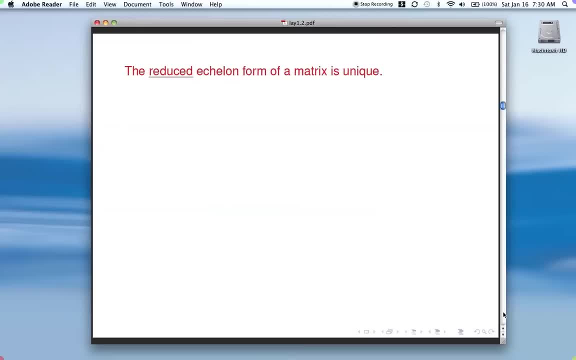 Now I'll show you a couple of things about these forms. One thing to note is that the reduced echelon form of a matrix is unique, So that means that no matter what sequence of row operations you use to get a matrix in reduced echelon form, 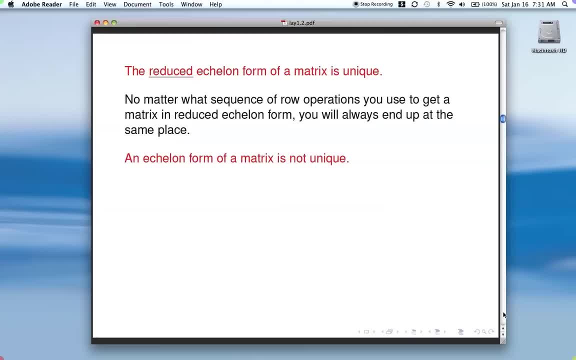 you'll end up at the same place. Not so for the echelon form. It's not unique. It means that all of you could be working on the same matrix and end up with a different echelon form of the same matrix, And that's because you can scale a row, multiply a row by a constant and get a different echelon form. 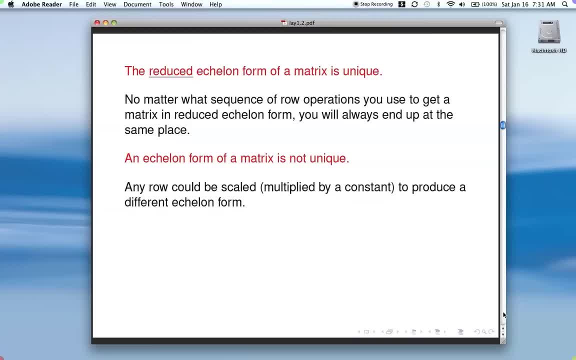 It would still be an echelon form, but it would be a different matrix. So the reduced form is unique. The echelon form is not Okay. So you either want to get your matrix in echelon or reduced echelon form when you're solving a system. 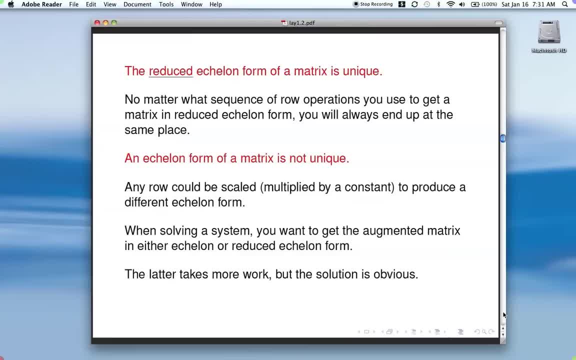 And the latter, to get it in reduced echelon form takes more work, But when you do that, the solution is obvious, And so let me show you what I mean by that. Here we have an augmented matrix that's already in echelon form. 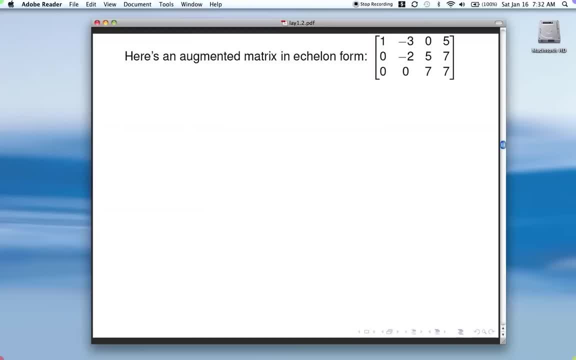 Notice: leading entry zero's underneath, Another leading entry zero's underneath And no rows of zero's. Each leading entry is to the right of the one before it, So it's in echelon form, And then we use back substitution to solve for the variable. 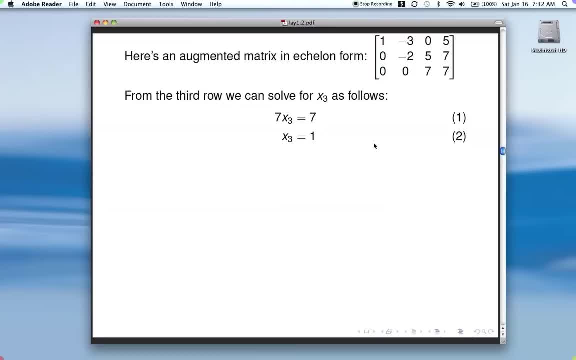 So start with the third row And the equation for the third row we get: 7 times x3 equals 7.. So we solve for x3.. Then we back substitute to solve for x2 in the second row. So second row: 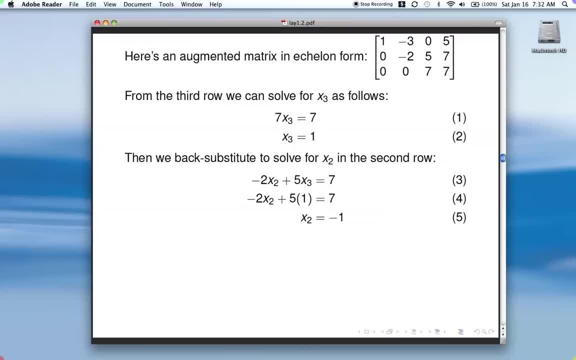 So second row says negative 2 times x2 plus 5x3 equals 7. And we know that x3 is 1. We just solve for that, So we plug that in here And we end up with x2 equals negative 1.. 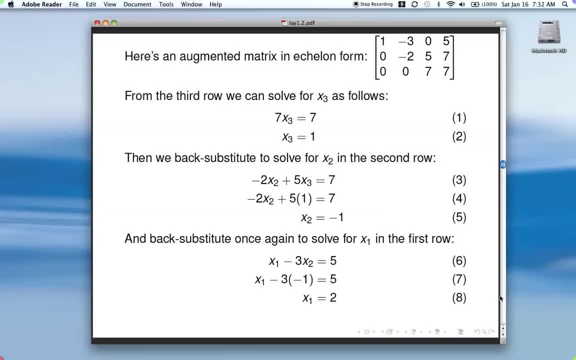 And then we keep going back up again to the first row. Equation for the first row looks like: x1 minus 3x2 equals 5. And we know what x2 is because we just solved for that. So we plug it in. 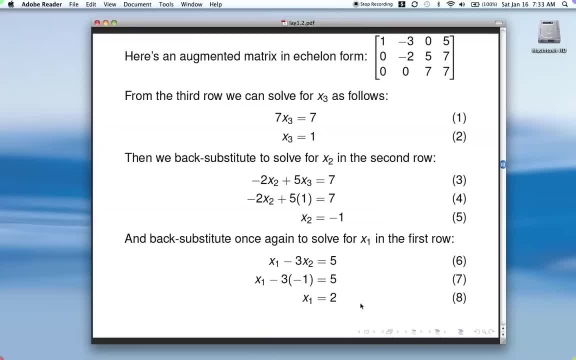 And then we end up with x1 equals 7.. So that's the method that we were using in section 1.1. And probably what you want to continue using for the most part. However, if you choose to get your matrix in reduced echelon form, 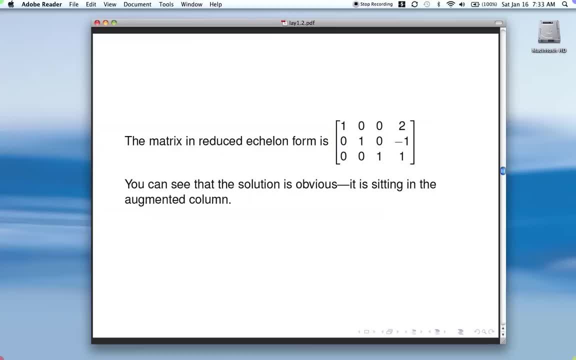 So this is the same matrix but in reduced echelon form. Then notice that you end up with the solution values of your variables just sitting in the right hand column, Because if you look at each row You know the first row says 1 times x1 equals 2.. 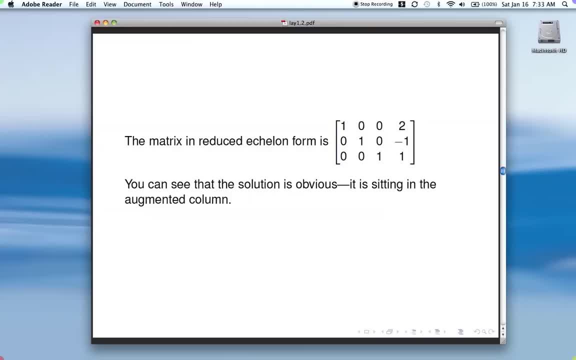 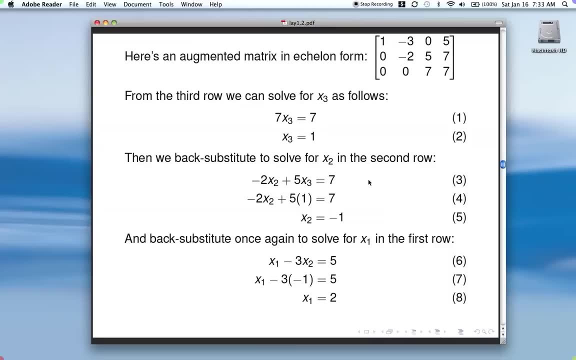 Second row: 1 times x2 equals negative 1. And so forth. So if you go back up You can see we got x1 is 2.. x2 negative: 1, 1.. So 2 negative 1, 1.. 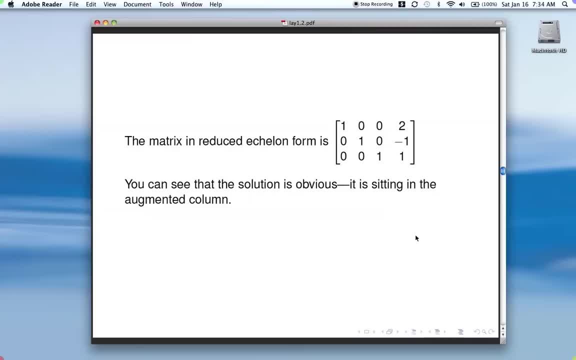 And there's 2 negative 1, 1.. So that's one advantage of getting it in reduced echelon form, Because then the solution is obvious And you don't have to actually do any back substitution. So it's kind of, your mileage may vary. 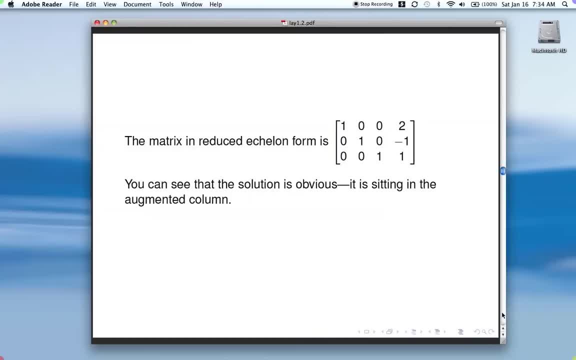 Whichever you like Will be fine. I think at this point we'll stop here And we'll pick up here in the next video. Okay, so, picking up from the previous video, Let's talk a little bit about a couple more pieces of terminology. 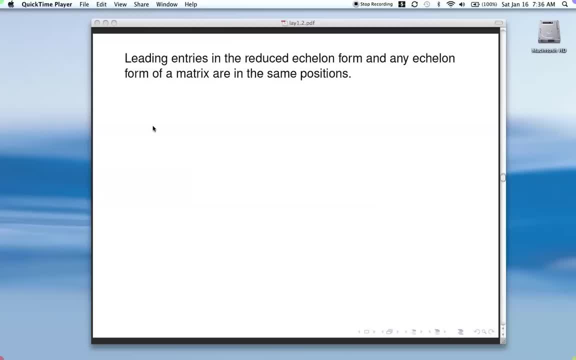 That we'll be using extensively throughout the course. Okay, so Remember, the leading entry is the first non-zero entry in a row In a matrix in echelon form. So it turns out that the leading entries in the reduced echelon form And in any echelon form, 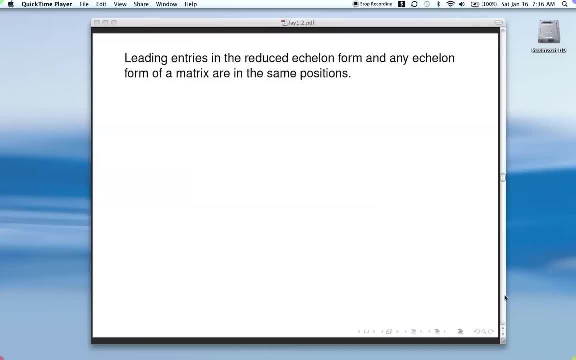 Are in the same position, I mean same location in the matrix. So here's the one we were just looking at. There was a leading entry in the 1, 1.. First row, first column. Second row, second column. Third row, third column. 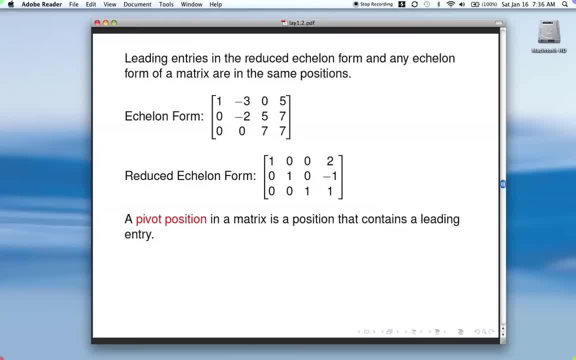 And, in the reduced echelon form, Same positions in the matrix. So it's convenient to talk about those positions As opposed to the actual value. The leading entry is the actual value, But we really are more interested in the position, And so we call that a pivot position. 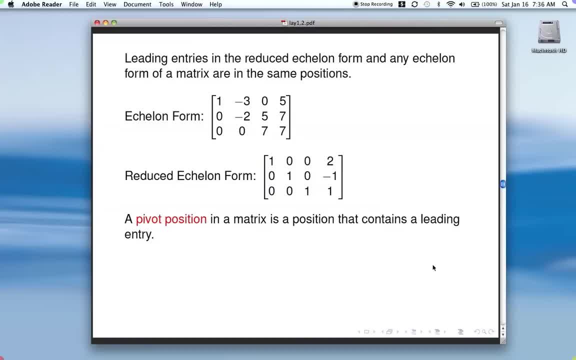 So a pivot position is a position that contains a leading entry, So the 1,, 1., 2,, 2., 3,, 3. Positions would be pivot positions in this matrix. As I said, the leading entry is the actual value. 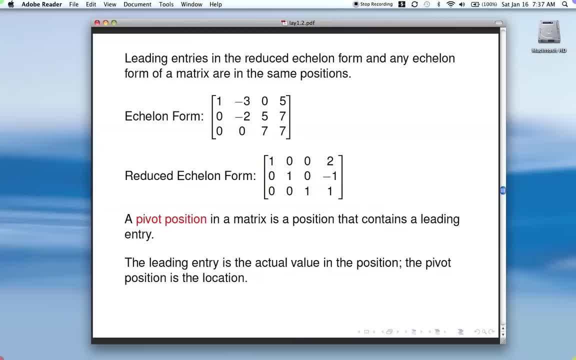 The pivot position is the location. So the leading entry here is 1. It's in the first row, first column. So that's the pivot position Here, this row, the leading entry is negative. 2. It's in the second row, second column position. 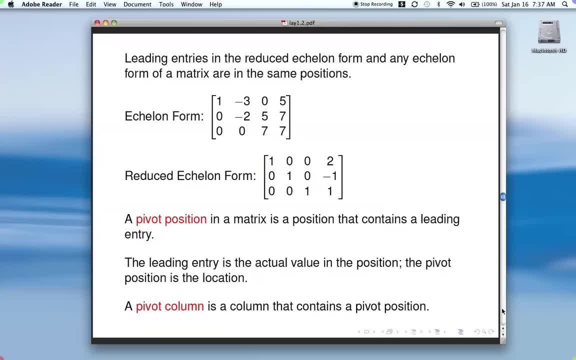 Okay, Another term is pivot column. Pivot column is a column that contains a pivot position. So I'll be using the terms pivot position and pivot column until probably the last day of the semester, So you will hear that quite a bit To make sure you understand what those are. 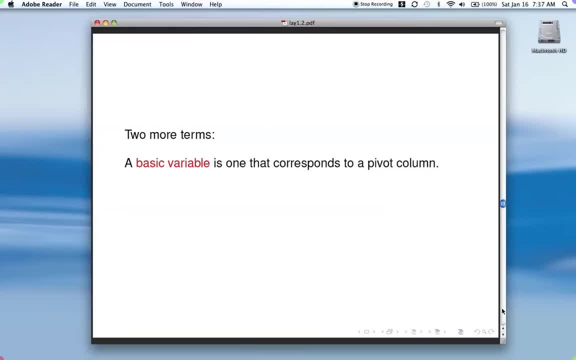 Okay, Two more terms. A basic variable is one that corresponds to a pivot column, And a free variable is one that corresponds to a pivot column, A non-pivot column. Okay, So for each column, except for the augmented column, there's a corresponding variable. 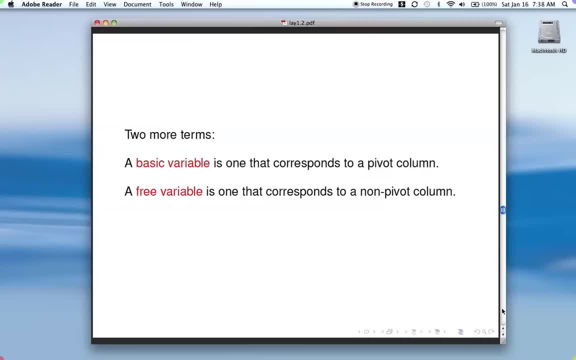 So if you look and there's a pivot column, that means that variable is basic. If the column is not a pivot column, that means that variable is called free. Okay, So let's look at how all this relates to Solving the system of the equation. 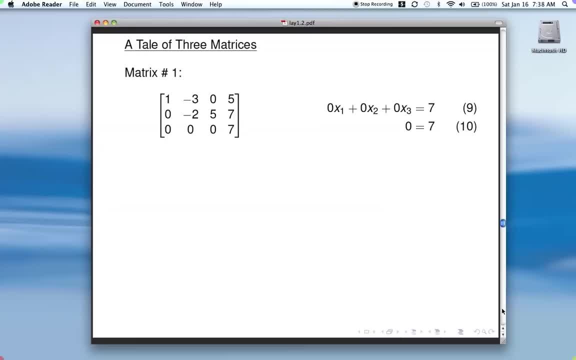 So I've got a tail of three matrices. Here's number one. Now notice this matrix If we It's already in echelon form Right. Here's leading entry. Zero's underneath Leading entry. Zero's underneath Leading entry. 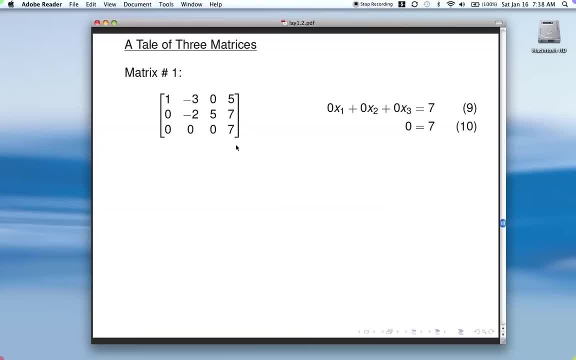 You don't need to worry about zero's underneath yet. So we start the process of solving the system. So we start with row three, And here's the equation that corresponds to row three. And if I simplify the left side, it's just zero. 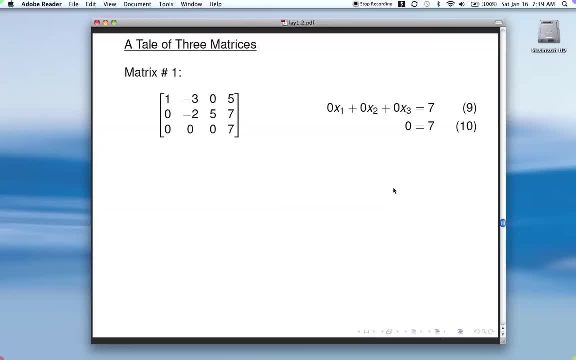 So I end up with zero equals seven. Well, we know that can't happen. So that is our clue: that this system has no solution. Okay, So if the echelon form of an augmented matrix has a row of this form, Okay, Where on the left you've got all zeros? 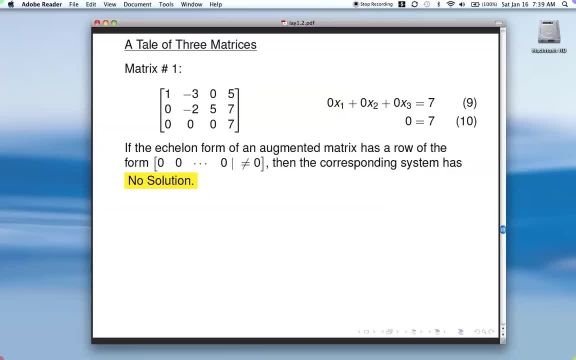 Then in the augmented column you have something not zero. Okay, So all zeros on the left, Not zero on the right. That's what we have here: All zeros on the left, Not zero on the right. Then the corresponding system has no solution. 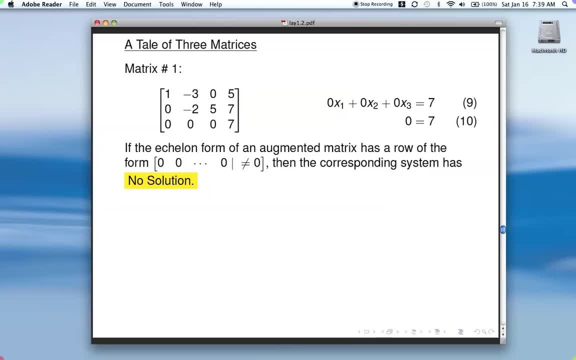 Okay, So that's the marker. That's what you need to look for to see if your system is consistent or not. Alright, Matrix number two: Change that first one just a little bit, And I put a number here, I put a non-zero value here. 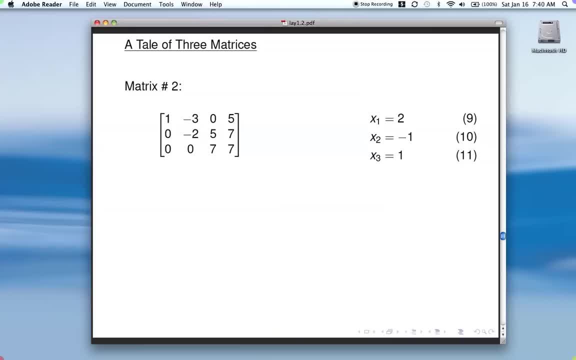 And so we've got leading entry Zero's underneath Leading entry, Zero's underneath Another leading entry. So this one's in echelon form. So we solve- And this is the same one we solved earlier, So I'm not going to go back through that. 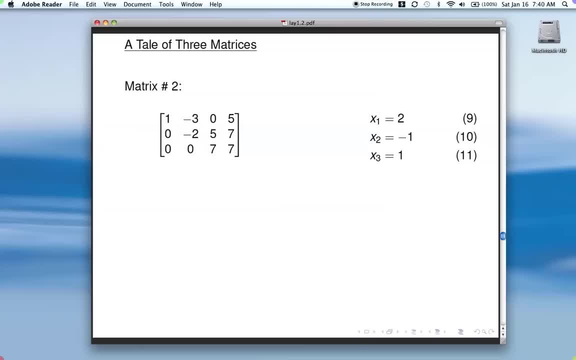 And this was our solution, And so this one. What Has a unique solution? The system is consistent. It's consistent because it doesn't have a row where there's all zeros and then something not zero, And it has no free variables. 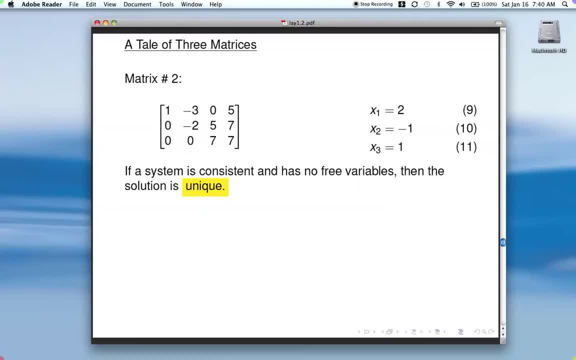 That's the key here for unique solution. Notice that there's a pivot position in every column of the coefficient part of the matrix. So pivot position in column one, So x1 is basic. Pivot position in column two, So x2 is basic. 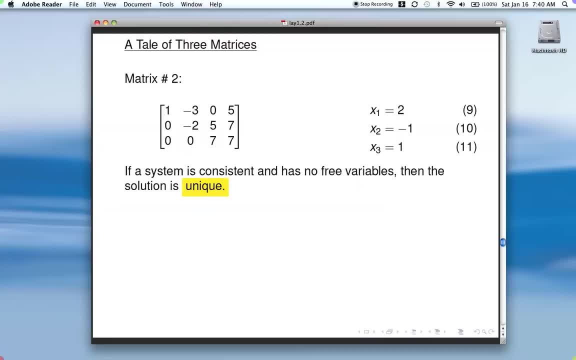 Pivot position in column three. So x3 is basic, So system is consistent. All the variables are basic. There's no free variables, And so we get a unique solution. All right, One more matrix. Notice here that we've got a row of all zeros. 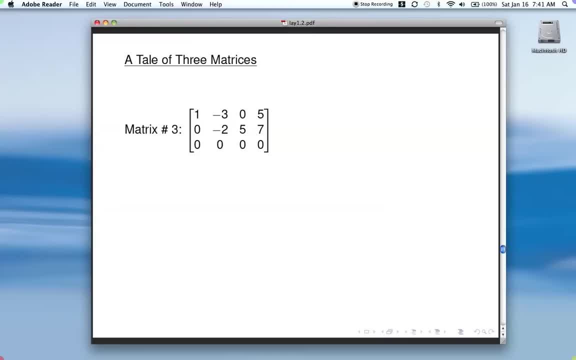 This one is in echelon form, But we've got a row of all zeros. Let's look for just a second. x1 here has a pivot position. The column two has a pivot position. Column three does not have a pivot position. 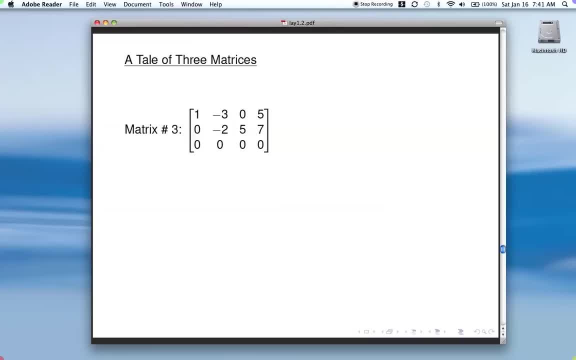 So that means that we have a free variable, right? x1 and x2 are basic, But x3 is a free variable because there's no pivot position in column three. OK, So if we try to solve it, here's what we get from row two. 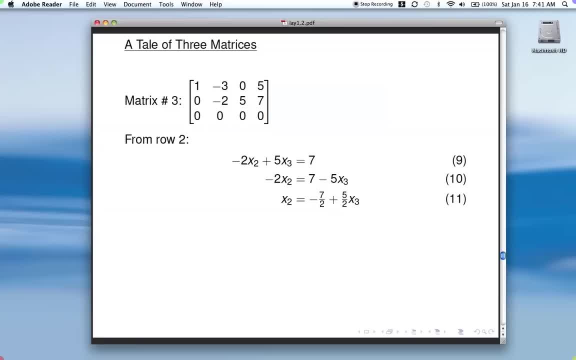 Negative: 2x2 plus 5x3 equals 7.. We solve for x2.. And notice that it's written in terms of x3. And then we back up to row one And we've got x1 minus 3x2 equals 5.. 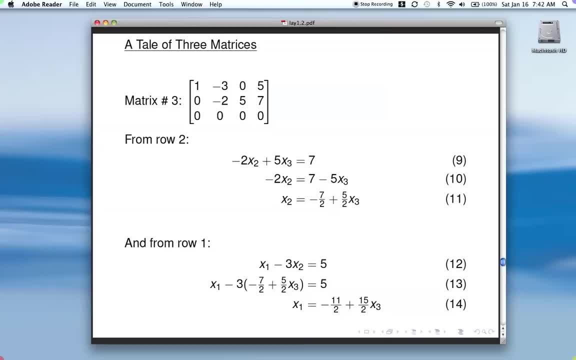 We substitute in for x2.. And here's what we end up with for x1.. Notice, it's also written in terms of x3.. Notice that. that's all. we've got these two equations, And so there's nothing constraining x3. 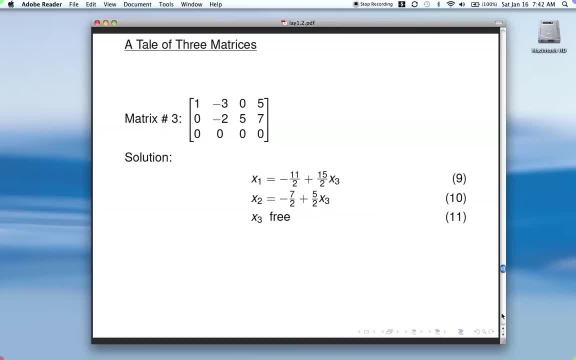 And that's because x3 is a free variable, And so if we write our solution, here's what it looks like, And in your book that's what they call the general form of the solution. OK, So this is just for x1, x2 what we just computed. 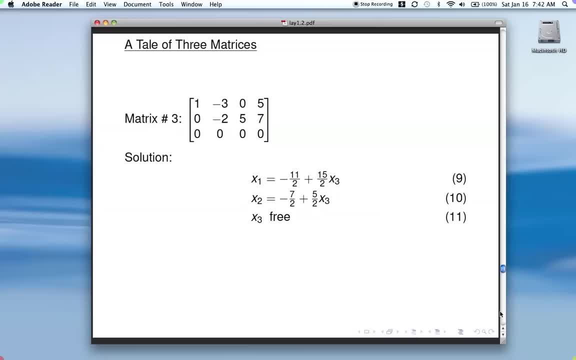 x3 is free. This is the general form of the solution, OK, So notice that we can plug in any value for x3 that we want, And any value of x3 produces a different solution. So that means we have an infinite number of solutions to this system. 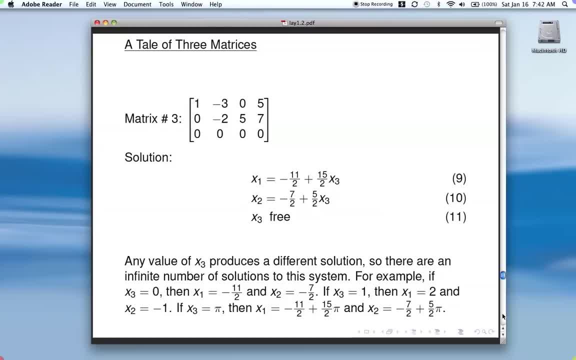 The easiest thing. if you want a specific solution, the easiest thing is to just plug in 0 for x3.. If you do that, then you get: x1 is negative, 11 halves, x2 negative, 7 halves. x3 is 0.. 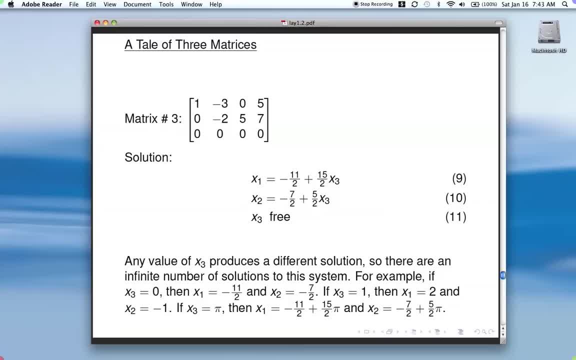 All right, Or you could plug in: x3 equals 1 and get another solution. I always tell my students: plug in your favorite number. So if your favorite number is pi, plug in pi for x3. And if you do that, then here's what you get for x1 and x2.. 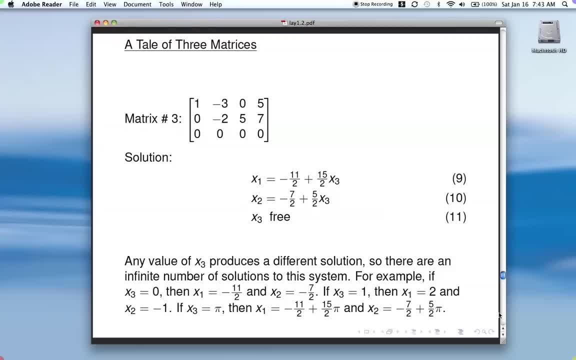 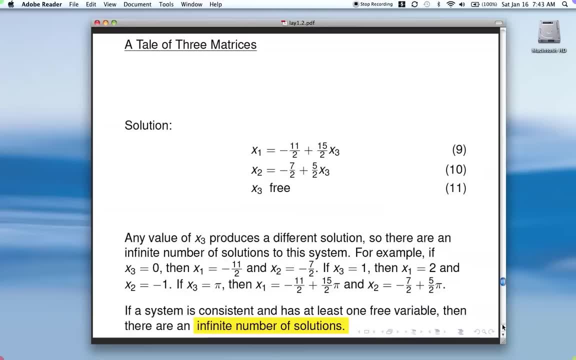 OK, So no matter what value of x3 you plug in, that generates a different solution, And so you have an infinite number of solutions. And so the bottom line is that if the system is consistent- and that's a key you got to- 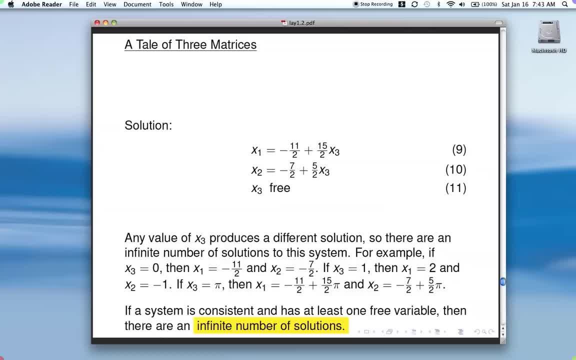 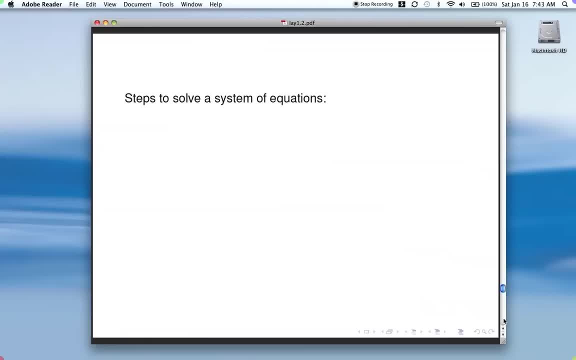 make sure it's consistent to start with and has at least one free variable, then you will have an infinite number of solutions. OK, So let's recap. When you're solving a system of equations, number one, put the augmented matrix in echelon form. 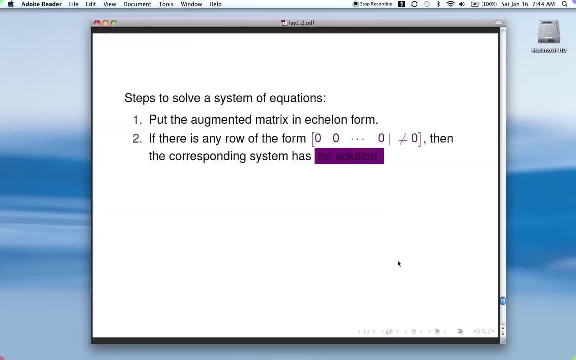 Number two: if you have a row of this form, all right, and this form is again all 0s on the left, something not 0 in the augmented column, then that means the corresponding system has no solution. At that point, stop, because you've got no solution. 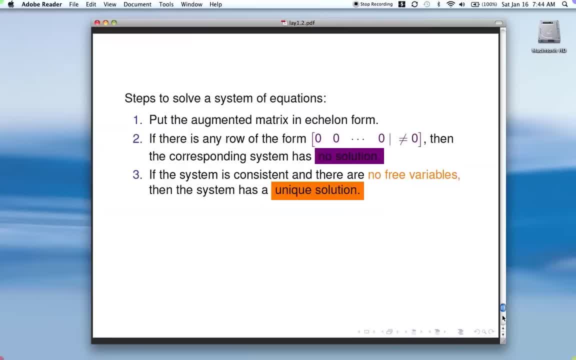 If that's not the case, then that means the system is consistent. So at that point you look to see if there are free variables or not. If there are no free variables, that means the system has a unique solution. If it's consistent and there's at least one free variable, then you have an infinite number. 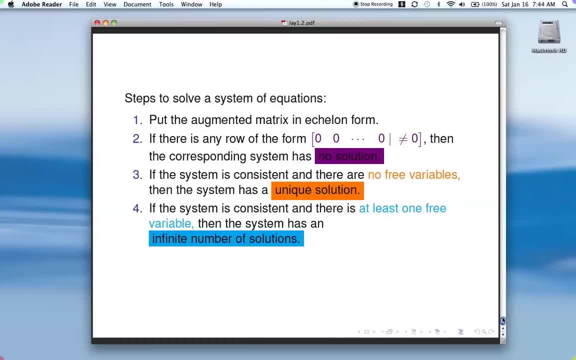 of solutions, All right. So that's really your algorithm there for how to determine how to solve a system and determine which case it is. Is it no solution? Is it a unique solution or an infinite number of solutions? OK, And that is it for this video. 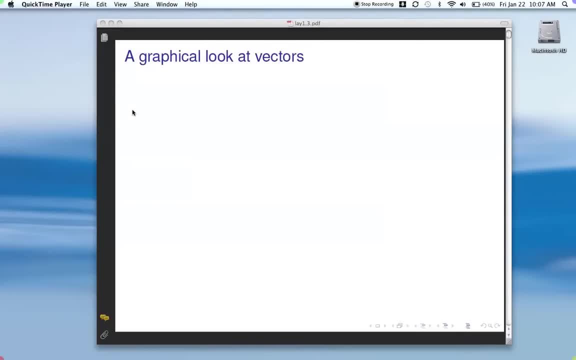 All right, We're going to start here with a graphical look at vectors. So we've kind of seen we've played around With matrices and augmented matrices and solving systems. But let's take a look at vectors from a graphical point of view. 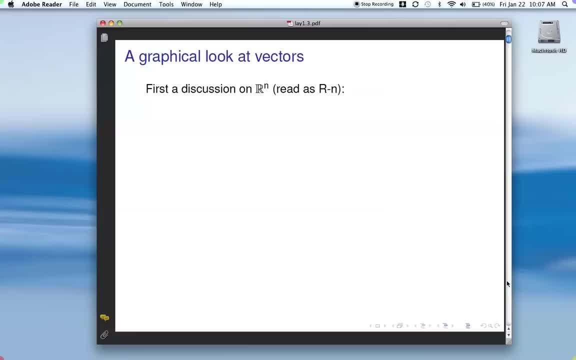 Before we do that, though, we need to discuss some terminology, So we'll start with RN. So you've seen this symbol, the fancy looking R That stands for the real numbers, And when you see a superscript, like here, with an N, excuse me, that indicates that you're. 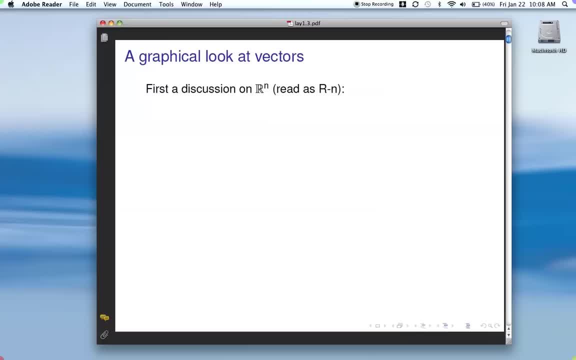 talking about vectors And so this, as I see here, you just read this as RN. OK, So RN is the set of all vectors having N components or N elements, each of which is a real number. So from a set point of view, you can look at it like this: 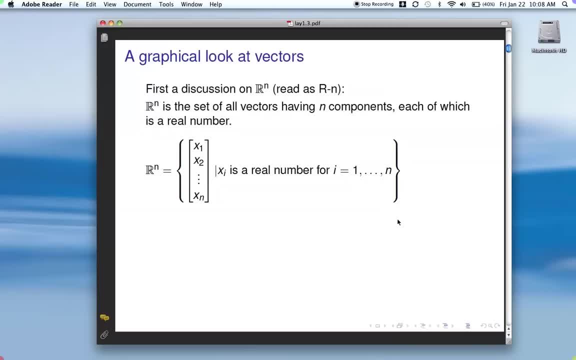 Set notation: OK. All vectors look like this: N components, where each one of them is a real number. A lot of times we'll just talk about R2.. Excuse me, In R2, the two indicates vectors with two components. 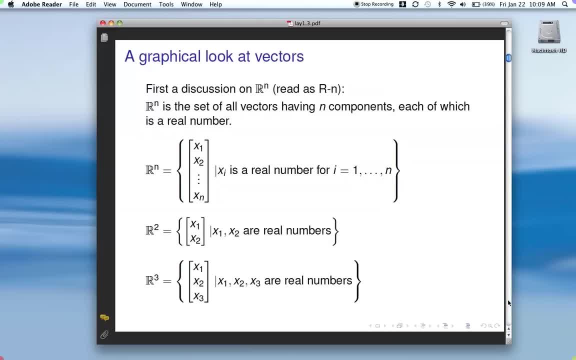 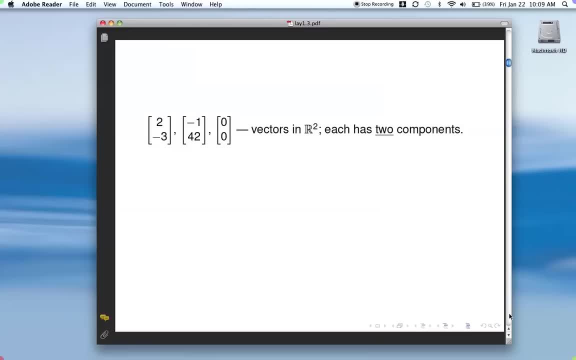 So there you go, And there's R3, similar sort of thing. We've got three components where each one is a real number. OK, So that's the set of all vectors. So, for example, here are three vectors in R2.. 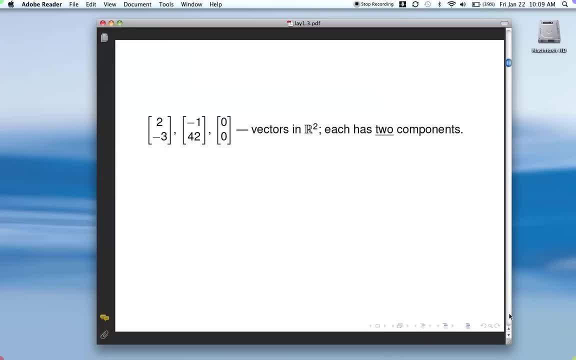 You know they're in R2 because they're vectors with two components. Each component's a real number And here they're vectors in R3 because they have three components. There are two operations that we need to know how to perform on vectors. 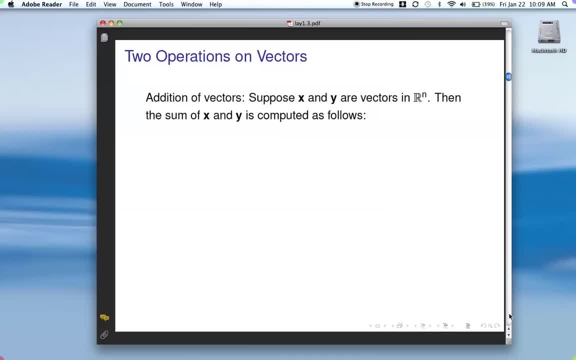 The first of these is addition of vectors. So if we have two vectors, x and y- in Rn, then we can compute their sum as indicated here. OK, Here's x, Here's y. Both have N components. To compute their sum, you just add components that are in the same position. 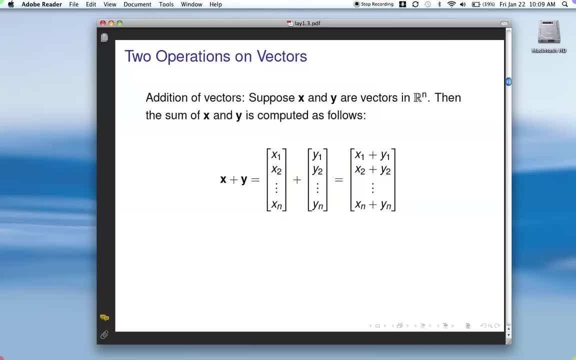 So first position: x1 plus y1, gives you the first position in the sum, Then x2 plus y2 and so forth to xn plus yn. So for example, If here's x and here's y to get their sum 0 plus 2 gives you the 2 here. 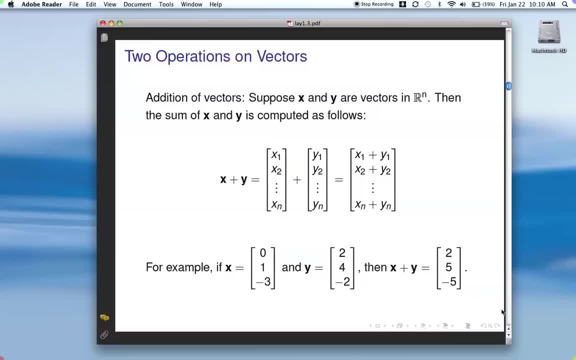 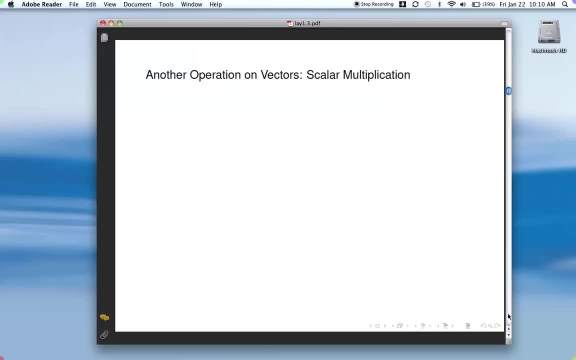 1 plus 4, 5. And negative 3 plus negative 2 gives you negative 5.. The other operation that we need to know how to perform on vectors is scalar multiplication. Excuse me again Um Scalar multiplication of vectors. 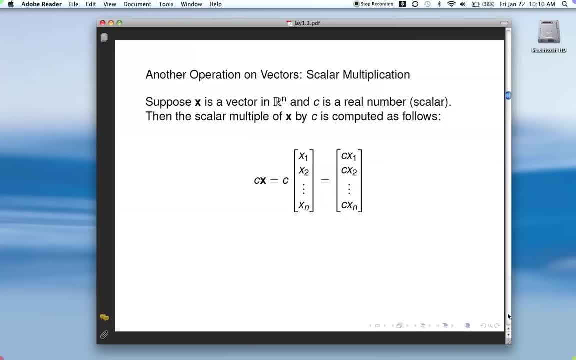 Scalar multiplication of vectors is based on the idea that you have a scalar which is just a real number, a single number that you want to multiply by a vector, And so the way you do that, as indicated here, you just multiply that number by each element. 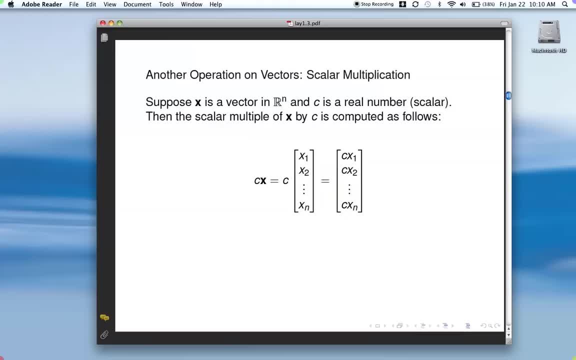 in the vector. So we get Cx1,, Cx2, down to Cxn. So for example, if here's your x and you want to multiply 4 times x, then you just multiply each component in the vector by 4.. 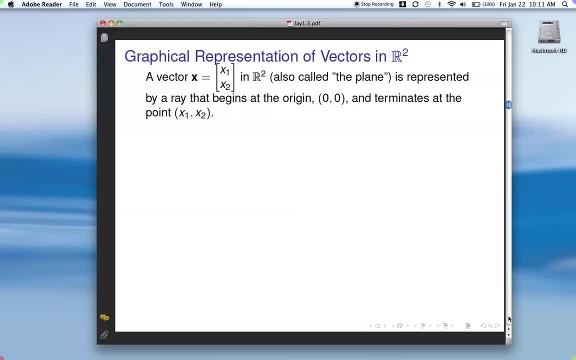 Okay, now, with that we can start to talk about a graphical representation of vectors, and we'll restrict our attention, at first at least, to R2.. Pardon me, A vector in R2, also called the plane- you're probably familiar with that terminology- is: 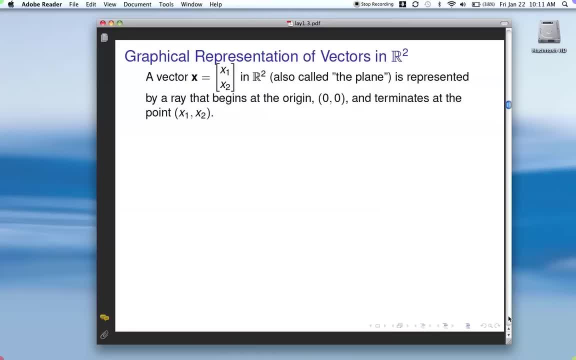 indicated by a ray Ray. A ray begins at the origin and terminates at the point defined by the vector. So here's a couple of vectors and you can see how they look on a graph. Okay, so U is 2, 1,, so we have a ray that begins at 0, 0 and terminates at 2, 1,. similarly, 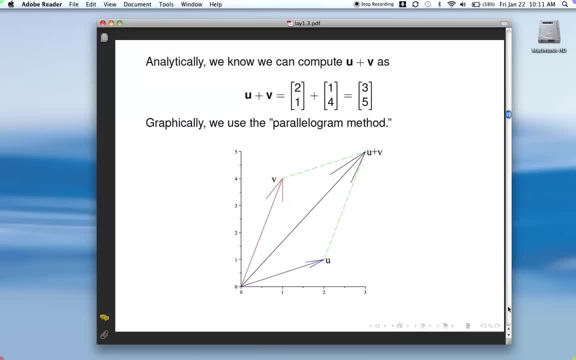 for V. Um analytically, we know we can compute U plus V in this fashion. right, just some like terms: 2 plus 1,, 1 plus 4, give you 3, 5.. Graphically, um we use the parallelogram method. 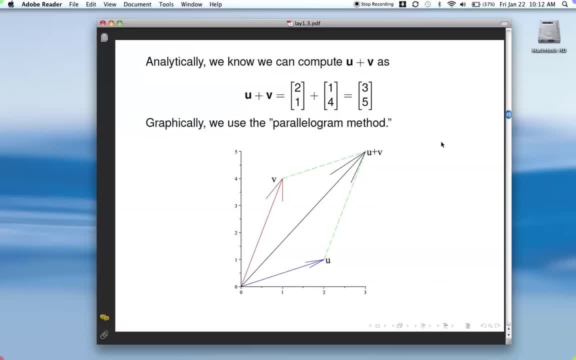 You might be familiar with this from your physics class or engineering or um, or maybe even like Calc 3 if you had that. So the way that works is you go to the end of uh, one of the vectors, and you draw a. 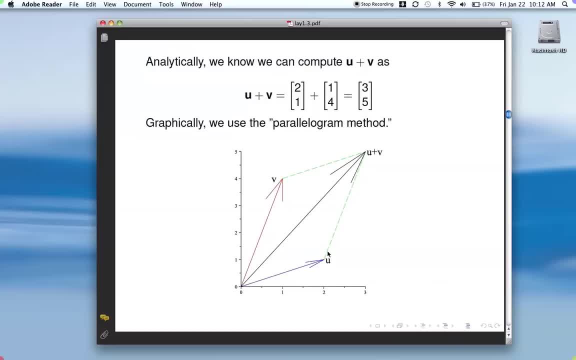 line that's parallel to the other one. Okay, So this line here would be parallel to V, And we do the same thing for the other vectors. So go to the end of V, draw a line that's parallel to U. See, this line is parallel to U. 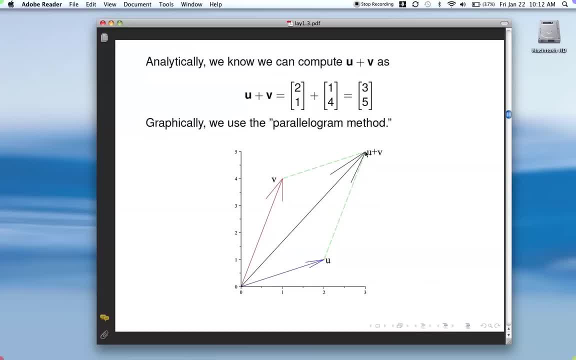 And where those two lines intersect. that is the sum of the two vectors. So this vector here would be U plus V, And you can see that it's at 3, 5.. Um- scalar multiple of a vector, Um. I did a couple of examples based on those. 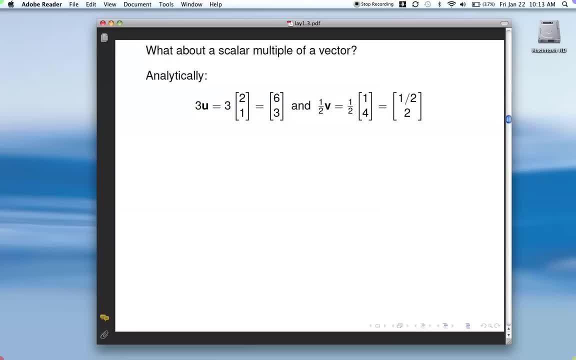 We were just looking at 3 times 2, 1.. It's just uh, 6, 3.. And here's a half of V. If you look at that graphically, um 3 times U is a vector, that's. 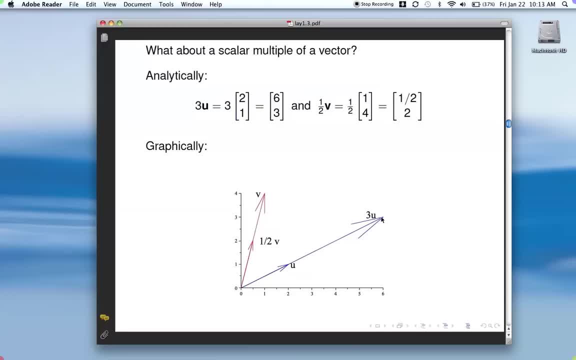 in the same direction as U And it's just 3 times uh as long. So basically you got 3, 3 U's uh stacked there, And so you can see that it corresponds. There's 6, 3.. 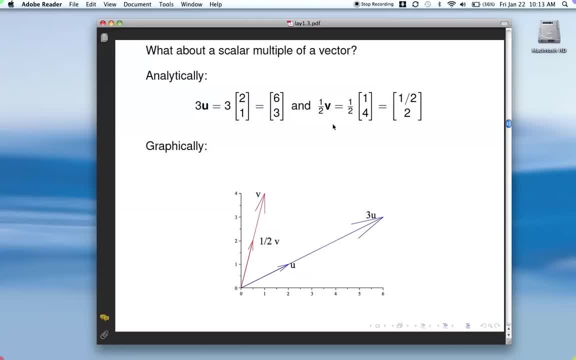 Okay, And uh, one half of V is is, uh, what you would think? One half of V. So you can see that it's a vector, same direction as V, but half the length. Um, we can add those two together. 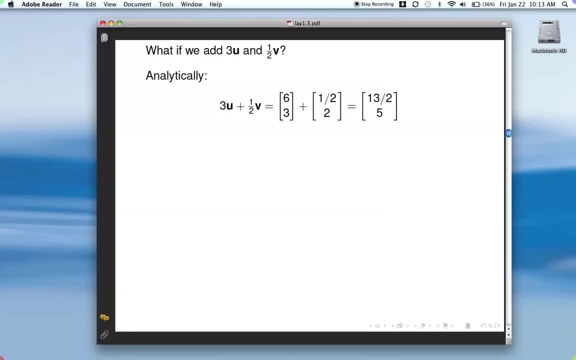 All right. So this is how we do it: 3 times U plus a half V. We already know how to do these operations And graphically take our one half V. Okay, So Align parallel to 3. U Do similarly over here. 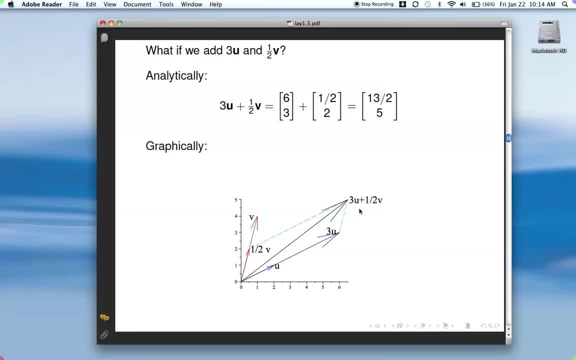 And the resultant vector. here is what we think it should be about: 13 halves 5.. Okay, So notice that you can scale U to whatever length you want, You can scale V to whatever length you want, And then add those two vectors together. 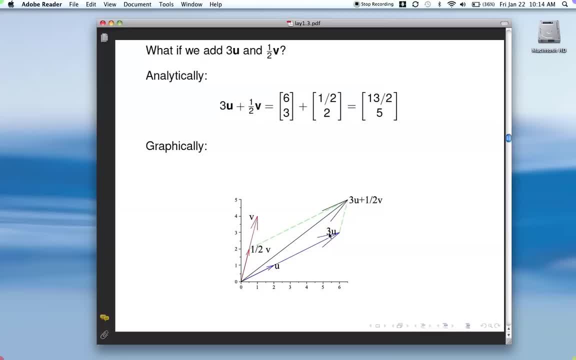 And if you do that, then think about where the vectors would end up, Any vectors that you can: scale U however you want, scale V however you want, and then add them together And let's think about that. Um, so this would be any multiple of U, uh, any multiple of V, And for the moment, let's 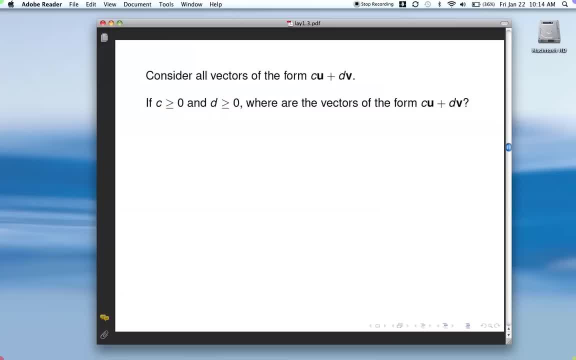 restrict our attention to positive multiples or non-negative multiples. Okay, So let's uh assume that C and D are both non-negative. If we do that, Then The vectors that we can produce or generate um are here in this cone defined by U and. 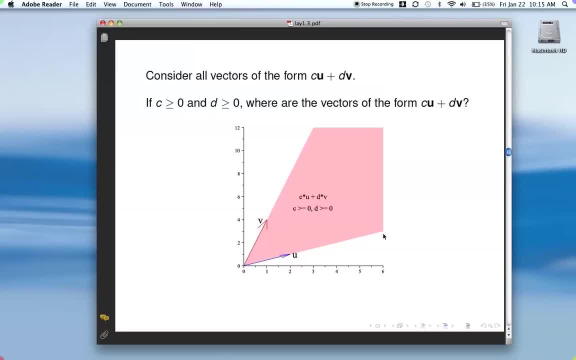 V. Alright, Because again, we can scale U to whatever length we want, we can scale V to whatever length we want and then, when we complete the parallelogram, then we can end up with any vector in this cone area here. 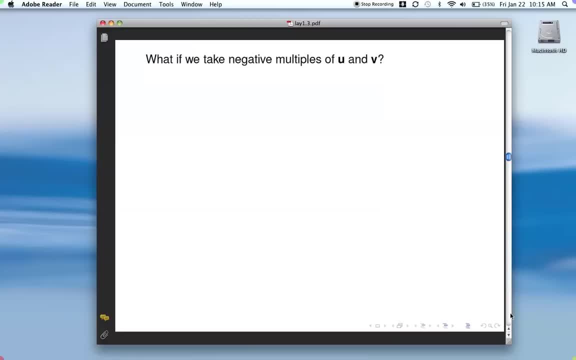 Um, If you allow yourself to take negative multiples of U and V, Okay, Um, then think about where those vectors would be in the plane. The easiest way, I think, to think about this is to um, instead of thinking about taking. 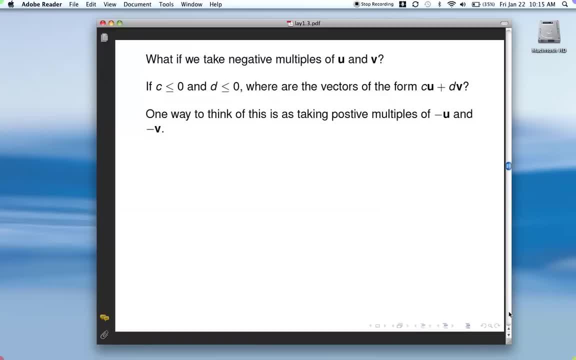 negative multiples of U and V, about thinking of it as taking positive multiples of negative U and negative V. Alright, And if you do that, then it's a similar thing as to what you just saw. Okay, So Here Is. 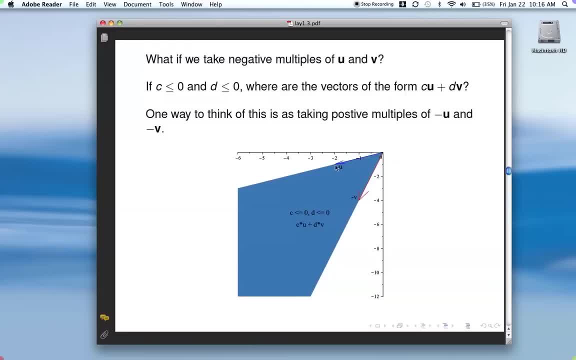 Negative V, Here's negative U, And so when you take positive uh multiples of U and V uh, or positive multiples of negative U and negative V, and then uh, add those two vectors together, you end up with uh vectors in this region here. 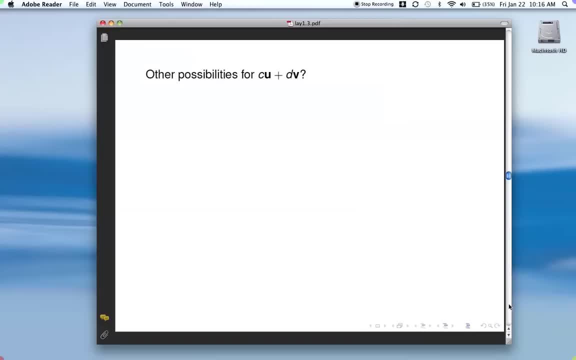 Okay, So um other possibilities for for um, uh, C and D. Let's think about that. Okay, Um, if we allow um positive multiples of U and negative multiples of V, then we're in this yellow region here. 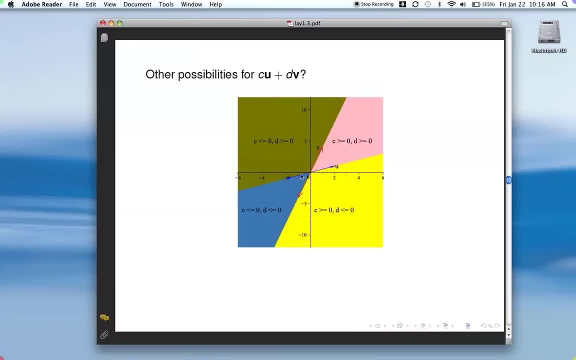 And, uh, if we allow positive multiples of V but negative multiples of U, then we're in this region here, And so what you see is that, um, we can generate any vector in the plane that we'd like, just like, just by taking a multiple of U and a multiple of V and adding them together. 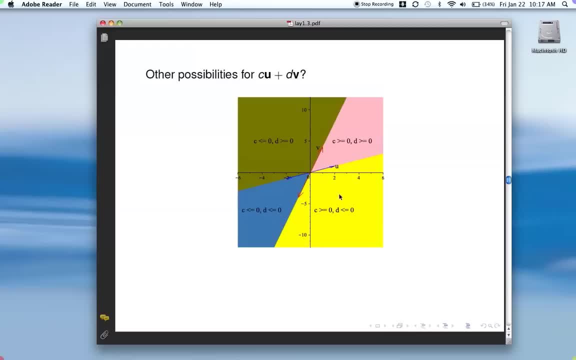 Okay, So we're gonna see in a little bit that this means that U and V span the plane, So we can take multiples of each one of those and add them together and generate any vector in the plane. That's what it means to span R2.. 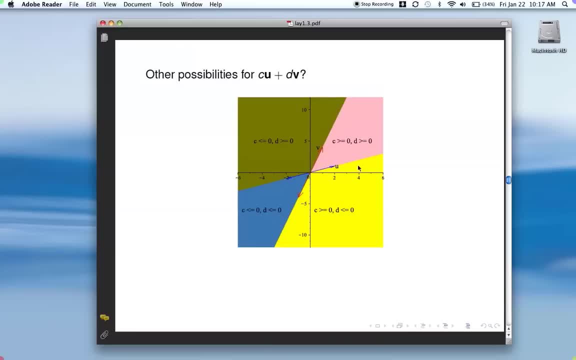 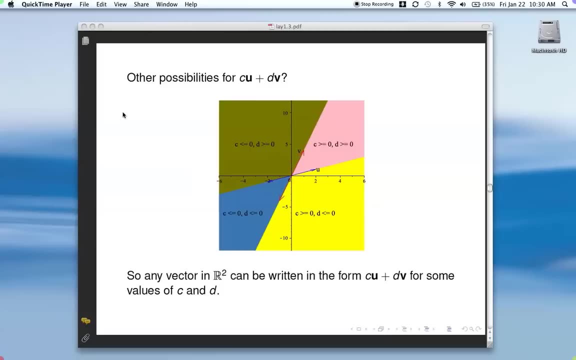 All right, So I'm gonna stop here for now And then we'll pick up this in our next. Okay, We're back uh, where we left off of the first video and we were looking at this picture where we determined that, uh, based on our vectors U and V, here we could take uh multiples. 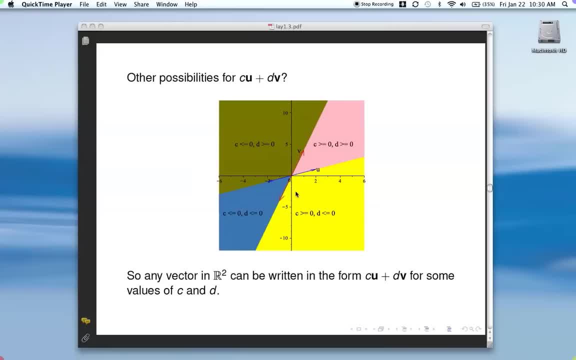 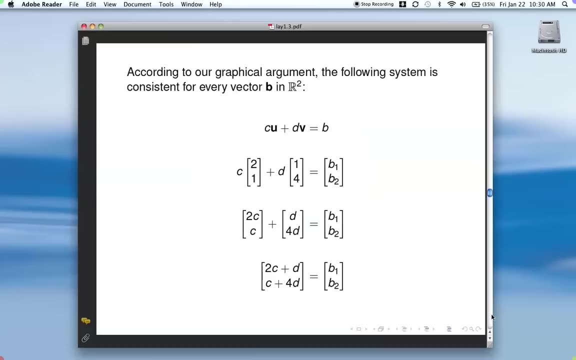 of each one of those and add them together to produce any vector in the plane. So any vector in R2 in the plane can be written in the form C times U plus D times V for some values of C and V. Okay, Let's look at that analytically now. okay. 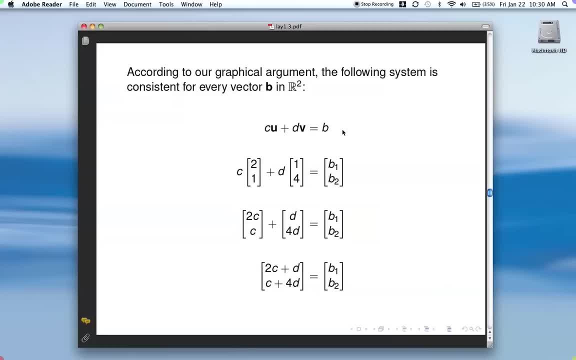 So, according to our graphical argument, this system is consistent for every B in R2.. You can take some multiple of U, some multiple of V, add them together and get any vector in R2.. So if we break that down um, we can uh multiply C times U. This is U, This is V. 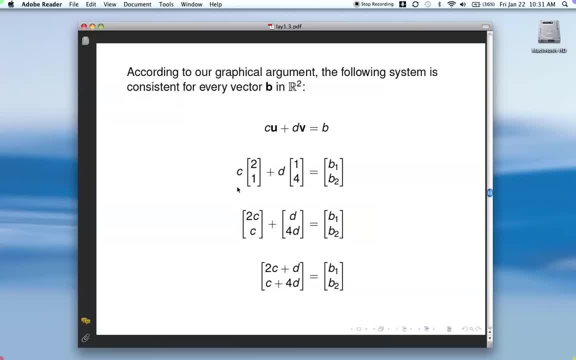 Here's our generic Right-hand side vector. We multiply through by the scalars, We end up with this, And then adding these two together gives us this matrix here. Now, what does it mean for two vectors to be equal? Well, it means that component-wise they're equal, okay. 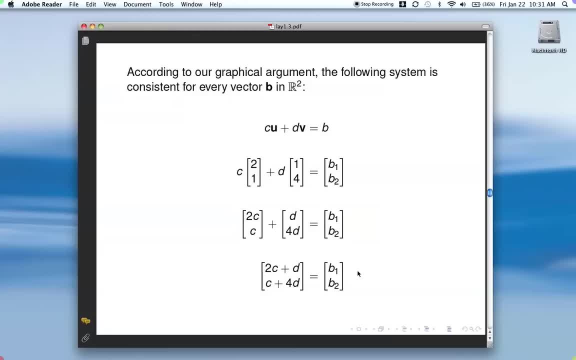 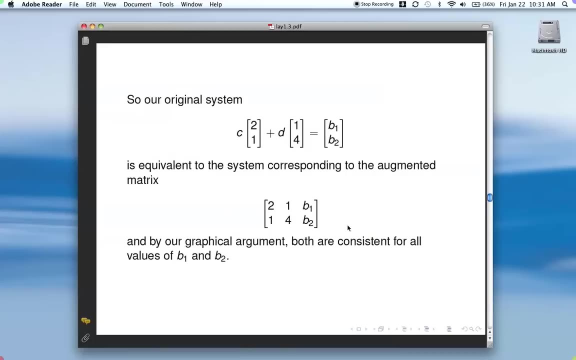 So the first component here is equal to the first component here And likewise the second component. So what we have is a system of equations: Two C plus D equals B1.. C plus 4D equals B2.. So we can put that in an augmented matrix and that's what I've got here and notice. 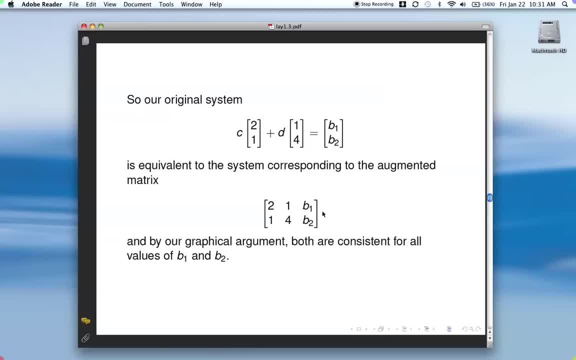 that, again, according to our graphical argument, our picture that we looked at um this uh system corresponding to this augmented matrix is consistent, no matter what B1 and B2 are, And also notice that these are equivalent. Okay. 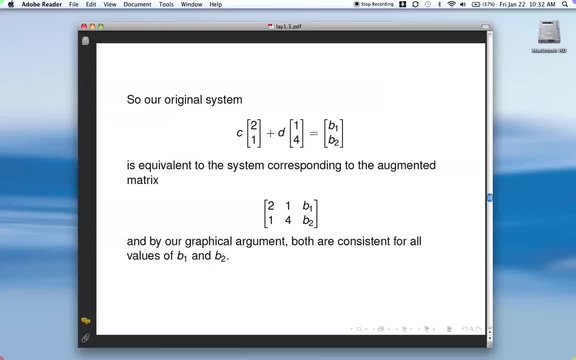 So when we have a multiple of vectors- A vector plus uh, another multiple of a vector- then uh equals some right-hand side vector. Notice how this system relates to this augmented matrix. So the first vector here just goes in the first column. 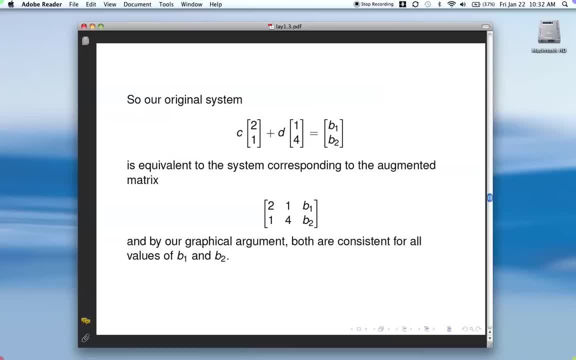 Second vector goes in the second column and the right-hand side's just in the right-hand side column. So these are equivalent. Okay, Let's look at this system a little more closely. Um- I- I swapped rows to um. make the arithmetic look. 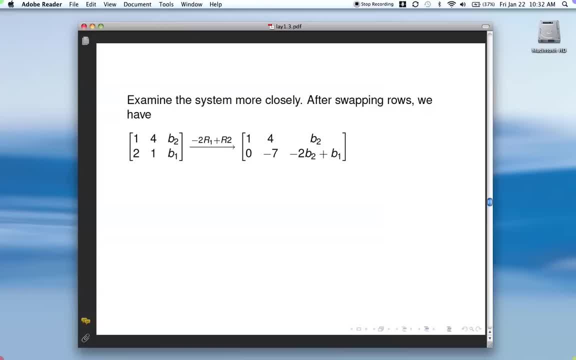 Okay, It's gonna take a little easier to get the one in the pivot position here and we can do a row operation to zero out underneath and we end up with this matrix. Now, remember, this has a solution, no matter what the right-hand side is. 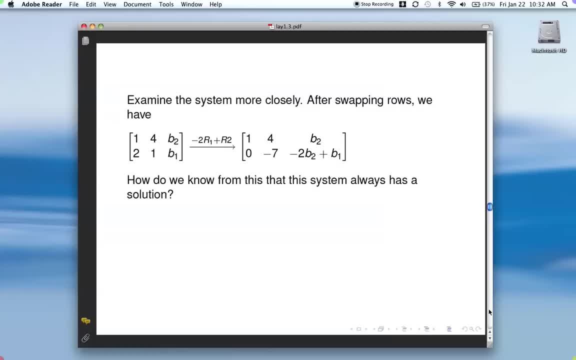 Okay, Now, how do we know that that's the case? Um, we know it graphically. but how can we look at this augmented matrix and tell that? Well, notice that there's no way to have a row of this form: a zero, zero, something. 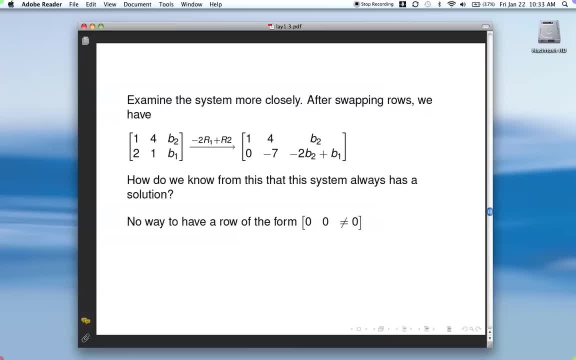 not zero. uh, form Okay, And that's because in each row we have a pivot position, a pivot position here, so that's never gonna be zero. We have a pivot position here, so that's never gonna be zero, So there's no way to have a row of this form here. 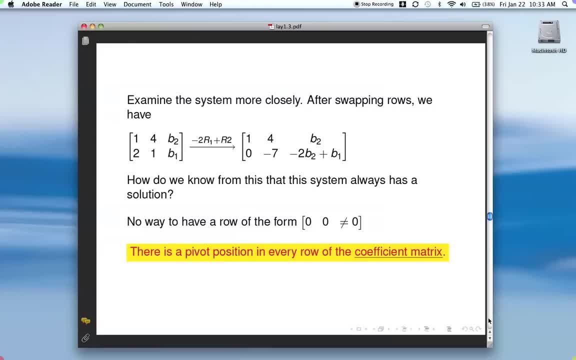 Okay, So the bottom line is that your system will be consistent, no matter what the right-hand side is, if you have a pivot position in every row of the coefficient matrix. Okay, Remember, we're talking about the coefficient matrix, because I'm talking about just this. 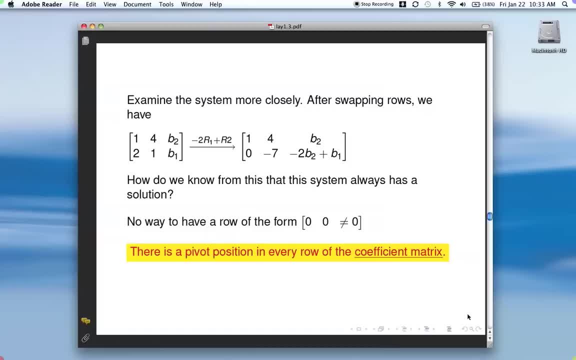 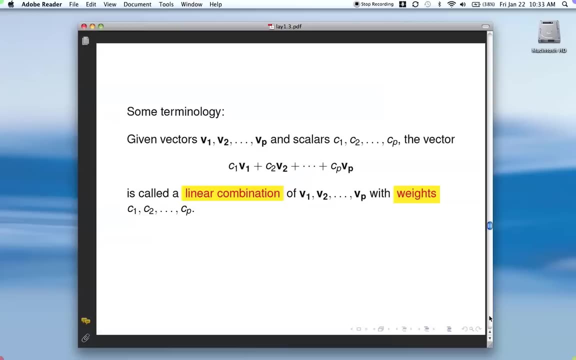 part here not looking at the right-hand side. You don't want your right-hand side to be a uh, to have a pivot position, because then that would indicate the system's inconsistent. Alright, Let's uh kind of take what we've looked at so far and put it in the terminology: um. 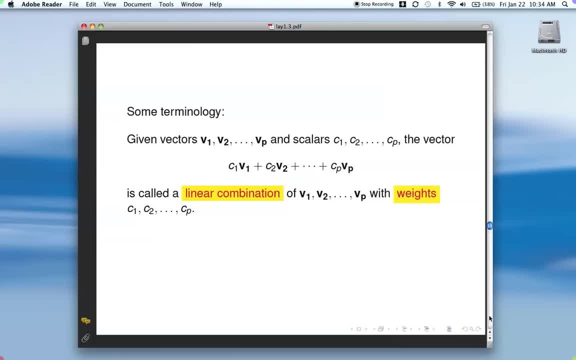 of uh data Okay, The uh text Okay. So, um, if we start off with an arbitrary set of vectors v1 through vp and scalars c1 through cp, then if we, if we apply the scalars to the vectors and add them up and 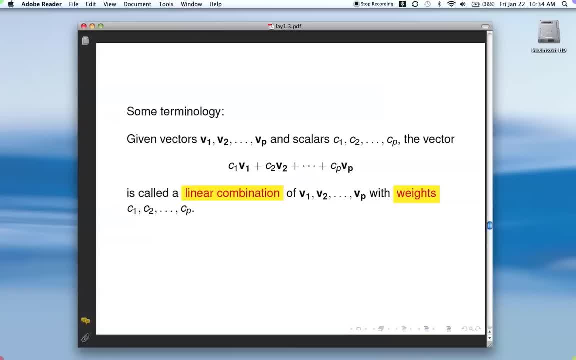 that's what we were doing earlier. we only had two vectors, but here we've got an arbitrary number of vectors. Okay, This is called a linear combination of the v's With weights c1 through cp. Okay, So, um, this, these, when we've been multiplying by a scalar and adding vectors together. that 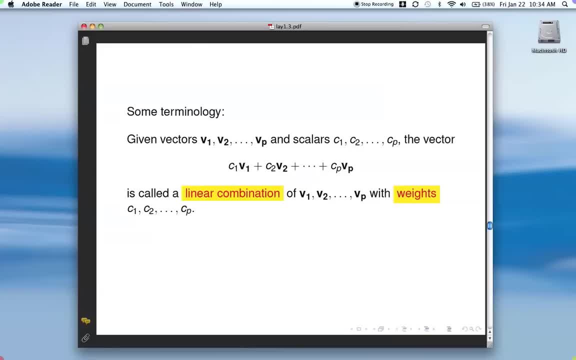 we were taking linear combinations. Okay, So a linear combination just looks like this: You've got a scalar multiplied times a vector, um, and you have that uh for however many vectors you have, and then you add them all up. 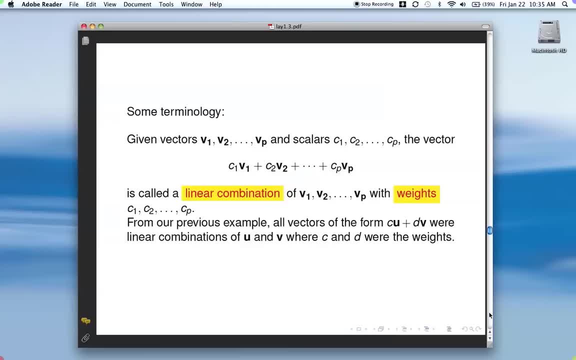 That's what a linear combination is. Okay, So we were doing c times u plus d times v. That was a linear combination of u and v, where c and d were the weights we were using. Okay, Now here's a linear combination. 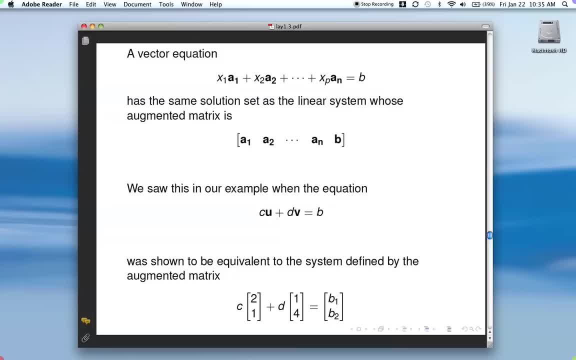 Okay, Here the x's are being the weights and the a's are vectors. Okay, So this is uh x1 a1 plus x2 a2 and so forth. Um, oh, that should be xn an. 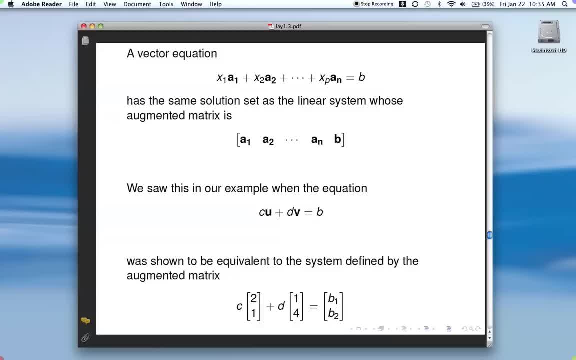 And um, Okay And uh, that has the same solution set as uh, the system given by this augmented matrix. Now, if you remember, before we started off with an equation like this, We just had two vectors. But um, then, when we got it into matrix form, remember, I showed you, you take your first. 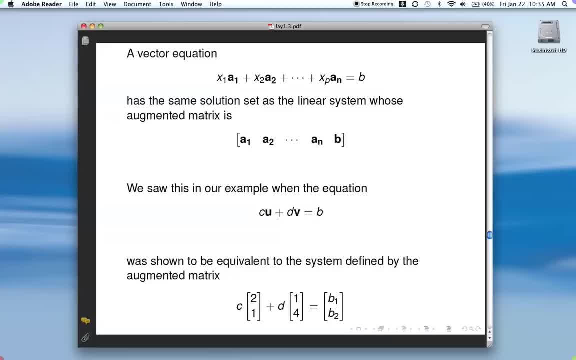 vector. here it goes in the first column in the augmented matrix. Second vector goes in the second column, and so forth. Last vector goes in the last column. and then you got your right-hand side. Um, here we see that, uh, we've got, uh, u ended up. uh c times u plus d times v. 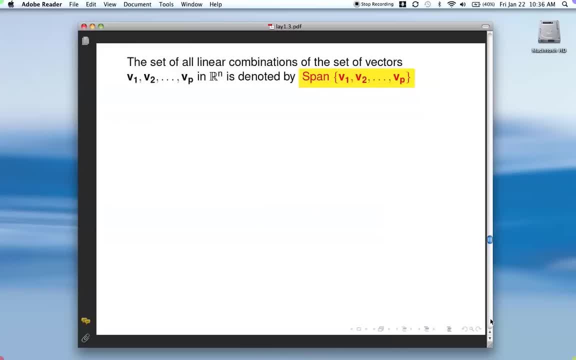 And, uh, we ended up with that augmented matrix that we saw earlier. Okay, Uh, one more term, and I used this in the previous uh video, but, uh, we'll uh define it more formally here. 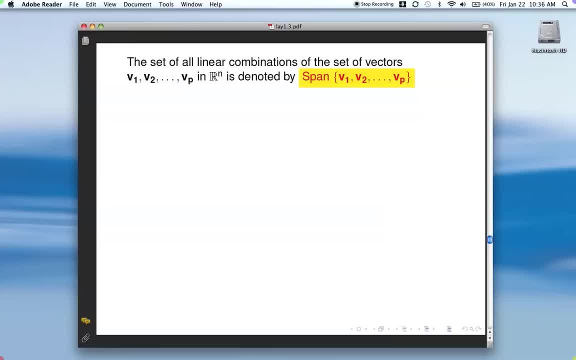 The set of all linear combinations of the set of vectors v1 through vp in Rn is denoted by the span of v1 through vp. Okay, So set of all linear combinations of vectors is the span of that set of vectors. Okay. 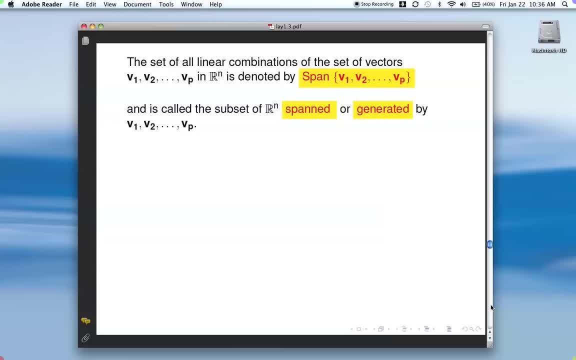 And the span of that set of vectors is is just, uh, called the subset that is spanned or generated by those vectors. Okay, So if you recall back, um, when we were looking at our example, um, we, uh, I talked about 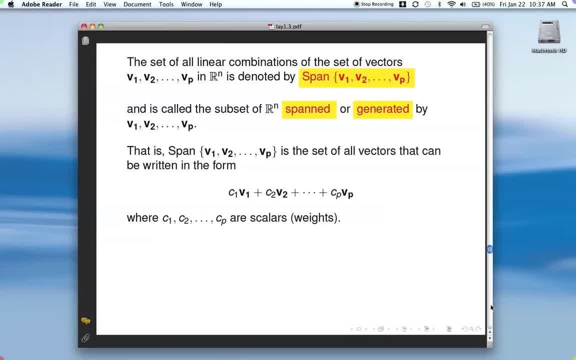 how you could span, uh, my two vectors, u and v, that we had. they spanned R2.. We're going to look at that in just a sec. Um, here's another way of looking at it. The span of v1 through vp is all vectors that can be written in this form. 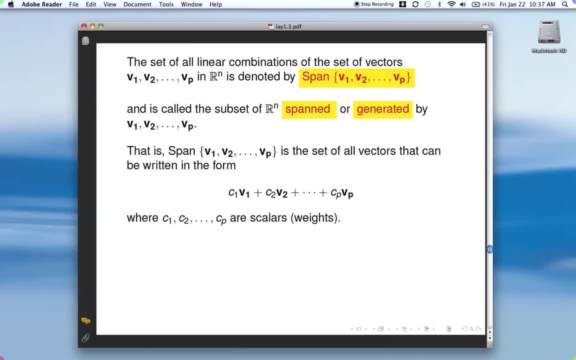 And what is this form? It's just linear combinations. Okay, So the span is just the set of all linear combinations of those vectors. And here's the previous example. Um, we've got c times. this is u plus d times v equals v1, v2.. 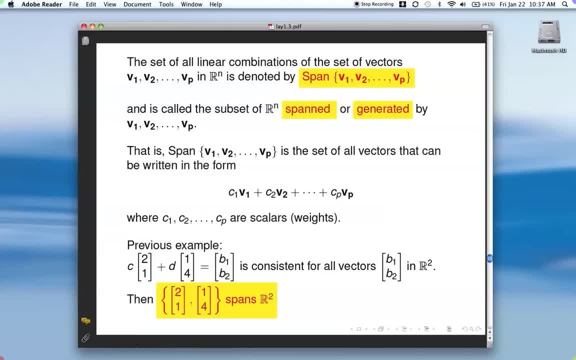 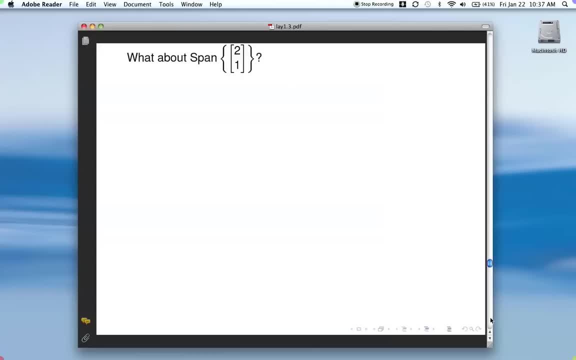 Okay, So that means that these vectors span R2.. Uh, let's back up just a little bit. What? what If we looked at the span of a single vector? what would we get there? Well, back to the definition: all linear combinations of that vector and linear combinations of 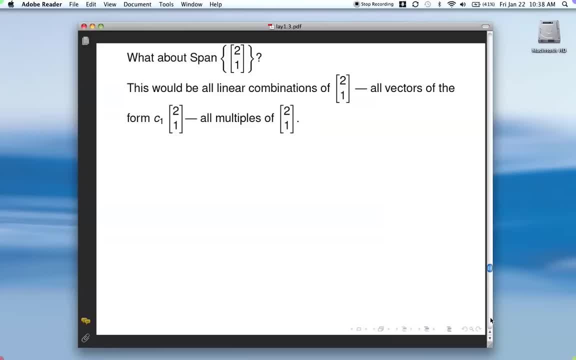 just one vector means just all multiples of that vector, And so, graphically, what that is is just the line that goes through the origin and, uh, that vector. So it's just all multiples of u, So anything on this line. 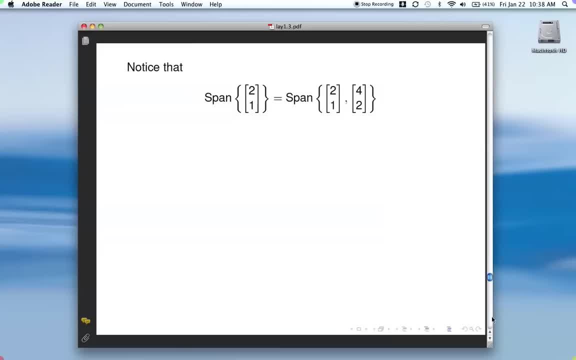 Uh, here's another thing to think about. Um, the span of the vector is the same as the span of this set of vectors. Now, why would that be? Well, here's definition: A span of is just all multiples of Span of the two of them is all linear combinations of the two. 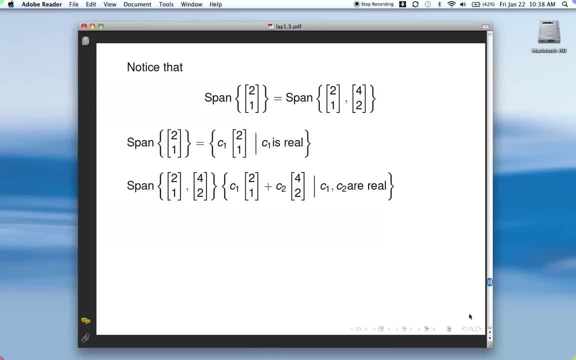 Now, why would these two sets be the same, Okay? Well, the key is to notice that is a multiple of, So it really doesn't add anything because you can take a multiple of to get. So by adding to the set, as I did here, it doesn't get you any more vectors, okay. 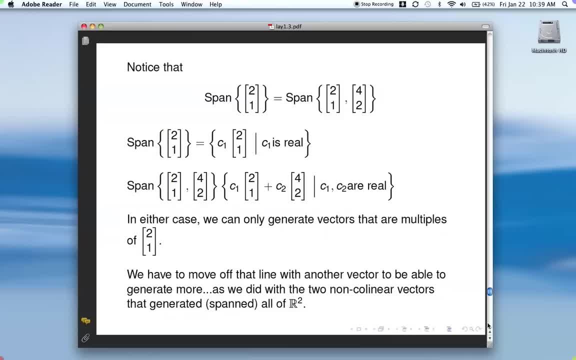 And so you have to move off that line defined by the vector uh to generate uh more vectors, And that's in our example. before we had two uh vectors that were not collinear, And so in that case you could generate or span all of our two. 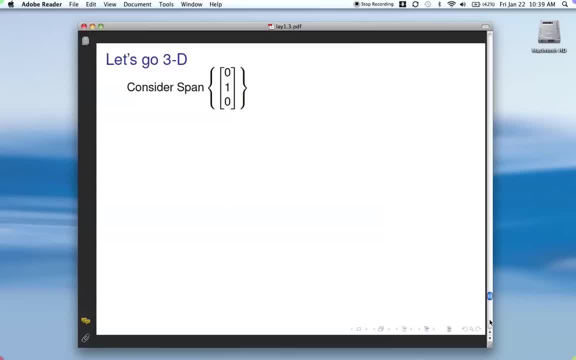 Okay, let's. let's look a little bit in uh, at a three-dimensional example. So if we look at the span of this vector, uh, that would just be all multiples of that vector And graphically, um, we're saying, that's that x has to be equal to x. 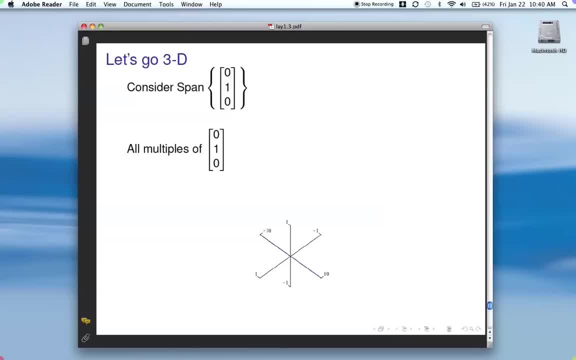 Uh, so that's, that's what we're saying. Okay, So x has to be zero, z has to be zero, but y could be anything, because you can multiply anything by one. So essentially you're on, uh, the y-axis, alright. 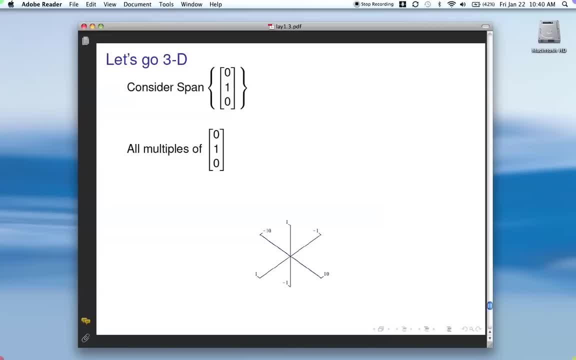 So x has to be zero, z has to be zero, so anything along the y-axis If we add another vector to it. so I throw in this one now. we take all linear combinations of these two And notice that in this case you get all vectors. 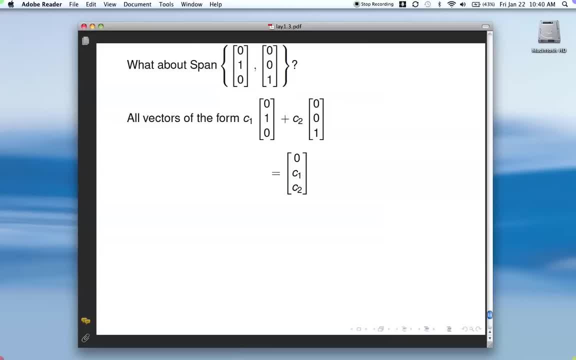 They look like this. So it means x has to be zero, but y and z can be anything we want them to be, And so that gives us a plane, okay, where x is zero but y and z are anything that that we want them to be. 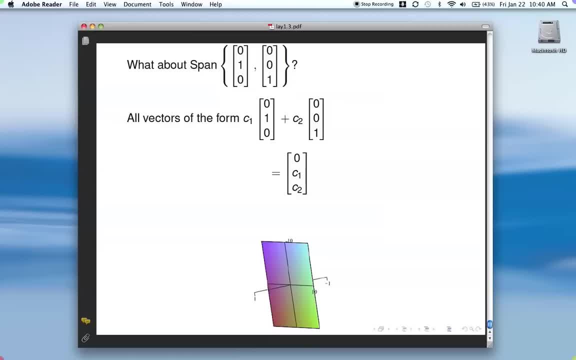 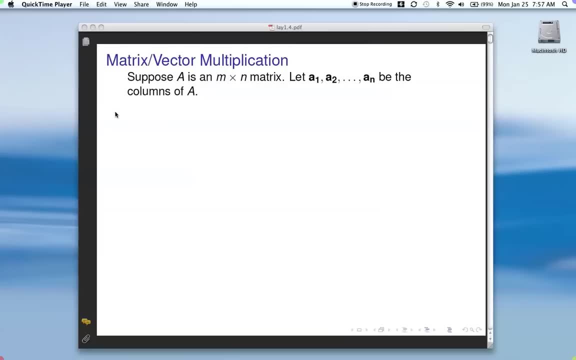 Okay, so these two vectors in our three generate a plane. Okay, we're going to start off uh Today talking about uh, multiplying a matrix, uh with a vector. So some terminology there. um, let's suppose that we start off with an m by n matrix a. 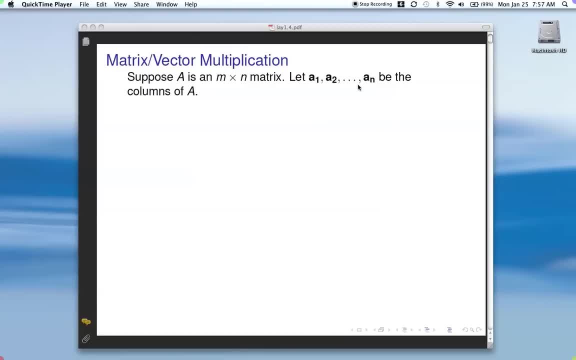 And we're going to let a1,, a2, through a n, be the columns of a. okay, So each of these is is a column vector and not a scalar. okay, Each a sub, i is a vector. Okay, So our m. since there are m rows in a, each column would have m entries. 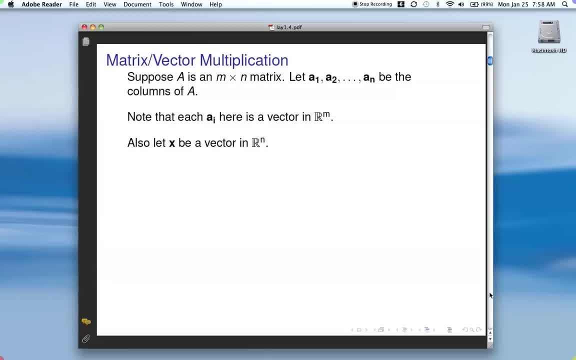 And, uh, let's let x be a vector in our n. Then the product of a and x is computed as shown here. okay, So here's a. and remember, each of these is a vector. okay, a column of a. Here's x. 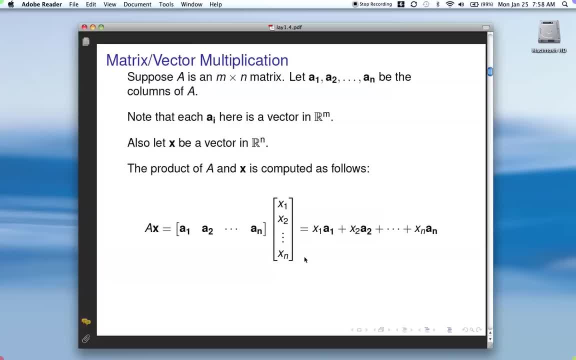 And so to compute a times x um, Basically we just match up um the components of x with the columns of a. So we end up with x1 times a1, plus x2 times a2,, plus out to xn times a n. 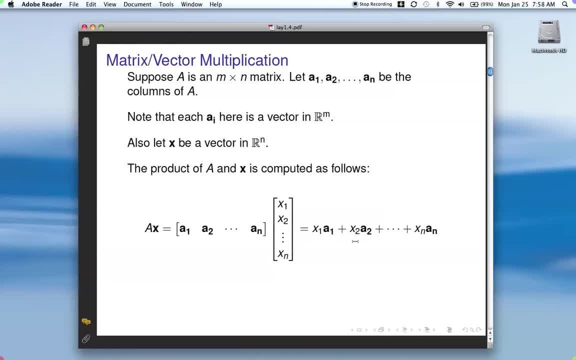 You'll recognize this as a linear combination of the columns of a. okay, So here's the deal. A- x is a linear combination of the columns of a, using the corresponding entries in x as the weight. Okay, So here's the deal. 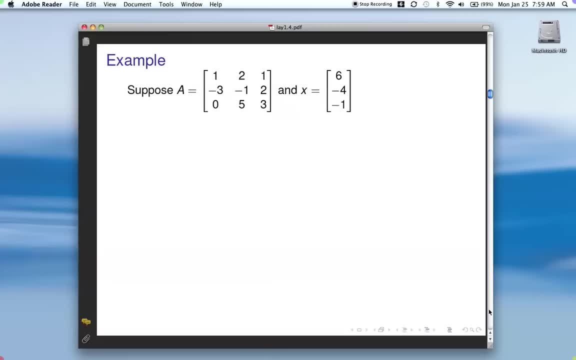 A. x is a linear combination of the columns of a, using the corresponding entries in x as the weight. So here's an example. Here's a matrix a and a vector x. Uh, then, to compute a times x, um, we've got the first entry in x times the first column. 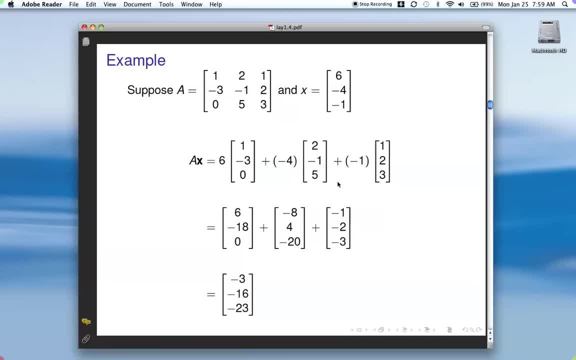 of a plus the second entry in x times the second column of a, and then plus the third entry in x times the third column of a, And we did a scalar multiplication. add them together and here's our result. All right, so notice what we have. 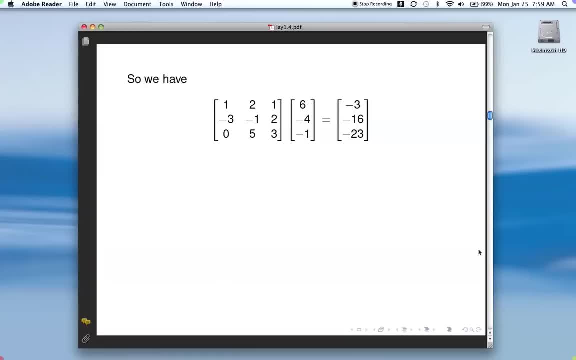 Here's a matrix times a vector and we get this vector, or another way of looking at it. here's a linear combination of, uh, the columns of the matrix, um yielding the same vector clearly. And then here's another way to look at it: um, if we um looked at this augmented matrix. 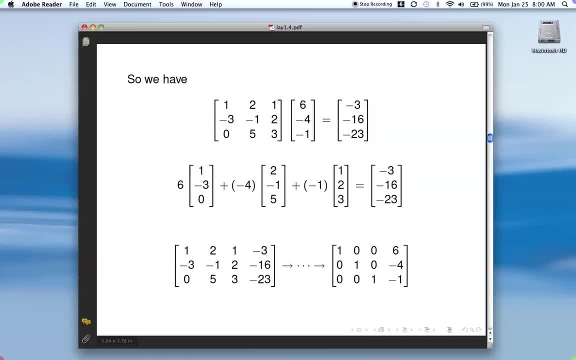 okay, so this is a here, the coefficient uh matrix a, with, um, this vector augmented onto the right-hand side. okay, so, um, we essentially have the uh, the augmented matrix here that corresponds to this system. 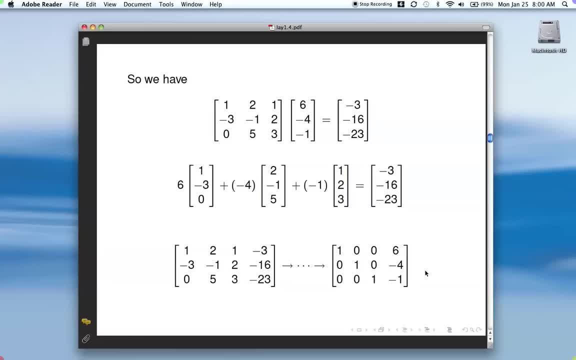 So if we put it in uh reduced echelon form, which I have here, notice that we get what we think we should get right. The solution to the system, The solution to the system is just the vector x that we started out with up here. 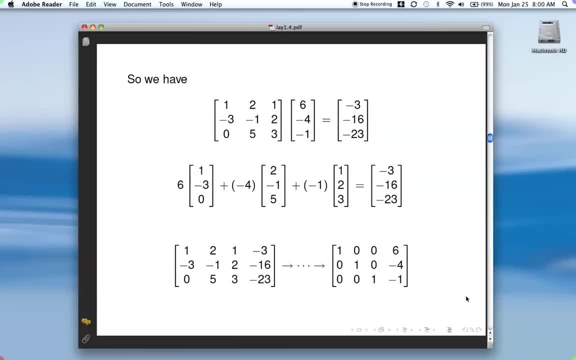 So these are three different ways to look at the same uh system. So let's uh formalize that idea. So if we have uh a, matrix a, that's m by n, with columns a1, a2 to an, and uh b is: 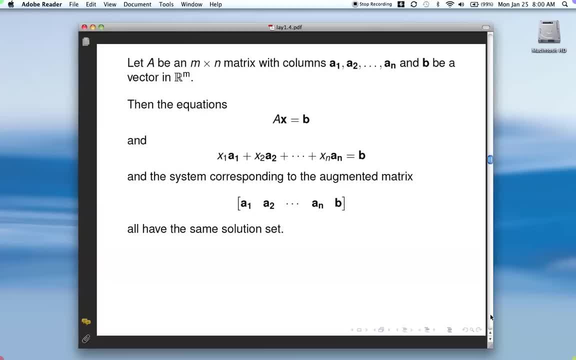 a vector in rm. Then these uh equations: ax equals b and this linear combination of the columns of a set equal to b and the system corresponding to this augmented matrix. we got all the columns of a with b tacked on the augmented uh column. all have the same solution set. 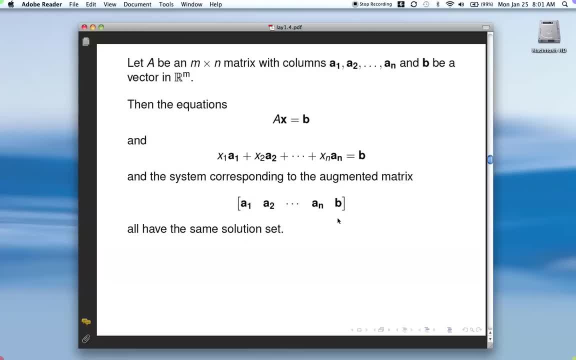 So these all essentially mean the same thing. They're just different ways of looking at the same problem. So notice that the equation ax equals b has a solution if, and only if, b is a linear combination of the columns of a. And since these are all equivalent, this is a linear combination of the columns of a. that 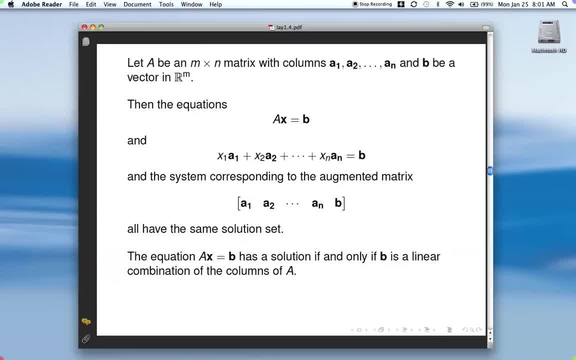 we're setting equal to b, So if that has a solution, that means ax equals b has a solution. And another way of stating that is that ax equals b has a solution if, and only if, b is in the span of the column of a. 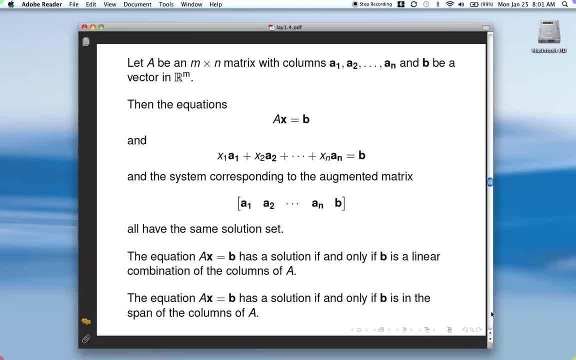 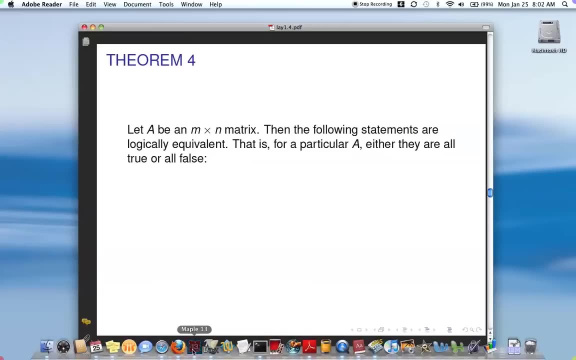 Okay, Okay. So if b is a linear combination of the columns of a, that means b is in the span of the columns of a. Okay, We're going to um, move over to um, a Maple session. uh, at this point, um, because it's. 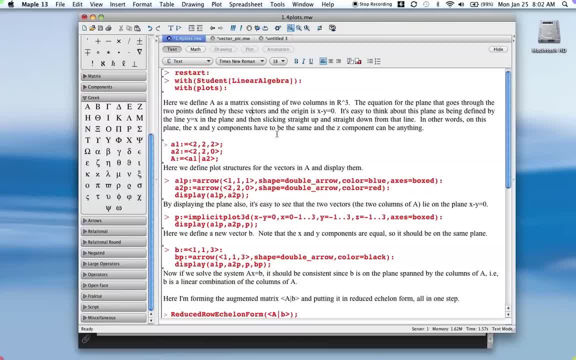 uh, easier to show you some of this with some of the graphics that Maple, uh lets me use, And so, um, also give you a little, Um, uh, a little lesson in using Maple as well. So, um, I'm loading here, uh, the uh uh student linear algebra package and the plots. 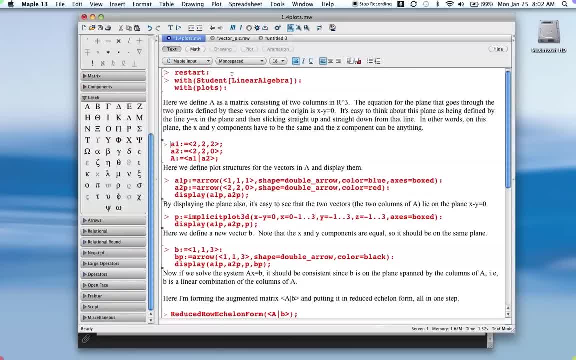 package. And then, um, I'm uh defining two vectors here, uh, a one and a two. and then I'm, I'm creating with this command: Um, a matrix, Um, a matrix, a, uh, whose columns are the vectors a one and a two, um, so you see the 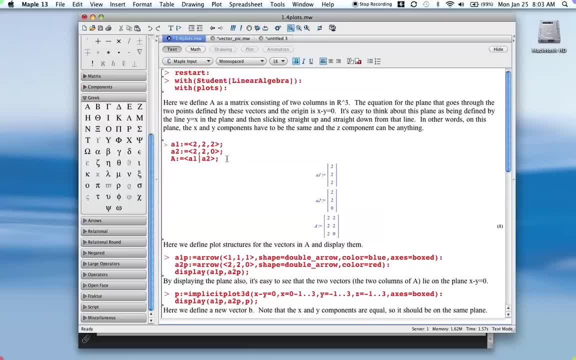 the output that you get from that. um. I'm defining these vectors, um, because I want to look at the plane that they lie on And um, as I explained here, um, this plane is, uh, uh, defined by this equation: um. 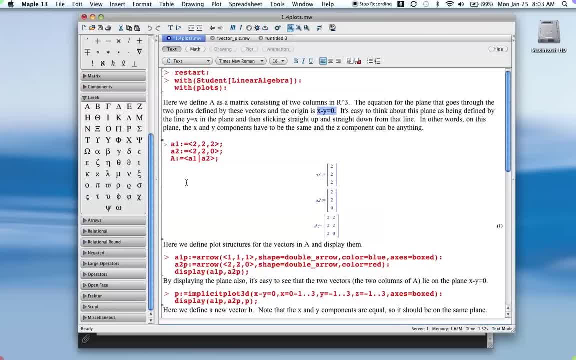 X minus Y equals zero. Okay, So notice that both of my uh uh vectors here have uh. X minus Y equals zero, and Z can be essentially whatever it wants to be, And so what that amounts to is a plane that, uh, if you think about the line, Y equals X. 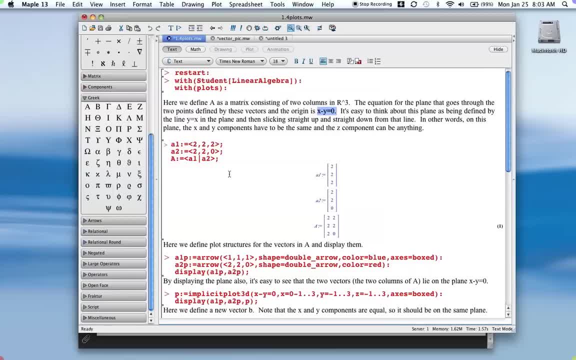 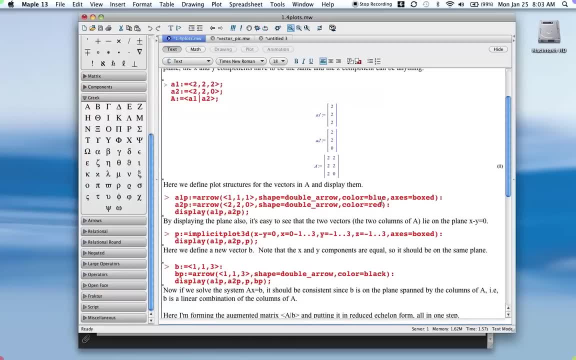 in the plane, uh, so it's kind of defined by that line and then just straight up and straight down from that line. So, um, let's uh come back. Can we get a picture? here I'm defining uh plots so that we can see what these look like. 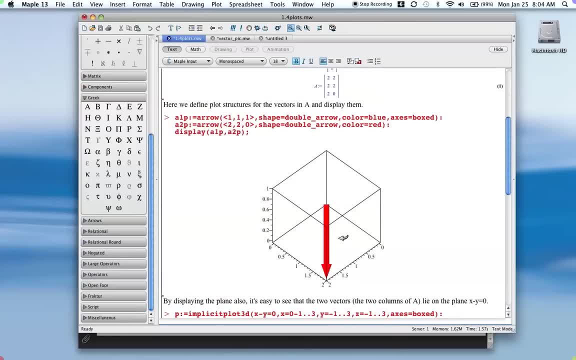 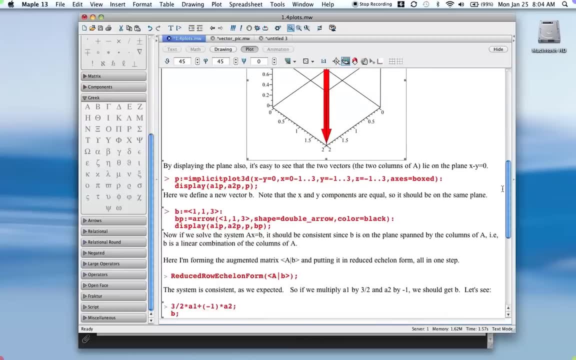 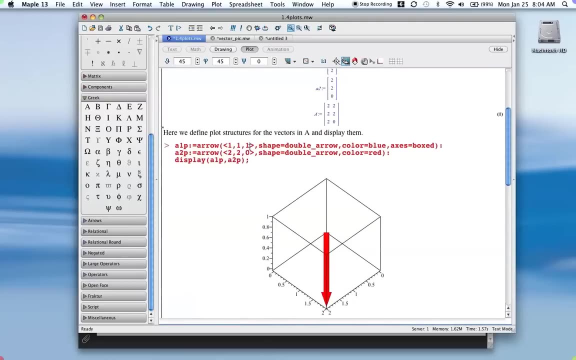 Okay, So uh, uh, let's see. oh, it looks like I've uh changed this. just, uh, let me change this. This is supposed to be two, two, two. really doesn't matter, but just to be consistent. 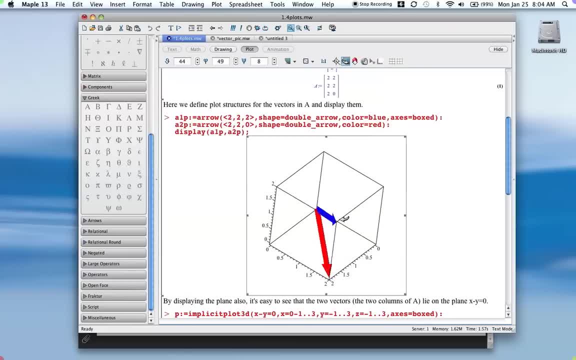 make that change. Okay Then, um, so here's what, uh, those two vectors look like. you know, let me kind of rotate this to make it look like what I want Basically. if you look, you can kind of see that, uh, they lie on the same plane. um. 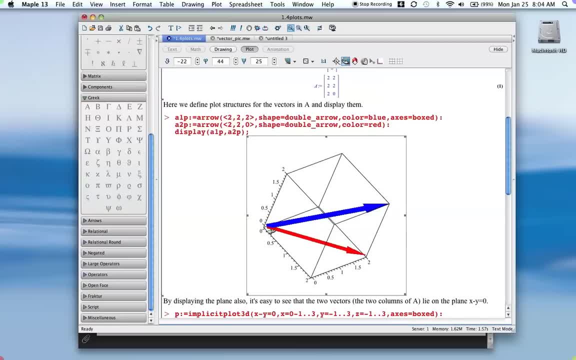 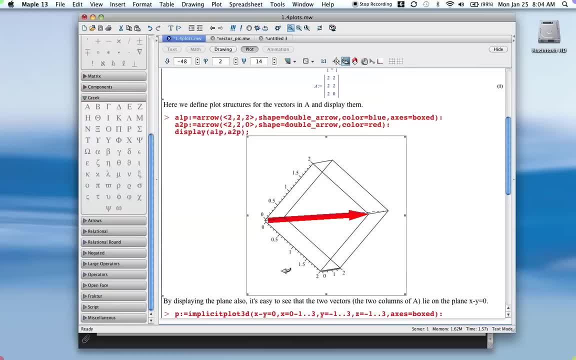 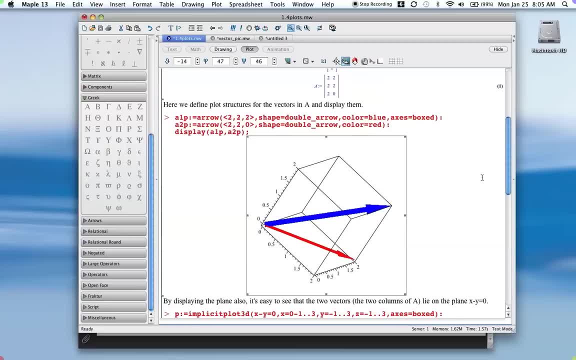 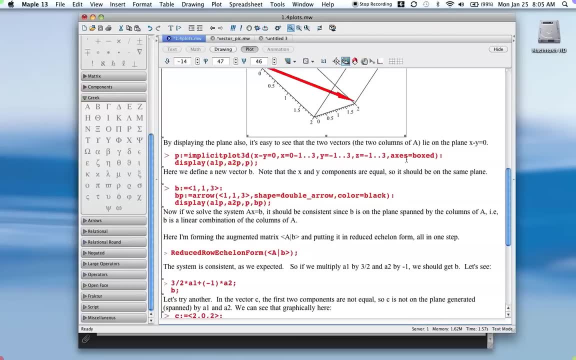 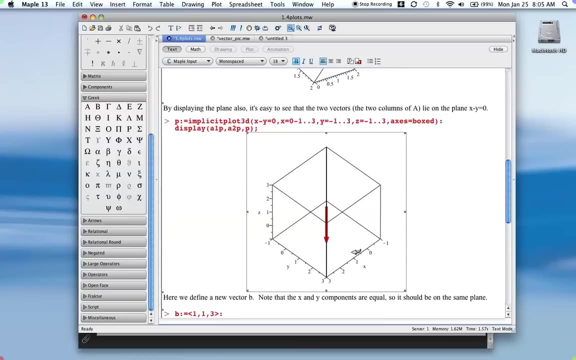 Y equals X, So they both lie on that line. Um, it's easier if you look at the plane, uh, also, and you, and then you can see the vectors as well. So let's do that here: You can see the plane and you've got the two vectors that are lying on that plane. 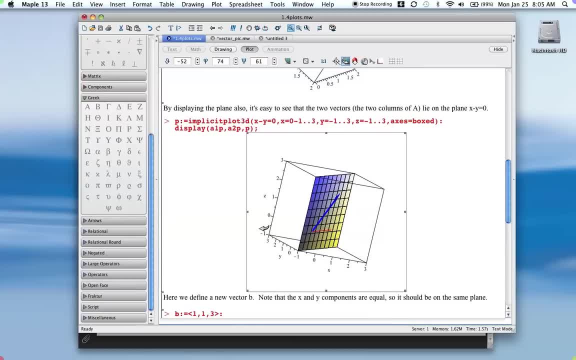 So you can see here's the x-axis this way, y going this way and z's up and down. You can see there's the plane and looking from up above, you can see that we're cutting across on the line y equals x. 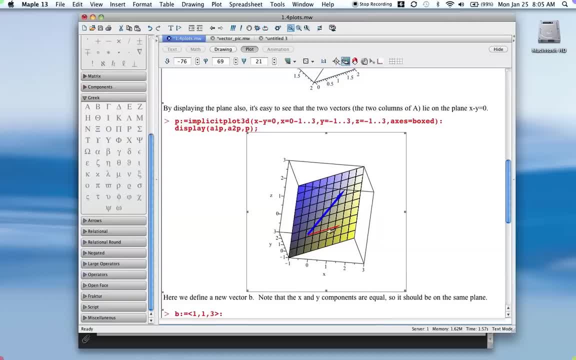 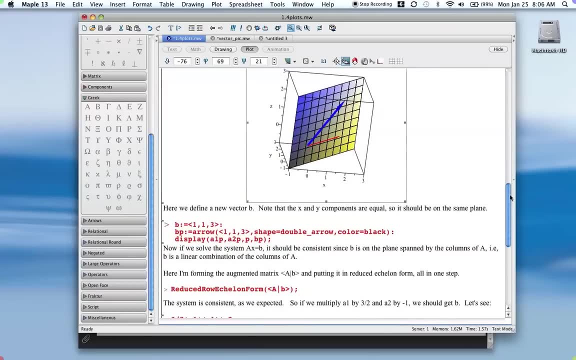 And both those vectors lie in that plane. So if we look at any other vector in that plane, any other vector where the x and y components are the same, it should lie on that plane. So I've defined a new vector at 1,, 1,, 3.. 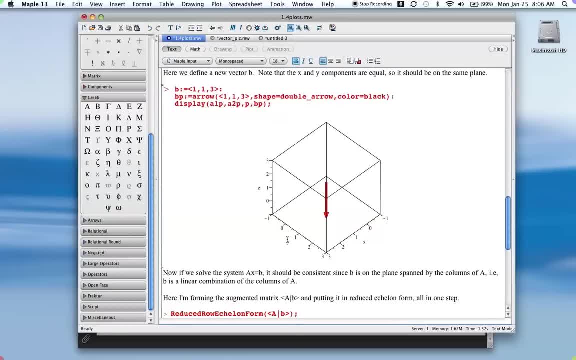 And then I've plotted it on this same set of axes, and so if you look- let's look at it like this- there you can see the new one- 1, 1, 3- I made it black so you can see it here- and then, looking at it from above again, you can see that those are all on. 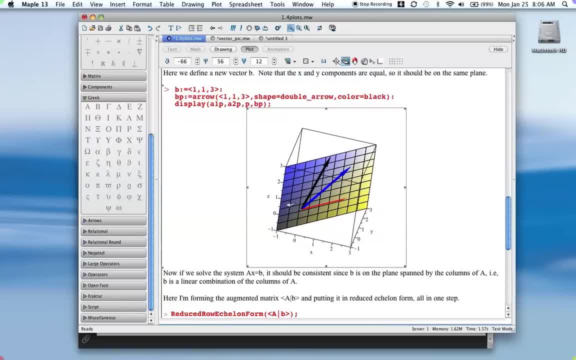 the same set of axes or same plane. so all those lie on the same plane. so that means that B here is in the span of the original two vectors that we started out with, or it's a linear combination of the two vectors we started out with. so if we 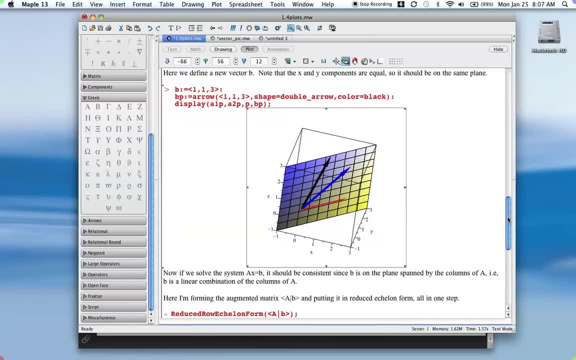 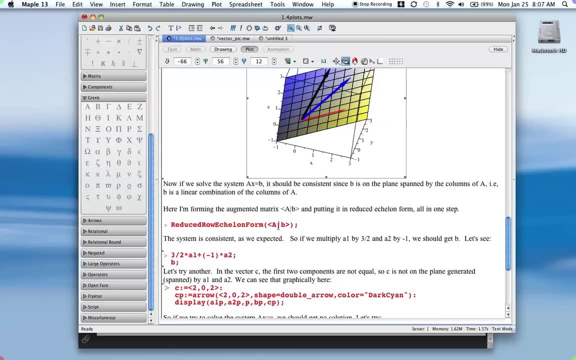 solve the system: ax equals B. it should be consistent. so that's what I'm doing right here. I'm forming the matrix. you can see that I'm giving the matrix an augmented matrix here. so I've got my matrix a and then I'm augmenting on the new vector B here and all on the same. 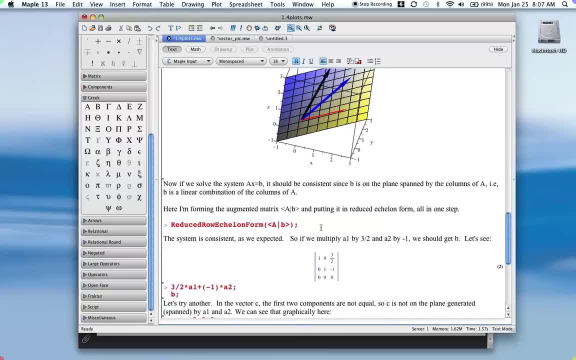 command, I'm reducing that matrix to echelon form: a row, echelon form, and here's what we get. okay, clearly, this system has a solution, because we have no rows, we're, and then something, not zero. you can see we've got a row of all zeros, but that's okay. 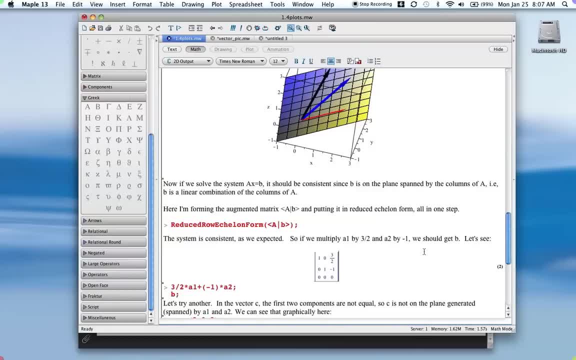 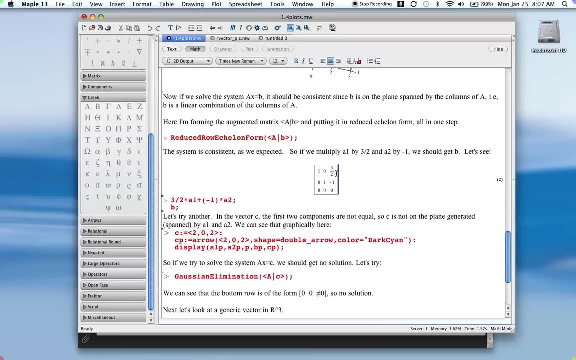 And in fact we have a unique solution because there's no free variables And the solution says that x one is three halves, x two is negative one. so if we take that linear combination, okay, three halves times the first column of A, plus negative. 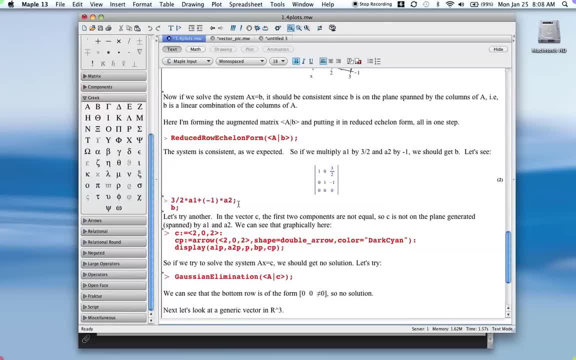 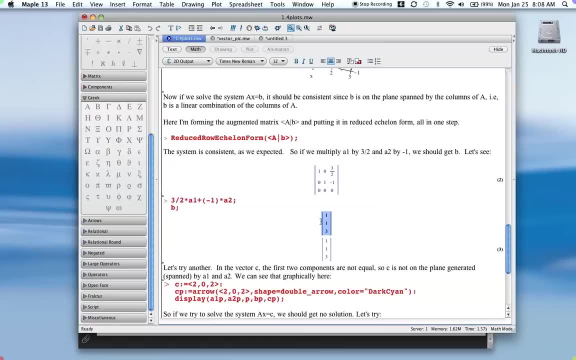 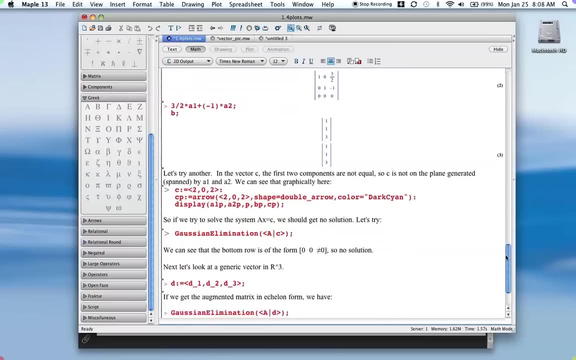 one times the second column of A, we should get B, because that's the system we just solved. So, if you look, indeed, this is that linear combination here and this is B. All right Now, looking ahead, if we choose a vector whose first components are not equal, then it should. 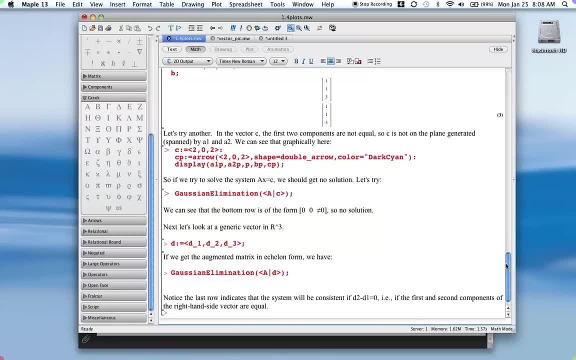 not be on that plane, and if we solve the system with it on the right-hand side, we should get no solution. So let's get B. Let's give that a try. So I create another vector C, which has the x and y components are not equal. all right, 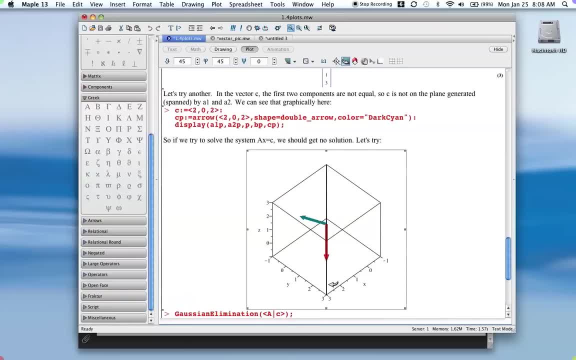 and I plot it in. So here's that vector. give it a view on that. there you can see, there, there, that's a good view, right there You can see. this new vector is the cyan-colored vector. This is the cyan-colored one. 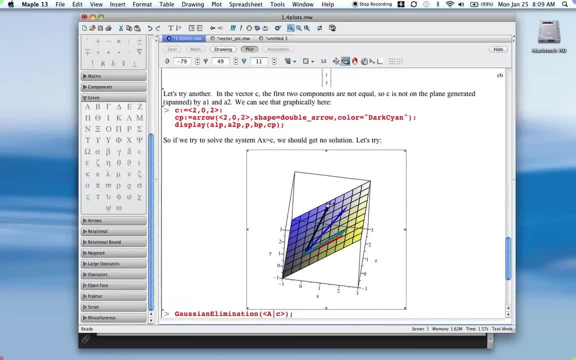 And clearly it's not on the plane that the other three vectors lie on. All right, It's coming off off the plane. So that means that it is not in the span of the other three, So it's not a linear combin- I mean of the other, well, the other three, but really we're 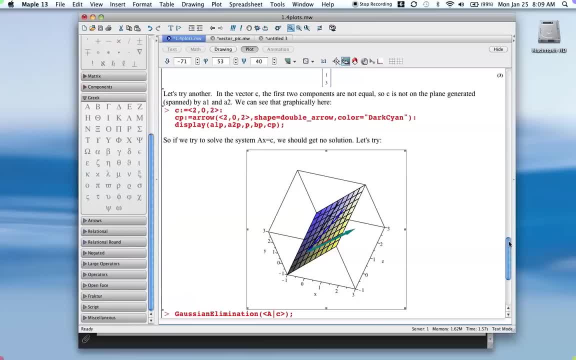 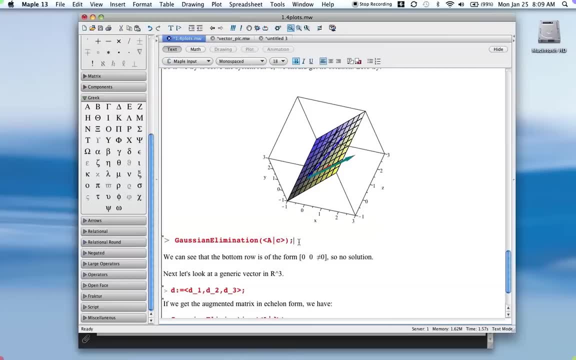 only interested in the other two. It's not a linear combination of the columns of A. So if we solve the system with C on the right-hand side, then here's what we end up with. Okay, so I didn't get it in reduced echelon form. 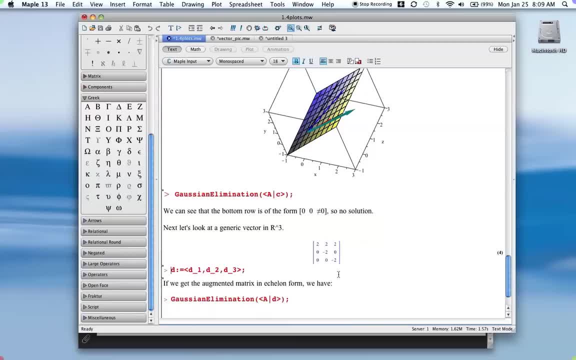 I wanted to leave it like this. So this is just echelon form. But notice the third row. you got 0, 0, and then negative 2. So 0, 0, something not 0. So that tells us there's no solution. 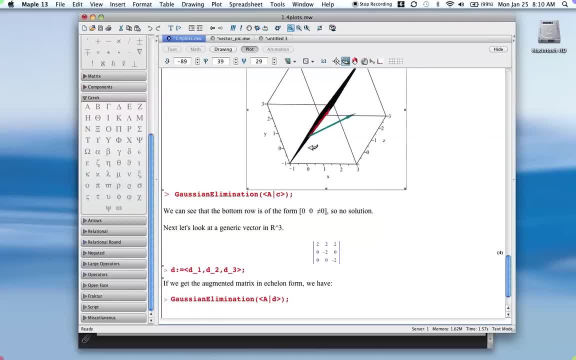 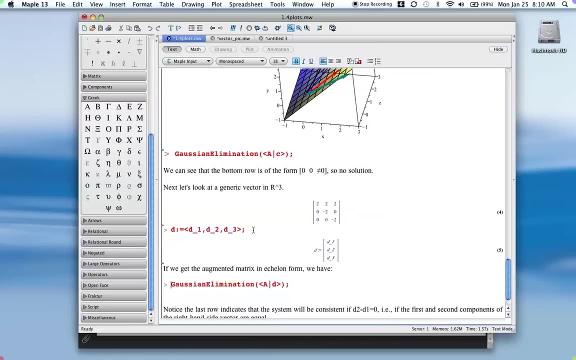 Okay, and then again, because that vector is not in the span, it's not in the space that's generated by the columns of A And one more. look, I just created just a generic vector I call D. And then let's look at the echelon form of the augmented matrix with A and D. 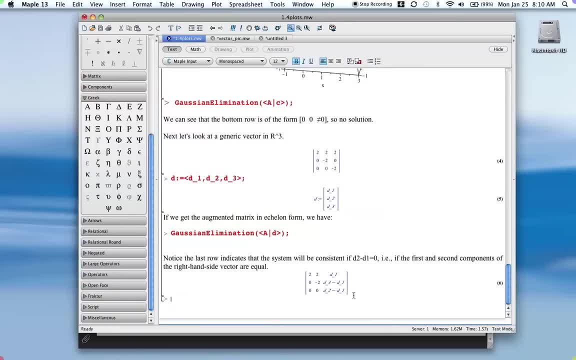 All right, so it looks like this. This is the nice thing about Maple: It does the symbolic computation, So you can do the computation with variables or parameters instead of all just constants. And so we can see. notice the bottom row: we got 0,, 0, and then something else over here. 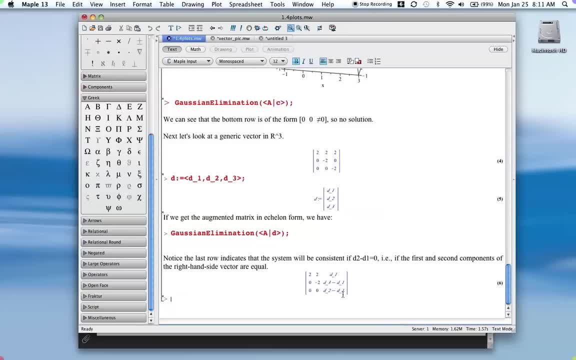 And notice what that says. It says that if this system has a solution, then D2 minus D1 has to equal 0. So if this system has a solution, then D2 minus D1 has to equal 0.. All right, because if this is non-0 over here, then we've got 0, 0, something not 0- in the augmented column. 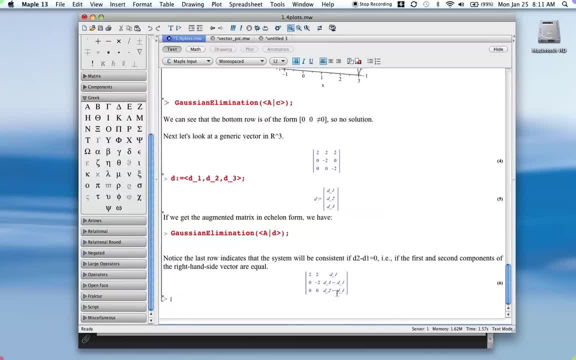 which means no solution. So for this system to have a solution, D2 minus D1 has to equal 0, which of course means that D2 and D1 are equal. And since those back up here, those are the first two components. 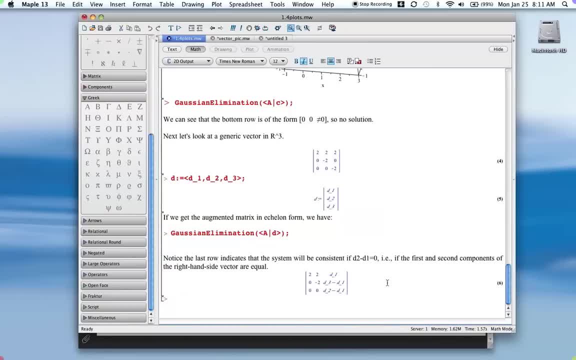 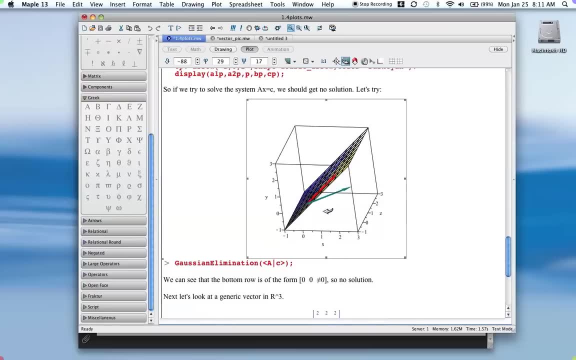 that's just saying that the X and Y components have to be equal for this system to have a solution. Or, graphically, the first two components have to be equal for this system to have a solution, Or graphically, the first two components have to be equal for the vector to lie on the plane. 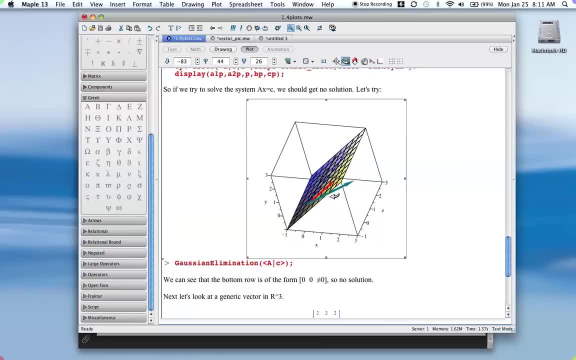 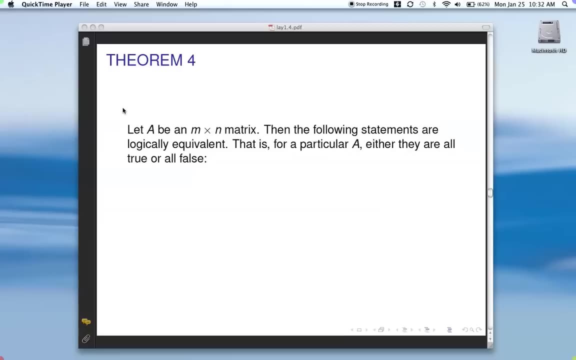 that is spanned by A1 and A2.. Okay, I'm going to stop there and we'll pick up the next slide in the next video. Okay, I want to start back here with theorem 4.. This is a very important theorem in your book, so you want to pay close attention to this one. 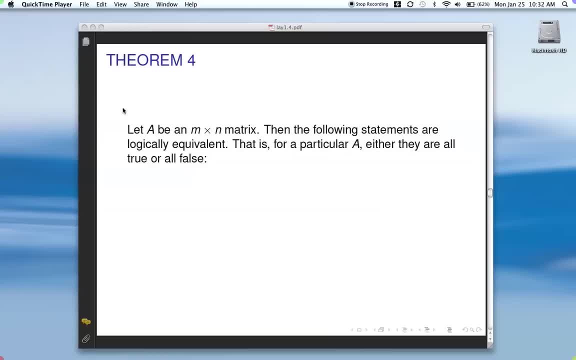 So it says: Let A be an M by N, Then the following statements are logically equivalent. That means, for a particular matrix A, either they are all true or they're all false. Okay, so that's a powerful theorem that we have here. 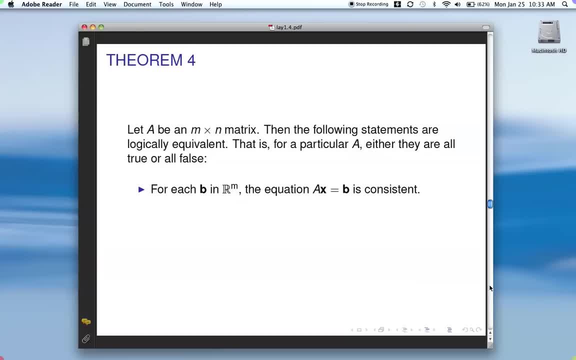 Okay. first statement is: For each B in Rm, the equation AX equals B is consistent. So that's saying, no matter what the right-hand side is for this particular matrix, A, AX equals B is always consistent. Another way to say that is that each B in Rm is a linear combination of the columns of A. 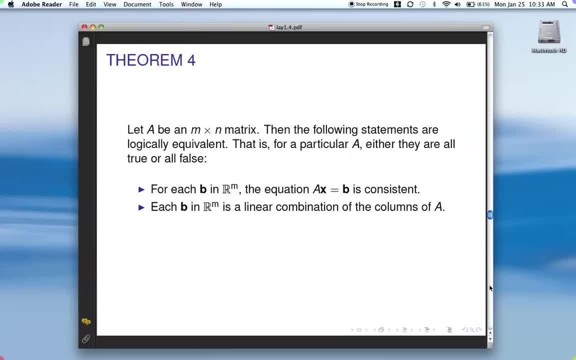 Okay, because we saw just earlier that A times X, when you multiply A times X, you're actually taking a linear combination of the columns of A. This also means that the columns of A span Rm. right, because you can produce any vector in Rm as a linear combination. 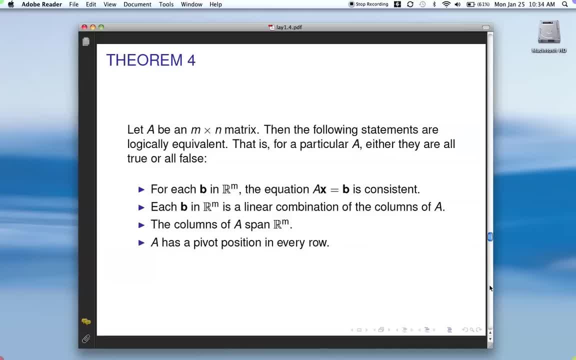 Okay, so that's the linear combination of the columns of A, And then down to the nitty-gritty. how you actually determine whether this is true or not is by putting A in echelon form. and these are all true if A has a pivot position in every row. 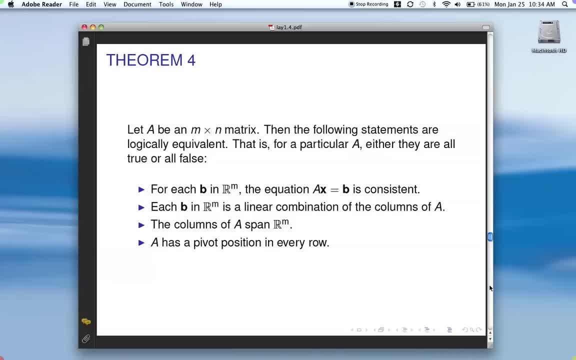 So we saw that in the last in the Maple demo. Okay, if there's a pivot position in every row of A, that means of the column, if there's a coefficient matrix, then there's no way the system could be inconsistent. 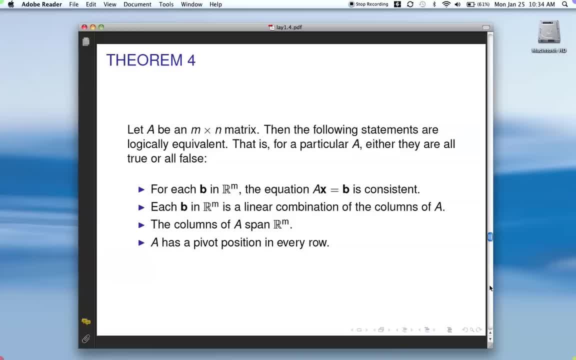 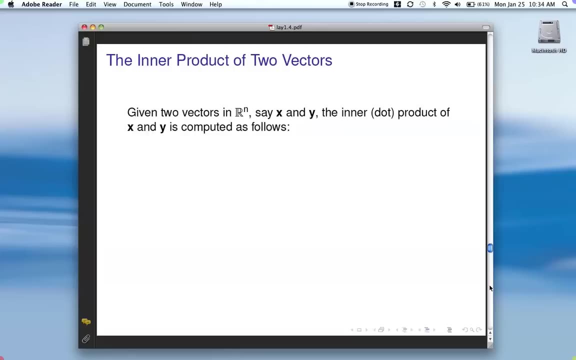 because you could never have a row of all zeros and then in the augmented column something non-zero. Okay, we're going to look at one other way to compute A times X, But first we're looking at the inner product of two vectors. 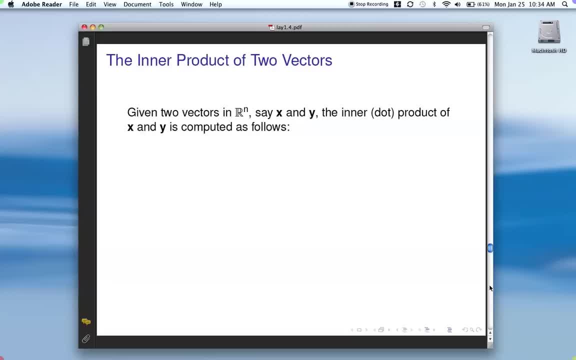 because we're going to use that. So if we're given two vectors in Rm, say X and Y, then the inner product, which is also called the dot product, of X and Y is computed as follows: Okay, it's just X1 times Y1 plus X2 times Y2, plus so forth, plus Xn times Yn. 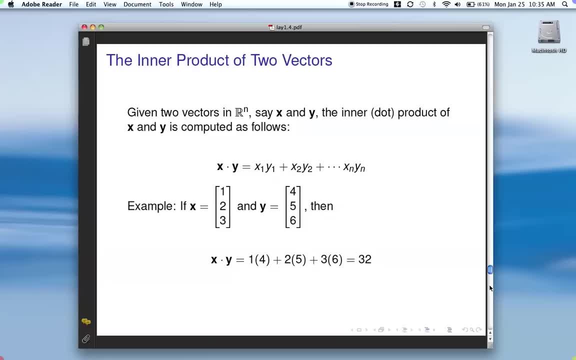 Okay, so just multiplying like components and adding them up. So here's an example: We've got: X is 1,, 2, 3,, Y is 4,, 5, 6.. Then the inner product of Y is 1,, 2,, 3,, Y is 4,, 5, 6.. 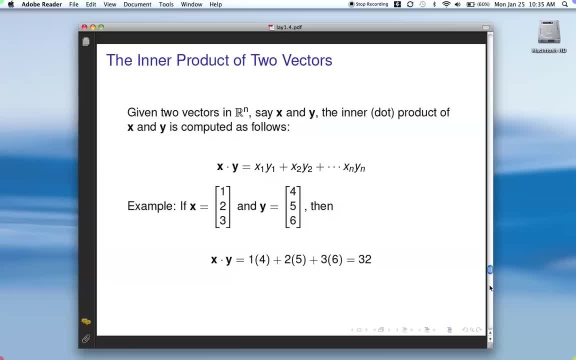 Then the inner product of X and Y, or X dot Y, is 1 times 4 plus 2 times 5 plus 3 times 6.. Okay, so now let's talk about two ways we can compute A times X. We already looked at one of these. 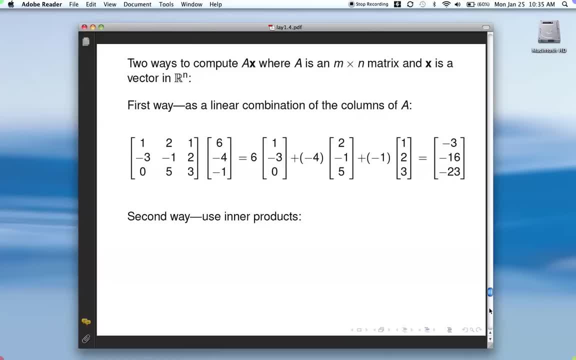 That's by taking a linear combination of the columns of A. So here's an example: to compute the product of this matrix, A times X, Then we take the first element of X and apply that to the first column of A, Then second element negative 4, times the second column of A, and so forth. 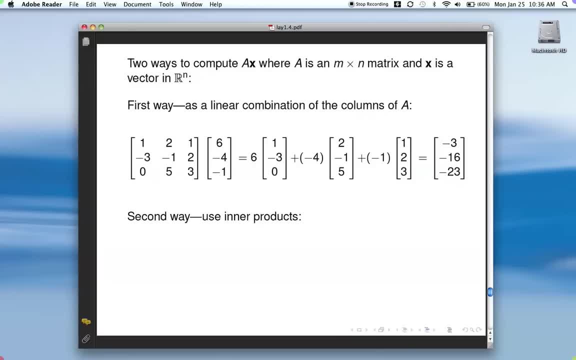 So we generate this linear combination and end up with this vector. Now the second way. we use inner products And the ith element of the inner product, the ith element of AX, is the inner product of the ith row of A with X. 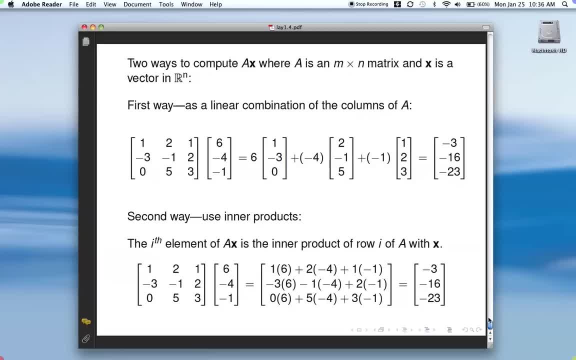 Alright, so looking at that, you look at to get the first element here, the negative 3, then it's the first row of A inner product with X. So that's going to be 1 times 6 plus 2 times negative 4 plus 1 times negative 1.. 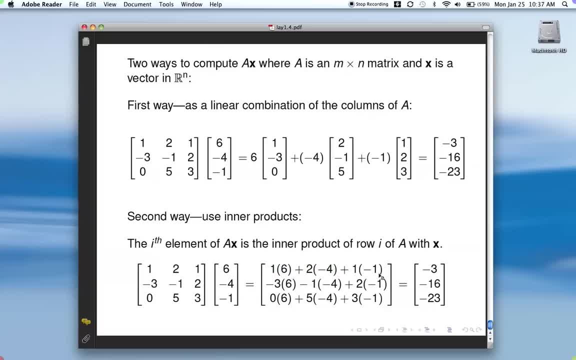 Which is what we have here in this first element here. Okay, then, to get the second component of A times X. it's the second row of A inner product with X, So negative 3 times 6 plus negative 1 times 4 plus 2 times negative 1.. 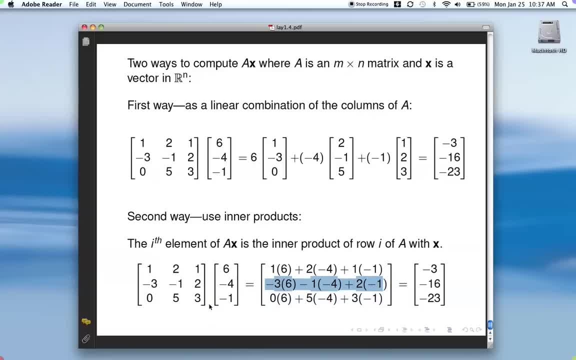 Okay, as we see here Then, to get the third element, it's the third row of A inner product with the vector X. okay, So those are two different ways you can compute the product of a matrix and a vector. For the most part, we will use this method: the linear combination of the columns of A. 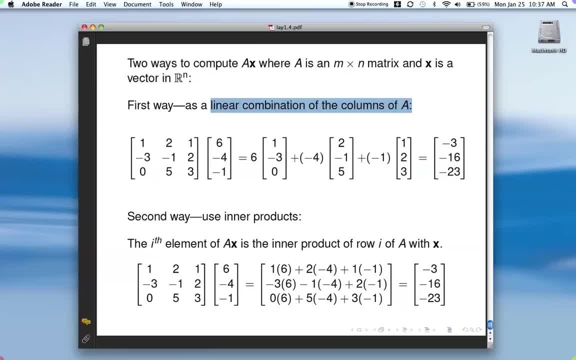 just because that fits in with the way I want you to be thinking. However, this method down here is probably quicker, So if you just need to compute the product of a matrix and a vector, you might want to just use this method, Using the inner product method, just because it's faster. 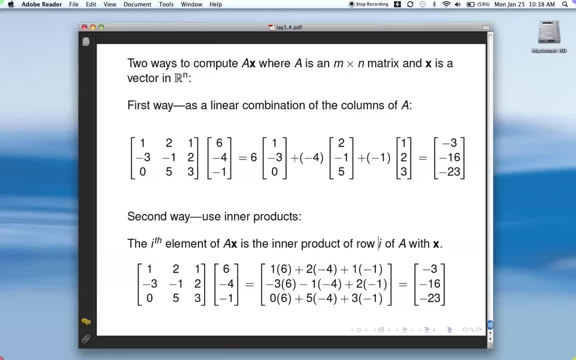 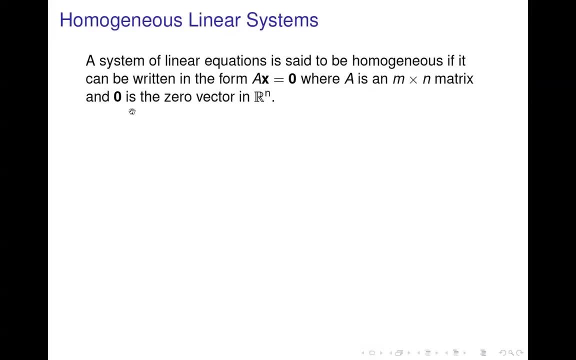 So you should practice both, just to make sure you know how to do each of these methods. Okay, and I think that's it for this lesson, Alright, so today we're going to talk about homogeneous linear systems, And a homogeneous linear system is simply one in which the right hand side is the zero vector. 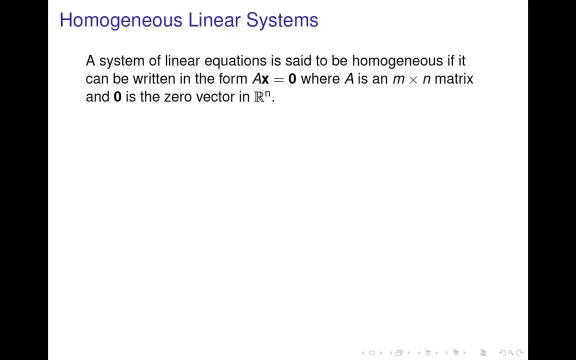 The zero vector is just a vector, It's the vector of all zeroes. So here's another way to look at it. We look at A times X as a linear combination of the columns of A, as in here: X1, A1, plus X2, A2, plus dot, dot, dot, Xn, An. 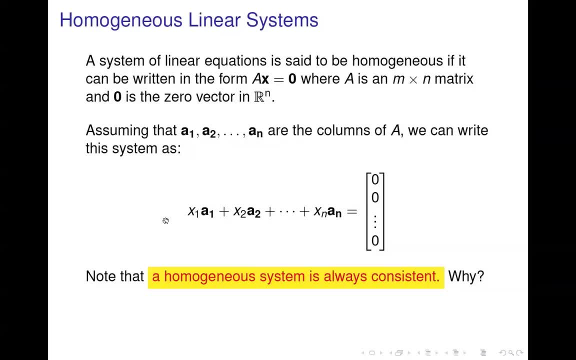 And we want that to equal the zero vector. Now, how can that happen? Well, if you look at it a little bit, it's pretty clear that if you set each one of these X values equal to zero, then you did a linear combination. 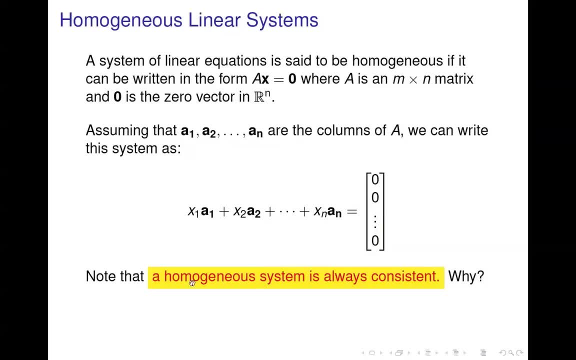 and you'll end up with the zero vector. So therefore, a homogeneous system is always consistent. X equals zero. okay, all X values equal to zero is always a solution. And since it's always a solution, and it's obvious that it's a solution- 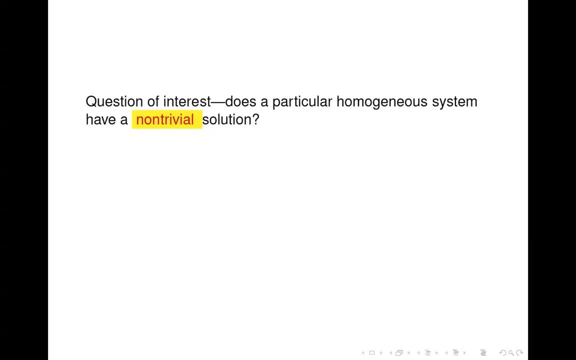 we call it the trivial solution. So we know that the system's consistent. And so, if you think back to the two questions that we ask when we're solving a system, the first one is: is it consistent? So now we know this one is. 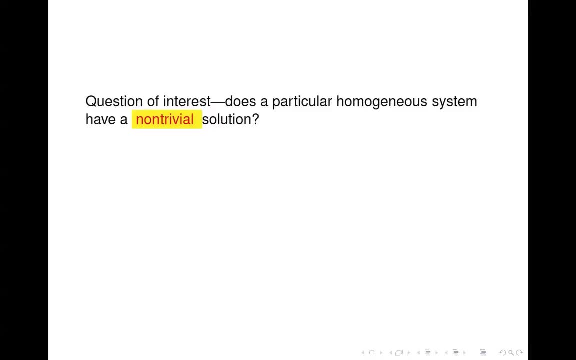 So we move on to question two, which is okay. is the solution unique or are there an infinite number of solutions? So in our case, if the solution is unique, that means you only have the trivial solution. So what we want to know is: do there exist any non-trivial solutions? 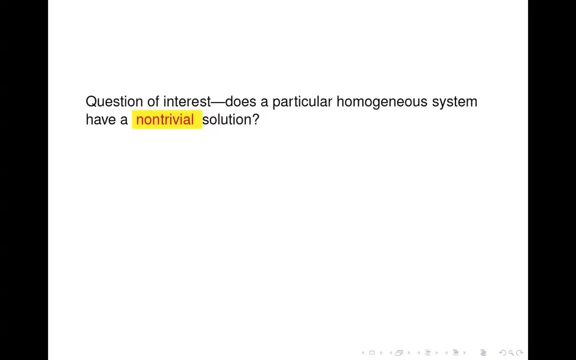 Okay, is the solution set an infinite set? Well, the answer is just like it would be for any other system: You'll have non-trivial solutions or you'll have an infinite number of solutions if, and only if, your system of equations has at least one free variable. 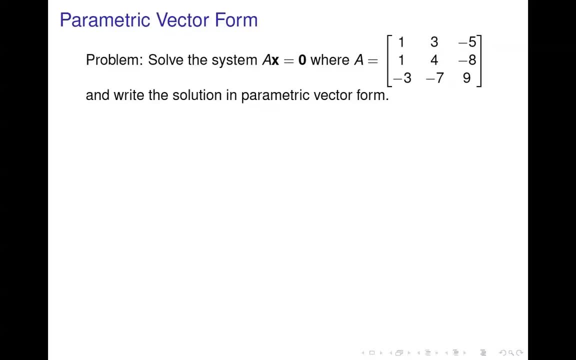 So we're going to look at a system here and solve it, And we're going to write our solution in parametric vector form. So that's that's something that's new in this section. All right, so here's the system. 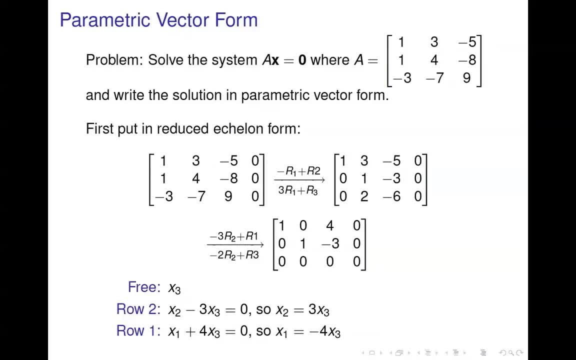 We want to solve. x equals zero. So we put it in an augmented matrix and tack on the column of zeros and we do some row operations and notice that I have put my augmented matrix in reduced echelon form. not just echelon form, but reduced echelon form. 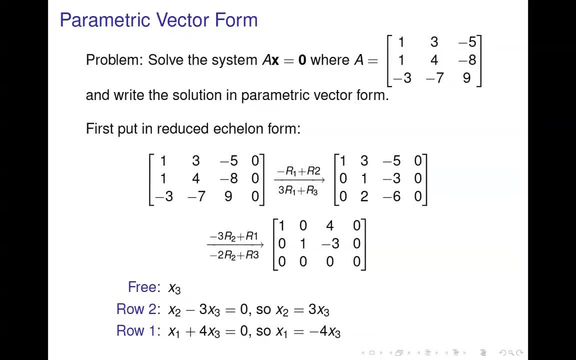 And that is because that makes it easier to not only write the solution in general form, but it makes it easier to write it in parametric vector form. So anytime your system has an infinite number of solutions, then it tends to be easier to write out the set of solutions if you put your matrix in reduced echelon form first. 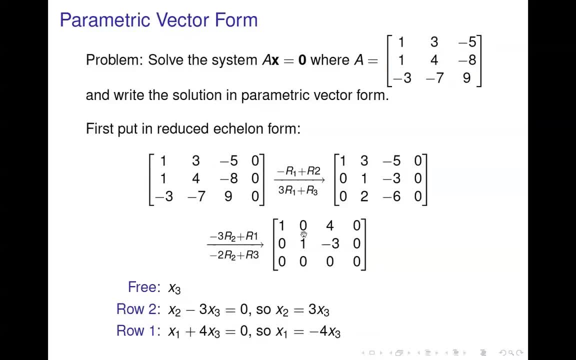 So looking at this matrix here you can see that x one and x two um they're pivot columns in the in the x one and x two columns, pivot positions in the x one and x two columns. So those are basic variables in the x three column. 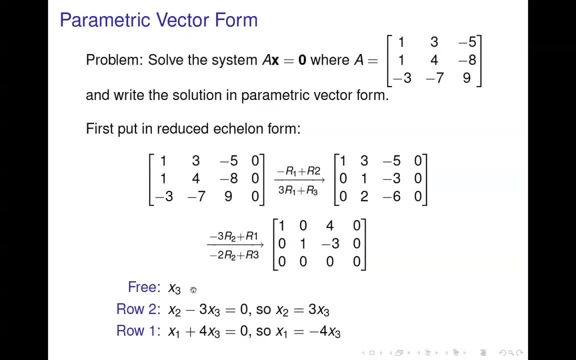 We have no pivot position. so therefore, x three is a free variable. okay, So that means we've got an infinite number of solutions, or this homogeneous system has non-trivial solutions. So what do they look like? Well, we can, uh, look at the second row and we get that um x two. it must be equal to 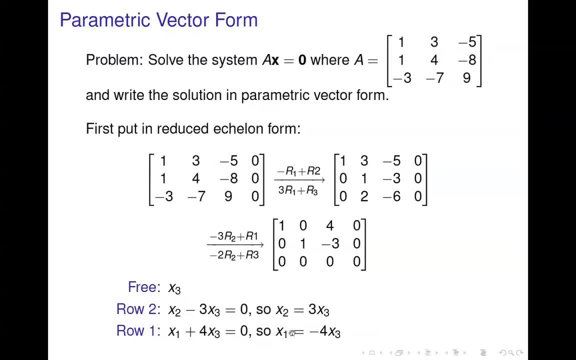 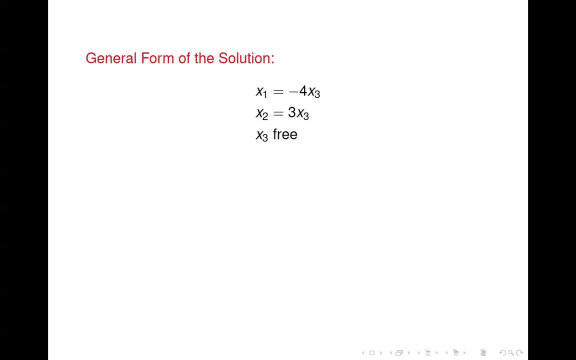 three times x three and uh, x one is going to be equal to negative four times x three. So we can write the general form of the solution as it's given here: X three is free, x one and x two are written in terms of the free variable. 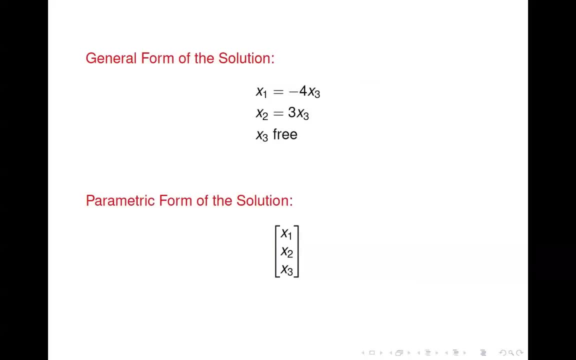 Now to get the parametric vector form of the solution. we start off with just a generic solution vector and basically just uh, copy down the general form of the solution. So this, uh, what you see here, comes straight from looking at the general form of the solution. 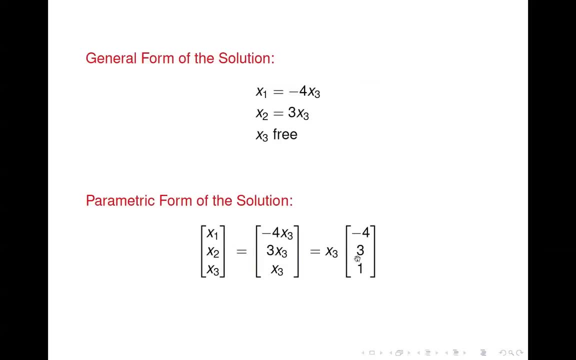 And then to write it in parametric vector form, we simply factor out the parameter. In this case, x three is the parameter, because we can set x three to be whatever we want in order to generate, uh, as many solutions as we want. 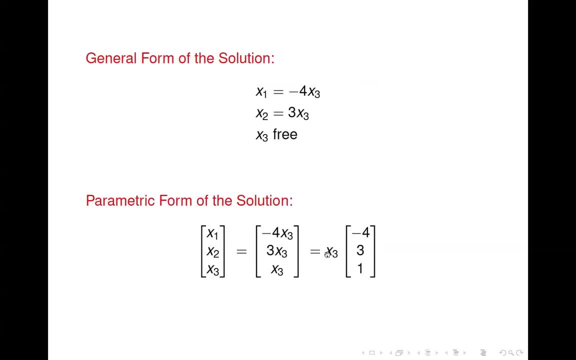 So we have it now in parametric vector form. Here's our parameter and here's our vector, Um. you should note that if you have more than one free variable, then you're going to have more than one um parameter and um vector when you write your solution in. 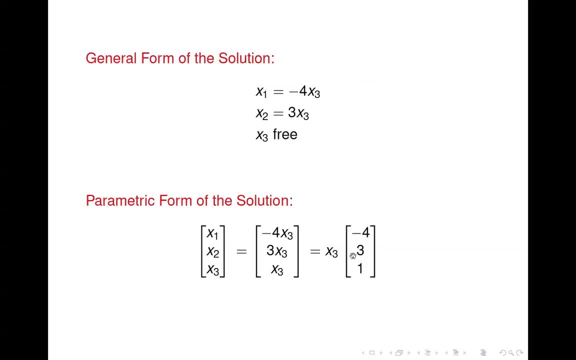 parametric vector form. So you'd have you know, if we had x four- that was a free variable- we'd have x three times this vector, plus x four times some other vector, and so forth. You'd have a vector for each. 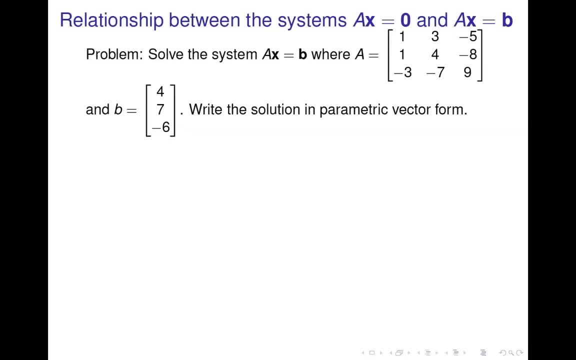 Okay, Uh, let's think about the relationship between the systems ax equals zero and ax equals b. So what we've done to this point is solved: ax equals zero for a particular matrix, a, and now I want to keep that same a and solve the system ax equals b for this vector b given. 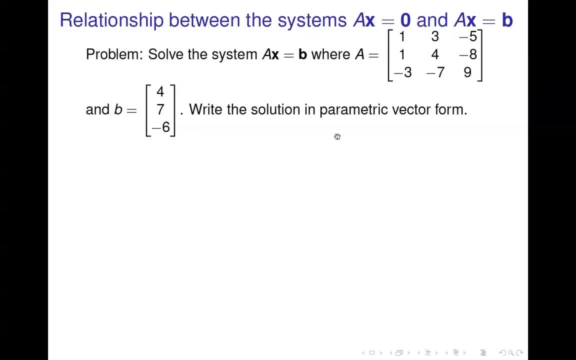 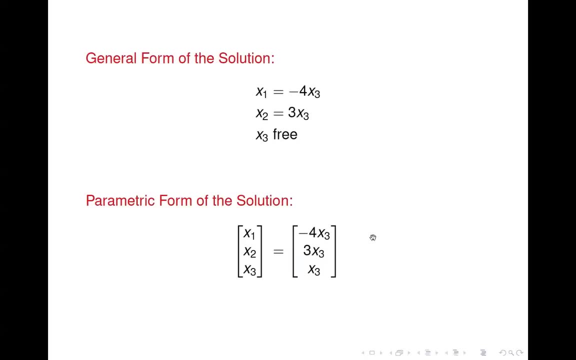 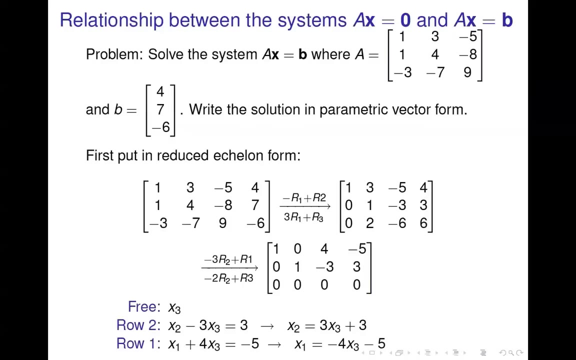 here and we'll write our solution in parametric vector form. So we approach it the same way. Here's our augmented matrix. We do row operations, Oops, sorry, Backing up. There we go, Um, we're doing row operations um to get the matrix in reduced echelon form. 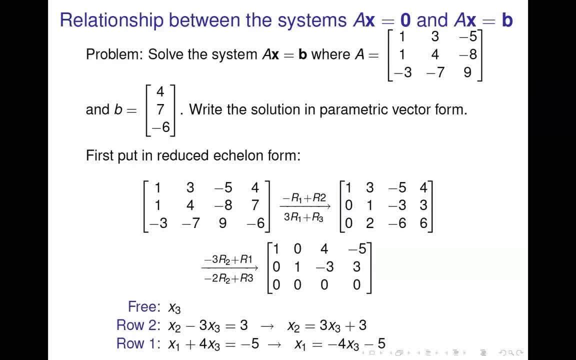 And if you want to go back and compare with: uh, what we did with ax equals zero, these are the exact same row operations And that's because they were based on what was in the coefficient part of the matrix Um, and so that hasn't changed. 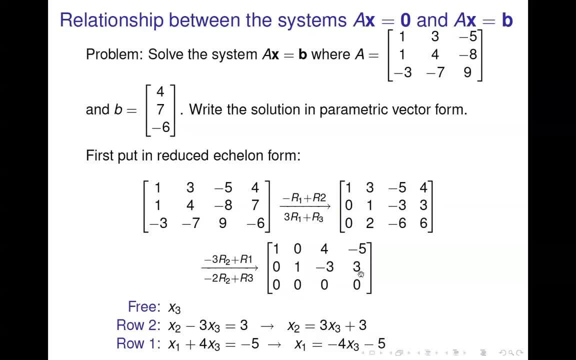 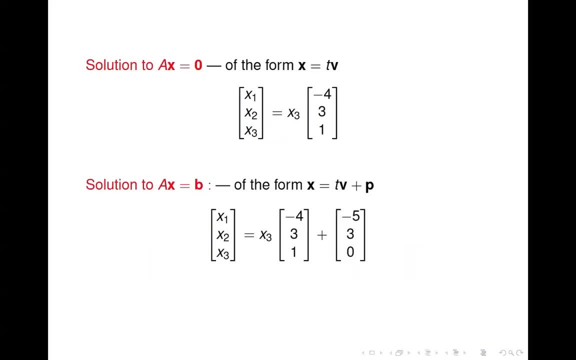 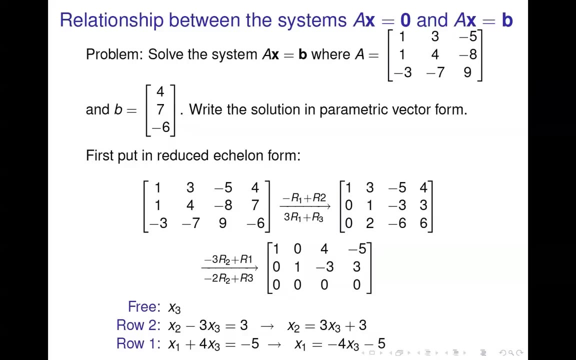 So we do the same operation. So the only thing that's changed is what's on the right hand side. Um, let me, um, whoops. I'm backing up again, Trying to get used to my mouse track pad here. Sorry about that. 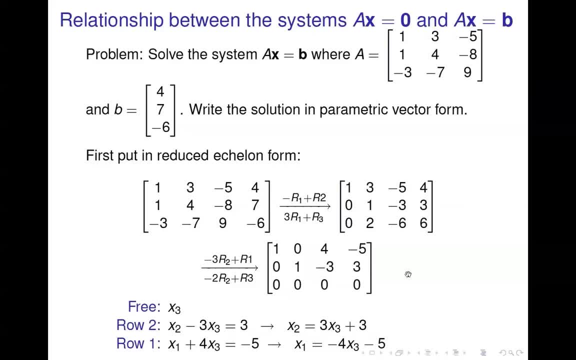 Let me point out that, um, Um, when you're solving uh, ax equals zero and you have all zeros on the right hand side, then those zeros never change, because when you do uh elementary row operations, any of those three uh elementary row operations, they will never change. 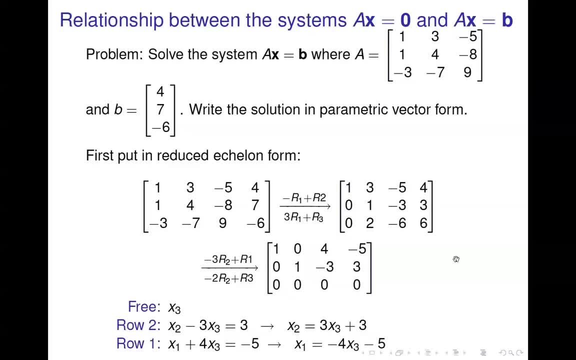 If you start off with all zeros, you'll end up with all zeros, Okay. So back to this example. though, when we um write out our solution, those X three is still free variable Um, and now X two. when we write X two, then it's uh, going to be three, the three here. 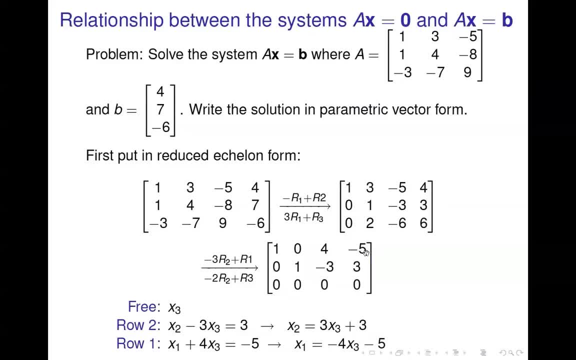 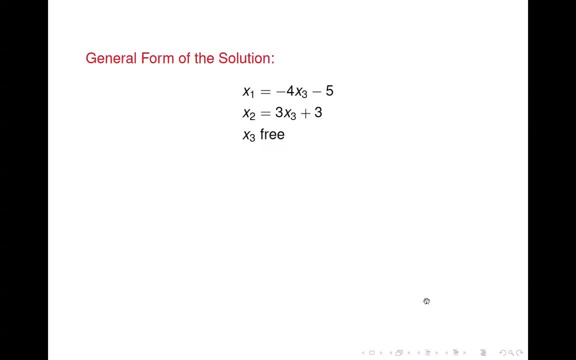 uh, plus three X three and X one is going to be negative. five minus four X three. So here's our solution, And if we just write it in general form, here's what it looks like: and um, parametric vector form. 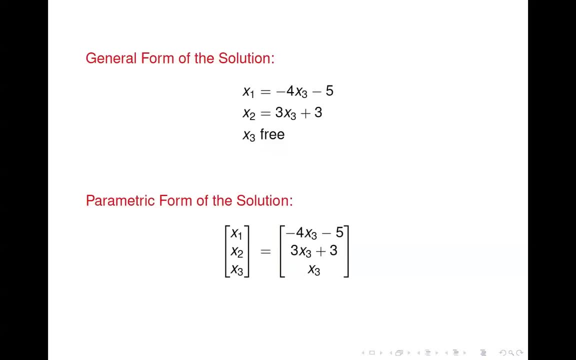 We start out just like we did previously: Right out: Uh, This is what the form looks like in a vector, uh format. And then, uh, we're going to separate out the part that involves a parameter and the constant part, and then take it one step further and uh, factor out the parameter. 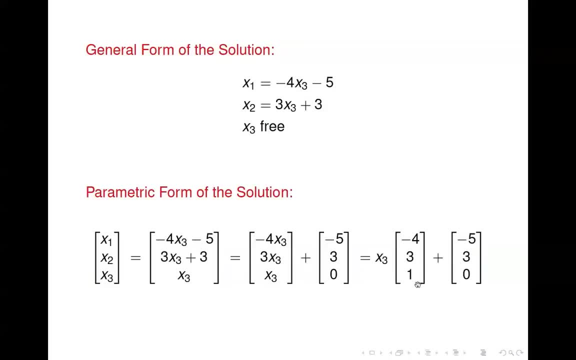 And so notice that, um, what we have here, uh, is exactly the solution that we had to ax equals zero And uh, then with ax equals b, We have that plus this constant vector. Now notice that the constant vector doesn't have a parameter associated with it. 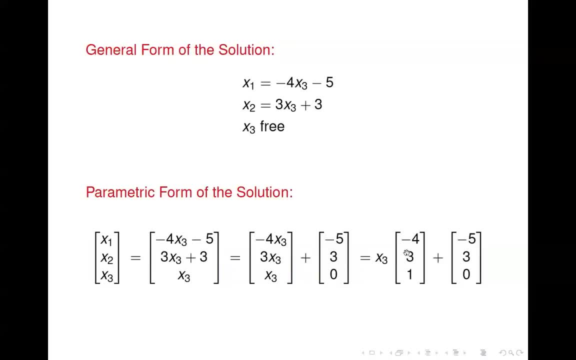 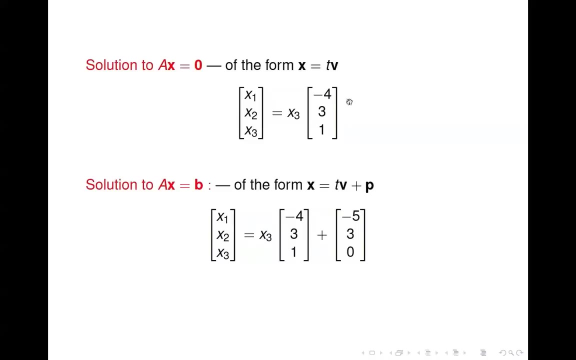 It's just constant and it doesn't change. but here we can multiply, we can set our parameter X, three to be anything, and scale this vector. Okay, So, um, in general the solution looks like this: um, here was solution to: ax equals zero. 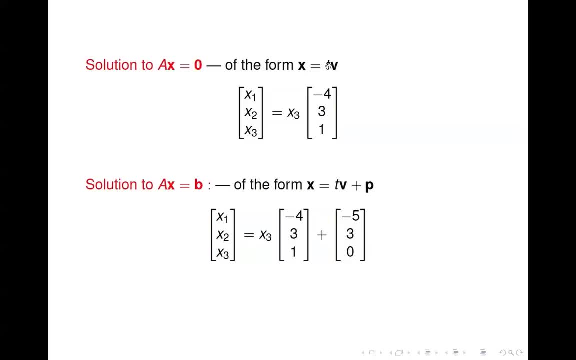 and notice that it's in this form. It's in the form some parameter T times a vector V. So in this case, X three is playing T and this is the vector V. So it's just a vector that we can scale any way we want. 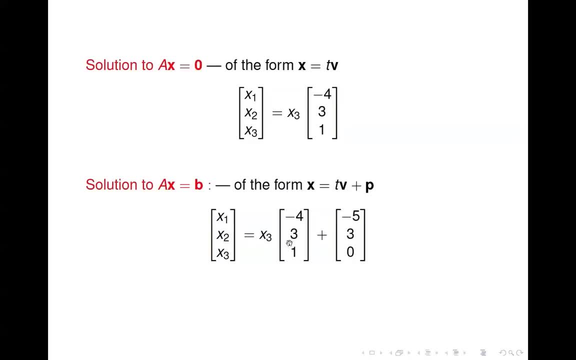 Whereas for ax equals B, you've still got the TV part right, Got X, three times this vector, but you've got this constant vector, So that's what I'm calling P. And so for ax equals zero, you just have. 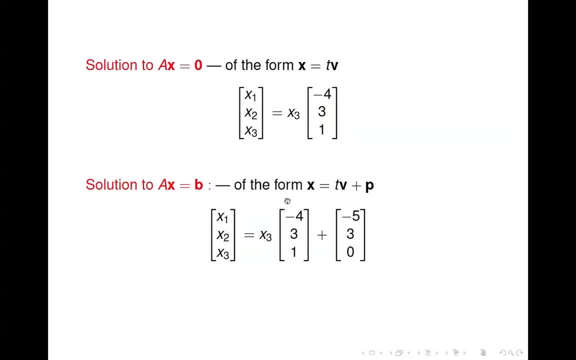 A vector that you can scale for uh. ax equals B. You've still got the vector you can scale, plus this other vector. So let's look at graphically: uh, what is going on there now for uh. for this I'm. 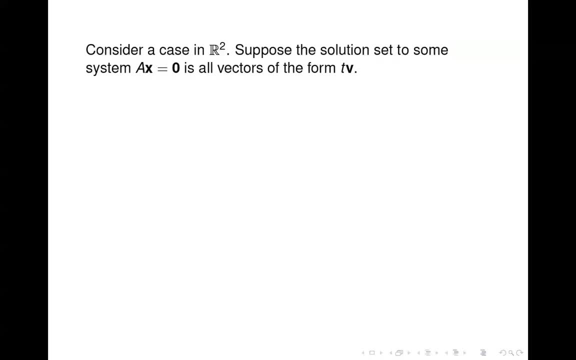 going to just, uh, uh, look at a case in our two, So I'm so. what you're going to see here is not the solutions to the system we were just looking at, because that was in our three. Um, but it's a little bit easier. 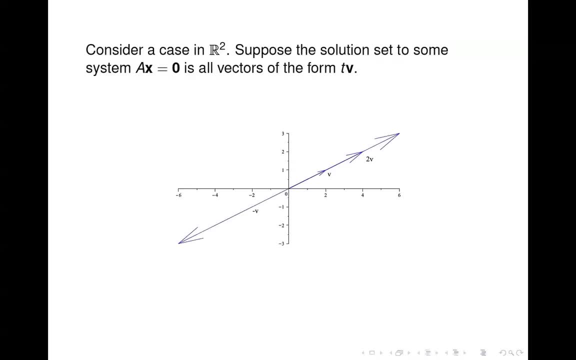 When you draw pictures in our two. So that's what I've got here. So um, for ax equals zero. the solution set is all vectors of the form T times V. So here's a vector V, and we know that T times V is just any vector on this line. 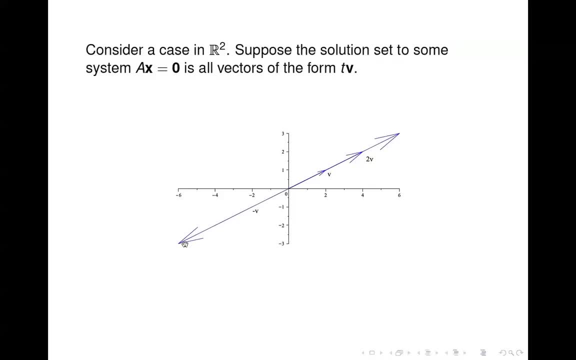 So the line that you see here is the set of all solutions to ax equals zero. Now let's look when we consider the vector P. Okay, So for um. uh, solution set for ax equals B is um of the form TV plus P And um. 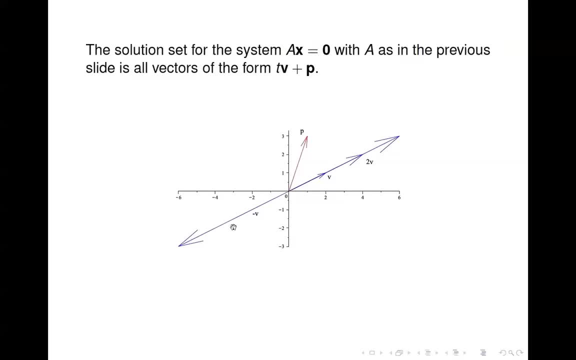 so remember all all the vectors along. here are the T, times, V, And then so for any of these vectors, any point on this line, you can add P and you'll have a vector of the form TV plus P. So for here's one. 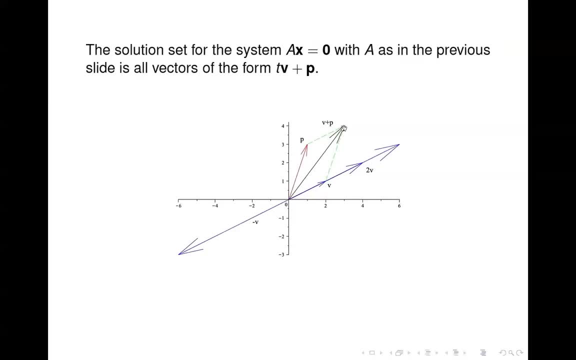 I just did V plus P, So one times V plus P And uh, like doing the parallelogram method, you end up with this vector here. Um, we can do it for other vectors. So here's uh P plus two times V. Um, here's P plus zero times V. Here's P plus negative. 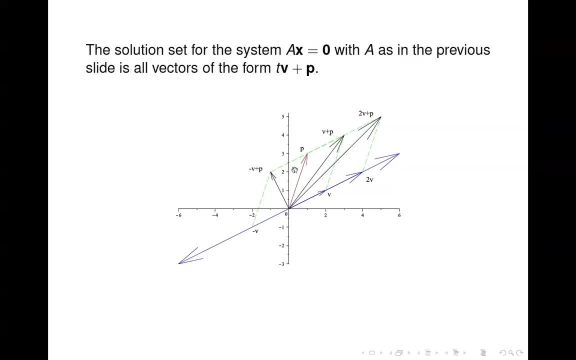 one times V. Okay. So notice though that they all fall along this line, You know so right. here would be P plus a half V, Here P plus three fourths V, Here P plus three halves V, and so forth. So, um. so, for every vector, every solution to ax equals zero. that you have on this line. 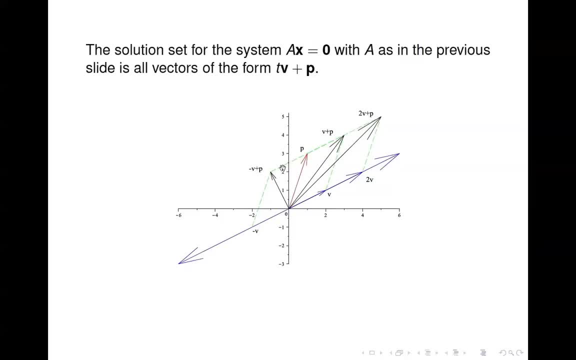 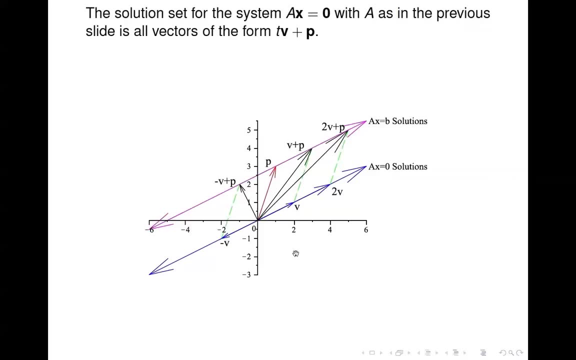 there's a corresponding solution to ax equals B over here on this line, And so we end up with this um approach where along the blue line, that's all the solutions to ax equals zero. along the magenta line, here, all solutions to ax equals B. So notice that. 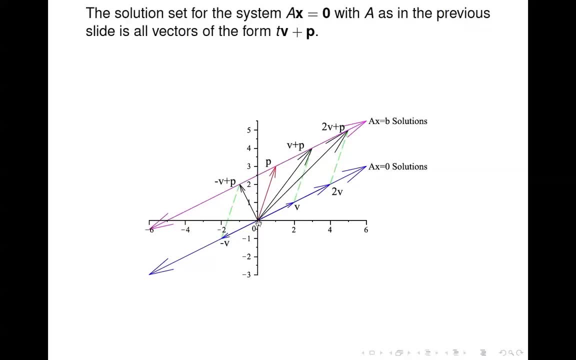 uh, for ax equals zero, it's aligned through the origin. because, uh, that's the trivial solution to ax equals zero and for ax equals B, you're moving off the uh away from the origin. So, off this line, but parallel to the solution set for ax equals zero, 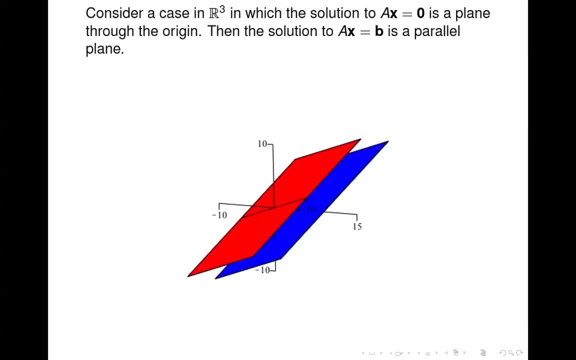 Okay And uh, if you look in three dimensions, let's suppose we have a uh problem where the solution set is a plane in three dimensions. So for ax equals zero. um, it's a plane like this red one that's going to go through the 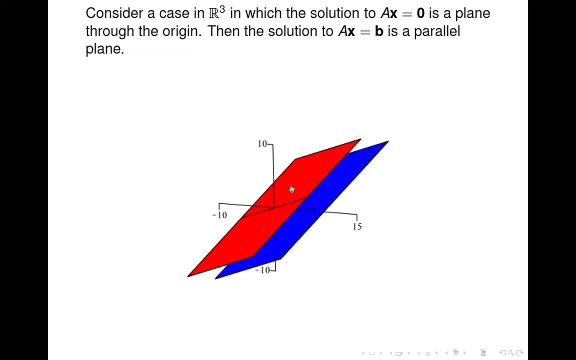 origin And then for ax equals B, you get a parallel plane that's moved off the origin. So for the for ax equals zero, you'd get this red plane that goes through the origin. for ax equals B, You get a parallel plane that's off the origin. 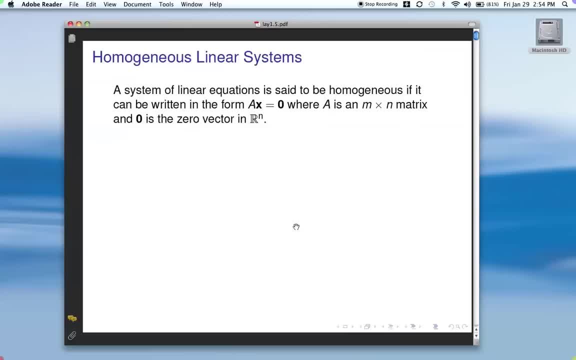 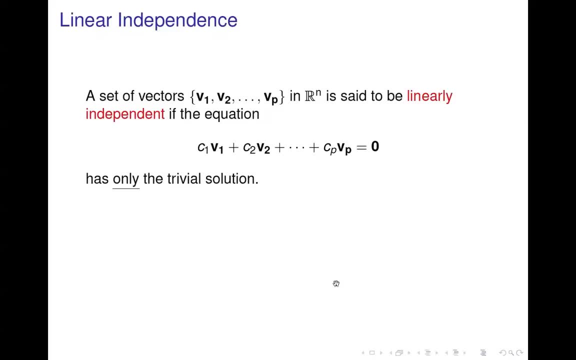 All right, today we're going to talk about the concept of linear independence. So if we have a set of vectors, um, let's say P vectors, in our end the set is said to be linearly independent. If we take a linear combination, set it equal to the zero vector. 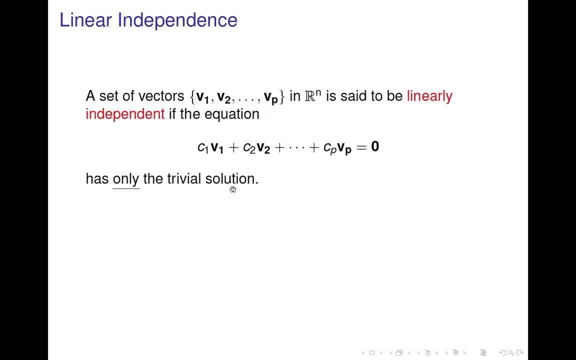 And this equation has only the trivial solution. So the only way, uh, we can take a linear combination of the vectors and get the zero vector is if all the coefficients are equal to zero. um, since this, this uh equation here is equivalent to the system defined by this augmented matrix. then we also say that 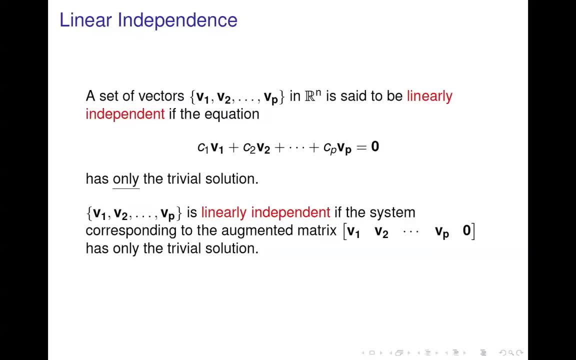 the set is linearly independent. And then if the system corresponding to the augmented matrix, where we put all the vectors in as the columns augment on the zero vector, um, if that uh has only the trivial solution. So these are equivalent. 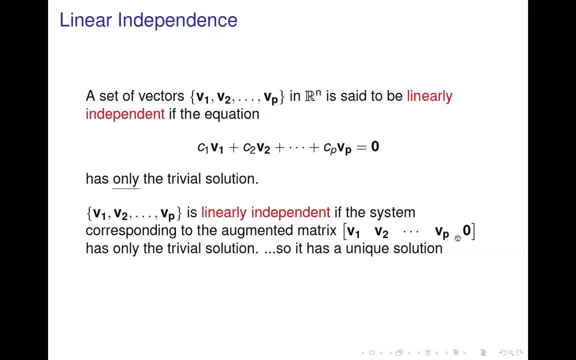 Now, if this has only the trivial solution, then that means it has a unique solution. right? Has only the trivial solution. So, um, all the C's equal to zero is the only solution. So it's unique. So that means it has no free variables. 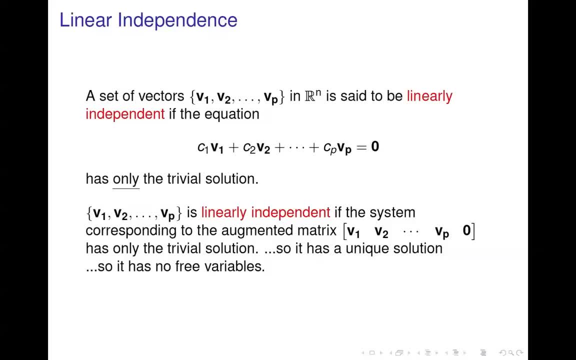 So uh kind of the uh typical method of determining if a system or if a uh set of vectors is linearly independent is to stick them in the columns of a matrix, as I've done here. uh tack on the zero vector for the augmented column and see if that uh matrix. 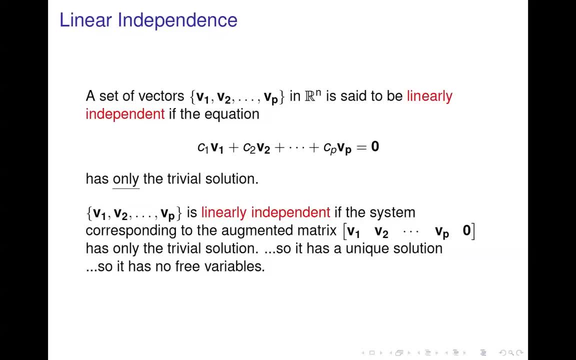 has is if there are any free variables In that system. if uh there are no free variables, then you know the the uh vectors are linearly independent. If you do find a free variable, then you know that there are an infinite number of solutions. 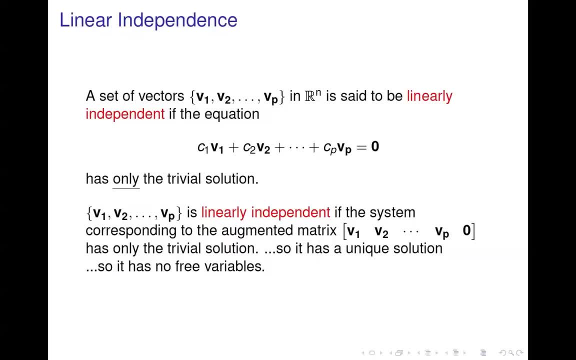 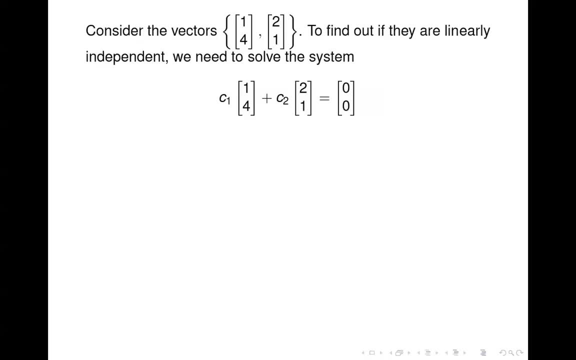 to that system and therefore the vectors are not linearly independent. In that case we say they're linearly dependent. So here's a couple of vectors And if we want to find out if they're linearly independent, then, as I showed you before, 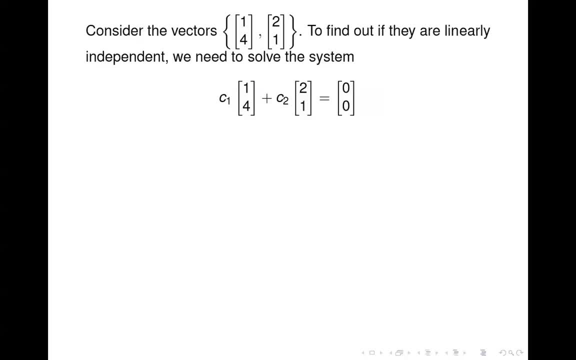 take a linear combination of them and set it equal to zero, as I've done here. We put that into an augmented matrix. It looks like this, with just the two vectors stuck in the columns and the zero vector tacked on as the augmented column. 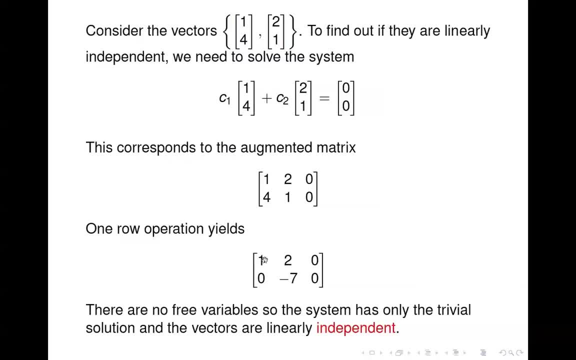 And we can do one row operation and uh, zero out, uh, in this position and notice that we have no free variables And therefore that means that, uh, we have only the true variables. Trivial solution. I think you can see that the solution's unique. 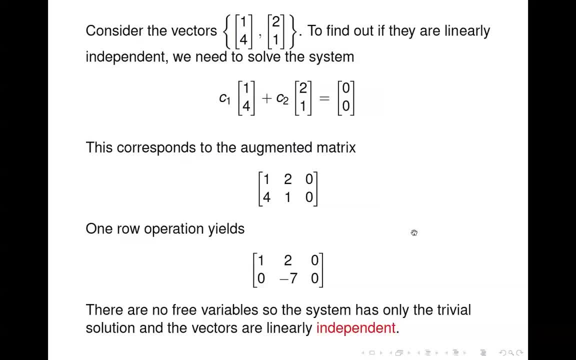 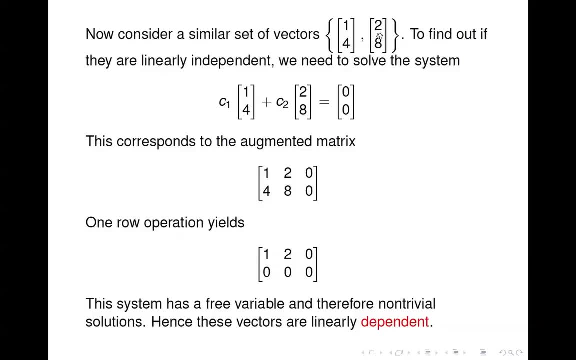 And so these vectors are linearly independent. Uh, here's another set of vectors, right? Uh, just changed just a little bit. Let's see if they're linearly independent. So again, we take a linear combination, set it equal to zero, stick that in, uh, as an. 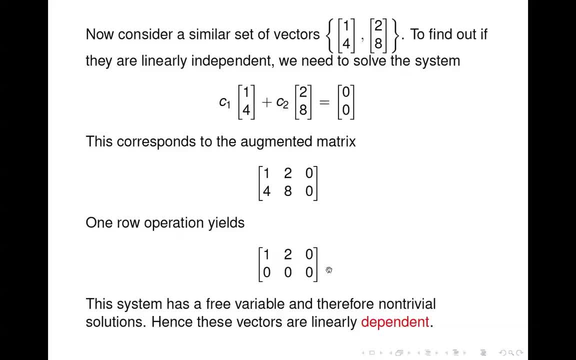 augmented matrix, Do one row operation And we end up with three. Okay, So we take this matrix here and notice that, um, we've got a free variable, X two. here, The second column, uh, has no pivot position, So X two is a free variable. 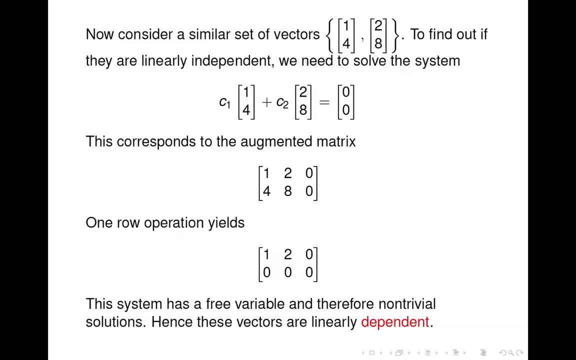 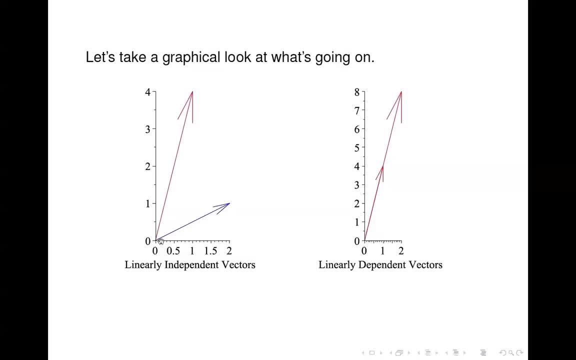 So, therefore, these vectors are linearly dependent. Now, if you look at the vectors that we had um the first set, if we graphed them, looks like this: Uh, we had two one and one, four, So they look like that. 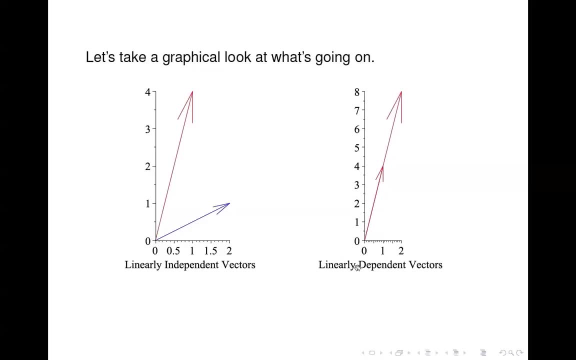 They're linearly independent, Whereas that second set, Um, I believe we had one, four and two, eight. Let's back up Yep: One four and two eight, And so they're multiples of each other. So they're uh indicated in this picture and they're linearly dependent. 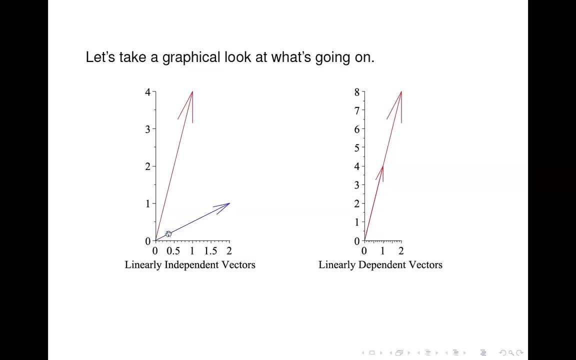 Interestingly, you can see that these two vectors uh, um, do uh if you, if you think about the span of these two vectors, Okay, You can take a linear combination of these two and produce any vector in R two. 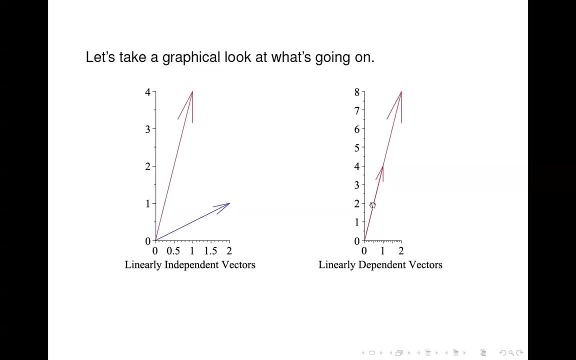 However, for these two, any linear combination of these two vectors only gets you vectors on the line that's defined by these vectors and going back in the negative direction here, but you get no vectors off that line. Uh, we're, we've been looking at the two vector case, which is uh, at times can be misleading. 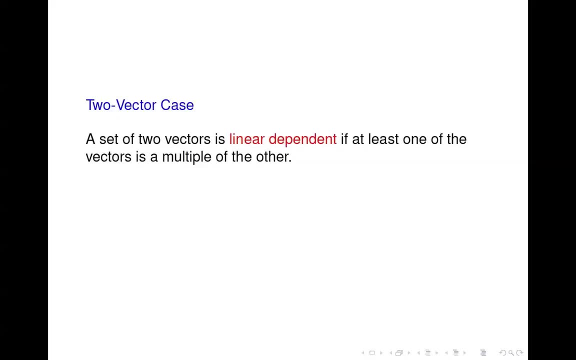 but let's examine. Let's examine what we can say about it. Um, when you have just two vectors, then they are linearly dependent. if, uh, at least one is a multiple of the other, All right. So if they're multiples of each other, or one's a multiple of the other, then, uh, they are. 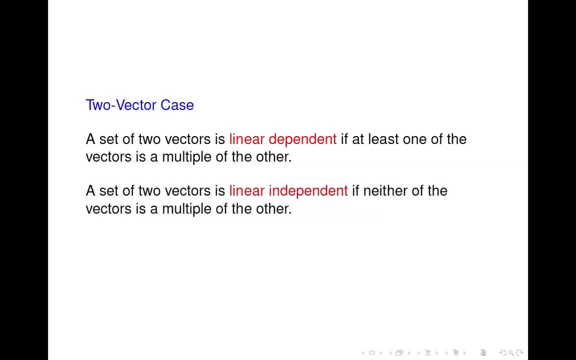 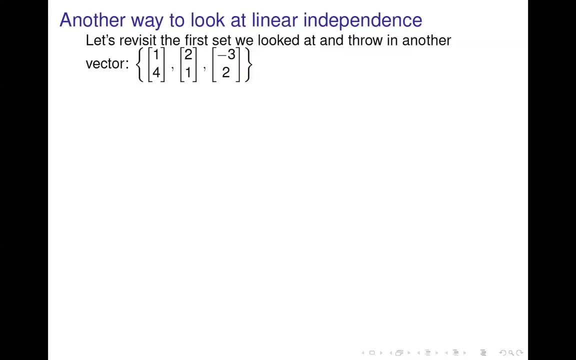 linearly dependent. They're linearly independent if neither is a multiple of the other. So that works when you only have two vectors. Okay, Let's, let's kind of expand our uh scope here and um, we'll get a set with three vectors. 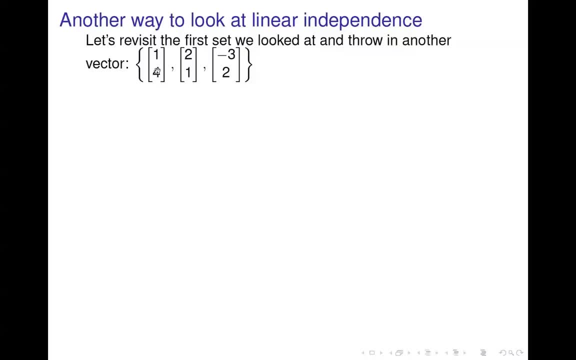 So, um, I took the set we were looking at initially- one, four and two one- and threw in another vector in there. Now, what do you think? Are these vectors linearly independent? Well, if we take a linear combination of them, set it equal to zero. vector like this is: 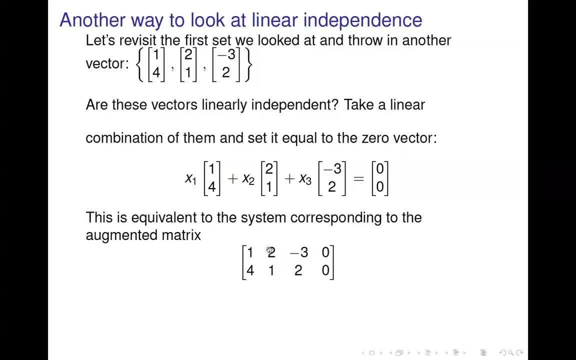 just going back to the first definition we talked about, And throw that in an augmented matrix, you end up with this. And what happens? Hm, No need to do any row operations. Why is that, You know? let's think. 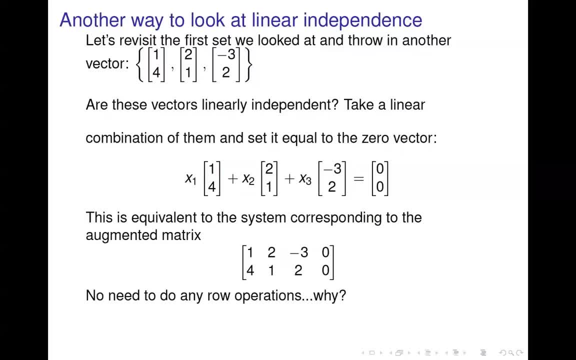 How do we know if the system is uh or if the uh system? we want to know, does the system have uh- only the trivial solution- or not? Or another way is: does it have any free variables? Well, we can look at this one and say, yep, there's at least one free variable. 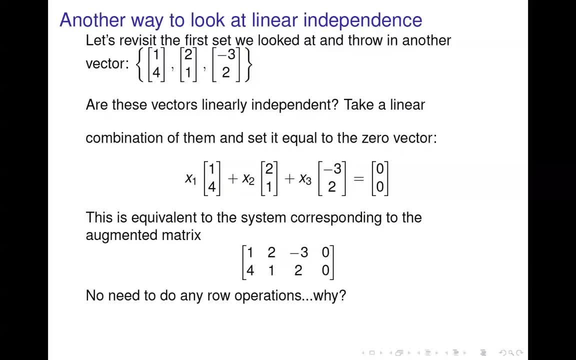 There has to be, because we have three variables and only two equations. So three columns, only two rows. So we have to have at least one free variable so we can have at most two pivot positions Right. So these vectors are linearly dependent. 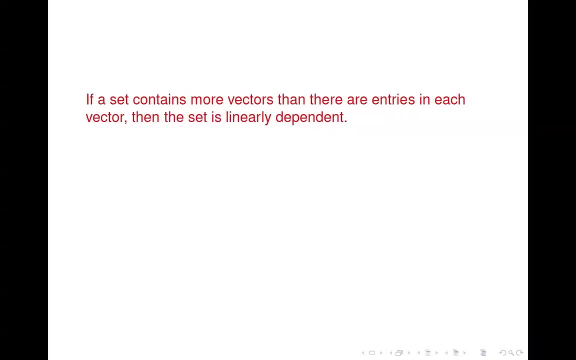 Okay. So here's a rule: If the set contains more vectors, then there are entries in each vector. then the set's linearly dependent, And that's the case we just looked at. We had three vectors in R2.. So more entries, more vectors, then there are entries in each vector. 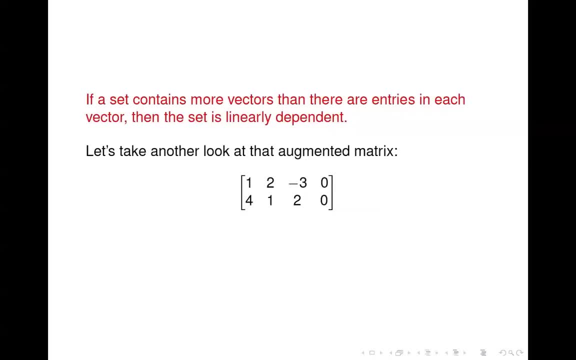 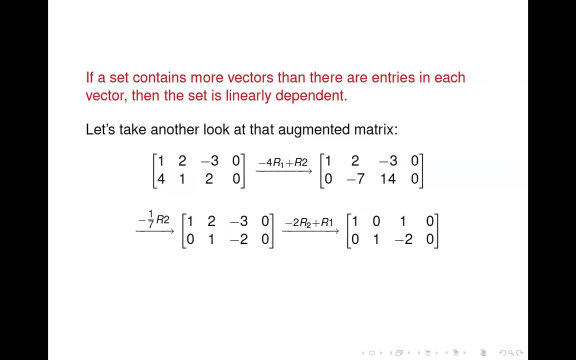 Okay, there it is. Got uh three vectors and uh only two entries in each vector. Um, if we look at that augmented matrix and, um, do some row operations on it, uh, we end up at this point. 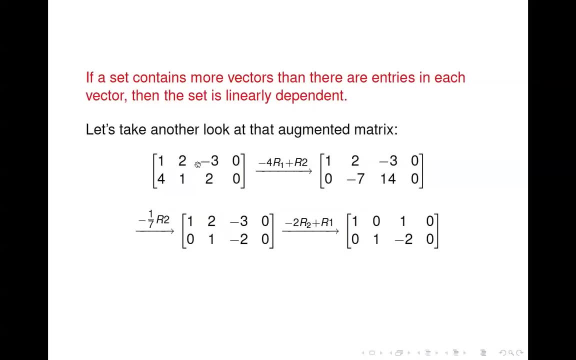 Now remember back here. just looking at this, you knew they were linearly dependent because you had more vectors than there were entries in each vector. But if we do these row operations and get this matrix in reduced echelon form, then we end up here. 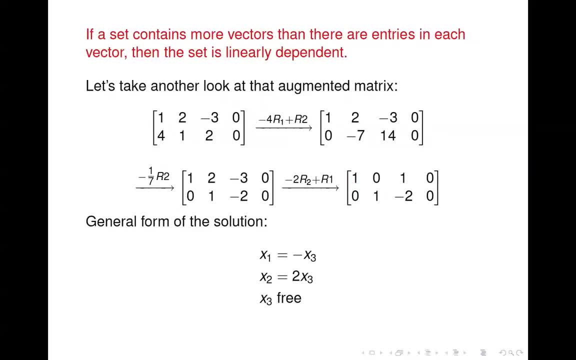 So if we wrote the solution um of that system, uh, it looks like this: you know, from the second row you get: X2 is going to equal 2X3.. X1 is equal to negative X3.. And X3 is a free variable. okay, 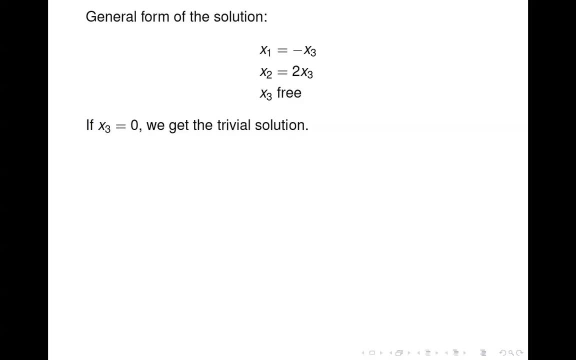 So you can plug in uh anything you want for X3 to generate specific solutions. For instance, if we said X3 equals zero, that's going to give us the trivial solution right, Because X3 is zero and based on uh what X1 and X2 are, defined in terms of X3, they're. 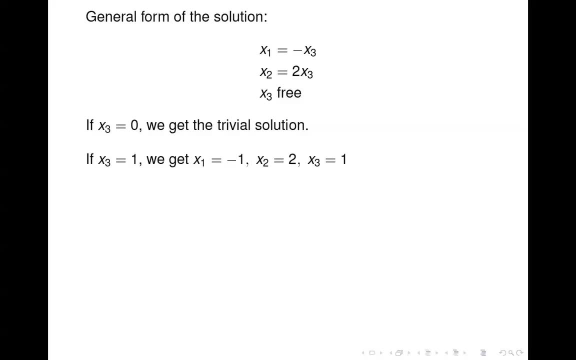 going to be zero. also, If we said X3 equal to one, then we get: X1 is negative one, X2 is two And X3 is one. Now why don't we- where does that apply? to? Well, notice we're, we were trying to find a solution to this equation, right? 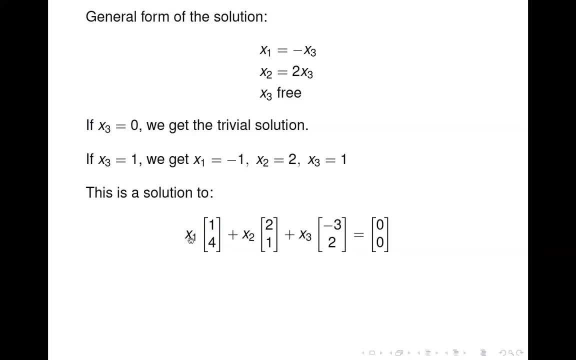 We were trying to see, can we find non-zero values for X1,, X2, and X3, or at least one of them, non-zero, um, so that we can produce the zero vector, And so, um this uh general formant solution tells us how to form uh the values for X1,. 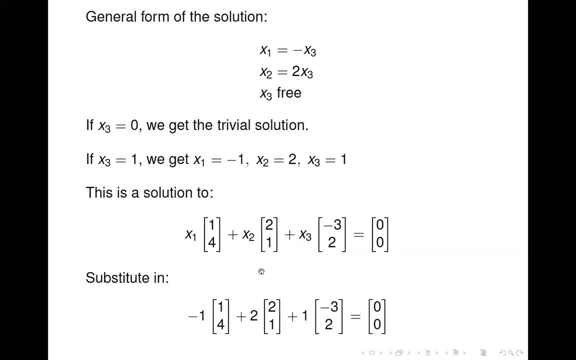 X2, and X3. So we can take our uh values that we got for X3 equals one, plug them in. So notice, if we do that we end up with negative one times. one is negative one plus four here. 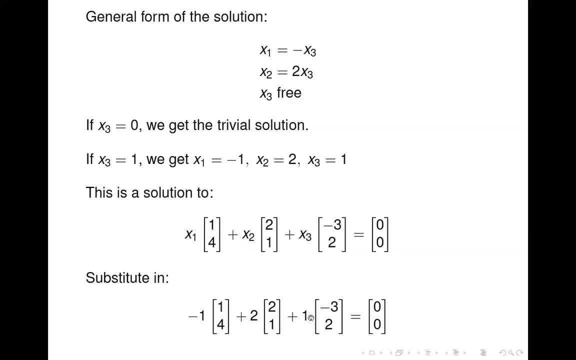 is negative. three- uh, I mean positive- three minus three gives us zero, and in the second position we get negative. four plus two is negative. two plus two is zero. So we can find specific values, uh, for these coefficients, so that we can produce the zero. 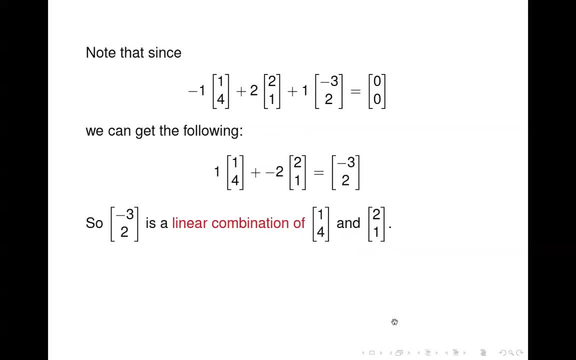 vector. Now notice from this we can take that equation and solve it. um for negative three, two. So we can just take this over to the uh, the other side and notice that negative three- two can be written as a linear combination of one, four and two, one. 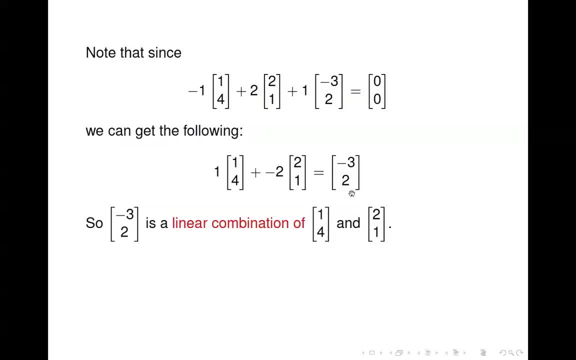 Right, That's what we've just done here. We've written negative three two as a linear combination of the other two vectors. Another way of saying that is that negative three two is in the span of these other two vectors. Right. 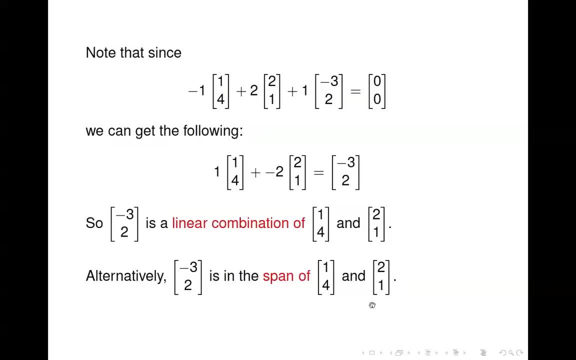 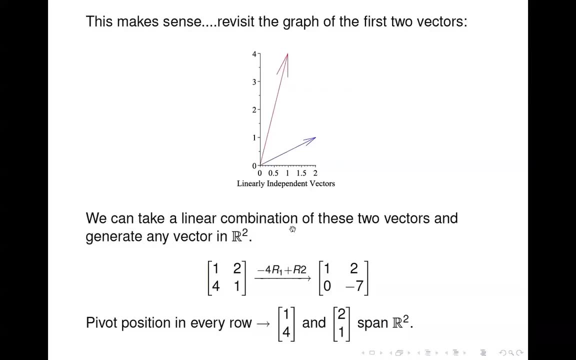 It's a linear combination of them, so that means it's in the span of those two vectors And if you think back to our picture, that makes sense Right. Here were, uh, the first two vectors: two one and one four. 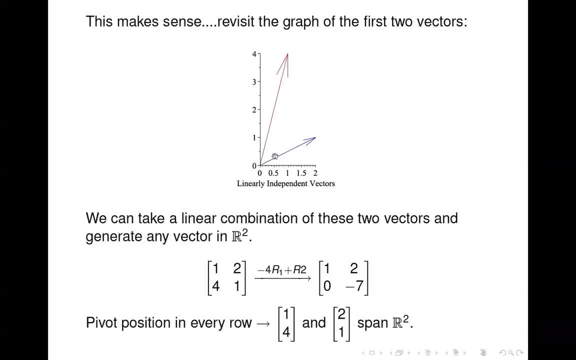 But before I talked about how these span R2.. Right, We can take a linear combination. we can scale each of them and then add those scaled vectors together to produce any vector in R2.. And uh, how do we know that? 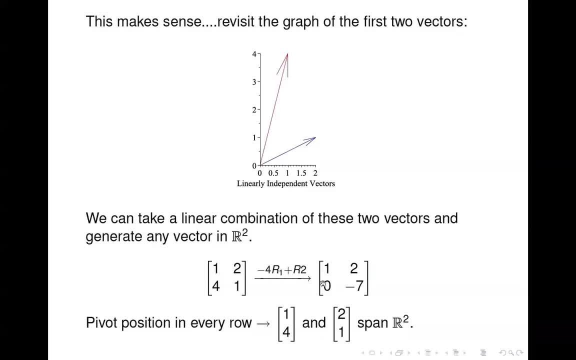 Well, just look at those two vectors, do a row operation and look, We have a pivot position in every row. So by theorem four, going back to section 1.4.. Theorem four, that says that, uh, the vectors span R2.. 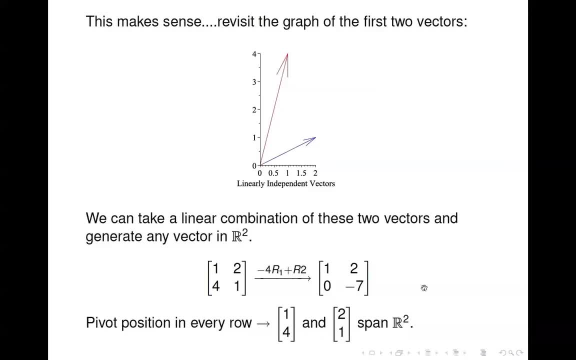 Right. One of the things in theorem four is if you have a pivot position in every row, that means the columns of the original matrix span uh, the uh space in which they live, which in this case we're in R2.. 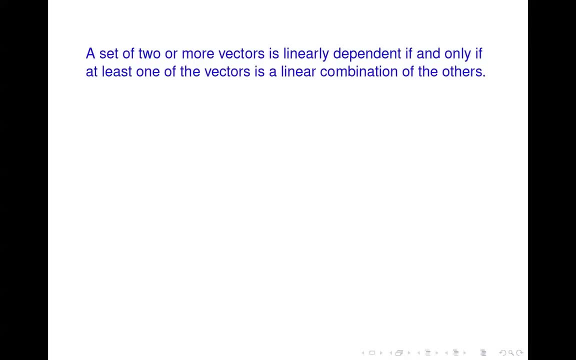 Okay. So here's another rule that, uh, relates to linear dependence. A set of two or more vectors is linearly dependent, Okay. A set of two or more vectors is linearly dependent if, and only if, at least one of the vectors. 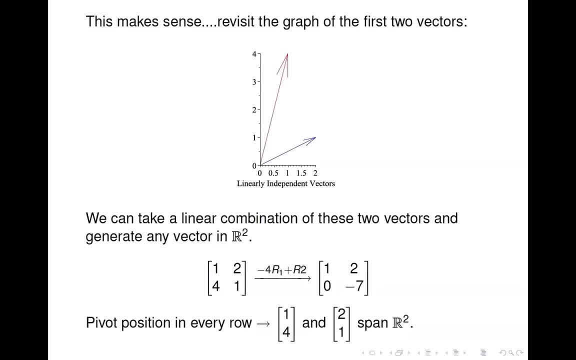 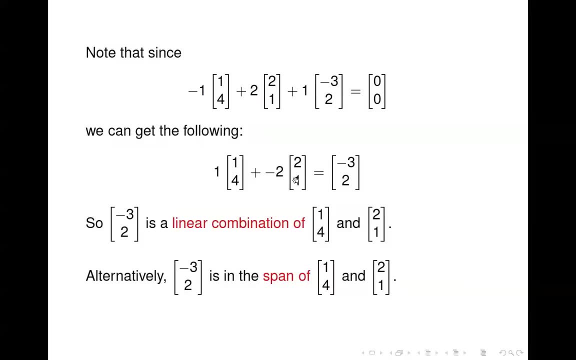 is a linear combination of the others. So back here we saw that, uh, negative three. two is a linear combination of the other two vectors And in fact we could have solved this system for any of these three vectors. We could solve for any of these three vectors in terms of the other two. 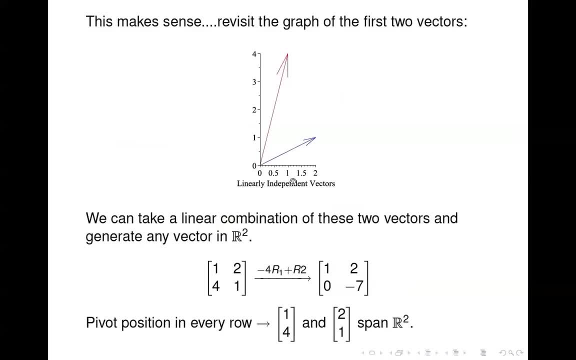 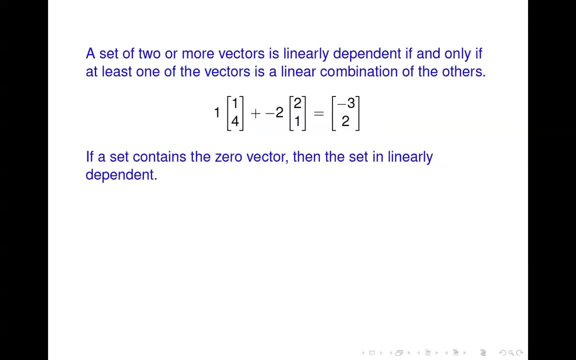 So any of these vectors is a linear combination of the other two. Okay, there you see it. Um again, all right, moving on, um, if there's another rule, keep in mind: if a set contains the zero vector, then that set is linearly dependent. 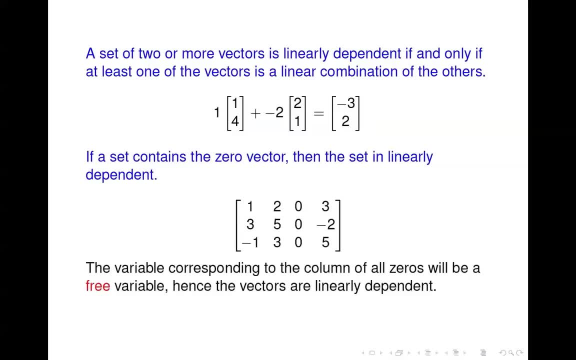 So if you have a zero vector in the set, then the set has to be linearly dependent. Here's an example of that. You got the zero vector. Notice that it's always going to be a free variable. Okay, The variable corresponding to the zero vector is always going to be free, and hence uh. 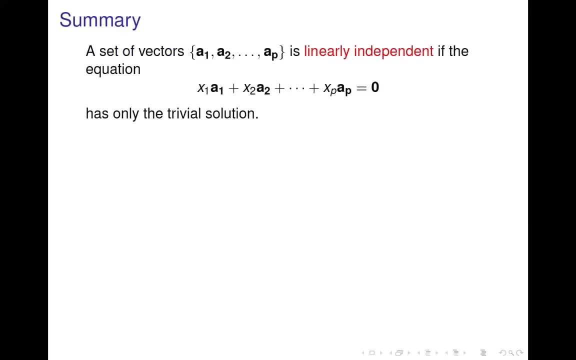 the set would be linearly dependent. So summary: um set of vectors is linearly independent. If you take a linear combination, set it equal to zero and you have only the trivial solution. So so all the x's equals zero is the only solution. 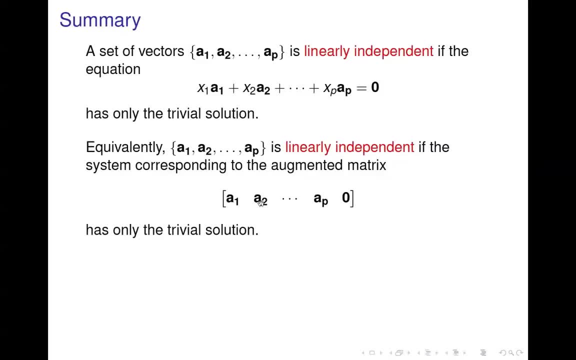 Equivalently. you throw all those those vectors into a matrix, tack on the zero vector for the augmented column, solve that system, and you get only the trivial solution, Okay. On the other hand, it's linearly dependent if the system has at least one free variable. 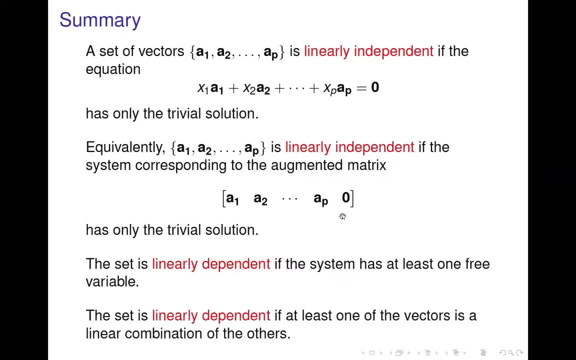 because in that case you would have an infinite number of solutions. And uh, another way of characterizing linear dependence is a set's linearly dependent if at least one of the vectors is a linear combination of the others. Okay, And that's it for, uh, section 1.6.. 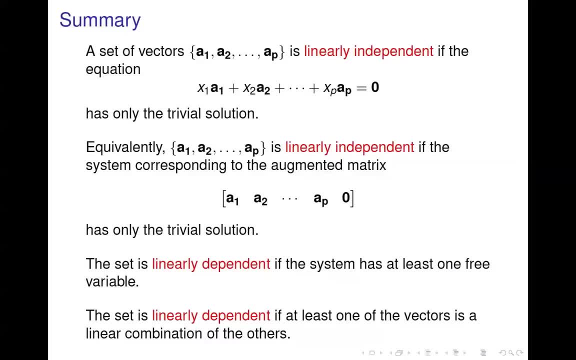 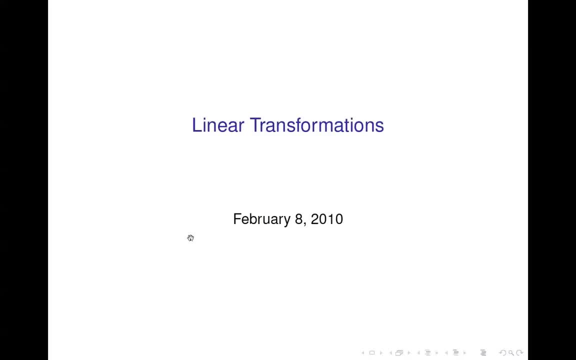 1.7.. Okay, we're going to start uh today talking about linear transformations, Um. first we're going to um. look back at um, uh, something you're familiar with from algebra or calculus, um, and we'll just look at a basic function. 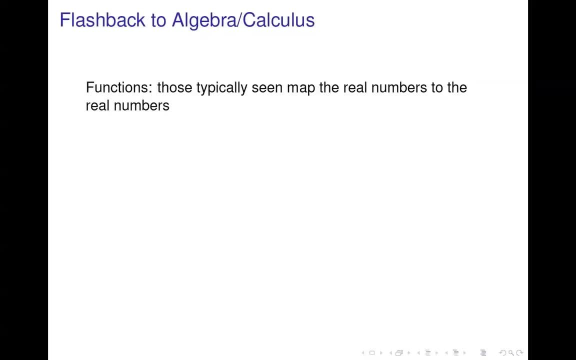 Which, Uh Uh, Typically maps some real number to another real number. We map the set of real numbers to the set of real numbers. So, for example, um, here's a graph of a function: f of x equals x squared. And so, um you, um input a real number. okay, x is a real number. 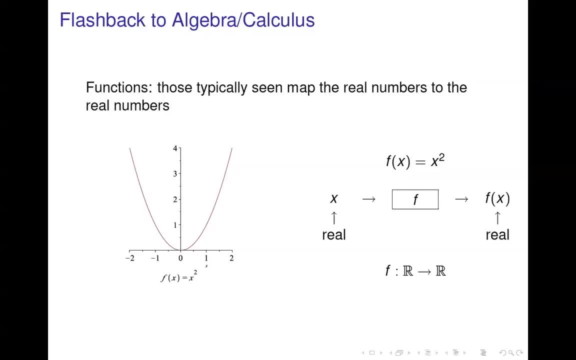 You square it and you get another real number. So it's mapping the real numbers to the real numbers. Here's a little picture view. Uh, here you're putting in uh, a real number into your function and and uh, for our purposes. 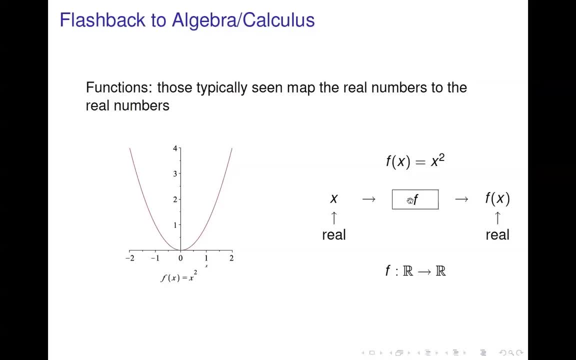 here. we know what the function does: it just squares the number, but you really don't have to know exactly what the function does: Um. you uh know that. what comes out, though, is another real number. So this notation down here at the bottom: um is read: f is a function that maps the real. 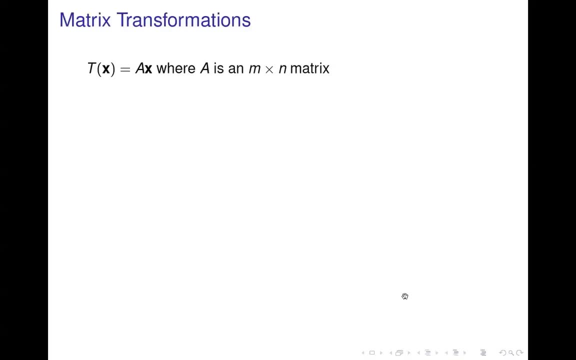 numbers to the real numbers. Um, now let's move to talking about uh, matrix transformations. And it's the same basic idea as a function. Um, it's just defined in terms of a matrix. So here, t of x, t for transformation, uh, so we, we apply our transformation to x. 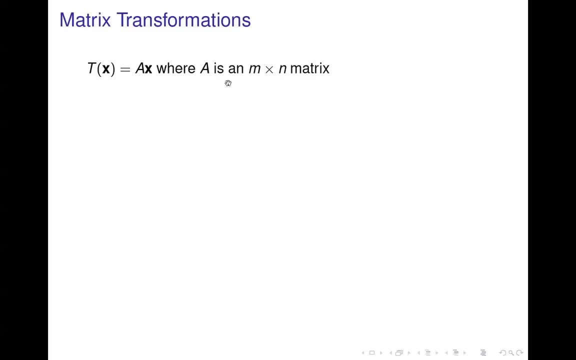 We multiply a times x, where a is some m, by n matrix. That defines this transformation. So here's a picture view of what's going on. You have a vector from Rn that is the input to your transformation and the output is: 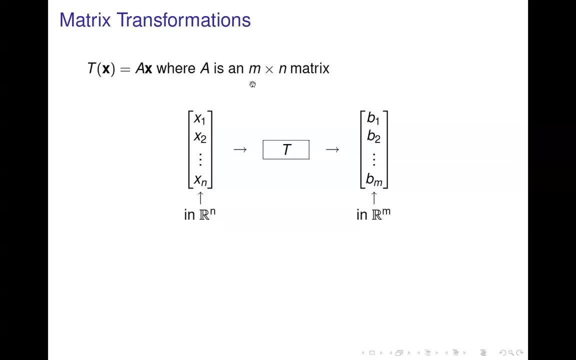 a vector in Rm. Okay, so the key here is that a is an m by n matrix and the transformation occurs by multiplying a times x. so that means that x has to have as many entries as there are columns of x. So we need an x component to match up with each column of a, because a times x is just. 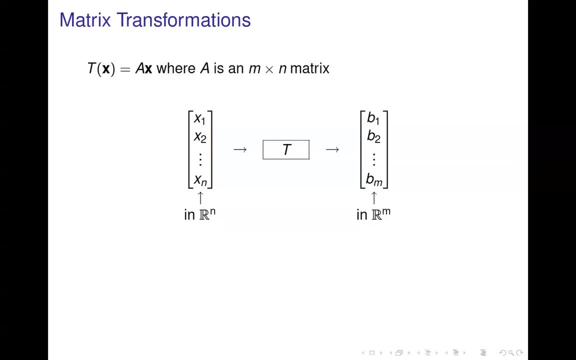 a linear combination of the columns. so we need an x component to match up with each column of a, And then each column of a has m entries. so when we do that linear combination, we're going to end up with a vector with m entries and hence, uh, we end up with a vector in. 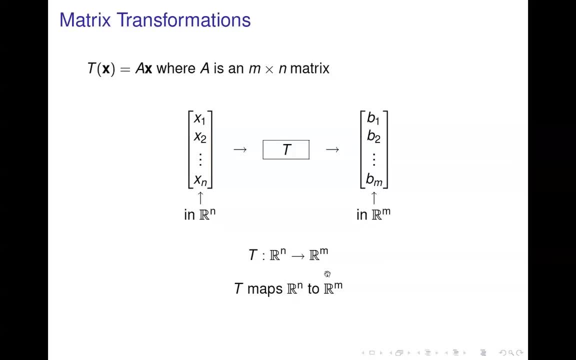 Rm. Okay, so we say that t uh maps Rn to Rm. So, for example, here's a matrix A and let's suppose that we have a transformation t defined on this matrix. So t of x equals a times x. 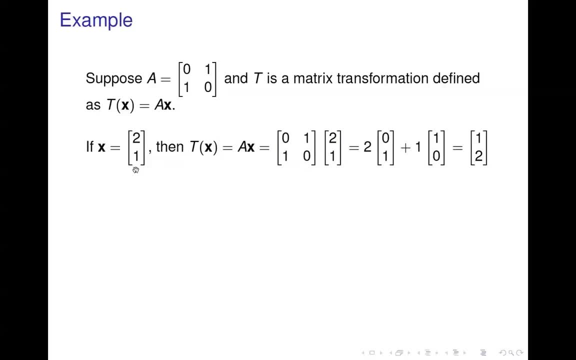 So here's a vector: x equals 2, 1.. Then t of x is a times x. so we do that multiplication, take a linear combination and we end up with 1, 2.. Okay, so we started with a vector in R2.. 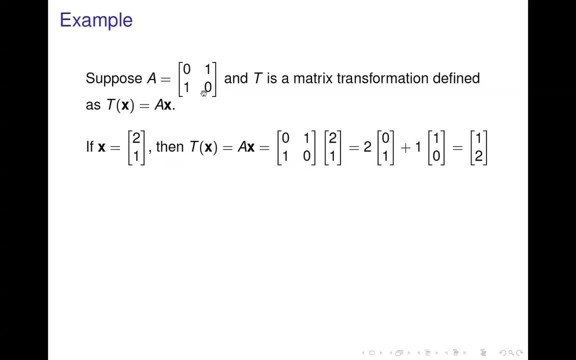 Okay, in r2, which makes sense since a is 2 by 2. here's another example: we're applying the transformation to the vector 4 negative 2, so we multiply a times that vector, and so we take the linear combination of the columns of a and end. 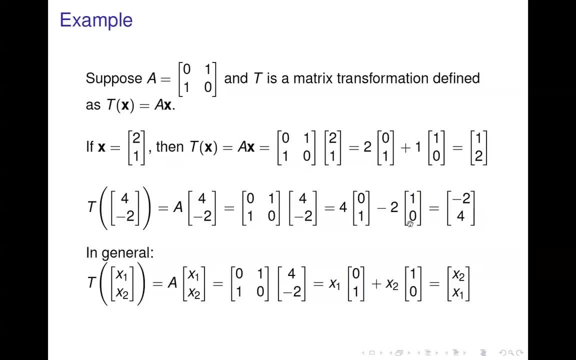 up with negative 2, 4 if we look at it in a general case. so we just apply T to a generic vector, x1, x2 from r2 did the same way as we did the previous two and notice we end up with x2, x1. so this transformation has just reversed the. 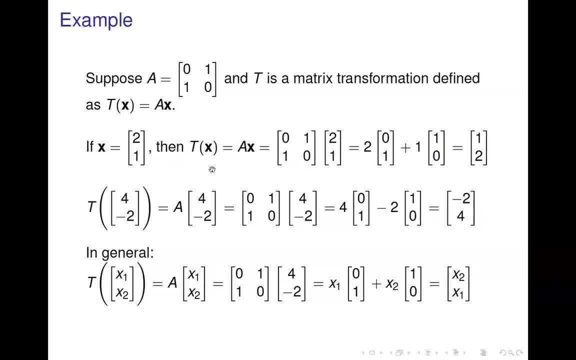 order of the elements. if you look back up at these other two, you know 2. 1 went to 1, 2, 4, 2 went to 4, negative 2 went to negative, 2, 4. so that's all this transformation is doing, swapping the order of the elements in the input. 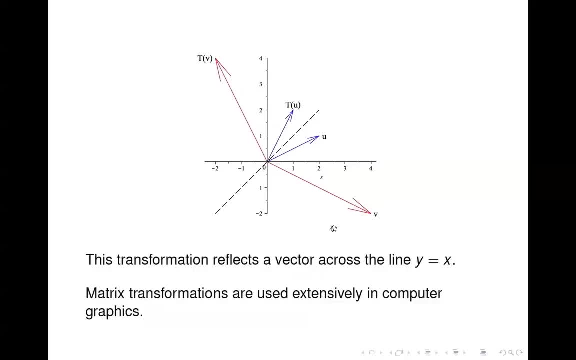 vector. if you look graphically, it's what's going on. here's one of the vectors: 2, 1, and here was its transformation, which is 1, 2, and here's the other one, 4, negative 2, which was transformed into negative 2, 4, and so you can see from this picture: 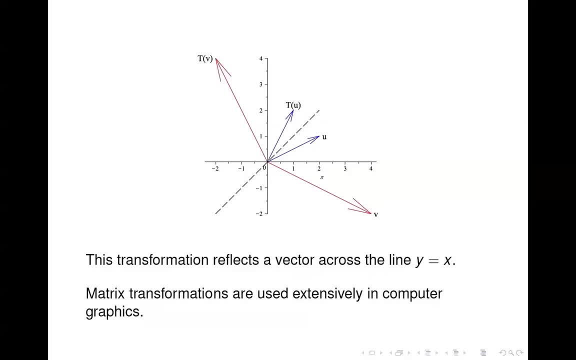 that this transformation is reflecting a vector across the line y equals X. okay, okay, this is kind of standard sort of thing that you see in computer graphics, and so matrix transformations are really the fundamental element in computer graphics. so if you were to go on and take that course in the computer science, 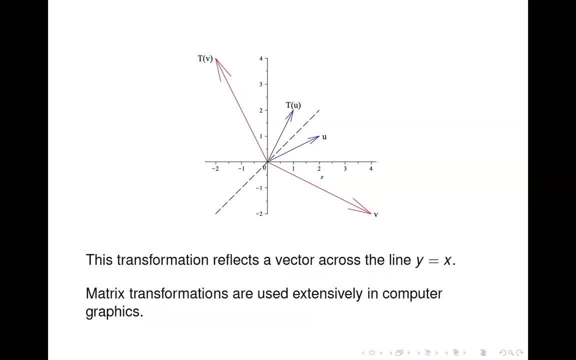 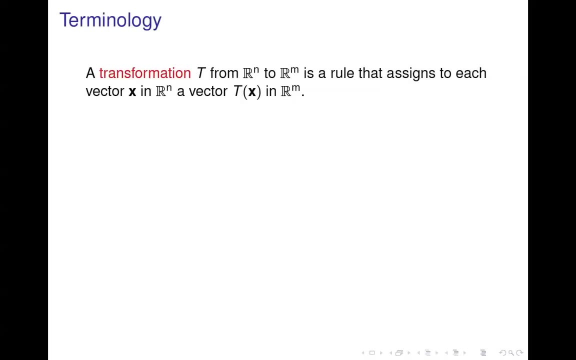 department you would be seeing a lot of matrix transformations. okay, so to be a little more precise, we say: a transformation T from our end to our M is a rule that assigns to each vector X and our in a vector T of X in our M more terminology. here our N is called the domain of T, in our M is: 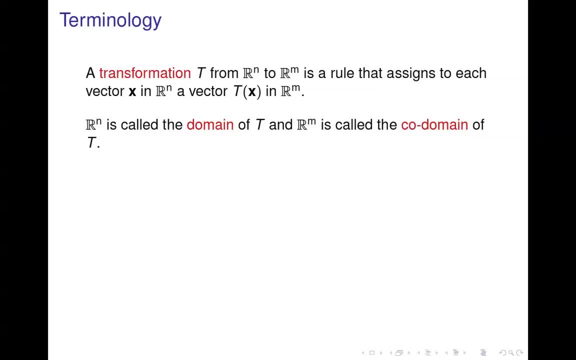 called the co-domain of T. so our N is where the inputs to the, to the transformation, come from. our M is where the outputs come from. okay, for a given X. in our N, T of X is called the image of X. okay, so the image of X is just the vector that X maps to. if we look at all images, all possible. 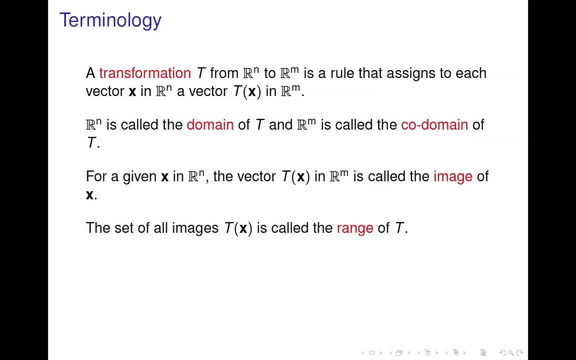 images that we get under the transformation T. this is called the range of T. okay, so the range of T is all images that we get when we map all possible vectors X through this transformation. now you might be thinking that well, in that the co-domain. and the answer is: sometimes it is, and sometimes 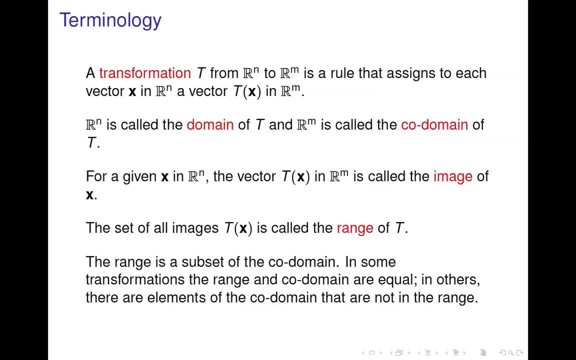 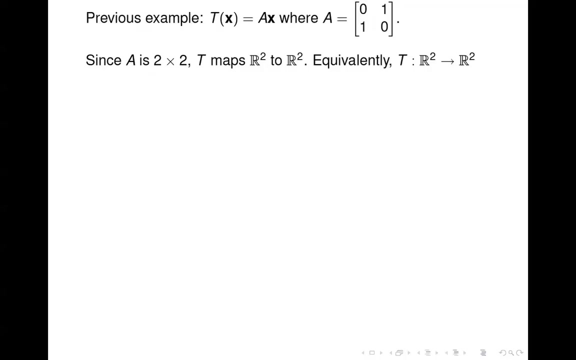 it isn't okay. in general, the range is a subset of the co-domain. in some cases they are equal. in others they're not. their elements, the co-domain that are not in the range. so not in general, not everything in the co-domain is mapped to necessarily okay. so here's back to our previous example. 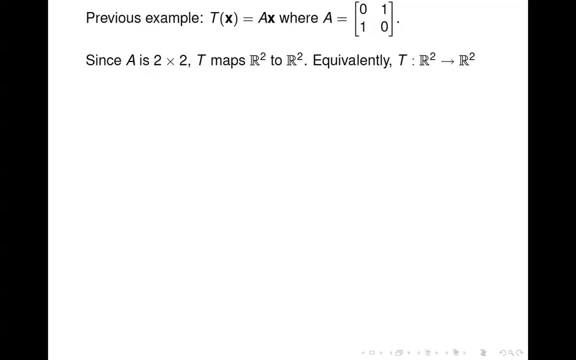 we've got this transformation maps R2 to R2, so the domain is R2 and really the domain is the first set that you see here when you write down the transformation in this fashion. the co-domain is also R2, so we're mapping vectors from R2 to vectors in R2 also. now the range. let's think about that. 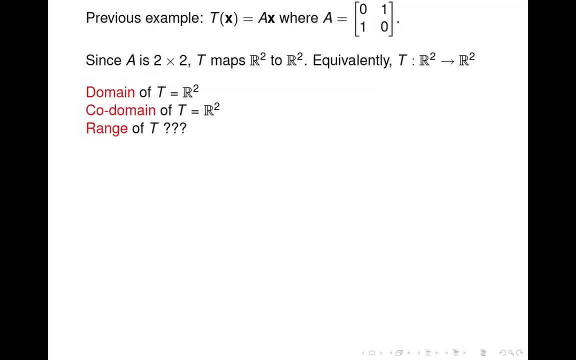 another range. think of the range as just everything that gets mapped to under this transformation. and if you look at the picture, okay, that we had before you, if you wanted to produce any vector, then you can figure out what vector you need. that would map to it, because you just need to. 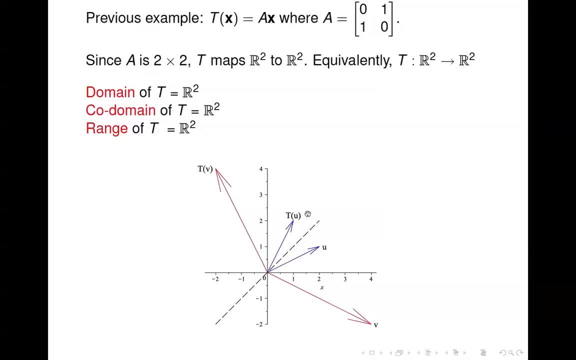 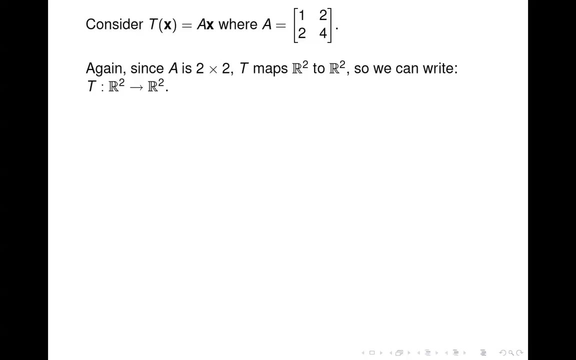 reverse the order of the elements. so that means that the range of this transformation is all of R2. so the co-domain and the range are equal in this case, because any vector in R2 is mapped to. all right, let's look at a different example. okay, here's one defined by different matrix A, still a two by two matrix. so 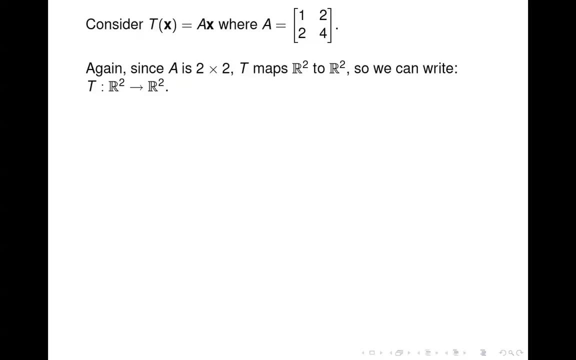 this transformation also maps R2 to R2, so the domain is R2, the co-domain is R2. let's think about what is the range of this transformation. well, let's play around with it for just a little bit. let's take our old vector 2: 1 and see: 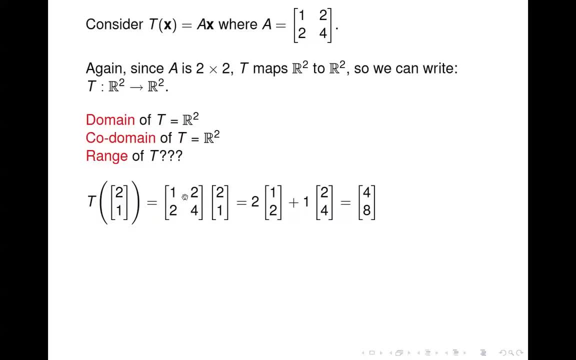 what it maps to. if we apply the transformation to 2, 1, multiply a times 2, 1 and we end up with a vector: 4, 8. okay, how about another one negative, 3, 2 a times that vector? take the linear combination, you end up. 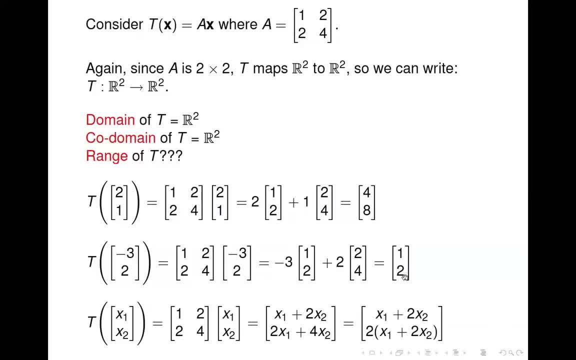 with 1, 2. so let's look at the general case. what happens? we apply it to just a generic vector: x, 1, x 2, do that matrix multiplication and we end up with this vector, which I can rewrite in this form to illustrate that the second component of the vector is just twice the first. 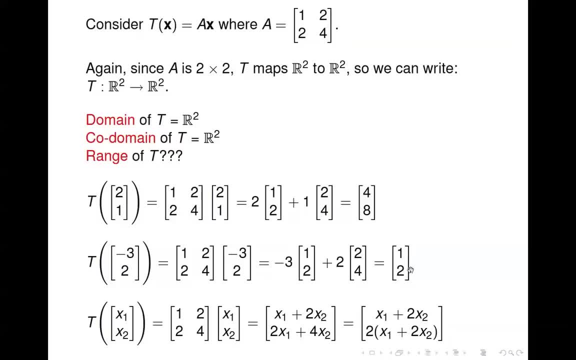 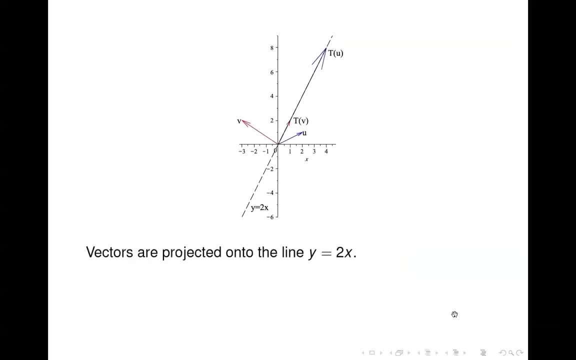 one. and you see that in these other two that we did right here, the second components two times the first. here again, second components two times the first. so if we look at that, graphically, every vector that we can map to is of this form: the second components two times the. 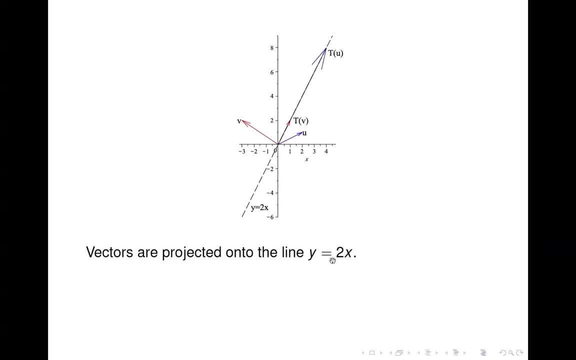 first. so that's actually all vectors on the line y equals 2x guys. second component is two times the first because here's 2, 1 and it maps to four, eight. so it's on this line the vector negative, three, two. I believe it was that we looked at it. 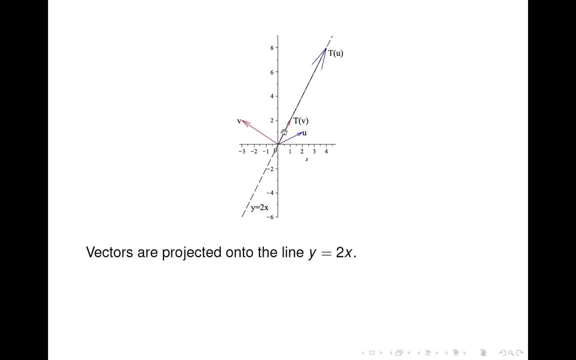 mapped to one, two. so here it falls on the line. so no matter what vector you choose, it's going to be projected onto this line. so the range of this transformation is simply this line. the line y equals 2x, or all vectors of the form x1, 2x1. so we're all vectors where. 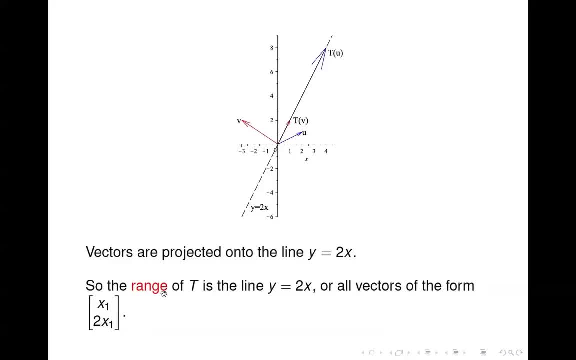 the second component is just 2 times the first, so here the range is is not the same as the codomain, right? the codomain is r2, but the range is just this line: y equals 2x, so it's just part of the codomain. okay, suppose at this point we 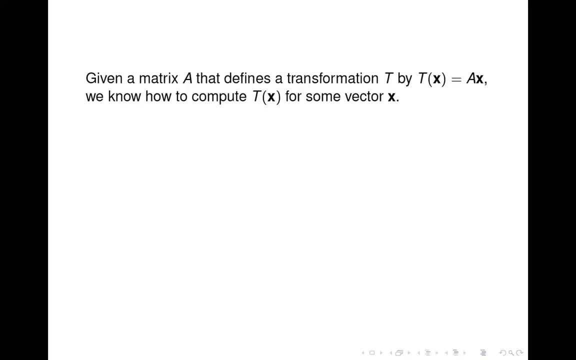 know, given a transformation in the matrix that defines it, we can compute T of X and just multiply a times X. a little more difficult question is this one: how do we determine if a given vector B is in the range of a particular vector B, and how do we determine if a given vector B is in the 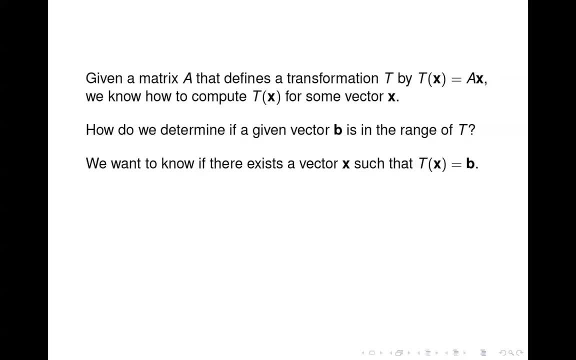 range of a particular vector B, and how do we determine if a given vector B is in the range of a particular transformation? right? so we're asking: is there a vector X that maps to B, or is there a vector X such that T of X is equal to B? and since T of X equals a times X, we can say: does there exist a? 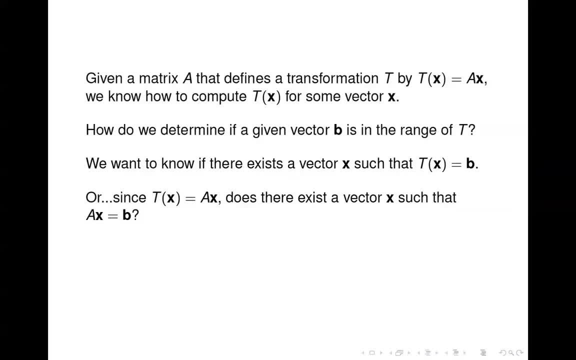 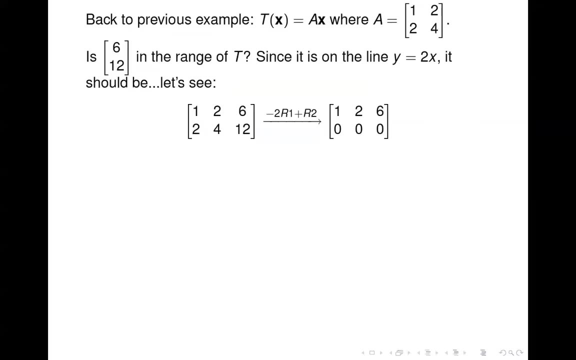 vector X, such that a times X equals B. and now we're back into the realm of looking at systems of equations, and we're very familiar with that. okay, so simply a system of equations to solve, all right. so let's go back to that previous example and suppose you were asked: is 612, is this vector 612 in the? 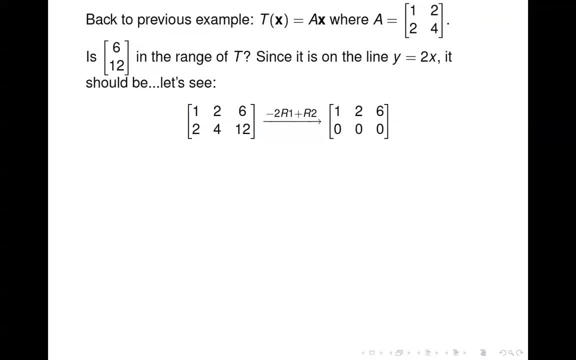 range of T and we know that since the range of T is all vectors on the line y equals 2x, then it should be, because the second component, 12, is 2 times the first. so let's solve the system of equations. all right, here's the system of equations. 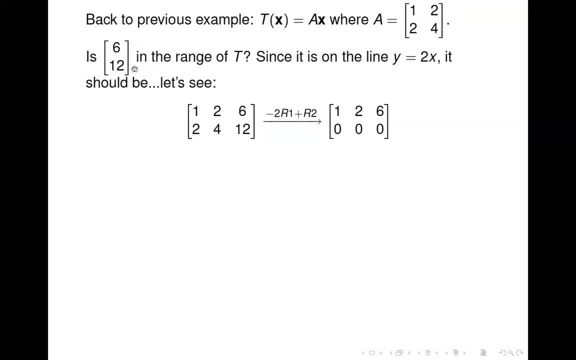 the augmented matrix corresponding to ax equals B, where B is 612. when we do one row operation and here we go, it's an echelon form and clearly the system is consistent. so therefore the vector is in the range of T, about another one about 610. now, in this case- notice- the second component is not 2 times the first, so 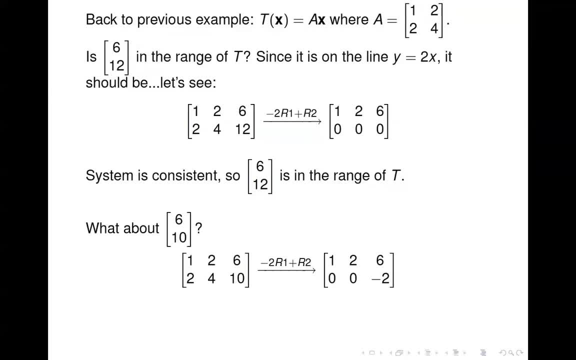 you would expect this vector not to be 2 times the first, so you would expect this vector not to be in the range of T, which would mean that this system should be inconsistent, and, as you see, do one row operation and you end up with 0, 0 and 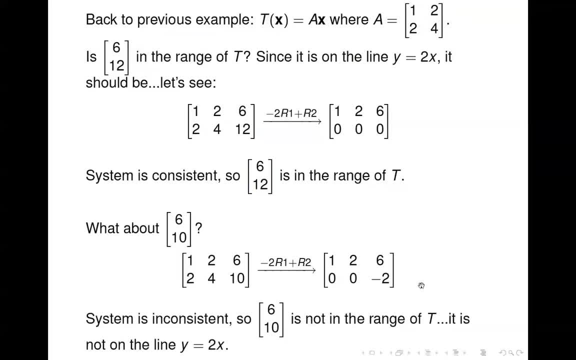 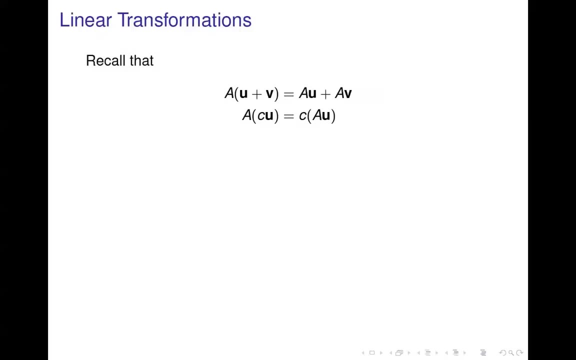 then negative 2. so that's clearly the system is inconsistent. so this vector is not in the range of T. okay, so to determine if a vector is in the range of a linear transformation, you need to solve a system of equations. okay, changing gears just a little bit. previously we learned that matrix. 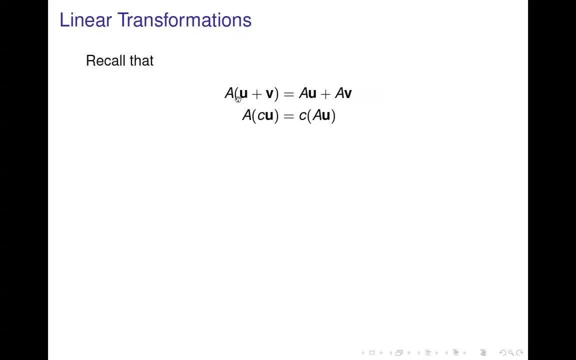 multiplication has certain properties, and one of them is this one: that if you multiply matrix times the sum of two vectors and you can distribute. okay, so a times u plus V is equal to a u plus a V. and similarly, if you multiply a times a, a scalar times a vector, then you can move the scalar out. okay, so a times C U. 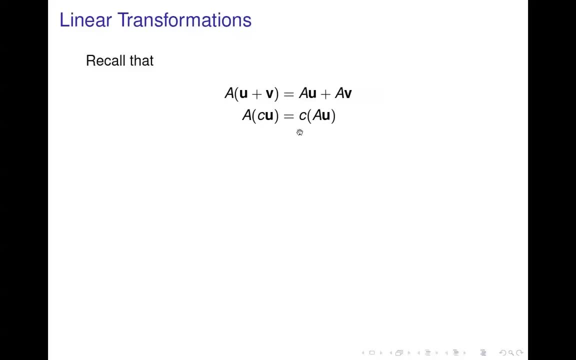 is the same as C times a? u. okay, now I bring that up because that applies here. okay, so a transformation is said to be linear if the following conditions hold that: T of u plus V is T of u plus T of v, and T of C times u is C times T of u. okay, so these two conditions look very. 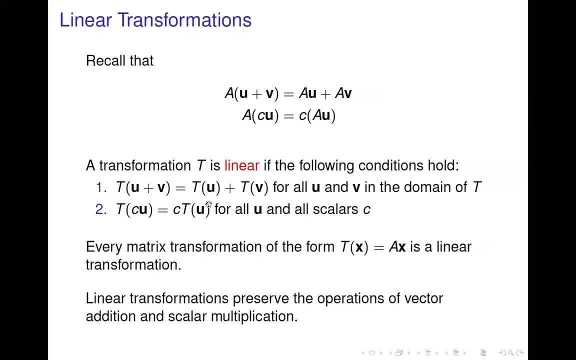 similar to what we have up there, and, in fact, since we define our transformation as a times X, then these are really equivalent. okay, so linear transformations preserve the operations of vector addition and scalar multiplication, and we'll stop here at this point, and then the next video will be for section 1.9. 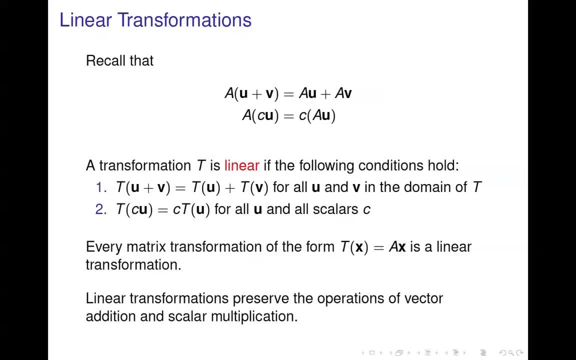 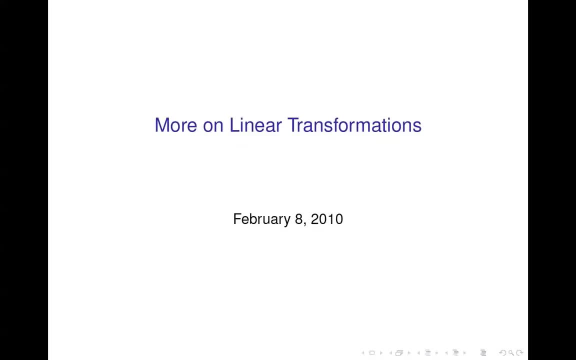 which will include more information on linear transformations. all right, we're going to start with more on linear transformations. let's suppose we have a transformation T and suppose that all you know about T is that the vector 1, 0 gets mapped to 2, 0, 1, and you know that 0, 1 gets mapped to this vector. so just 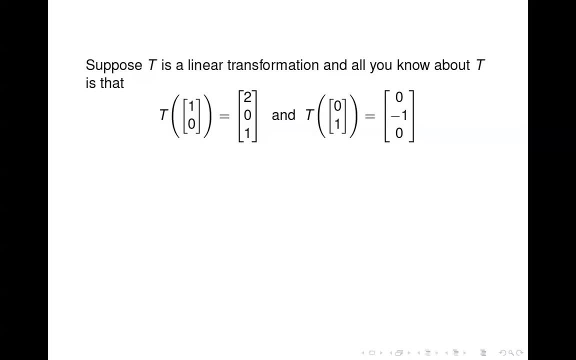 from looking at this, you can tell that T maps R 2 to R 3. so we're taking vectors in R 2 and we're mapping them to R 3, but how could we find a general rule for how to determine T? well, to Frage these 2, we need to. you know, all of this turns out once we go very 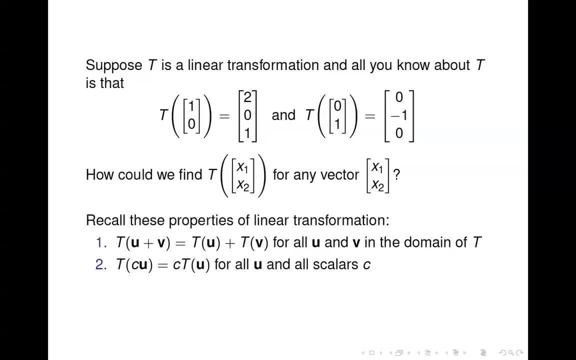 smoothly. is that the two characteristics? again, it is often used for the conversion that the GeSt of horse discussions and such kind of the ancient A idiot. So I thought I'd make an example here. first of all, Want a And t of a scalar times a vector. is that scalar times t of the vector? 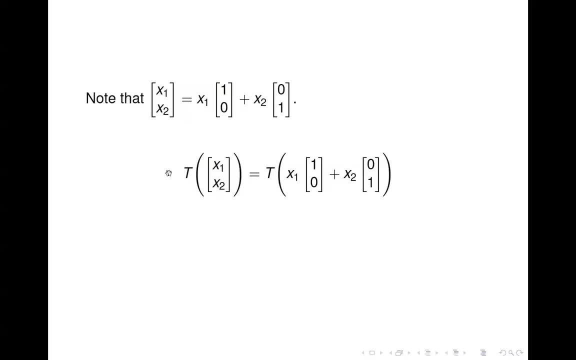 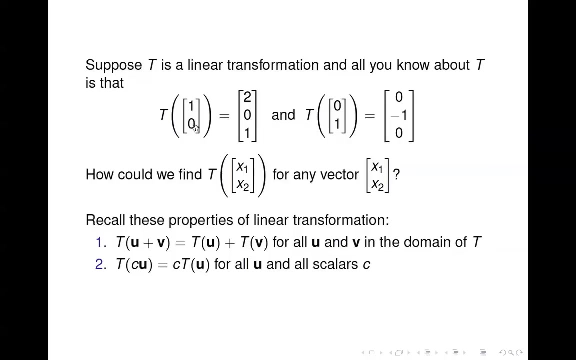 So let's examine what we have. Notice that we can write a generic vector x1, x2 as x1 times 1, 0 plus x2 times 0, 1.. Now remember on backwards, we know what we get when we apply t to 1, 0.. 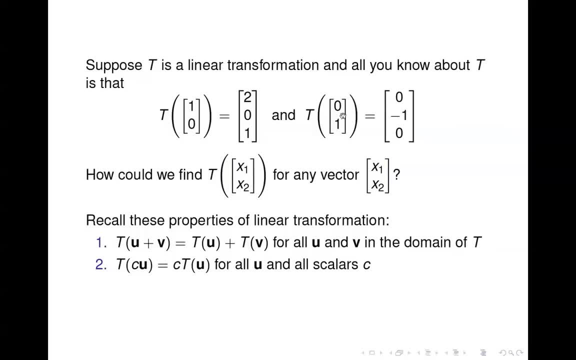 And we know what we get when we apply t to 0, 1.. So keep that in mind. So we're going to write x1, x2 as x1 times 1, 0, x2 times 0, 1.. 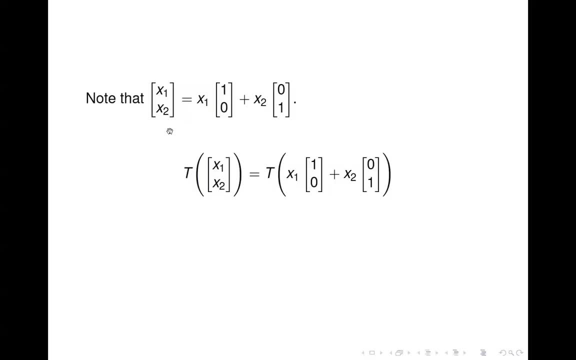 So then I'm going to apply t to both sides of this equation, So I'll have t of x1, x2 is equal to t of this stuff here. Now, since t is a linear transformation, t of this is like t of. 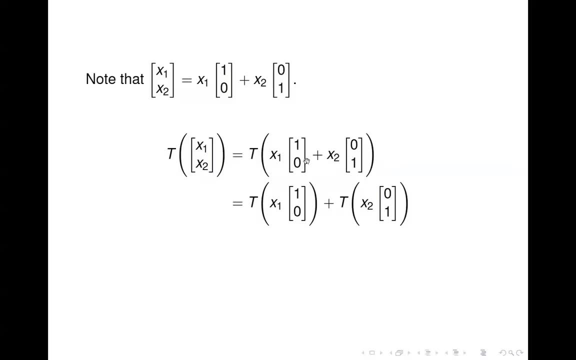 t of a, t of a, t of a, a plus or u plus v, if you want to think of it like that. So we can break it up into t of u plus t of v, And then this is like a constant times a vector. 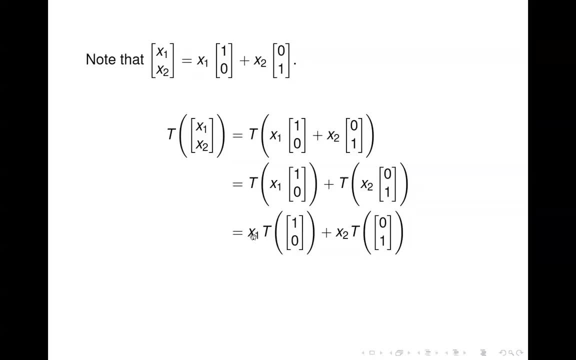 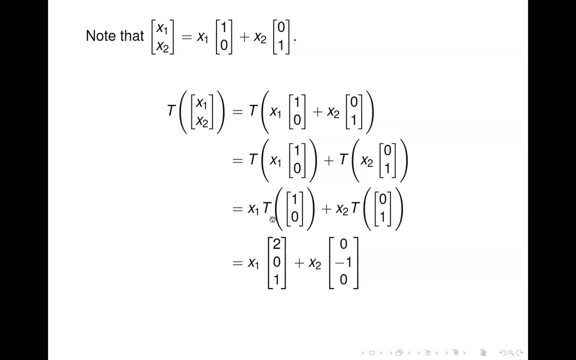 So t of a constant times a vector we can rewrite as that constant times t of that vector. Okay, so we end up with this And we know what t of 1, 0 is. It's just this vector. And we know what t of 0, 1 is. 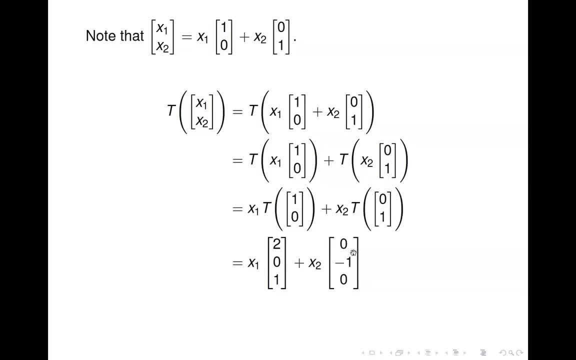 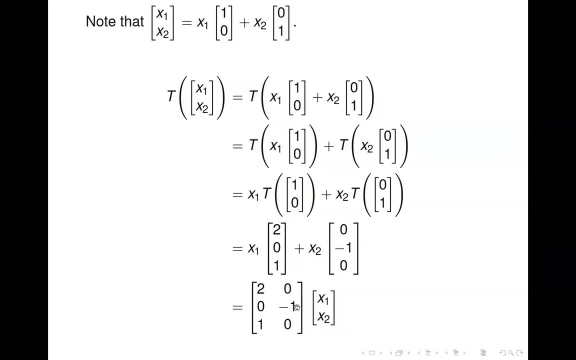 It's this vector. So here's what we end up with. And so notice, this is just a linear combination of these two vectors which we can rewrite in this form as a matrix, with those columns times the components x1, x2.. So notice that we've written t of x. okay, generic vector x as a times x. 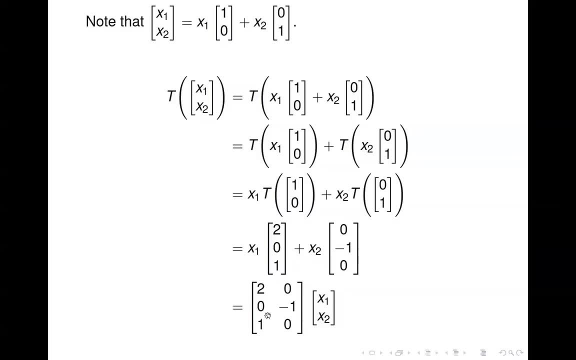 So now we have the matrix with which to apply the transformation And, as you can see, that matrix is simply the vectors that you get when you apply t to the vector 1, 0, and 0, 1.. All right now, those columns that we just looked at- 1, 0, and 0, 1, those are special vectors. 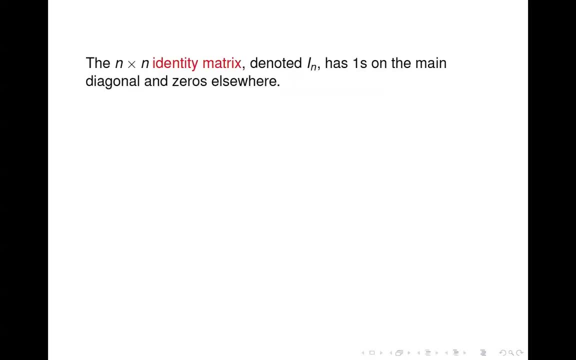 Okay, and to talk about that, let's first define the identity matrix. So the identity matrix, The identity matrix, is an n-by-n matrix, okay, so it's square and we write it as i sub n. okay, and it has 1s on the main diagonal. 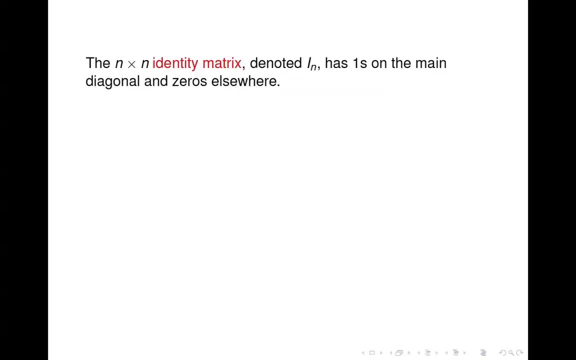 Main diagonal is the 1, 1 position. 2,, 2,, 3,, 3,, 4,, 4, okay, So it has 1s down the diagonal and 0s everywhere else. So here are a few examples. 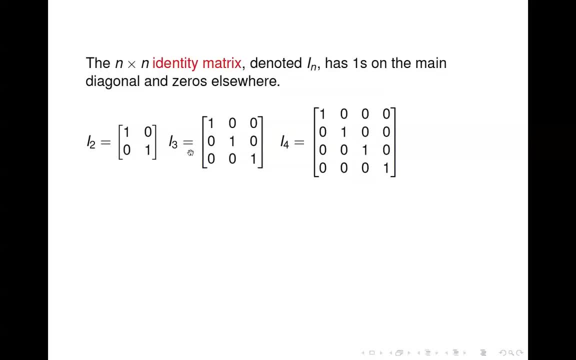 i2 is a 2-by-2, got 1s on the diagonal. i3 is a 3-by-3,: 1s on the diagonal, 0s everywhere else And here's i4.. Okay, so i sub n is just an n-by-n identity matrix. 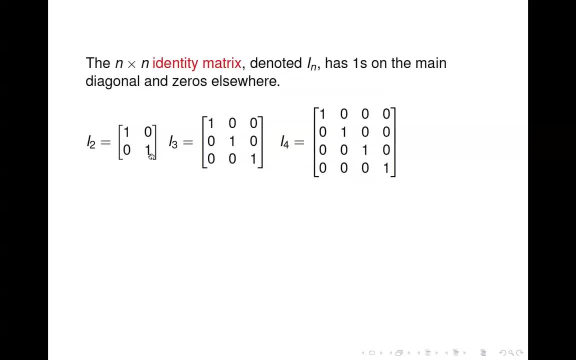 Now notice i sub 2.. You see those columns that we were just dealing with, those vectors 1, 0, and 0, 1.. So they are the columns of the identity matrix, Okay, and they are so special that we give them their own names. 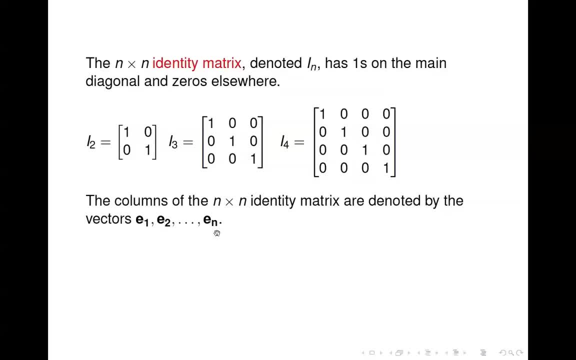 We call them e1, e2, so forth to e sub n, depending on what n is. So this column here would be e sub 1, this one e sub 2, and a 2-by-2 matrix Here for 3-by-3,. this would be e sub 1,, this e sub 2, this e sub 3, okay. 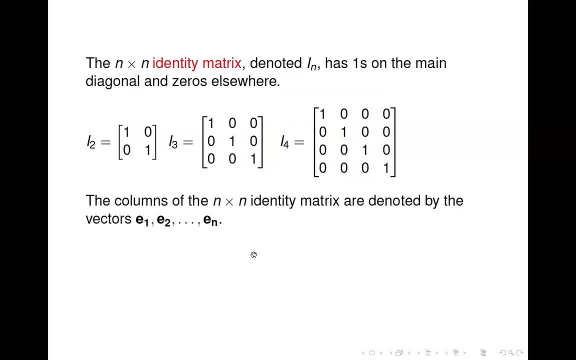 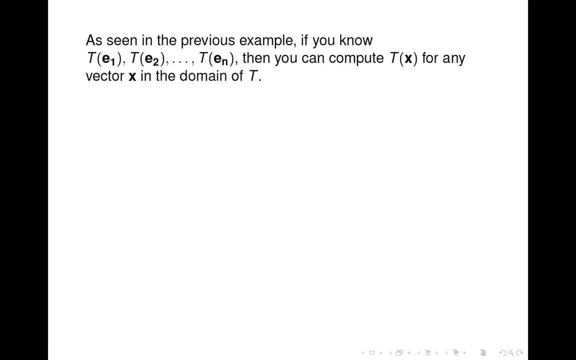 So the what they actually are depends on the size of the matrix that we're talking about. And there it is, with 2-by-2,. okay, Now, as we saw in the previous example, if you know, T of e1,, T of e2, and so forth. 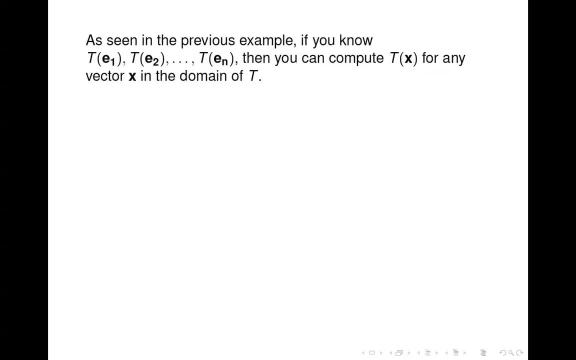 if you know what you get when you apply the transformation to these columns, you're going to get a 2-by-2 matrix. If you know what you get when you apply the transformation to these columns of the identity matrix, then you can compute T of x for any vector x, all right. 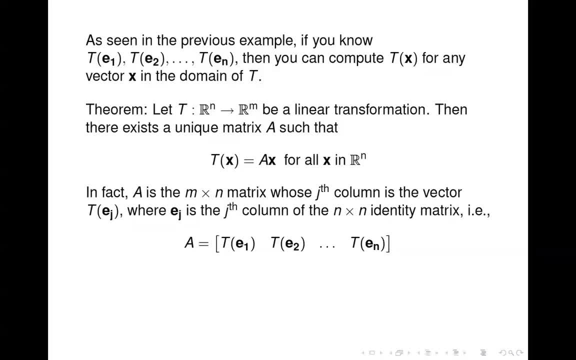 That's what we showed in that earlier example. Okay, so here it is written in a little more formal manner. We have T that maps Rn to Rm. Then there is a unique matrix, A, such that T of x equals Ax. In fact, A is the m-by-n matrix, whose jth column is the vector T of x. 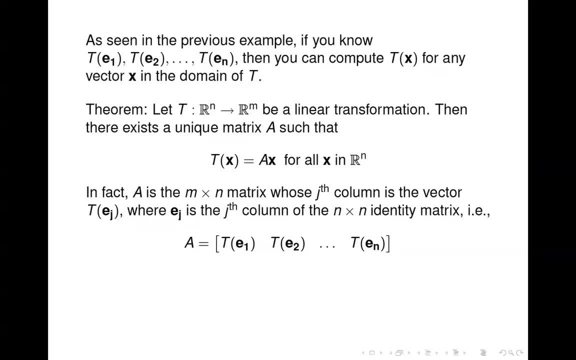 Okay, And so if you think back to the example we just did, this is exactly what we came out with. we came out with our matrix A was T of e1 and T of e2, because we had a 2-by-2. 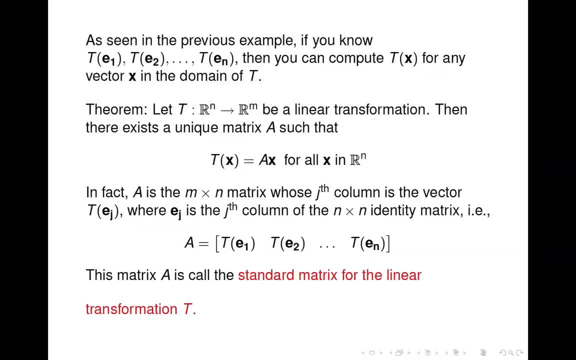 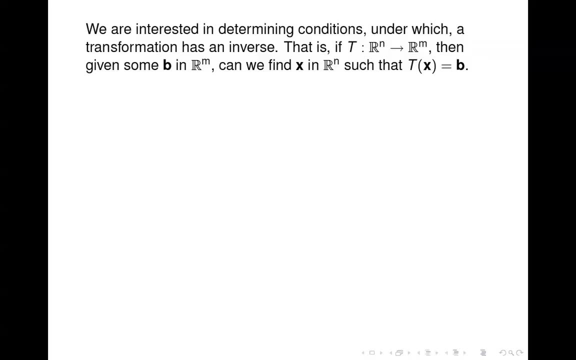 example: okay, This matrix A is called the standard matrix for the linear transformation T. okay, So it's a special matrix. Now We're interested in determining conditions under which a transformation has an inverse. okay, So that means if you have a transformation that maps Rn to Rm, then given some b in 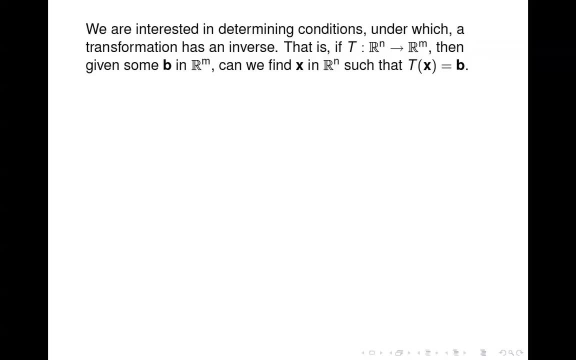 Rm. can we find an x in Rn that maps to that b? Or can we find x, such that T of x equals b? Okay, All right. Well, let's go back to our function, And we're going to look at some functions, just defining real numbers first of all. okay, 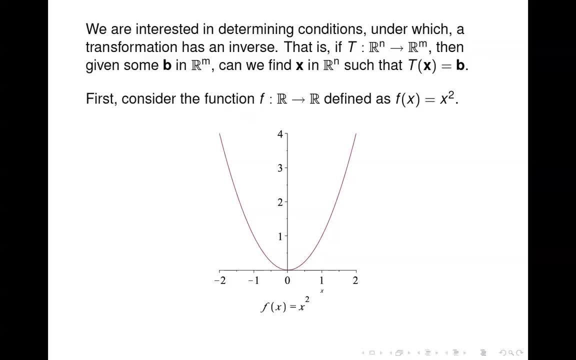 So, before we looked at the function F of x equals x squared right. So, and this is what it looks like Now, a couple of things to notice. One is that you never get a negative number right When you plug in any x, no matter what x you plug in. since we're starting with real numbers, 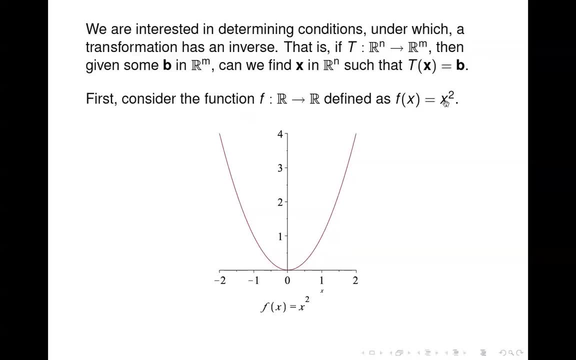 it's a number. what real number? x you plug in, you always get a non-negative value. guys, keep that in mind And also note that we can get the same y value. so if I drew a horizontal line I would hit a couple of places on this graph. 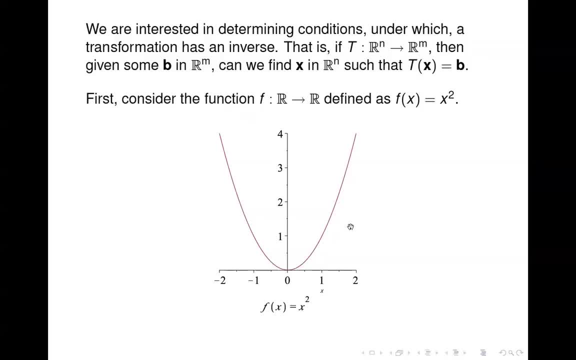 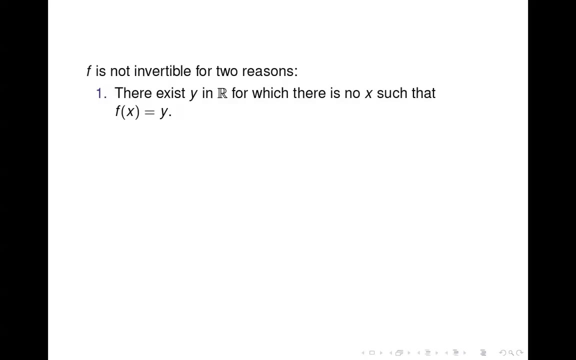 So for a given y value, we've got a couple different x values that can produce that y value. So keep that in mind. Alright, f? f of x equals x squared. that we just looked at is not invertible for two reasons. 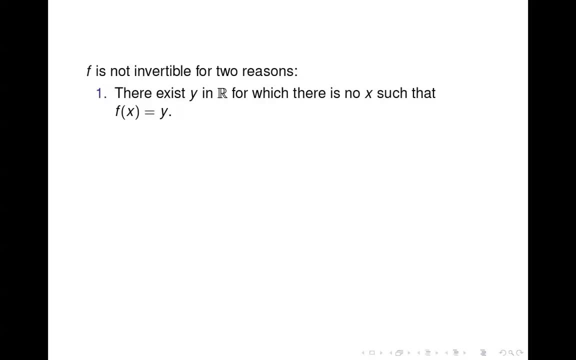 One. there exists y in R. so there's some real numbers for which there's no x, such that f of x equals y. There's no x such that x squared equals y. So consider y equals negative. 1. We cannot come up with a real number x. 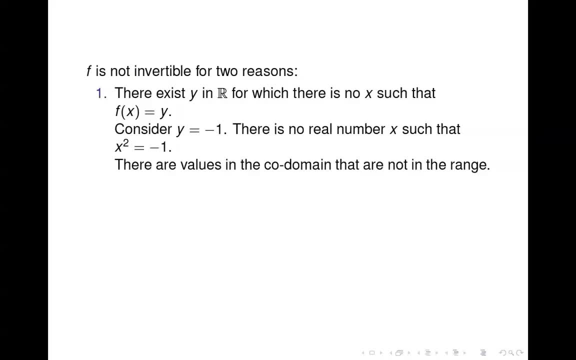 Such that x squared equals negative 1. That means that there are values in the co-domain that are not in the range. The co-domain here is the real numbers, but the range for this function is all non-negative real numbers, So we can never get a negative number when we apply this function. 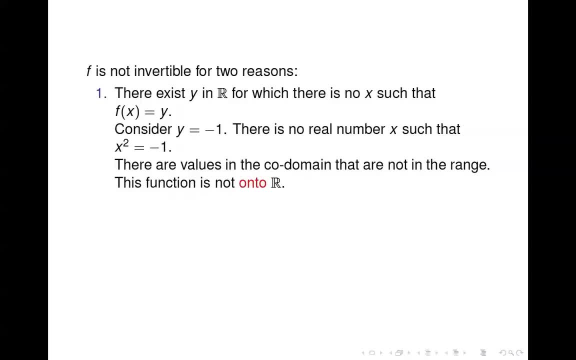 So we say that this function is not onto the real numbers. There are real numbers that don't get mapped to. Alright, so I'm going to define that term in just a minute, but I want to give you an example of something that's pretty easy for you to grasp. 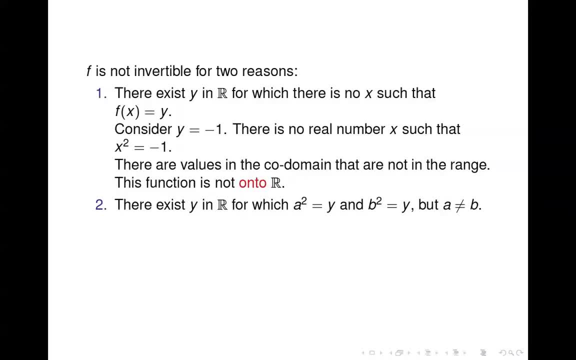 So I said f is not invertible for two reasons. Here's the second one: That there exists y in R. Okay, There are real numbers, y, for which a squared is y and b squared is y, but a and b are not. 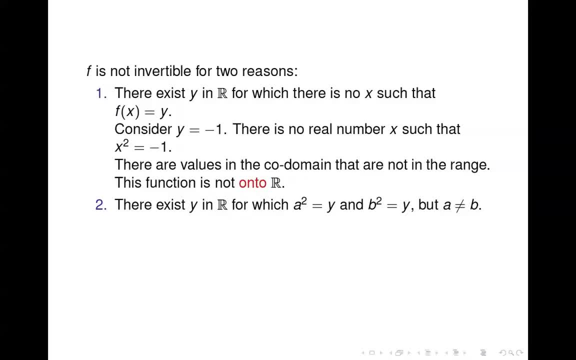 equal. Okay, That, and that's that horizontal line thing I was talking about earlier. So, for example, if y is 4, we can get that with 2, because 2 squared is 4.. We can also get there with negative 2, because negative 2 squared is 4.. 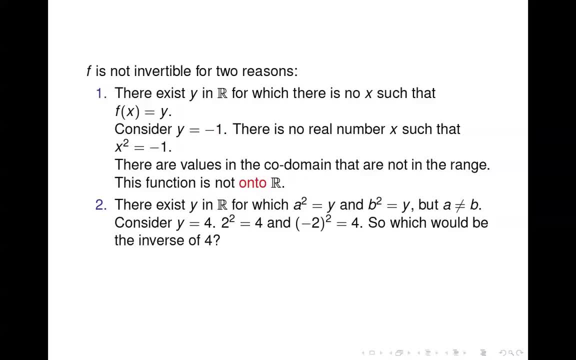 So if we were trying to get an inverse right, if we started with 4 and we wanted to know, how did we get there? well, we don't know, because it could have been from 2, or it could have been from negative 2.. 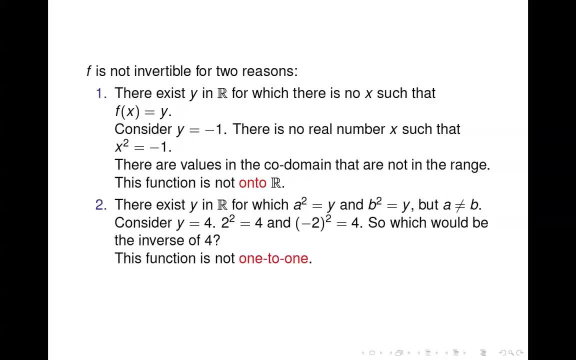 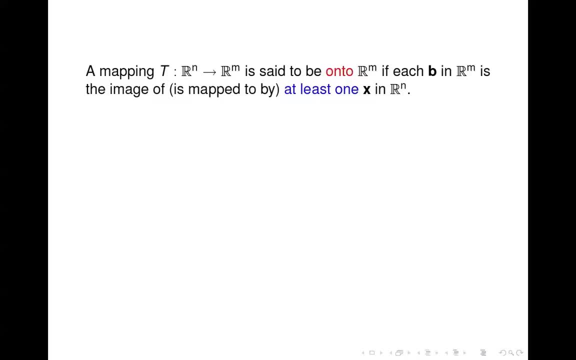 So we say that this function is not 1 to 1 because of this reason. Okay, so here's a little more formal way to look at it. We say: a transformation from Rn to Rm is onto Rm, right onto the codomain, if each b in 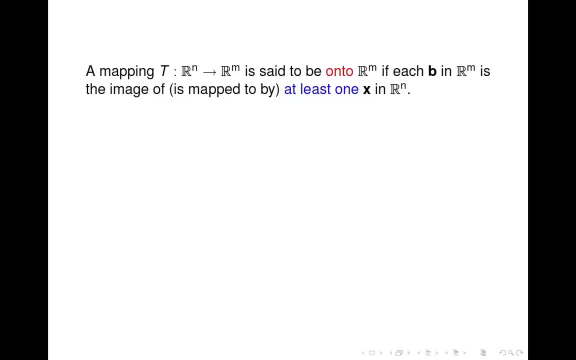 Rm Is the image of or another way to think of it is is mapped to by at least one x in Rn. So every b in the codomain is mapped to by at least one x in the domain. So every b gets mapped to. 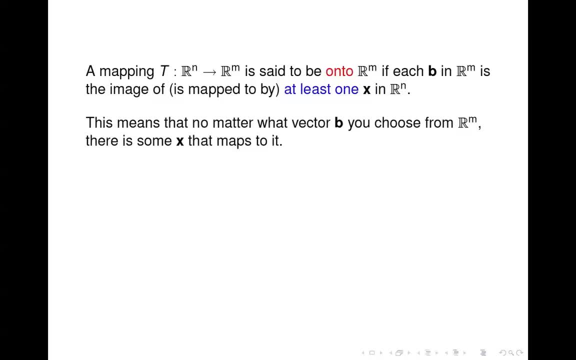 Okay, so this means that no matter what vector b you choose from Rm, there's some x that maps to it. So for every b in Rm there's some x, such that t of x equals b. And since t of x equals a times x, this means that for every b there's some x, such that. 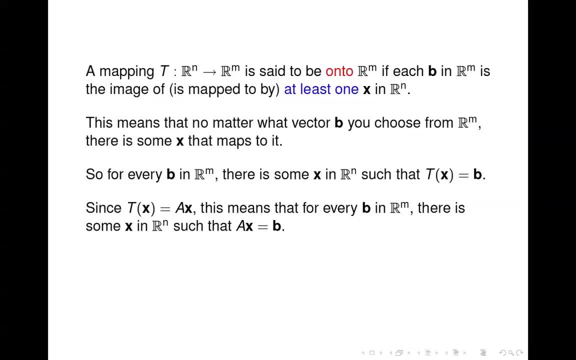 a times x equals b, right? If there's an x such that t of x is b, then it has to be the same x. that makes a times x equal b. All right now. when is it true that, no matter what right-hand side you have, you have to? 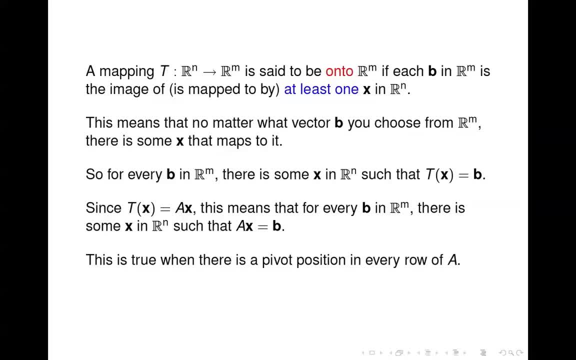 have. uh, you'll always have a solution. Well, that's true when you have a pivot position in every row of A. Okay, so if there's a pivot position in every row of A, then the transformation will be onto. Okay, let's talk about one-to-one. 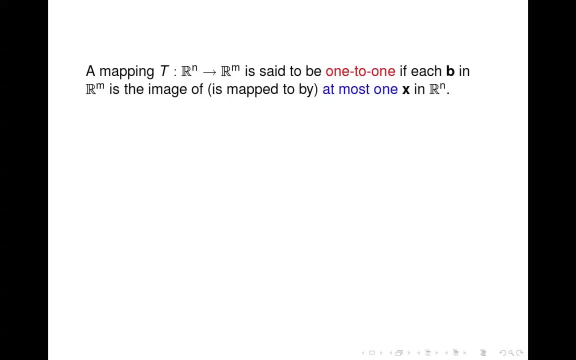 Transformation from Rn to Rm is said to be one-to-one if each b in Rm is the image of or is mapped to by, at most one x in Rn, At most one. So remember back to the function: f of x equals x squared. 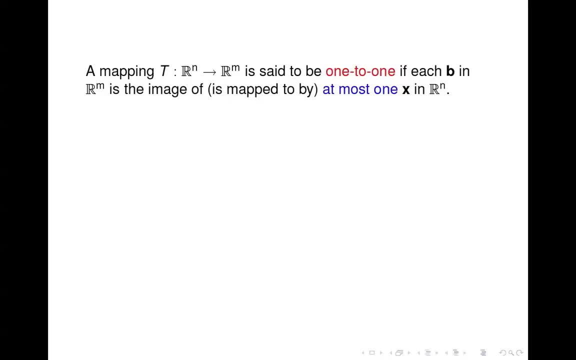 This wasn't true, because you could get to four from two and from negative two. So there was an element in the range that was mapped to by more than one element in the domain. So it wasn't one-to-one. Here, One-to-one means each b in Rm is mapped to by at most one x in Rn. 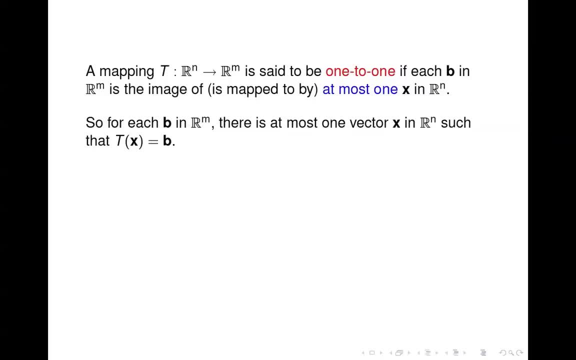 So that means that for each b in Rm there's at most one vector x, such that t of x equals b. All right, so that means that um, since t of x equals Ax, if we look at the system, Ax equals b, it can't have an infinite number of solutions, because then there would be more. 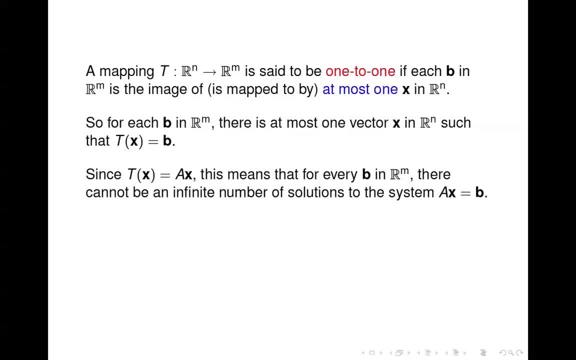 than one x that maps to that b. And if our system can't have an infinite number of solutions, that means it can't have free variables. Okay, So Ax equals b can have no free variables, And if it has no free variables, that means there must be a pivot position in each column. 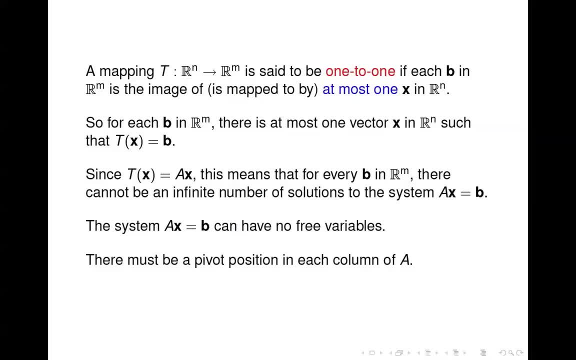 of A. All right, So the transformation is one-to-one. If there's a pivot position in each column of A, All right, So one-to-one. there's a pivot position in each column Onto, there must be a pivot position in each row. 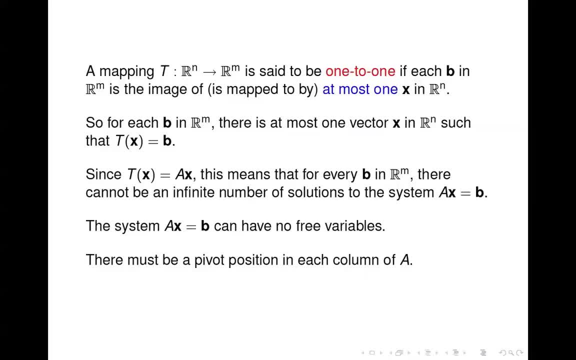 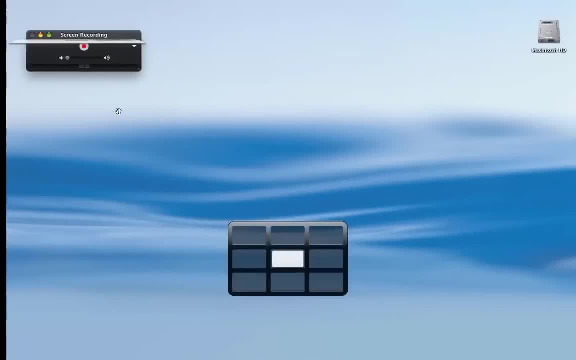 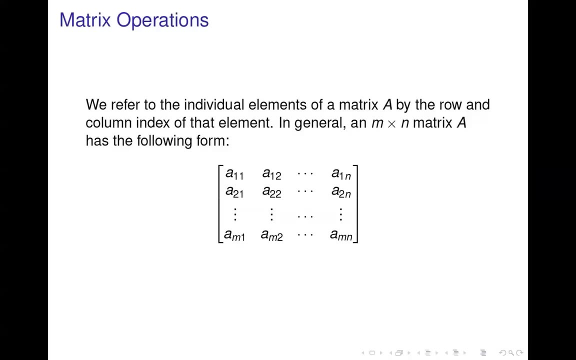 Okay, So that's how you can keep straight one-to-one and onto. This is section 2.1.. Um On matrix operations. just some um basics out of the way. first, um we refer to uh, an m-by-n matrix, A uh as a matrix with m rows and n columns, and uh the individual. 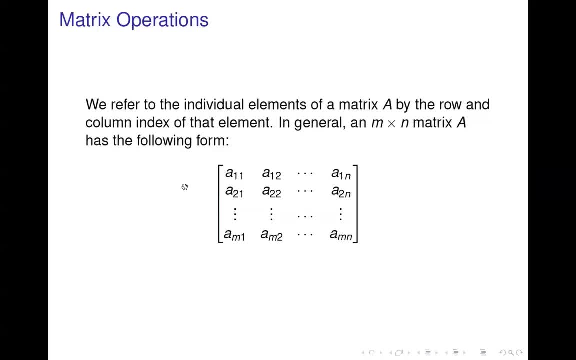 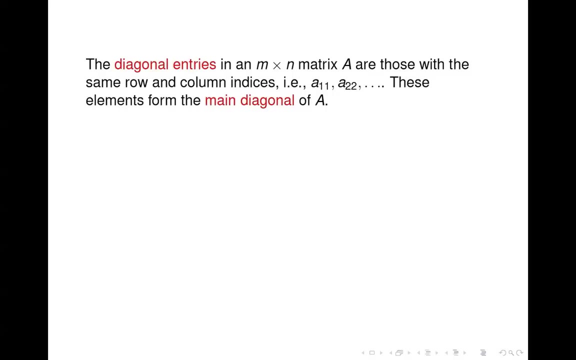 elements in the matrix we denote by uh. lowercase a with a subscript um ij, where i is the row index and j is the column index. Okay, The diagonal entries uh in a matrix A are those where the row and column indices are. 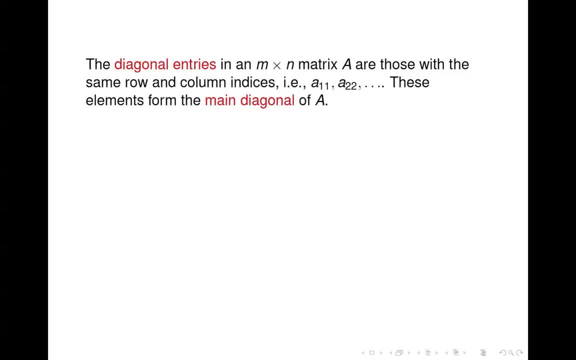 the same. So, like a11, a22, and so forth, These elements we call the main diagonal of A Um. a diagonal matrix is a square matrix where all the entries off the main diagonal are zero. So the only place you can have non-zero uh values is on the diagonal. 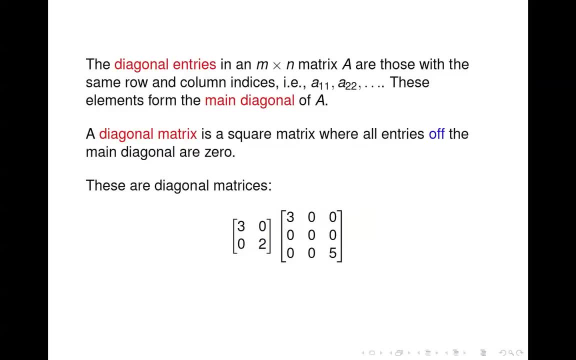 So here are a couple of diagonal matrices. Notice that the, the key is off the diagonal um, you have all zeros. So the main diagonal is just uh, uh, 1, 1,, 2, 2, and so forth, um 3, 3 in this case. 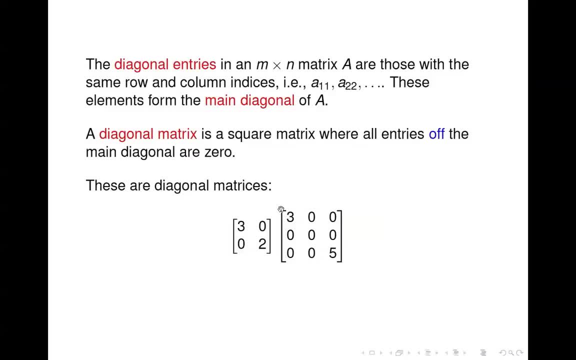 So off the diagonal, off the main diagonal, you have all zeros. It's okay to have a zero, Okay, Okay, Okay, Okay. So on the diagonal, we really don't care what's on the diagonal, We just want zeros off the diagonal. 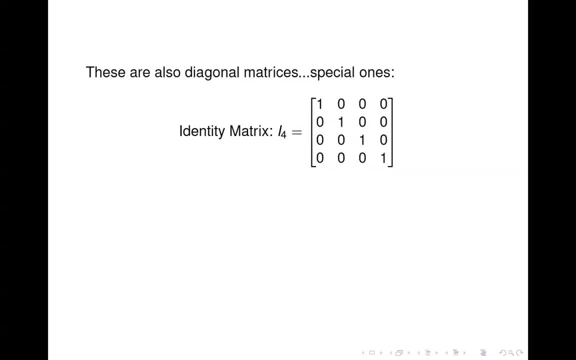 Um, here's another uh diagonal, uh matrix. This one has uh a name: We call it the identity matrix. So it's a um diagonal matrix, because everything off the diagonal is zeros. And uh, the zero matrix is uh technically a diagonal matrix, because everything off the 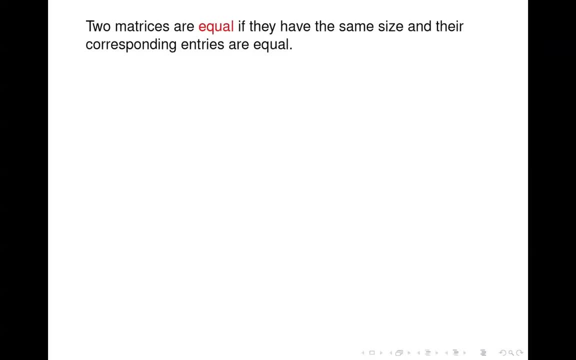 main diagonal. So it's a uh diagonal matrix, because everything off the diagonal is zero. We say that two matrices are equal if they have the same size, so the same number of rows, same number of columns and their corresponding entries are equal. 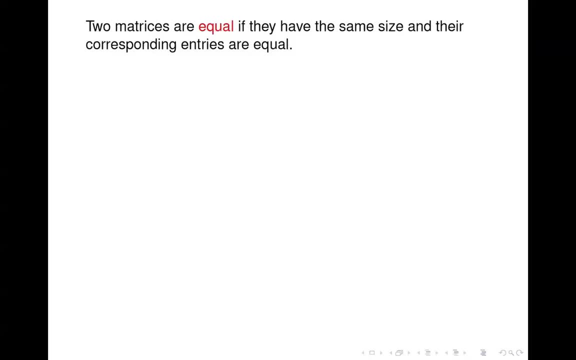 So the 1, 1 entry in one is equal to the 1, 1 entry in another. In general, the ijth entry in one is equal to the ijth entry in the other. We can compute the sum of two matrices. 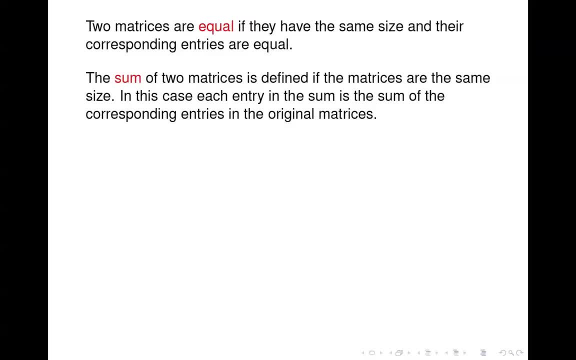 We can add two matrices together. Um, this is defined if both matrices are the same size. so you have to have the same number of rows and same number of columns And in this case, uh, the uh. ijth entry in the sum is just uh, the sum of the ijth. 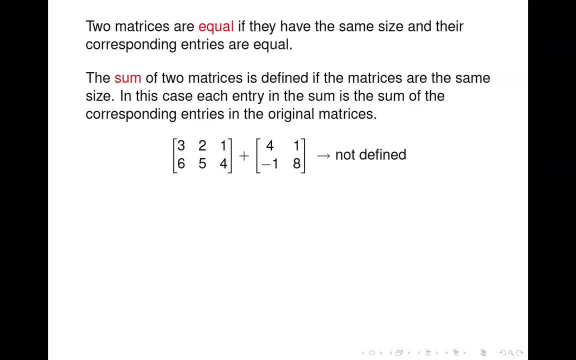 entries in each of the original matrices. Um, so here's an example, one that, uh, this sum cannot be computed because these matrices are not the same size. Um, here's one where we can't compute the sum and notice, uh, the 7 here is just the. 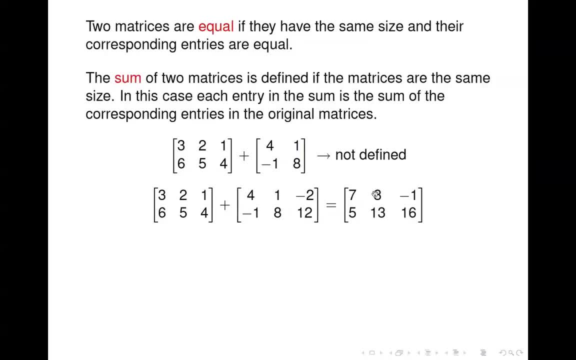 3 plus 4,. uh, to get the 3,, it's this 2 plus 1, and so forth. So to get uh the ijth entry over here you sum the corresponding ijth entries in the two original matrices. 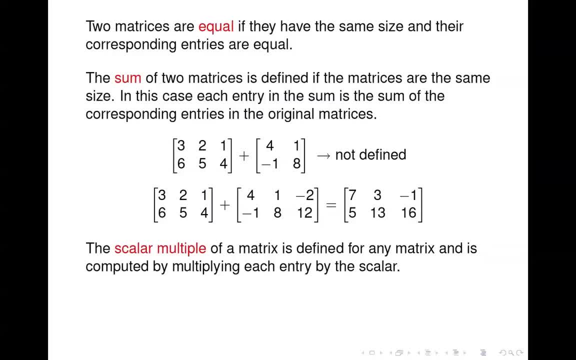 We can compute the scalar multiple of a matrix In the same way we compute the scalar multiple of a vector. we just multiply each entry by that scalar. So here's an example: multiply 3 times each entry in this matrix and, uh, we produce. 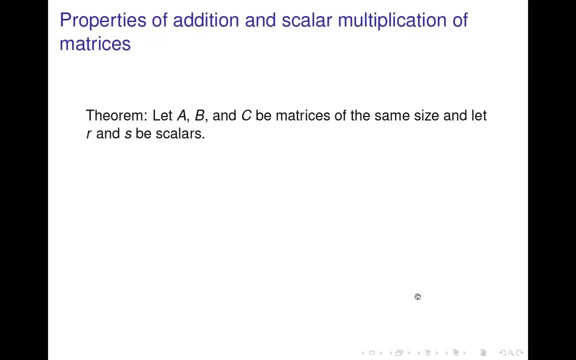 uh, this one, Uh, your book lists some properties of addition and scalar multiplication of matrices. Um, The first three, uh, Uh, regarding uh, addition, So, um, you'll find that, since addition of matrices is is defined essentially the same, 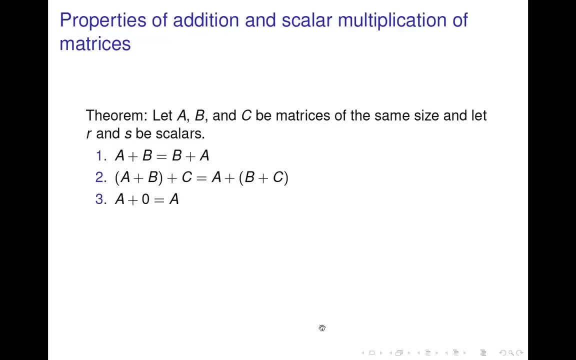 as addition of real numbers, then a lot of those same properties carry over. So a plus b is b plus a, Uh. the second one, um, allows you to um associate the parentheses uh, as you'd like. So that's the associative property. 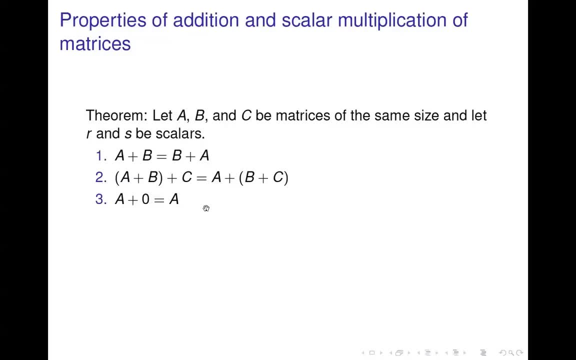 And, uh, If you add the matrix to the zero matrix, uh, you get the same matrix back. Then the. the last three are regarding scalar multiplication And essentially, um, they say that you can uh kind of stick the scalar wherever you'd. 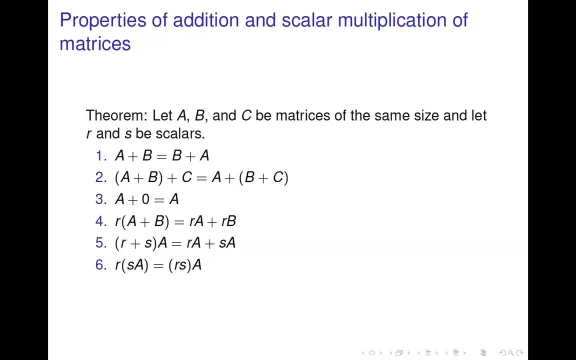 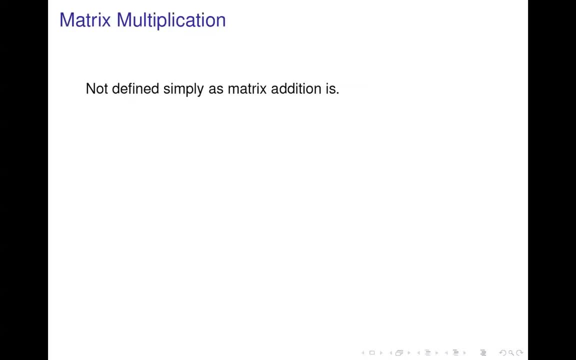 like to, wherever it's convenient, um um it. it all is uh equivalent. Okay, Let's move on to matrix multiplication. Okay, So matrix multiplication is uh not defined um simply as matrix addition is. 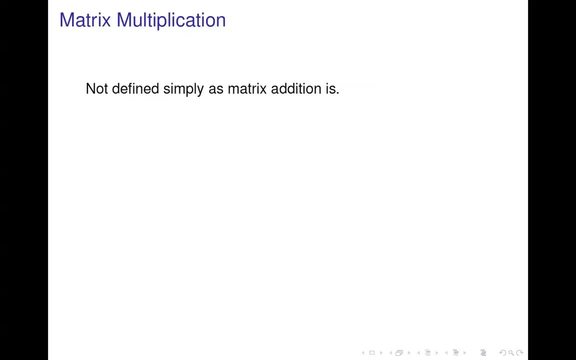 Um, it's a little more complicated. It's not just multiplying the corresponding entries together. So here we go, Um, if a is an m by n matrix and the sizes are important here, um, so suppose a is m by n and b is n by p. 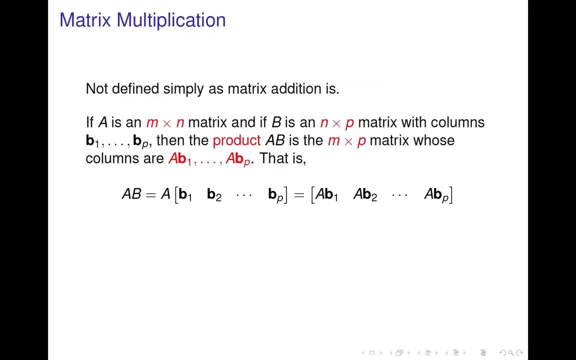 Okay, So that's the key. Um, The number of columns in the first has to equal the number of rows in the second for the product to be defined. Okay, Um, so if you have that situation, uh and uh, we say that the columns of b are b1 through. 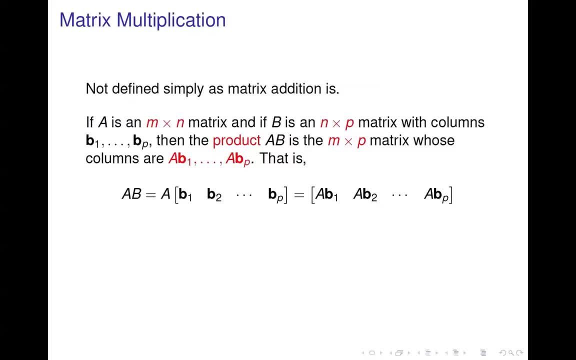 bp. then we define the product ab as the m by p matrix And notice that the m is the number of rows in a, p is the number of columns in b. So, uh, we kind of always look to see if these inner dimensions match up. 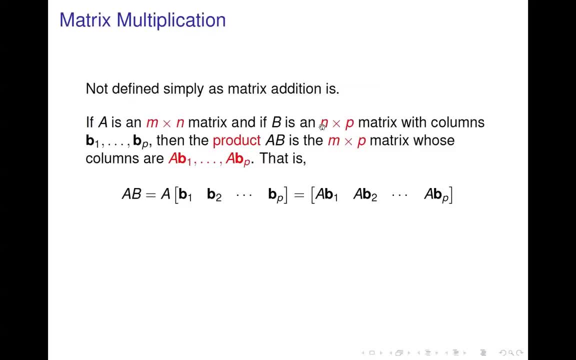 So the n here matches up with the n here, And that means the product is defined and then the the product itself, the dimensions of it will be the first, uh the number of rows, which is m uh by the number of columns. 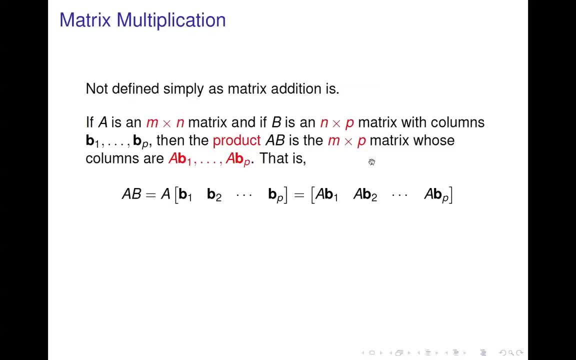 of of b, So it will be m by p. Okay, So how do we compute a times b? Well, we're going to compute a times b, Okay? Well, notice what this is. It's the m by p matrix, whose columns are a times b1 out to a times bp. 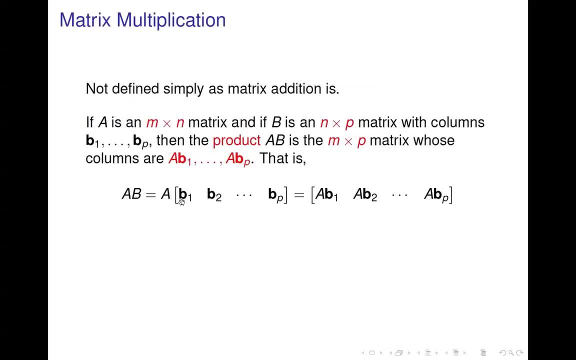 That is um, we want to multiply a times b and we look at it as a times each of the columns of b. Okay, So the first entry, the first column of the product, is a times the first column of b. The second column of the product is a times the second column of b. 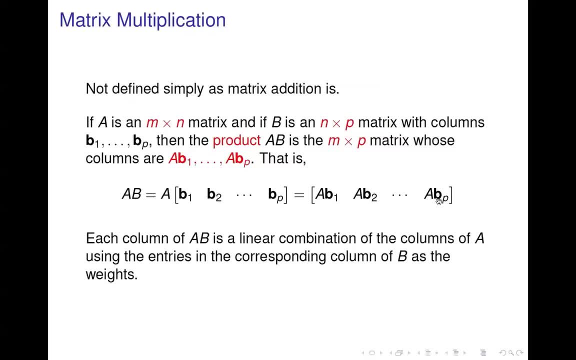 And so forth. So notice that each column of the product, each column of ab is, is of the form a times b1 or a times b2.. And we know that that when we compute a times some column, then we are taking a linear combination. 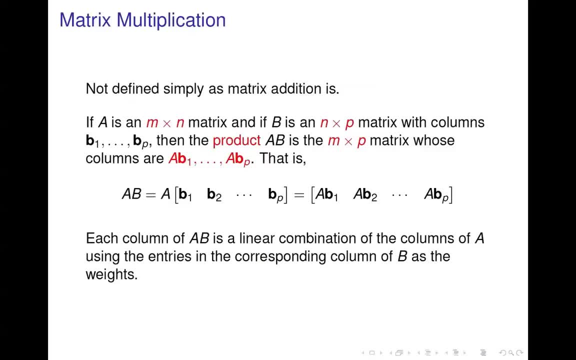 of the columns of a using uh, the entries in the vector as the weight, To get the first column of a times b. we're taking a linear combination of the columns of a using the first column of b as the weights To get the second column. another linear combination of the columns of a using the entries in the: 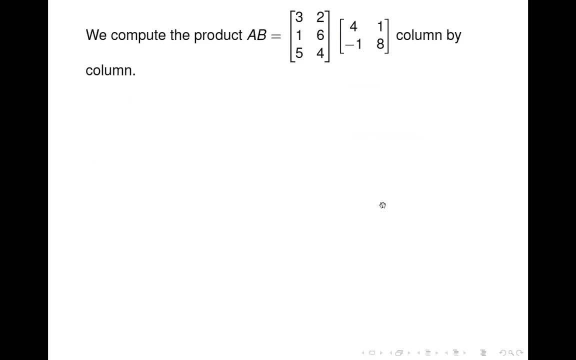 second column of b as the weights and so forth. Okay, So if we want to compute uh the product ab uh, where here are matrices a and b, then we're going to do it as I just described First. uh note that a is a three by two matrix and b is two by two. 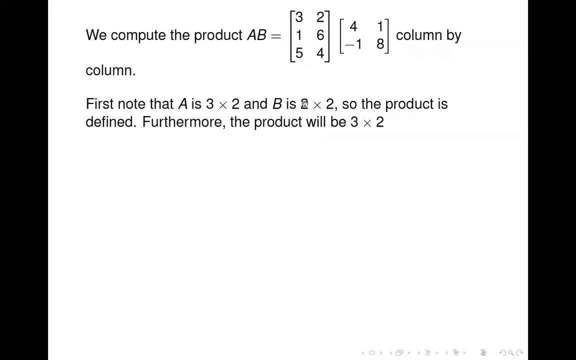 So we check to see if the two here matches up with the two here, which it does, And then we look at the outer dimensions, the three and the two, and that will be the uh dimensions of the product. So our product will be three by two in this case. 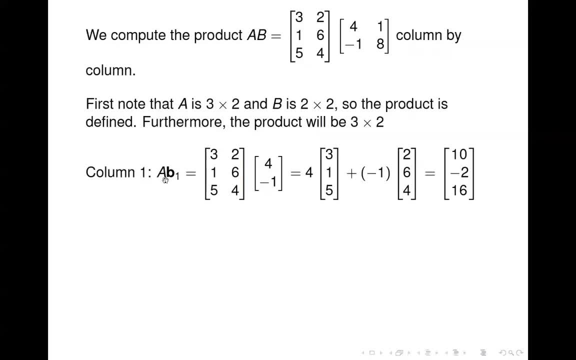 All right To get the first column of the product. it's a times the first column of b. So here's a first column of b, four negative one, and this is just a linear combination. So four times the first column of a, minus one times the second column. 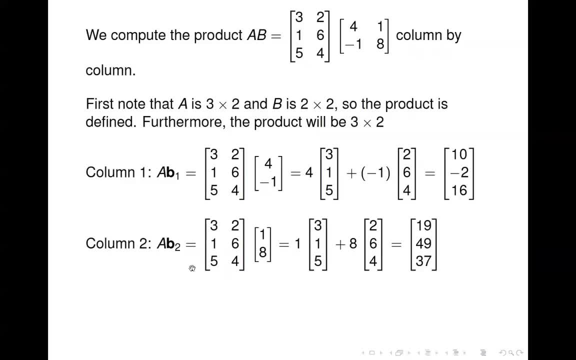 And, uh, this is what we get. Do the same thing to get the second column of the product. It's a times the second column of b. Second column of b is, uh, one eight. So we take that linear combination: one times this first column of a, plus eight times the. 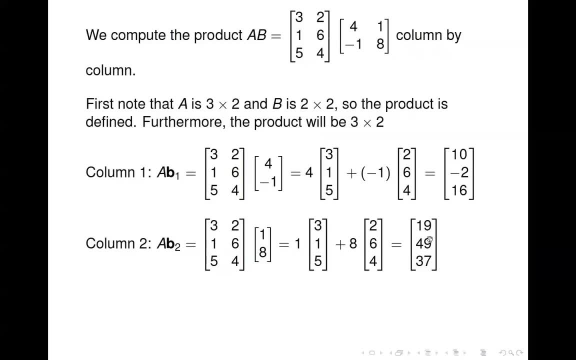 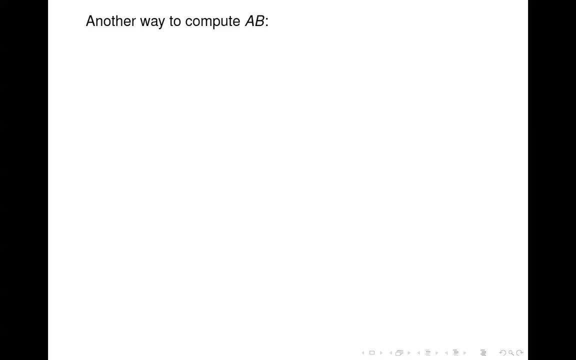 second column. Do that linear combination And now we have our first uh and second columns of the product And uh, so we're done. There is a times b. Um, there's another way to compute a b. 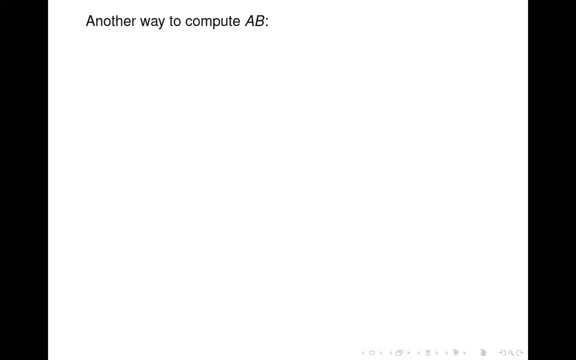 Probably most of you learned this when you took algebra college, algebra probably Um. notice, uh, that it's defined in terms of inner products. All right, So the ij3.. The ijth entry in the product a b is the inner product of row i of a, with column j. 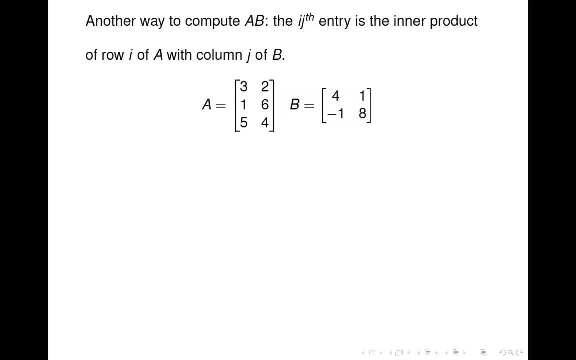 of b. So let's see how that works. So this is back to our same a and b And to get the one, one entry in the product, um, then it's going to be row one of a times, uh, column one of b. 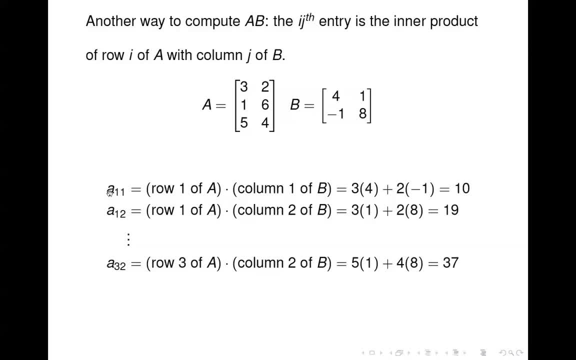 Actually these are uh, three columns, Uh, Uh, Uh Should not be a's, It should be the product. I'm talking about the product here. So row one of a times, column one of b, um, do that inner product. 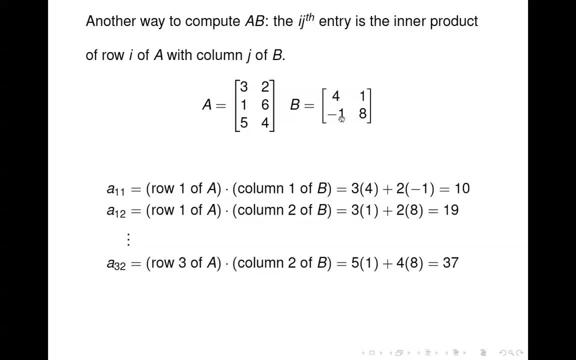 So it's going to be three two, inner product with four, negative one, to give you ten in this case, And so forth. So to get to the three two, entry of the product, it's row three of a times, column two of b. 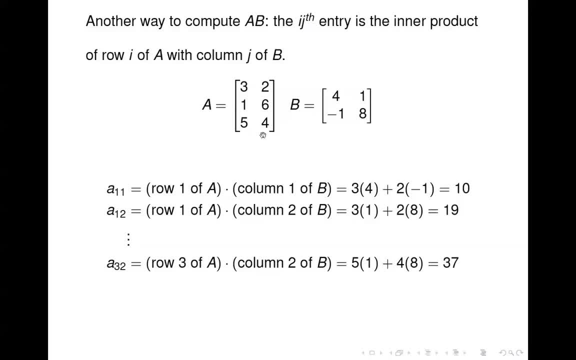 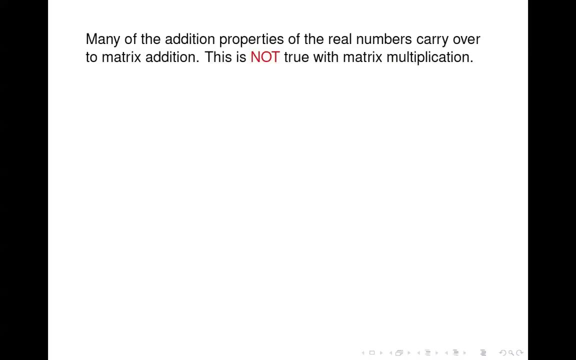 Okay, Okay. So five times one plus four times three times 8, and gives you 37, and so there you go, you have the same matrix as we ended up with before. okay, now you should note that, since matrix multiplication is is not defined simply because not a simple operation like matrix addition is, 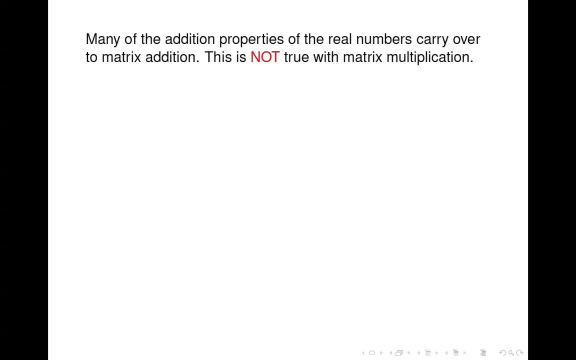 then properties of real numbers that apply to addition multiplication do not follow over to matrix multiplication. you know they did with matrix addition, they don't with matrix multiplication. so some warnings: if you're dealing with real numbers, a times B equals B times a. that does not hold true for matrices, matrices. 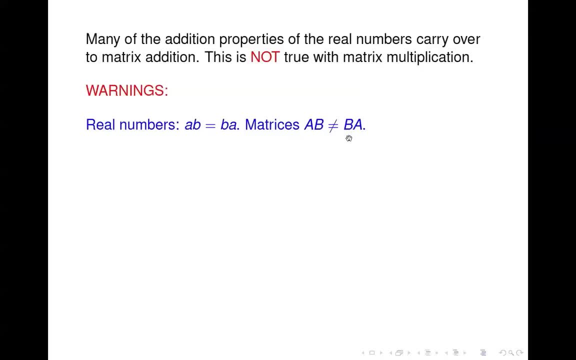 a times B is not necessarily equal to B times a. of course it sometimes could be, but in general a times B is not equal to B times a. one thing, one reason is that sometimes they're not even both defined. right, not even both defined. maybe you can multiply. 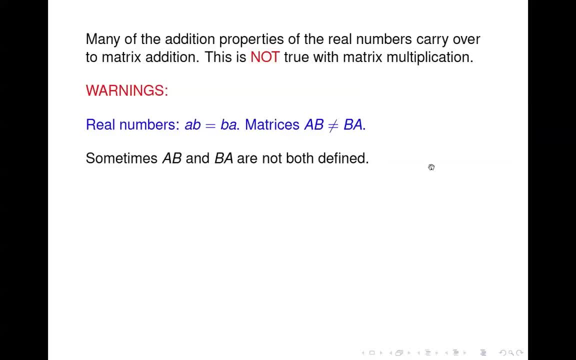 a times B, but you might not be able to multiply B times a and vice versa. however, even if they are both defined, you can't guarantee they'll be equal. so here's an example, here's a matrix: a times B. and we get this product if we reverse the order. 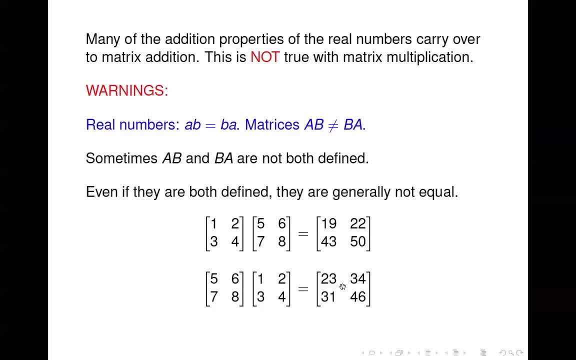 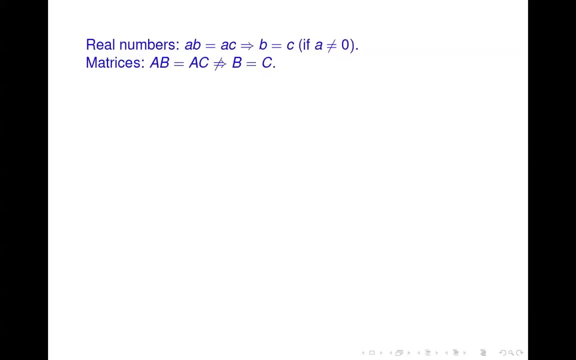 multiply B times a, we get a totally different matrix. so just because you can multiply both, compute both products, that doesn't mean that they'll be the same result. so don't make that mistake. second warning for real numbers, if you know that a times B equals a times C, 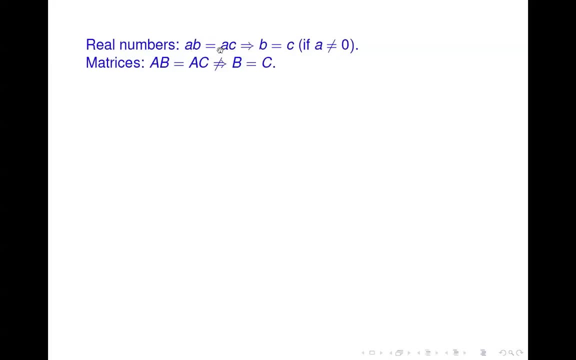 and you know that a is not equal to zero. you can divide both sides by a and end up with B equals C. can't do that with matrices. if a B is a C, that doesn't mean that B equals C. okay, here's an example that. here's a matrix: a a times B is. 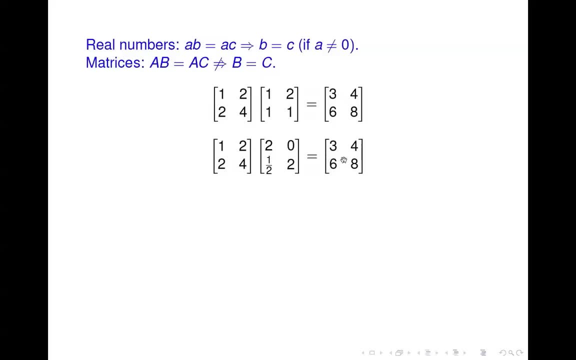 this matrix. here's a times C. get the same matrix, but B and C are clearly different. and another one, the last warning for real numbers: if eight times B is equal to zero, you can assume that either a or B is equal to zero, or perhaps both are. 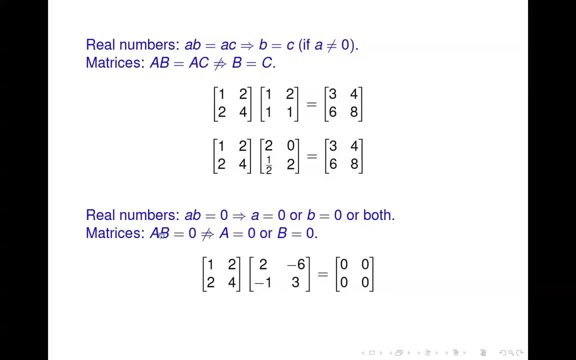 equal to zero, not true for matrices. you've have product of two matrices that equals the 0 matrix. that doesn't mean that a or B is equal to the zero matrix. and here's an example left. here's matrix A times B and we end up with a zero. 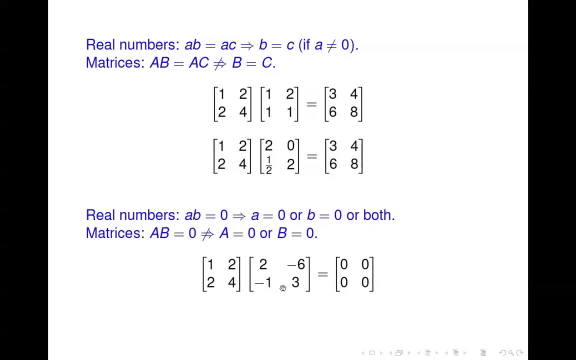 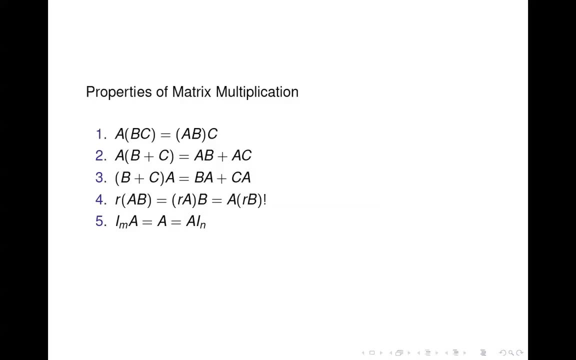 matrix, but neither these is equal to the write matrix, zero matrix, far from it, in fact. okay, some properties of matrix multiplication, that you have the associative property, so you can move the parentheses around, but notice that the order that the matrices appear is unchanged. okay, so we. 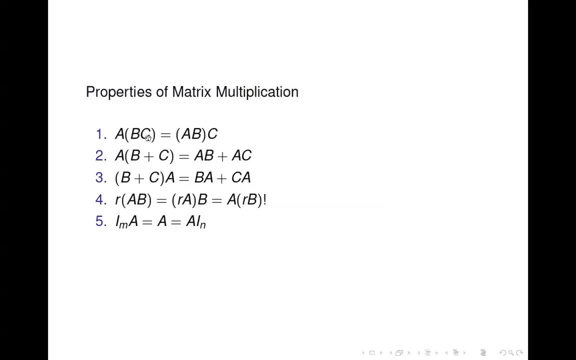 can't move the. we can't change the order that the matrices appear. can change the order in which we do the multiplication. we can distribute either from the left or from the right here in numbers, two or three, oops. and if we have a scalar we can move it wherever we'd like, and apparently I thought that was quite a. 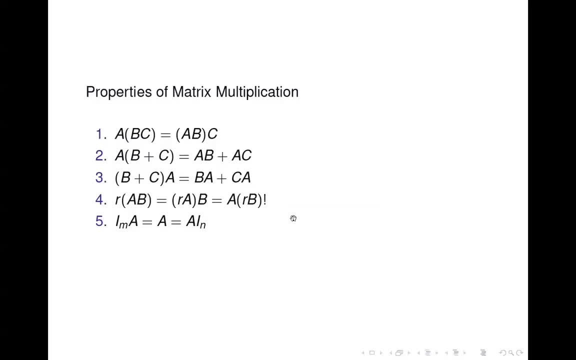 important thing, since I've been an exclamation mark there and any matrix multiplication by the identity has just itself now notice that I'm assuming a is m by n here, so if I multiply on the left I have to multiply by the m by m identity, whereas 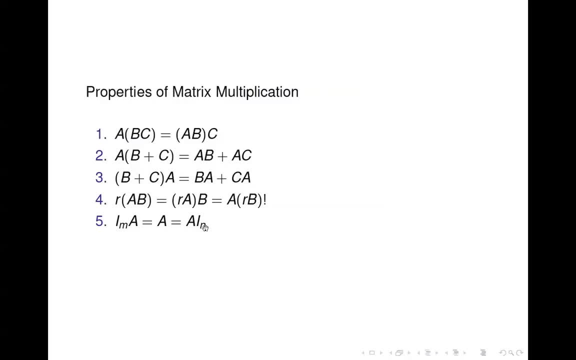 if I multiply on the right, I have to multiply by the n, by n identity. okay, one other thing: the transpose of a matrix is computed by taking the, the, the きた, and attribute the that trivia to. so, for example, I'm partecipate in the matrix A shown here. 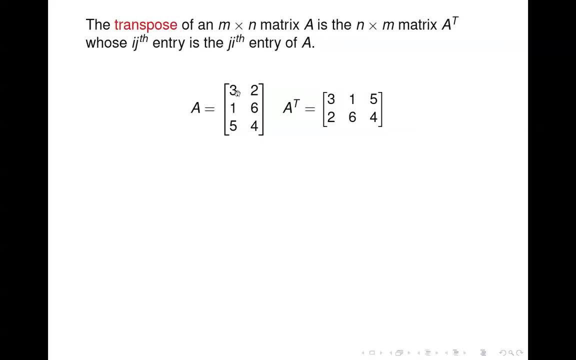 and I measured the entrance to the c c with the one two entry and that goes to the one two entry that turns out to be a three to so and so forth. Then that perhaps an easier way to go is of the columns of A, Because the rows of A transpose. 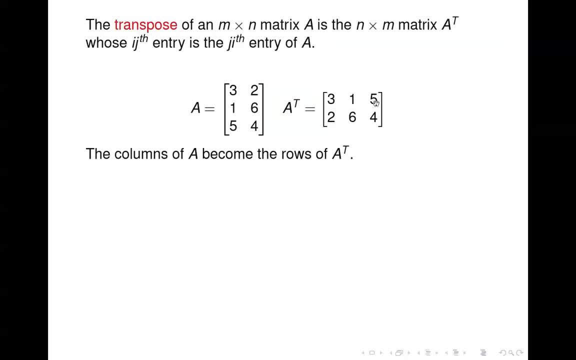 so that's column read three, one, five column and three operations transpose: 3, 1, 5 and so forth. or alternatively, the rows of a become the columns of the transpose. so here's a row first row here: 3, 2. first column here: 3, 2. 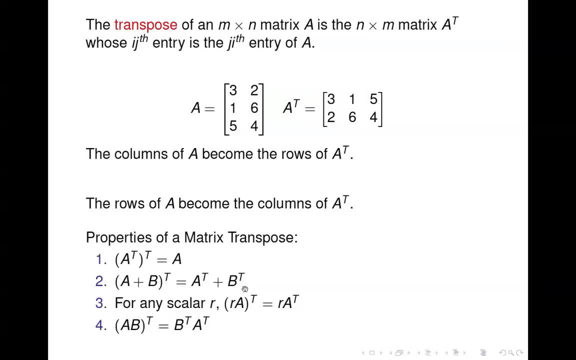 and so forth. some properties of the transpose: if I take the transpose of the transpose of a matrix, I'm back where I started. you can look here. if I take the transpose of this matrix, then I end up with a row. one here becomes column 1 of. 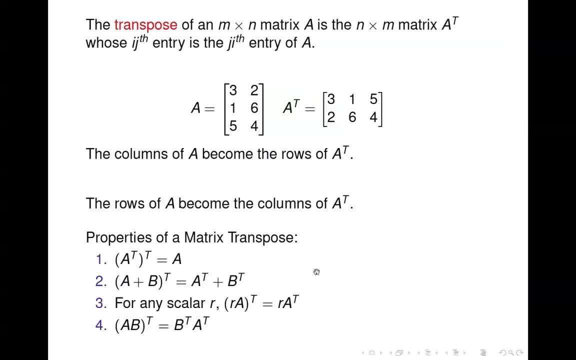 a and so forth. so the transpose of the transpose is the original matrix. transpose of a sum is the sum of the transposes. number two if you move a scalar around. number three, number four, kind of interesting. if you want to take the transpose of a product, that is the product of the 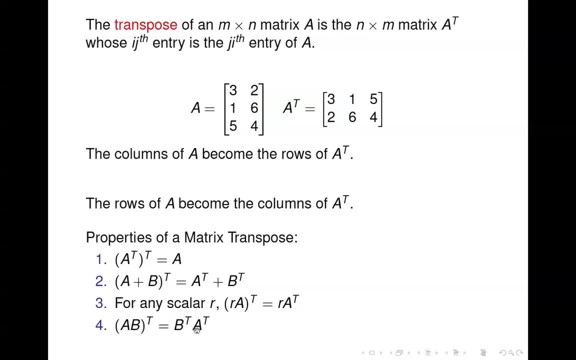 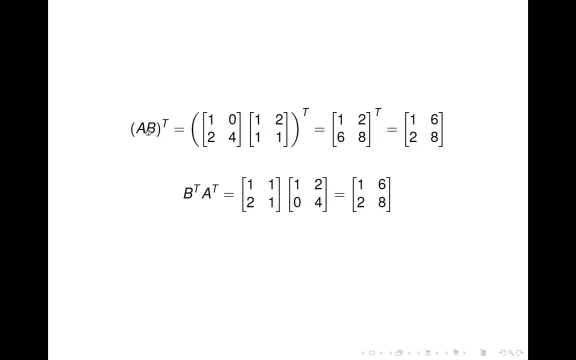 transposes, but in reverse order. okay, reverse order. so here's an example of that. if I want to compute the transpose of a product, A, B, all right. so here's A, here's B, I want to. 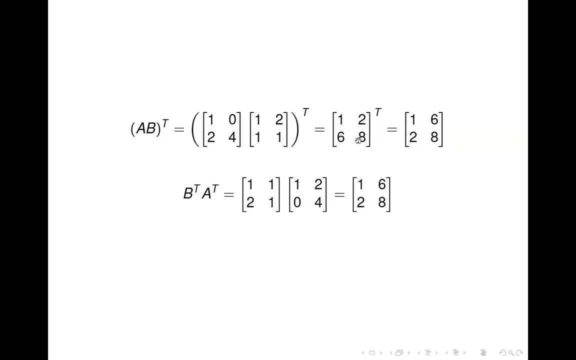 compute their products, then take the transpose. so I compute the product, here it is, transpose that and end up with this matrix. or I could do it this way: transpose each of them initially, but reverse the order that I do the multiplication. so here's B- transpose. 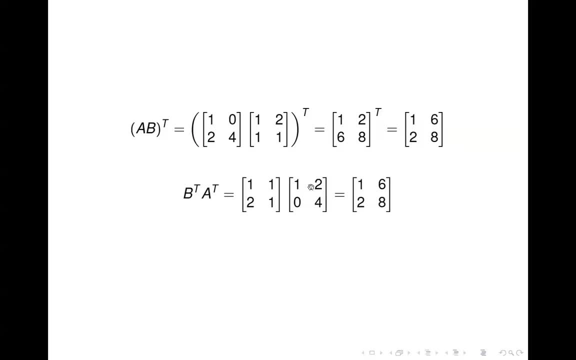 right, here's B up here. so I take the transpose that's here- here's A transpose- and I compute that product and I get the same thing as I did previously. Okay, let's talk about the inverse of a matrix. First, let's go back and think about the inverse. 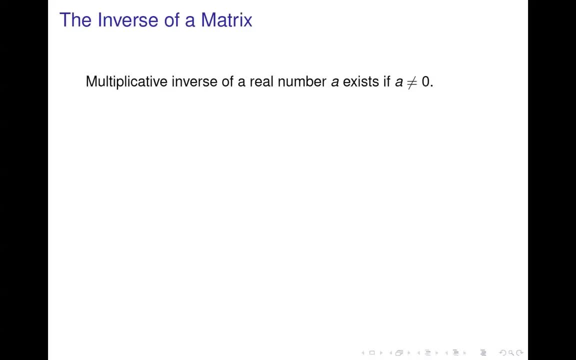 of just a scalar, a real number A. The multiplicative inverse, as opposed to the additive inverse of a number A is just 1 over A, assuming A is not equal to 0, because if we multiply A times 1 over A we get 1,, or 1 over A times A equals 1, and 1 is the inverse of A. 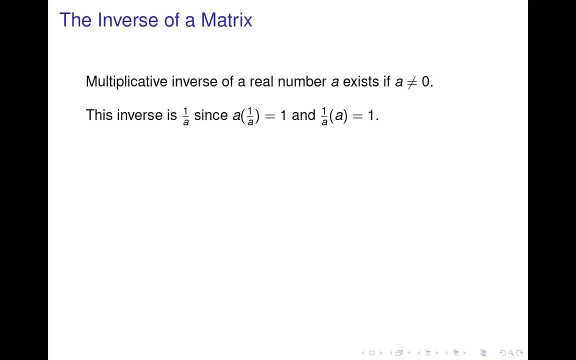 so 1 over A is just 1 over A. So if we multiply A times 1 over A, we get 1, or 1 over A times A, identity element for multiplication. we can use the same idea for matrices, the inverse of a matrix, a, exists only under certain conditions, so not every matrix. 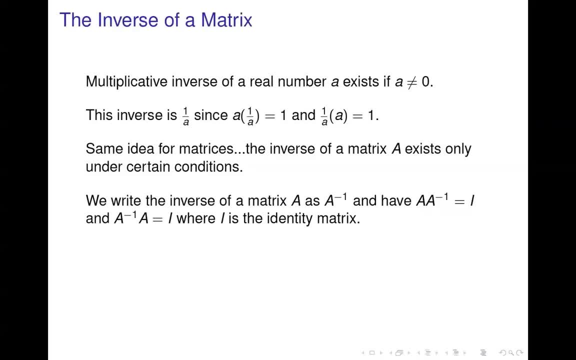 has an inverse, just like not every number has an inverse, zero doesn't have an inverse. okay, we're going to write the inverse of a as a with a superscript- negative one- and we have a times a inverse. we just read this as a inverse equals the identity matrix. okay, this is not the number one, this is the identity. 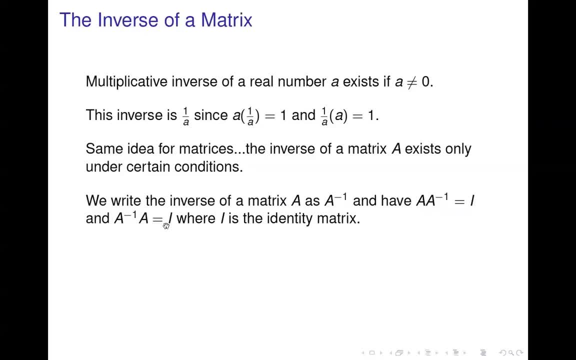 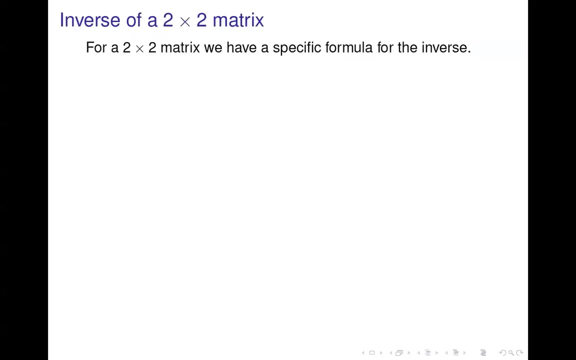 matrix and also a inverse times. a is the identity matrix- okay. one of the requirements for a inverse to exist is that a is a square matrix- okay, and you have to have that so that you can multiply on the left and on the right by the same matrix. okay. let's start off by talking about finding the inverse of a two by. 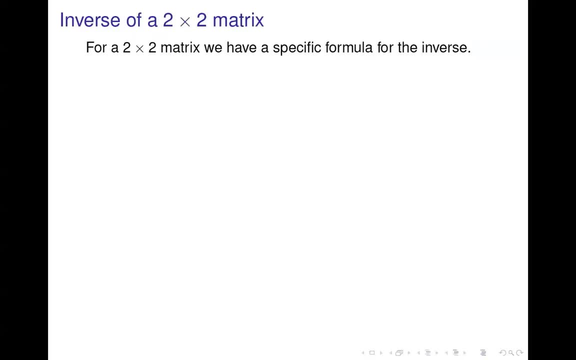 two guy. in this case there happens to be a specific formula for the inverse. so if we have a two by two matrix a that looks like this ABCD, then a inverse exists. if a times D minus B times C is not equal to zero, okay, so that's a times D. so 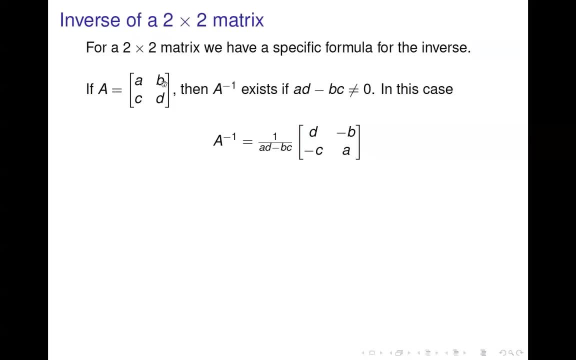 multiply the elements on the main diagonal and subtract off the product of the elements on the off diagonal, so a times D minus B times C. I call it the crisscross applesauce: a times D minus B times C. all right, so if that's not zero. 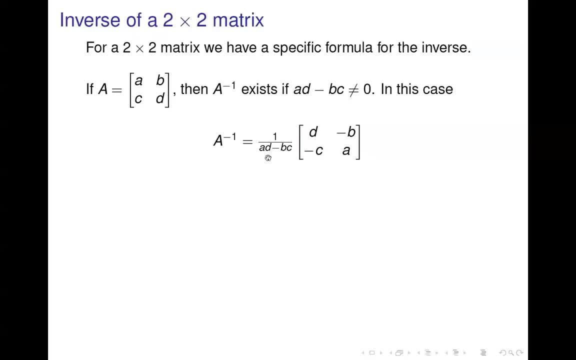 a inverse exists and here's a formula for it. notice that we divide by a D minus BC. that's why it has to be nonzero. and then the matrix is a. grad짓MSB is form from a by swapping the n, the numbers in the a and d positions. 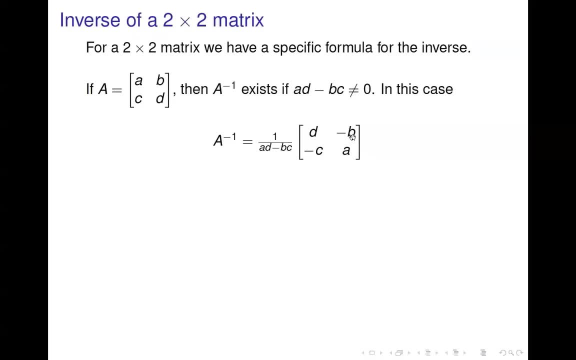 so we swap a and D and negと ca. so thats our memory数. and you swap A and D, neg B and C. so for example, here's a matrix a: if we look at the ad minus BC, thats four times negative three, so negative twelve minus. 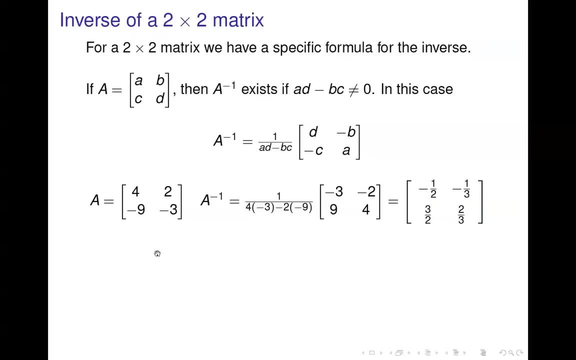 bc: negative nine times two, that's negative eighteen. so negative twelve minus negative eighteen would be negative twelve plus eighteen, which is six. so we're dividing one over six. this thing here is six, and then we swap the four and the negative three, they swap positions and negate the negative nine and two and then multiply that out and we get this matrix. so 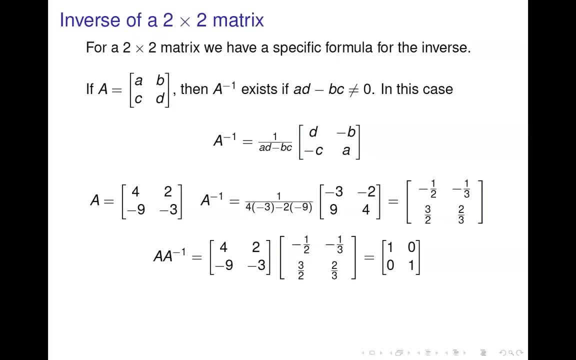 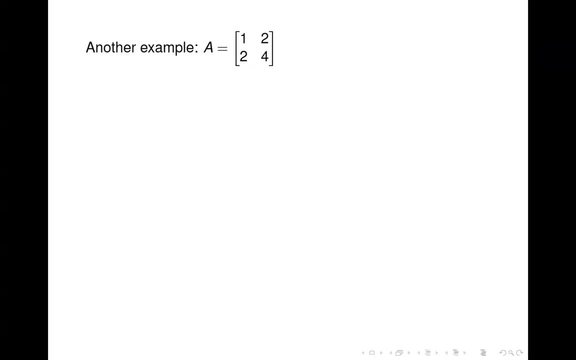 that's the inverse of a. and if you check, multiply a times the inverse, You get the identity matrix. if you multiply a inverse times a, we also get the identity matrix. Let's look at another example. Here's another. two by two, uh matrix, um, but uh, OAPS. in this case, if we multiply, do the. 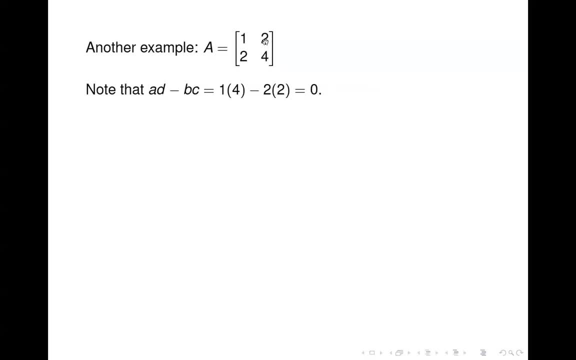 a, b minus bc, we got one times four minus two times two, which gives us a zero. so that tells us that this matrix does not have an inverse. and if you look at that matrix a little bit, you see that the second column is just two times the first and those 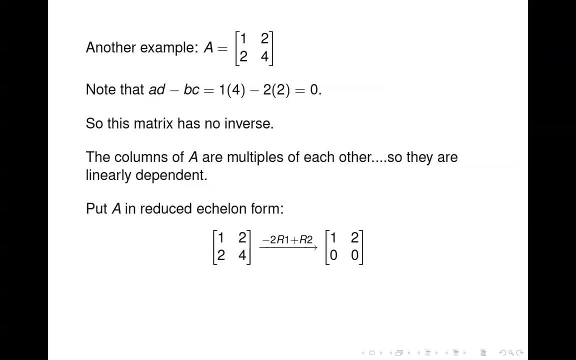 columns are multiples of each other, so they're linearly dependent. if we look at a and reduce special on form, it has a row of all zeros. nice, we have a free variable. to the point we say a is not row equivalent to the identity matrix. okay, it turns out that if a, any matrix- 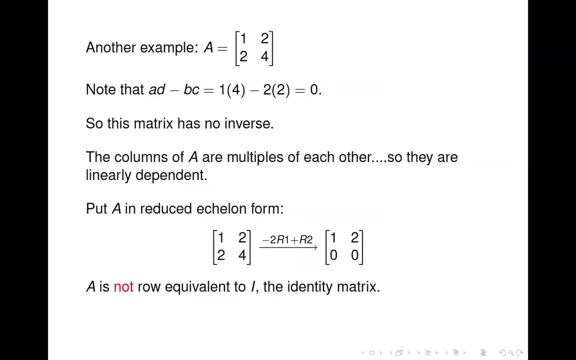 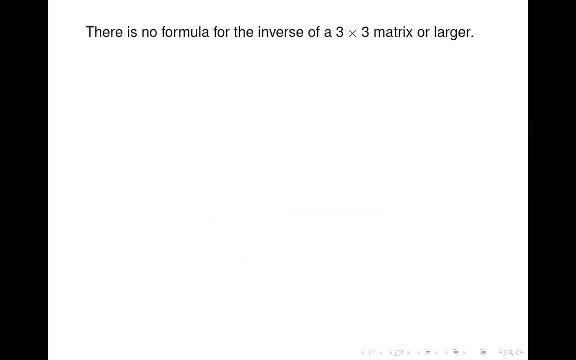 a. if it's not row equivalent to the identity matrix, then it will not be invertible, and if it is row equivalent to the identity matrix, it will be invertible. we don't have a formula for the inverse of a three by three, so we need to develop a method. 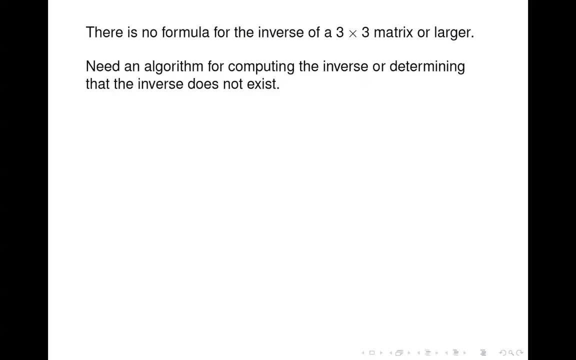 for computing the inverse or for determining that the inverse does not exist. so what we'd like to do is find a matrix- let's just call it b- such that a times b is equal to the identity matrix. okay, so we assume that a is in by n. then that means that b also has to be a. 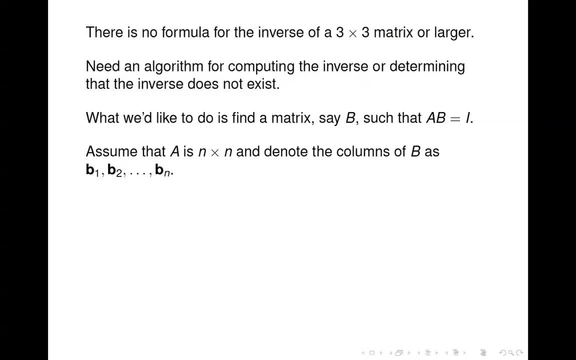 and in by n and we'll know the columns of b by the column vectors b1, b2 through bn. so, recalling from the previous section, if we multiply a times b, we can write that in this form: a times the matrix, here's b, the columns of b, b1 through bn, and that equals: 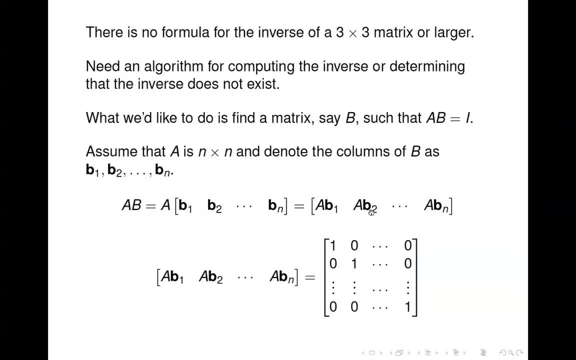 just a times b1 in the first column and b1, through bn and bd, accept machinehad. we did times b2 in the second column and so forth. so remember this: that a times b you get the first column as a linear combination of the columns of a, using the elements in b1 as the multipliers. 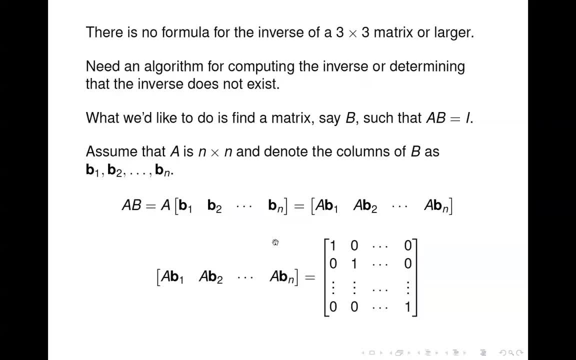 and so forth for the other columns. so remember, we want that to equal the identity matrix. so here's the identity matrix. so we want a times b1 to be the first column of the identity matrix, a times b2 to be the second column, and so forth. so in order to determine the matrix B here we need to. 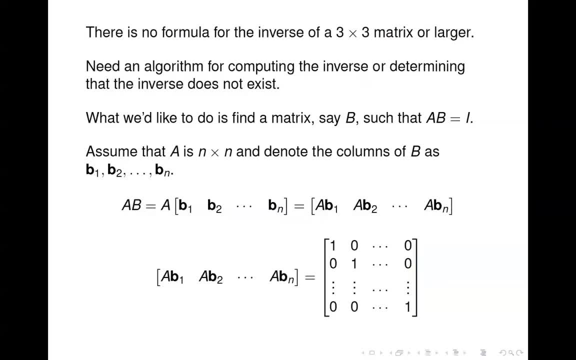 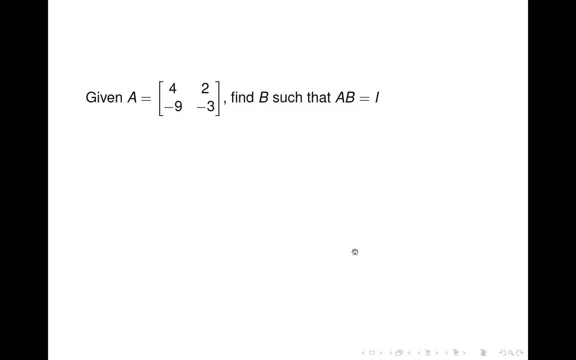 solve in systems of equations. okay, so if we solve those in systems of equations, we'll have a inverse, if it exists, all right. so let's look at this matrix and see if we can follow that method. it's a two by two, so we could just use the formula we have. 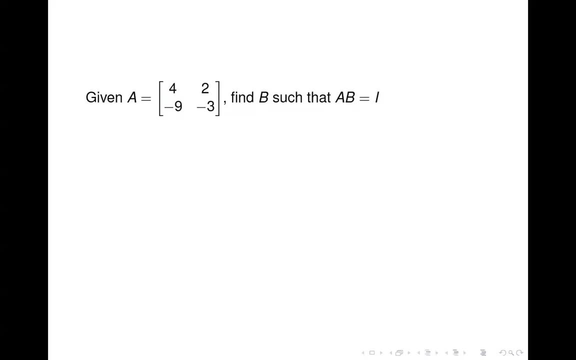 but let's try applying this method that we just discussed. all right, so a times B, a times B 1, a times B 2, and we want that to equal the identity matrix. so we have these two systems to solve: a times B 1 is 1, 0, a times B 2 is 0, 1. so here we go to solve this system. 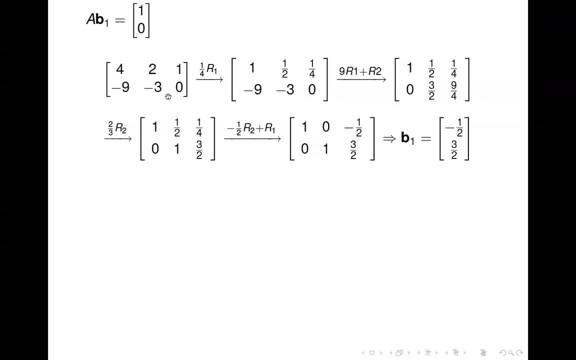 set up an augmented matrix. do some row operations and notice that a. get to this point, see that a is row equivalent to the identity matrix. so that means that a inverse does exist. and here's the first column: B 1 is negative, 1 half, 3, half. so that's the first column of the inverse. and to 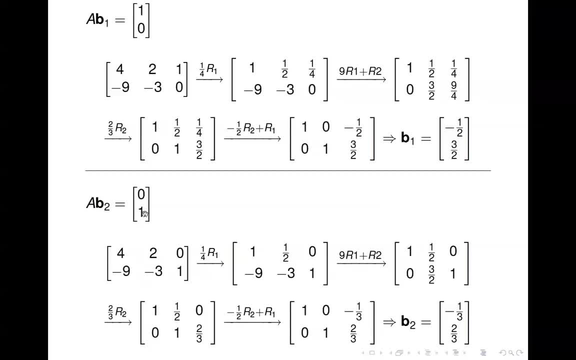 get the second column. we solve this system a times B: 2 equals 0, 1, the second column of the identity matrix. and again I set up my augmented matrix. tack on 0- 1, do some row operations and notice that the row operations that I'm doing here are exactly the same ones. 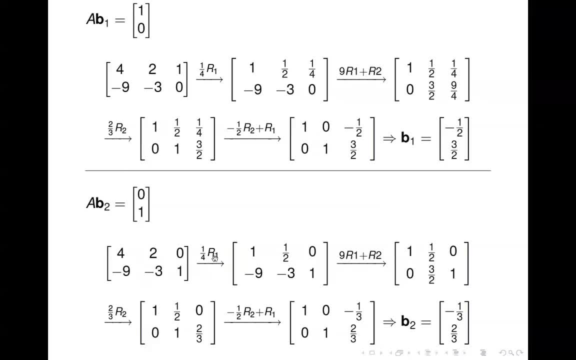 that I did up here. so first multiply row 1 by 1, 4th- same thing down here, then 9 times row 1 plus row 2, same as down here, and so forth, and that carries through the whole way, and if you give that some thought, you're going to be able to solve this problem. so let's go ahead, and let's go ahead and 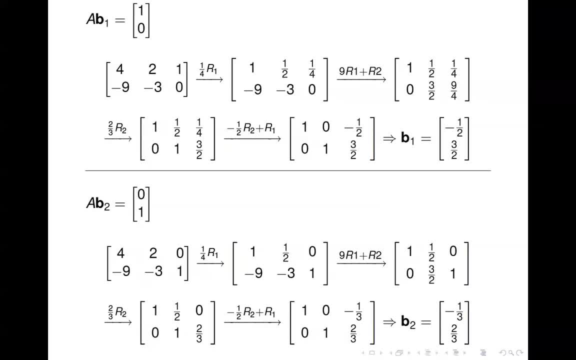 go ahead and solve this problem. so let's go ahead and solve this problem. so let's go ahead. and you'd say: oh yeah, that makes sense, because the row operations that I'm doing are based on the entries in a right. I'm trying to get a and reduce to echelon form. so, since a doesn't change same, 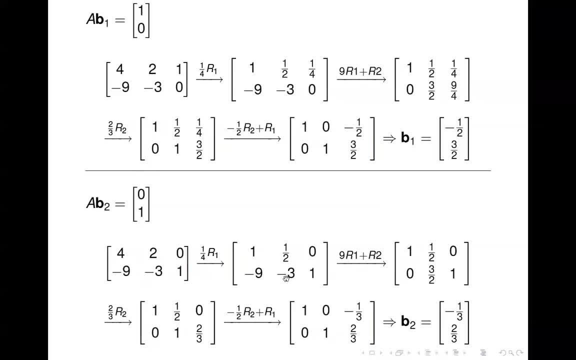 same a here and up here, then it makes sense that the row operations I do don't change. the only thing that's changed is what's in the last column, okay, and so we end up with a row operation that the entire row automations that are in the last row part is now going to be pię assembly uniquely. 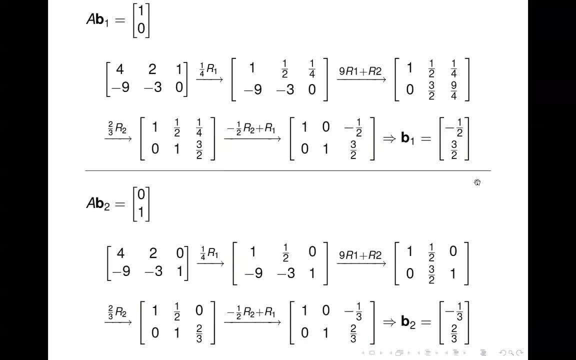 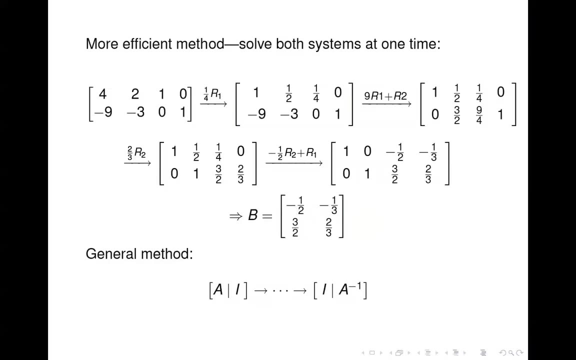 and then on the middle row, pl wishing the class is going knocked under and we are going to end up with this for b2. so I've got my two columns of B, which is what the inverse of a is, and and if you look at this, you think what it seems like to be a lot of repetitive work, and it is, and so we. 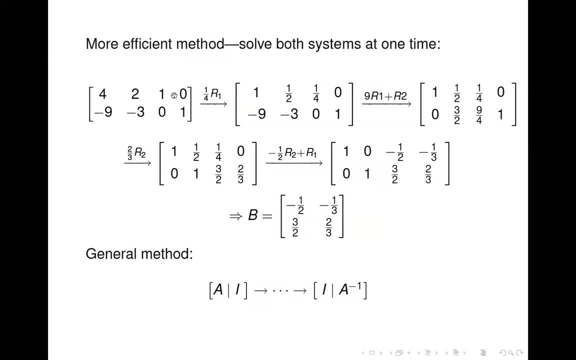 have a more efficient method, and that is to solve both systems at one time. okay, so instead of just in an augmented matrix, we tack on both columns or the whole identity matrix, depending on what size your original matrix is. And here we go through that same sequence of row operations. 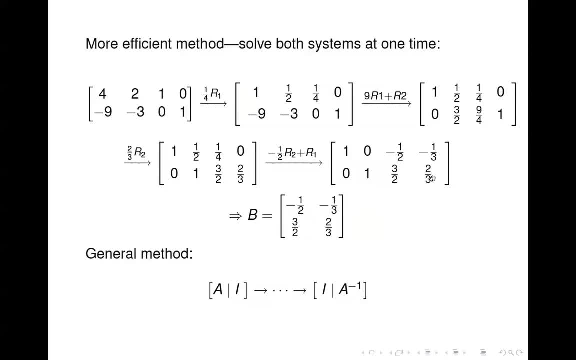 and we end up with the two columns of B that we found earlier. Okay, and this, of course, is the inverse of A. Now, in general, what this looks like is: you start off with this matrix, okay A, on one side, then augment on the identity matrix and you do row operations. 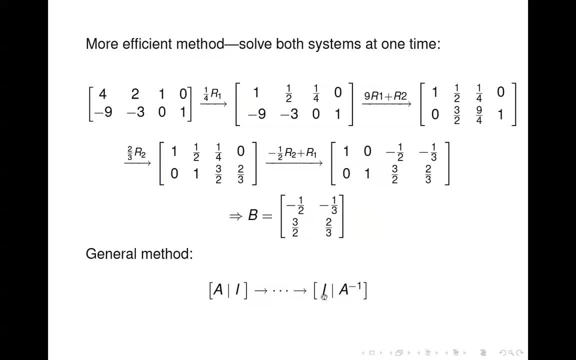 until you get A in reduced echelon form And what you're aiming for is to make it look like the identity matrix, And I said that may or may not be possible, depending on the echelon A. If it is, then you'll end up with the identity matrix here and the inverse. 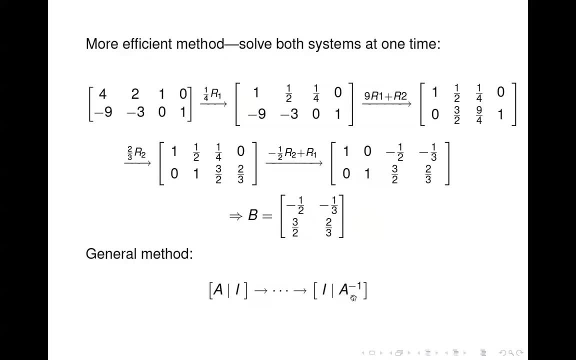 of A on the right. Alright, so that's what you're aiming for. And just while we're here looking at this, notice that we could go backwards, because we know that all these row operations are reversible. We could go backwards and look what happens. We start off with A inverse 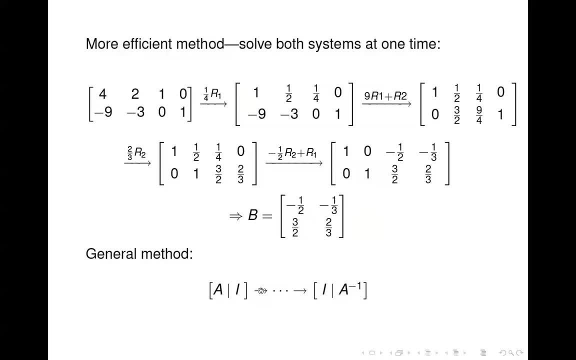 with the identity tacked on, and we get back here and we can make A inverse, and we get back here and we can make A inverse, and we can make A inverse, and we can make A inverse look like the identity matrix And so with A over here. so that tells you that if you 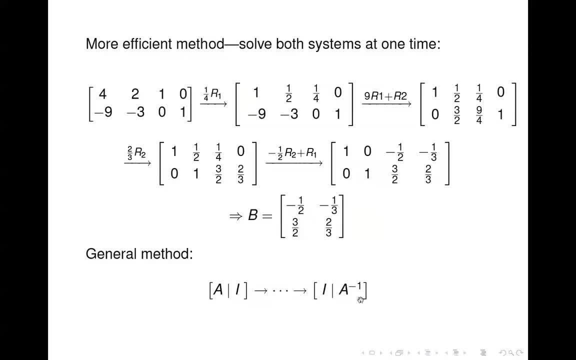 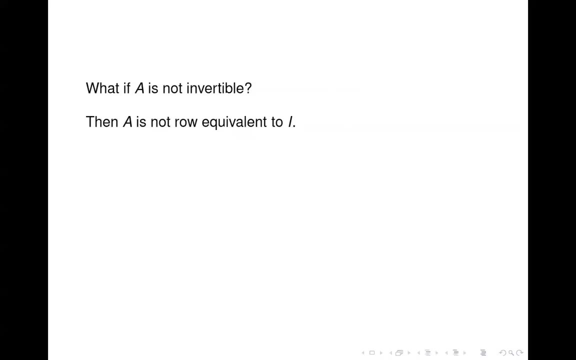 wanted to take the inverse of A inverse. then you just get the original matrix A back. So the inverse of A inverse is just A. Okay, so what happens if A is not invertible? In this case, it's not row equivalent to the identity, So 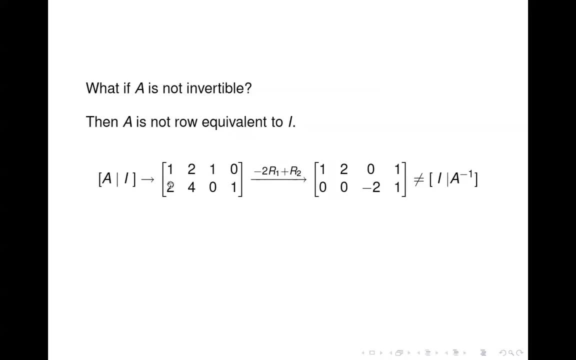 here's the example we had before, where the second column is a multiple of the first. Tack on the identity matrix. Do one row operation here and you get to this point and you say, oh, A is not row equivalent to the identity matrix and hence I can't get it in this. 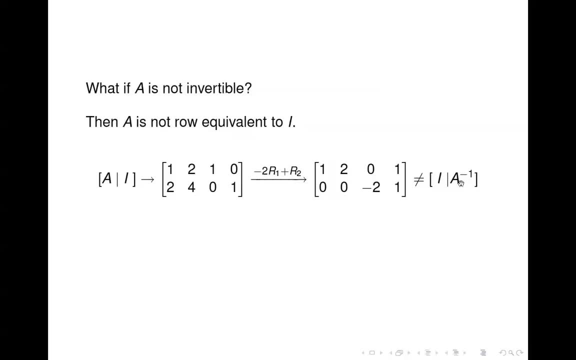 form where I've got the identity and then A inverse That tells you that the matrix A does not have an inverse. Okay, so if you can't get A to look like the identity matrix by doing row operations, then A is not invertible or A inverse does not exist. 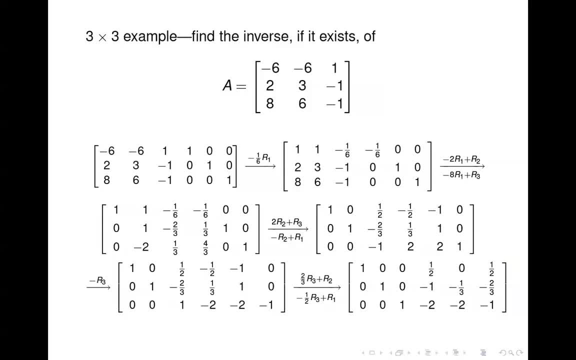 Alright now. this method works no matter what size your matrix is, so I scaled it up for a 3 by 3.. Okay, start off with this matrix A and tack on the 3 by 3 identity matrix and go through some row operations. 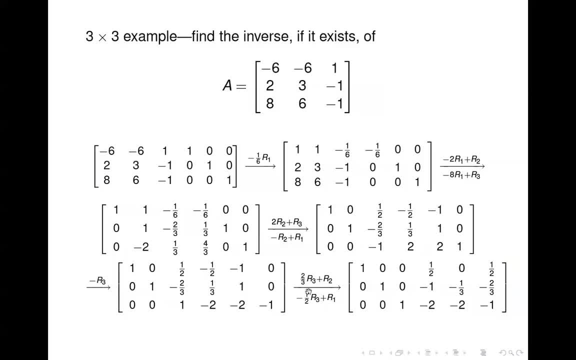 A lot of arithmetic here and if you look the last matrix i have here, look the first three columns- look like the identity matrix and so sitting over here would be the inverse of a. all right, so this, these last three columns, will be the inverse of my matrix, a. 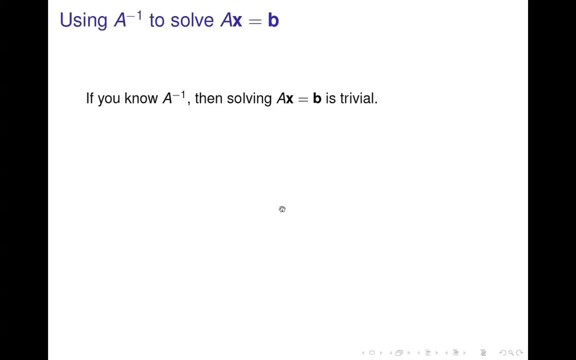 um, if you know a inverse, then solving ax equals b is trivial, right? because our whole focus in this course is solving ax equals b, solving systems of equations, and so if you know a inverse, then it turns out that it's super simple to solve a system of equations involving a. 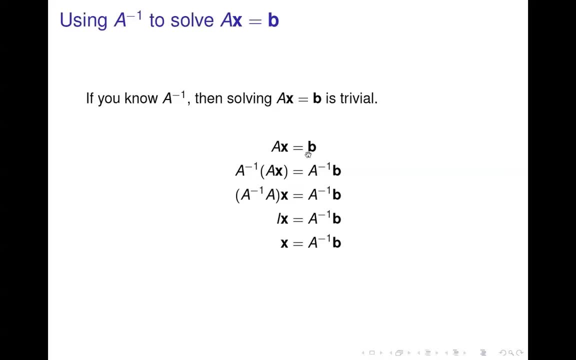 and basically here's the rationale: um, start off with ax equals b, um, and you know, a inverse exists and that means you can multiply both sides of your system by a inverse. so i do that, and the reason to do that is because, if you look over here, we can uh, re-associate the parentheses and so we can end up with a inverse. 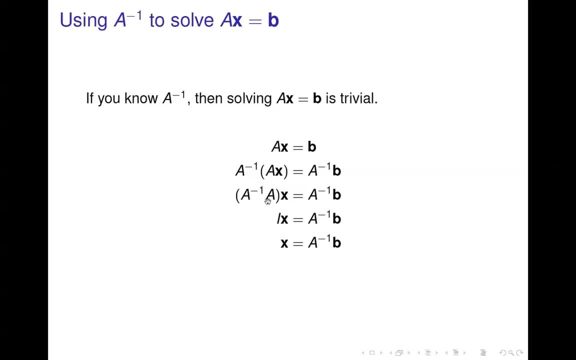 times a together, and the advantage of that is that that equals the identity matrix. so we end up with just the identity matrix times a, and that's what we're going to do here. so we're going to do that. x and anything times the identity matrix is just that anything. so i times x is x, so x is simply a. 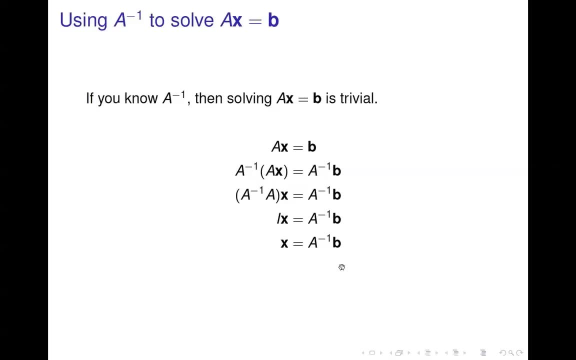 inverse b. so if you know a inverse, then you don't need to do row operations, you don't need to do any of that stuff. just multiply a inverse times b and you have the solution to your system. okay, clearly that's going to save you a lot of work if you have a inverse. 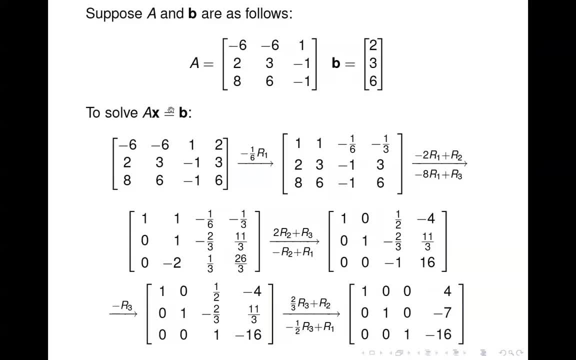 so if i have this matrix a and this vector b and i want to solve ax equals b, then i'm going to do row operations. so if i have a matrix a and this vector b and i don't know a inverse, then i gotta go through, you know, set up my augmented matrix, do all these row operations. 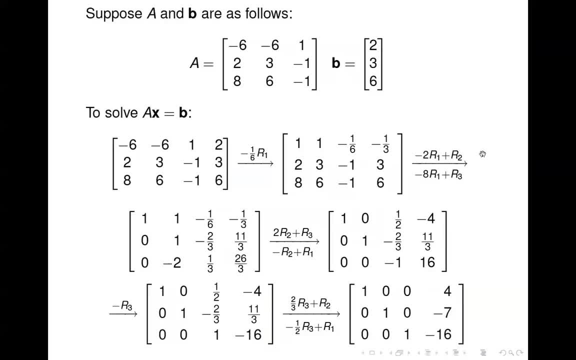 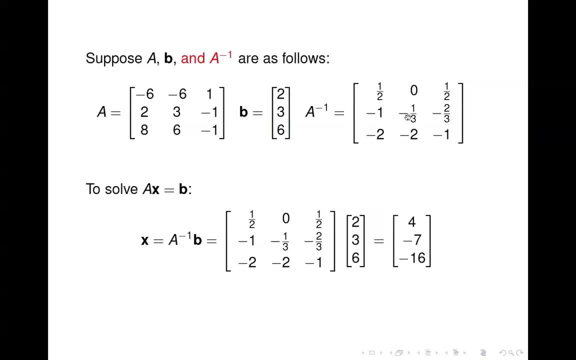 and i end up here with my solution for negative seven, negative sixteen, okay, but if i know a inverse, okay, so i know a inverse. so here's a, here's b and i know a inverse. then to solve ax equals b, as i said, just multiply a inverse times b and here's your solution. all right, so 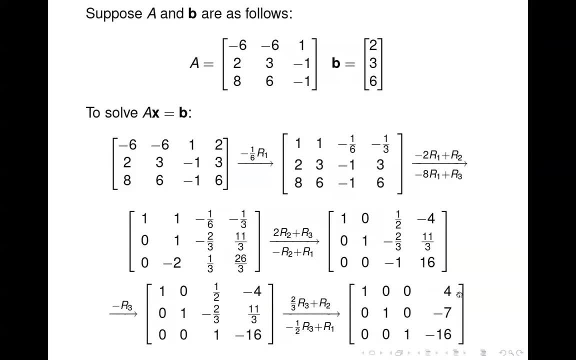 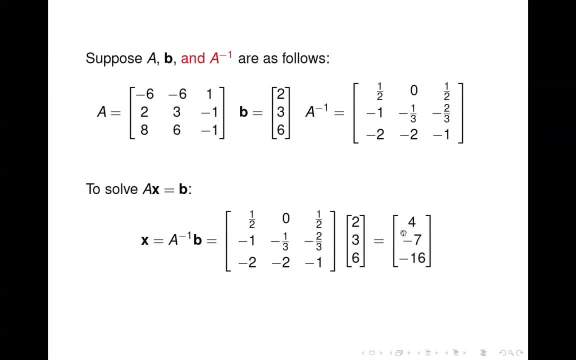 went through all this work to get 4 negative, 7 negative, 16. here, if you know a inverse, all you do is simple multiply matrix times the vector and you have the solution. now, of course, the downside is that most of the time you don't have a inverse. and to get a inverse, well, you saw what work is. 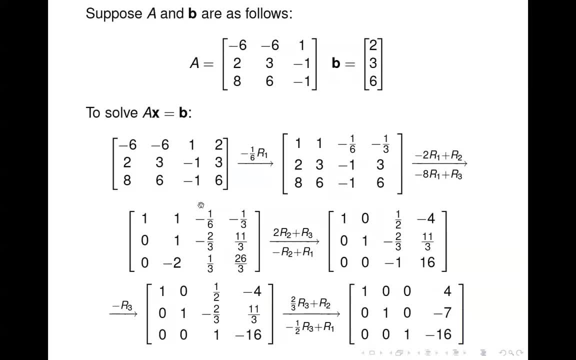 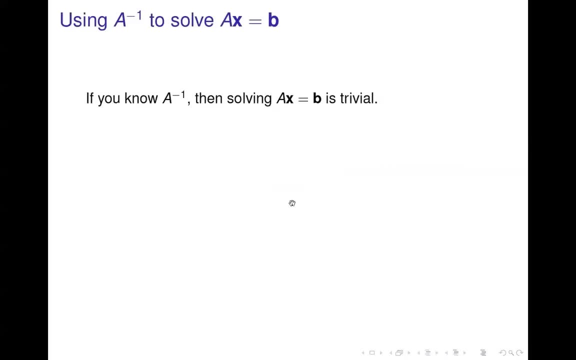 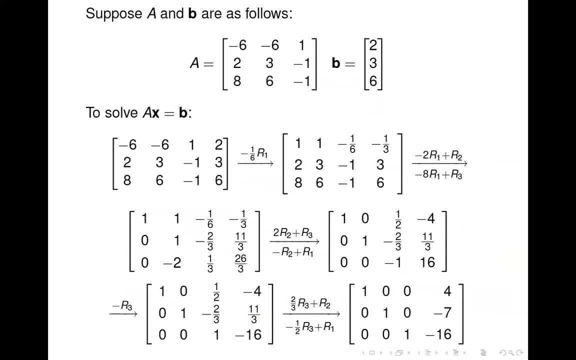 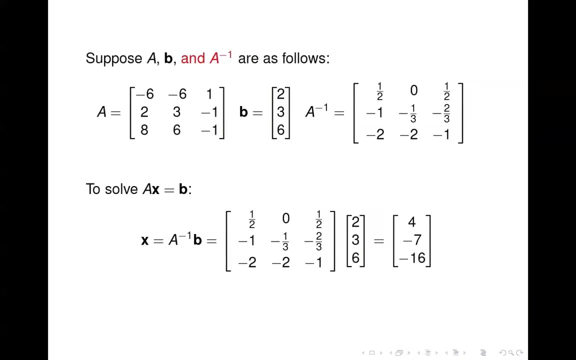 required in that more work than simply going back and through to do this, because to find a inverse for 3 by 3 we had to solve- let's go back right. we had to solve three systems of equations just to solve this system. you solve one system of equations, but if you know a inverse, then solving system is. 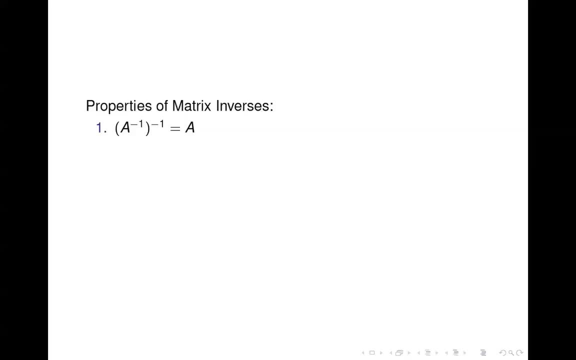 trivial, okay, um, let's say your book lists and properties of matrix inverses, this one we've already talked about. take the inverse of a inverse, you get a back if you have the inverse of a product. so a B quantity inverse, that is the product of the inverses, but in reverse order. so B inverse times. 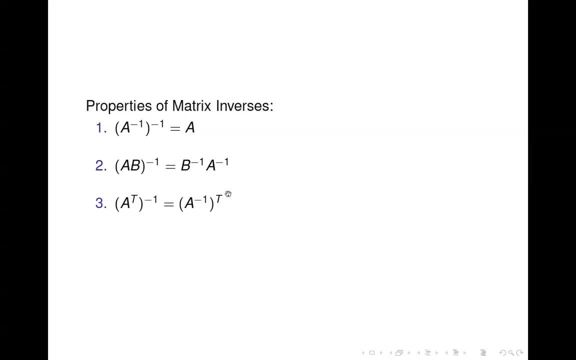 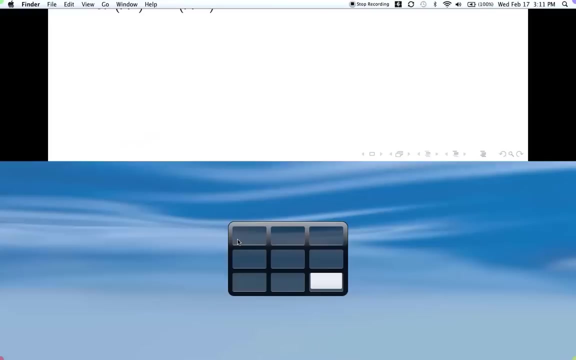 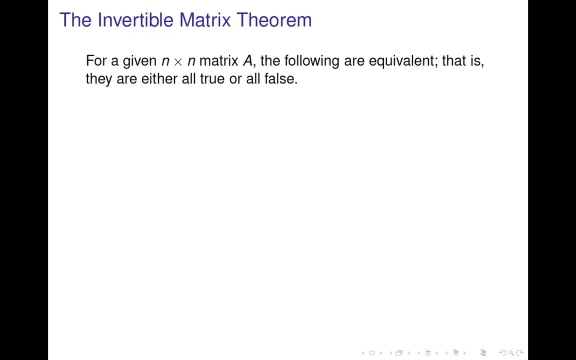 a inverse instead of a inverse times, B inverse and. And if you take the inverse of a transpose of a matrix, that's equivalent to transposing the inverse. Okay, the main part of section 2.3 is the Invertible Matrix Theorem. 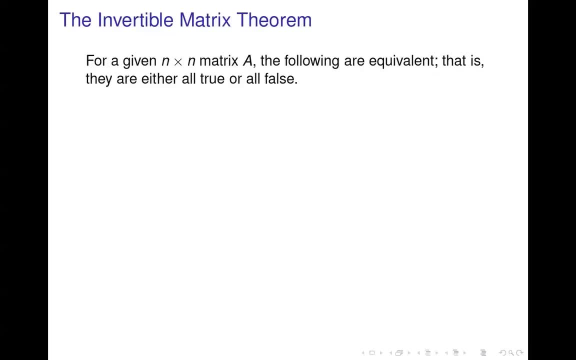 And this theorem actually ties together everything that we've done so far in the course, actually In Chapter 1 and up through Chapter 2, where we are. So this theorem says: if you have a given n by n, matrix A, the following are equivalent: 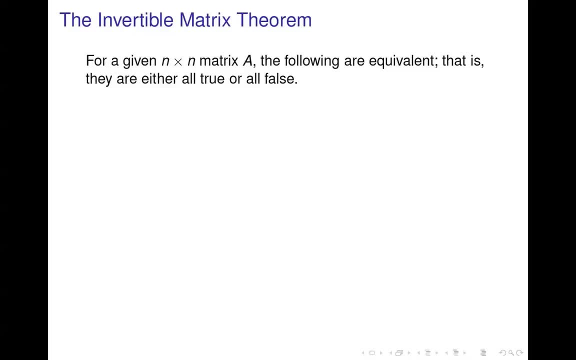 That means that they're either all true or all false. Okay, the first two look like this: one, A, is an invertible matrix and number two, A, is row equivalent to the identity matrix. So that should make sense, Because the way we found out if A is invertible is to do those row operations and try to get. 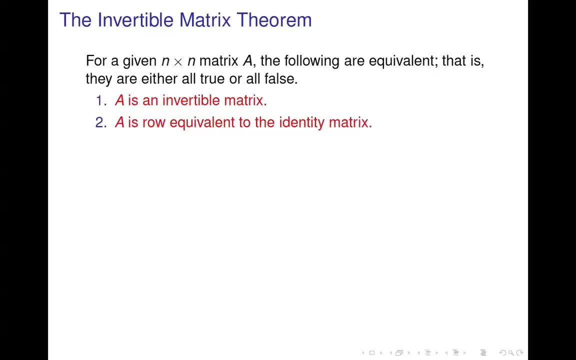 it in the form of the identity matrix, And if we could do that, then that means A is invertible. If we couldn't do that, then A is not invertible. Okay, another statement: A has n pivot positions. So this is actually the key to the whole theorem, in my opinion. 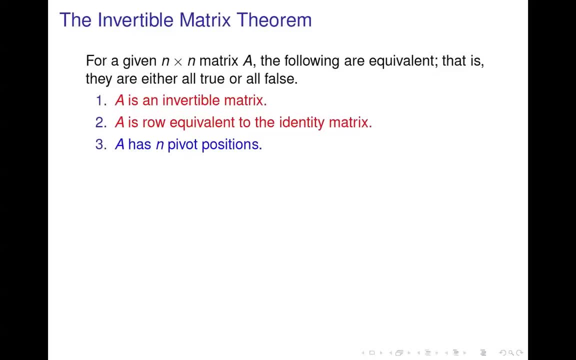 Everything here To pivot positions, and that's how I would recommend that you approach this. So, looking ahead, you need to know what this theorem says. You need to be able to write down parts of this theorem. I don't suggest that you memorize it, because I think that's somewhat difficult. 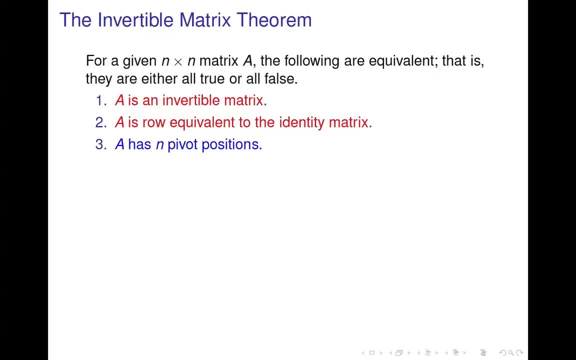 But I don't. So don't memorize it, Unless that works for you. But the way I would suggest that you remember it is to relate everything back to pivot positions, Because that's what we've done up to now and that should still work for you. 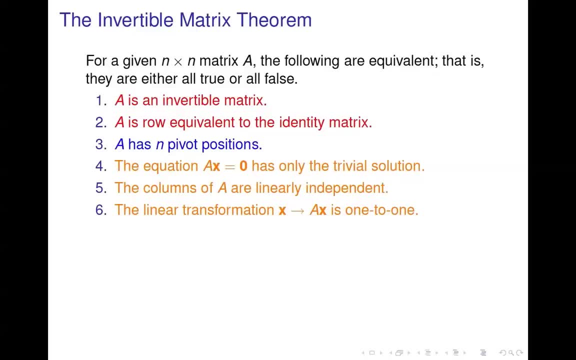 So let's look at these next three. And number four says the equation AX equals zero has only the trivial solution. Okay, so if it has only the trivial solution, then that means that there are no free variables. That means every column of A is a pivot column. 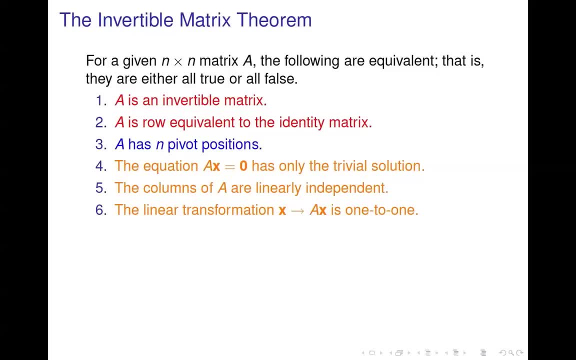 And so that means, since they're in columns, there's n pivot columns, So n pivot positions. So that relates back to pivot positions Number five. the columns are linearly independent. How do we know that? Well, again, no free variables. 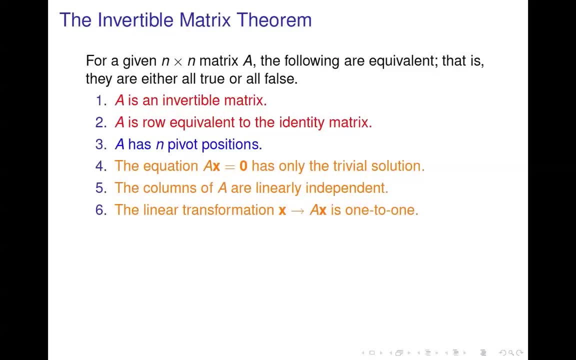 So pivot position in every column are n pivot positions And number six, the transformation X to AX is one to one. And how do we know that? Well, that means we want to have a unique solution to every system. AX equals B Or at 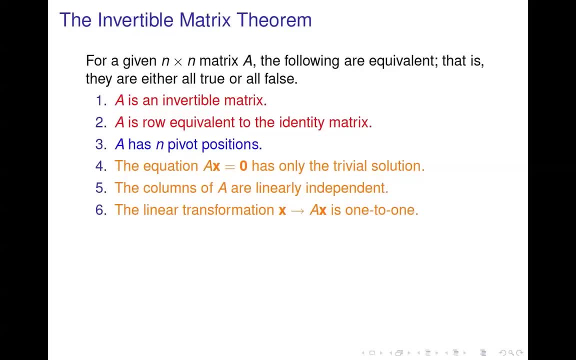 most one solution And no multiple solutions for any right-hand side. So that means that we can't have any free variables. So again, pivot position in every column. So four, five and six all relate to the fact that you need a pivot position in every column. 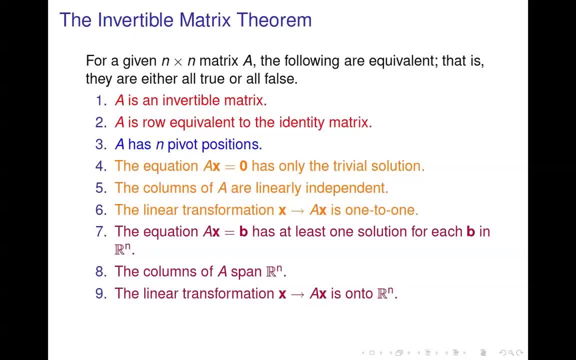 These next four relate to To having a pivot position in every row, Which, again, since it's an n by n matrix, that would mean you have n pivot positions. So number seven says AX equals B has at least one solution for each B in Rn. 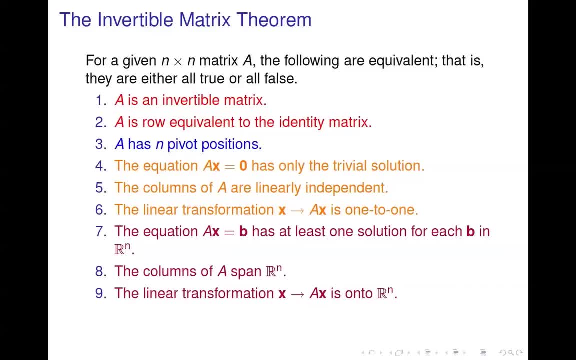 So if that's true, that means that system is consistent, no matter what the right-hand side is. That only happens when you have a pivot position in every row. N rows means n pivot positions: Okay. Columns of A span: Rn- Okay. 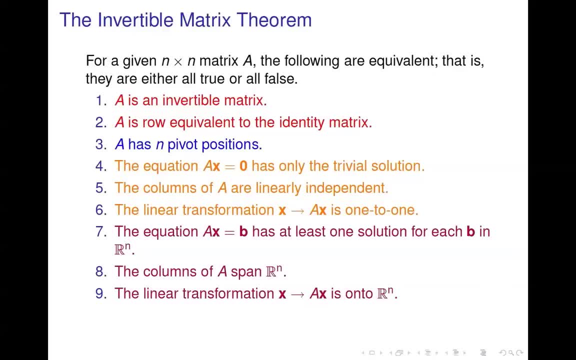 That again means that there's a pivot position in every row, So that no matter what you put on the right side, the system will be consistent. So again, pivot position in every row. So n pivot positions. And number nine, X to AX, is onto Rn. 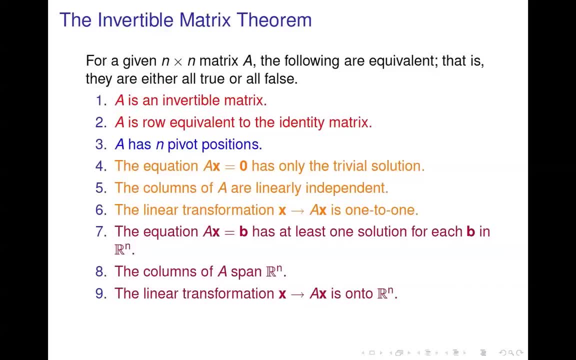 So that means again, there's a solution, no matter what the right-hand side of the system- AX equals B- is. So there has to be a solution, There has to be a pivot position in every row And then last A transpose is invertible. 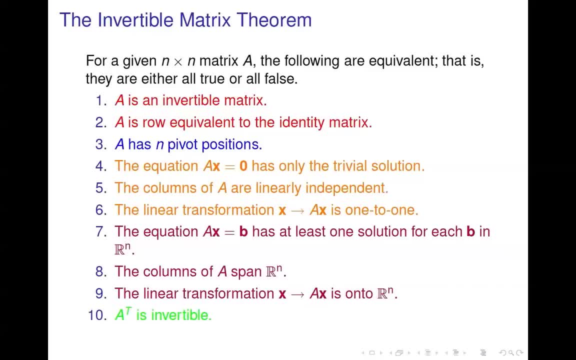 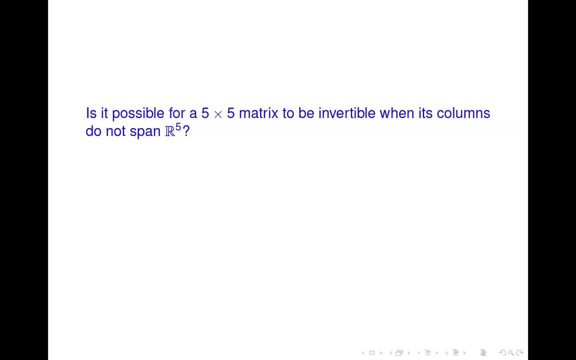 It's kind of a tag along there, but if A is invertible, A transpose is invertible. Okay, So I've taken a few of the even-numbered problems from this section just to kind of talk through those, to give you an idea about how to go through some of the logic here. 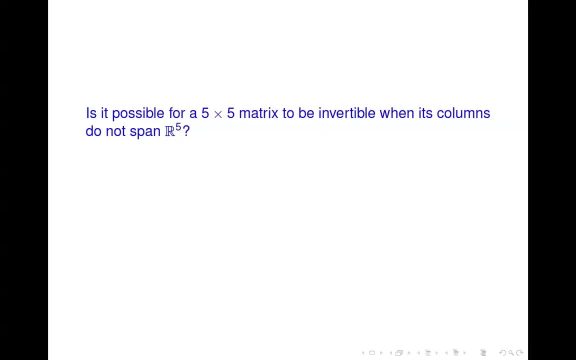 So here's one. It's possible for a five-by-five matrix to be invertible when its columns do not span R5.. Okay, Well, let's see. If the columns don't span R5, then that means that there's not a pivot position in every. 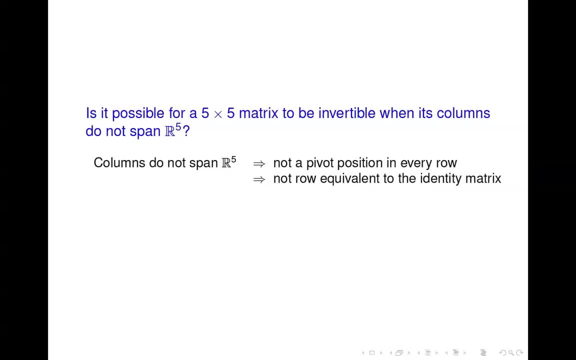 row, And that means that the matrix is not row equivalent to the identity matrix. Or you could say that there's less than five pivot positions. Either one of those gets you to R5.. Okay, So the matrix cannot be invertible. All right. 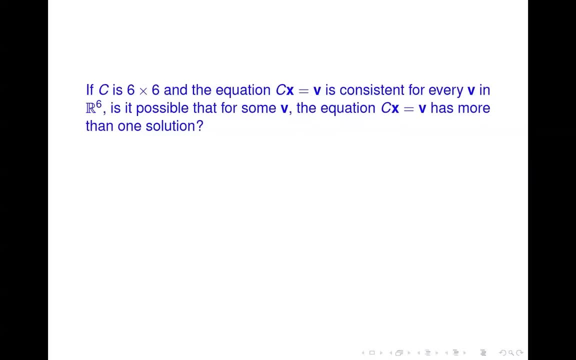 Here's one. I've got a six-by-six matrix and the equation CX equals V is consistent for every V in R6.. Is it possible that for some V, the equation CX equals V has more than one solution? Okay Well. 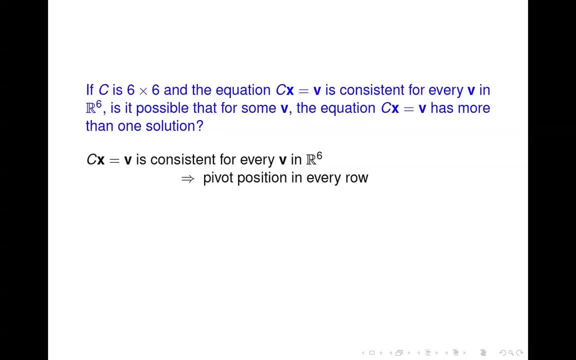 So if CX equals V is consistent for every V in R6, then that means that there must be a pivot position in every row. And since this is a square matrix, if there's a pivot position in every row, then there's also one in every column. 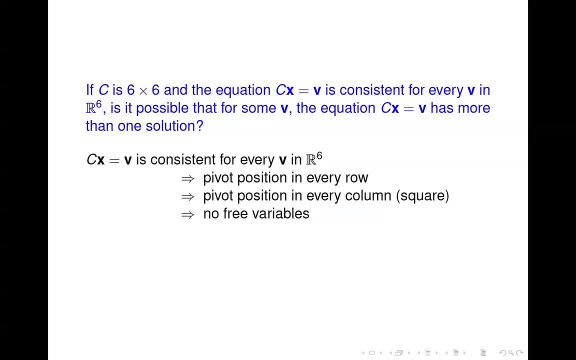 And if there's a pivot position in every column, that means there's no free variables, And so hence, any system will, uh, uh, there will be no system that has a pivot position Um an infinite number of solutions. 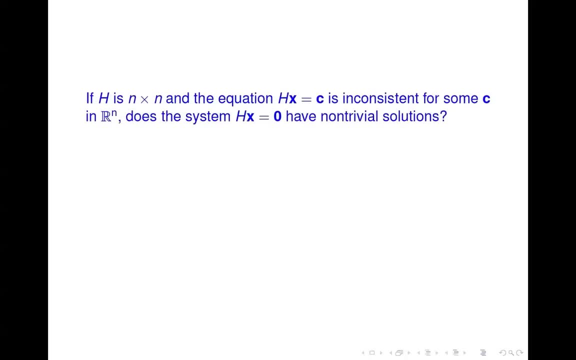 Only a unique solution. All right, Let's suppose H is N by N and the equation HX equals C is inconsistent for some C. Does the system HX equals zero have non-trivial solutions? Hmm, Well, if HX equals C is inconsistent for some right-hand side, then there can't be a pivot. 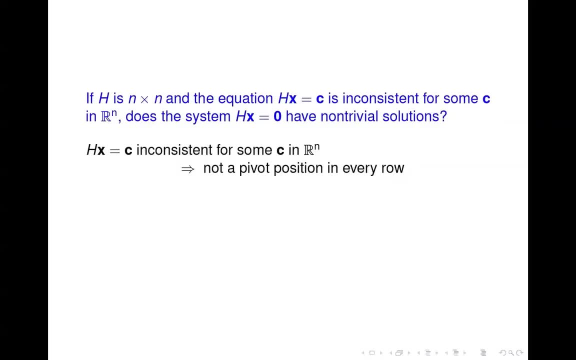 position in any of the rows. Okay, There can't be a pivot position in every row, And that means that there can't be a pivot position in every column, since H is a square matrix, And if there's not a pivot position in every column, then that means you have free variables. 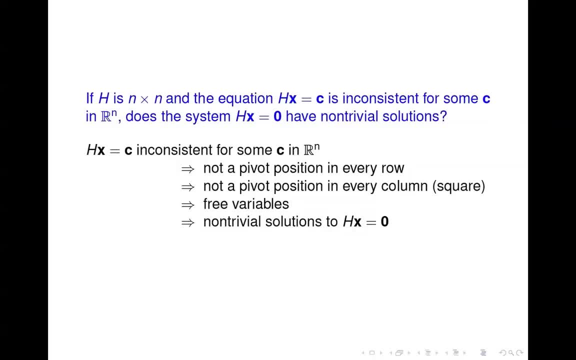 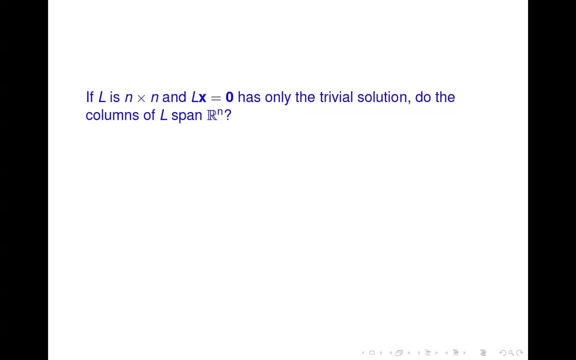 And hence there are non-trivial solutions to HX equals zero. Okay, Another one. If L is N by N and LX equals zero has only the trivial solution, Do the columns of L span R, N? Well, if LX equals zero has only the trivial solution, then that means there's no free. 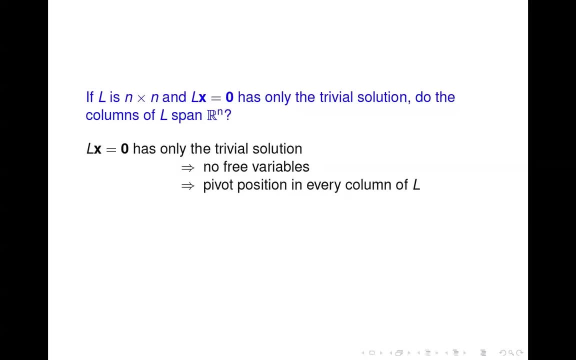 variables. So we have a pivot position in every column of L, which means we have a pivot position in every row of L, since L is square, And if there's a pivot position in every row, then that means that the columns span R, N. 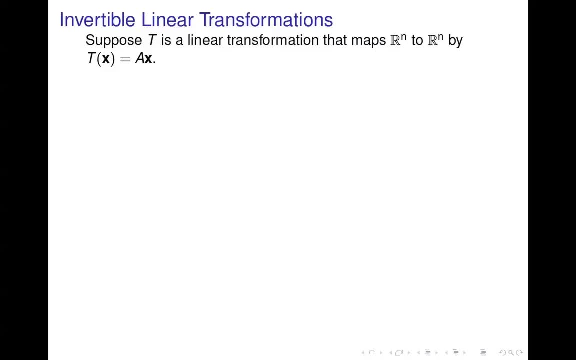 All right, Let's move on. Talk about invertible solutions. Okay, Okay, Let's talk about invertible linear transformations. Let's suppose we have a linear transformation, T from RN to RN that's defined by the matrix A, So A here would be N by N. All right, 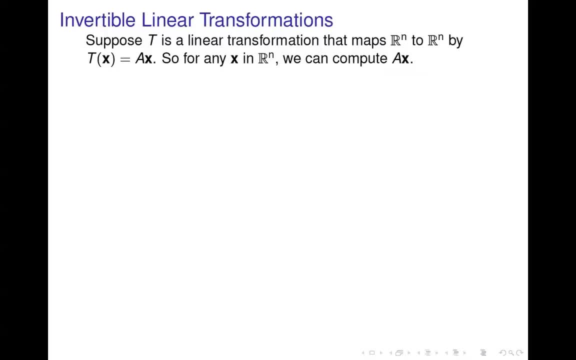 For any X we can compute AX. right, For any X, we can compute T of X or A times X. Let's think about going backwards though, Okay. So suppose you have some B and you would like to know: is there a unique vector X? 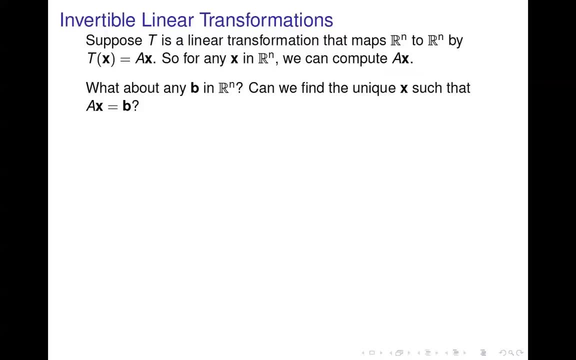 such that AX equals B. Okay, So think of B as being in the codomain and we want to go backwards to see what X mapped to that B. All right, Well, this works If T is both 1 to 1 and on. 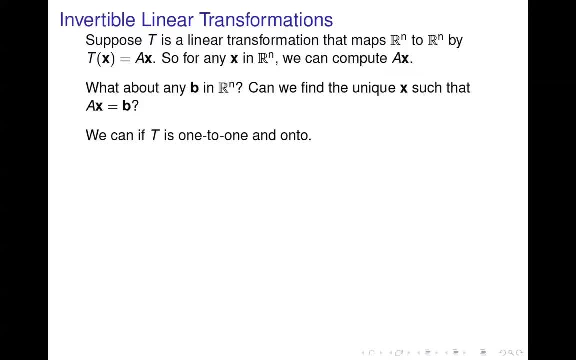 Okay, So for us to be able to go backwards and find out what X mapped to B. we can do that if we know that T is 1 to 1 and on 2.. Okay, So why is that? Well, if T is on 2,, then that means that every B in RN is mapped to by at least one X. 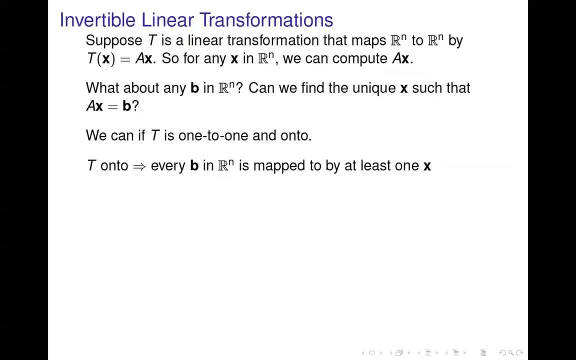 All right, Every B is mapped to by at least one X. So that means that If we go backward, there's an X to go back to. If it's 1 to 1, then that means that every B is mapped to by at most one X. 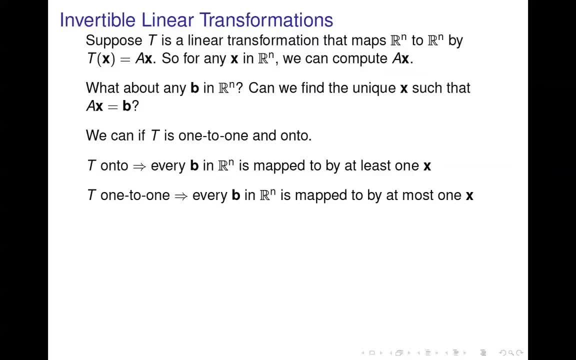 All right, Every B is mapped to by at most one X. So that means that if we can go backwards, there's only one vector to go backwards to. All right, We don't have multiple vectors mapping to the same B. So if you put those two things, 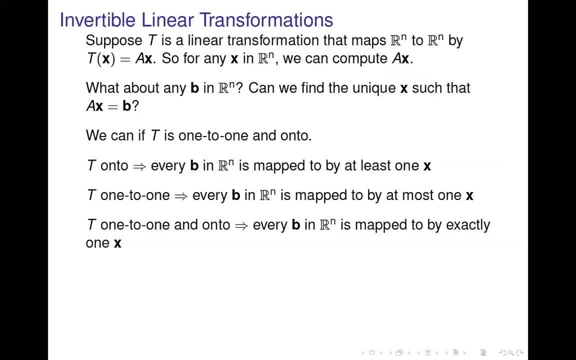 together. If T is 1 to 1 and on 2, then every B is mapped to by exactly one X. Okay, Which means there's a unique solution. So how do we find that X Given a particular vector B? how do we find out what X mapped to it? 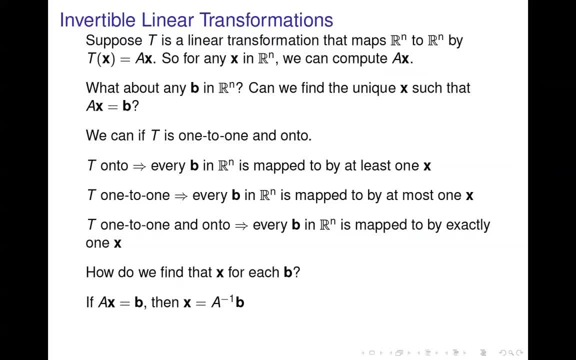 Well, we need to solve: AX equals B, And the way to do that, if we know that A is invertible, is to simply, Okay, To simply multiply A inverse times B. So the matrix that defines the inverse transformation, T inverse, is simply A inverse. 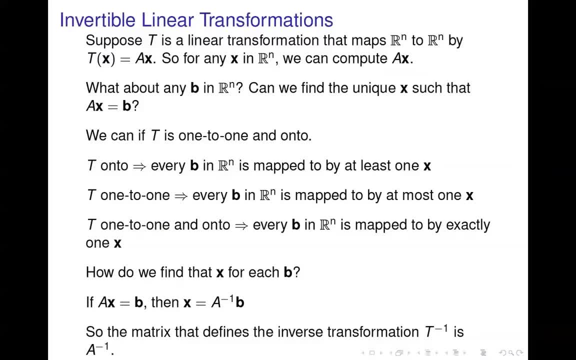 Okay, So A takes you forward right from X. You multiply A times X to get B in the codomain to go backwards. to reverse that, You multiply by X, You multiply by A inverse. So T is defined by A, T inverse is defined by A inverse. 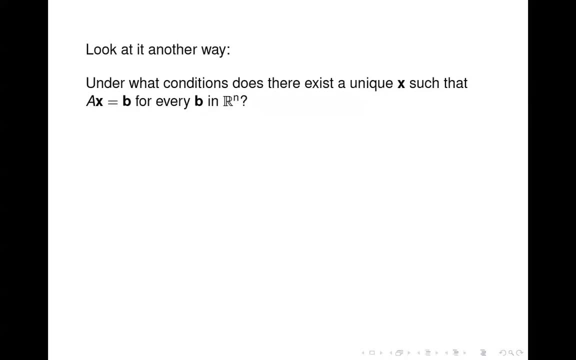 Another way to look at it is this: Under what conditions does there exist a unique vector X such that AX equals B for every B in our N? All right, When can we know that the system AX equals B is always consistent And Always has a unique solution? 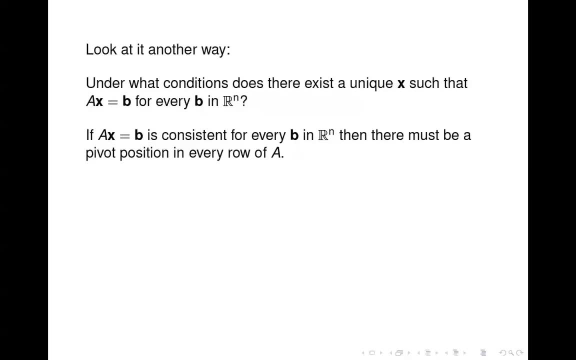 Well, it's consistent if there's a pivot position in every row of A. right AX equals B is consistent for every B. if there's a pivot position in every row of A And if the solution is unique, then there has to be no free variables. 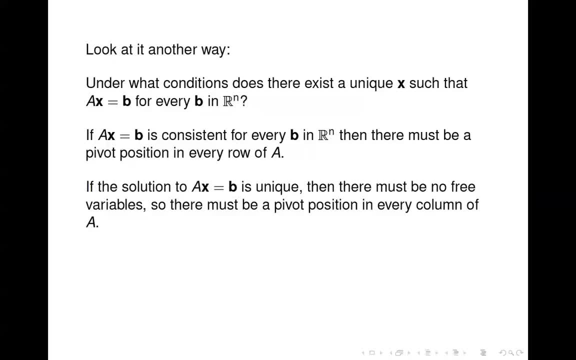 So that means there has to be a pivot position in every column of A. So backing up, it's consistent. Uh, If it's consistent for every B, we have to have a pivot position in every row. If there's a unique solution, then that means we have no free variables, so we have to have 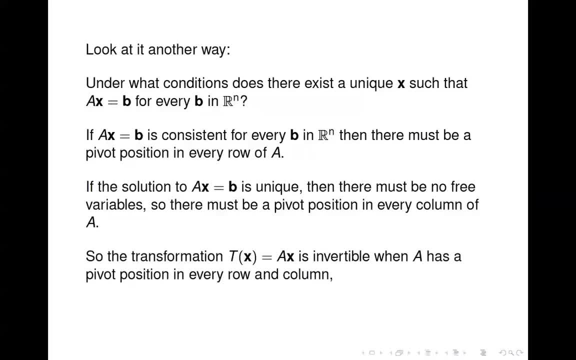 a pivot position in every column. Okay, So T of X equals AX is invertible when A has a pivot position in every row and column, ie when A has N pivot positions, ie when A is invertible. Okay. 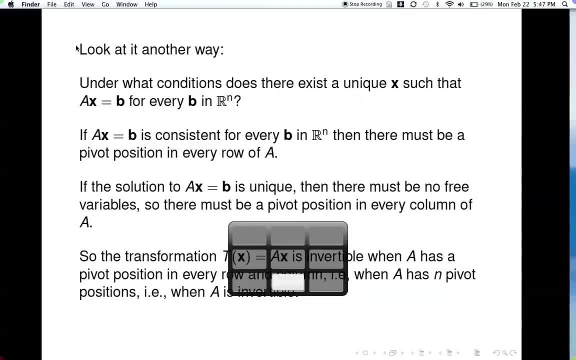 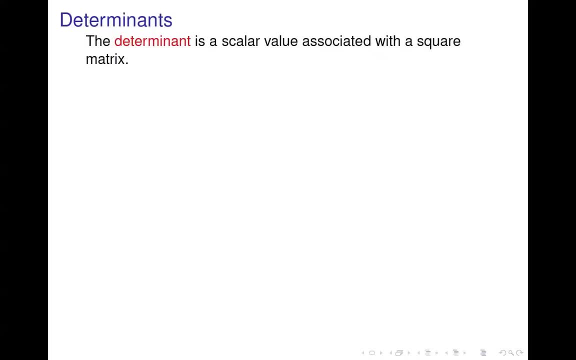 Okay, We're going to talk about determinants. The determinant of a matrix is just a scalar value that is associated with any square matrix, So we only talk about the determinant of a square matrix. The notation is DET of A, Or sometimes you see it with DET of A. 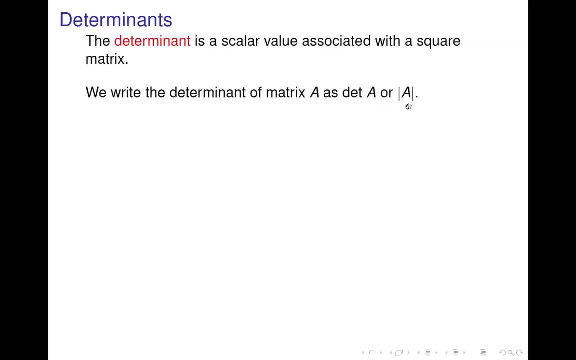 Sometimes you see it with A, It looks like the absolute value of A, with the vertical bars around A. We've actually already seen the determinant in the 2x2 case. If we have A, it's just this generic matrix, ABCD. 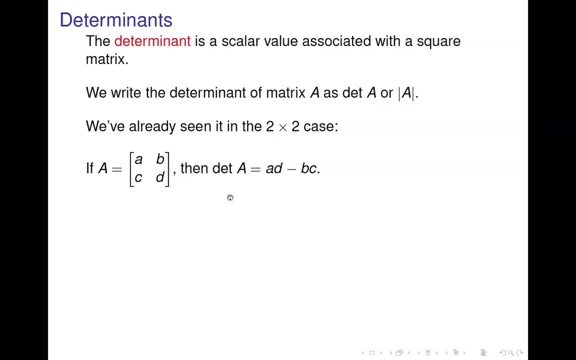 Then the determinant of A is A times D minus B times C, And we've seen that because we saw that in the little formula for the inverse. So remember we multiplied by 1 over AD minus BC. So we're multiplying by 1 over the determinant of the matrix. 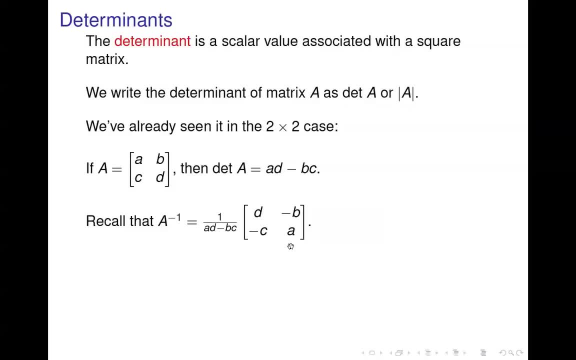 And then we kind of rearrange the terms and negate a couple to get the inverse of a matrix. So notice that at least in the case of a 2x2 matrix, we can see that the inverse exists when the determinant of the matrix is not equal to 0. 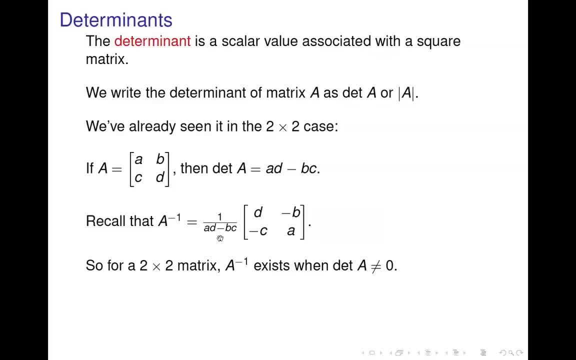 Okay Here. in this case, if AD minus BC is equal to 0, then A inverse does not exist, And it turns out that this is true for any square matrix. If the determinant is not equal to 0, that means the matrix is invertible. 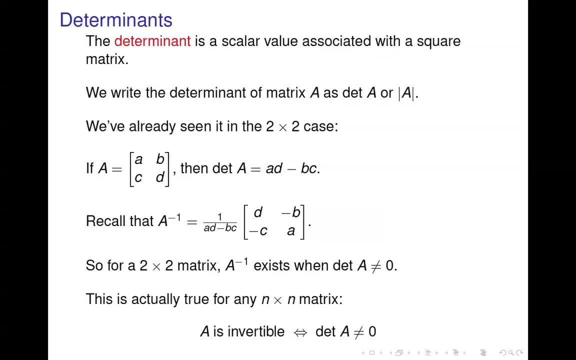 And if it's invertible, then the determinant is not equal to 0.. So this is actually another installment in the invertible matrix theorem which we had from section 2.3.. Okay, So determinant of A not equal to 0 is logically equivalent to A is invertible. 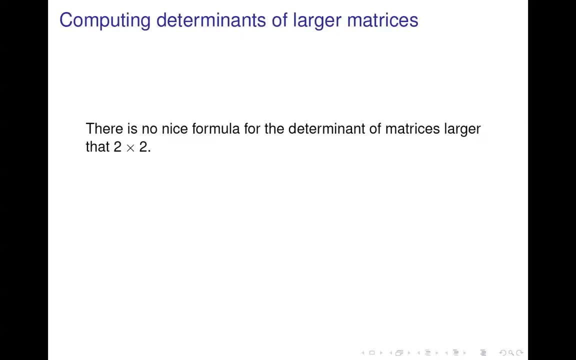 All right If we move up beyond a 2x2, there's no nice formula for computing the determinant like there was for a 2x2.. And we use a method called cofactor expansion And this method works for any size matrix, 3x3 on up. 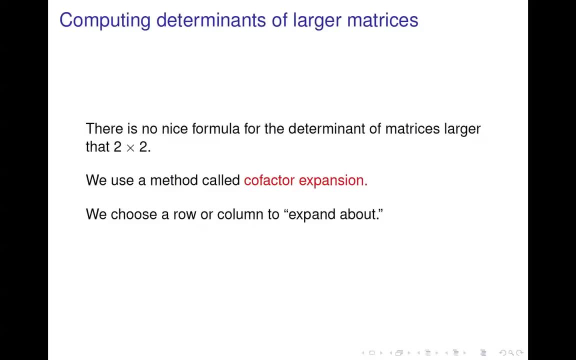 In this method, We have to choose a row or column to expand about. Okay, That's what we call it. We're going to choose a row or column to expand about. You'll see as we go on that it's advantageous to choose a row or a column that has the most. 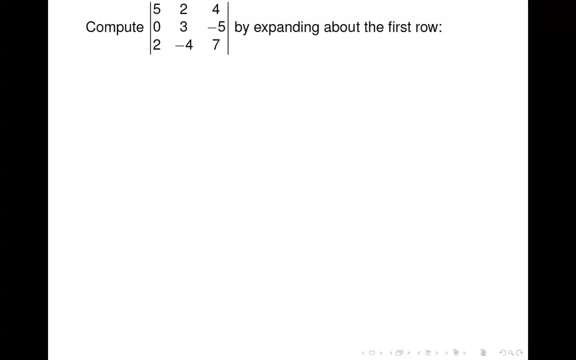 zeros in it, because that eliminates some of the terms. But for our first cut here I'm just going to expand about the first row And I've kind of color coded this to make it easier for you to see where the terms come from. 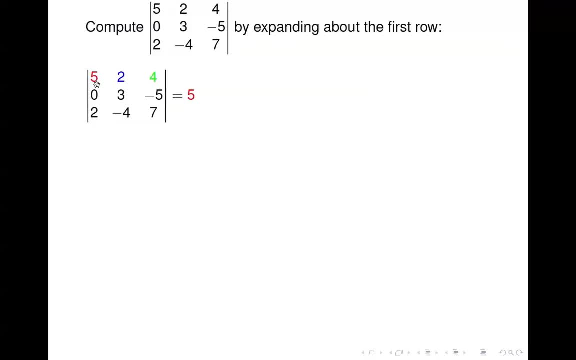 Okay, So if we expand about the first row, we start with the first entry, which is the 5.. And then we multiply 5 by the determinant of the matrix that you're left with if you eliminate the row and the column that contain the 5.. 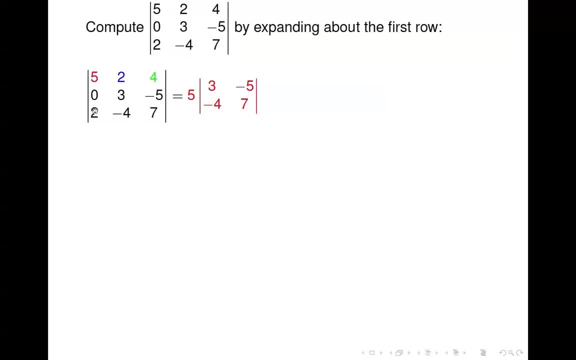 So if you eliminate the first row and eliminate the first column, then you see that you have this little 2x2 matrix that's sitting right here. Okay, So we take the determinant of that And then we move over to the next entry in the first row, which is the 2.. 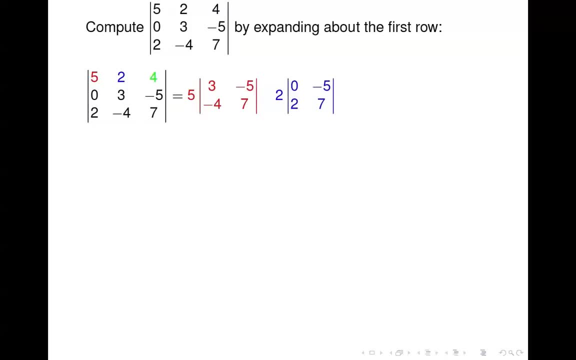 And we multiply that by the determinant of the matrix that you get if you eliminate the first row and the second column, Okay, The row and the column containing the 2. So we're left with the 0, 2 here and the negative 5, 7 here. 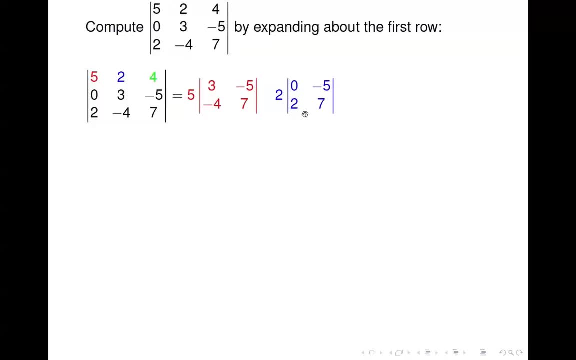 Okay, So that's how we get this matrix here And we continue moving across The first row. Then we've got a 4.. And we multiply 4 by the matrix that you get if you eliminate the first row and the third column. 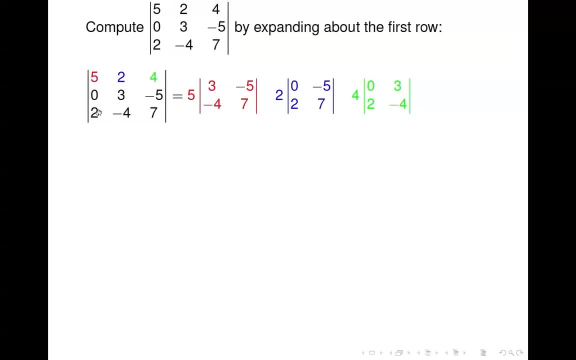 Okay, Eliminate the row and the column containing the 4.. So you're left with this little 2x2 here: 0,, 3,, 2, negative 4.. And that's what we have here Now. notice, I haven't combined these terms at all. 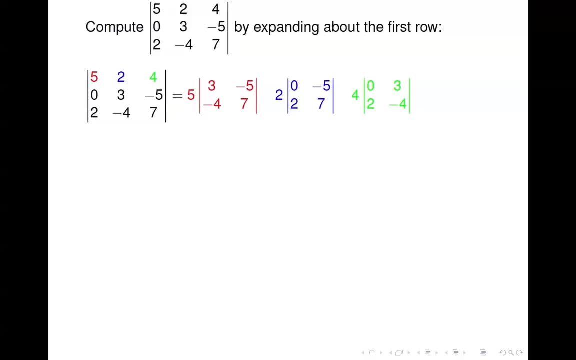 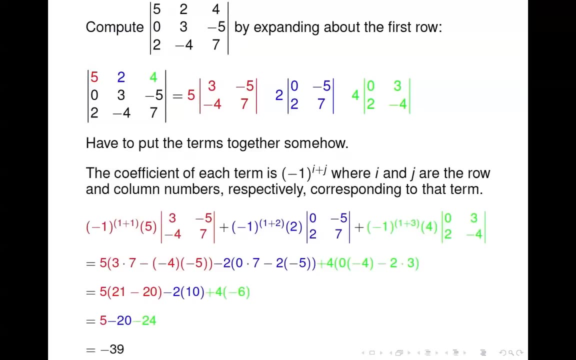 I've just written them out here, And that's because there's a method for combining the terms. Okay, We have to put them together somehow And basically you apply a coefficient to each term which is negative, 1 to the i plus j. 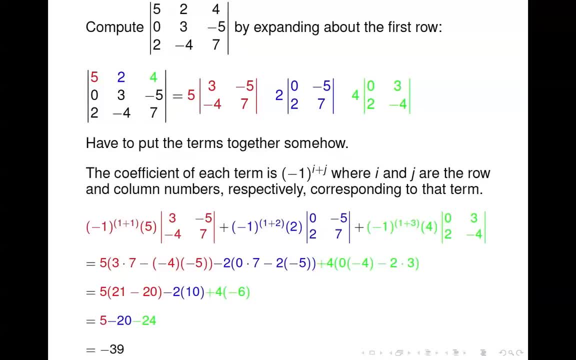 where i and j are the row and column indices corresponding to that term. So if we look back up the 5, 5 came from row 1, column 1.. So the coefficient that we put in front of that term is minus 1 to the 1 plus 1.. 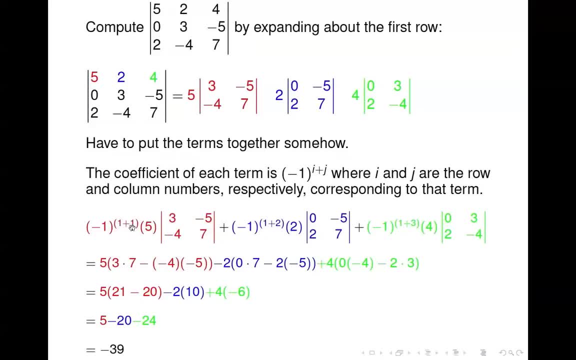 Because 5 came from row 1, column 1.. Alright, Then for the next term, this one, the 2, the blue term came from this entry. here The 2 is in the first row, second column. So that means the coefficient here is minus 1 to the 1, plus 2.. 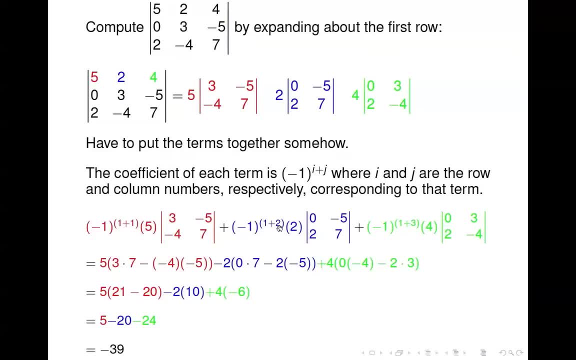 Row 1, column 2, that's where the 1 plus 2 comes from, And then for the 4, the green term. okay, it's in the first row, third column. So we have minus 1 to the 1 plus 3 as the coefficient in front of that term. 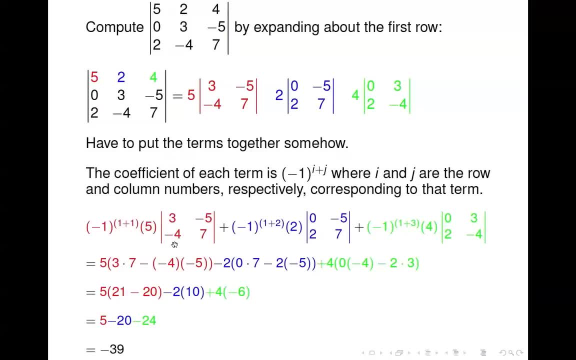 Okay, And so if we multiply and add, then what do we get? We get minus 1 to the 1 plus 1, so that's minus 1 squared, So that's just plus 1 times 5.. So we bring down 5.. 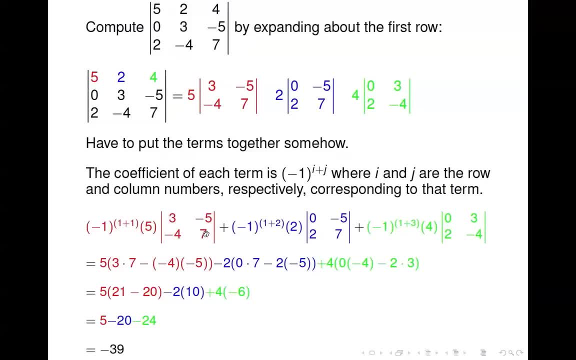 And then the determinant here, remember, it's just the crisscross: 3 times 7, minus negative, 4 times negative 5.. So that's what we have here. Alright, Then, moving on here to the blue, we've got minus 1 to the 1 plus 2.. 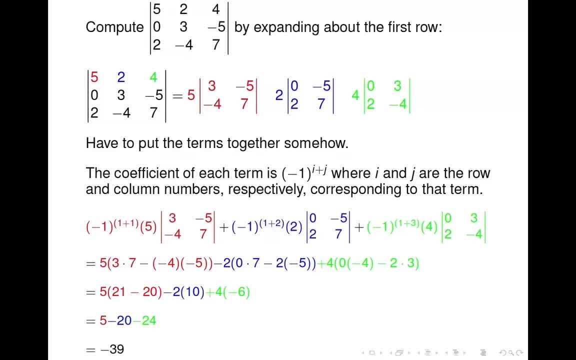 That's minus 1 cubed, So that's negative 1 times 2, gives us the negative 2 here times the determinant, which is 0 times 7 minus 2 times negative 5.. Alright, Then, moving over to the next term. the green one comes from the 4.. 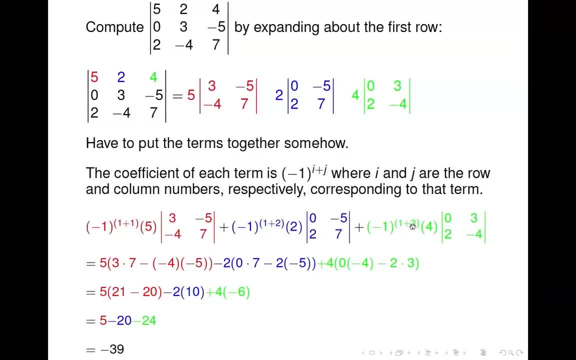 And that's first row, third column. So that's the minus 1 to the 1 plus 3.. Which is minus 1 to the 4, which is positive 1 times 4.. And so you get a plus 4 in front of that term times the determinant, which is 0 times negative. 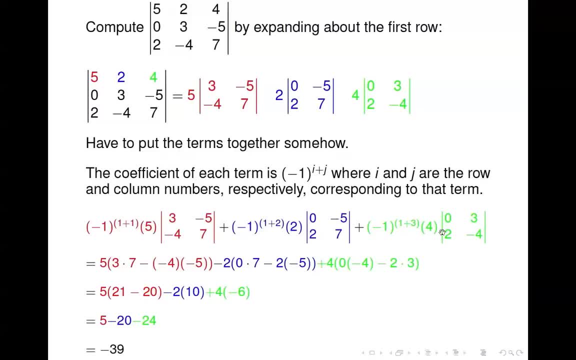 4, minus 2 times 3.. Alright, And then, combining a little more, we've got 21 minus 20 here times 5. Then we've got 0 plus 10. So just a 10. There. 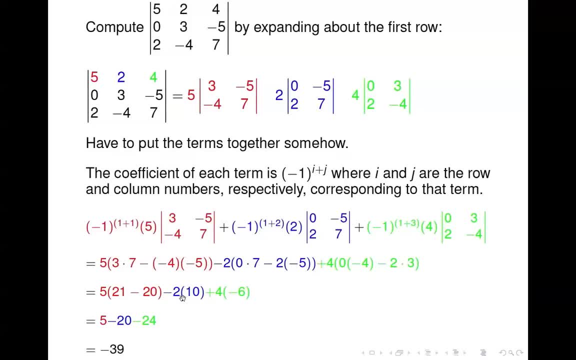 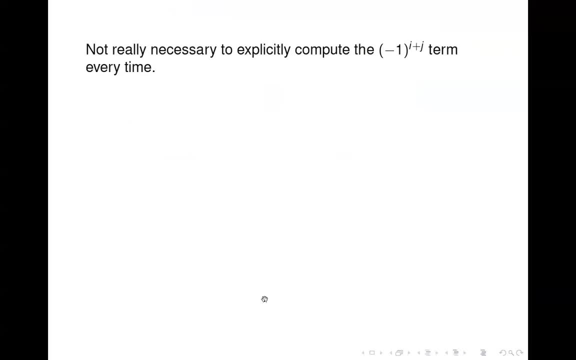 And then here's 0 minus 6. So negative 6 there, And we combine and we end up with negative 39 for the determinant of this matrix. Okay, Now just a little aside. it's really not necessary to explicitly compute this minus. 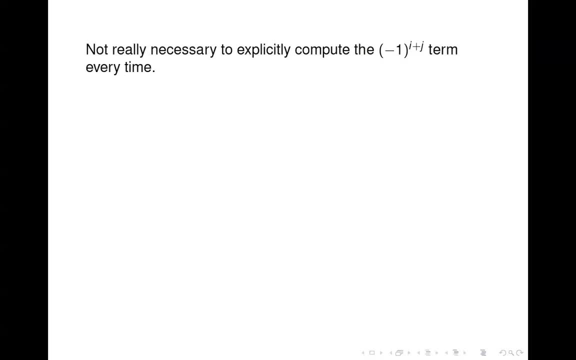 1 to the i plus j term every time. If you just look, here's a 4 by 4, where I've put as the entries in the matrix just the row index plus the column index. So 1, 1 position, we've got 1 plus 1.. 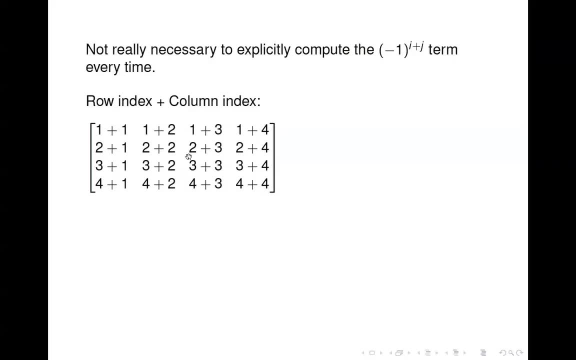 1, 2 position, 1 plus 2, and so forth. So if we look at what that is, we end up with these numbers And remember we want minus 1 raised to each of these powers. And so you can see, since they all differ by 1, going from one term to an adjacent term. 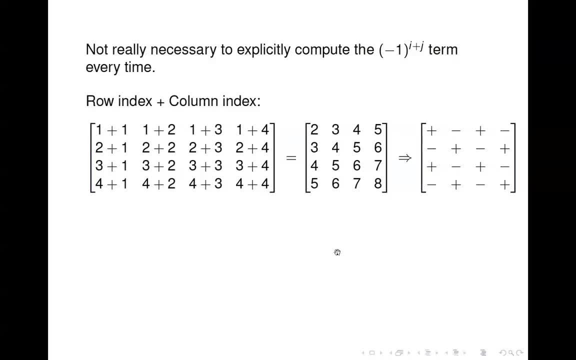 either in the same row or the same column, you either go from an even number to an odd or an odd to an even, So in any case, you're going to end up with an odd. So, in any case, alternating terms are always going to have opposite signs. 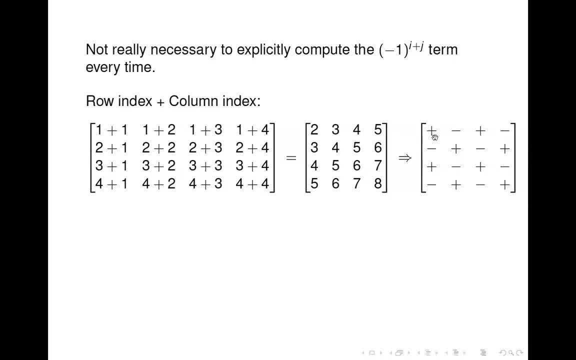 And you always start off in the upper left with a plus plus 1,, because that's minus 1 to the 1 plus 1, or minus 1 squared. So you always know that the 1, 1 position is a plus term. 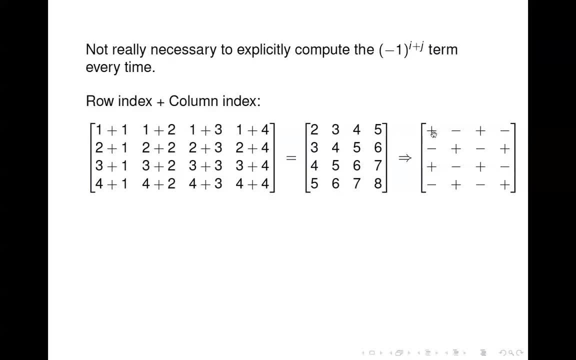 And then everything alternates after that, So it's always plus minus, plus minus. So if you know the sign that goes with the first term In the row or the column that you're expanding about, then you only need to alternate terms. 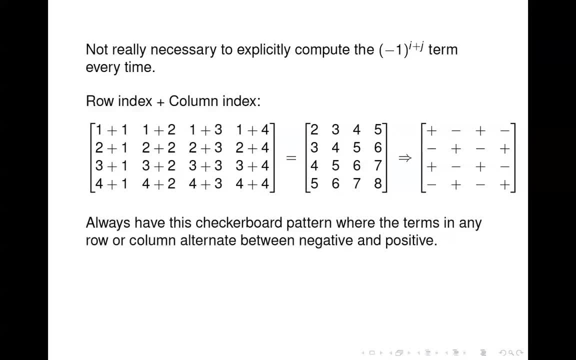 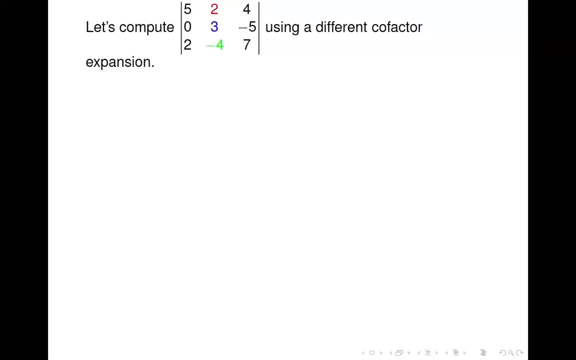 after that: Right, So you always have this checkerboard patterns And you just need to alternate terms based on the sign of the position where you start. So let's look at this matrix again. It's the same one, but I'm going to expand about the second column this time. 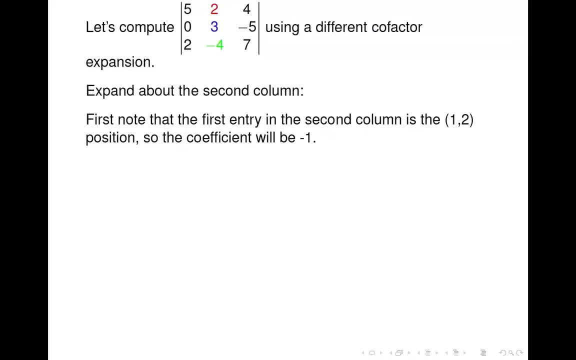 All right, Just for something different. Now, first note that the second column, or the first entry there, is the 2. And it's in the 1, 2 position. So minus 1 to the 1 plus 2, if you want to compute it like that. 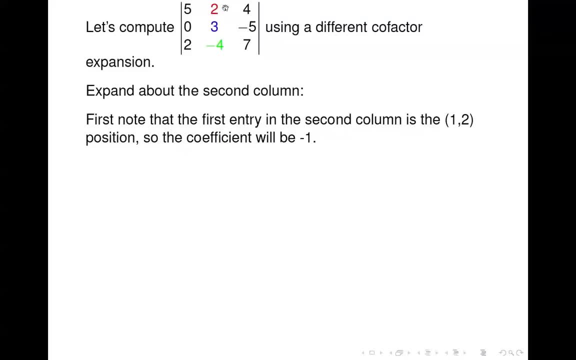 Minus 1 cubed, that's a negative 1.. So this is a negative position here. Or you can say: I always know that the 1, 1 position is a plus, So this is plus. The next one over has to be a minus. 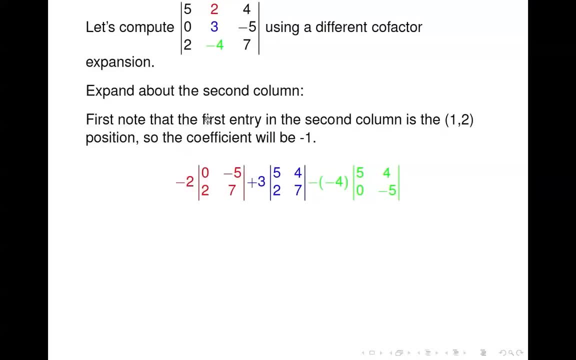 That's typically how I do it, All right. So we end up with minus 2 times All right Times, again the determinant of the matrix that you get if you eliminate the row and the column containing the 2.. So we end up with a 0, 2, negative 5, 7.. 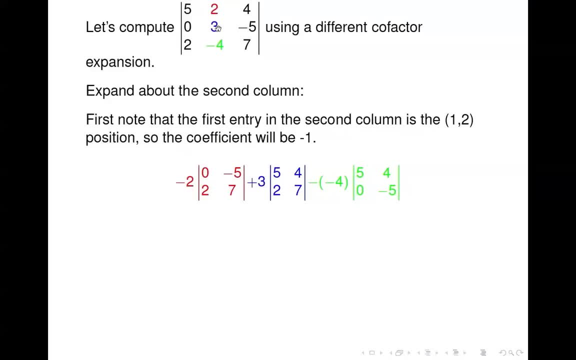 So that's where we end up with that matrix, All right, And then we move to the 3.. Now, since the 2 was a negative, the 3 is going to be a plus, And we eliminate the row and the column containing the 3.. 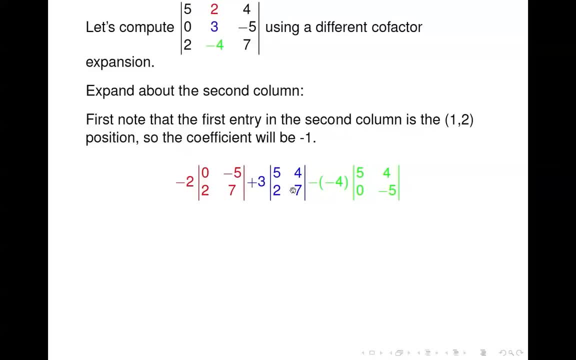 So we're left with 5,, 4,, 2,, 7.. And then we move on to the 3. We move on to the negative 4.. So again, if you forget, we'll go back to the 1, 1.. 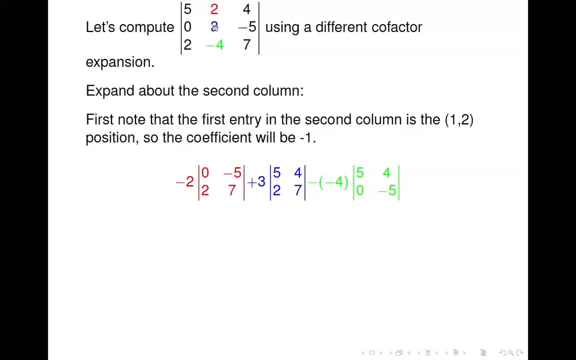 That's a plus. Moving over, that's a minus. Moving down, that's a plus. Moving down again, that's a minus. So we're going to subtract off: That's where the minus comes from. Minus negative: 4 times the matrix that you get if you eliminate the last row. 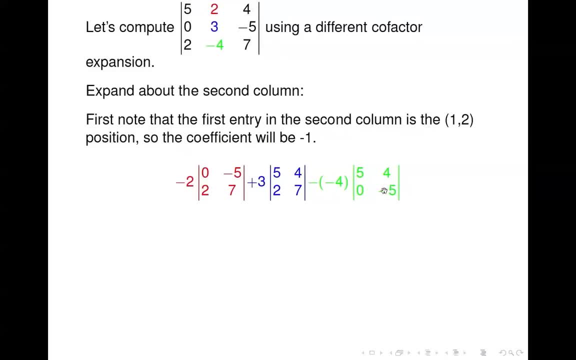 and the middle column. So we've got 5, 0, 4, negative 5.. All right, We compute those determinants Here. we're going to have 0 times 7.. Minus, Minus, 2 times negative 5.. 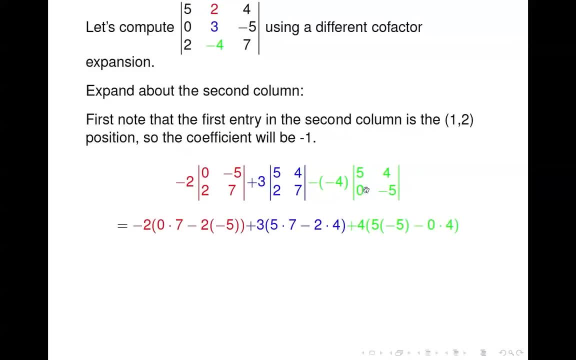 Here 5 times 7. Minus 2 times 4. And here 5 times negative 5. Minus 0 times 4. And we can simplify And we end up with negative 39 again, which we should. 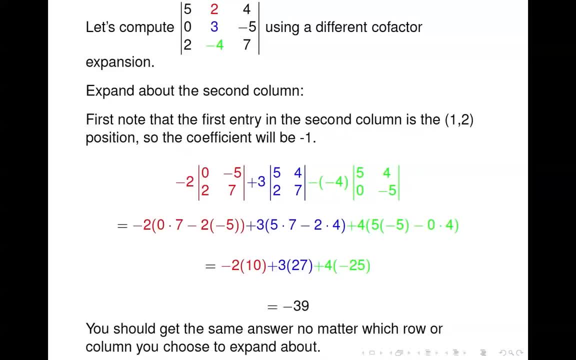 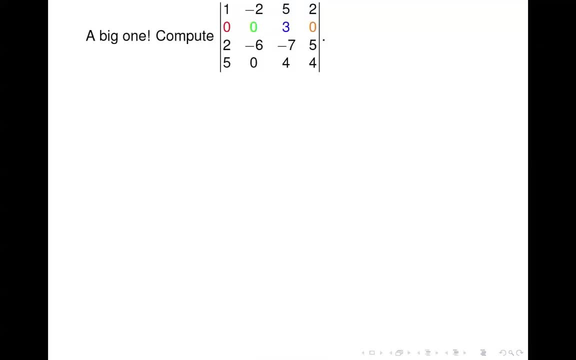 Because no matter which row or column you choose to expand about, you should end up with the same answer. Let's move on to a 4 by 4.. Now we're going to take advantage of the fact that we've got a row with three 0s in it. 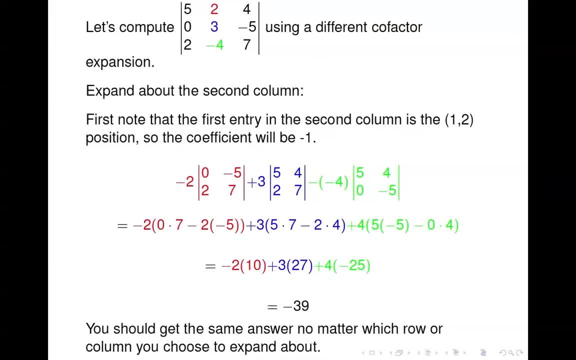 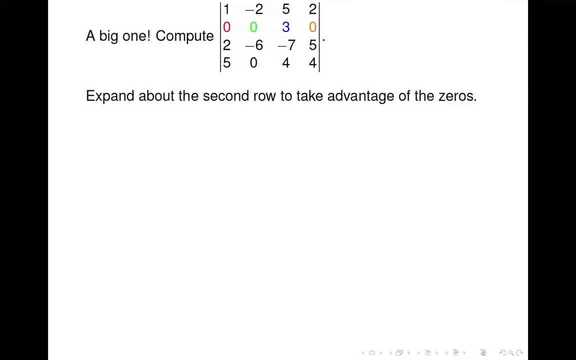 So I'm going to expand about the second row And if you notice the first entry in the second column, oops. OK, there we go. Expand about the second row to take advantage of the 0s. So if we look, 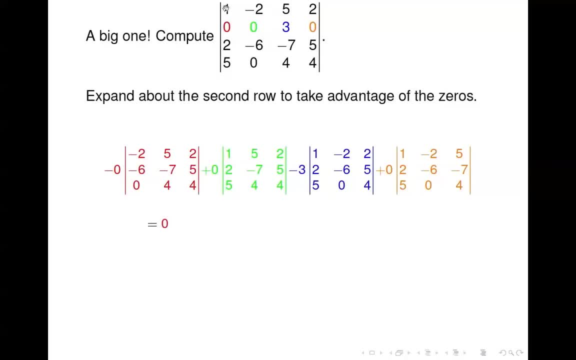 But the 0 here is, or go back to the 1, that's a plus position, So we move down. That's a minus. So the first term is going to be minus 0 times the determinant of the matrix that you get. 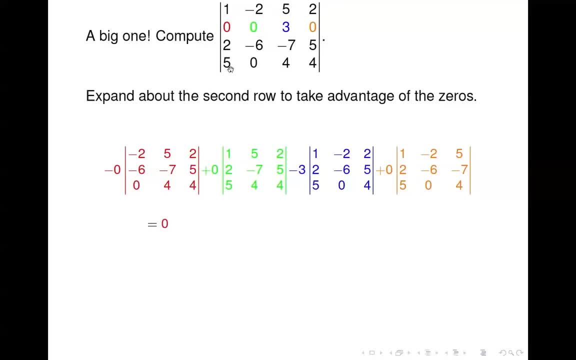 if you eliminate the second row and the first column, So you can see how the first row is going to be negative: 2, 5, 2.. That's what we get there. Then we've got these two rows right here as the second two. 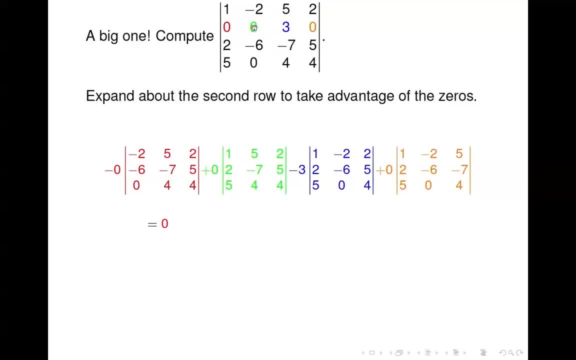 rows. All right, then we move over to the next entry. OK, plus here, minus, So this is a plus entry. So it's plus 0 times the determinant of the matrix that you get when you eliminate the second row, second column. 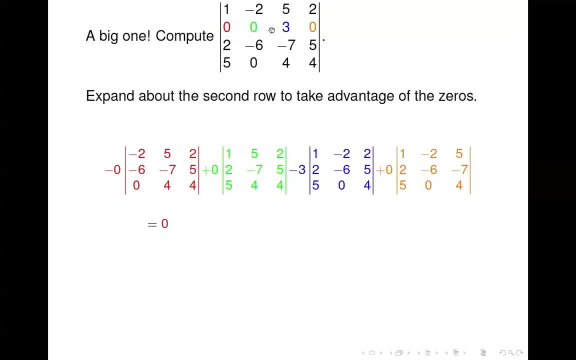 All right, then minus the next term, So minus 3 times the matrix that you get if you eliminate second row, third column, And then plus 0 times the determinant of the matrix, So you get minus 0 times the determinant of the matrix. 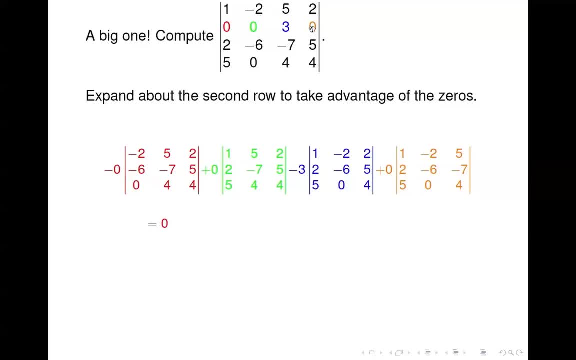 that you get when you eliminate the last column and the second row. So that's where all these terms come from And you can see the advantage of choosing a row with a bunch of 0s, because the red term, the green term and the orange term 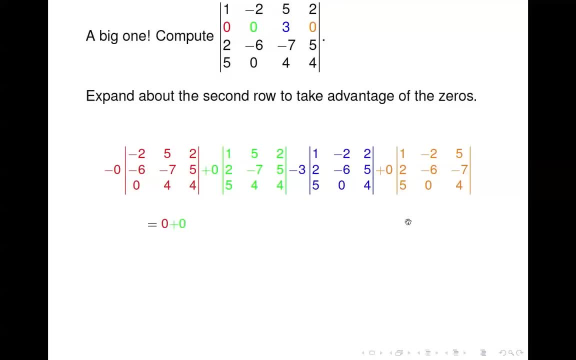 all just disappear because they are all multiplied by 0. The blue one, though. we have to compute now A 3 by 3 determinant, So we have negative 3 times the determinant of this matrix. So we use the same method. 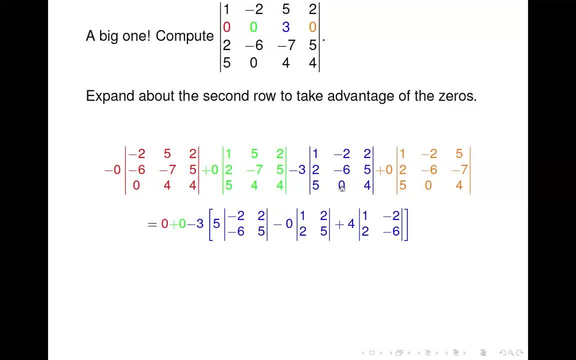 Choose a row or a column to expand about. I chose the third row. OK, So I've got plus minus plus 5's in a plus position, So it's 5 times this 2 by 2 determinant here. 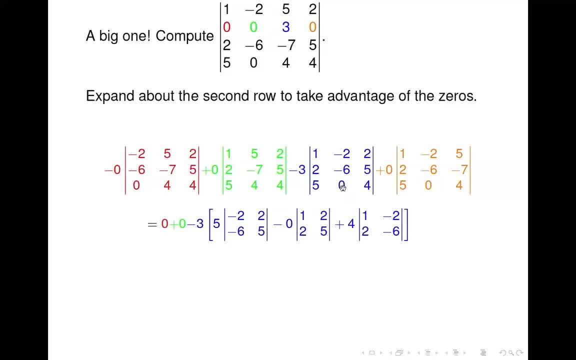 Then move over: minus 0 times the 1,, 2,, 2,, 3.. 2,, 5.. And then plus 4 times the determinant of this little matrix up here right, And then plus 0, because this term is multiplied by 0.. 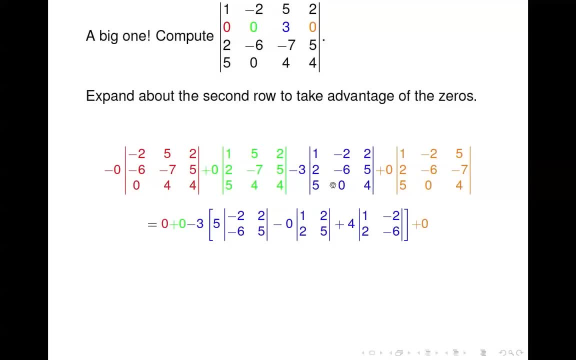 So you can see that everything simplifies except for this blue part. And we go through and evaluate these determinants And combine terms and simplify and we end up with negative 6 for the determinant of the matrix. Now just stop for a minute here and think about how much more work would have been required. 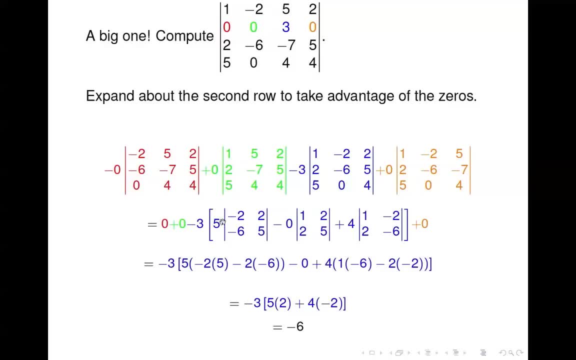 if we didn't have any 0's in this matrix, You know we would have had to done. you know what we did with the blue part. We would have had to do that for the red and the green and the orange. 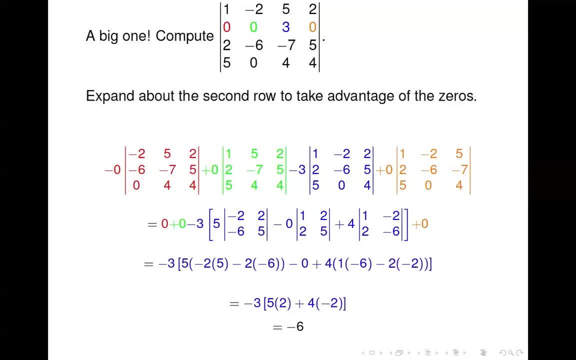 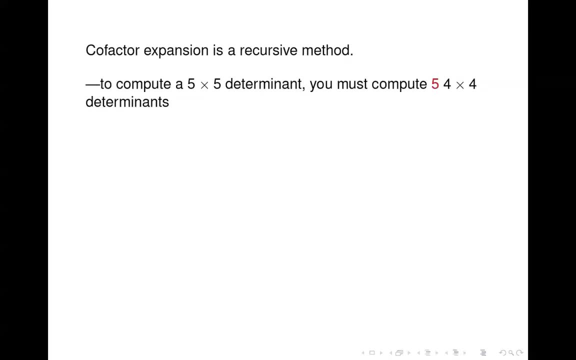 So we get this turns into significant work fairly quickly. OK, It's a recursive method because, for example, to compute a 5 by 5 determinant you have to compute 5, 4 by 4 determinants. Now this is assuming there's no 0's in the matrix. 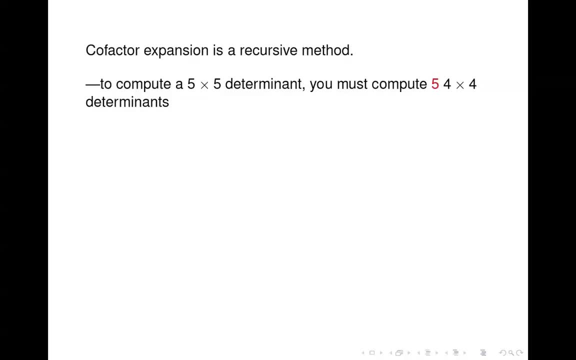 So the worst case for a 5 by 5, you have to compute 5, 4 by 4 determinants And each of those 4 by 4 determinants requires competing 4. 3 by 3 determinants And each 3 by 3 means you have to compete 3, 2 by 2 determinants. 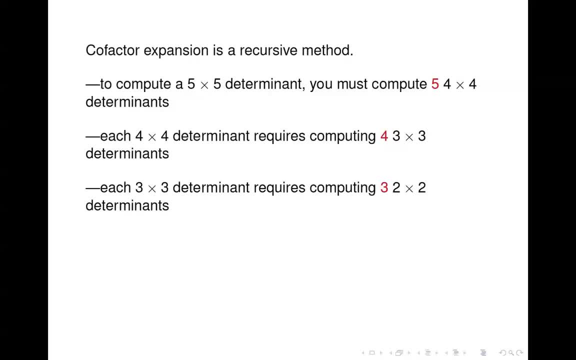 As you can see, this gets very work intensive very quickly. The amount of work increases exponentially. so clearly this method does not scale well at all. as your matrix gets bigger, the amount of work required increases exponentially. so it's not a good tool in our good method to use to compute the determinant for an. 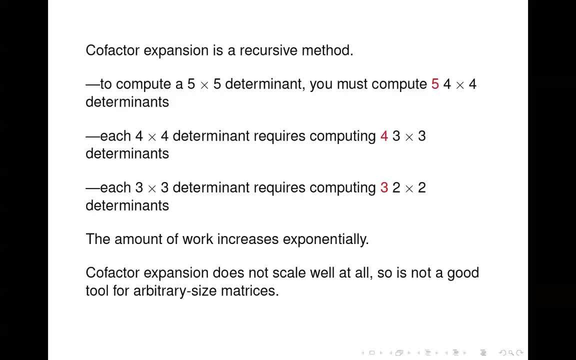 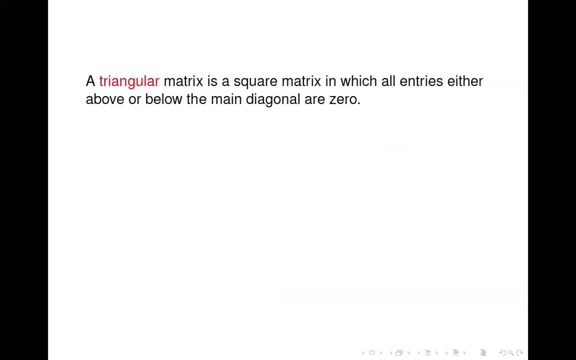 arbitrary size matrix. three by three is okay, four by four really turns into too much work, unless you've got some significant number of zeros there. okay, now let's let's go off on a little different tangent here for a bit and first define what a triangular matrix is. a triangular matrix is a square matrix. 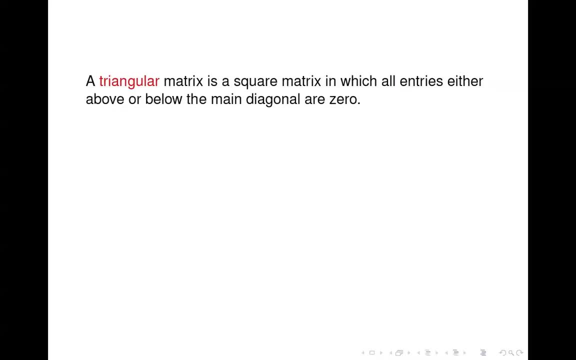 in which all the entries either above or below the main diagonal or zero. okay, so here are some examples. I've highlighted the zeros in red just to make it clear. the first one here has all zeros below the main diagonal. so we say that this matrix is upper triangular. 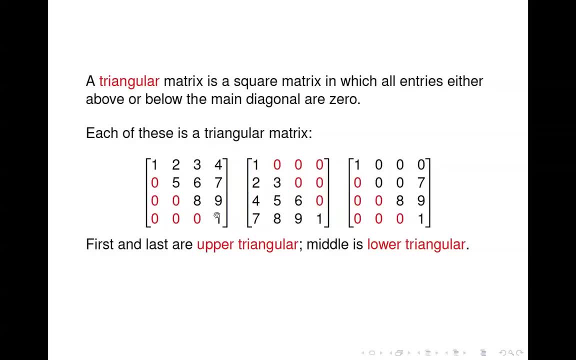 so all the interesting stuff is in the upper part of the matrix. this next one, the middle one, is lower triangular, because all the interesting stuff is in the lower part of the matrix. everything above the diagonal is zeros. and then here's another. you can see that the matrix is a square matrix and the upper part of the matrix 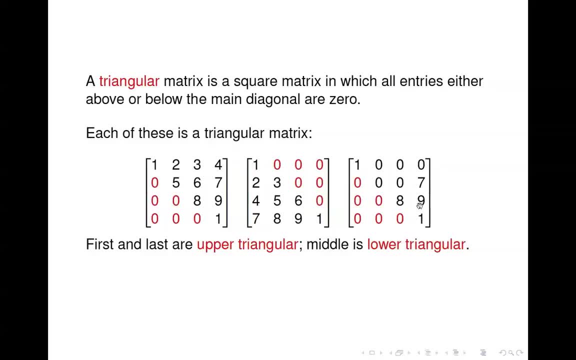 is also a square matrix. and then here's another one. this one is upper triangular also, and I just want to make it clear that what defines a triangular matrix is that either above or below, or even both the diagonal, you have to have all zeros. so this one is upper triangular because below the diagonal we have all zeros. 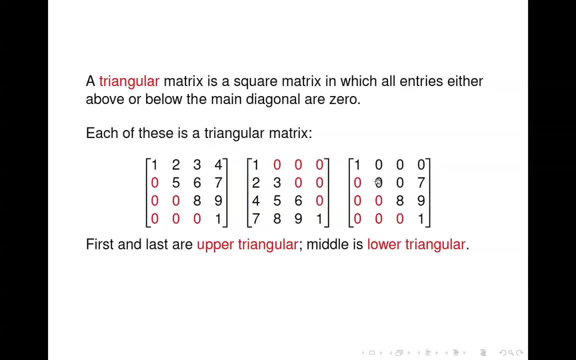 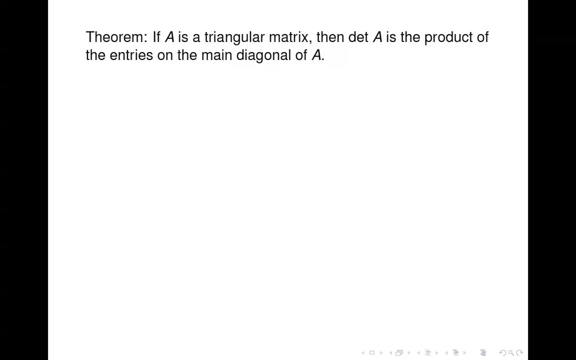 that's okay to have some zeros above the diagonal or even on the diagonal, but that has really nothing to do with whether this is a triangular matrix or not. this is a triangular matrix because everything below the diagonal is zeros, all right. so we have a theorem that says: if a is a triangular matrix, 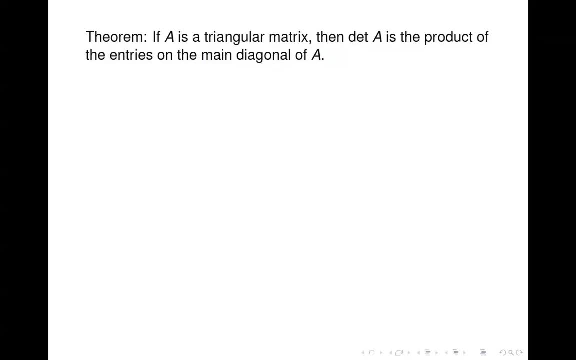 then the determinant of a is the product of the entries on the main diagonal of a. okay, so this is this is making it easy to compute the determinant if your matrix is triangular. okay, it's pretty easy to see how that works if we take a triangular matrix. 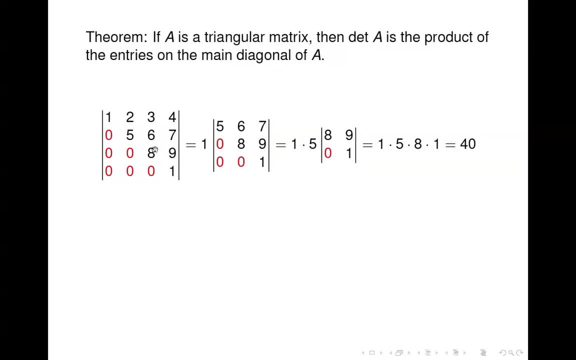 Then if we were going to compete the determinant directly, then I would expand about the first column, So my determinant would be 1, that's a plus, So 1 times the determinant of the matrix that you get if you eliminate the first row and 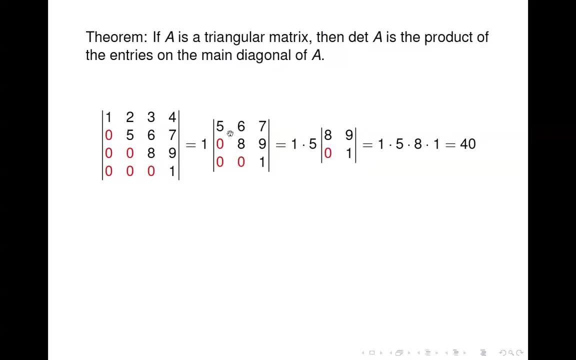 first column. So you got this 3 by 3 that we take here And notice that all the rest of the terms would be 0. So it's 1 times this determinant plus this 0 here times. actually, minus this 0 here times. 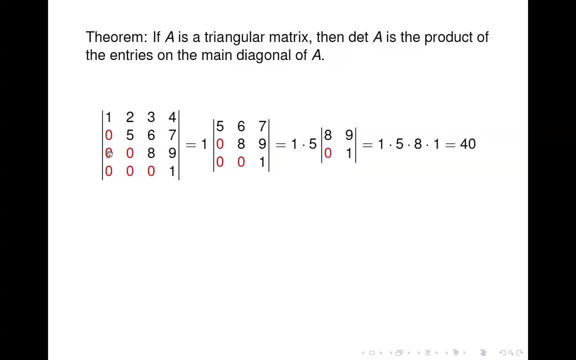 another determinant, plus this 0 times another determinant, minus this 0 times another determinant. So the only term that's non-zero is the one associated with the 1. So that's the only one I've written here. And then, if we take the determinant of this 3 by 3, notice we do the same thing: expand. 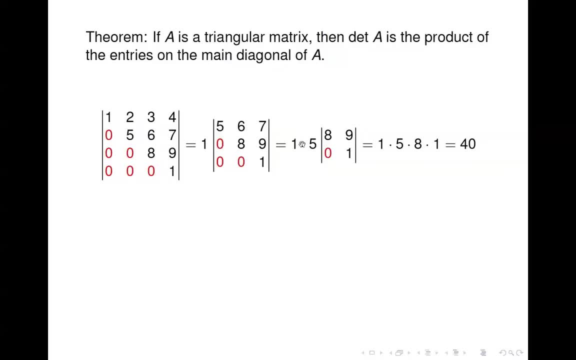 about the first column. So we've got 1 times 5.. Because 5 is in the 1, 1 position, So that's a plus. So 1 times 5 times this, 2 by 2, sitting right here. 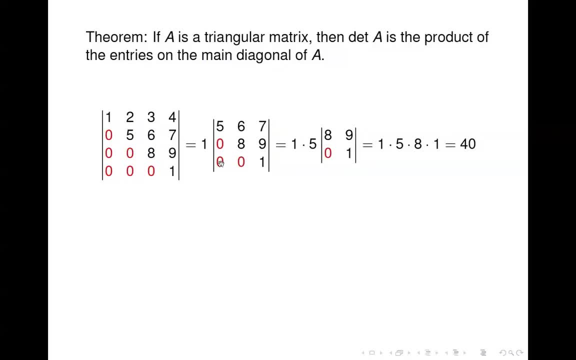 And notice again, all the other terms in that column are 0. So we don't need to worry about them, And so we end up with 1 times 5 times this determinant, And so it's going to be 8 times 1 minus 0 times 9.. 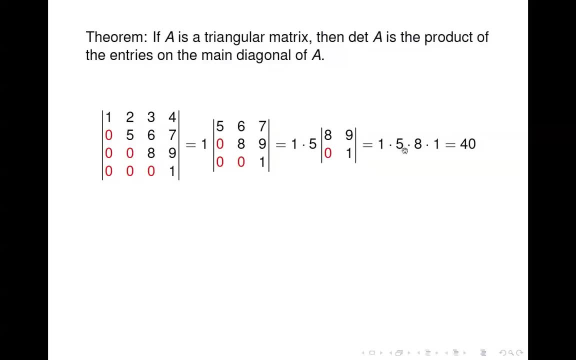 So it's just 8 times 1.. So our determinant is 1 times 5 times 8 times 1.. Which, you see, are the intervals. Okay, So we're going to multiply the entries on the main diagonal. So if your matrix is triangular, life is good, life is easy. 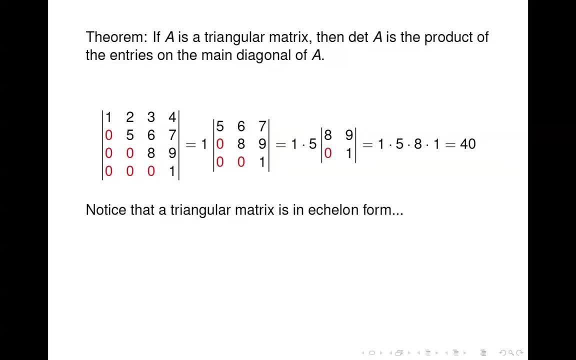 Just multiply the entries on the diagonal. Just thinking ahead just a little bit, notice that a triangular matrix is in echelon form. Or if it's upper triangular, it's in echelon form. If it was lower triangular, we could swap rows. 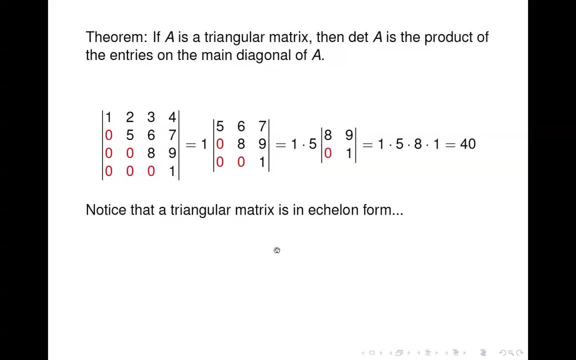 We could swap some columns too, But let's just think about upper triangular at this point Now. so something to think about. To compute the determinant of a large matrix, let's just say large is 4 by 4 or bigger- could we first put it in echelon form and then just take the determinant by multiplying? 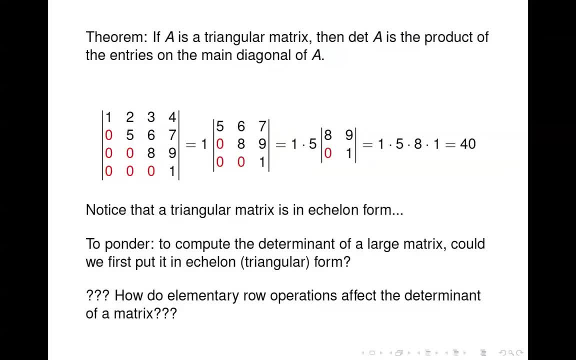 the diagonal entries. Would that work Well, to answer that, we need to explain, We need to explore how elementary row operations affect the determinant of a matrix. Okay, So if we can nail that down, then it is indeed possible that we could just put our matrix. 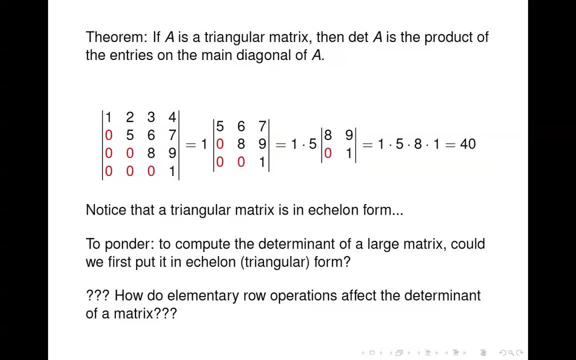 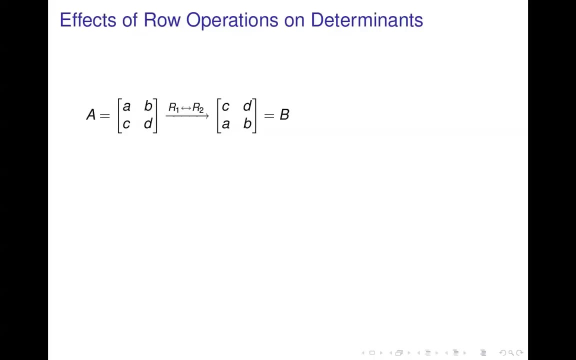 in echelon form and then easily compute the determinant that way. So that's what we'll ponder and we'll discuss that in the next section. Okay, Last time we talked about Okay, We talked about how to compute the determinant of a matrix and we discovered that, as the 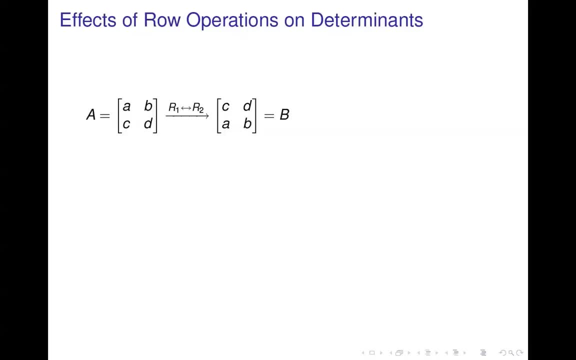 matrix got larger, the amount of work required to compute the determinant increased dramatically, Even a 4 by 4 without any zeros in it is a considerable amount of work to take the determinant of. So we thought that. Oh, We also saw that. 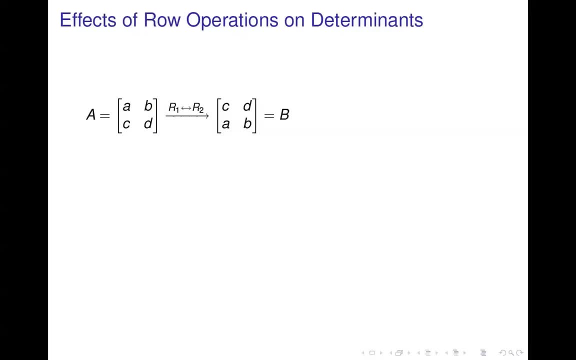 For If the matrix is triangular, then computing the determinant is easy: Just multiply the diagonal elements. And so we thought: hmm, I wonder if we could just do some row operations and either just generate some zeros or get the matrix totally in echelon form. 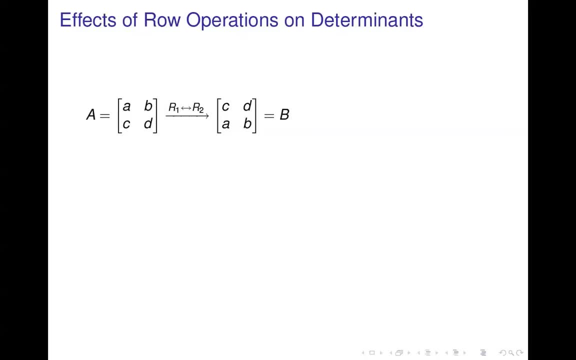 Which would be upper triangular form, and then compute the determinant to, just so we can eliminate some of the work required. So we're going to first talk today about how row operations affect the determinant, Because if you do row operations, you need to know what effect that has on the determinant. 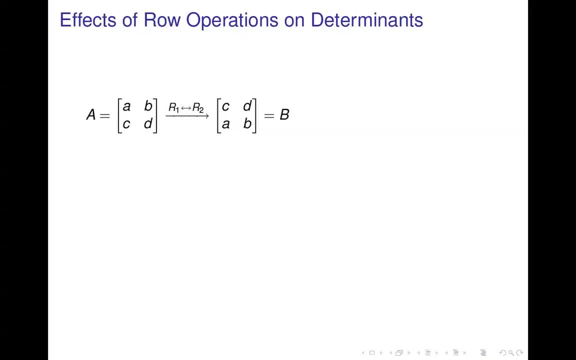 If you're going to try to go down that road in order to compute the determinant. Okay, So the first thing we'll look at is the effect of swapping rows. So the example I have here: I just swapped the rows. So the first matrix I call A, swap the rows, call that matrix B, And obviously we know. 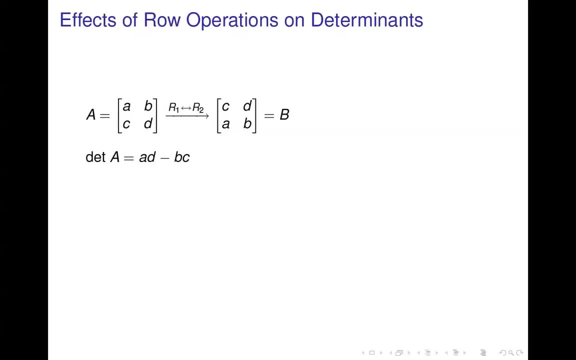 the determinant of A is just AD minus BC. The determinant of B is BC minus AD, Which is the negative of AD minus BC. Okay, So we have the determinant of A equals minus the determinant of B, And this holds true no matter what size your matrix is. 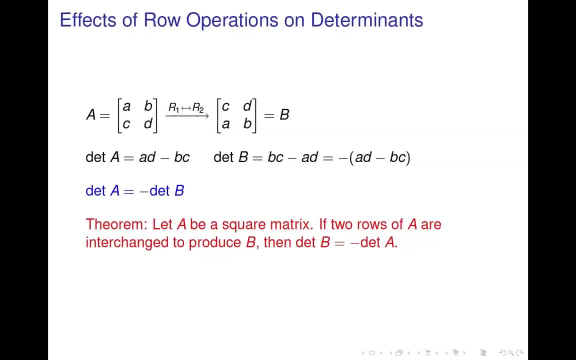 So we have a theorem that says: if you have a matrix A and you exchange two rows or swap two rows of A to produce B, then the determinant of B is just the negative of the determinant of A. Okay, Okay, So if you swapped rows again, you'd negate the determinant again. 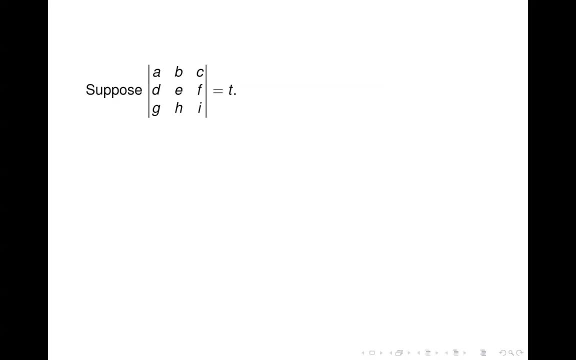 So suppose we have this example. It's a three by three. Let's just suppose the determinant of this matrix is T. Then we swap the first two rows and the determinant of this matrix. we've negated the determinant of the original one. 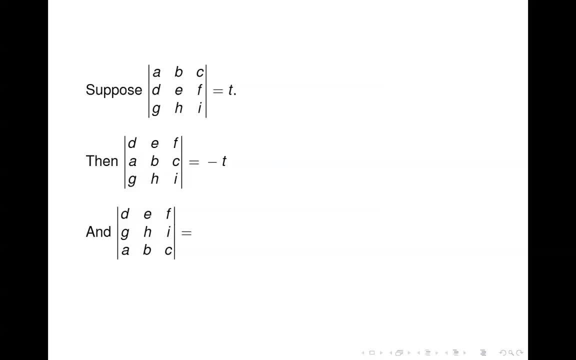 So the determinant of this one is negative T. Then if we swap two rows again, then we've got the determinant of the original matrix. Okay, so to get to this, this matrix- here I have interchanged the second, third rows of the previous matrix and so I've negated the determinant again. so it's. 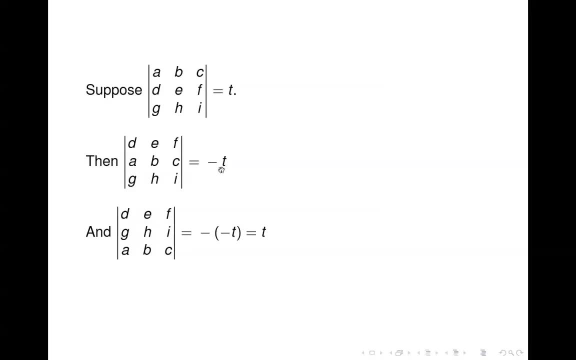 the determinant will be negative of the determinant here, which is negative T and notice, we're back to where we started. so as you interchange rows, that just negates the determinant. so it if you do two of them, then you're back to where you started. all right, another row operation. here we're. 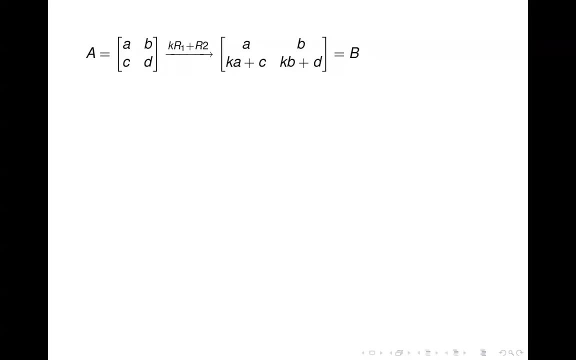 multiplying a constant by one row and adding to another. so again the term of a is just a D minus BC. determinant of B is a times K B plus D minus B, times K a plus C, and we can do a little algebra. notice that the K a, B terms of 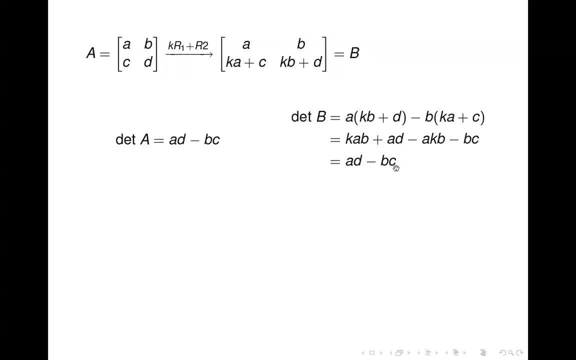 two of them and they cancel each other out. so you're just left with a D minus BC. so this: with this row operation you don't change the determinant at all, which is kind of nice, because we know that when we're doing row operations on a matrix, this is the one we're doing 99% of the time, and so it has absolutely no. 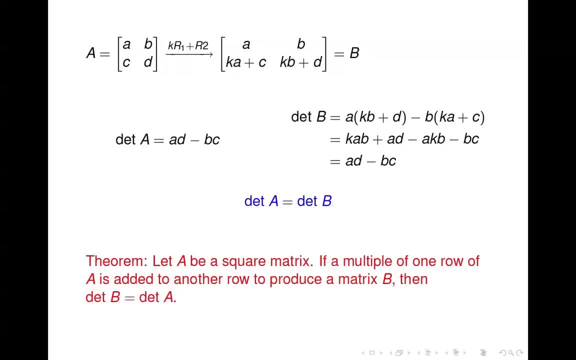 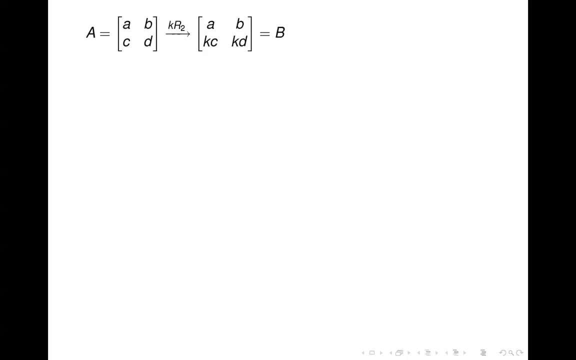 effect on the determinant. okay, so another theorem: if you multi, if the multiple of one row of a is added to another row to produce a matrix B, then the determinant of B is equal to the determinant of a. okay, the third row operation is multiplying a row by a. 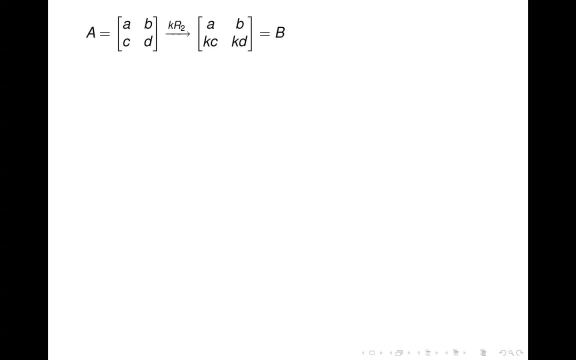 constant. so here I've multiplied row two by K, so again determinant of a, a, D minus BC. determinant of B: it's a times K, D minus B, times K C, and factor out a, K and you know K times a, D minus BC. so we see that. 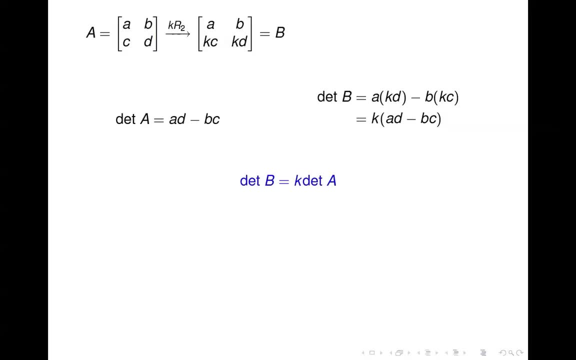 the determinant of B is K times the determinant of a. or when you're going backwards, you know if you were using the determinant of B to try to, to go back, to get the determinant of a term- a, B 1 over K times the determinant of B, so another. 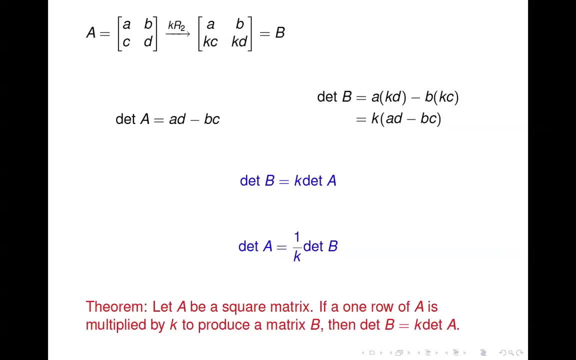 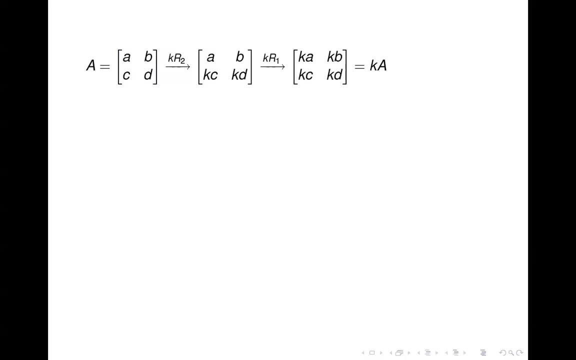 theorem: if a row of a is multiplied by K to produce a matrix B, then the determinant of B is equal to K times the determinant of a. that holds true for any square matrix. a kind of tagging along with this. I said what happens if we multiply the whole. 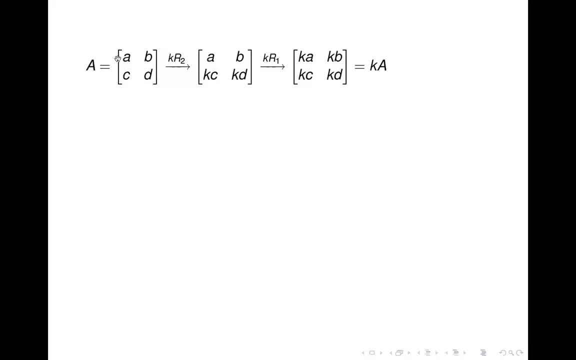 matrix by a constant. okay, so start off with our ABCD. multiply one row- this is the matrix we had before. multiply it by row two, by K, to get this matrix. then I multiply, Wrote one by say, to get this one's, which is just equal to K times the whole matrix. so we know. 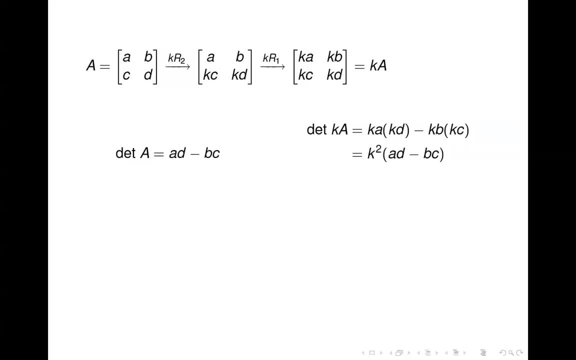 determinant of a is 80 minus B C, the eternal K a. take the term to this matrix. we end up with K squared times a D minus b c, which makes sense because we know. we know what the determinant of this one is. one is right, it was the one we looked at previously and it was just K times the. 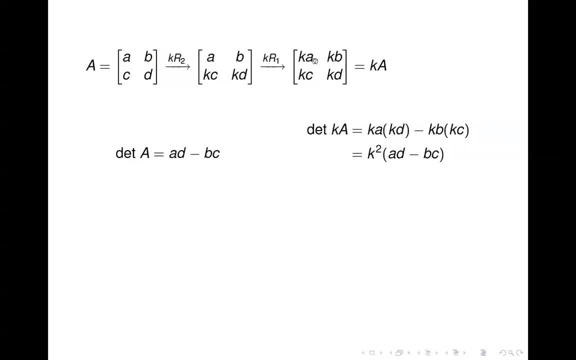 determinant of a. so we just did one more row operation, multiplying a row, another row by K, and so we should incur that K term one more time, and hence we get the K squared. okay, so the determinant of K times a matrix. now this, this is just in. 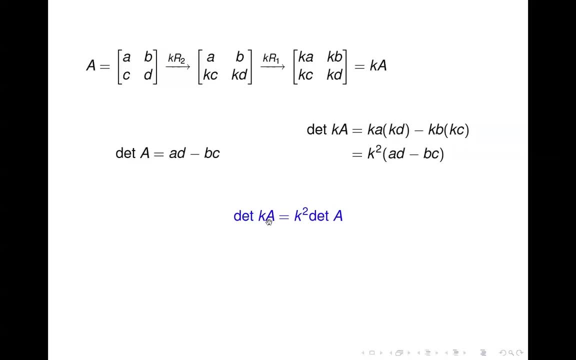 general not a row operation here, but if you just multiply K times the whole matrix, you get K squared times the determinant of a. that's for this case with a two by two. notice that if a had been 3 by 3 we would have had to. 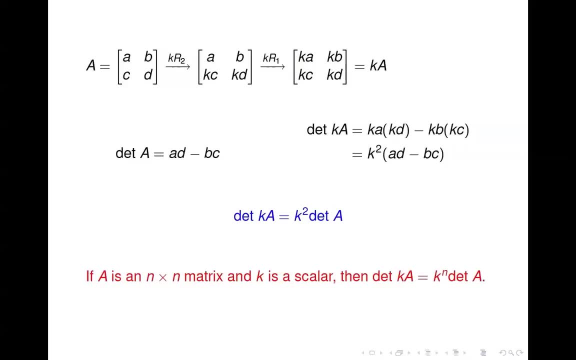 multiply each of three rows by K and we would incur that K term three times, not two is in this case. so in general, if a is n by N and K is the scalar, then the determinant of K times a is K to the end times the determinant of a as a Gesetz. am I right? 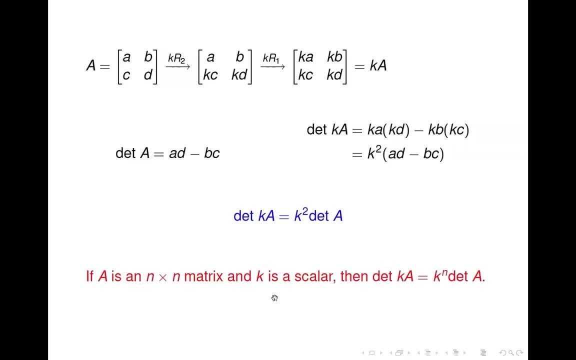 determinant of A. So if A is 3 by 3, you're going to get k cubed. If it's 4 by 4, you're going to get a k to the fourth term. Okay, so here's an example of how. 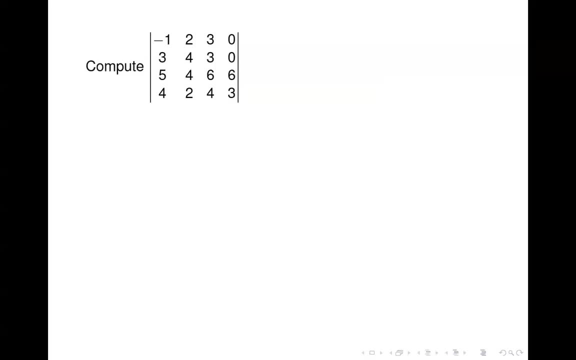 you can use these ideas that we've talked about to compute the determinant. Now, if we were just doing this one straight away using cofactor expansion, we would clearly expand about the fourth column here. But notice that it's simple to do one row operation here. 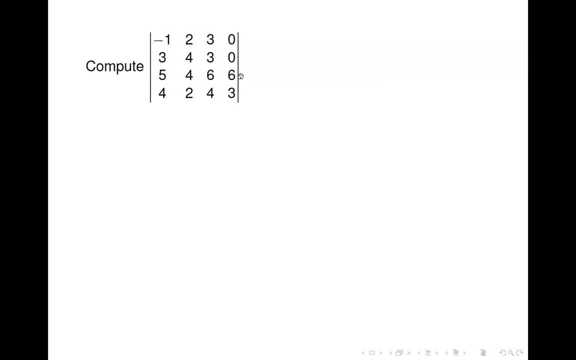 and generate another zero in this column, which will eliminate a significant amount of work. You know, as it is, we would need to do two 3 by 3 determinants, But if we do one row operation to generate a zero here where the 6 is, then we've 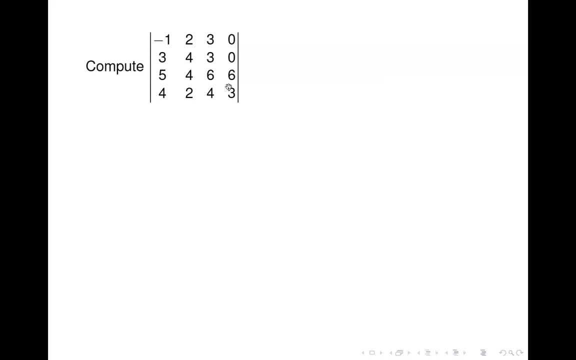 cut our work in half, because then we only need to evaluate one 3 by 3 determinant. So let's do 2 times row 4, or negative, 2 times row 4 plus row 3. And notice that that kind of row operation 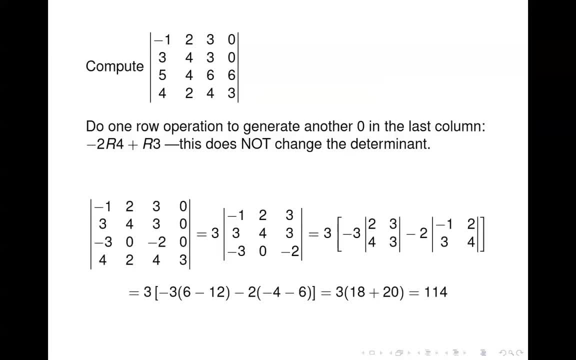 does not change the determinant. Okay, so if we do that, we can do this row operation. We get this matrix, Notice the zero here where the 6 was, And then we just expand about the last column. So we need this 3. We need to figure out. 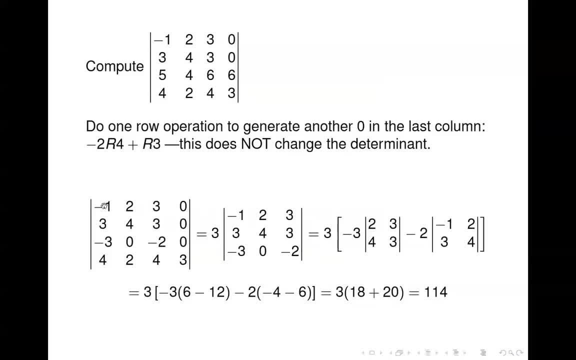 what sign goes with 3.. So start here. 1, 1 positions a: plus minus, plus, minus, plus, minus, plus. So that's plus 3 times the determinant of this 3 by 3 matrix sitting right here. 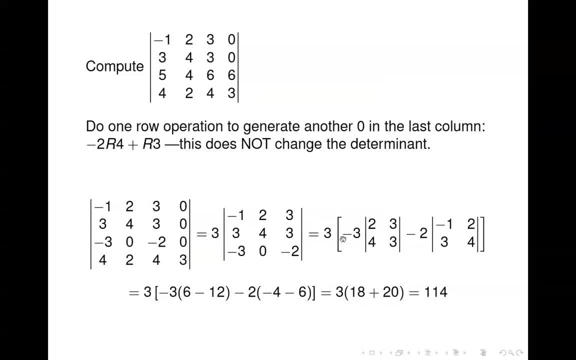 Okay, so that's what I have here. And then I've expanded about the third row And now I did 2 times the 3's on the 3 of boards. This should be a plus, Which now I'm seeing that this is not looking right. 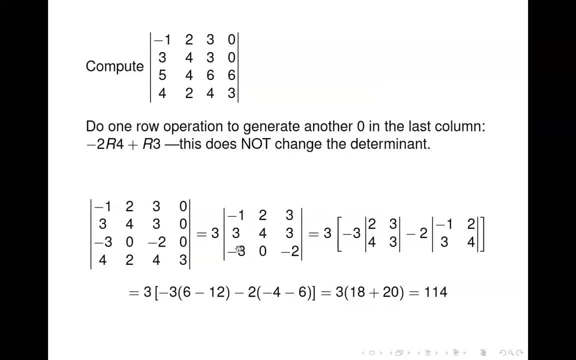 because this should be negative 3 here. Oh, no, Negative 3 here. My mistake. This 3 here comes from the ones outside. And then, when I expand about the third row, the negative 3 is right here. Alright So, and the negative 3 is in a plus position because we a start with 1, 1.. That's plus, minus plus. So we have plus negative 3 times negative five, but already multiplied which, and again times negative three and plus two here, which is negative patterns. 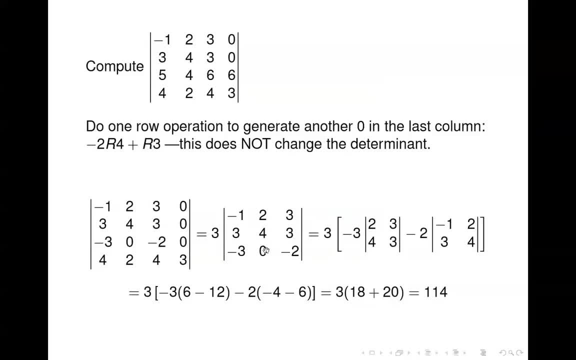 this 2 by 2, and then we got a 0, so we can skip that, so it will be minus 0, then plus negative 2, so here's the other term, and if we continue to work it out, we end up with 114. okay, so that was pretty straightforward. I want to show you one. 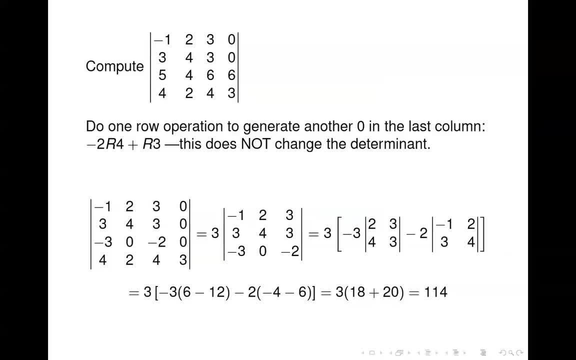 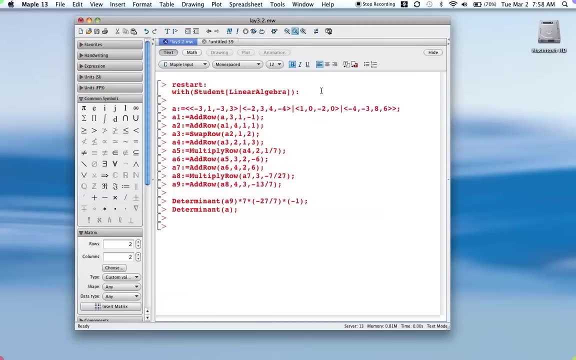 more. just that has a little more work involved, and for that I'm going to go to maple, just because that kind of makes it a little bit easier. so I've got it set up. here's the matrix that we're going to start with and notice this, I guess I 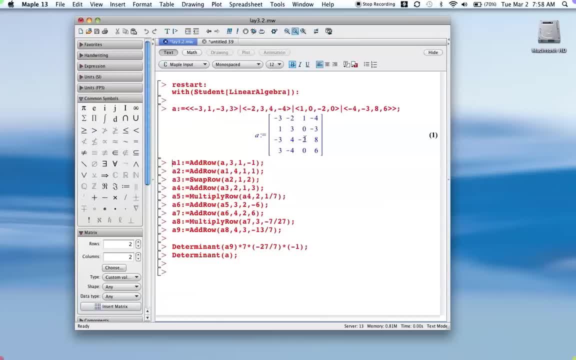 could do a row operation to generate a 0 in the third column here. that would probably make life easier be much. actually. that would be the way to go, again, if you're actually doing this by hand, but I would have wanted to illustrate the concept of of how you could use these row operations, so I have actually done. 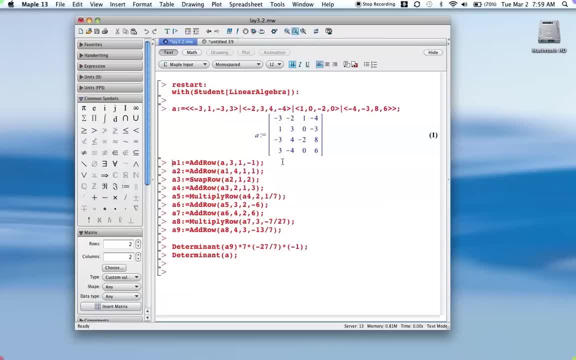 the row operations to get it in triangular form. and then I want to show you how to go back and recreate the determinant of the original matrix based on the row operations that we've done. okay, so the first thing I did was I just started out to eliminate or generate 0s in the first column, so I used the negative 3 here to 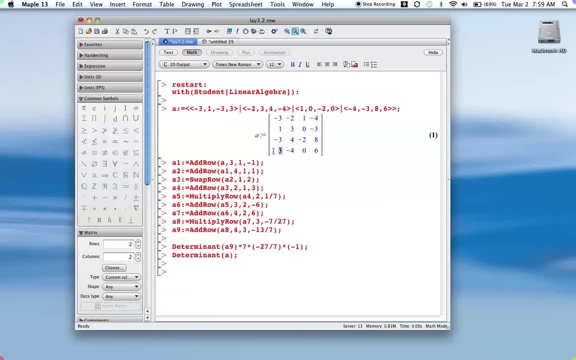 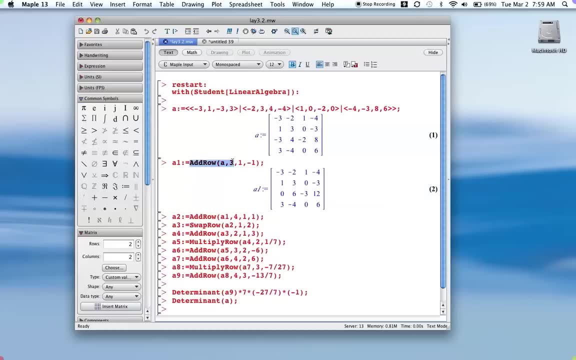 generate a 0 here and here. so first operation i did was to this: come and here, add row. what it does is take row a, so we're operating on the original matrix a and we just had the same command. all we do is go back and create row again and again, so we'll 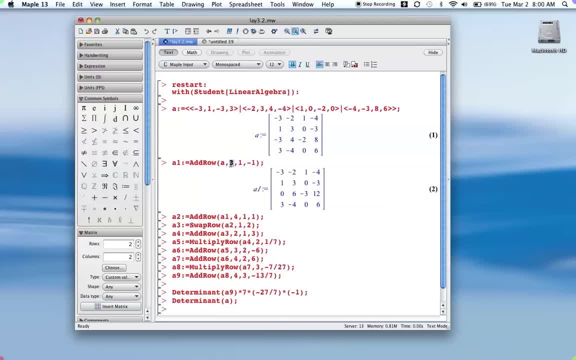 do exactly the same thing. the hand красив Fatamy. let me show you. we've got to eliminate or generate zeros in the first column, so I used the negative 3 And we're going to change row 3 by multiplying row 1 by negative 1, okay. 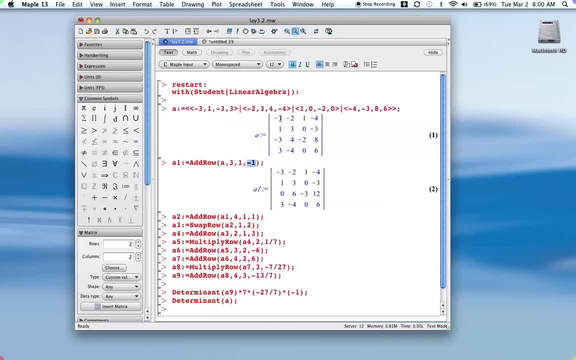 So this operation is negative 1 times row 1 plus row 3, and we generate a 0 in row 3.. Then I do row 1 plus row 4, okay, So that's the next command. Now I'm operating on A1, this matrix here, and I'm going to change row 4 by multiplying row 1 by 1,. all right, 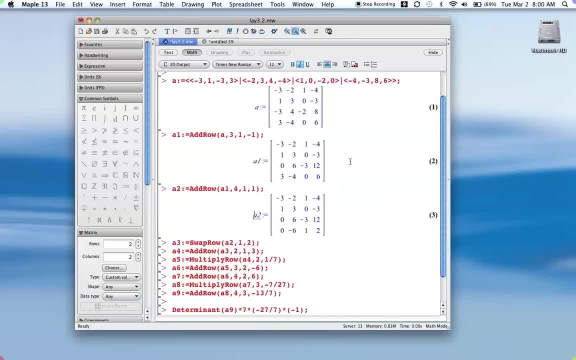 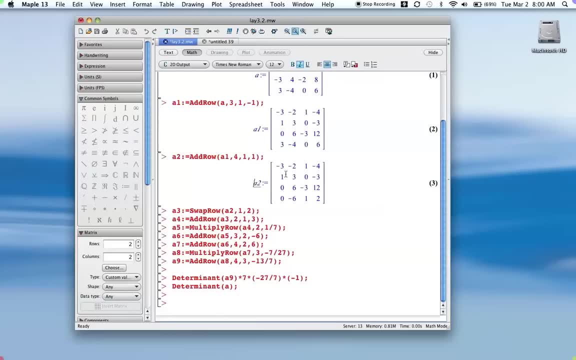 So negative: 3 plus 3 gives me a 0 here. all right, Then I'm going to swap rows. I'm going to swap the first and the second row, because then that gives me a 1 in the row 1, 1 position. all right. 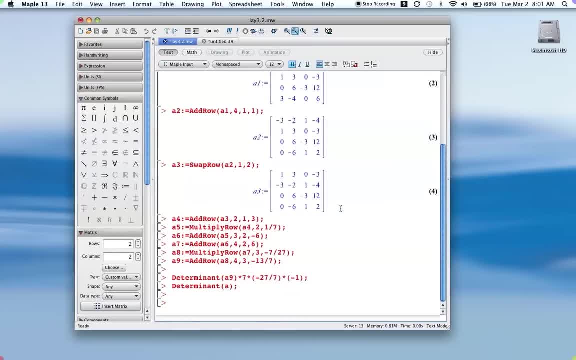 So I'm just swapping rows. Now notice, at this point we've negated the determinant. So, whatever, if I took the determinant of A3, it would be the negative of the determinant of the original matrix, okay, So keep in mind that we've done one row swap. 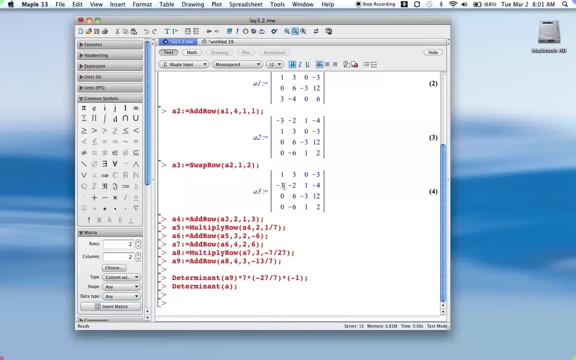 All right, now I'm going to generate a 0 here where the negative 3 is, And so to do that, I'm operating on A3, matrix A3.. I'm going to change row 2 by multiplying row 1 by 3, all right. 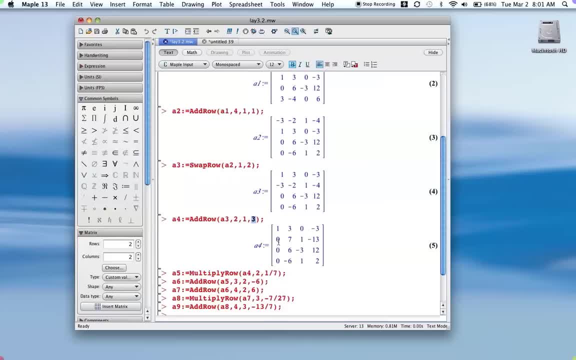 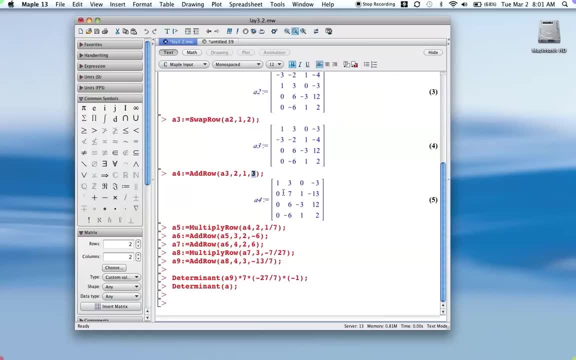 So 3 times, row 1 minus 3 gives me- or minus row 2 gives me, a 0 there in that first position. Okay, now I'm ready to move over to the next column, And so the first thing I'm going to do here, since there's no nice numbers here to work with. 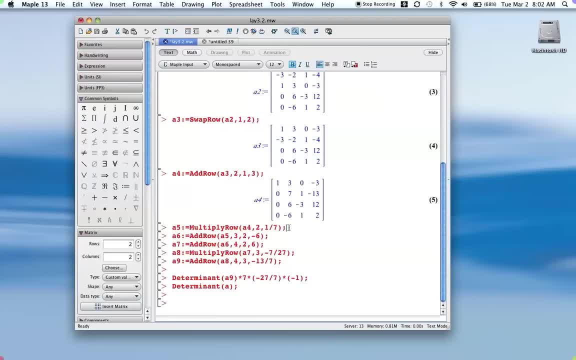 I'm going to just multiply row 2 by 1- 7th. So the command to do that is this: one multiply row. So I'm going to multiply row. working on A4, I'm going to multiply row 2 by 1- 7th. all right, 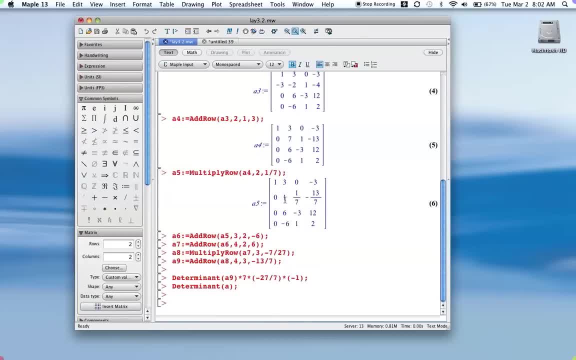 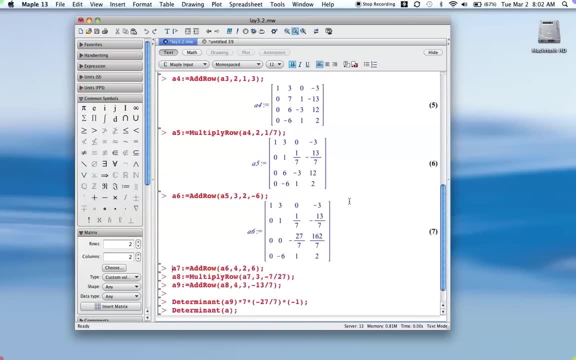 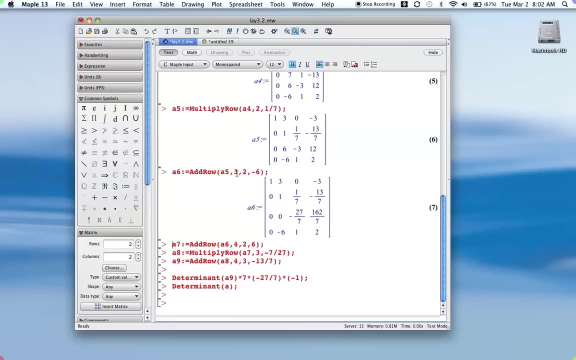 So that gives me a 1 in the 2, 2 position, And now I'm ready to 0 out underneath that. So my next operation is to work on A5.. I'm going to multiply. I'm going to change row 3 by multiplying row 2 by negative 6,. all right. 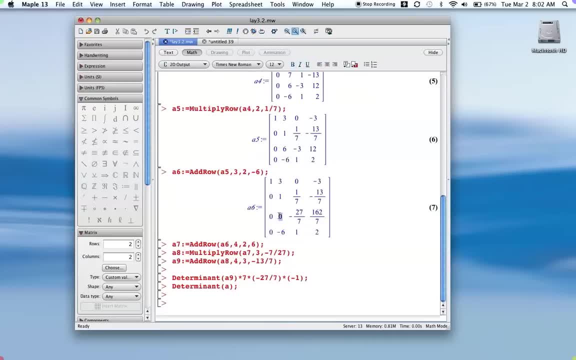 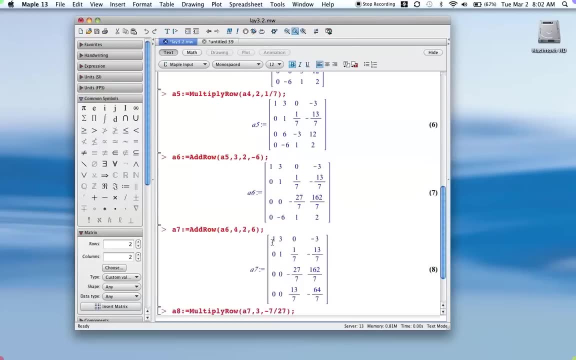 So negative 6 times 1 plus this 6 gives me the 0 here, And then I need to do a similar thing to generate a 0 in this position. So I'm working on A6, multiply, or I'm going to change row 4 by multiplying row 2 by 6.. 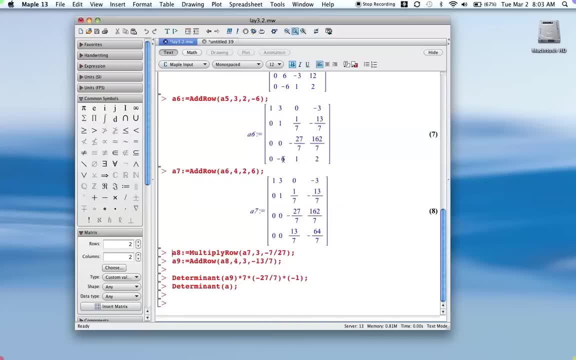 So 2 times row 2 plus row 4.. I mean 6 times row 2 plus row 4 gives me a 0 here. So up to this point, the only thing that I've changed in terms of the determinant of the original matrix. 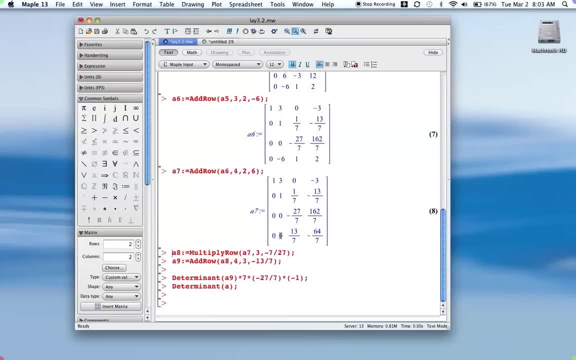 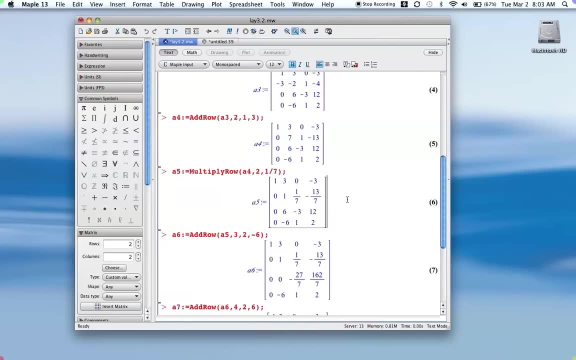 is doing the one row swap, So we've negated the determinant. Oh, we did the multiply row, So we've changed the determinant by a factor of 7 also, All right. so keep those two things in mind, And here the next thing I'm going to do is generate a 1.. 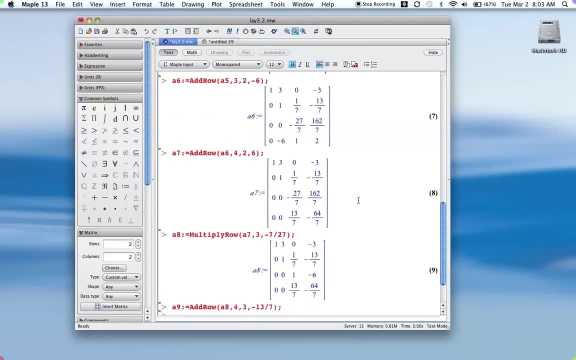 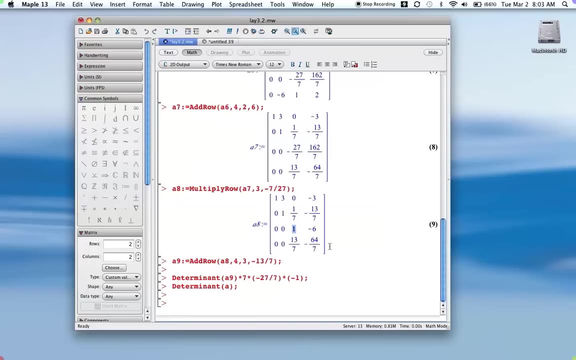 So I'm going to do another multiply row. multiply row 3 by negative 7 over 27.. And that gives me the 1 in this position. So now we've done a row swap and we've done two operations where we multiplied a row by a scalar. 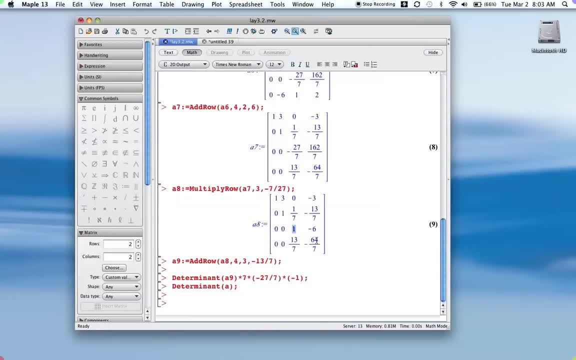 So keep that in mind. I'm going to do one more row operation, So I'm going to get a 0 in this position. So I'm going to multiply row 3 by negative 13 sevenths and add that to row 4.. 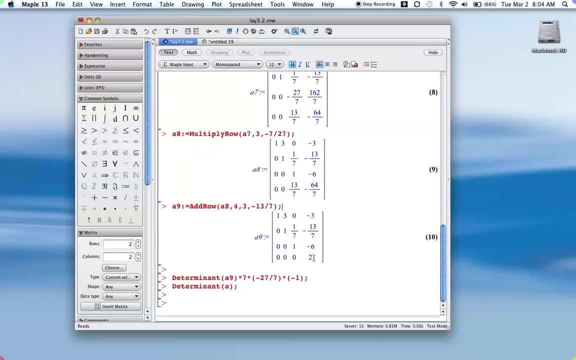 So I get a 0 there. Now my matrix is in triangular form, upper triangular form. So to take the determinant of this matrix, it's just 1 times 1 times 1 times 2.. And then to, To go back to get the matrix, the determinant of the original matrix. 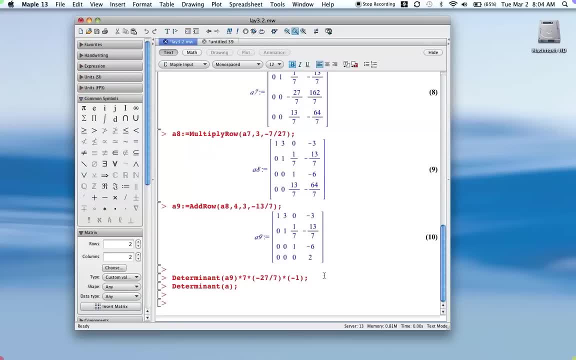 I've got to back out these row operations, So that's what I've done here. Okay, so I've taken the determinant of A9, which is, as I said, 1 times 1 times 1 times 2.. So we could just do that times 7, and I'm multiplying times 7 to 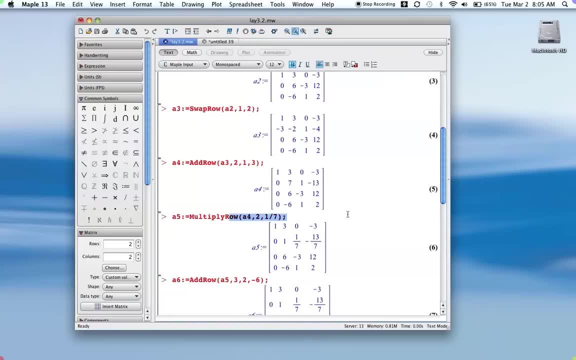 Because of this row operation, because I've multiplied by 1- seventh. so to back that out, to get the original determinant, I need to multiply by 7.. And then I multiply by negative 7 over 27.. So I'm multiplying by the reciprocal of that. 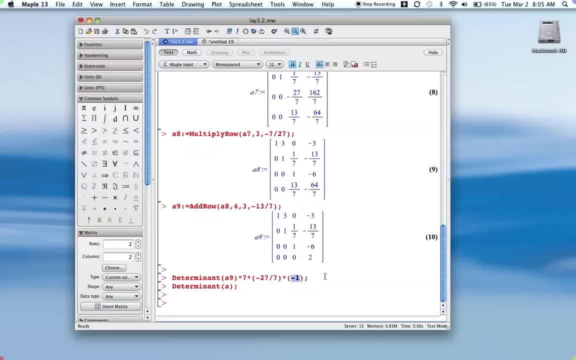 And then multiplying by negative 1, because we did the row swap. So put all that together, I get the determinant of the original matrix is 54.. And then, just to check, I'll just use MAPL to determine that original determinant and we get 54 again. 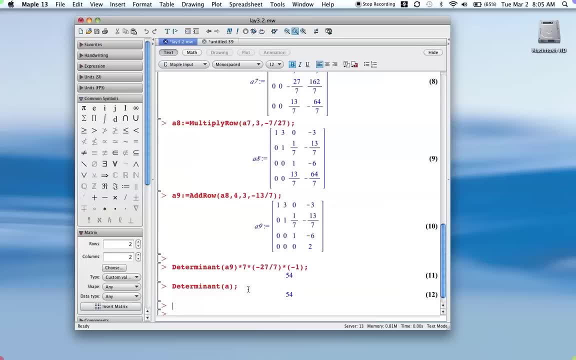 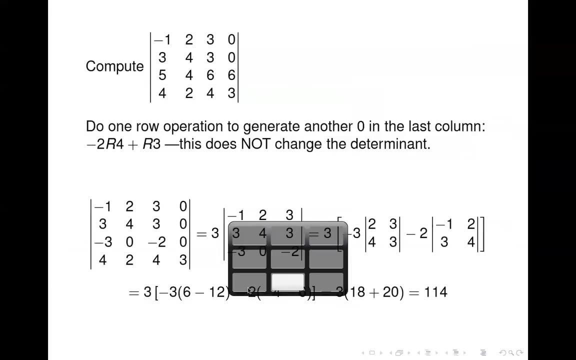 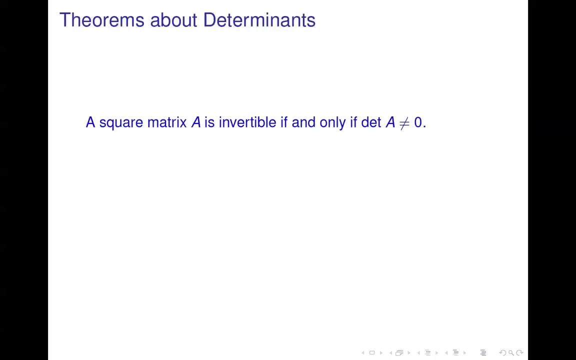 So this is a way you can back out the determinant of the original matrix by keeping track of the row operations that you did and how they affect the determinant. Okay, so back to this. We're ready to To look at a few theorems about determinants. 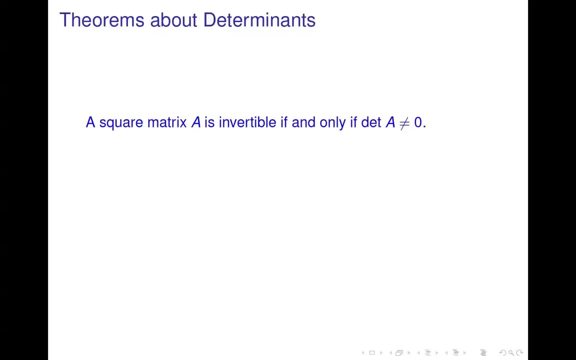 This first one here is actually another installment in the invertible matrix theorem. Okay, so it says a square matrix, A, is invertible if, and only if, the determinant of A is not equal to 0.. So we've seen this. We saw this last time. 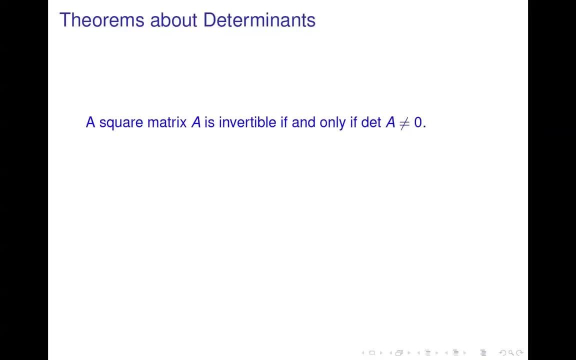 But add that on to the invertible matrix theorem. So this is an Equivalent statement. Determinant of A is not equal to 0, is equivalent to A is invertible. The determinant of A transpose is equal to the determinant of A. 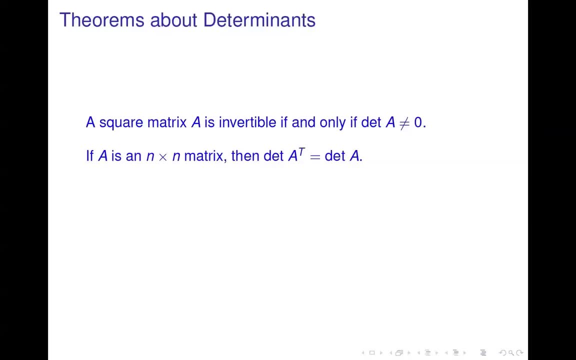 Think about that for a little bit. It actually is. It's pretty easy to see how Why that is true, Because if you think about taking the determinant of A, It's pretty easy to see how Why that is true, Because if you think about taking the determinant of A, 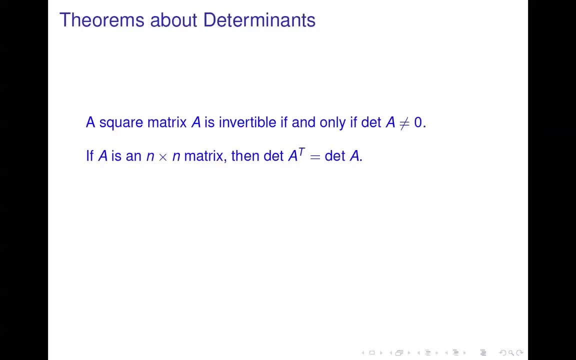 you choose some row or column to expand about- You know, for example, maybe expand about the first row- Then if you're taking the determinant of A transpose, then you can do the exact same operations by expanding about the first column, Since the first column of A transpose is equal to the first row of A. 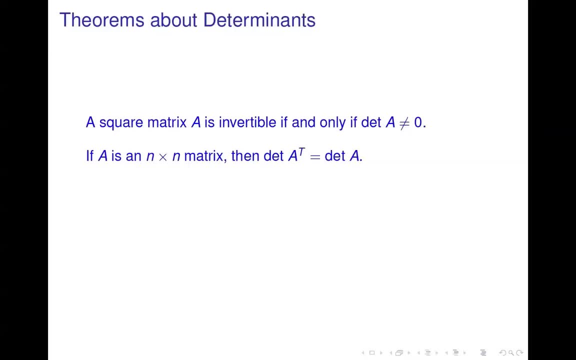 then you would be computing the determinant of A transpose exactly how you would compute the determinant of the matrix A. So you end up with getting the same result. So you end up with getting the same result. So you end up with getting the same result. 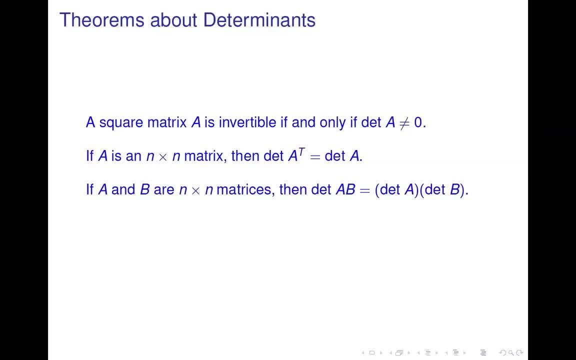 Okay, another theorem: If A and B are square matrices, then the determinant of the product- A times B- is the determinant of A times the determinant of B. The determinant of the product is the product of the determinants. Notice, though, that that doesn't apply to sums. 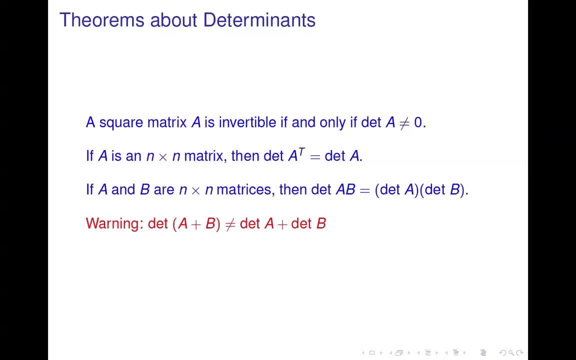 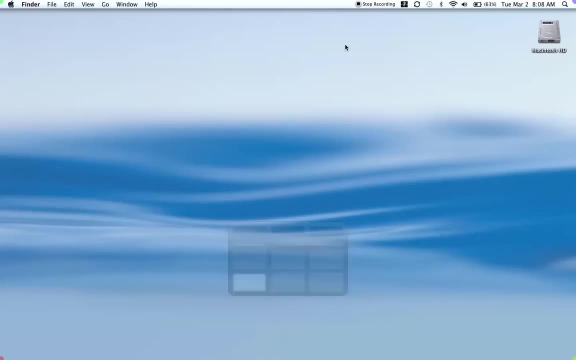 So the determinant of A plus B is, in general, not equal to the determinant of A, is, in general, not equal to the determinant of A is, in general, not equal to the determinant of B, So don't make that mistake. Okay, and that's all we have for this section. 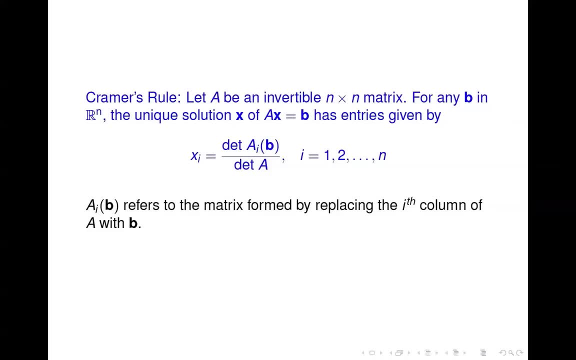 Alright, let's talk about Cramer's Rule. Cramer's Rule is actually one of the beautiful things in mathematics. I believe It's just a neat little idea. It's a way to solve a system of equations using only determinants. 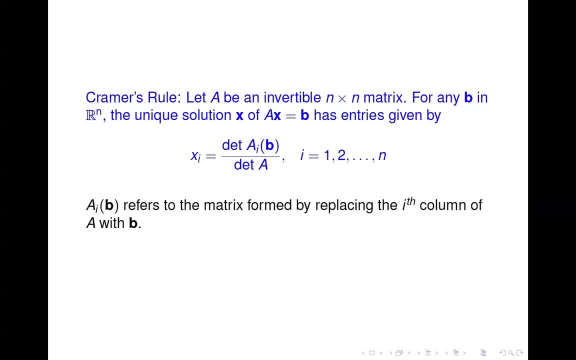 So it's just very interesting. So here's the way it works. Cramer's Rule We have: A is an n by n matrix. Then for any B in Rn, the unique solution x of Ax equals B, is given by this formula here: 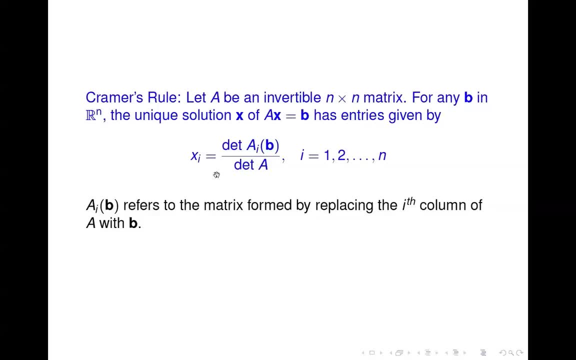 which looks rather odd. Notice that we've got a way to compute x of i for each i And it's just a ratio of determinants. In the denominator we've got just the determinant of A In the numerator, it's the determinant of A sub i of B. 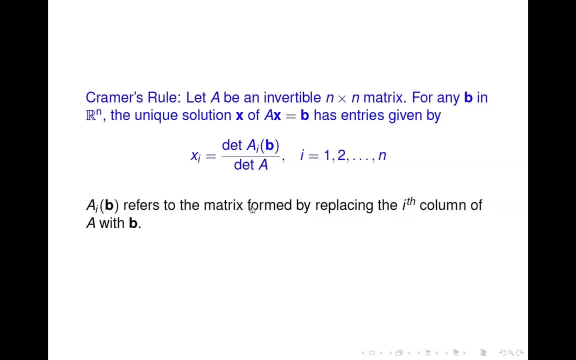 So A sub i of B refers to the matrix formed by replacing the ith column of A with B. So we replace the ith column of A with B So to get x1, we replace the first column of A with B and compute that determinant. 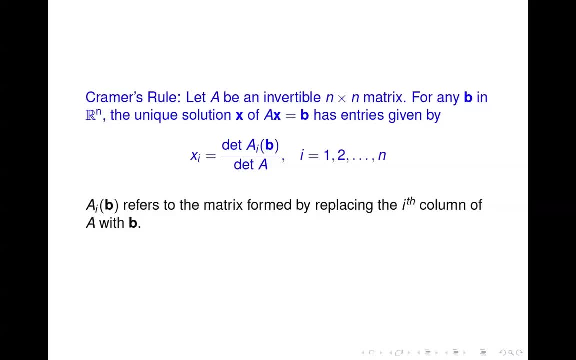 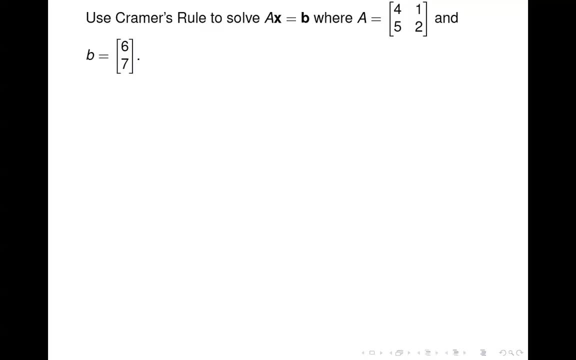 Divide by the determinant of A, That's the value for x1.. And so forth. It's a neat idea, So let's just use it to solve this system. So we need the determinant of A, That's just 8 minus 5, which is 3.. 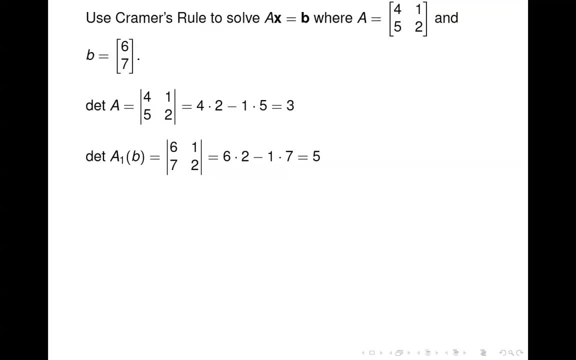 The determinant of A sub 1 of B. So notice that I've just taken B 6, 7.. Plopped it into the first column of A. Take the determinant Get 5.. Same thing: A sub 2 of B. 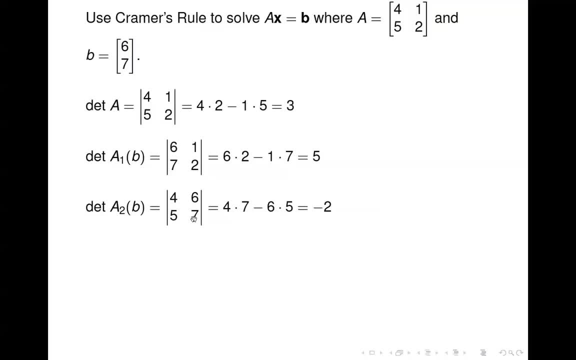 We take B And plop it in the second column of A And take that determinant, We get negative 2.. And so x1 is just the 5 divided by 3.. And x2 is the 5. And negative 2 divided by 3.. 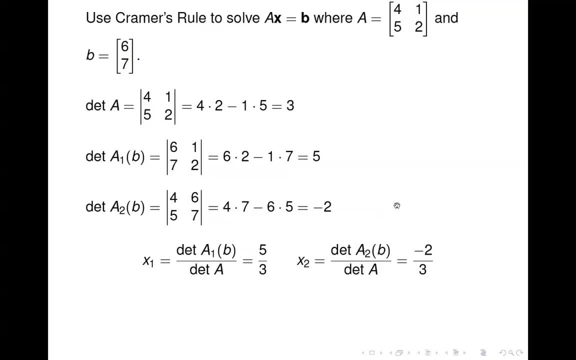 And those are the values of x1 and x2.. Just to check, take 5 thirds times the first column of A minus 2 thirds times the second column of A, And we indeed get 6, 7.. Yippee. 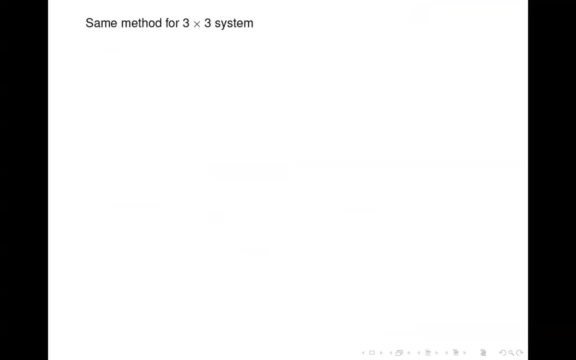 It's nice when things work like they're supposed to. I'll use the same method for a 3 by 3 system, Although this time we're going to use a determinant for each of three variables plus the determinant of A. So here's a matrix A in the right-hand side, B. 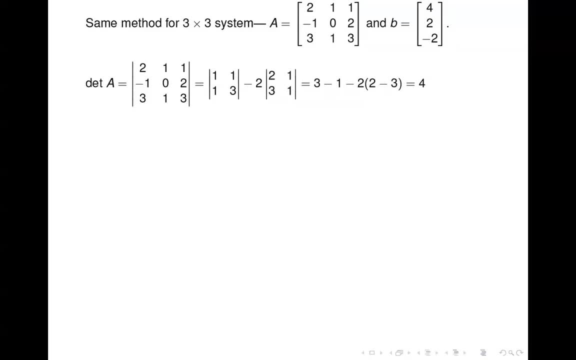 Compute the determinant of A first, And then we compute the determinant of A sub 1 of B. So again, take B, Take the vector B, Stick it in the first column of A, Leave the rest of A alone, And compute that determinant. 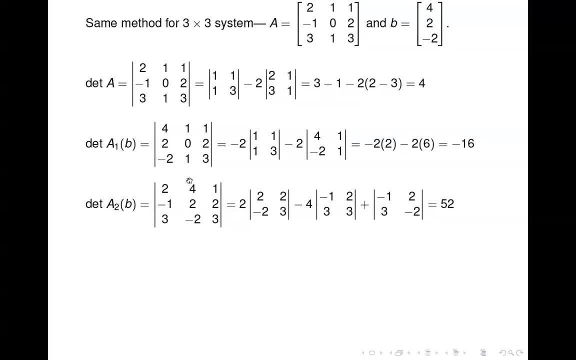 Same thing: A sub 2 of B. We take B, Stick it in the second column of A And leave the rest of A alone. Compute that determinant A sub 3 of B. We take the B Replace the third column of A. 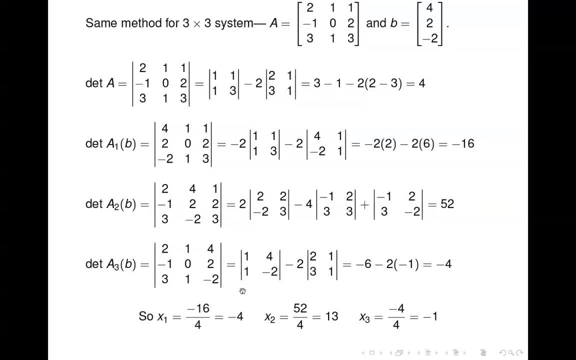 Compute that determinant And then put it all together: x1 is going to be negative 16 over 4.. x2 is going to be 52 over 4.. And x3 is going to be negative 4 over 4.. And so there's your solution to this system. 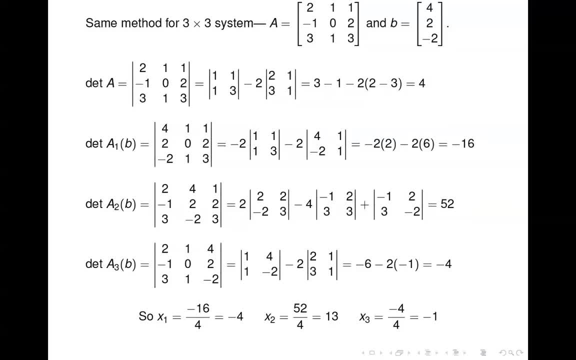 So just a really neat idea And a neat way to solve systems of equations, But clearly we run into the same problem for this 3 by 3. It really wasn't that bad, But if it was a 4 by 4 system, 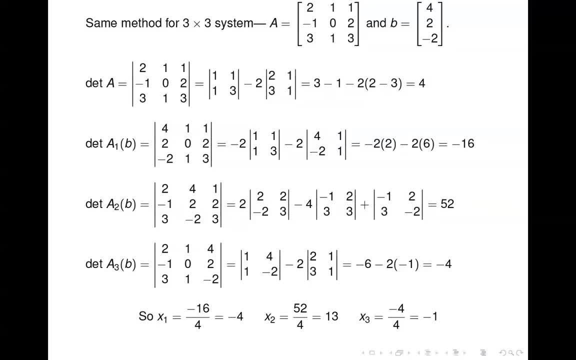 then you're computing five, 4 by 4 determinants, Because you have to compute one for each variable, one for each column. So you'd have A1, A2, A3, and A4 of B, Plus you need to compute the original determinant. 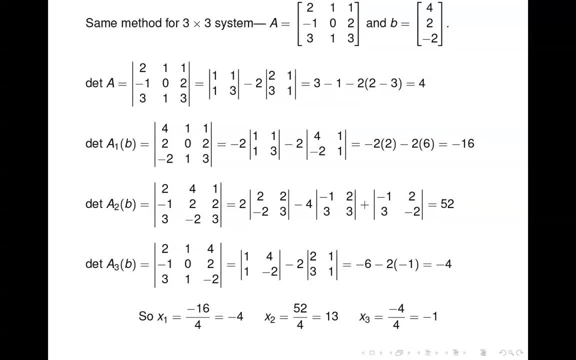 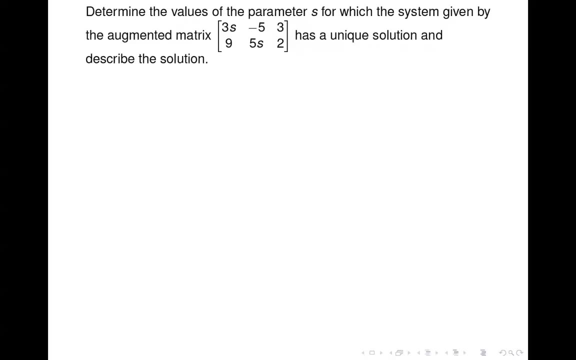 So you have five 4 by 4 determinants And that would be a lot of work. So this is not practical in a general sense, But for theoretical and for small matrices like this it's kind of a neat idea. We can also apply it to a question like this. 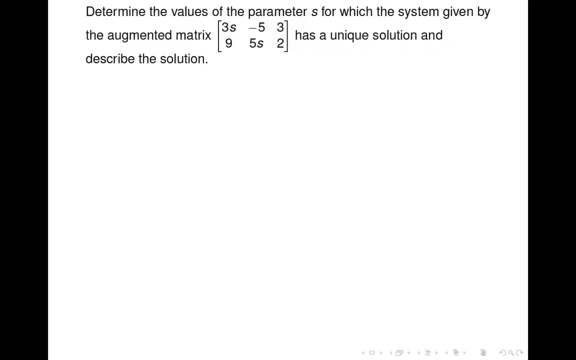 Determine the values of the parameter S, for which the system given by this augmented matrix has a unique solution, And then describe the solution So we know it has a unique solution when the determinant is not 0. Because if the determinant is not 0,, 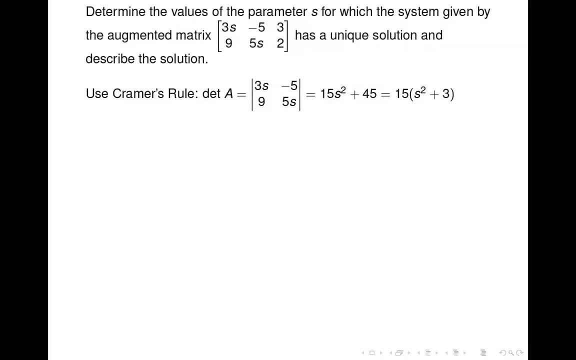 A is invertible and there's a unique solution. So if we take the determinant of the coefficient part of that matrix, we end up with 15 times S squared plus 3.. And note that 15 times S squared plus 3 is not equal to 0 for all values of S. 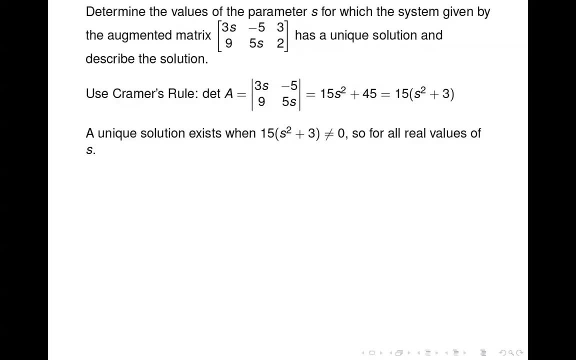 And you can never end up with that equal to 0 as long as S is a real number, Because S squared plus 3 is always going to be positive, And so this system's going to have a unique solution, no matter what the value of S is. 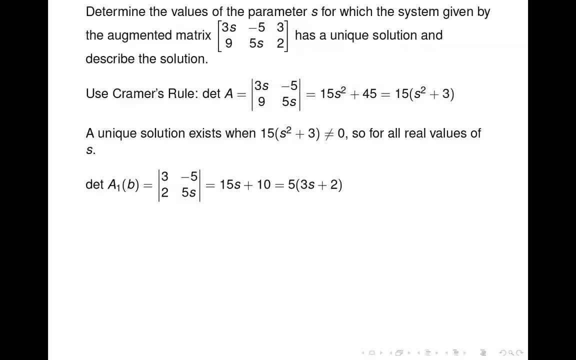 So we compute. To be able to describe the solution, we can use Cramer's rule, And so I've just computed A1 of B. That takes B, the 3,, 2, sticks it in the first column of A. 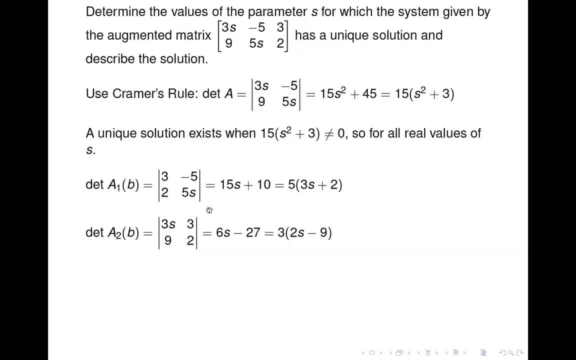 And we compute that determinant. Then, same thing, A sub 2 of B, We stick the right-hand side on the second column, Compute that determinant And then kind of massage things a little bit And we have expressions for the value of X1 and X2. 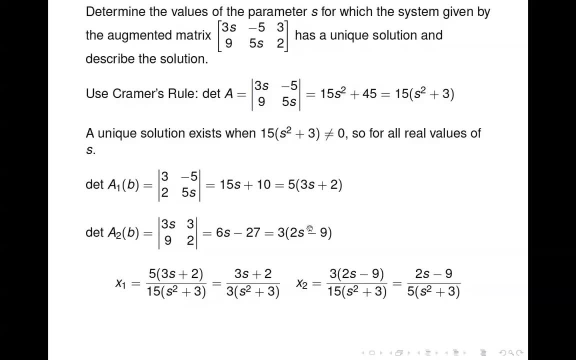 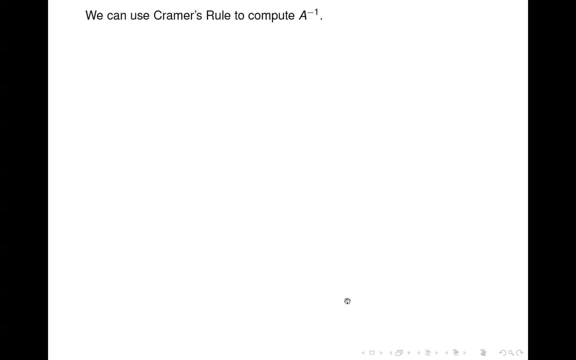 for any value of S. So it's just the 5 times 3S plus 2 divided by the determinant of A here, And the 3 times 2S minus 9 divided by the determinant of A for X2.. We can also use Cramer's rule to compute A inverse. 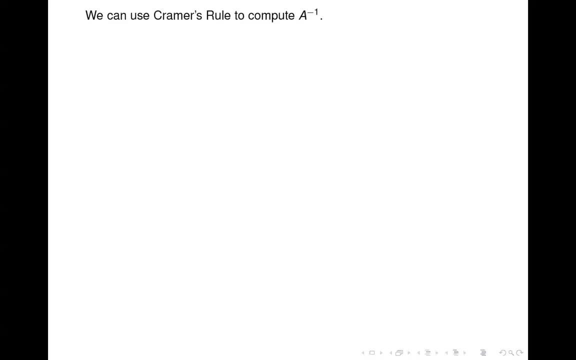 Because, as we saw in chapter 2, to compute A inverse we simply need to solve some systems of equations. So if we consider this matrix A, we want to find B, such that A times B equals the identity matrix. So B here would be the inverse of A. 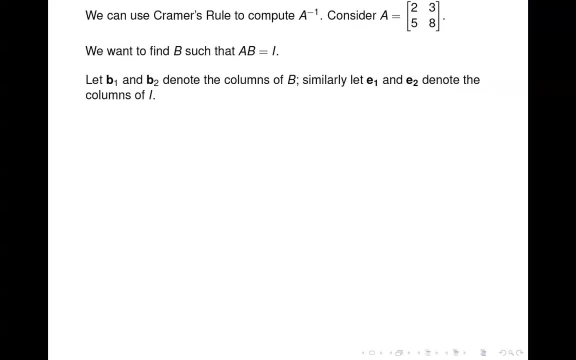 So let's let B1, B1 and B2 denote the columns of B And let E1 and E2 denote the columns of the identity matrix. And we've used that notation before, So we need to solve A times: B1 equals E1. 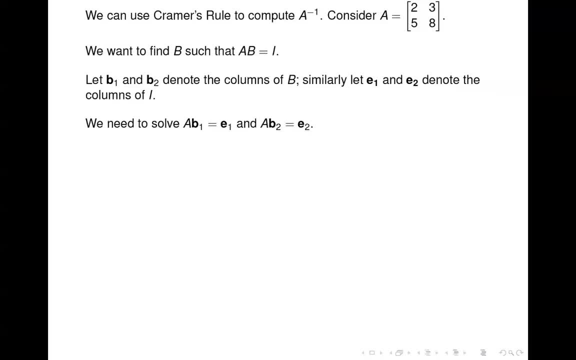 and A times B2 equals E2 here in this 2 by 2 case. Alright, so if we take the determinant of A, go back up and look at A here: 2 times 8 is 16.. Minus 3 times 5.. 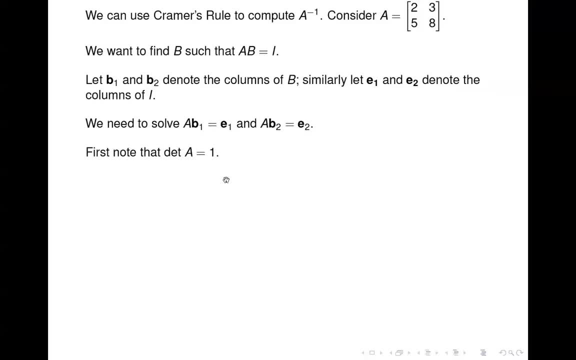 So 16 minus 15.. Determinant of A is just 1.. Okay, now to get B1, we're solving this system here. A times B1 equals E1. So to get the first entry in B1, that's the determinant of A1 of E1. 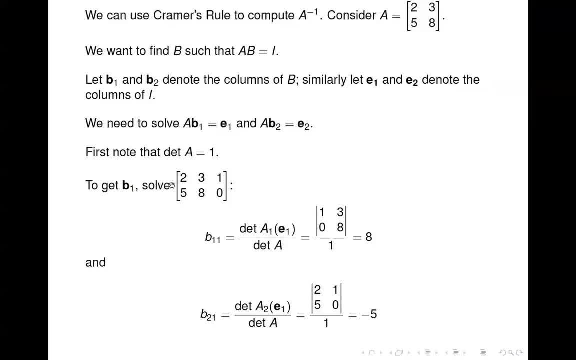 Alright, We're solving. look at this augmented matrix. So to get the first entry in the solution, we replace the first column of A by the right hand side, which is E1.. Compute that determinant, You get 8.. 8 over 1 is just 8.. 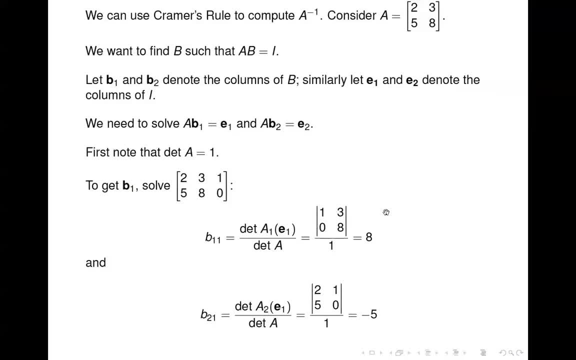 So the 1, 1 entry in the inverse is 8.. Alright, Now to get the second entry in the solution to this system. here we substitute E1 into the second column of A. Alright, So here we go with that. 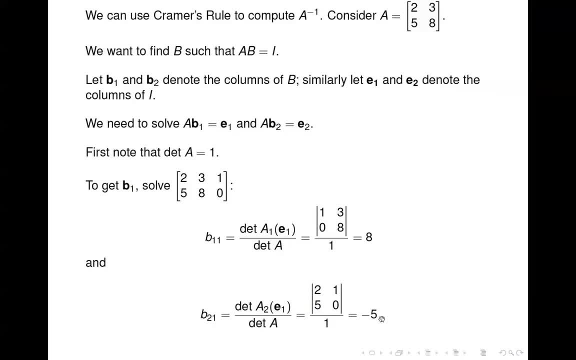 And compute that determinant Negative 5 divided by 1, we get negative 5.. So we've got the first column of the inverse right, Because we were solving this system. A times B1 equals E1. And so that's the first. 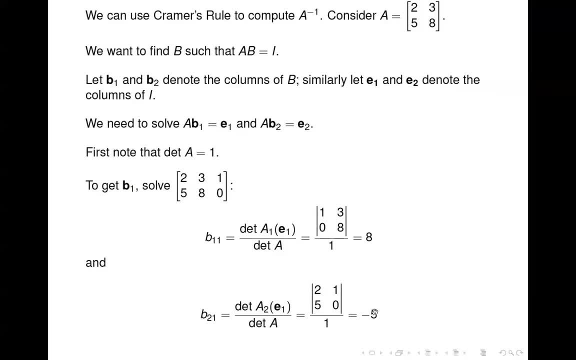 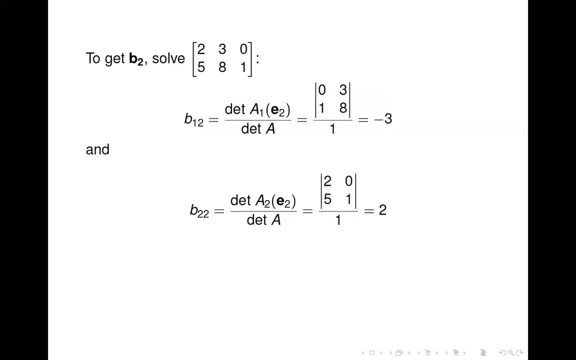 so we get the first column of the inverse B1, would be 8, negative 5.. To get B2, we solve a similar system just now. the right hand side is 0, 1 instead of 1, 0.. 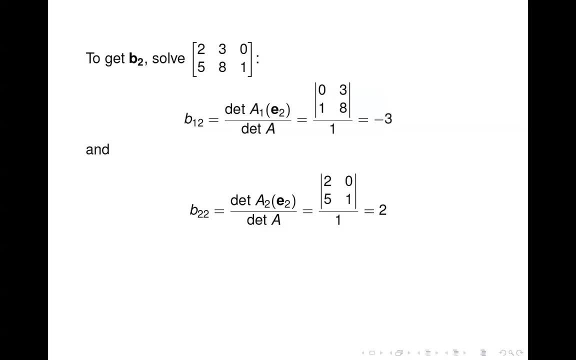 And so to get the first entry in the solution to this system, we substitute 0, 1 in the first column of A Alright, So we see that here. Compute the determinant, We get negative 3 divided by 1, negative 3.. 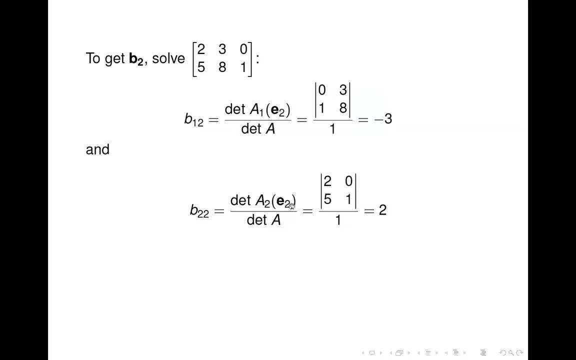 And then the second entry means substitute the right hand side and the second column of A, Compute that determinant. You get 2 divided by the determinant of A And we have 2.. So we have A inverse which is B, given by this matrix that we just computed. 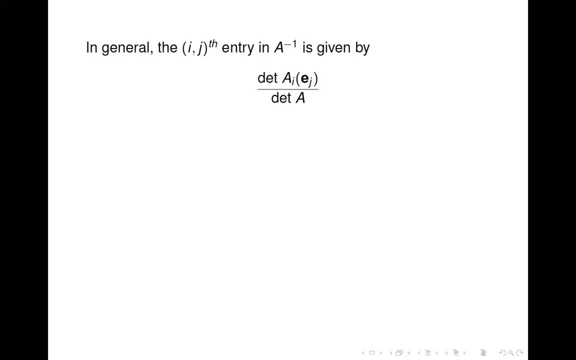 So in general the ijth entry in the inverse is given by the determinant of A sub i of Ej divided by the determinant of A. So if you go back for instance here to get the 1, 2 entry in the inverse, 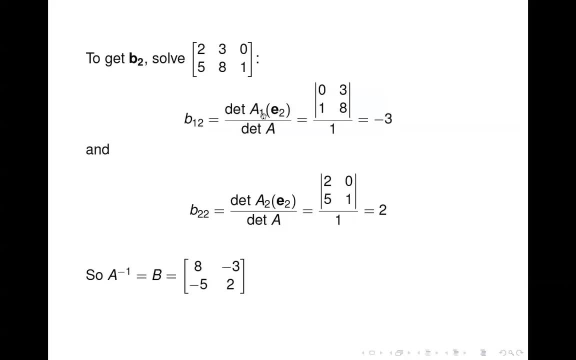 we computed the determinant of A sub 1 of E2 divided by the determinant of A To get the 2, 2 entry. it was A2 of E2 divided by the determinant of A, So in general the ijth entry in the inverse. 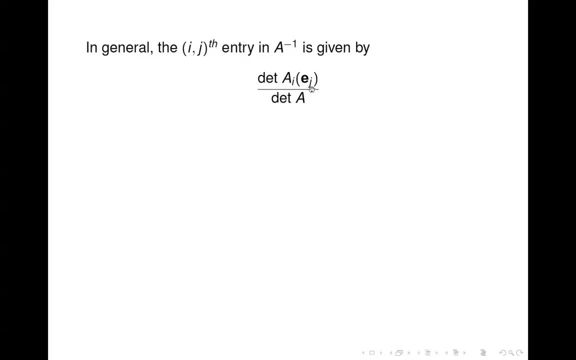 is the determinant of A sub i of Ej, divided by the determinant of A. We actually create a matrix, which we call the adjugate or the adjoint of a matrix, and stick in these values, these determinants of A sub i, E, sub j. 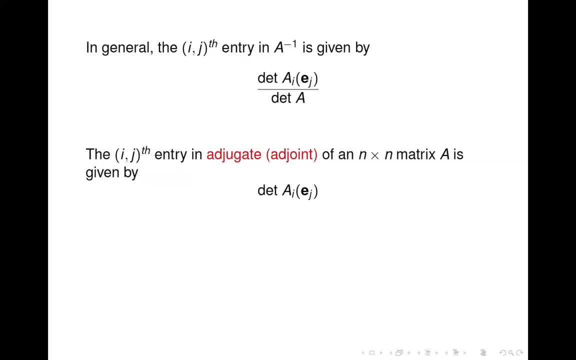 The book uses the term adjugate primarily. I typically use adjoint, so those are synonymous terms, But it's composed of all these determinants And so basically, it's just these things, but with the determinant of A term factored out. 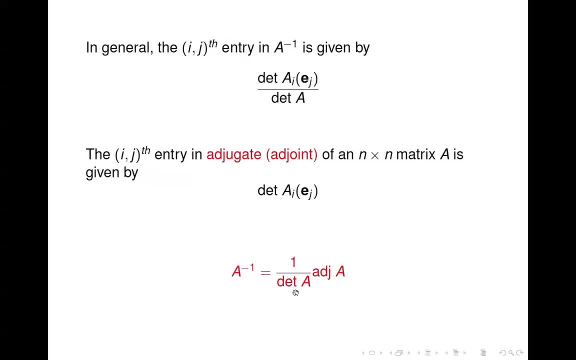 So in general, A inverse is equal to 1 over the determinant of A times the adjoint of A. Alright, So let's use that to find the inverse of this matrix here. Okay, so first we'll find the adjoint or the adjugate of A. 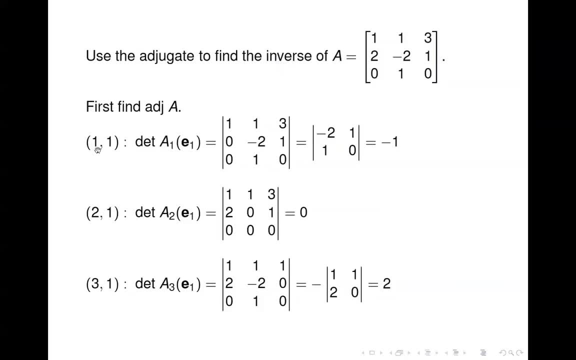 And remember to get the ijth entry in the adjoint it's the determinant of A sub i, E sub j. So for the 1, 1 entry it's the determinant of A1, E1.. For the 2, 1 entry: 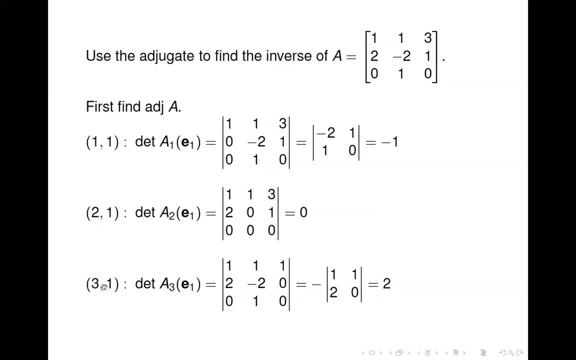 determinant A2, E1.. 3, 1 entry determinant of A3, E1.. Alright, so I've computed all those A sub 1 of E1, remember, E1 is the first column. It's the first column of the identity matrix. 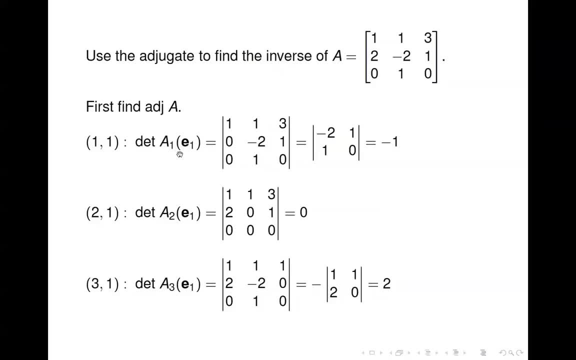 A1 says: substitute that into the first column of A. So there you have E1, 1, 0, 0. Substitute in the first column of A And take that determinant. A sub 2 of E1 says: put E1 into the second column of A. 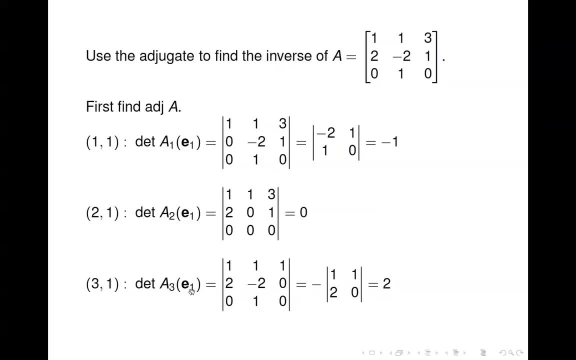 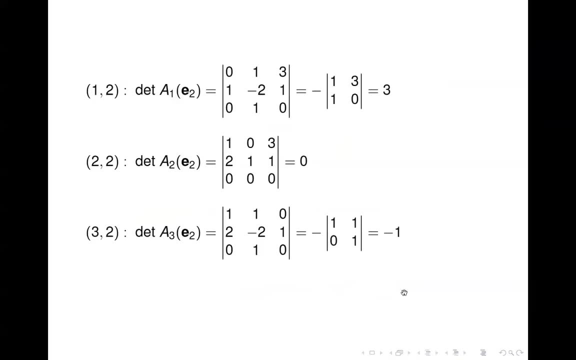 So there we have it. Determinant: there is 0. A sub 3 of E1 says: put E1 in the third column of A. So there we go, Take that determinant And do the same thing for the other 6 entries in the adjoint. 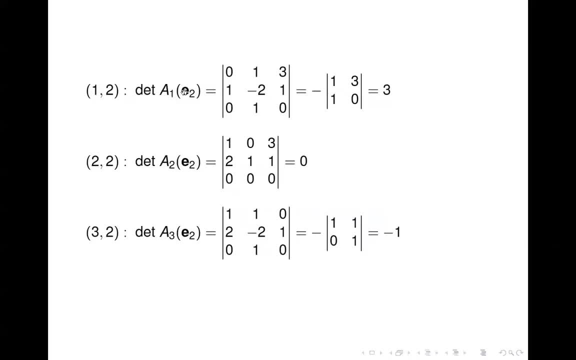 1, 2, position Determinant of A1 of E2.. So take E2, which is 0, 1, 0. And substitute that in the first column of A. So there, So you can see, here we have 0, 1, 0 in the first column. 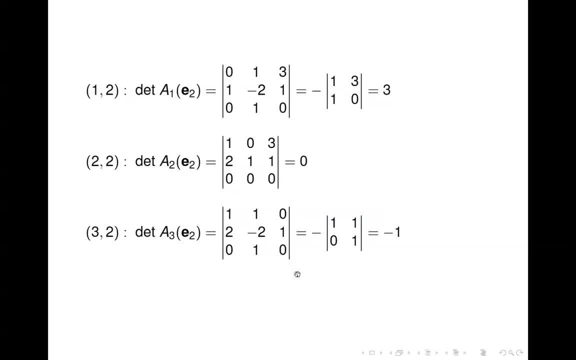 Here it's in the second column, Here it's in the third column, And we compute each one of those determinants. Then do it one more time. for the third column, Let's get the 1, 3, 2, 3, and 3, 3 elements. 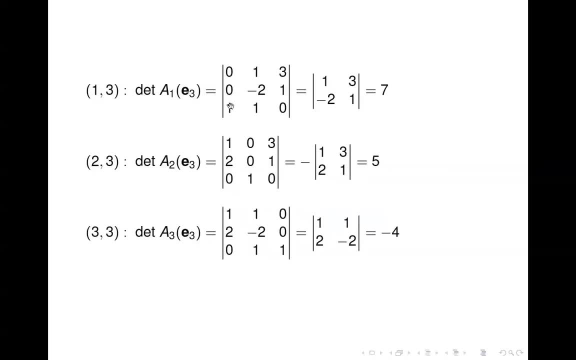 So E3 is 0, 0, 1.. So we stick it in the first column of A, Then the second column of A, Third column of A, And compute all those determinants, Then we put it all together. This is what we get. 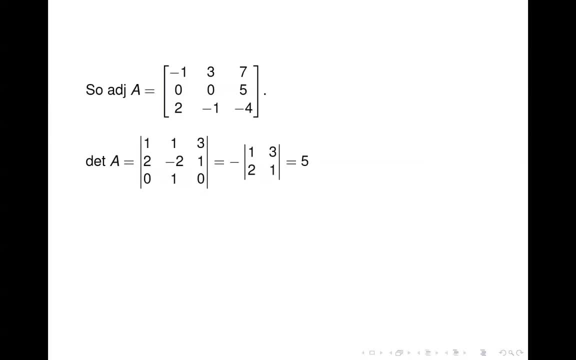 And we need the determinant of A Which we can compute, And that's 5.. So the inverse of A is just 1 over the derivative, It's just 1 over the determinant of A. So 1 fifth times the adjoint of A. 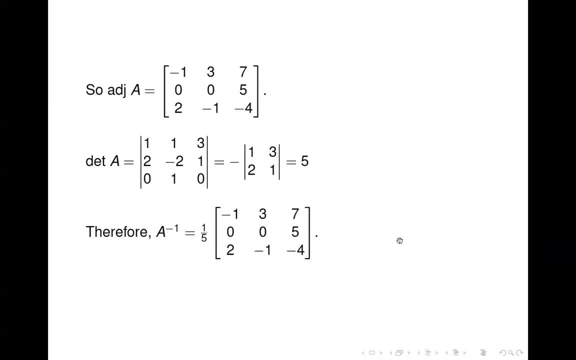 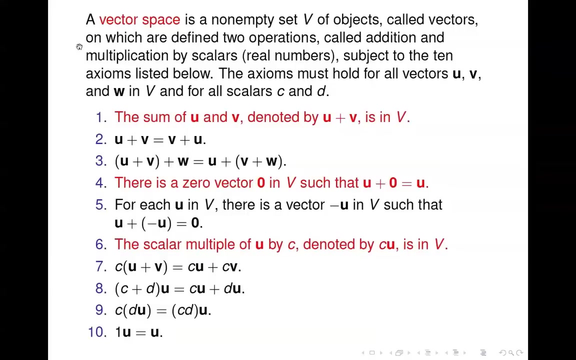 Which is this matrix. And there's your inverse, Computed totally by doing elementary, Not elementary row operation, Totally using determinants. OK, Today we're going to start section 4.1 on vector spaces. So we'll start with the definition. 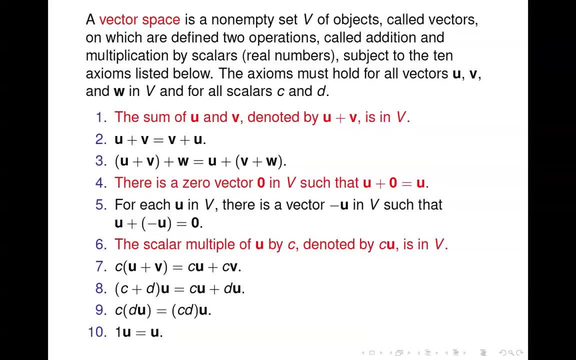 Of a vector space. You'll probably want to have your book out with you, Because we're going to refer back to this definition quite a bit. So in your textbook It's on page 217.. There's a lot to this definition. 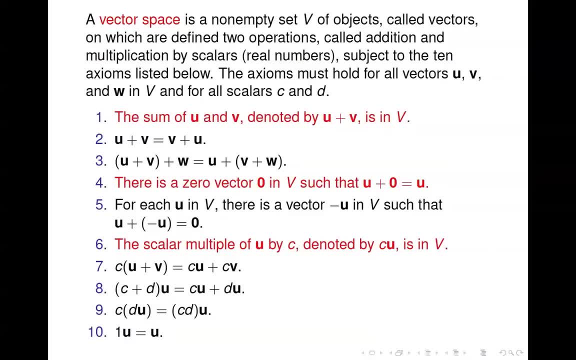 So we'll spend a little time just talking about it Before we move on from there. A vector space is said to be a non-empty set V of objects Called vectors. Let's stop there, because that's a little bit odd. It's a set of objects. 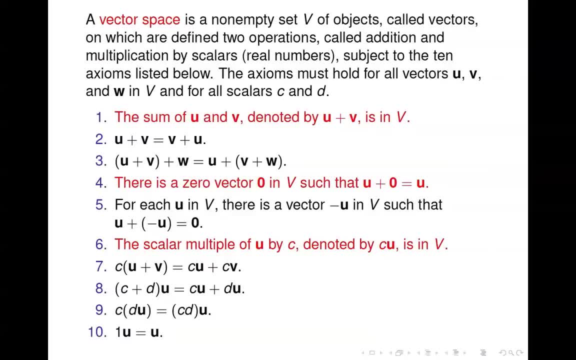 Called vectors. I want to make the point here That when The author uses the term vector in this context, He's not necessarily talking about a vector Of the type we're familiar with, Like in R2 or R3 or so forth. 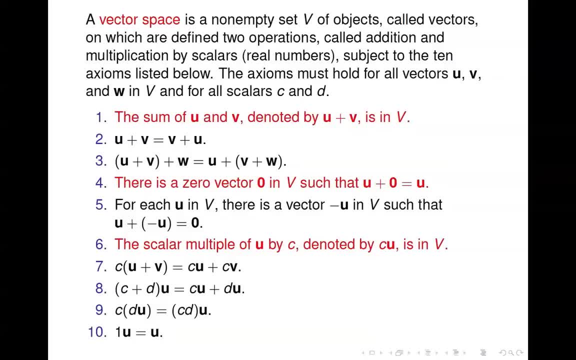 Yeah, He's using it in a more generic sense, And I actually like to use the term object Just to keep from Confusing you between Exactly what he's referring to by using the word vector And as we go along today. 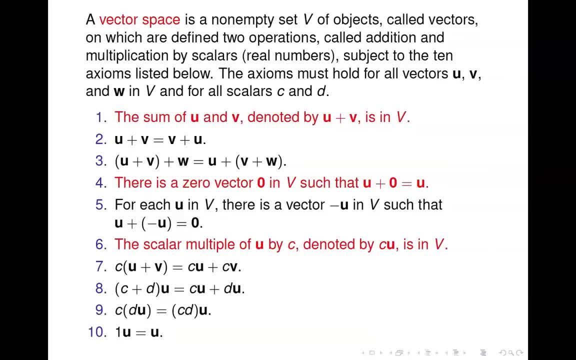 You'll kind of see what I'm talking about here. Okay, So, Starting over A vector, space is a non-empty set V of objects On which are defined Two operations Called Addition And multiplication by scalars, Which are real numbers. 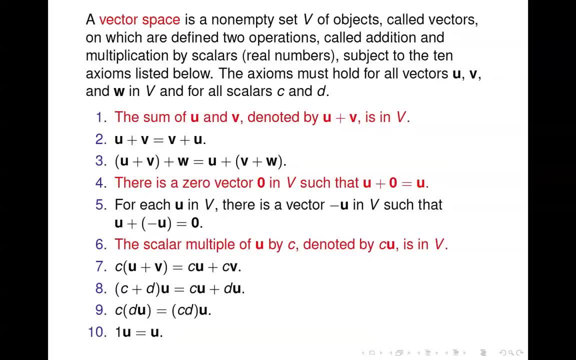 Now again, This seems sort of odd, I would think to you, Because he's saying There's two operations, And instead of saying two operations- Addition And multiplication by scalars- He's saying there's two operations Called Addition. 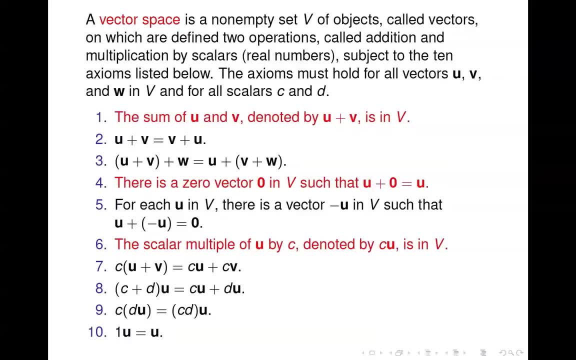 And multiplication by scalars, Which is kind of an odd way to phrase it, And the reason why he says it like that Is because, Since these objects Are not necessarily vectors In the traditional Sense that we're used to, Then addition and multiplication by scalars. 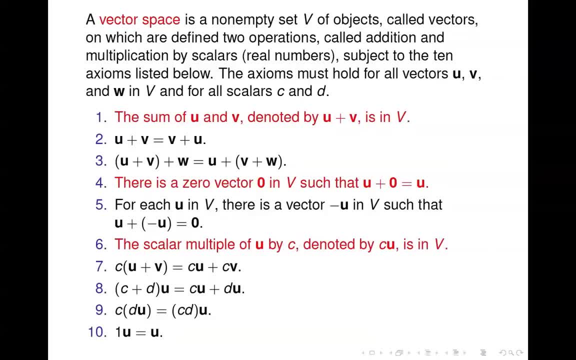 Are not necessarily defined As we're accustomed to. Okay. They can in fact be defined In any way that you would like, As long as these properties here are satisfied. So We're, We're, We're in an abstract sense here. 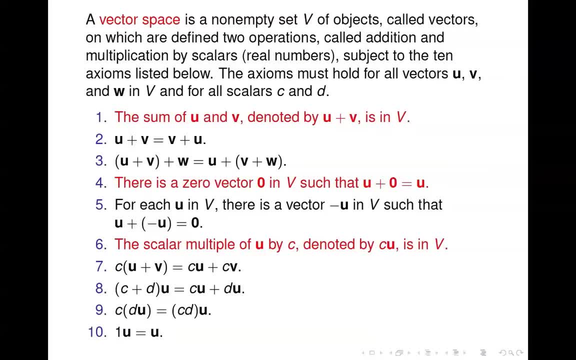 Okay, We're talking about objects And operations, And So don't Assume That we're talking about Vectors in the traditional sense, Nor Addition And scalar multiplication In the traditional sense. Okay, So We have these. 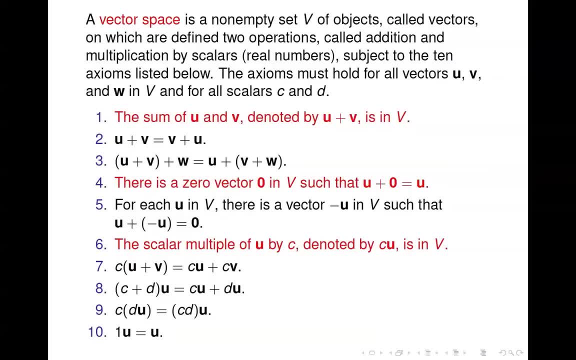 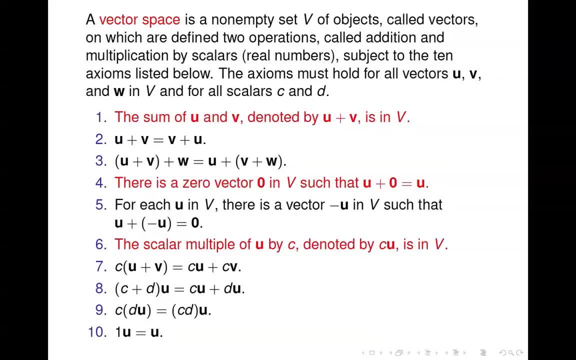 With the axioms, And they are subject to the 10 axioms Given Here, And These axioms must hold for all vectors v, U, V And W In the set V And For all scalars. 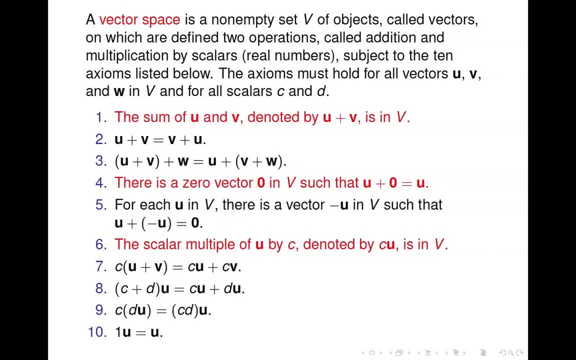 C And D Okay. So I've kind of highlighted Some, Because some are A little bit more Interesting from the set, and you add them together, then you get another vector that is still in the set. 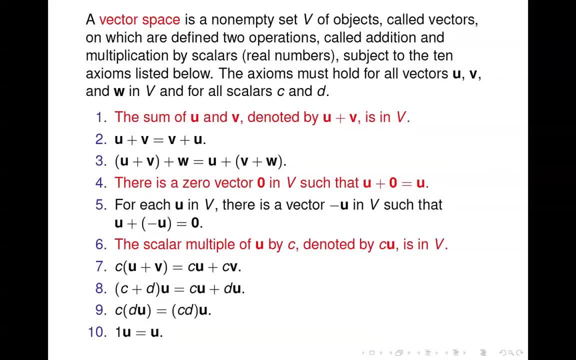 As we'll see in a minute, this property is called closure or we say that the set is closed under addition, if this property holds Okay, two and three are some standard properties. Number two: we have a commutative property, three associative. And number four says that in the set V there is a 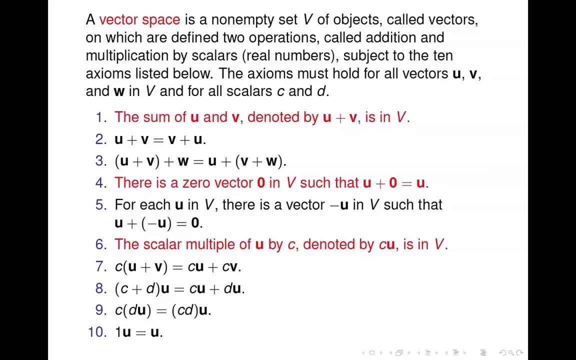 zero vector, such that when you add it to any vector in the set, you just get that vector back. Okay, so U plus zero is equal to U. Okay so notice. number one is referring to an element that has a set V. 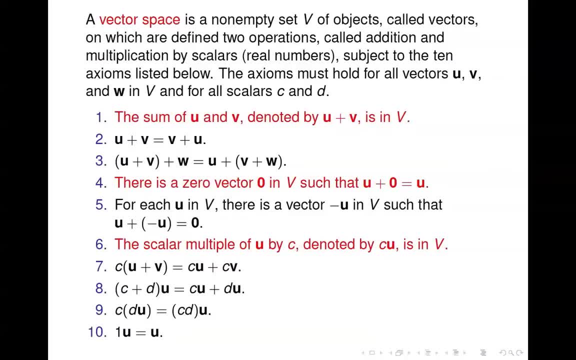 Okay. so notice number one is referring to an element that has a set V. It has to be in the set. Okay, if U and V are in the set, their sum has to be in the set. Number four also saying that there has to be this zero vector in the set, 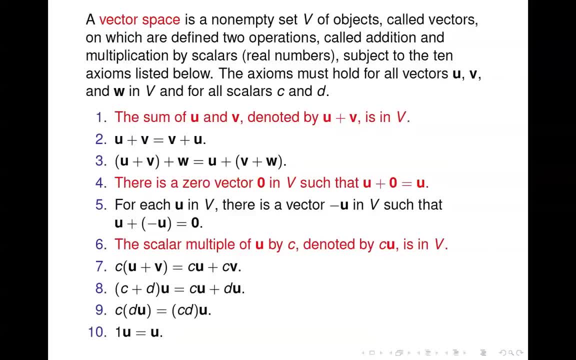 Okay, so we'll see that number six kind of follows along with that too. Number five, the first- says for each vector in the set you have another vector, such that when you add it to the first you end up with a zero vector. 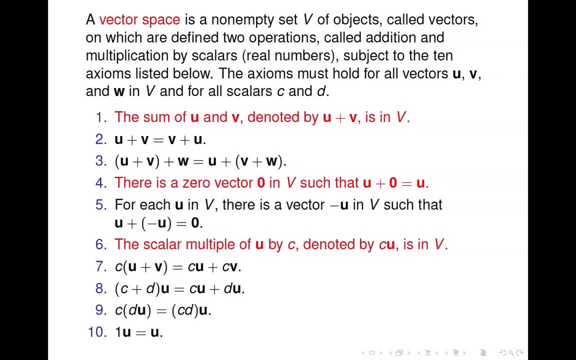 So it's essentially saying that every element has an additive inverse in the set. the number six says the scalar multiple of any vector by a constant C is denoted by C times U, and that is in the set. okay, so this is that when you take the scalar multiple of any vector in the set or any object in the 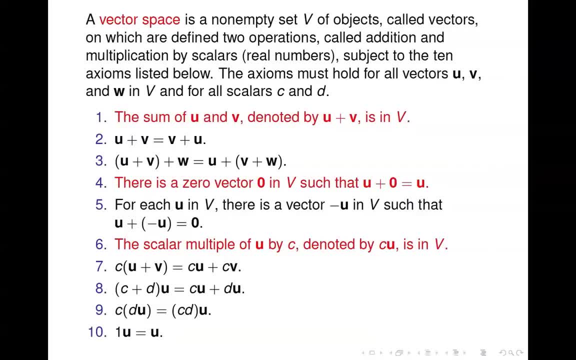 set. the result is also in the set. so you can see that number one, number four, number six, all are specifically referring to whether or not particular elements are in the set and that will be important as we go along. number seven through ten are again standard sorts of properties, have distributive properties. 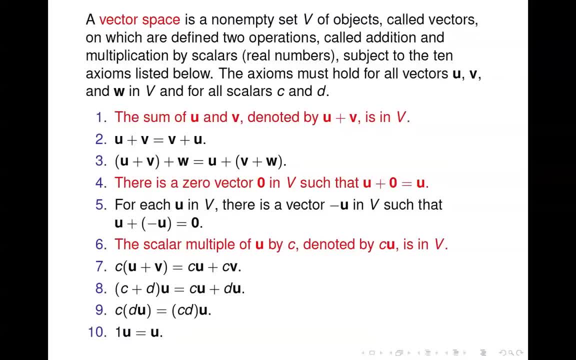 and number ten. we have a multiplicative inverse property. one times any element, the set is equal to that element. and you might be looking especially at number ten and going: well, when would that be? when would that ever not be the case? and the answer is going back to what I 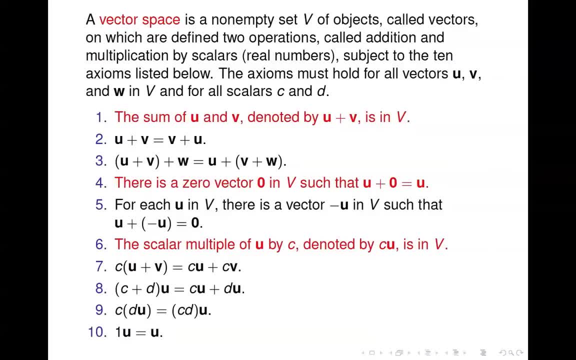 said originally is that these, the set V, can contain items other than just vectors like from R2 or R3, and these operations- addition and scalar multiplication- can be defined in non-standard ways, and so based on that, then sometimes it could be the case that number ten 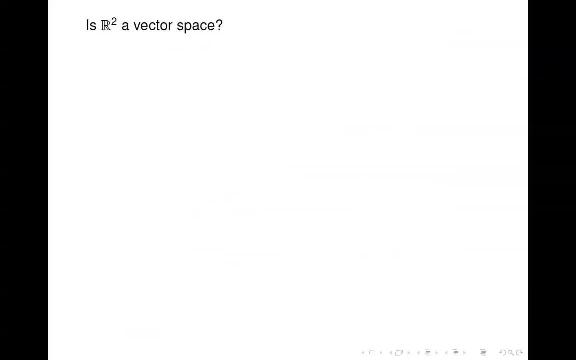 would not be true. ok, so let's start with R2. that's a simple set to think about, and let's talk about whether R2 is a vector space. the answer is yes, because all the properties except one and six were in fact explicitly given in section 1.3. so 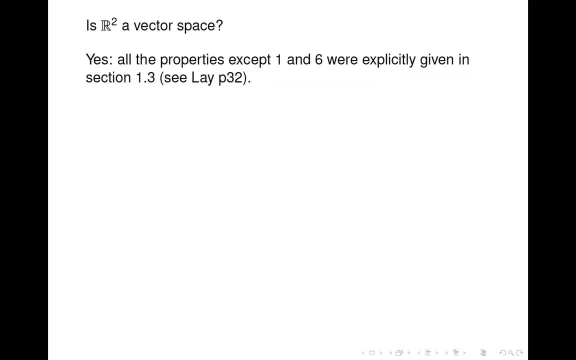 if you want to go back to page 32 and check that out, all the properties except one and six are explicitly listed there. so let's think about one and six. number one: we want to know if you take two vectors from R2 and add them together do? 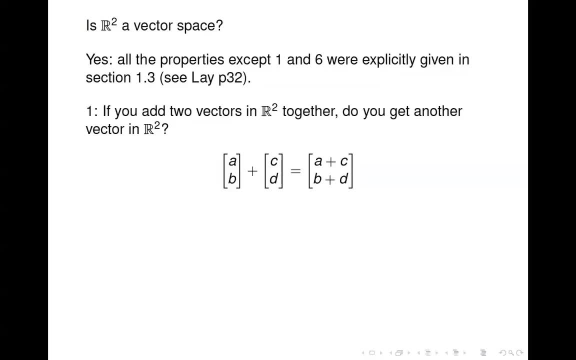 you get another vector in R2. well, here's two vectors in R2: A, B and C- D. when we add them together, we get A plus C, B plus D. that's another vector in R2. so the answer is yes. there number six: if you multiply a vector in r2 by a scalar do. 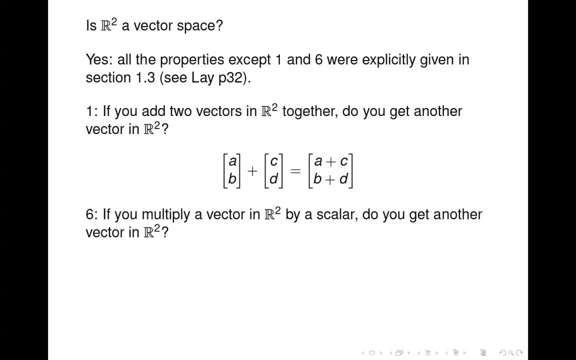 you get another vector in r2, as it closed under scalar multiplication, and here we see: multiply, a vector times the scalar. we get another vector in r2, both of whose components are real numbers and therefore r2 is a vector space and, in fact, the set of real numbers, a set of all vectors with two components, which is: 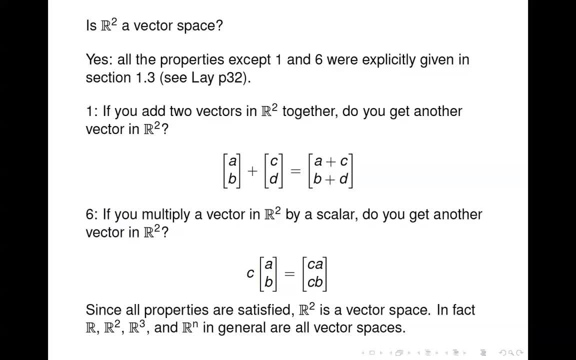 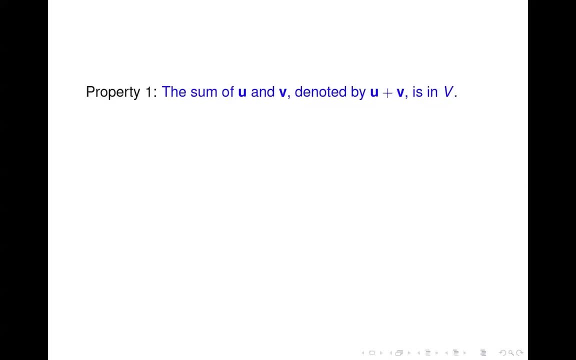 r2, r3 and RN in general are all vector spaces going back to these, property 1 and property six. just to take a second look at those property. one said that if you take any two from the set長, compute their sum then it is also in the set and if that is true we say that the 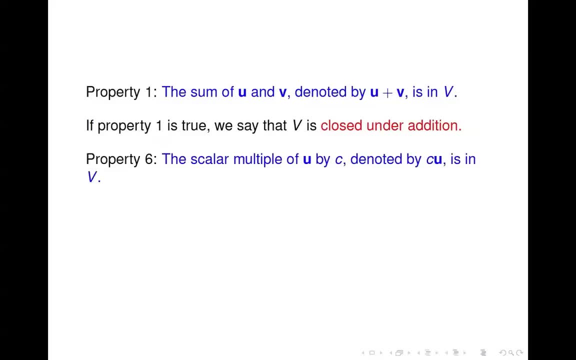 set is closed under addition. property 6 says you take a scalar multiple of a vector in the set, then the result is also in the set. then if this is true, we say that the set is closed under scalar multiplication. so keep those terms in mind. let's move on and consider another set. here's another set. this is a subset. 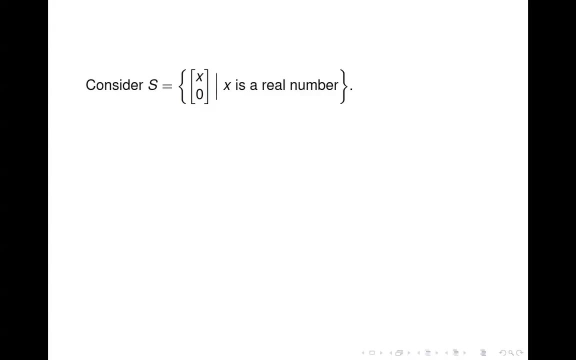 of R2. so I'm saying we have a set S here which consists of vectors of the form X- 0, where X is a real number. okay, so basically everything in R2 where the second component is 0. if you think about this graphically, it's just saying that. 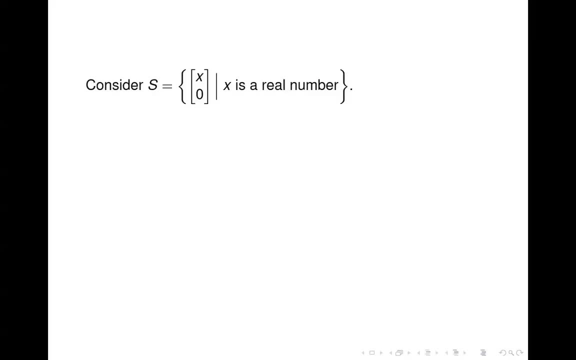 the white I completely just is 0. so therefore, graphically speaking, s would just be the x-axis. so I want to know: is s with the operations of addition and scalar multiplication as traditionally defined? okay, what you're used to is as a vector space. well again, 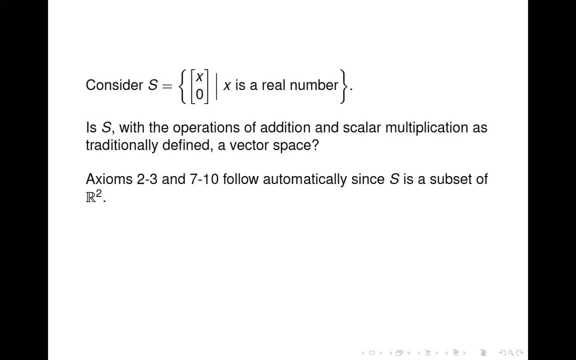 axioms 2 & 3 & 7 through 10 follow automatically. since s is a subset of r2, this 2, 3 & 7, 3, 10 are true of everything in r2 and I'm assuming here to get your book open so you know which of these are referring to. the other axioms depend on: 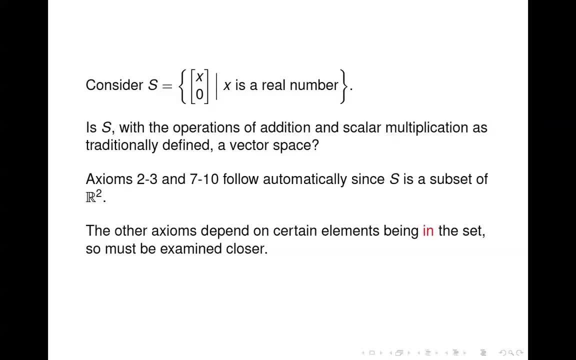 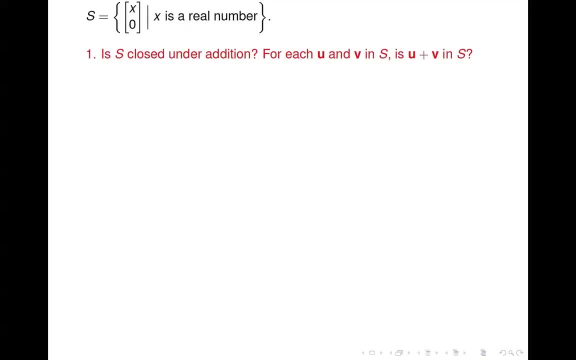 certain elements being in the set, so we have to look at this closer. so number Number one is S closed under addition ie, if you take two elements in the set, do you get another element in the set? Take two elements in the set and add them together, do you get another element in the. 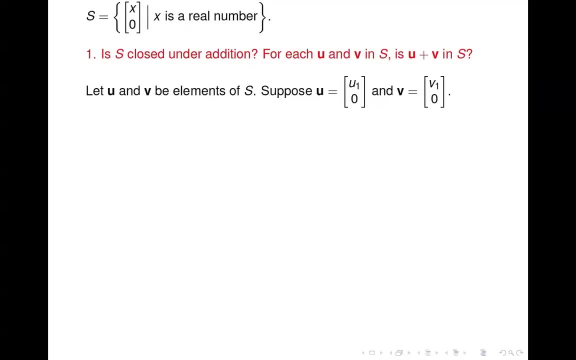 set. Well, here I've taken a couple of generic elements from the set u and v and if we add them together, as I've done here, notice that you get this vector of this form: u1 plus v1 in the first component, zero in the second component, and this vector is in it. 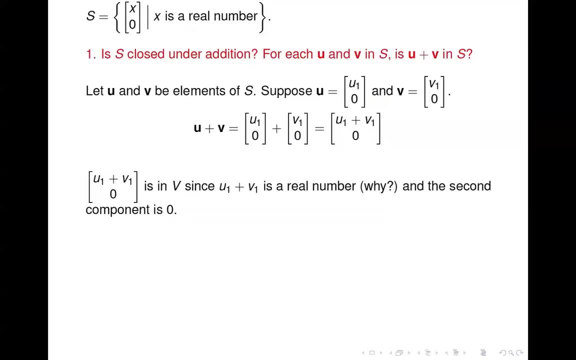 should be an S there. this vector is in S instead of v, Since u1 plus v1 is a real number. let's pause here. why do we know that u1 plus v1 is a real number? The reason we know that is because u and v are both real numbers. 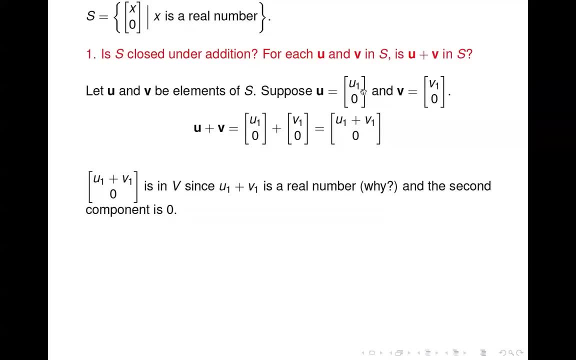 They're both an S, and therefore u1 has to be a real number, v1 has to be a real number. so we add two real numbers together, we get another real number. Okay, so we know the first component's a real number, second component is zero, and that's. 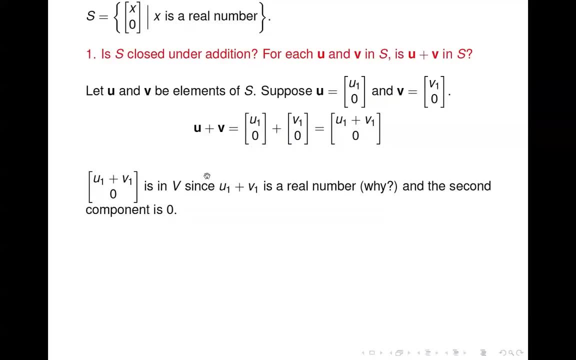 what it takes to be in the set S. so S is closed. under addition By number four: does S contain a zero element? Does S contain a zero element? Does S contain a zero element? Does S contain a vector zero, such that when you add zero to any vector in the set, you? 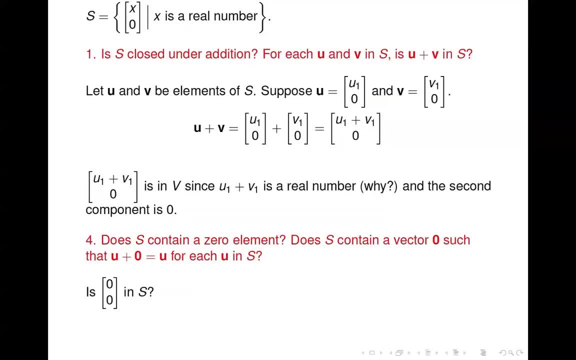 just get that vector back. Well, the obvious choice would be zero, zero. so the question is: is that vector in S? And the answer is yes, because, remember, to be in S, the first component has to be a real number, which zero is, and the second component has to be zero, which we have here in the 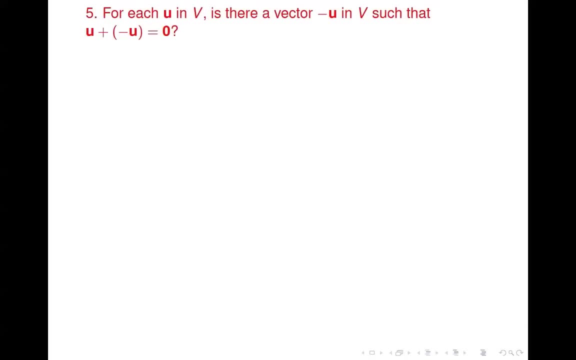 zero vector. Okay, number five. does each element have an additive inverse? Well, if we start off with a generic element of the set, say u equals u10,, we can add to that this vector, negative u10, and it is in the set. 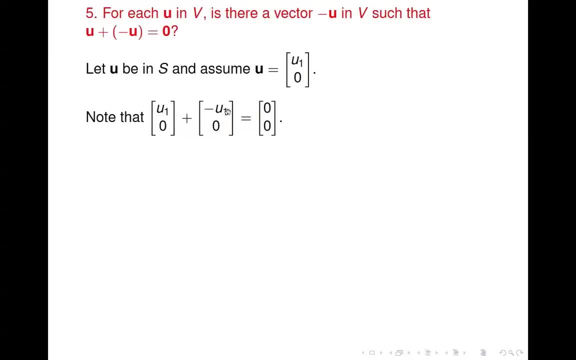 How do we know that? Well, if u1 is a real number, then negative u1 has to be a real number and we have the second component's zero. When we add those together we get the zero. vector Is S closed under scalar multiplication. 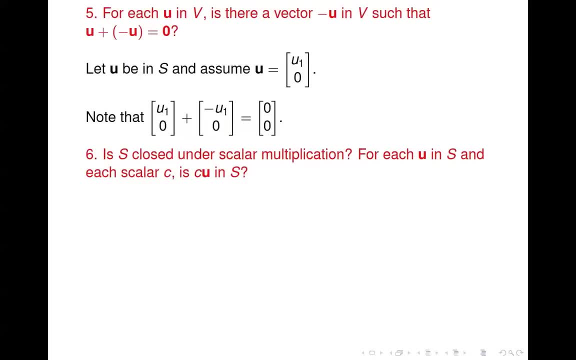 So if we multiply- take a generic element from the set, multiply it by a scalar- do we get another element in the set. Well, here's a generic element of the set: u equals u10.. C is a scalar, that just means it's just any real number. and if we multiply c times u, 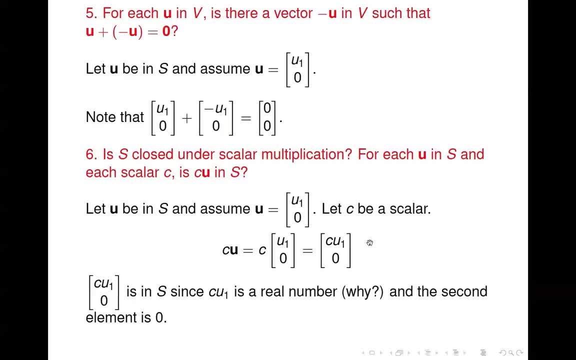 we end up with cu1 in the first component. now that has to be a real number, which it is, because c is real, u1 is real, got the product of two real numbers, and that's another real number, and the second component is zero. 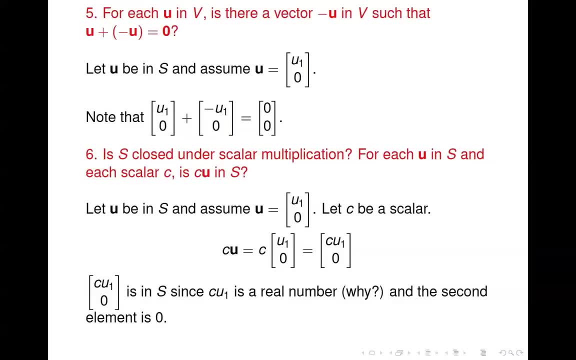 That's what it takes again to be an S. so S is indeed closed under scalar multiplication, and at this point we've established that all ten of the axioms are satisfactorily equal. Okay, number five: does each element have an additive inverse? 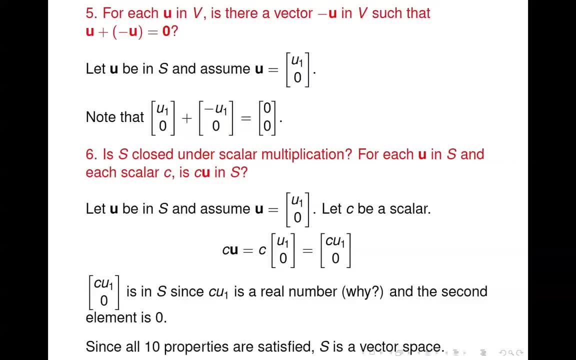 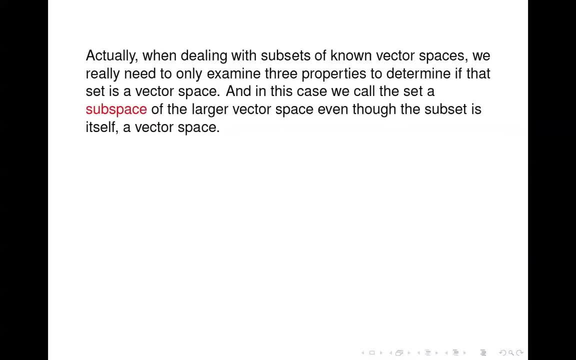 Well, if we start off with a generic element of the set, u equals u10, and it is in the set. We've established that the set is satisfied. so S, our set S, is a vector space. Okay, now it turns out that when you're dealing with subsets of known vector spaces, just 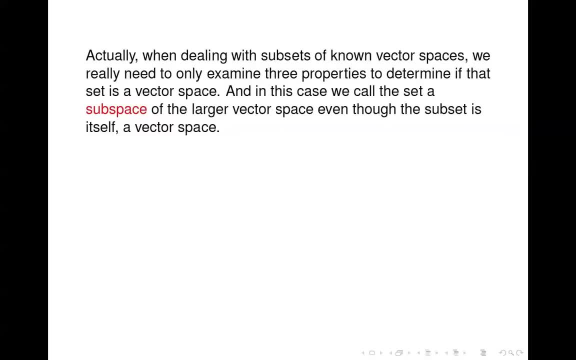 like we were here, S was a subset of R2, then we really need to only examine three of these properties to see if the set's a vector space- and actually we typically call it a subspace of the larger vector space, even though it is actually in itself a vector space. 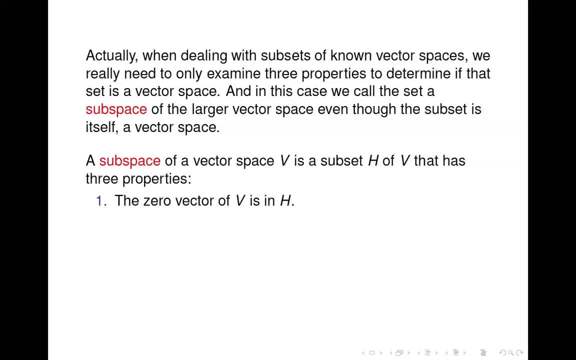 Okay, so there's the three properties are given here. We say a subspace of a vector space, V is a subset H of V. that has three properties. The zero vector of V is an H, H is closed under vector addition and H is closed under. 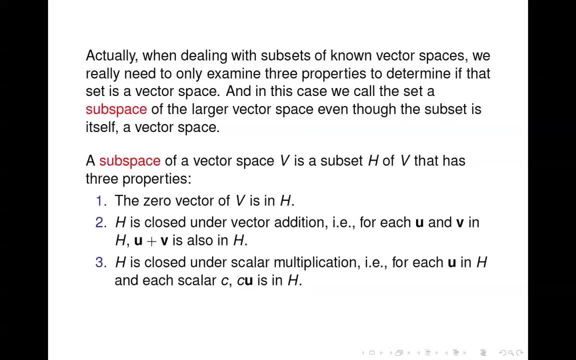 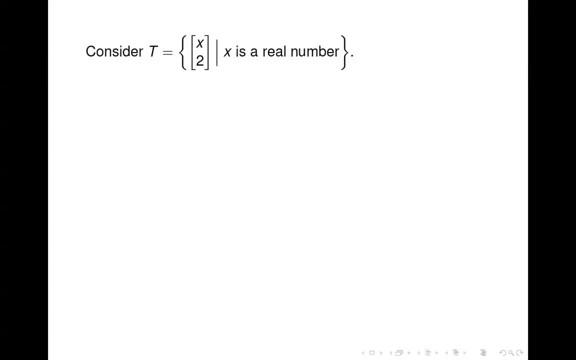 scalar multiplication. Okay, so if we want to check to see if a set is a subspace of a vector space, we need to only check these three properties. All right, so let's do that here. Here's another set, T, and T is a subset of R2, and it consists of all vectors where the 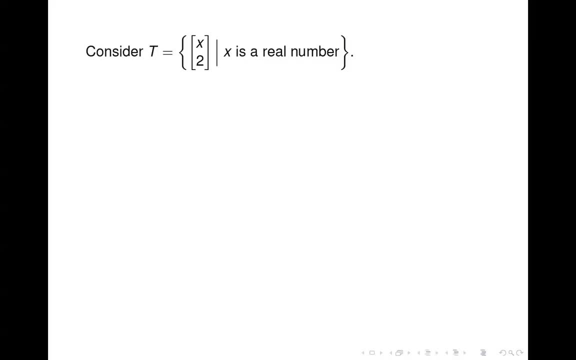 first entry is any real number and the second entry is a 2.. So I want to know: is T a subspace? It's a subspace of R2.. So, looking at the first one, does T contain the zero vector of R2?? 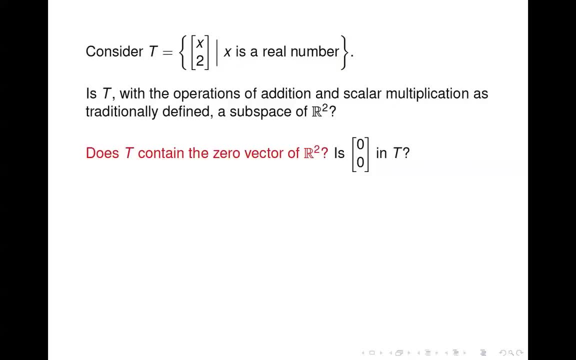 That was the first requirement to be a subspace. So I'm asking: is zero zero? is the vector zero, zero in T. And if you look up here at T, remember what does it take to be in T? First component's: any real number. second, component's 2.. 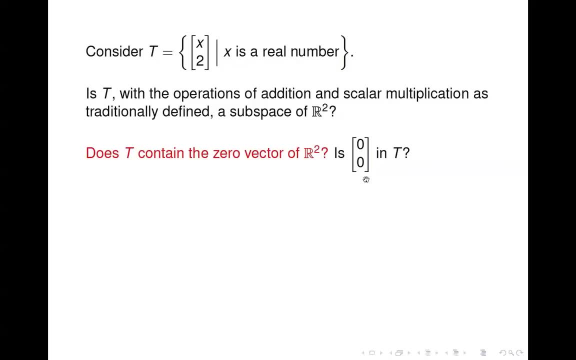 So we look at zero zero. does that fit that bill? No, it doesn't. Why not? Because the second component here is zero, To be in T. the second component has to be a 2. So zero, zero's not in T. and at this point we could stop and say no, T is not a subspace. 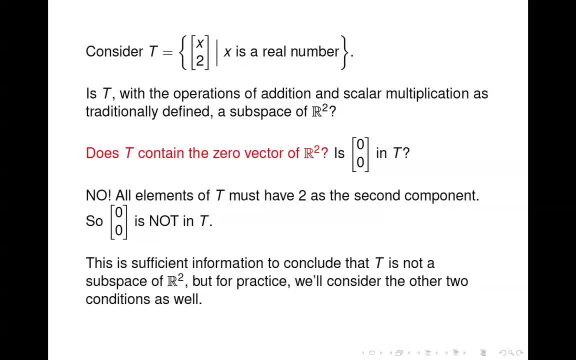 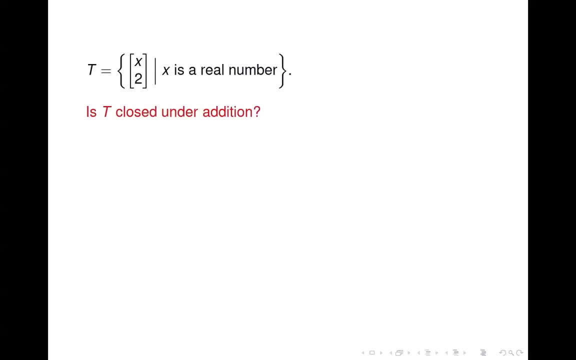 of R2, because it doesn't contain the zero vector of R2.. But for practice, let's just keep going and consider the other two conditions. So here's T again. Is it closed under addition? So if I take two elements of T and add them together, do I get another element of T? 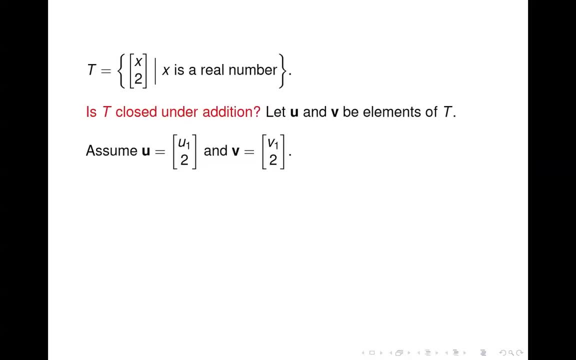 Well, here's a couple of generic elements of T. If I add them together, what happens? Oops, look at that second element here. Second element in the sum of these two is a 4.. So this is not in T, because to be in T, your second component has to be a 2.. 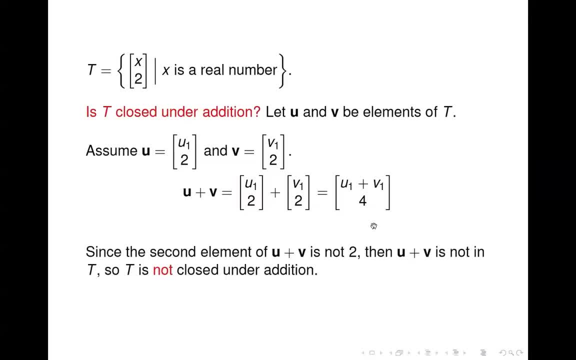 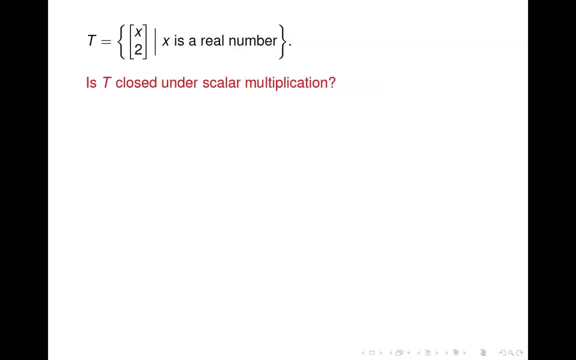 Here it's a 4.. OK, So T is not closed. under addition, How about scalar multiplication? Is it closed under scalar multiplication? Well, let's take a generic element of T. Here's one. got a real number on top 2 in the second. 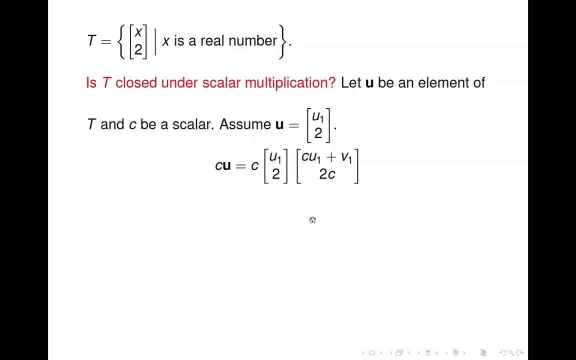 component. We multiply by scalar and what do we get? We get this vector. Actually, we shouldn't get that vector. OK, That vector. that V1 should not be there. I apologize for that. Should be just Cu1 in the top, 2C down in the bottom. 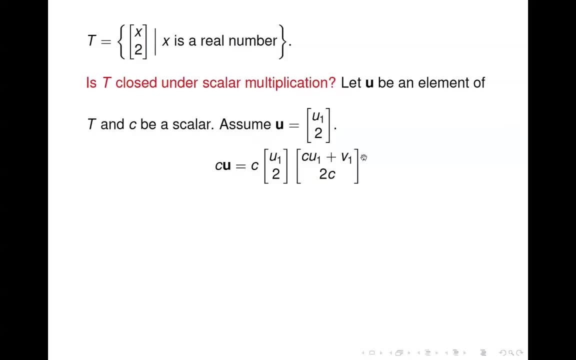 Make a note of that. So again, this plus V1 shouldn't be here. But let's look. What's important really is the second component, the 2C here, because what we want to know is: is that 0?? 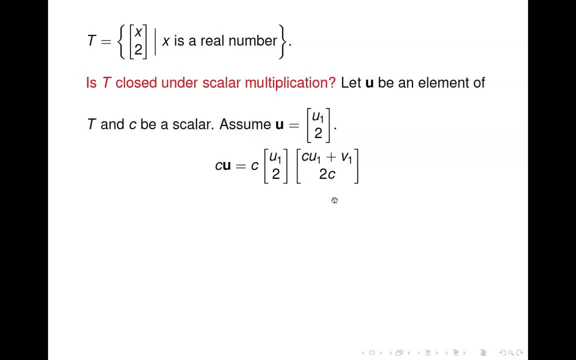 And the answer is: Well, it's 0 only if C is 0.. And C is not restricted to be 0. And therefore we can easily come up with a counter example to show that we can take a scalar multiple of an element of T and end up with something outside of T. So T is not. 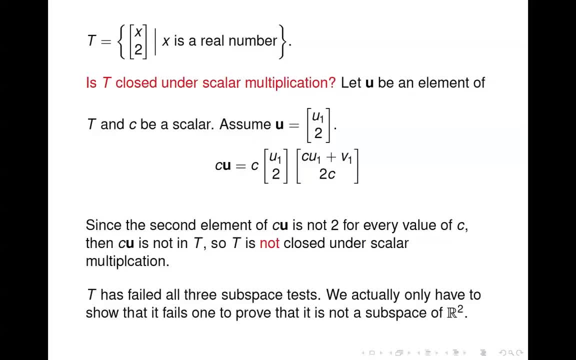 closed under scalar multiplication. All right, let me make one more note. All right. So in this case this set T failed all three of the subspace tests. Again, if you were simply trying to determine if T is a subspace of R2, you only need to. 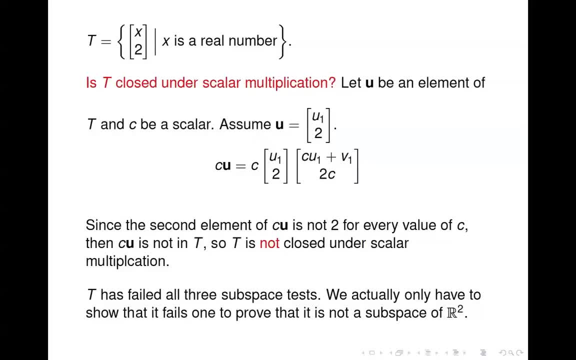 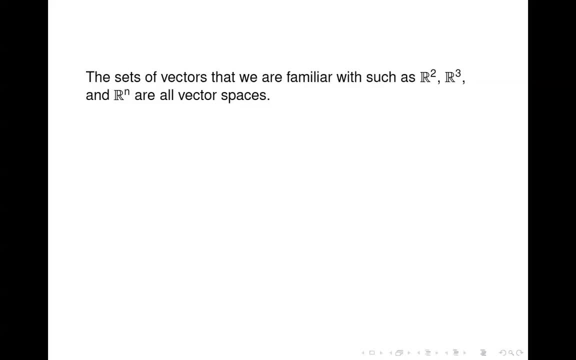 find one that it fails, and then you could stop there. I just showed you all three just for practice, OK, So, as I said before, these vector spaces such as R2 and R3 and Rn, Those we are familiar with, 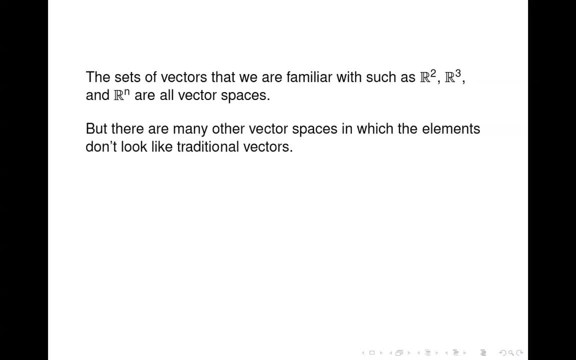 But there's a lot of other ones in which the elements don't look like traditional vectors. So let's kind of examine that a little bit. Consider this set. I'm calling M sub 2 by 2, which is the set of all 2 by 2 matrices. 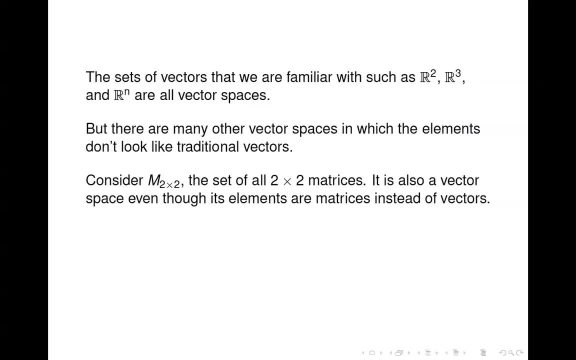 OK, where all the components are real numbers, Turns out that M sub 2 by 2.. M sub 2 by 2 is also a vector space, even though its elements are matrices instead of vectors in the traditional sense. So let's go back through those properties with M sub 2 by 2 in mind. OK. 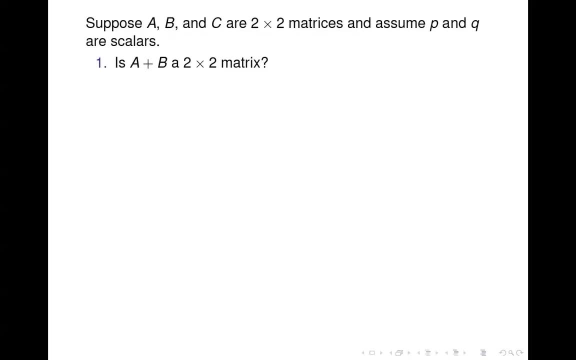 So let's start off and suppose that A, B and C are 2 by 2 matrices and that P and Q are scalars. So property number one, We add A and B together, Do we get another 2 by 2 matrix. 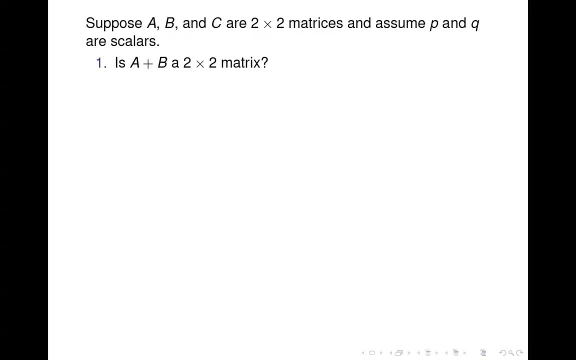 This is saying: is M sub 2 by 2 closed under addition? And clearly it is. If you add two 2 by 2 matrices together, you get another 2 by 2 matrix. All right, Here are the second and third properties. 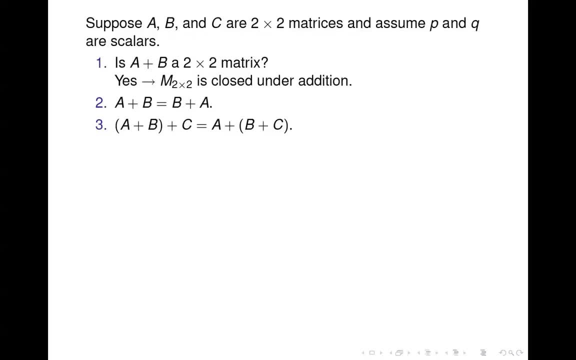 Those fall straight out from properties of matrices. Number four: Is there a zero matrix? All right. Is there some 2 by 2 matrix? OK, There is a matrix such that you can add to any other 2 by 2 matrix and get that same. 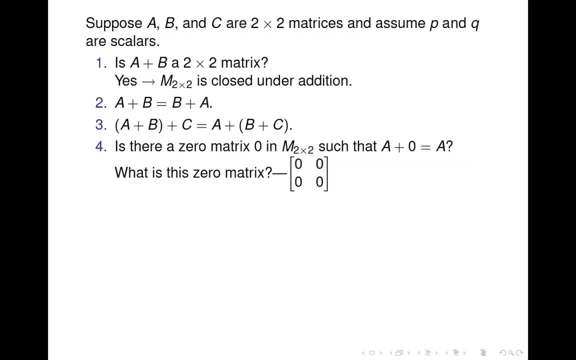 matrix back? Well, clearly there is. It's a matrix with zeros in all the positions And number five. If you add negative A to A, you get the zero matrix. Number six is M sub 2 by 2, closed under scalar multiplication. 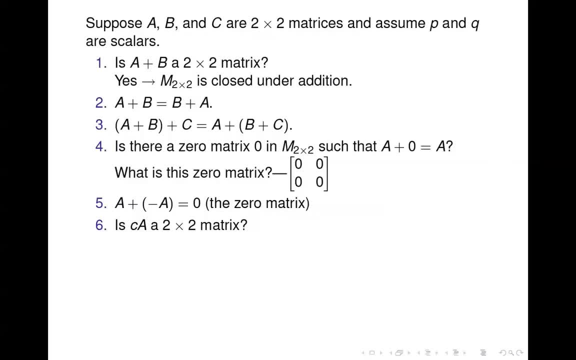 So if you take any 2 by 2 matrix And multiply that by 2. And multiply it by scalar, do you get another 2 by 2 matrix- And of course you do So. it's closed under scalar multiplication. And then these final four properties fall straight out from what we know about matrices. 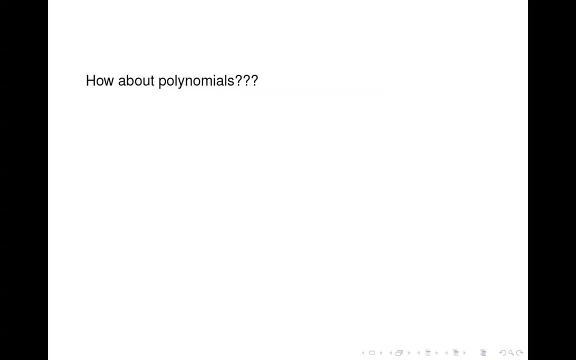 So M sub 2 by 2 is indeed a vector space. Another one about polynomials. Polynomials are some standard examples of vector spaces. OK, Let's first start with P sub 2.. P sub 2 is the set of all polynomials of degree 2 or less. 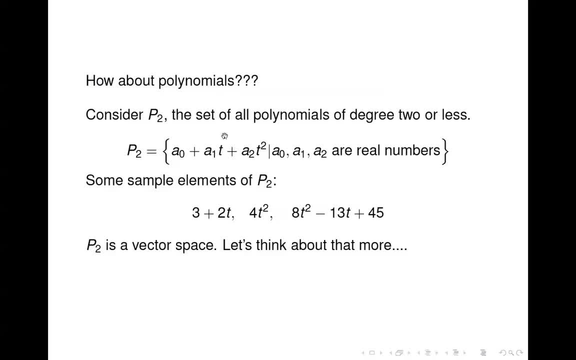 OK, So we wanted to write it in formal terms. It would look like this: A0.. Set of all A0 plus A1 times t plus A2 times t squared, Where A0, A1, A2 are real numbers. 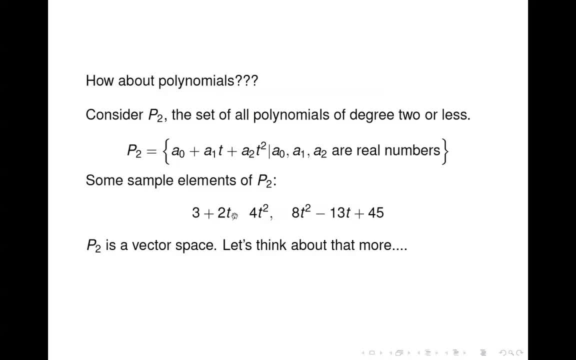 So here's some sample elements of P sub 2.. 3 plus 2t. OK, Here 3 is A sub 0 is 3, A1 is 2, A2, in this case would be 0.. 4t squared. 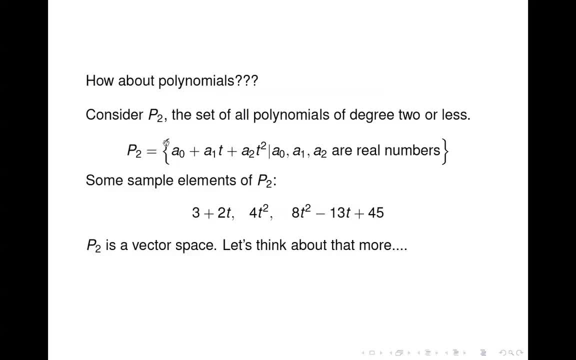 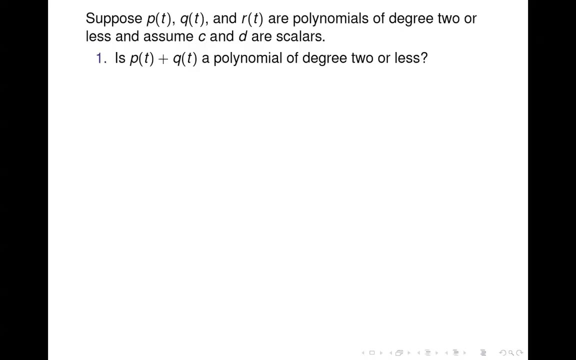 That's in there. 8t squared minus 13t plus 45.. That's in there, OK. Any polynomial of degree 2 or less, OK. And P sub 2 is indeed a vector space. Let's look at these properties in terms of P sub 2.. 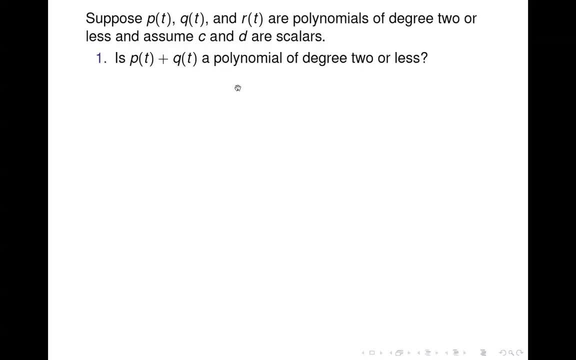 So if we add two polynomials of degree 2 together, do you get another polynomial of degree 2? OK, Well, yes, you do. Here's how that works. You've got two- Let's call it P of t- which looks like this: 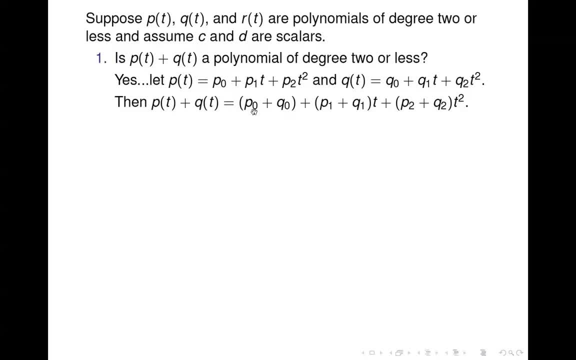 Q of t, which looks like this: And if we add them together then we get this polynomial here, which is again of degree 2 or less. OK, They satisfy the properties 2 and 3.. I'm going to let you explore that some more. 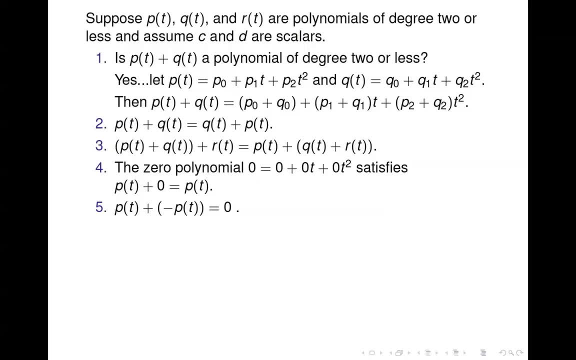 Number 4.. Do you have a 0 element? Is there a 0 polynomial? Well, yes, there is, It's just 0. We add 0 to any polynomial, we get that same polynomial back If we negate all the coefficients in a polynomial. 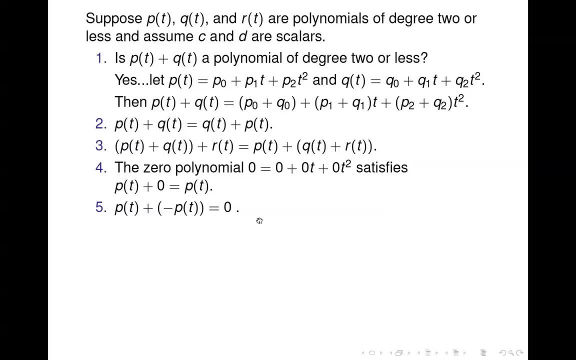 and add it to the original one, we get the 0 polynomial, OK, Number 6.. Is this set of polynomials closed under scalar multiplication? So if you multiply any polynomial of degree 2 or less by a scalar, do you get another polynomial of degree 2 or less? 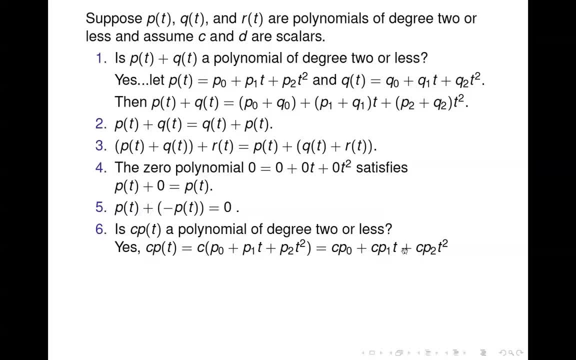 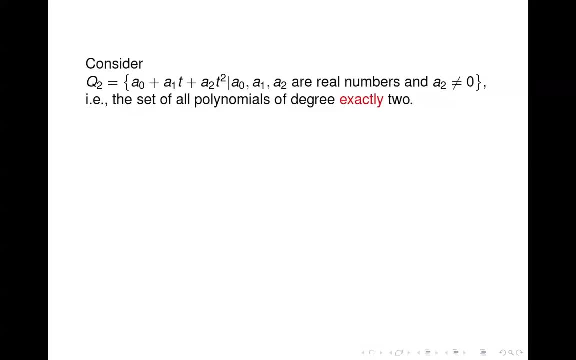 And the answer is yes, Guy here. Multiply by scalar and we get another polynomial of degree 2 or less, And again 7 through 10 kind of fall out pretty straight. OK, Very straightforwardly. Here's another set. 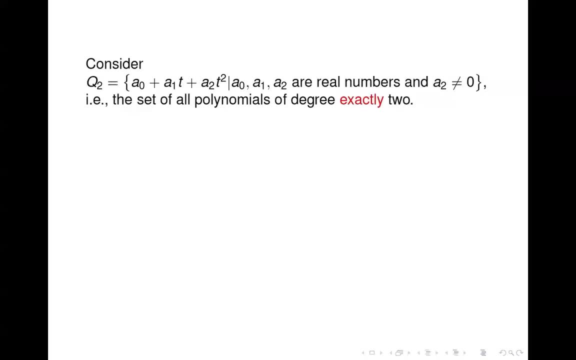 This is a subset Q sub 2. here is a subset of P sub 2.. Here I've got all polynomials not of degree 2 or less, but all polynomials of degree exactly 2.. So the way I've defined it is in this form: 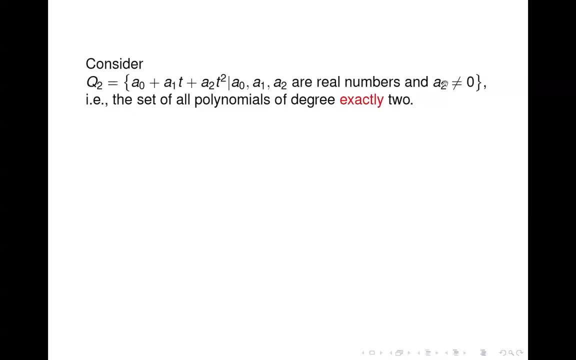 Looks like P sub 2. with this addition, A sub 2 has to be non-zero. OK, So that makes it, where you're going to have a second degree polynomial, Going to have a sub 2 not equal 0. So you're going to have the t squared term showing up. 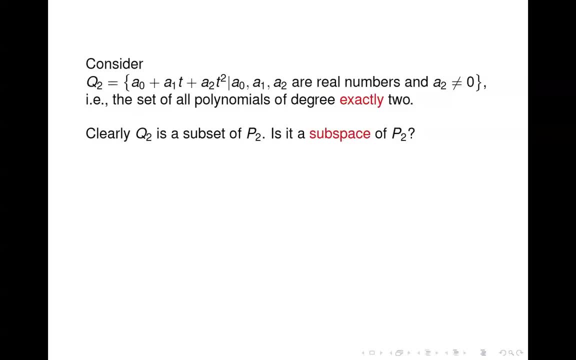 So I want to know: is Q sub 2 a subspace of P sub 2?? So to show that it's a subspace, we need to show that it satisfies those three properties. Includes the 0 element Closed under Addition. 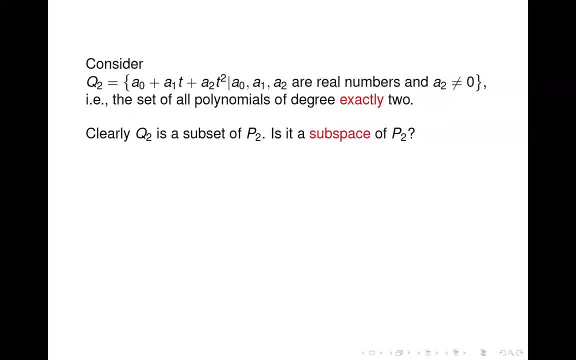 Closed under scalar multiplication. So is that the case? Well, let's start with number 1.. Does Q sub 2 contain the 0 element of P sub 2?? Well, the 0 element of P sub 2 is the 0 polynomial, just 0.. 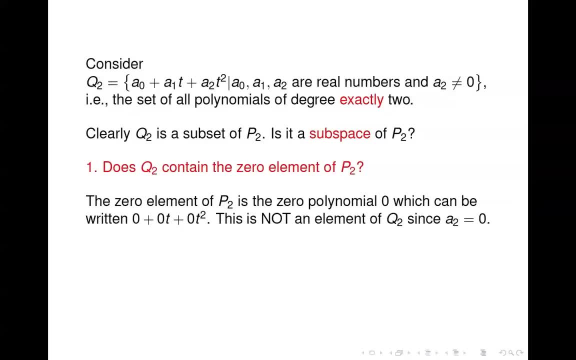 So is that in Q sub 2?? And the answer is no, because go back up and look at the definition of Q sub 2.. A sub 2 can't be 0. Right, But down here, the 0 polynomial, a sub 2 is 0.. 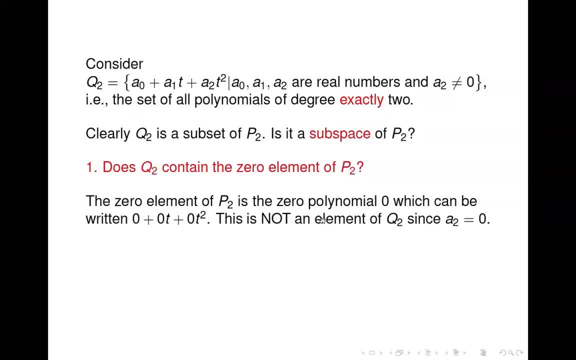 So Q sub 2 does not contain the 0 element of P sub 2.. So we could stop right here and say no, Q sub 2 is not a subspace of P sub 2.. But again, just for more experience. 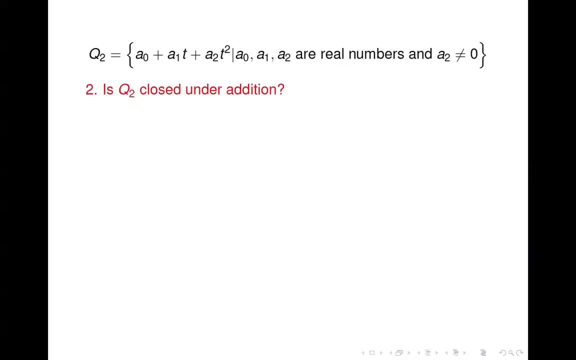 we're going to go on and look at the other two Um. So the second one is Q sub 2 closed under addition. So if we add any two elements of Q sub 2 together, do we get another element of Q sub 2?? 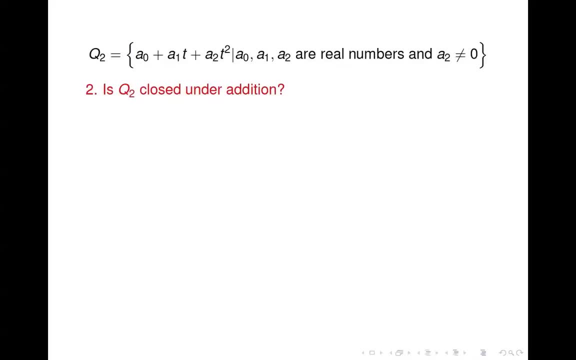 Or if you add any two polynomials of degree exactly 2, or less not or less a degree exactly 2, do you get another polynomial of degree exactly 2? There it is, there. So Here's an example. Let P of t be 6t squared minus 3t. 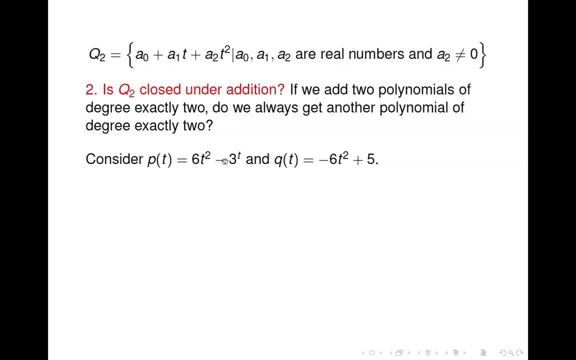 That is in Q sub 2, because we've got a 6. The a sub 2 term is not equal to 0. And here's Q of t, where the coefficient of t squared is not 0. So we've got two polynomials here of degree exactly 2.. 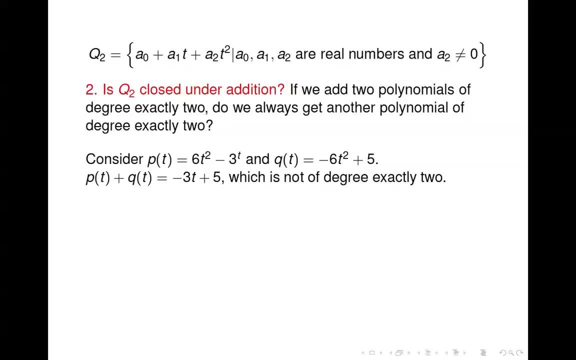 When we add them together, what happens? The t squared terms go away. We're left with negative 3t plus 5. And that is not of degree exactly 2.. So Q sub 2 is not closed. under addition, How about scalar multiplication? 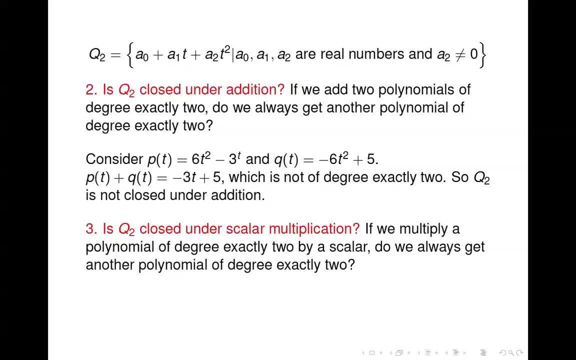 If we multiply a polynomial of degree exactly 2 by a scalar, do we always get another polynomial of degree exactly 2?? So think about that. So if you start off with any sort of polynomial, that's degree exactly 2 and you multiply it. 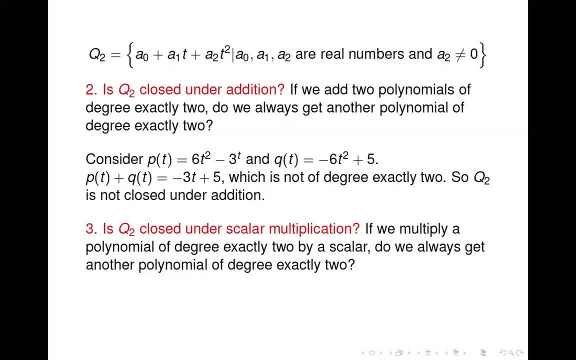 by any scalar, do you always get another polynomial of degree exactly 2?. And if you don't think about that very long, you might say: well, yeah, you multiply it by anything and you're going to get another polynomial of degree exactly 2.. 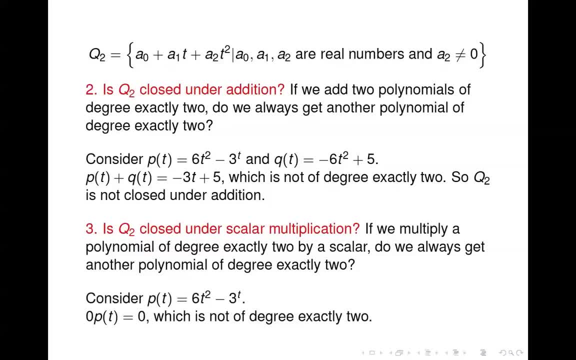 And that's almost always true. But there's one coefficient, one scalar you can use. If you multiply by 0, then you get the 0 polynomial and it is not of degree exactly 2.. So this means that Q2 is not closed under scalar multiplication. 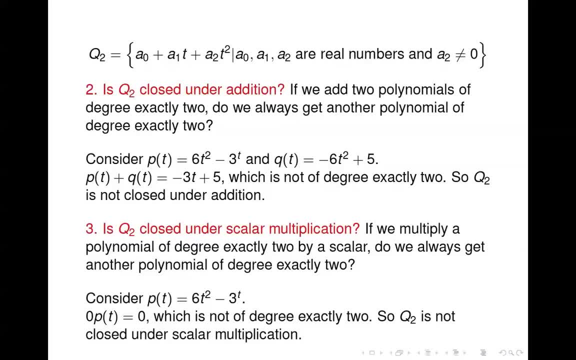 So Q sub 2 here failed all three of the requirements to be a subspace of P sub 2.. Yeah, Only has to fail one to not be a subspace. But this one in fact failed all three properties. OK. 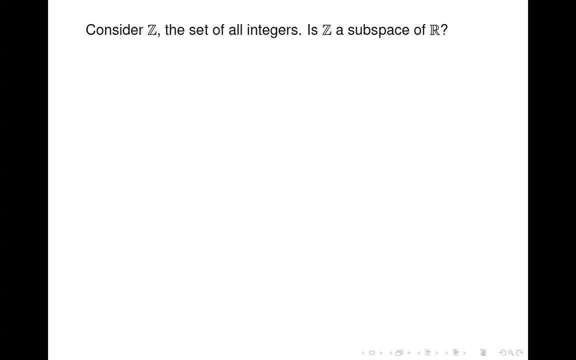 Let's look at one more. Let's look at z set of all integers. OK, And I want to know: is z a subset of the real numbers, a subspace of the real numbers? Excuse me Clearly, it's a subset of the real numbers. 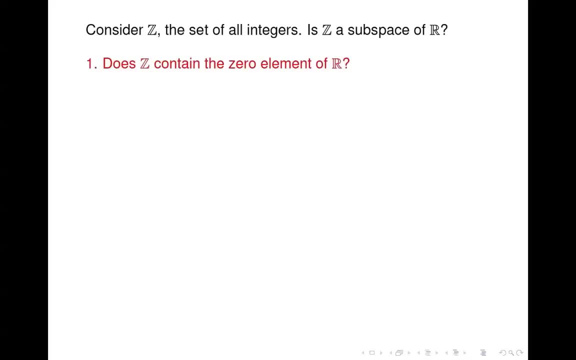 All right. So we want to know number 1, does z contain the 0 element of the real numbers? Well, the 0 element of the real numbers is 0.. OK, The sum of the real numbers is just 0, and 0 is an integer. so the answer here is yes. 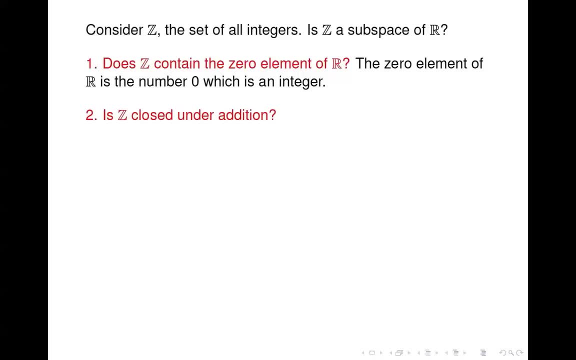 Is z closed. under addition, If you take two integers and add them together, do you get another integer? And the answer is yes, because the sum of any two integers is always an integer. So we passed number 1,, we passed number 2, how about number 3?? 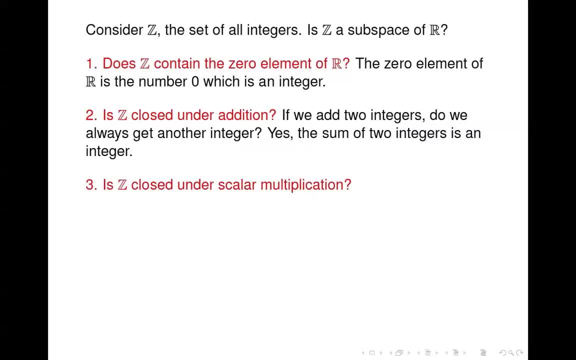 Is it closed under scalar multiplication? So if we multiply an integer by a scalar, do we always get another integer? Hmm, Let's think about that. Trick here is that the scalar could be a real number. You don't have to multiply it by an integer, right? 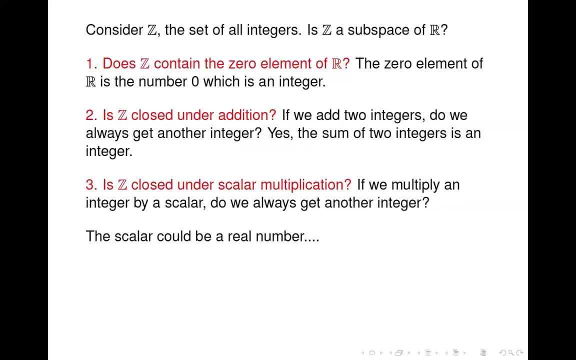 Scalar just means a real number. That real number might not be an integer. So if we multiply our integer by a non-integer, So if we multiply our integer by a non-integer, So if we multiply our integer by a non-integer, 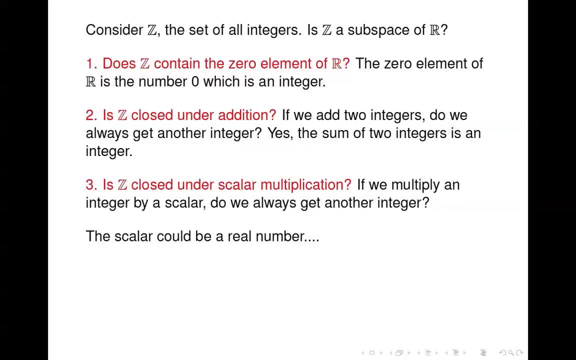 OK. So if we multiply our integer by a non-integer, then we open up the chance that we could end up with a non-integer. So the answer is no, it's not closed under scalar multiplication. and here's an example. 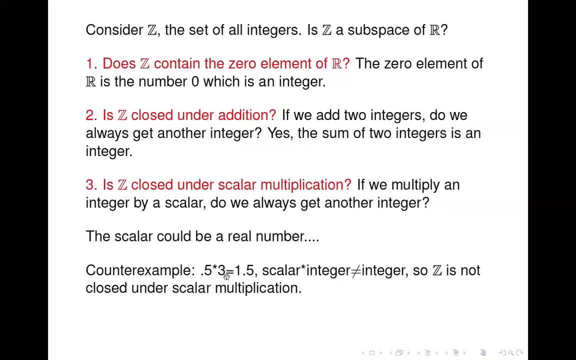 If I multiply 0.5, there's my scalar times 3, my integer: I get 1.5, 1.5 is not an integer. So here's a scalar times, my integer: I don't get another integer. 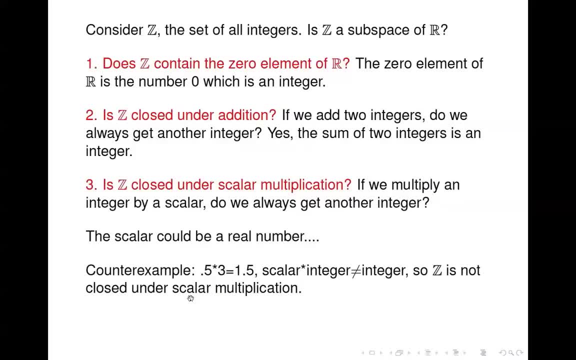 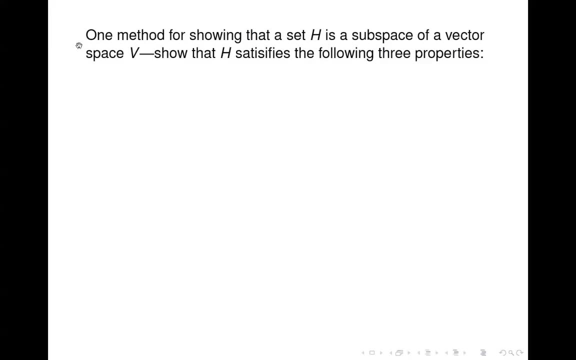 OK, So therefore z is not closed under scalar multiplication and therefore it's not a subspace of the real numbers. OK, we're continuing in section 4.1 with more about vector spaces, and there's one way that we've talked about for vector spaces. 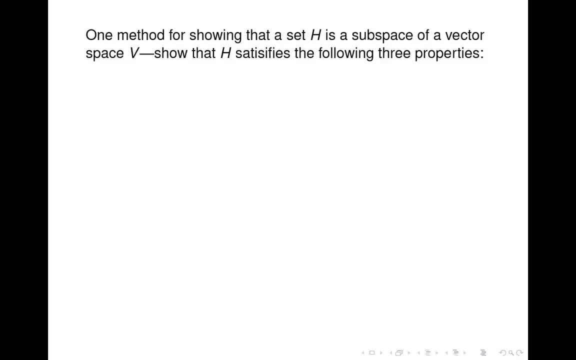 OK, So finding if a set is a subspace of another vector space is to show that it satisfies the three properties that it contains: the zero vector of the parent vector space. It's closed under addition and it's closed under scalar multiplication. 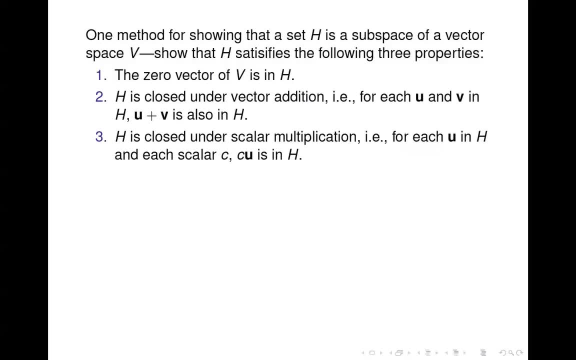 So to show that a set is a subspace, then you can show that these three things are a subspace. To show that these three things hold, or to show that it's not a subspace, show that at least one of these does not hold. 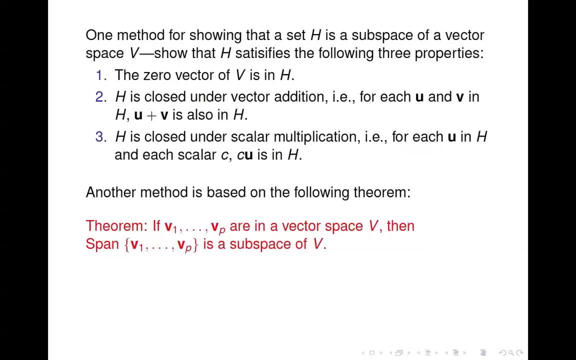 But we have another method for showing that a set is a subspace, and this doesn't work in all cases, but in some cases you can use this theorem and it makes life much easier because you don't have to go through and show those three properties hold. 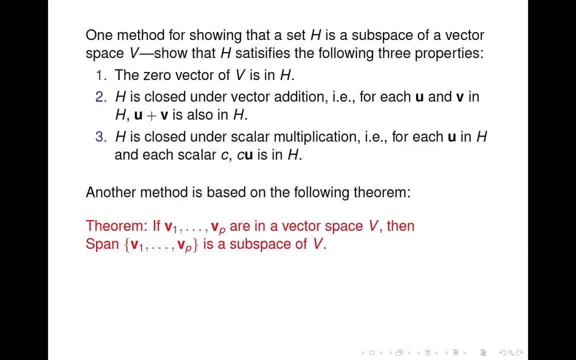 So the theorem says if v1 through vp is a subspace of a vector space, then it's closed under addition. So if v1 through vp are vectors in some vector space, v, then the span of v1 through vp is a subspace of v. OK, 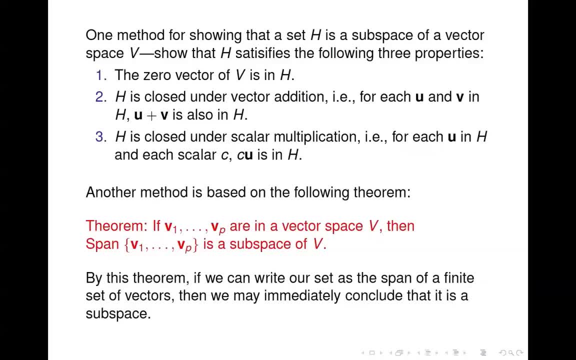 So what this says is that if we can write our set as the span of a finite set of vectors, OK, write it in this form: span of v1 through vp for some vectors. Then automatically we can conclude that the set is a subspace. 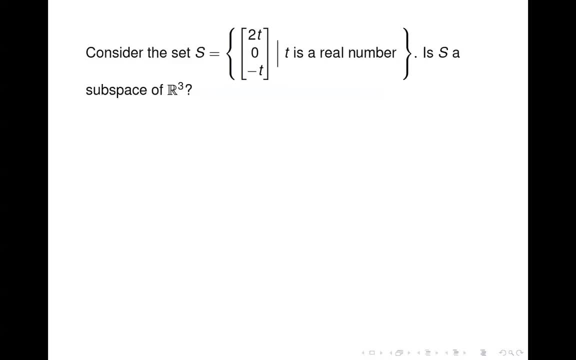 So let's look at this example. We have a set S which consists of all vectors of this form. OK, a subset of R3.. First component is 2 times some real number, t. second component is 0, and the third component 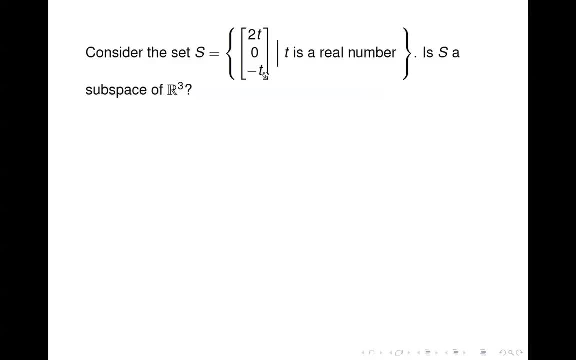 is the negative of that real number t that we had up in the first component. OK, so how? uh, we want to know if S is a subspace of R3.. If we use the original method, uh, that is to show that the three properties hold, then 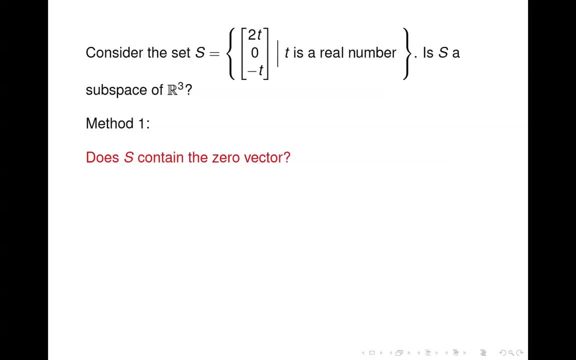 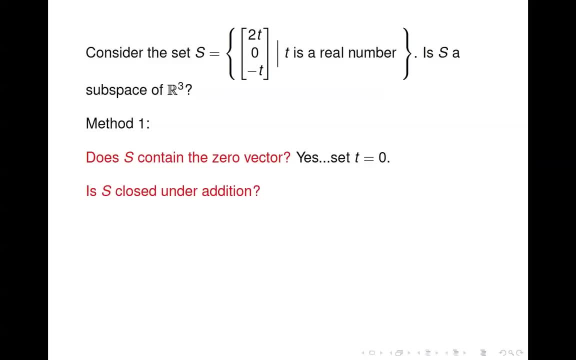 The zero vector is contained in the set S, So we go to um. the next property Is S closed. under addition, We need two generic vectors from S, um, so let's call those u and v And u. uh, looks like 2u- 0, negative u and we'll say v is 2v- 0, negative v, and we need 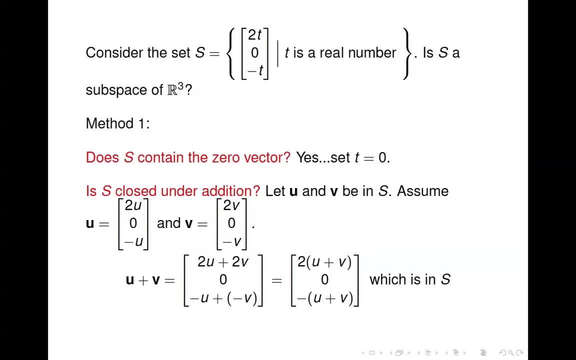 to add those together and see if the resulting vector is in the form uh, that uh has to be to be in S. So add u and v and uh. rearrange terms just a little bit and we end up with this: uh. 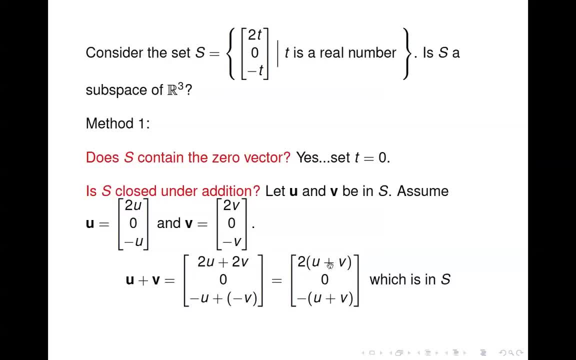 vector. here We got 2 times u plus v- uh in the first component, 0 in the second component, negative u plus v in the third component And this is in the form that it needs to be uh to be in the set S because u plus v here. 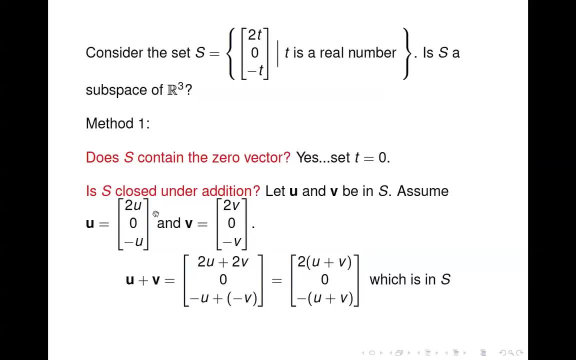 is a real number. Uh, we know that because uh, These, uh these came from the vectors u and v? um. so we have 2 times u plus v in the first component, negative u plus v in the last component, 0 in the middle. 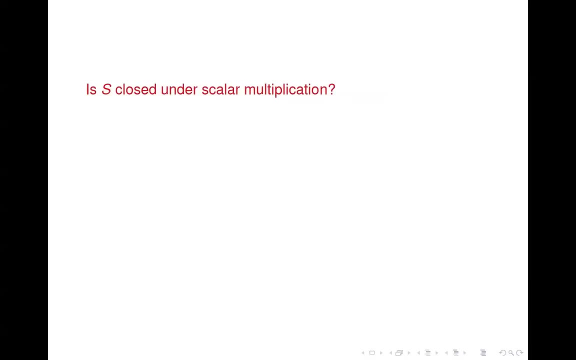 So it is in S. So S is closed under uh addition. So we move on to the third property, um. is S closed under scalar multiplication? Well, again, we need a generic vector from the set S in a scalar which we'll call C. 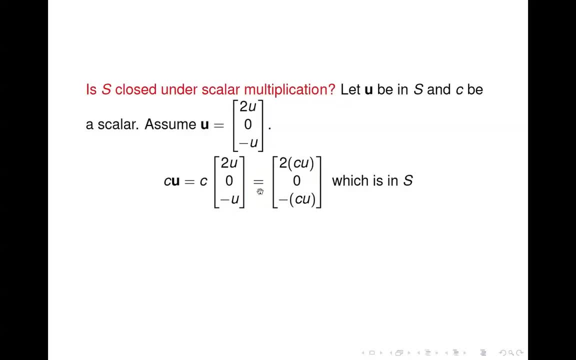 And we compute C times u and uh. again, rearranging terms a little bit, we can write it as: 2 times cu in the first component, negative C times u in the last component, 0 in the middle. And since both C and u are real numbers, then C times u is a real number. so this vector 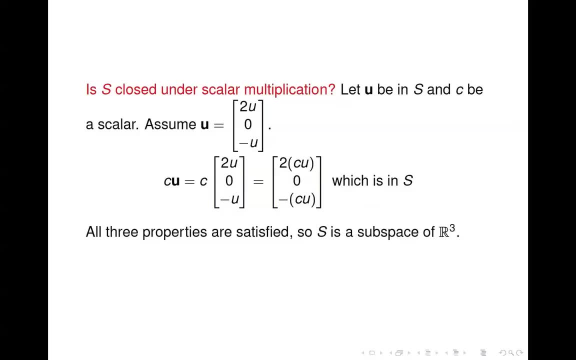 is in S, So we have all three properties satisfied and therefore S is a subspace of R3.. Now there's a fair amount of work that went into that Um, and so let's look at how we could use, or if we could use, this theorem to make the 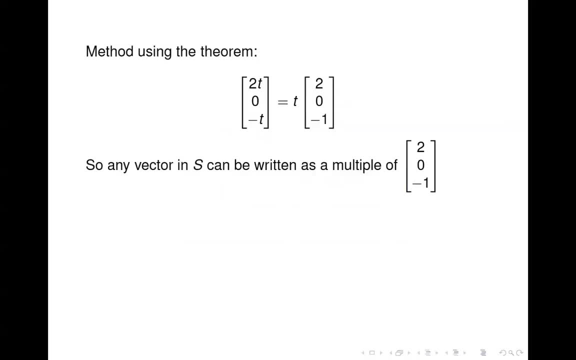 uh, the work a little easier, Alright. uh, if we take a generic vector from the set S and we write it in parametric vector form, so that means factor out the parameters. um, in this case there's only one, T and 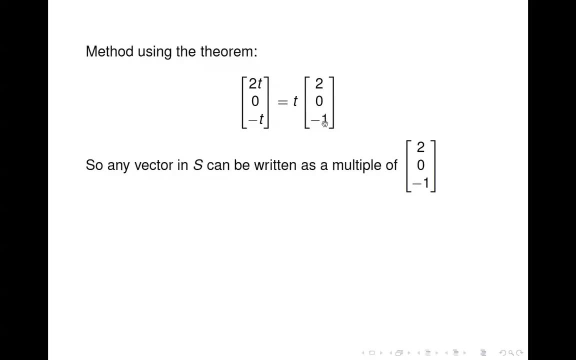 so we can write any vector in S as T times 0,, uh 2, 0, negative 1.. So any vector in S is a multiple of this vector. Therefore, uh S is equal to the span of this vector and since we've written S as the span, 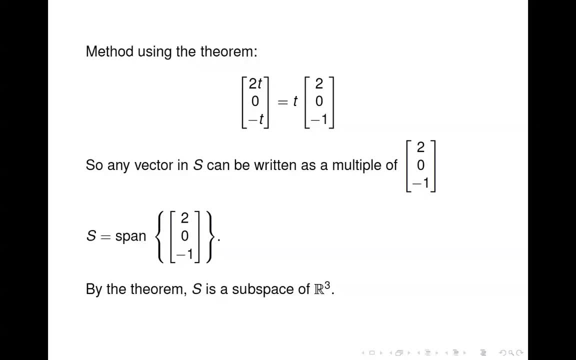 of a finite set of vectors. that means, uh, by the theorem S is a subspace of R3.. So you can see here that if you can, if your problem is one in which you can use this theorem, then, uh, it makes the work much easier. 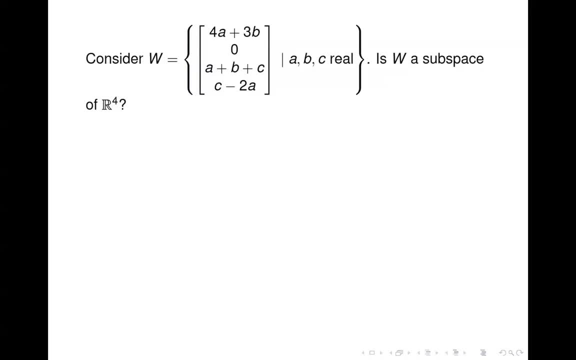 Here's another example: uh, in that set we'll call W, um it's a subset of R4, and uh, we want to know, is uh W a subspace of R4?? So again we could go through the three uh properties. you know, zero vector closed. 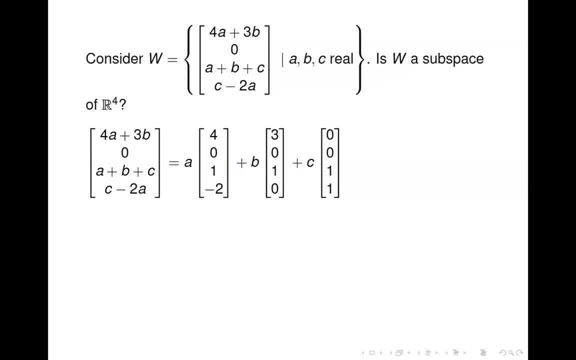 under addition closed under scalar multiplication. but it's much easier um to apply the theorem. So here we uh write this generic vector In parametric vector form. there are three parameters here: A, B and C. We factor those. 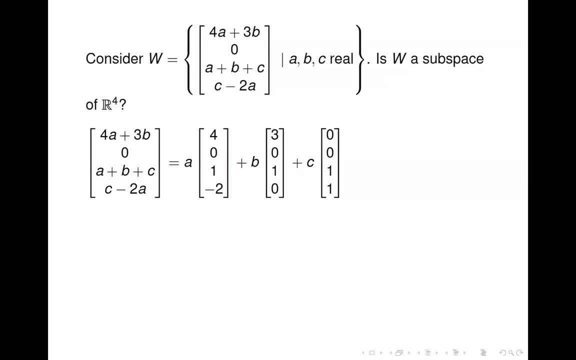 out and uh, and so at this point we have written uh, this generic vector as a linear combination of these three vectors. That is exactly what it means when we say that um, W is the span of those vectors. 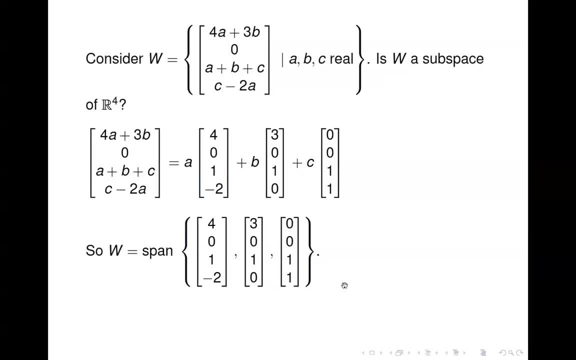 Because any vector in W can be written as a linear combination of these three. So again we've got W. That W is um the span of a, a finite set of vectors, and so by the theorem it must be a subspace of R4.. 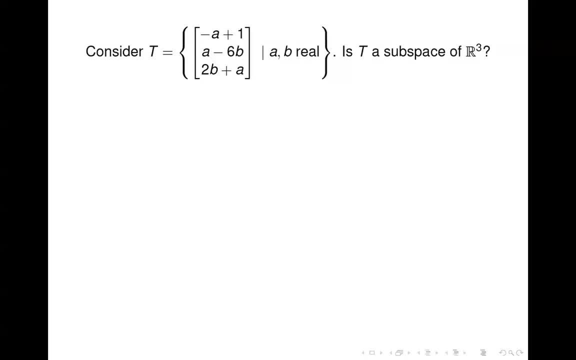 All right, here's another one: um set T, um given here, and uh we want to know: is it a subspace of R3?? So we proceed as we did before: apply uh, try, uh, try to write uh this generic vector. 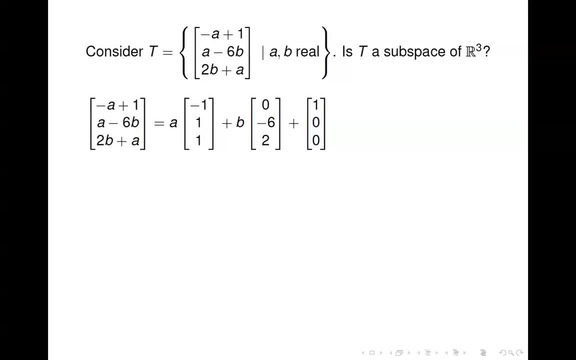 as a uh sub, as a uh linear combination- apologize for the phone there- linear combination of uh vectors in uh R3.. Um, and so we can write it, but notice what happens. Um, if we factor out the A and the B, we're left down here with uh a vector, but no. 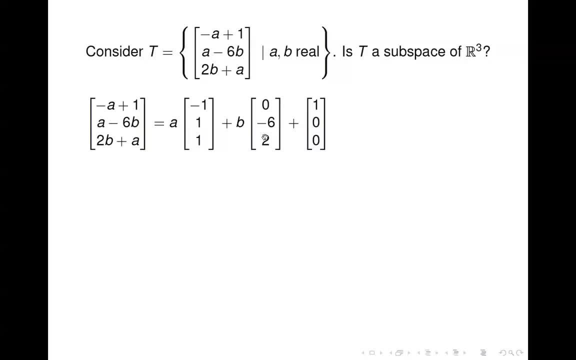 parameter associated with it. And so We can't write this vector as a linear combination of vectors, because a linear combination means you've got a, a parameter or a multiplier in front of each vector, And here, uh, the multiplier is set at 1.. 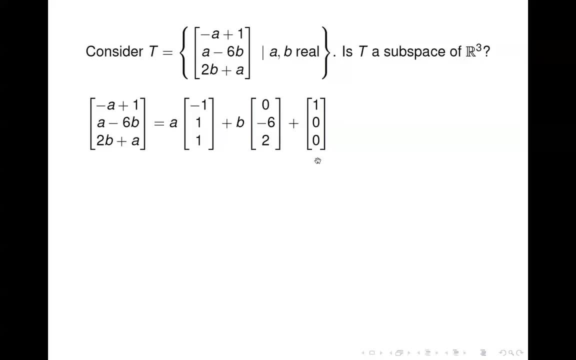 We can't uh alter this, So this is not a linear combination and so we cannot apply theorem uh the theorem here. All right, And so In this case Our only uh alternative is to go back to the first method. 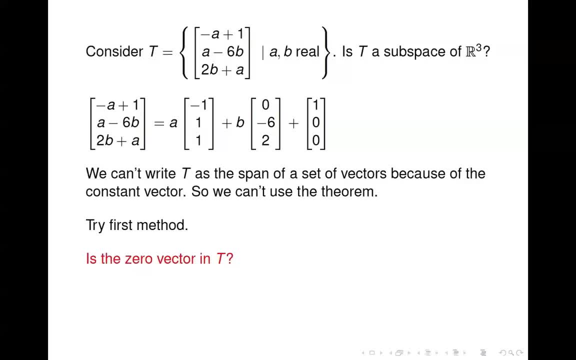 And so, uh, let's- I'm gonna go through that here just uh, because it's always good to have practice um in doing that. So we look and we say: is the zero vector in the set? And um, a lot of times when you have a constant term like this, uh, that's a red flag, um. 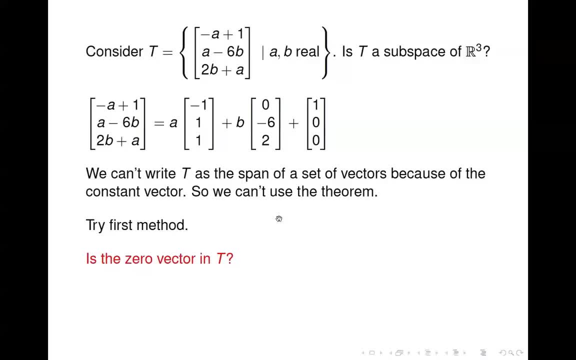 and you have to think about that very carefully because a lot of times, in those cases it's it will not be a subspace because, um, in a lot of cases it moves you away from the origin, which means that your set does not contain the origin. 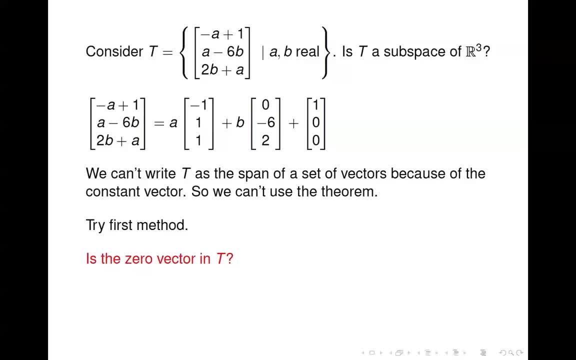 So that's what we're asking here. Is the zero vector in T? Well, uh, for the z, for the zero vector to be in there. that means that each of the elements, uh, we, we need to be able to make each of the elements equal to zero. 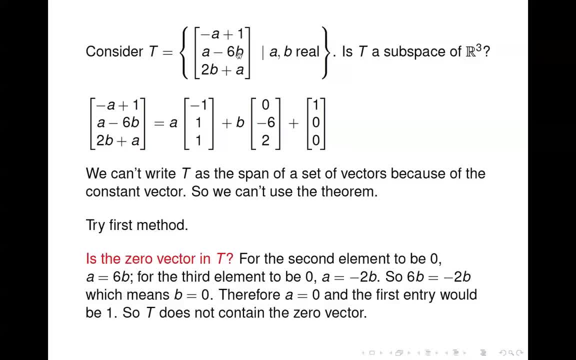 So if you look at the, the first, er, the second component, uh, for this to be zero, that means a has to equal six b. and then the third component: it would mean a has to equal negative two times b. 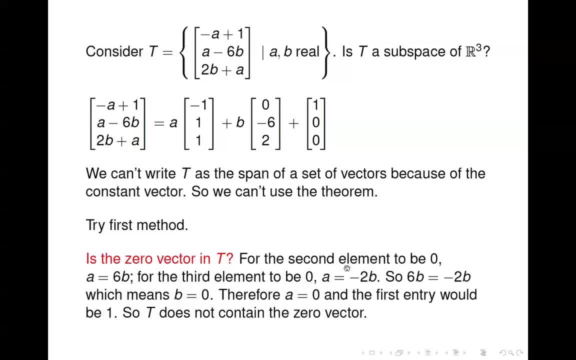 Okay, so if we put that together, uh, then that means that six b is equal to negative two b, and down here this point, and uh solving that. that means that b has to be zero, All right, And if b has to be zero, a is six b, so that means a is zero. 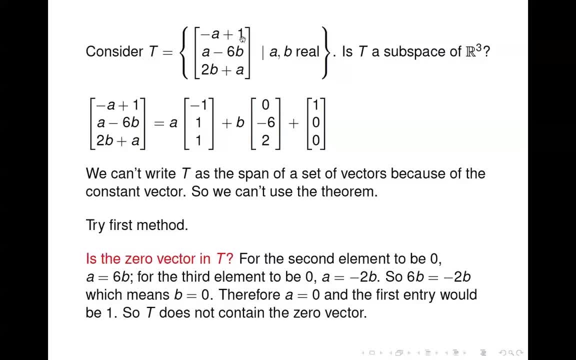 And in that case we look back at the first component That says: you get a one there And so therefore the origin is not contained in this set. all right, Because to get zeros in the second and third positions, that means uh, we're gonna end. 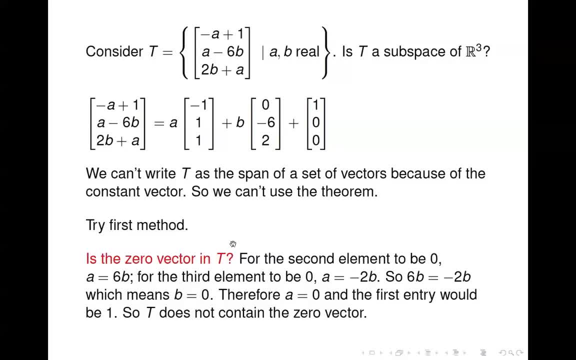 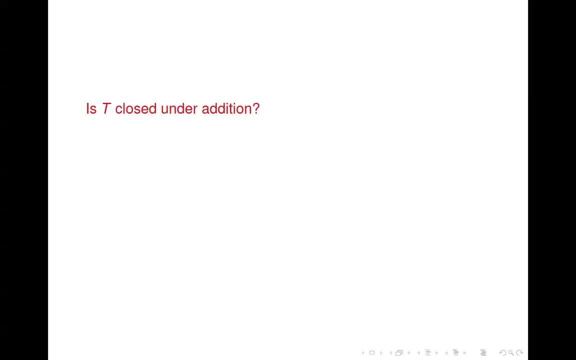 up with a one in the first position. So T does not contain the zero vector. Now, at this point you could stop and say T is not a sub uh space of R3, but just for practice I'm gonna continue on uh and say, um, is T closed under a? 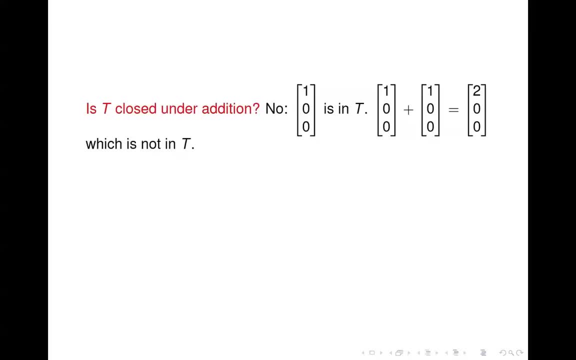 And the answer is uh, no, uh, it's not um. now, to show that we need to um, add two vectors together, We need to take two vectors from T, add them together and uh see if we get um another. 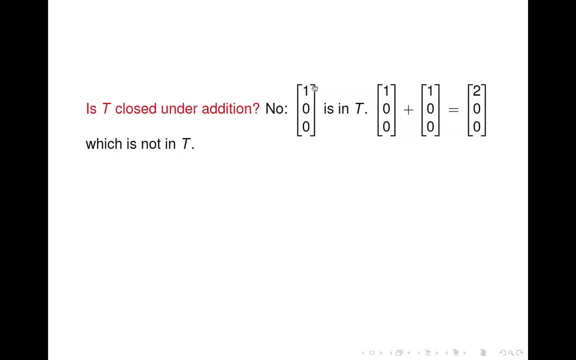 vector. that is in the set. So, um, I picked one zero, zero. It's in the set, uh, because it's what we just talked about. If the two second two components are zero, then the first one has to be one. 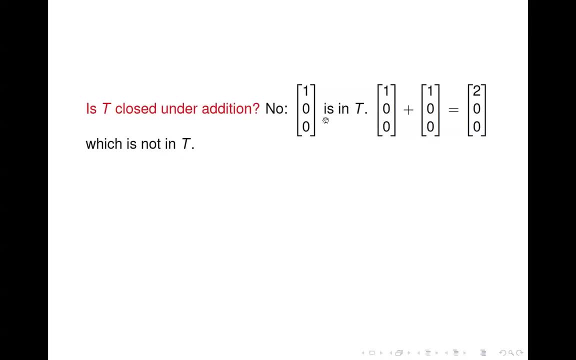 And so um, uh, so one zero zero is in the set, So I'm just gonna add it to itself and the result: um is two zero zero. And so let's think: um is that in the set. 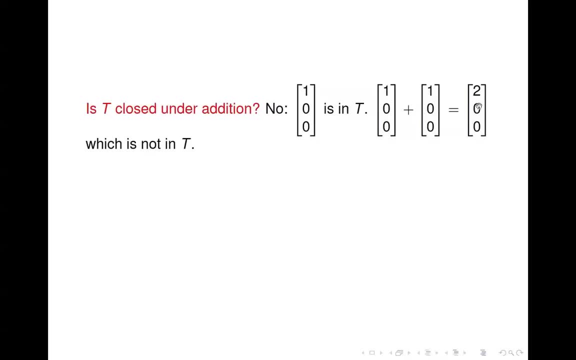 And uh? the answer is no because, as we said before, if the second two components are both zero, then the uh first one has to be one. So this vector's not in T and therefore T is not closed under addition. 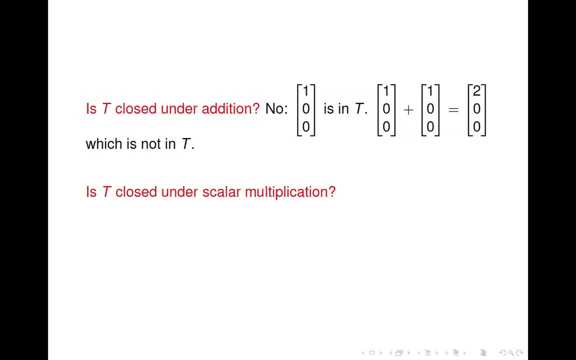 Um. so just for practice again, let's check: is it closed under scalar multiplication? And here we have: uh, no, the answer is no because we've got um again. I just chose one zero, zero, because we know that vector is in T- and multiply. actually we can multiply. 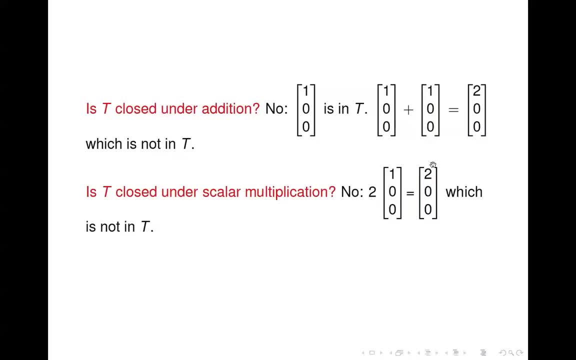 it by anything other than one. Uh, I multiply it by two, We get two, zero, zero. And that is not in T. All right, so, um, this particular set T fails all three of those properties. Um, now here's one that looks similar to T. Um, it's uh got the plus one, so it's got. 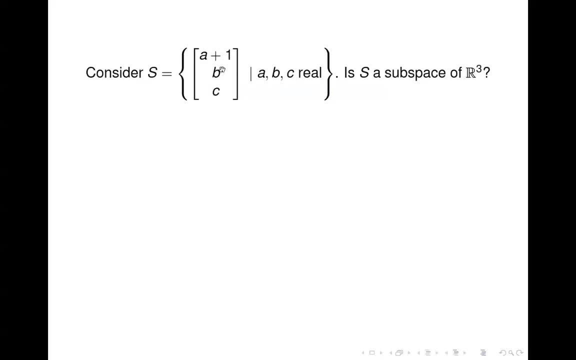 that constant term in it, um, but notice here that uh, the A in the first uh component, here uh, is not constructed. It's constrained by anything in the other two components, And so, um, this one's a little bit different. 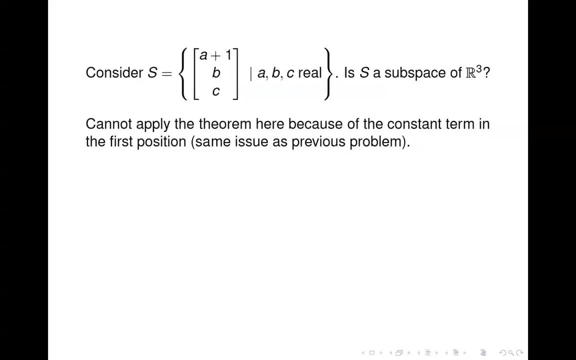 Still, we cannot apply the theorem because of that, that one in the first component. You know we cannot write S as a linear combination of uh, um, uh vectors, Um, because we can't uh account for that one, uh by doing that. 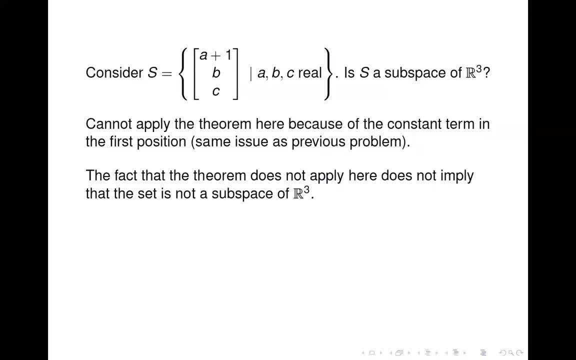 So, um, my point really, Uh, OK, this example is to show that just because you can't apply the theorem does not mean that the set is not a subspace and so, in fact, this one is a subspace of R3. so we're going to go through and just show that. so we have to go back to the 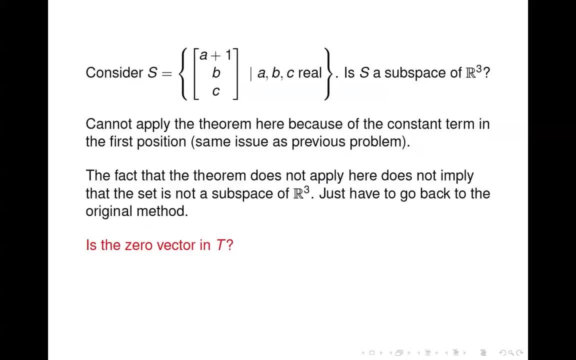 original method for that, and so we ask: is the zero vector in that should be in S? sorry about that. there's a zero vector in the set S, and the answer is yes, because B and C could certainly be zero and we can set a equal to negative 1 and. 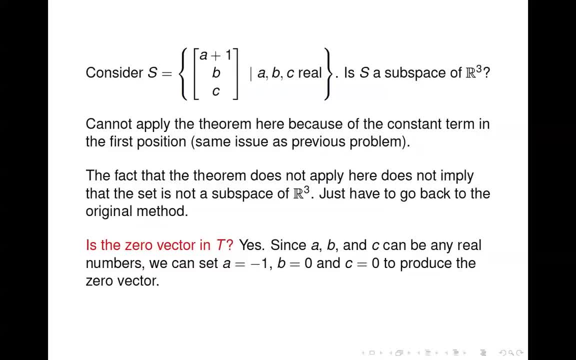 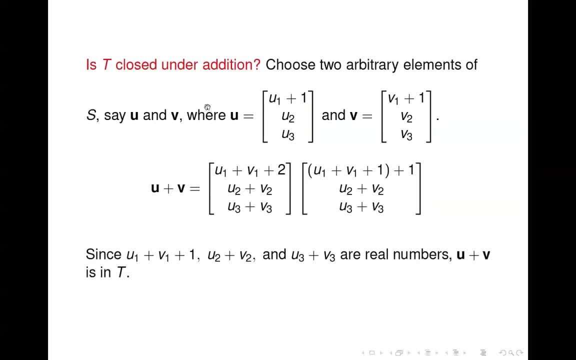 in that case we end up with a zero vector. is it closed under addition? and the answer is: well, we take two arbitrary elements of the set, say u and v. so here's what you looks like, here's what v looks like. So angry us Après uglier. 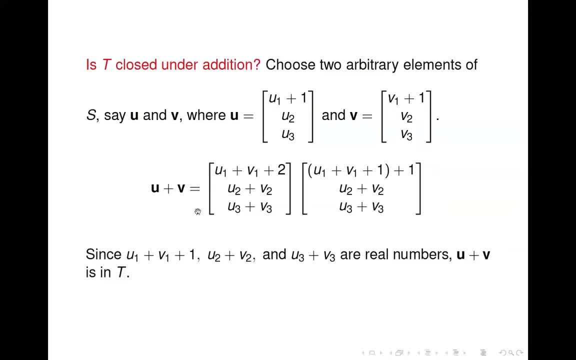 For the last two lines of the set. we only knew instantis max is looks like and when we add those together we get this vector. so just u2 plus v2 and the second component, u3 plus v3, and the third in the first, we get u1. 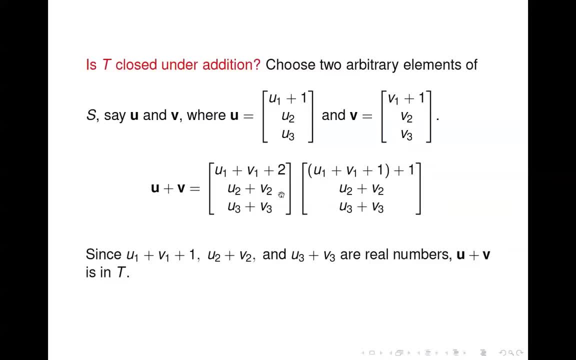 plus v1 plus 2. now you ask: is this vector in the set? and the answer is: well, it's not clear from looking at this whether it is or not. however, if we write it in this form: okay, then it's clear, because now you know this. obviously, the 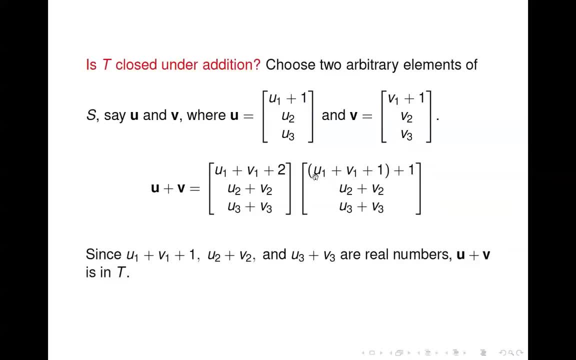 second two components are just real numbers, and the first one I, by, by factoring out a plus one and then gathering what's left here in parentheses. now this thing here, u1 plus v1 plus one, is a real number, and so now my first component looks like some real number. 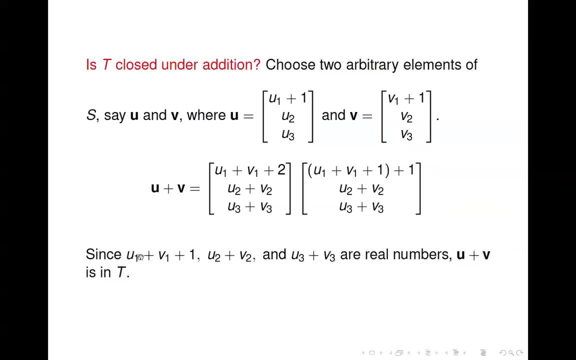 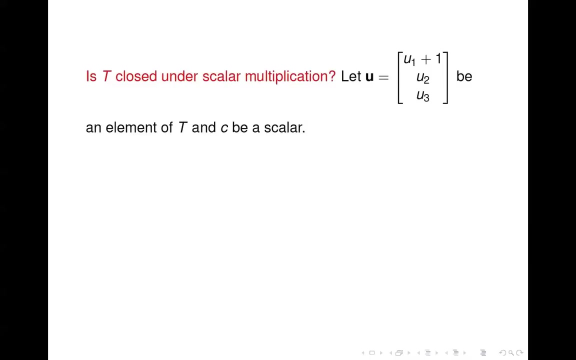 plus one, and so that's a real number. u1 plus v1 plus one is real, u2 plus v2 is real and u3 plus v3 are real. therefore, u plus v has to be in T or in S. sorry about that, so it's closed. under addition, we take a similar approach to show that it's. 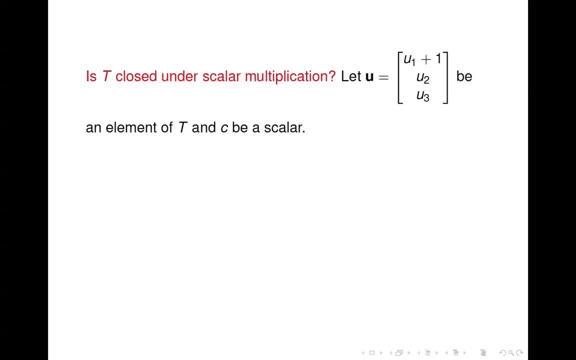 closed. under scalar multiplication again take a generic vector and a scalar multiply the 2, and again here I had to factor out that plus 1 so that I can make it look like the form that has to be to be in the set. and that leaves me in. 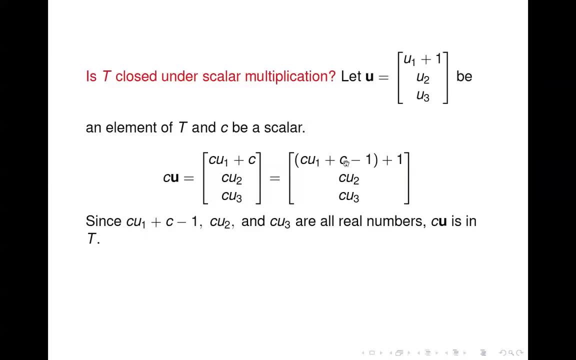 this case with this quantity here. but that's a real number, right? so see, is real, u1 is real, obviously 1 is real. so this quantity is a real number. so I got a real number plus one, and then the second two components are real, are clearly real numbers. that's what it takes to be in the set, so we can. 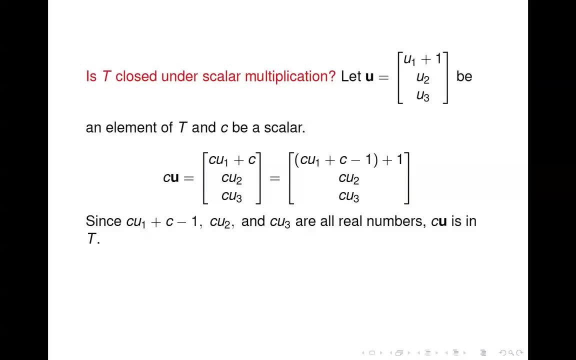 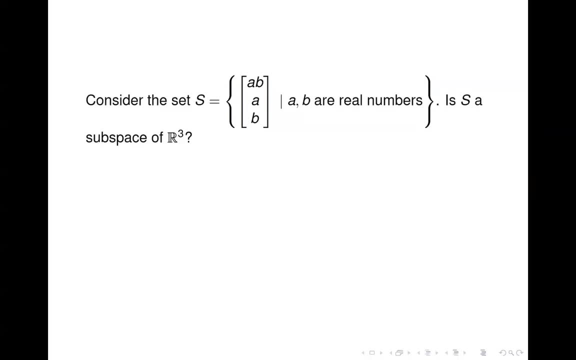 conclude that the set is closed under scalar multiplication and so it's a subspace of r3. another example: this one first glance looks like maybe you could use the theorem here, but it turns out that you can't with that: a times B in the first component. there's no way to break that up in a linear combination. 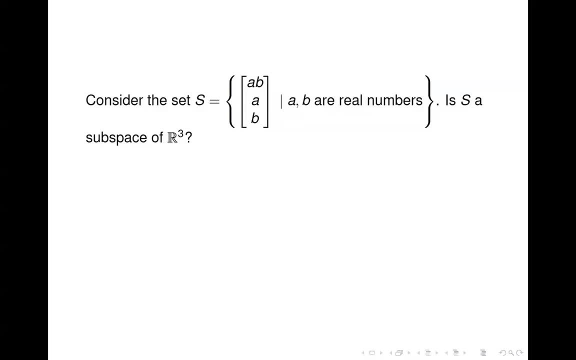 and so you this one. the theorem does not apply, and so we go back again to the original method and look and see: does this contain a zero vector? and clearly it does, because you can set a and B both equal to zero, and that gives you the zero vector. is it closed? under addition. 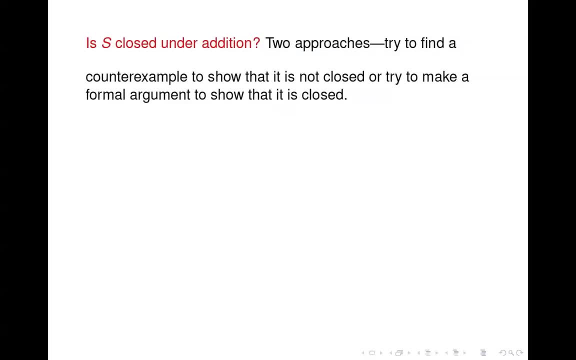 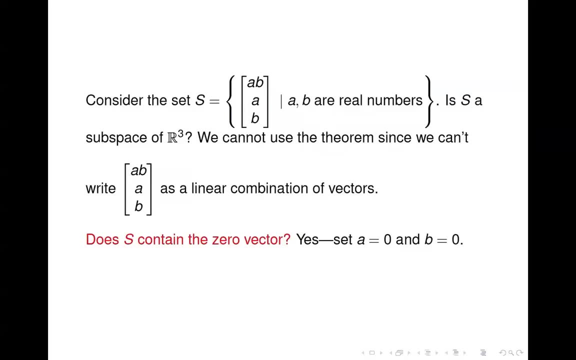 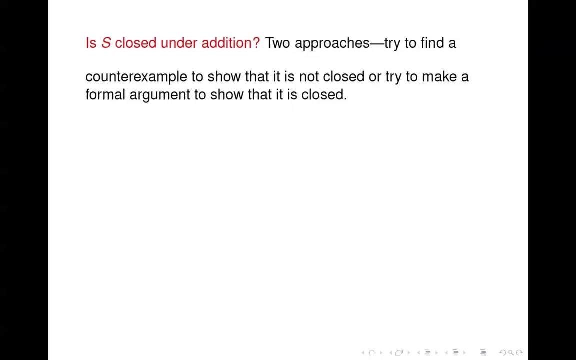 well, here let's go back and look at that set. maybe it's not clear just looking at that whether it would be closed under addition or not. you have to do some thinking, a little work, to arrive at a conclusion on that. so really there are two approaches you could take. one of them is to play around with the numbers. 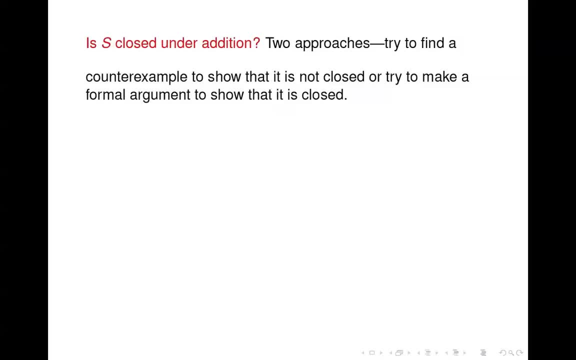 and try to find a counter example to show that it's not closed. so a counter example would be a specific example- okay, specific numbers that you plug in and show that the set is not closed. the other approach is to try to make a formal argument to show that it. 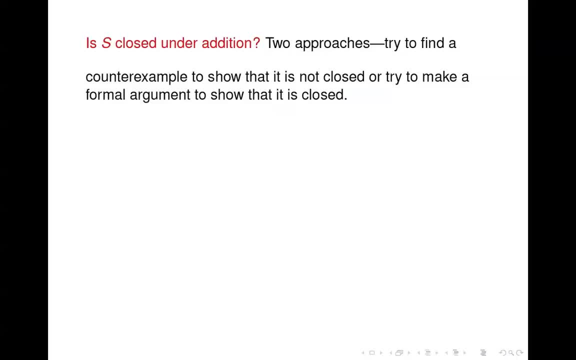 is closed. okay, and whichever one of these you pick really depends on the problem and whether you have some intuition one way or the other, and it also actually depends a little bit on your personality, would you? would you rather play around with the numbers and try to come up with a counter example, or would you rather? 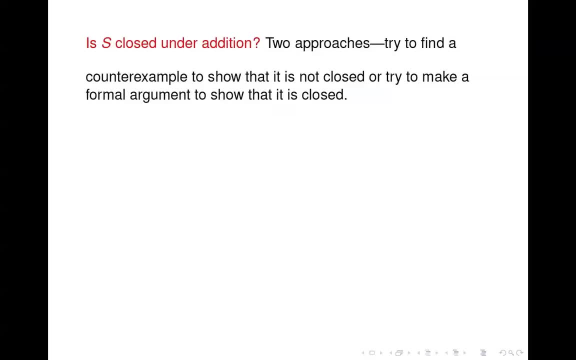 take a more straightforward approach, which is to try to show that it's closed, because a lot of times in that case you're trying to show that it's closed. you will either succeed or you will get to a point where you see why it's not closed, and so 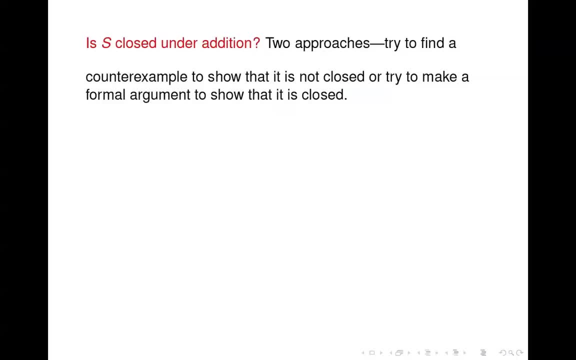 taking that route is a little more of a deliberate approach. playing with the numbers- try to find a counter example- is a little more of a random approach. but either either is valid and it kind of depends on us again, on your intuition, whether you have a gut feeling one way or the other and which you would. you 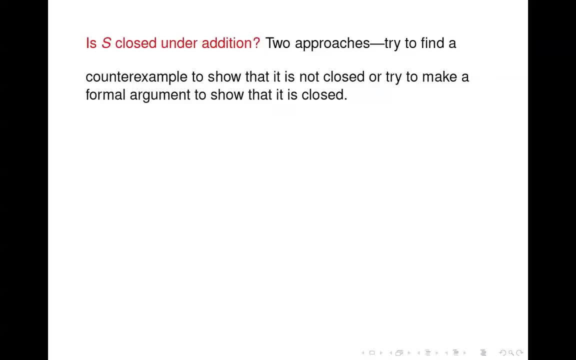 rather, do you know what, what you think is the better way to go with this one? I'm going to change the lateral approach because maybe I don't know. it's just not clear to me which you know, whether its closed or not closed. I don't have, maybe I don't have a 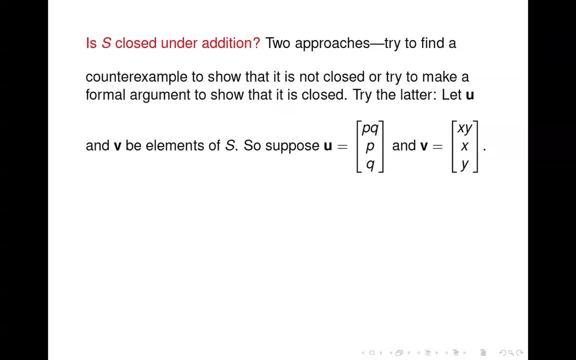 gut feeling on that. so I'm just going to take the safe, deliberate approach and try to show that it's closed and see where that takes me. so I picked two arbitrary elements from the set, these vectors I've written here P and U and V, and When I add them together I get this vector, and so what I want to know is if I multiply. 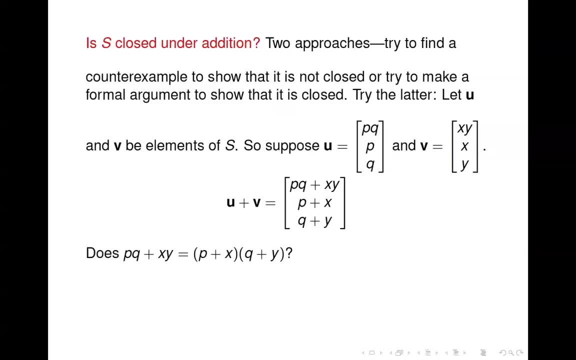 the second and third terms together, does that equal the first term right? So I'm asking, does first term PQ plus XY equal P plus X times Q plus Y? And as I look at that, I say, well, no. 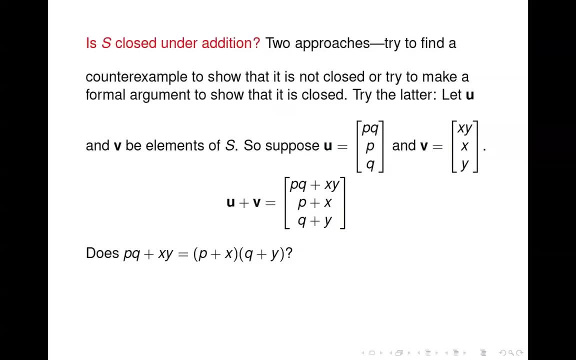 You know, sometimes it might, but in general, no, that does not hold. So that tells me, hmm, this is probably not closed under addition, and so I think I'm going to switch horses now switch gears and try to find a counterexample, right. 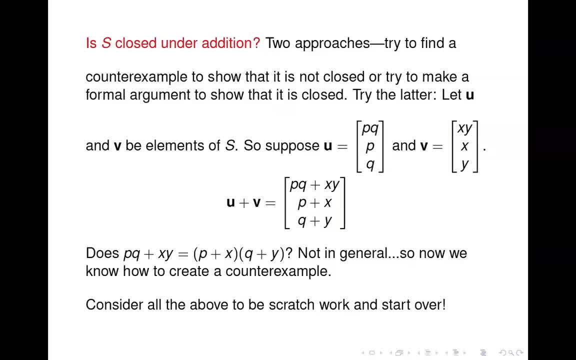 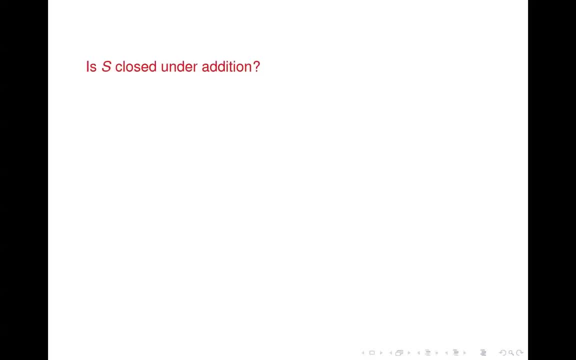 And so at this point you kind of scratch this out, consider that to be your scratch work, and you start over. okay, So start over here, and this time I'm going to try to find a counterexample. And so you know, my advice is: make life simple. 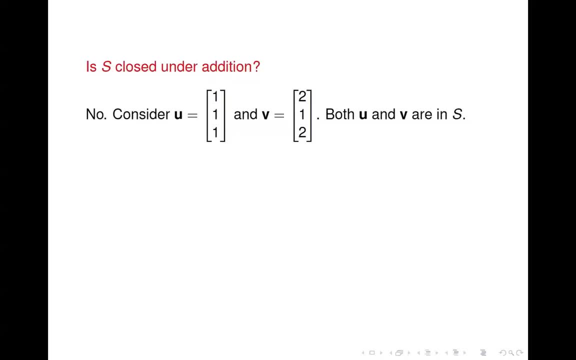 You know you can do a lot with just ones and zeros, So here I chose U to be 1,, 1,, 1, right. Second, two components are 1, multiply them together, you get 1, so that means first component. 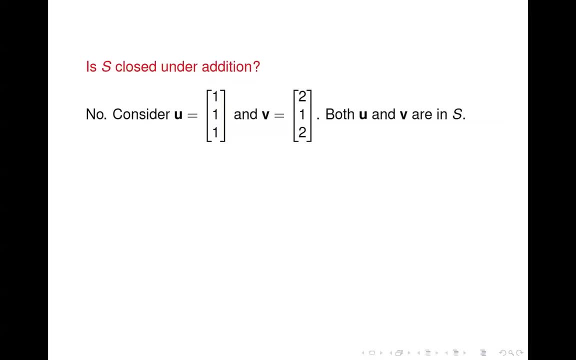 is 1. And V. I have 1,, 2, and the second and third components. multiply those together and get 2,, so the first component in V, V, has to be 2,. all right, So both these vectors are in S and I add them together and so I get this vector 3,. 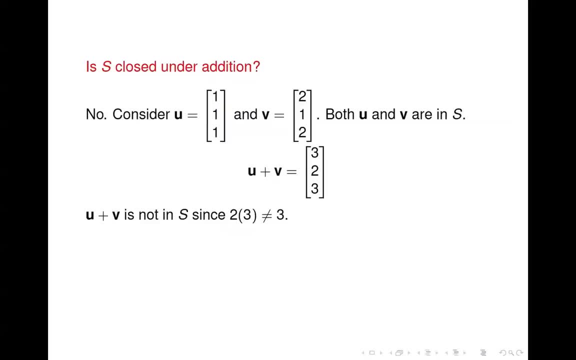 2, 3,, just adding component-wise U and V. And then I check: is this vector in S? And the answer's no, because when I multiply the second two components together 2 times 3,, I get 6.. 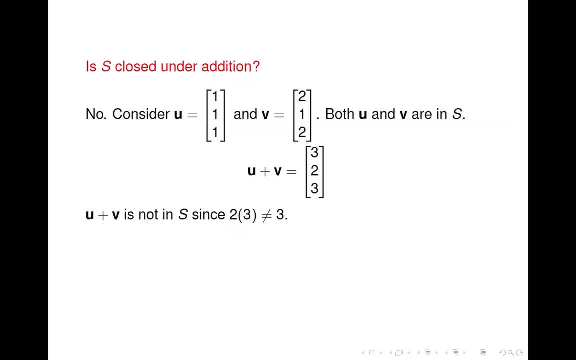 But my first component's not equal to 6. It's equal to 3. And so So this vector U plus V is not in S, So S is not closed under addition. Now, at this point we know that S is not a subspace of R3, but again for practice, 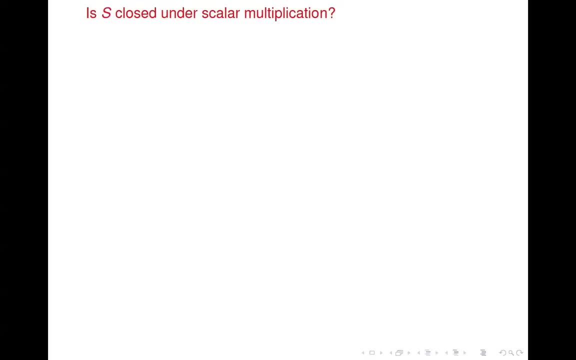 let's keep going and look and see: well, is it closed under scalar multiplication? And again you've got the choice which approach you want to take: find a counterexample or work on a formal argument to show that it is closed. 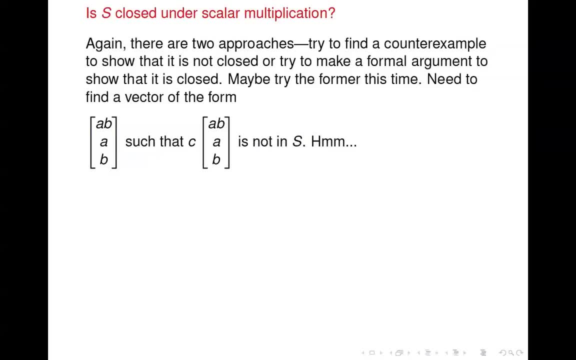 In this case I'm going to Let's think: hmm, you know it wasn't closed under addition, so I'm going to just bet that it's probably not closed under scalar multiplication. so I'm going to fudge around, see if I can. 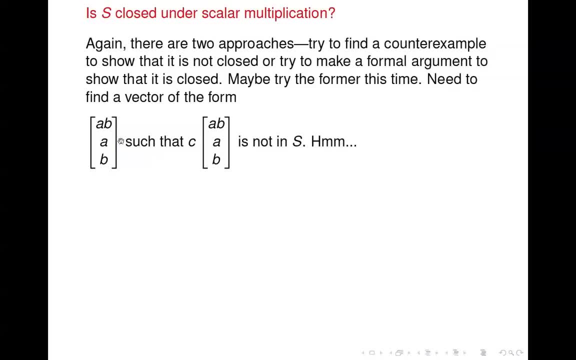 find a counterexample. So I need to come up with a vector that's of the general form and a scalar C, such that when I multiply C times the vector, I get one that's not in the set. This is a trial-and-error process. 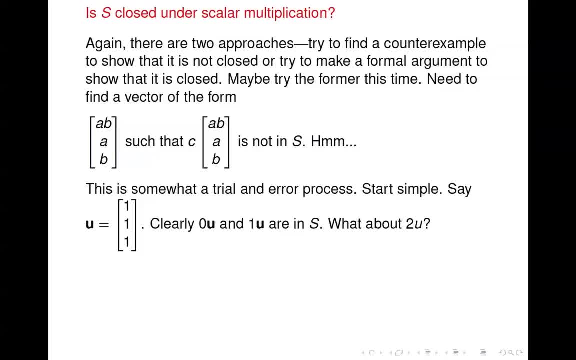 And again I would say: start simple Ones and zeros are good. Now, from before we know that 1,, 1, 1 is in the set because second two components one times one is equal to one, And so you know I might multiply by zero, but then I'm going to get 0,, 0,, 0, and that 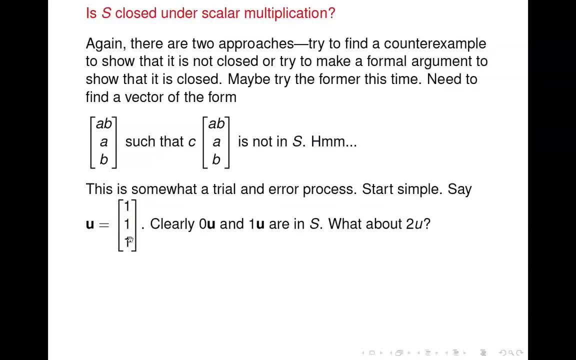 is in the set. Multiplying by one doesn't do me any good because that doesn't change the vector. I want something that's outside the set. So how about two? If I multiply two times U, I get 2,, 2,, 2.. 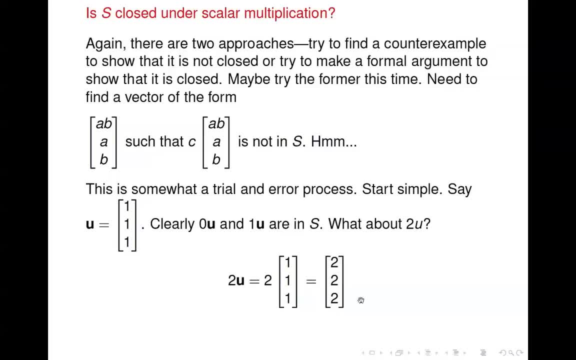 And then I multiply by one, I get 2,, 2,, 2.. And then I ask: is that in the set? And so you multiply the second and third components together. Two times two gives you four, but the first component is not four. 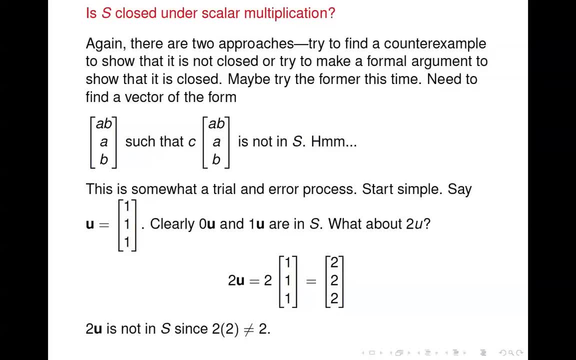 So, therefore, this vector is not in the set and we've shown that S is not closed under scalar multiplication. OK, and so now you have some examples, examples that you can apply this theorem on, and some examples that you can't. 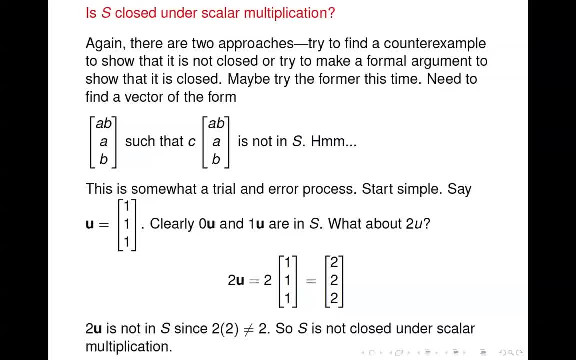 My advice is: you know to if you can apply that theorem, you want to, because it makes your life easier, much less work. If you can't, then you must go back to the original definition and show that the three properties either either show that they all hold or show that one of them doesn't hold. 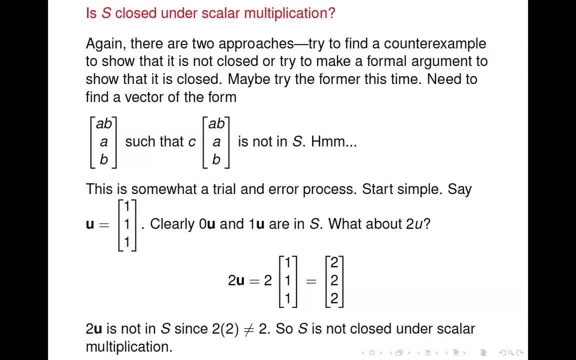 And when you're doing that, to show that, show that one of the properties holds, you must make a generic argument. you know, to show that a set's closed under addition or closed under scalar multiplication, you must make a generic argument. 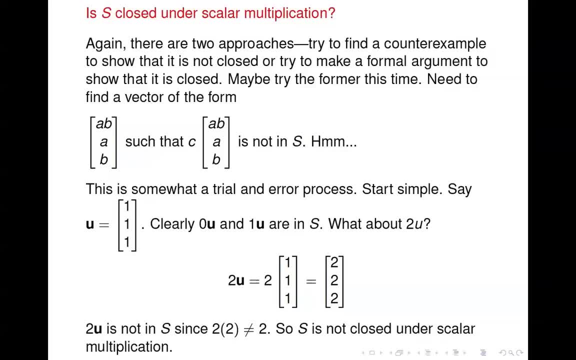 It's not sufficient to show that you can find two vectors that you can add together and get get one that's in the set. You have to show that that holds for any two vectors that you pick, and that means you must make a general argument to show that a set's not closed. 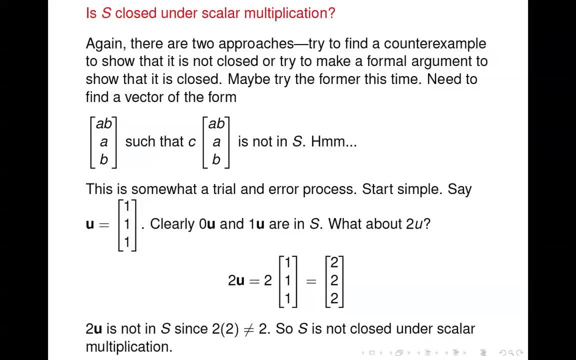 It's not sufficient to show that a set's closed under either addition or scalar multiplication. You need to find a counterexample, and a counterexample means come up with a specific example with real numbers, and by real numbers I mean actual numbers, just like this one, that's. 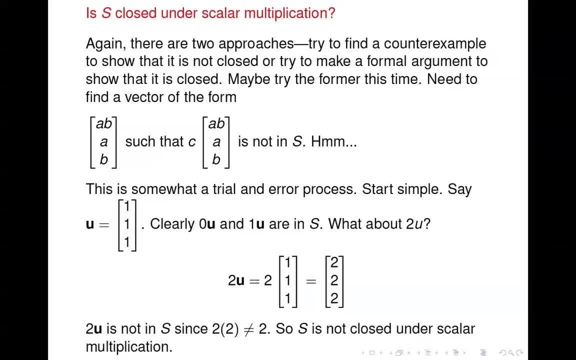 on your screen. now you know a specific vector, one, one one, a specific scalar, two. Multiply those together and see what you get and show that that's not in the set. Okay, So that's a counterexample. 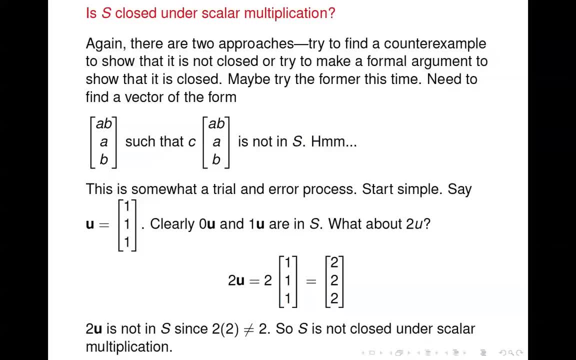 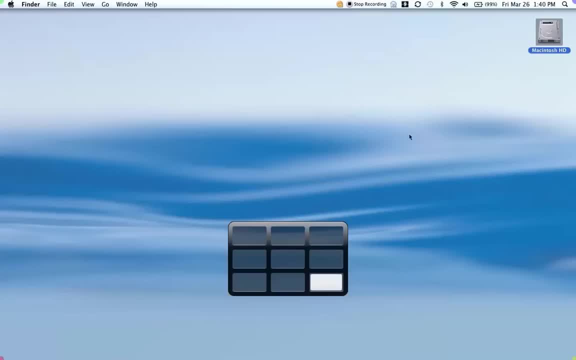 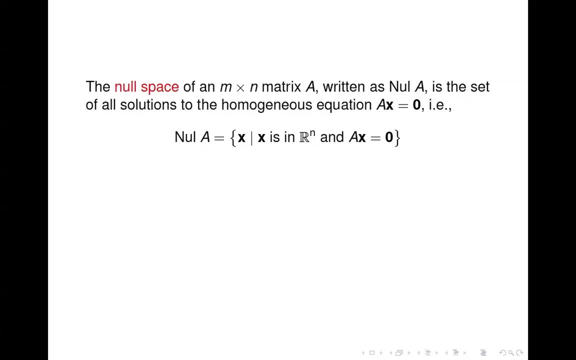 So to show that it is closed, make a general argument To show that it's not closed, find a specific example. In section 4.2, we're going to talk about a couple of concepts that we're not familiar with the terminology, but we are familiar with the concepts behind these terms. 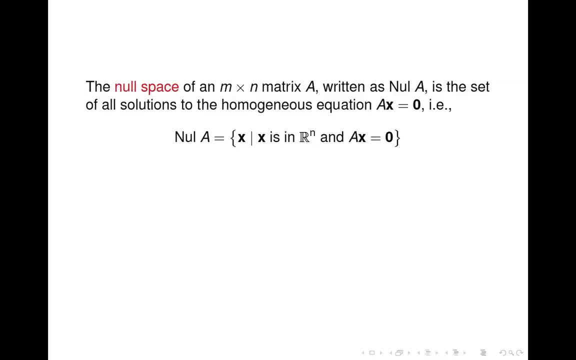 First of these is the null space of a matrix. We say the null space of an M by N, matrix A. written as null A is the set of all solutions to the homogeneous equation AX equals 0.. Okay, So null A is simply set of all X, such that X is in Rn and AX equals 0. 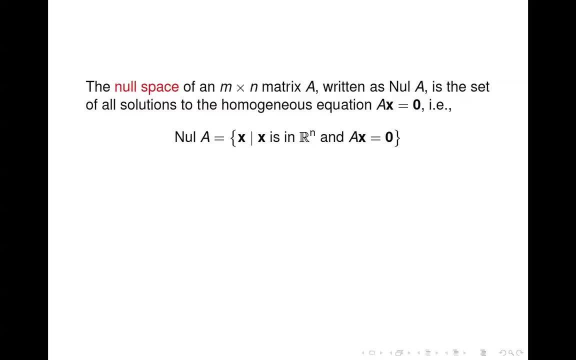 X has to be in Rn, because A is an M by N matrix and we want to be able to multiply A times X. Then there must be an entry in X for every column of A, and so X must be from Rn. 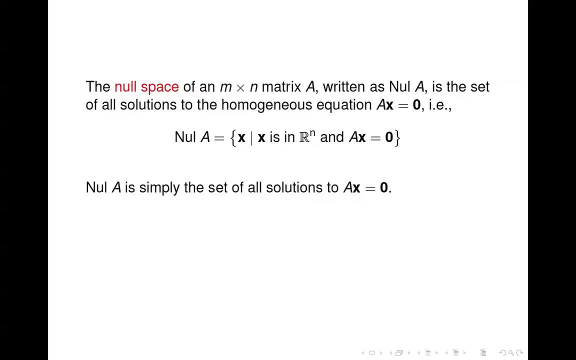 So null A is simply the set of all solutions to AX equals 0.. The fact that we're calling it the null space probably gives you a clue that it's a subspace, and indeed it is. The theorem here says: the null space of an M by N matrix is a subspace of Rn. 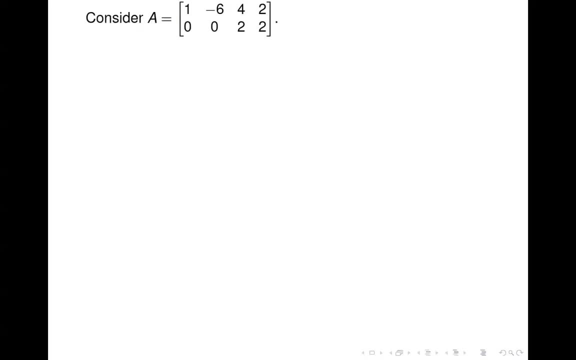 Okay, Let's look at this matrix A given here. To generate an explicit description of null A, we have to solve: AX equals 0, right, An explicit description means you can look at it and generate an entry in null A. Okay, 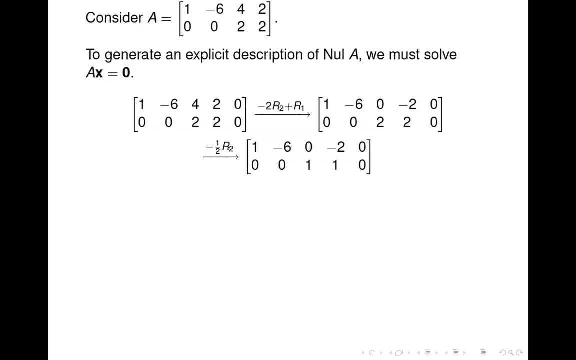 So to do that we have to solve: AX equals 0. So we throw that into an augmented matrix and do a couple of row operations giving us the matrix given here. So we see the general solution is X1 equals 6X2 plus 2X4, and X3 equals negative X4, and 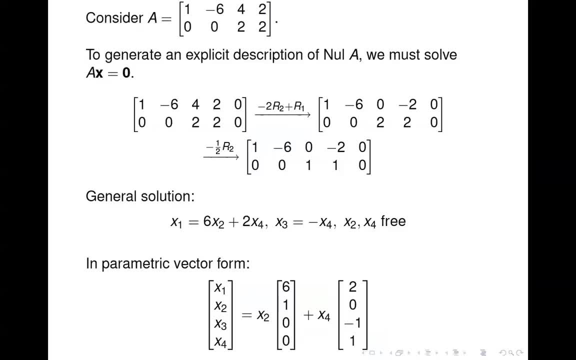 X2 and X4 are free variables. If we put it in parametric vector form, we have: X1 is 6X2 plus 2X4,, X2 is just X2, and so forth. So notice that any vector in the null space of A is a subspace. 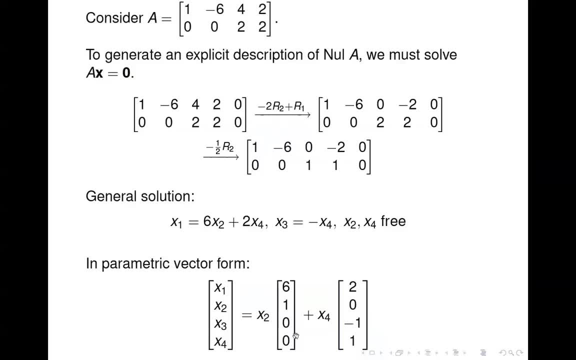 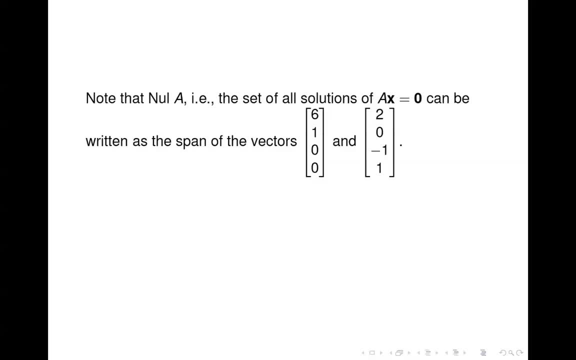 Okay, Any vector in the null space of A is a linear combination of these two vectors given here. So if we put those, if we look at those, we can say any vector in the null space of A is in the span of those two vectors. 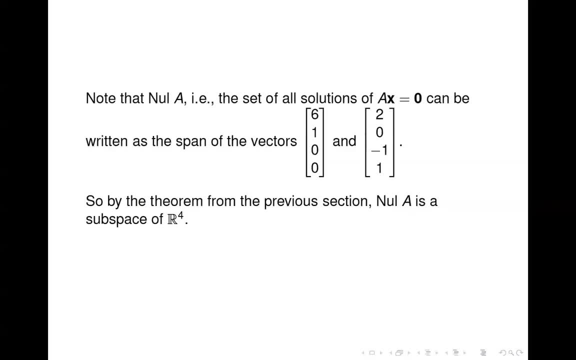 And if you remember the theorem from section 4.1, it said that if you can write your set as the span of a finite set of vectors, then it's automatically a subspace. So here we've written: for this particular matrix A, we've written a set of solutions. 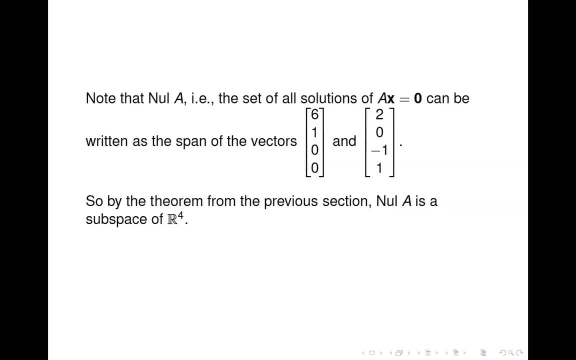 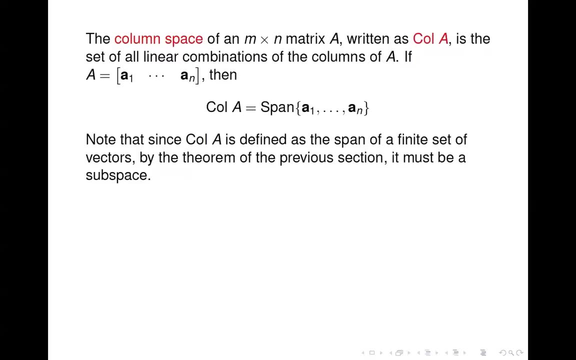 to AX equals 0 as the span of these two vectors. So therefore, the null space of A is a subspace of R4.. The second concept that we're going to talk about here in this section is the column space of a matrix. Okay, 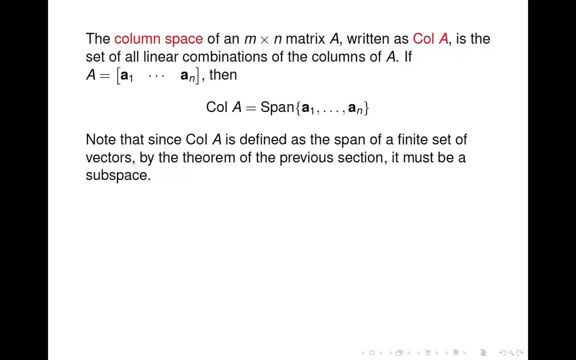 So once again it's new terminology but not new fundamental material here. The column space of an M by N, matrix A, which we write as col A, is the set of all linear combinations of the columns of A. All right, All linear combinations of the columns of A. We know that to be the span of the columns. 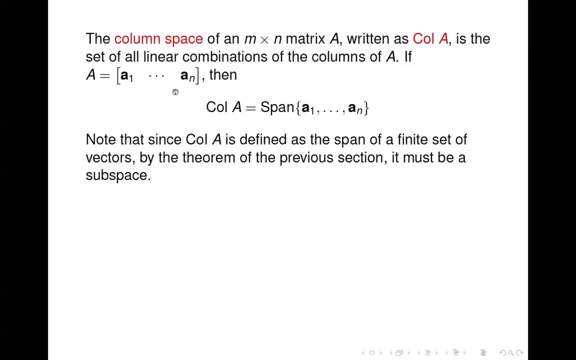 of A. All right. So if A is equal to A1 through AN, the column space of A is just the span of A1 through AN, And since we've the definition here is that column space of A is the span of a set of. 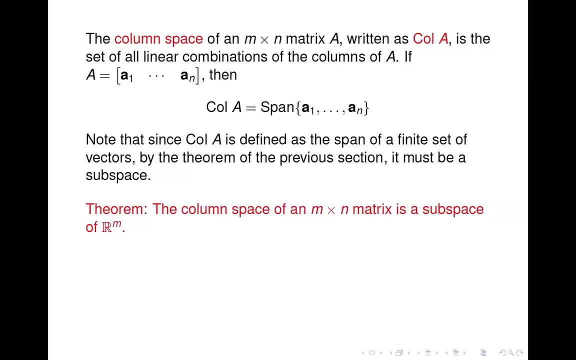 vectors. so it too is a subspace of some vector space. In this case, if A is M by N, then the column space is going to be in RM, because when you take a linear combination of vectors with M components, you're going to get a set of 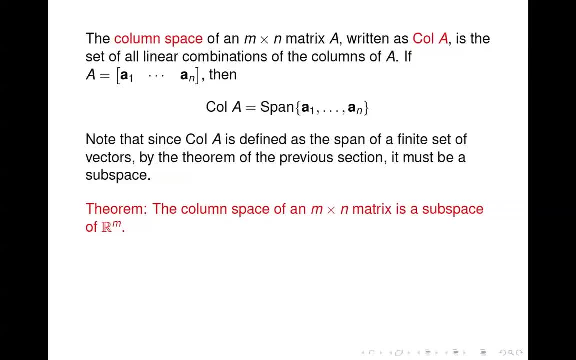 vectors with M components. Okay, So you're going to get another vector with M components, So the column space of A is in RM. Another way to look at the column space of A is to write it as a set of all B, such that 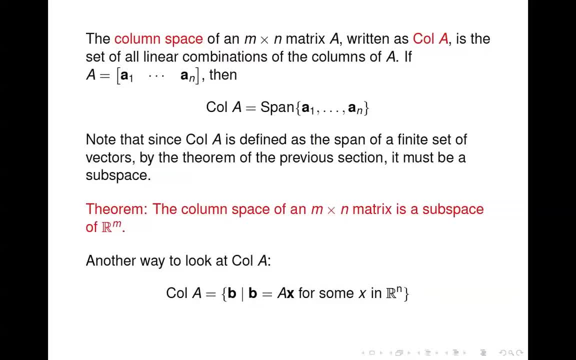 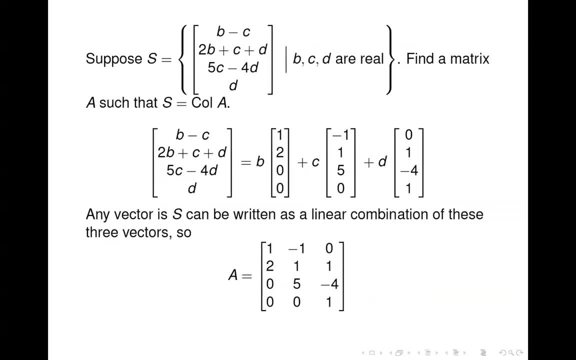 B is equal to A times X for some X in RN, Because when you multiply A times X, you're simply taking a linear combination of the columns of A. Here's a set S. Define that. Define it in terms of this generic vector. and you're asked to find a matrix A such that: 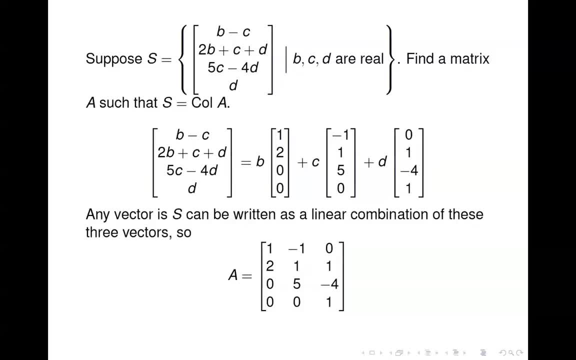 S is equal to the column space of A. So we simply take that generic vector, write it in parametric vector form so we can write anything in S as a linear combination of these three vectors given here. So if we put those vectors into a matrix then we can say that anything in S is a linear 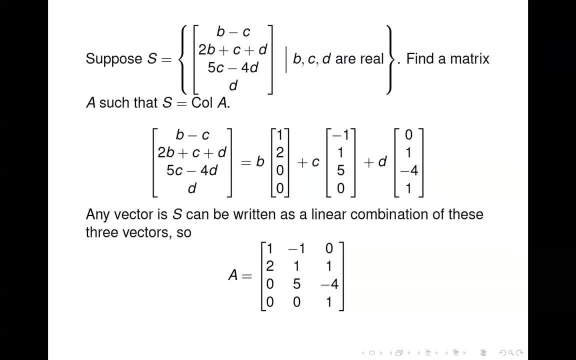 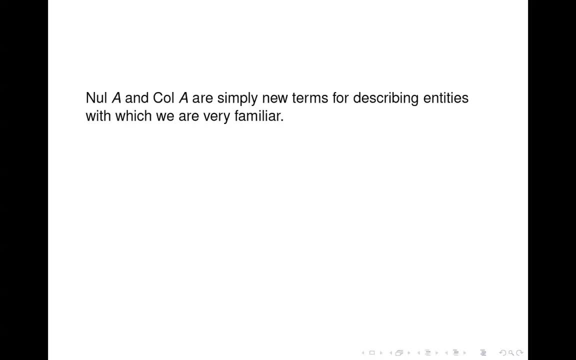 combination of the columns of A, And so S is equal to the column space of A. As I said before, the null space of A and the column space of A are simply new terms for describing entities with which we are already familiar. Null A is just the set of all solutions to AX equals 0.. 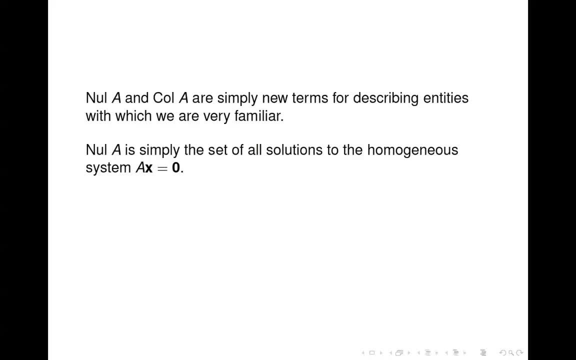 That dates back to section 1.3,, 1.4, or somewhere back there. A column space of A is just the set of all linear combinations of the columns or the span of the columns. So again we're going back to fundamental information that we learned in chapter 1.. 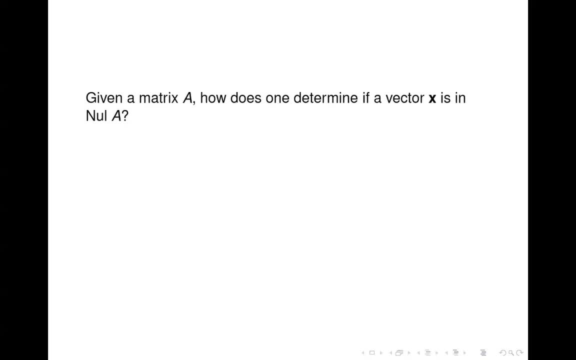 So if we have a matrix A, how do we determine if a particular vector, X, is in the null space of that matrix? Go back to the definition. Null space of A is the set of all vectors satisfying AX equals 0. So we just need to multiply A times X and see if we get 0. 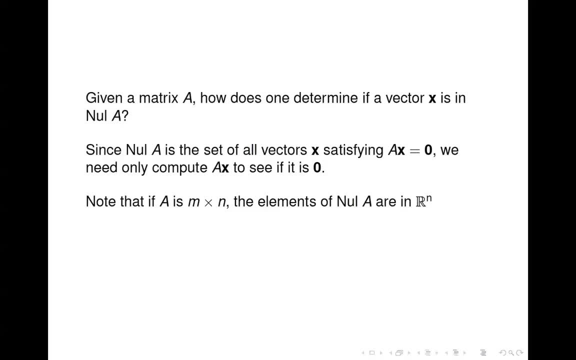 Again to multiply A times X. we're taking a linear combination of the columns of A, So there needs to be a component of X that corresponds to each column of A. There are n columns in A, So we need n elements in the null space of A. 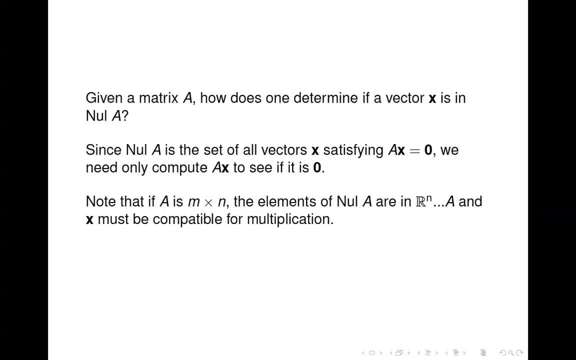 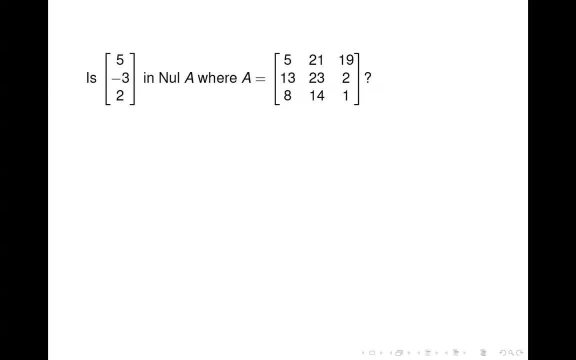 So null A is in Rn. So here's a vector and we're asked: is this in the null space of the given matrix? So we simply multiply the matrix times this vector, so that we're taking a linear combination of the columns here and go through the arithmetic and we end up with a 0 vector. 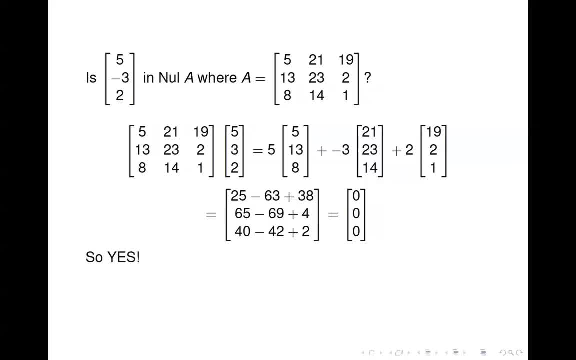 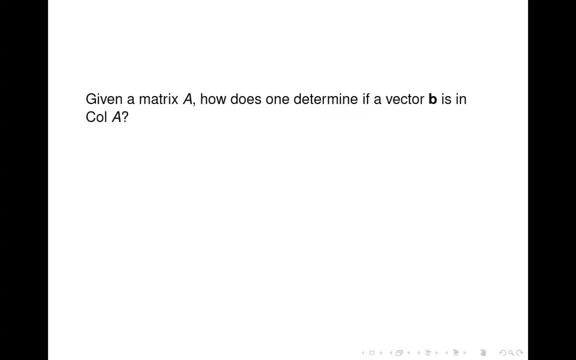 So the answer is yes, it is in the null space of A, Because A times X is equal to 0 here. All right, what if we have a matrix A and another vector and we want to know if that vector is in the column space of the matrix? 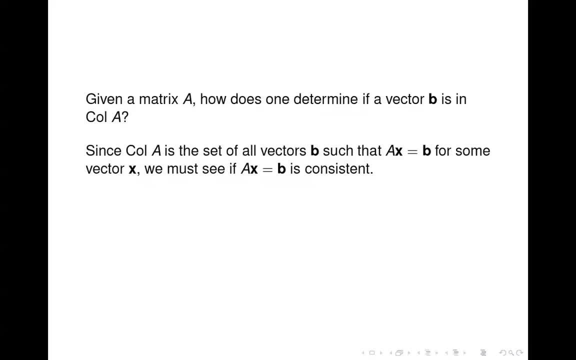 So again, look at the definition: B is in the column space of A if AX equals B is consistent. So we need to solve a system to determine if B is in the column space of A. And again, the column space of A is going to be a subset of our M because we're taking linear combinations. 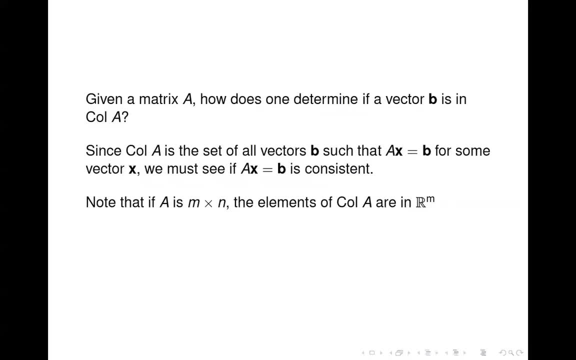 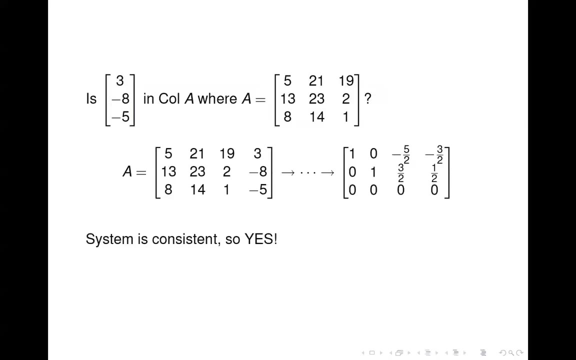 of vectors with M components, and so we get another vector with M components. All right, so here's a vector and we want to know if it's in the column space of A for the given matrix A. So we need to solve the system, set up the augmented matrix, solve. 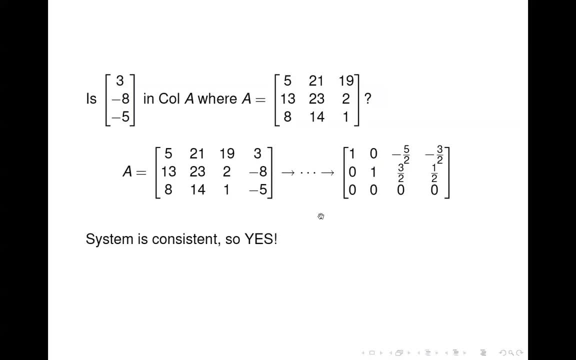 the system. So I've done that, left out the specifics, the row operations, but we end up with this matrix here, And so the question is: does this correspond to a consistent system? And the answer is yes, because we have no rows: 0, 0, 0, something not 0.. 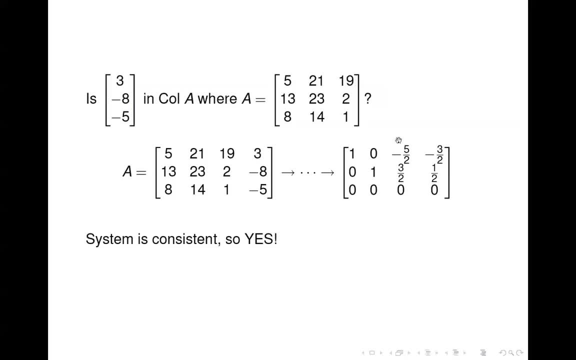 The fact that we have a row of all 0s is really irrelevant. The fact that we have a free variable is irrelevant. The only thing that's relevant is that we don't have a row that's 0,, 0, 0, not 0.. 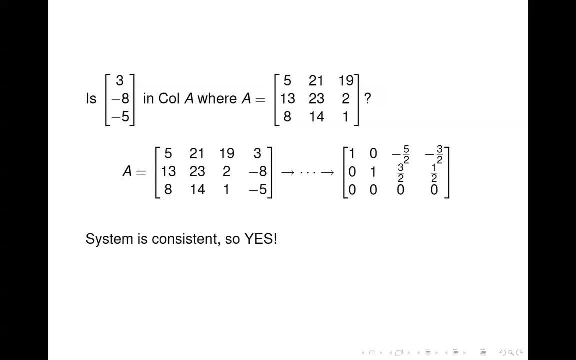 Because that would tell us it's inconsistent. So, since the system is consistent, that means that this vector is indeed in the column space of A. All right, let's look at this example. Here's the set W and we're asked: is it a subspace of R4?? 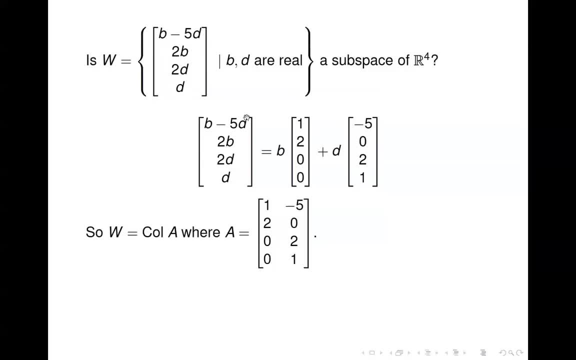 So we can write it, write any generic element of W as the linear combination of these two vectors. So we write it in parametric vector form And so we can say that W is equal to column space of this matrix, just taking these two. 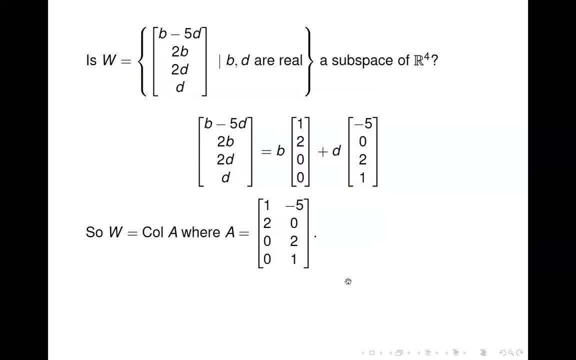 vectors, sticking them in the columns of a matrix. The column space of this matrix is all linear combinations of these columns, which is exactly W. So that means that W is a subspace. All right, how about this example? This one: 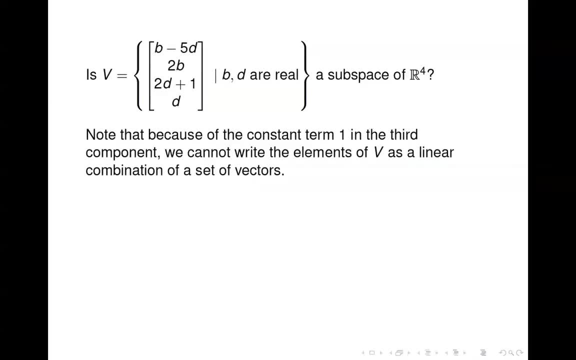 It's not so easy or so clear to see, because we have this constant term 1 here And so we can't write this set as a linear combination of vectors. So in this case we have to go back to the definition of subspace. 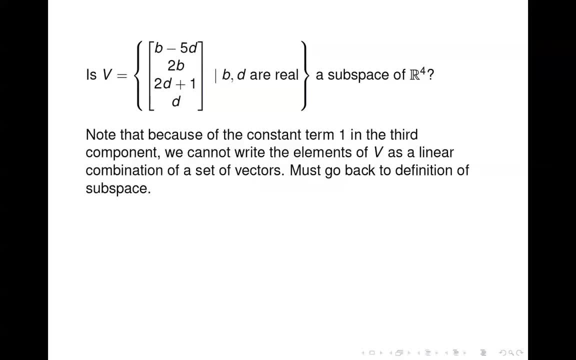 That's, those three properties that every subspace must have Satisfy. So first one was: does it contain the 0 vector? And if we look for it to contain the 0 vector, clearly d has to be 0, which would mean that 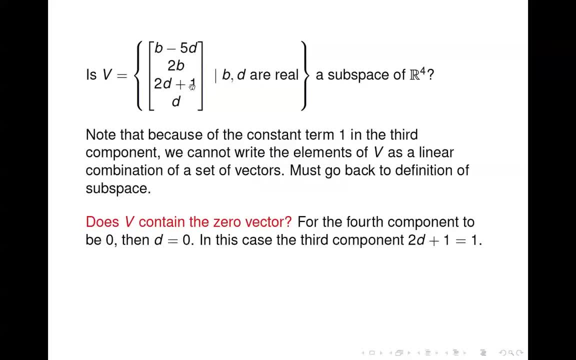 the second component would be 2 times 0 plus 1, which is 1.. And so if you get 0 here, you're going to have 1 up here, and therefore the 0 vector is not in this set. So it is not a subspace of R4.. 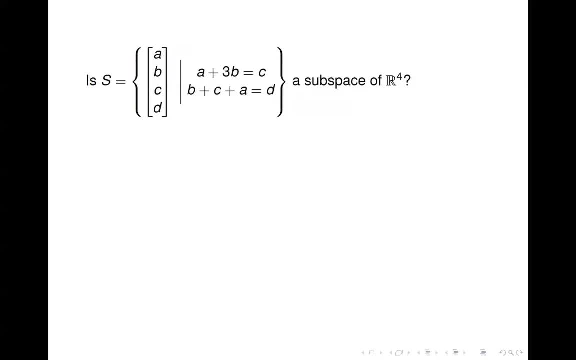 About this set. is this set a subspace of R4?? So we've got all vectors a, b, c, d that satisfy these two equations. There's actually two ways we could go about doing this, using what we've learned in this. 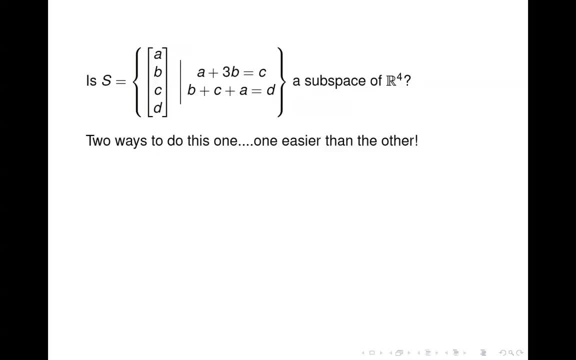 section One is easier than the other. Yeah, So we're going to do the hard way first And we're going to try to write s as the column space of some matrix A. So we need to figure out what A would be. 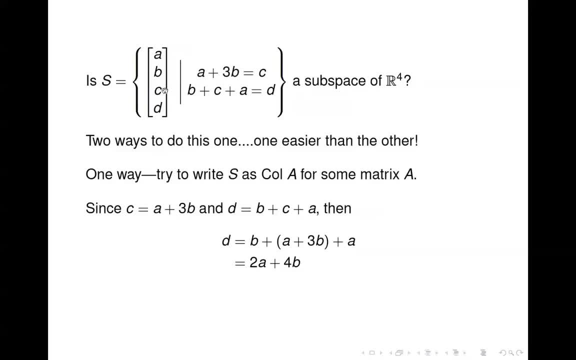 We're going to simplify things a little bit: Instead of c here we're just going to substitute a plus 3b, And then, instead of d, we're going to substitute a plus b plus c. but we're going to plug in. 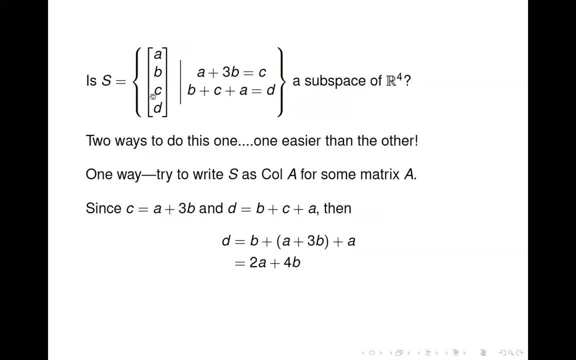 what c is, Since we're going to substitute a plus 3b, Since we've gotten rid of c. So d is b plus c plus a And c is a plus 3b. So plug that in for c And we end up with d equals 2a plus 4b. 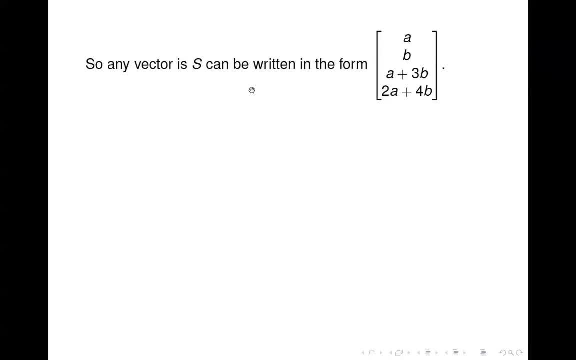 So we can write any vector in s in this form. So we replace c with a plus 3b and d with 2a plus 4b, And then it's just a matter of writing that in parametric order. So we're going to substitute a plus 3b and d with 2a plus 4b. 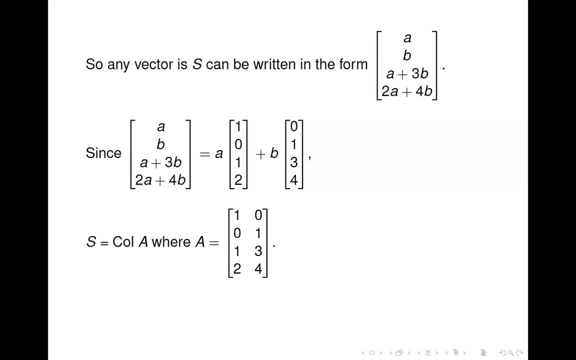 And then it's just a matter of writing that in parametric order. So we're going to substitute a plus 3b and d with 2a plus 4b, So we can write any vector in parametric order. So we can rewrite that in parametric vector form and throwing those columns into a matrix. 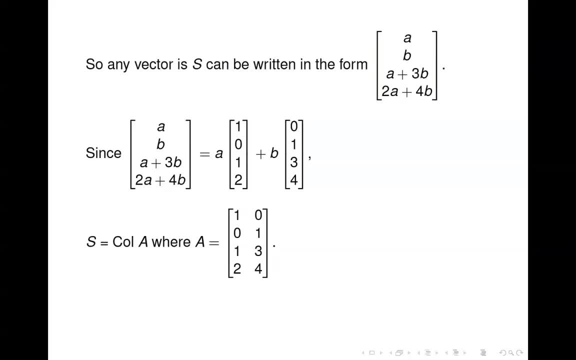 And so s is equal to the column space of a, where a is given here, And thus s would be a subspace of r4,, since the column space of any matrix is a subspace. Now the other way to look at it. 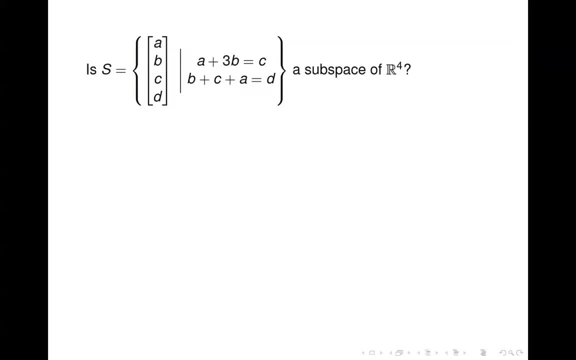 So I rewrite the problem here. The other way to look at it is to note that we could write s in this form. So, basically, I've taken these two equations that we have here and I've taken all the variables over to the left side, and so we've got zeroes on the right. 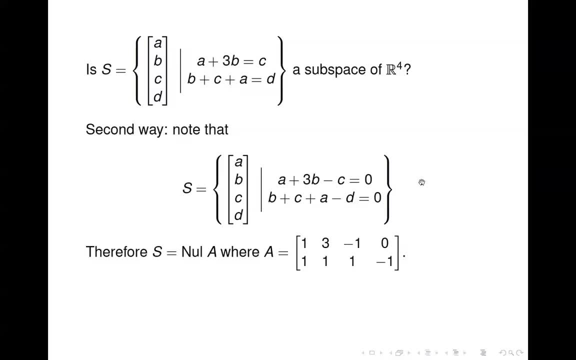 And so when you see zeroes on the right you should think that's a homogeneous system. And so we can write S as the null space of A, where A is equal to the coefficient matrix from this system of equations. So you see 1, 3, negative, 1 for A, B, C and then zero for D, and from the first equation, 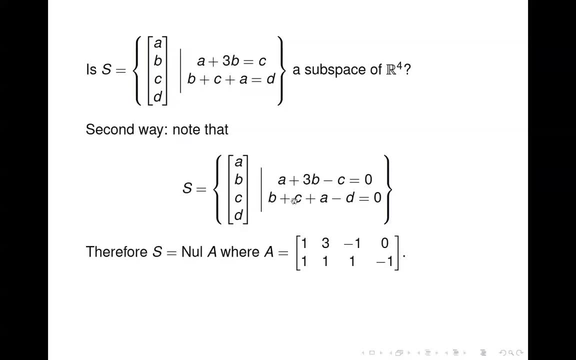 and then the second equation: we get 1 times A plus 1 times B, plus 1 times C minus 1 times D. so that's where this second row comes from. So remember what the null space of a matrix is. it's just the set of all solutions to. 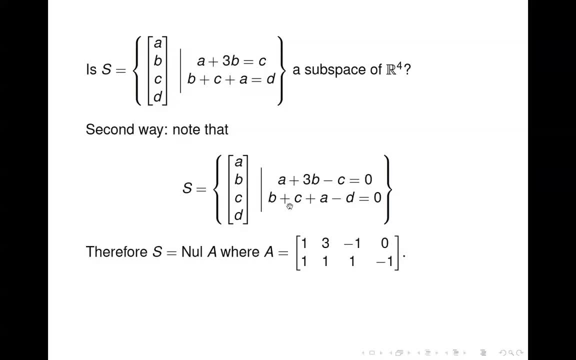 AX equals zero, and so I've just taken this system of equations, written it, or taken these two. I've taken these equations, written them as a homogeneous system, and then I can use the fact that the null space of a matrix is always a subspace, and we're done. 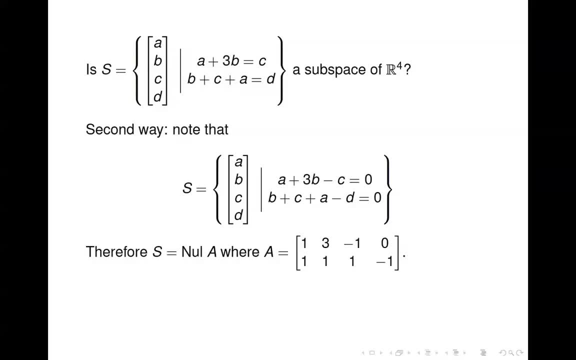 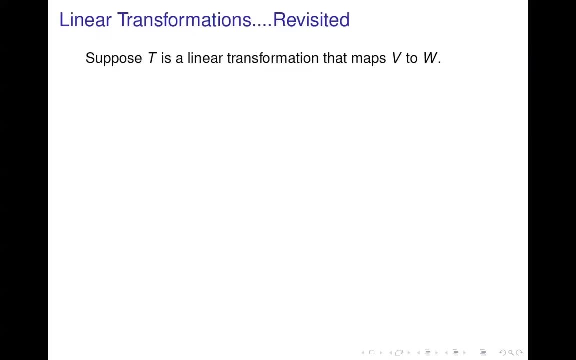 So that's why I said one was harder than the other. this is clearly the easiest way. Alright, let's revisit the concept of linear transformations for just a bit, And this is again back to chapter 1, where we talked about linear transformations. One new term that we didn't learn back in chapter 1 was the idea of the kernel of a. 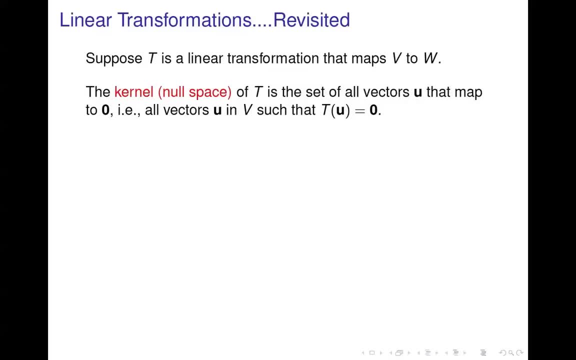 linear transformation. and the kernel of a linear transformation is simply the set of all vectors that map to the zero vector. so the kernel of a linear transformation is exactly the null space, the null space of the matrix that defines the transformation. So kernel and null space are analogous concepts. 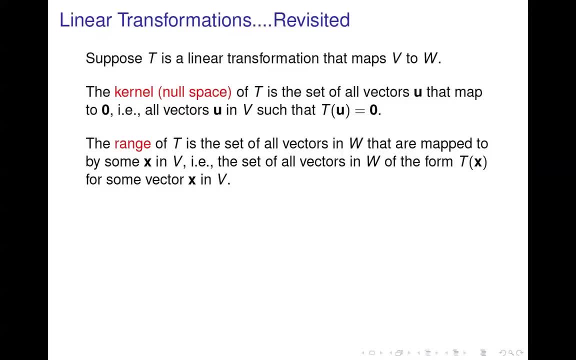 The range of a transformation is the set of all vectors that get mapped to. So the range is in the codomain. sometimes it's all of the codomain, sometimes not, but the range is the set of all vectors that get mapped to by some vector from the domain. 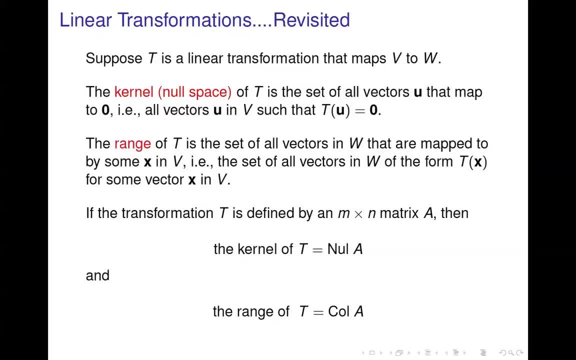 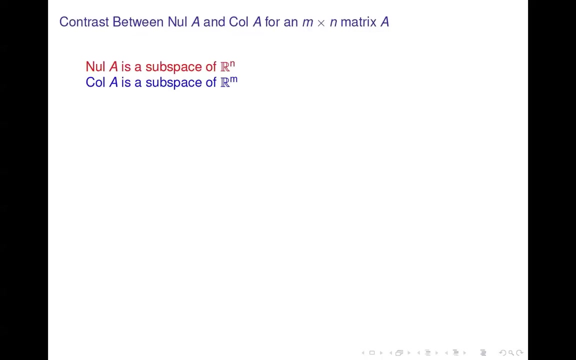 And so the range of T is actually the column space of A, where A is the matrix that defines the transformation. So the kernel of the transformation is the null space of A, the range of the transformation is the column space of A. Okay, last I want to talk about just looking at the contrast between the null space of 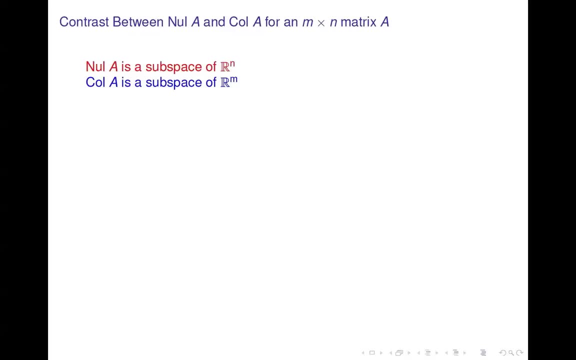 a matrix and the column space. These really on the surface are very different sets. We will kind of pull them together a little bit later on in this chapter, but for right now they're really very different sets and they don't share. They share analogous sorts of ideas, but that's kind of the extent of it at this point. 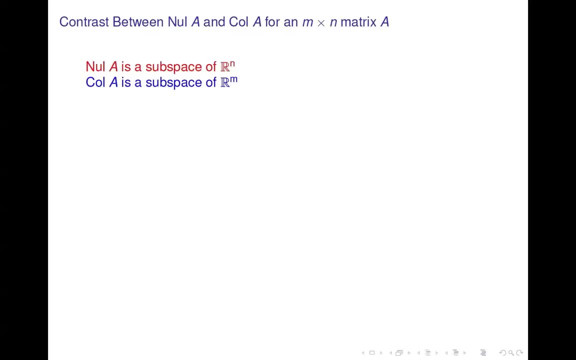 So let's assume A is an M by N matrix, Then the null space is in Rn, column space is in Rm. The null space is implicitly defined. that means you're given a condition that vectors in the null space must satisfy, but you can't look at a matrix A and know which vector. 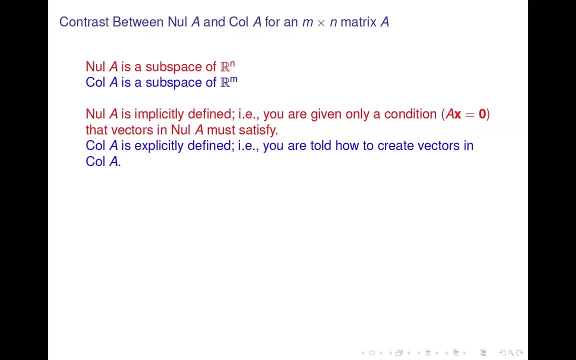 vectors are in it. You have to solve that system. AX equals 0.. On the other hand, the column space of A is explicitly defined because it's just the set of all linear combinations of the columns. So you can look at the matrix A and you know that the columns that you're looking at are. 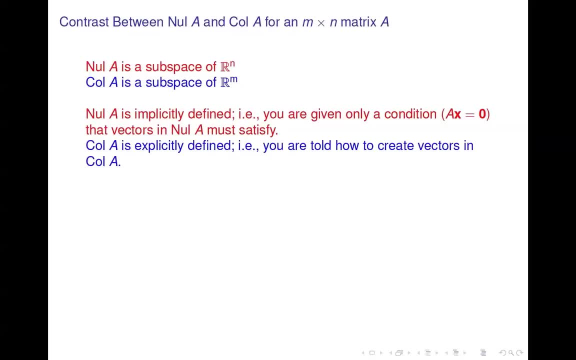 actually in the column space and you know how to create more entries in the column space. To find vectors in the null space requires work. You have to solve the system. AX equals 0. Okay. Note, however, that the 0 vector is always in the null space of A right because A times. 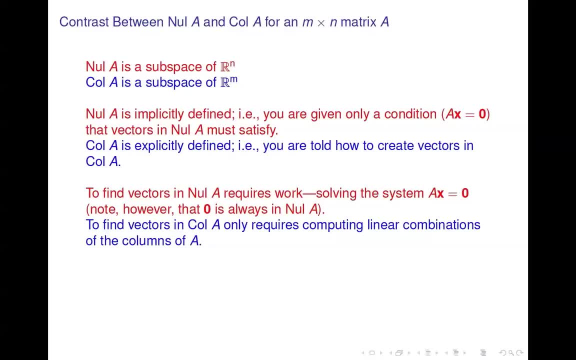 the 0 vector gives you the 0 vector To find vectors in the column space of A. you just compute linear combinations of the columns, So it's a direct process to do that. There's no obvious relationship between null A and the AX. 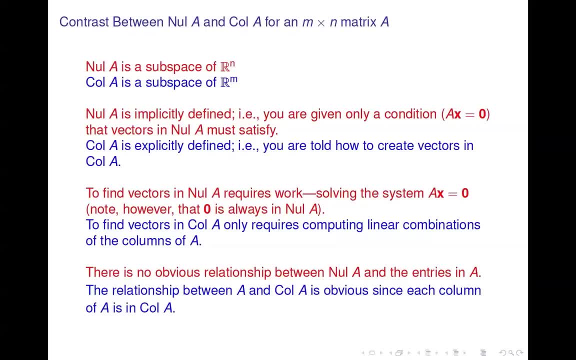 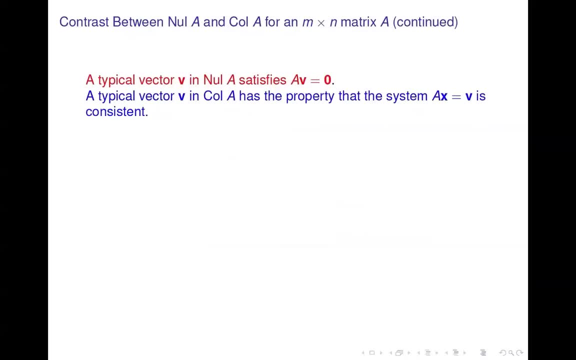 In the entries in A. on the other hand, the relationship between A and the column space of A is obvious, since each column is in the column space. The typical vector V in the null space satisfies: A times V equals 0.. Typical vector in the column space has the property that AX equals V is consistent. 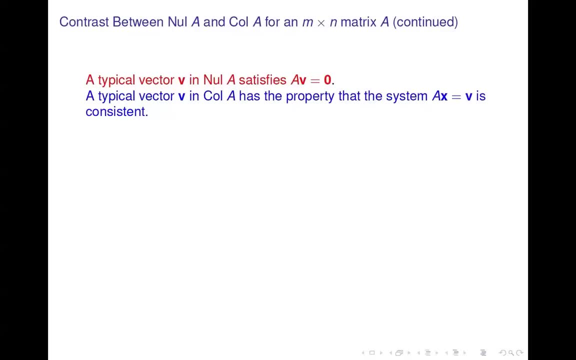 Okay, So for null space, Um, You're multiplying A times V to see if you get 0.. To see if a vector's in the column space, you're solving a system: AX equals V, So V's on the right hand side in that case. 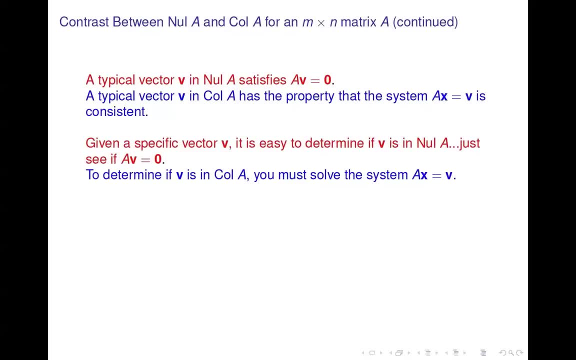 Given a specific vector, V, it's easy to determine if V is in the null space. You just see if A times V is equal to 0.. To determine if V is in the column space, you have to solve a system of equations. 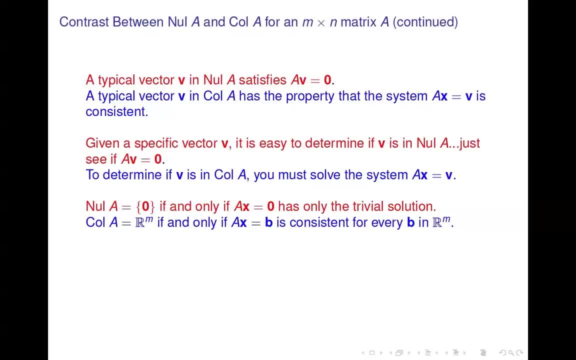 Alright, The null space equals 0.. The column space equals only the 0 vector. um, if, and only if, AX equals 0 has only the trivial solution. Okay. So how do you get what's in the null space? We have to solve AX equals 0.. 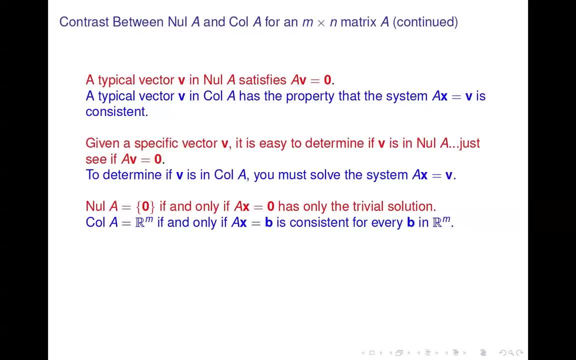 And if you get only the trivial solution, then that means there's only one solution, which is a 0 vector. The column space of A is equal to RM if, and only if, AX equals V is consistent for every B in RM. Alright, 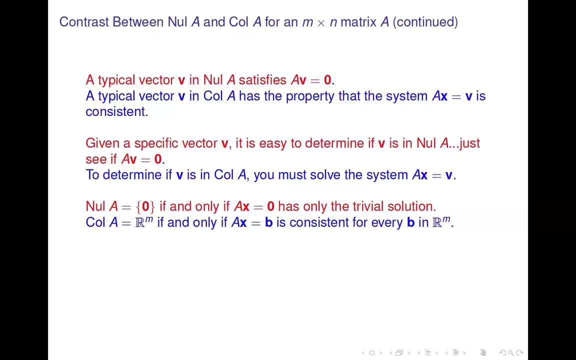 So that means that everything, uh, no matter what you put on the right hand side, uh, the system will be consistent. So every B is a linear combination of the columns of A And then, relating it to uh linear transformations, the null space of A is equal to the 0 vector. only if and only. 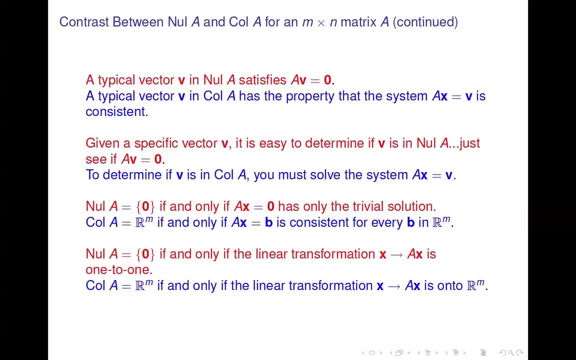 if, uh, the transformation X to AX is 1 to 1.. So if you back up to the previous one, uh, we had uh that uh, null A is equal to X. So we have to solve the 0 vector only if, and only if, uh, the transformation X to AX is. 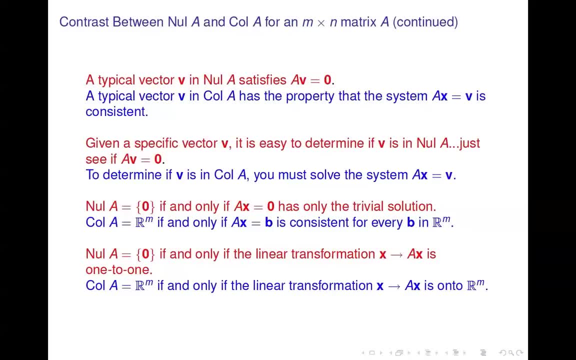 1 to 1.. So if you back up to the previous one- uh, we had, uh, that, uh, null A is equal to 1 to 1.. So if you back up to the previous one, uh, the transformation X to AX is 1 to 1.. 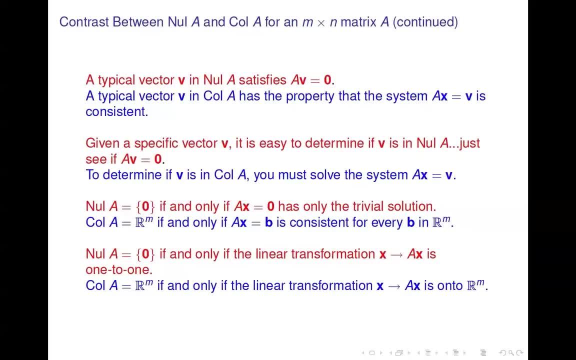 If null A is equal to only the 0 vector, if AX equals 0, has only the trivial solution. remember that's going to occur- uh when you have no free variables and uh, or if there's a pivot position in every column. 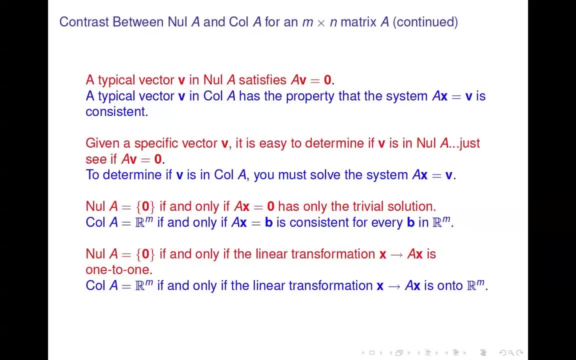 And so we know that indicates that that the transformation is 1 to 1.. And then the column space is equal to RM if, and only if, uh, AX equals B is consistent for every B, So that means every B in the co-domain gets. 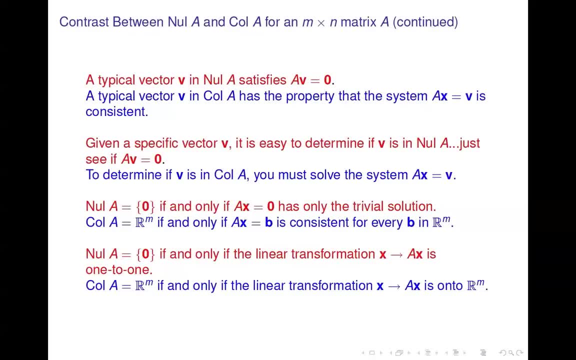 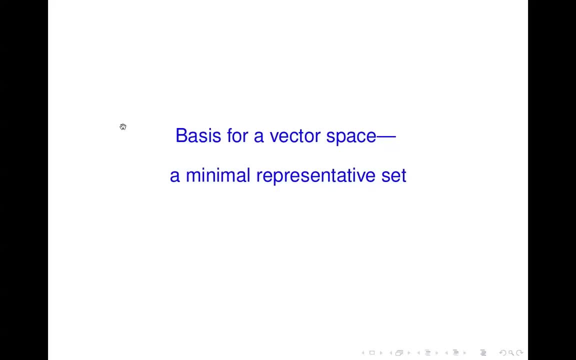 mapped to, so the transformation must be on to RM. okay, we're going to start today talking about a basis for a vector space, and the idea of a basis is that it's a minimal in terms of number of vectors and representative in that it represents the vector space set. so it's a minimal representative set. so let's 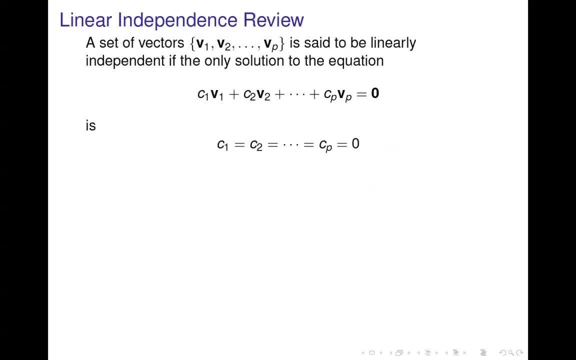 explore what that actually means. before we really get into that, let's back up a little bit and remember what a couple of concepts are that are key here. one is linear independence and the other is spanning. so let's start with linear independence. so here's the definition: a set of vectors- v1 through VP, is said to be linearly independent if 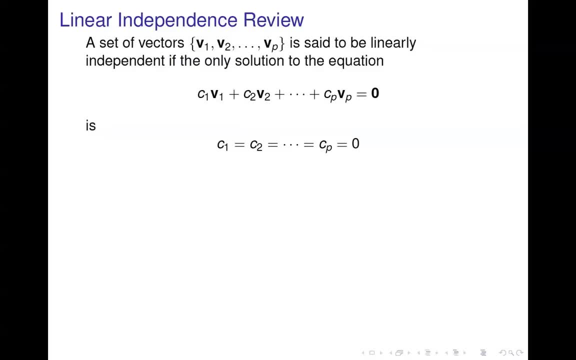 the only solution to the equation. we take a linear combination of the vectors and set it equal to zero. okay, this linear combination set equal to zero. the only solution to that is when you set all the coefficients equal to zero. note that this is always a solution. we can always. 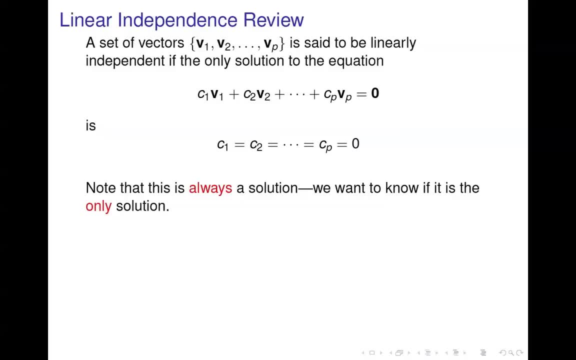 set the coefficients equal to zero and generate the zero vector. what we want to know is if this is the only solution. so, thinking in terms of the systems, of the system of equations, we know the system's consistent. we want to know if this, the solution, is unique or if they're an infinite number of solutions. 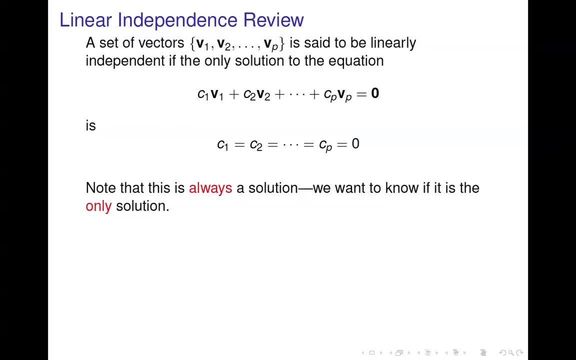 so that's when we get into talking about free variables. does the system have a free variable or not? okay, so we set up that augmented matrix for that system, we put in echelon form and we want to see if they're free variables. right, because we're free variables, that means an infinite number of solutions and the 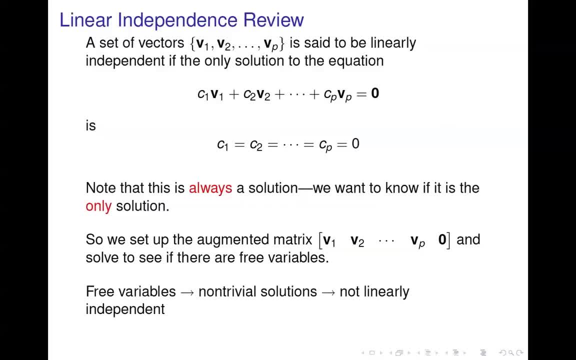 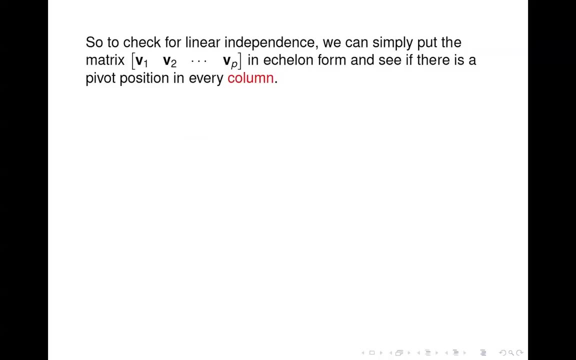 and the vectors would not be linearly independent. and if we don't have free variables, that means the solution is unique, so the vectors are linearly independent. okay, so to check for linear independence, we we really don't have to tack on that, that zero column on the augmented side. we can just look at the. 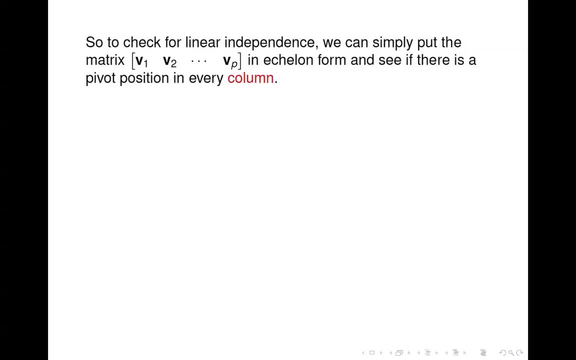 coefficient matrix, put it in echelon form and see if there's a pivot position in every column. okay, because we want to know: are there free variables or not. so is there a pivot position in every column? okay? there are a few cases that are obvious. one is where you have more vectors than 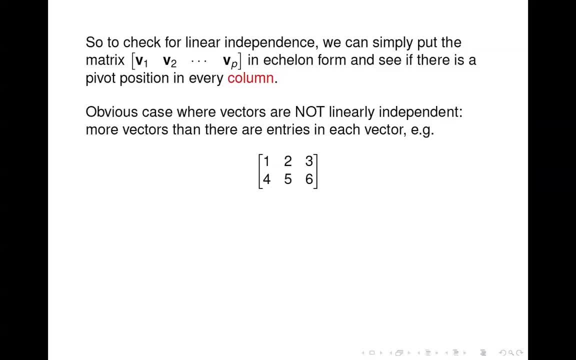 you have entries in each vector, like this matrix given here, these the three vectors could not be linearly independent. because you have three vectors in R2, there's no way you can have a pivot position into each column if you just have two vectors. they're linearly independent if neither is a multiple of. 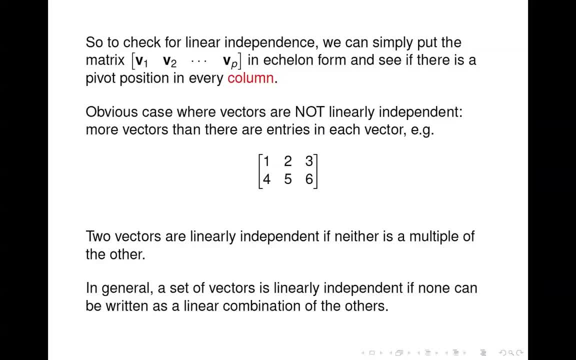 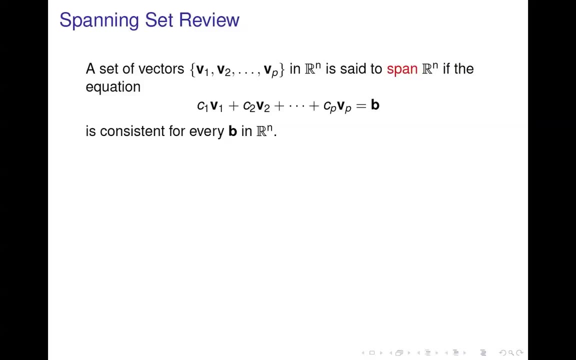 the other and in general, a set of vectors is linearly independent, if none. okay, I can't find any of the vectors in the set that can be written as a linear combination of the others. all right, let's move on to spanning sets. take that same set of vectors, V1 through VP, and assume they're in Rn and they are. 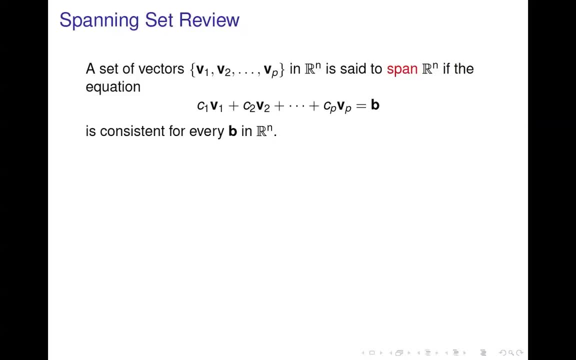 said to span Rn. if the equation- we take a linear combination of those vectors and set it equal to B- is consistent for every B in Rn, okay, that means you can take a linear combination of those vectors and generate any vector in Rn. now, obviously we can't solve this system for every B and 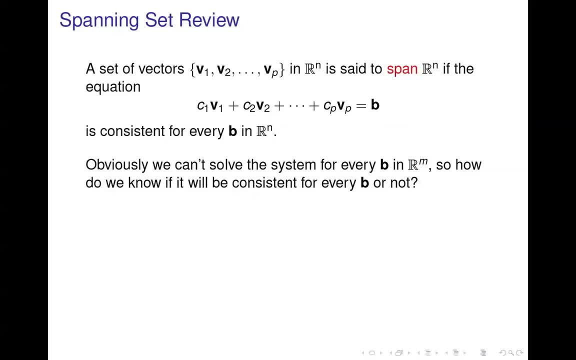 Rn should be Rn, Rm. so how do we know if it's going to be consistent for every B or not? right, then the linear independence, right hand side, with zero, we can solve that system. but here we want it to be consistent for every B. okay, so we can't. 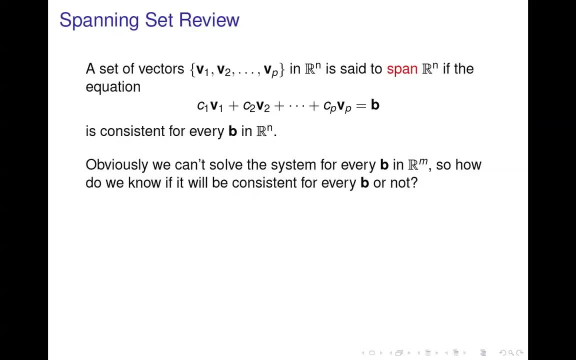 go and plug in every possible vector B on the right and solve the system to see if it's going to be consistent for everyone. so what do we do? well, we know that it will be consistent if we never end up with a row where we've got. 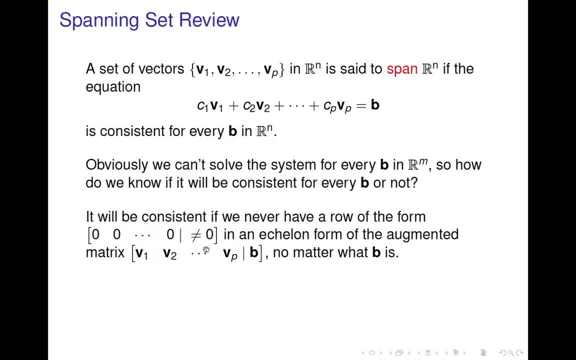 all zeros and then something not zero on the right hand side in when we put the matrix in echelon form, right. so if we have this, okay, we're all zeros and something not zero, then it's inconsistent. so we want to know if we never get that in the way. 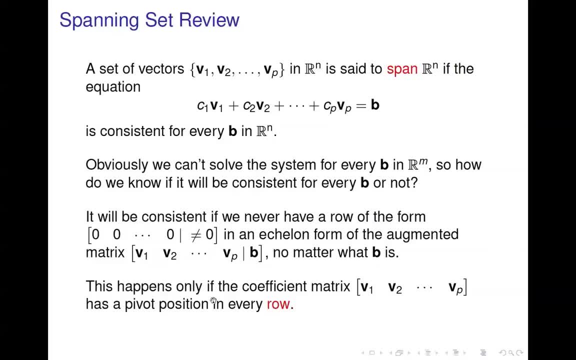 that happens is we have a pivot position in every row, right, there's a pivot position in every row of the coefficient part of the matrix. okay, then you'll never end up with all zeros in a row of the coefficient part of the matrix. so this, the sort of check to see if a set of vectors is linear, is spans, whatever. 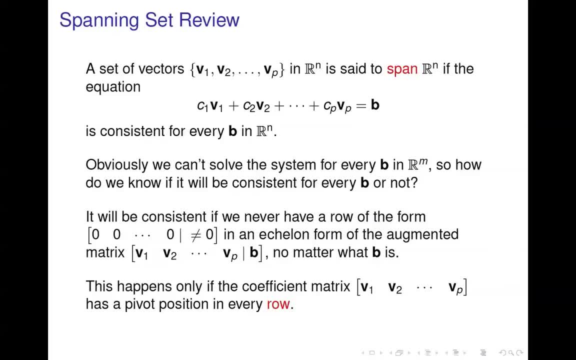 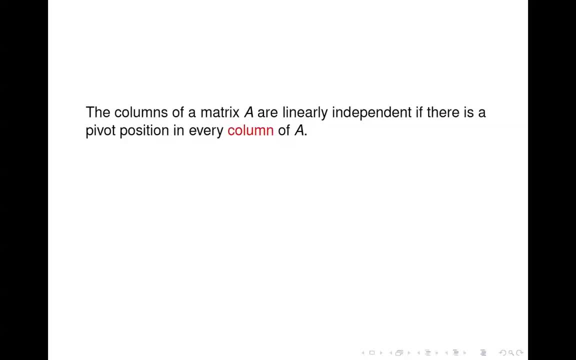 vector space they're in. we need to have a pivot position in every row. okay, so the columns of a are linearly independent if there's a pivot position in every column of a and they span our M if there's a pivot position in every row of a. yeah, it's assuming a is an M by N. matrix of the columns are in our M all. 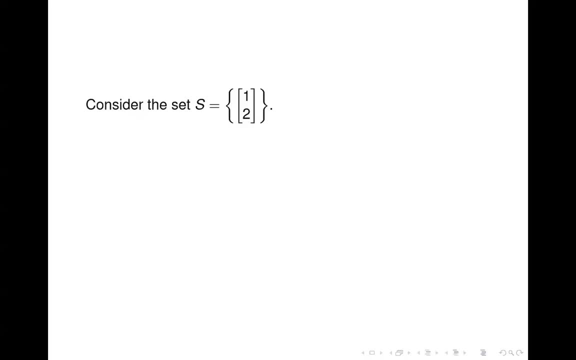 right, so let's look at some examples. here's a set with just one vector. okay, so let's look at some examples. here's a set with just one vector. okay, so let's look at some examples. here's a set with just one vector. okay, so let's. 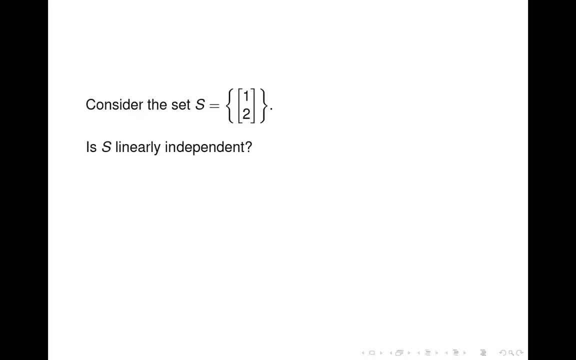 is it linearly independent? and the answer is yes, because you have a single nonzero vector is always going to be linearly independent, right? the only time just a single vector is linearly dependent is if that vector is the zero vector, okay. does this set span R2? and the answer is no, because if you look at 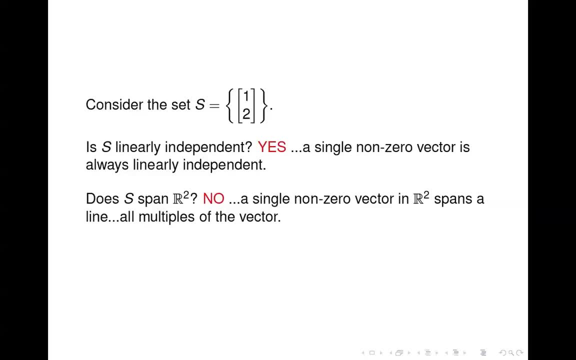 linear combinations of that vector. you're just getting multiples of that vector which is a line in r2, so you only get a line, not all of our two. it's all right. let's look at this set T. now I've got three vectors and first let's ask: is: 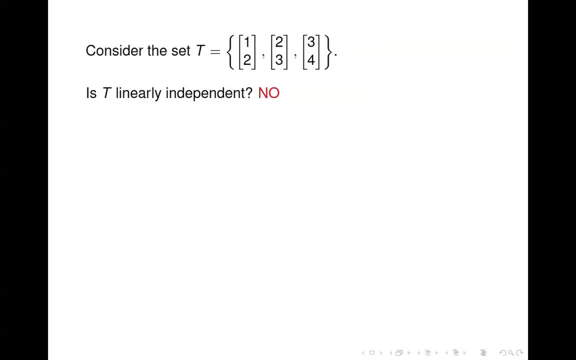 T linearly independent? and the answer is no, because you've got more vectors than there are entries in each vector, right? so if you put those vectors in a matrix there's no way you can have a pivot position in every column. this does the set span r2. yes, because you just even look at the first two vectors, they are: 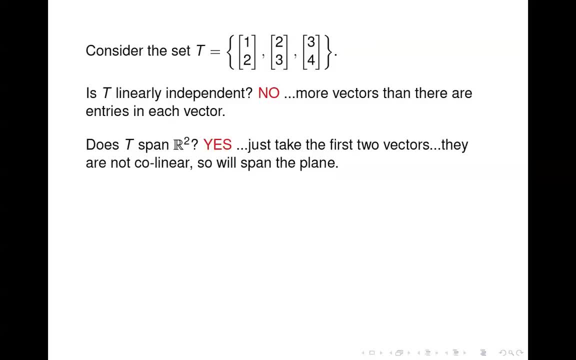 not multiples of each other and so not collinear, so they will span the plane. now, if you want to go back and just look at it in matrix form, take those vectors, put them in a matrix, put it in echelon form and look and see. do you have a pivot position? every column, 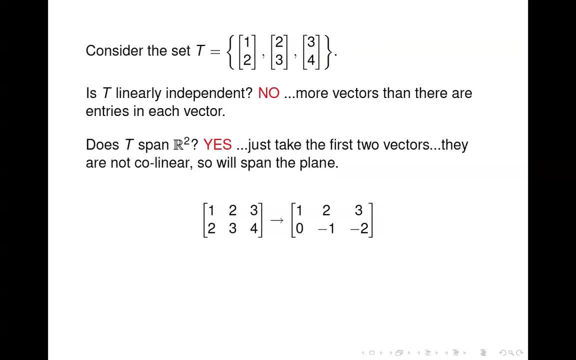 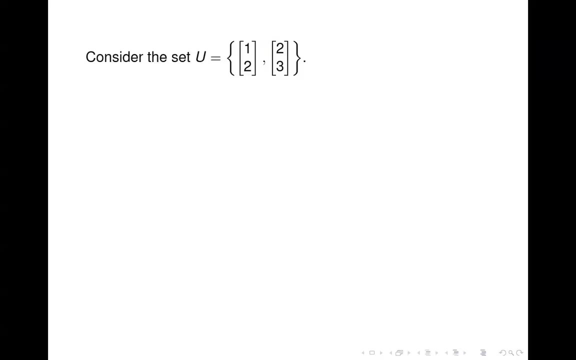 no, so they're not linearly independent. do you have a pivot position in every row? yes, so they do span r2. ok, now let's look at one more set. now, this one is like the other one, except I just took out that last vector. so again, is it linearly independent? yes, it's. 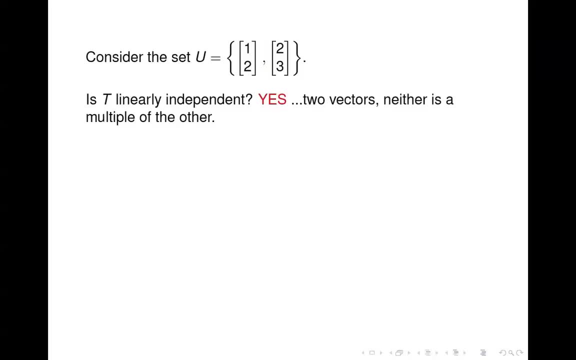 we've got two vectors and neither is a multiple of the other, so they're linearly independent. so span r2. you notice that should be u instead of t. there is it. span r2, span R2. and again it's yes, for the same reason that used before. look at it in. 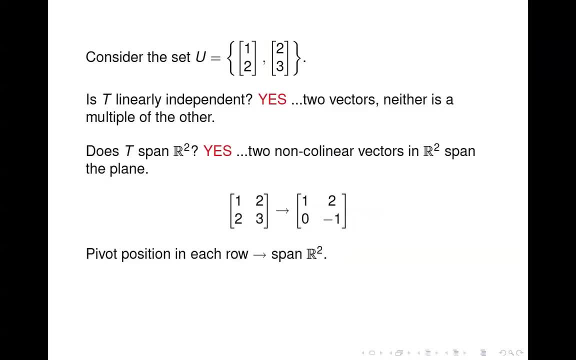 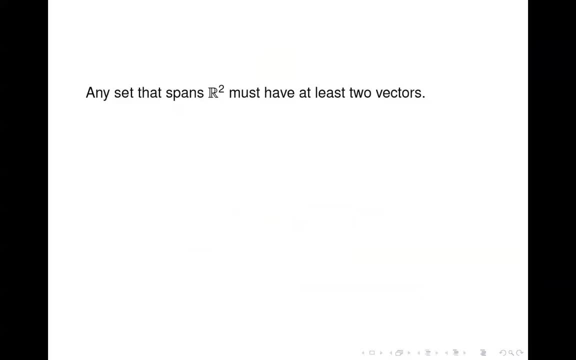 matrix form. you've got a pivot position every row so the vectors span R2. you have a pivot position in each column so they're linearly independent. so we see that any set that spans R2 has to have at least two vectors. because you have to. 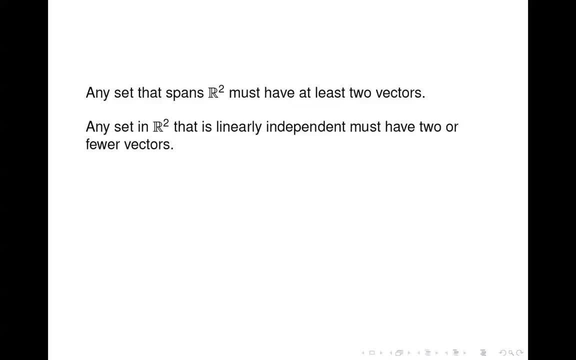 have one in each row. pivot position in each row. any set that's linearly independent must have two or fewer vectors. right, because once you get over two, you can't have a pivot position in each column. so any set that's both linearly independent and spans R2 has to have exactly two vectors, right, exactly. 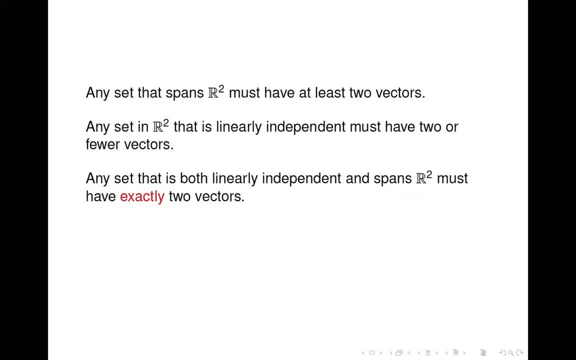 two, because to span it needs at least two. to be linearly independent It needs no more than two. so if you want both, then you have to have exactly two vectors: Such a set that's both linearly independent and spans. R2 is said to be a basis for R2.. 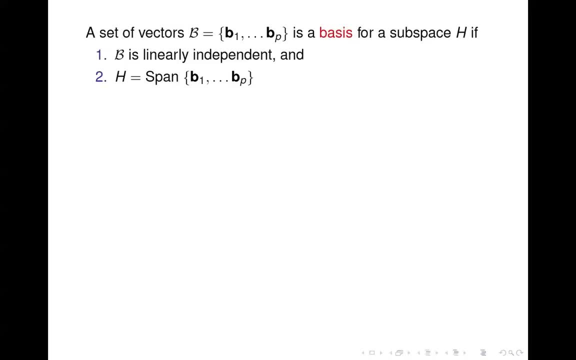 Here's a formal definition. Set of vectors B1 through BP is a basis for some subspace H if the set's linearly independent and the span of the set is the subspace. So you need two pieces to be a basis, One, linear independence, the other must span the subspace. 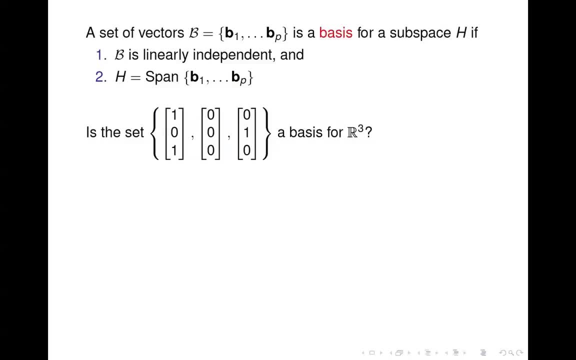 So let's look at a few examples. Here's a set and I want to know: is this a basis for R3?? So pick one of the criteria- either linearly independent or spans- And see if those are satisfied. So let's start off with: is it linearly independent? 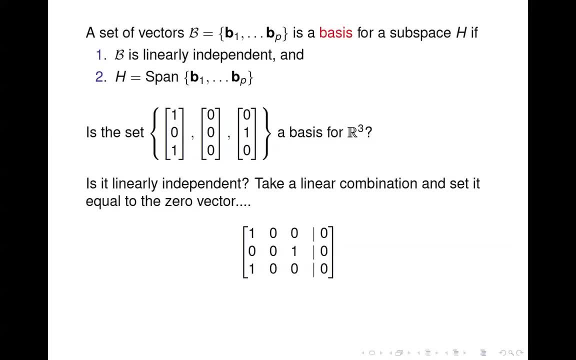 Well, if you set up the augmented matrix, set it equal to zero. then you can clearly see you don't have a pivot position in the second column here and so can't be linearly independent. So it's not a basis, All right. 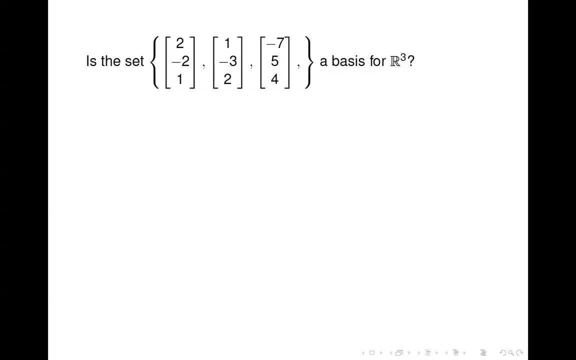 How about another set? Let's see Another set. There's one. not so clear here whether these vectors are linearly independent. So we put them in a matrix, do some row operations and we end up here with a coefficient matrix. 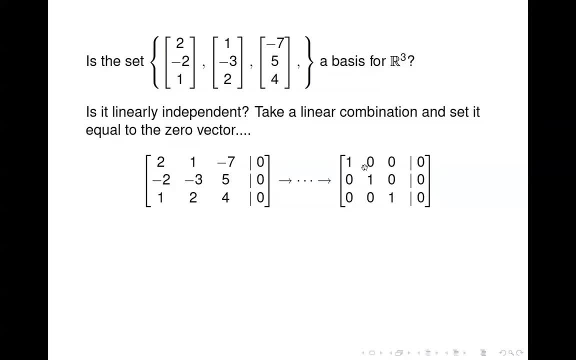 Notice, it has a pivot position in every column. So the only solution is the trivial solution. Therefore the vectors are linearly independent. We can also look at the matrix here and see that there's a pivot position in every row. So they span R3 and therefore they must be a basis for R3.. 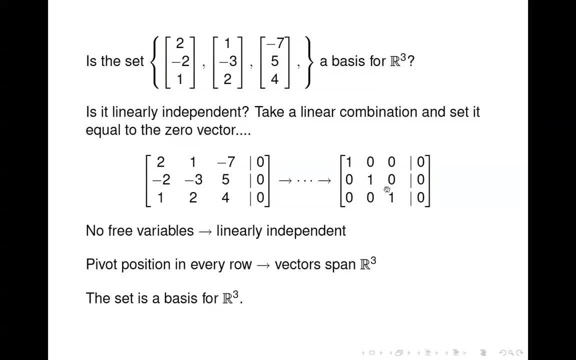 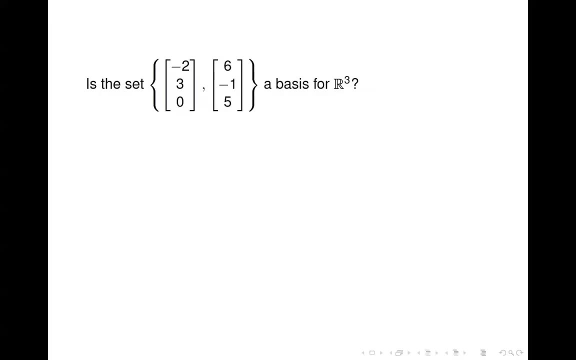 So the key is: looking at the coefficient matrix in echelon form, You can see a pivot position in every column, So they're linearly independent. pivot position in every row, So they span R3.. Here's another set. Is this a basis for R3?? 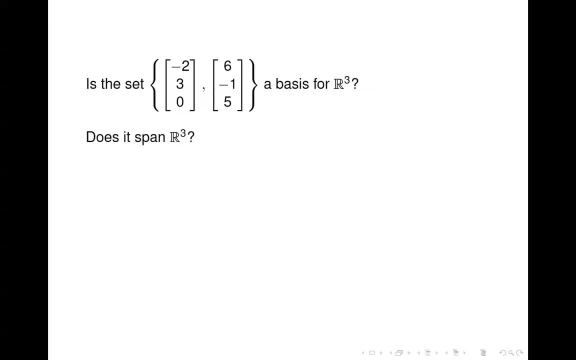 And you're probably thinking: well, there's only two vectors and in R3 you need three vectors to span. And that's right, Because if you look at that matrix you can't have a pivot position in every row. So therefore these vectors can't span R3 and therefore can't be a basis for R3.. 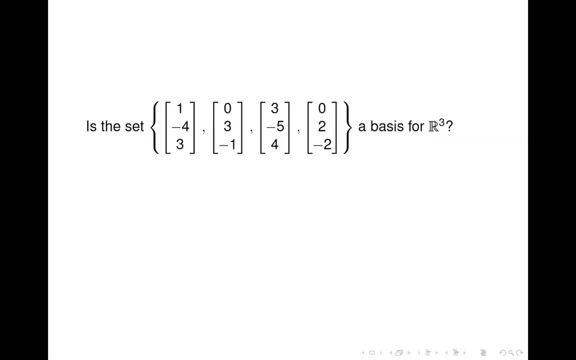 And how about this one? If you look at this one, Maybe you're thinking: oh, we've got four vectors in R3. They can't be linearly independent, right? Because if you put them in a matrix, there's no way to have a pivot position. oops, no. 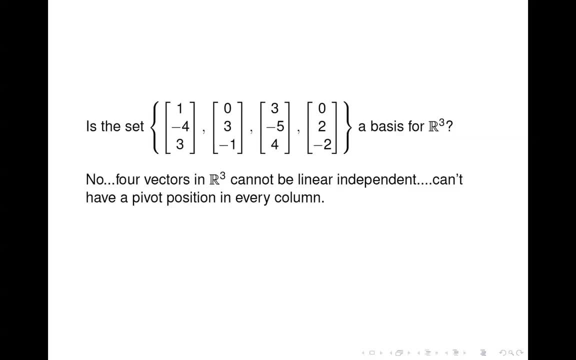 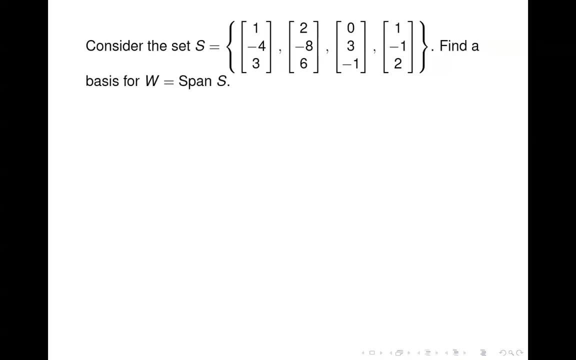 way to have a pivot position in every column. We've got four vectors. only three rows Can't have a pivot position in every column, So not linearly independent. Now here's a little different question. Here I've got four. 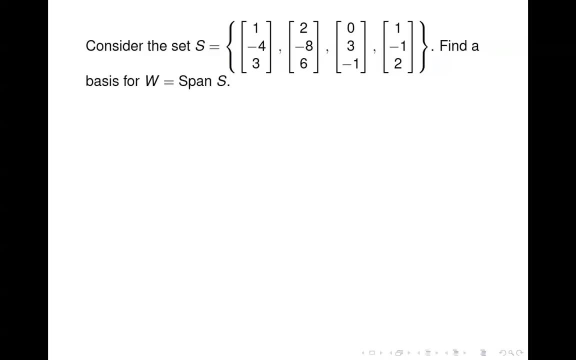 A set of four, A set of four vectors, And I'm not asking, though: is this a basis for R3?? Clearly it's not, because four vectors can't be linearly independent. What I'm asking, though, is for you to find a basis for the span of this set. 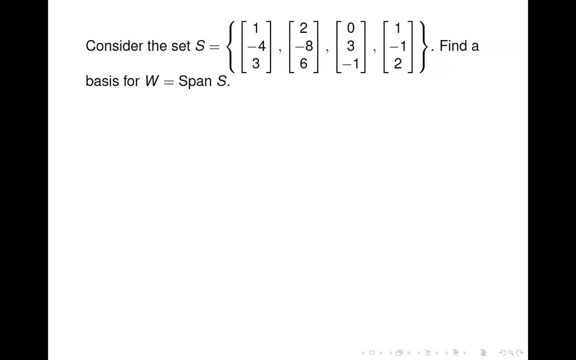 OK. So we don't really know what the span of this set is. It's some either all of R3 or some piece of R3.. We don't know. So We want to know: whatever that space is, what is the basis for it? 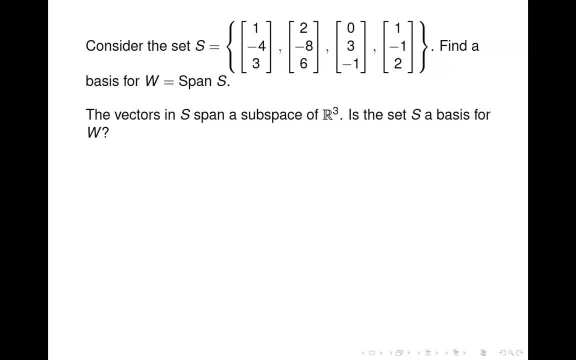 Well, you know, one of the criteria for basis is that it spans the set. So clearly, if we just take all four vectors, they're going to span W, because that's how W is defined. So the question is: are they linearly independent? 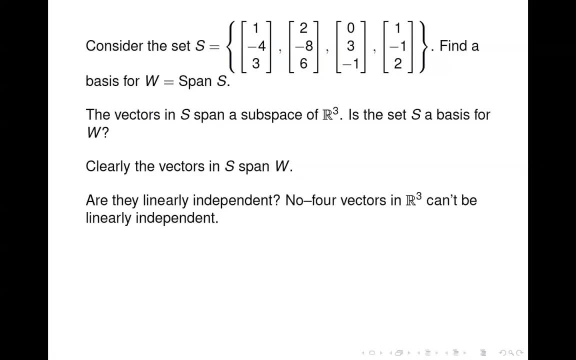 And we already know that they're not OK Because there's four vectors in R3. So remember, since they're not linearly independent, then that means that at least one of them is a linear combination of the others, And so one strategy would be to throw out the ones that are dependent on the others. 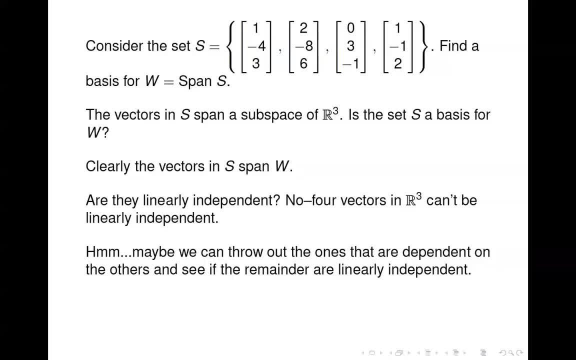 and then reduce that down to where we have a linearly independent set. All right, Now, in this case, I'll point out to you that the second vector here is twice the first. You can look at that: 2 times 1 is 2.. 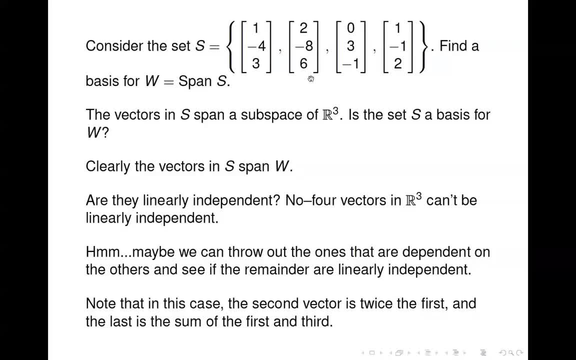 2 times negative 4, negative 8, and so forth. And the last one, OK, vector 4. here is the sum of the first and the third. So we've got 1 plus 0 gives you 1, negative 4 plus 3 is negative 1, so forth. 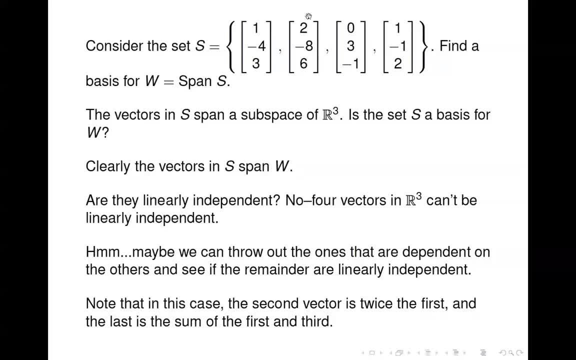 All right, So that tells us that the second vector is dependent on the first. OK, It's a linear combination of the first And the last one is a linear combination of the first and the third, So it seems like we should be able to throw those out, OK. 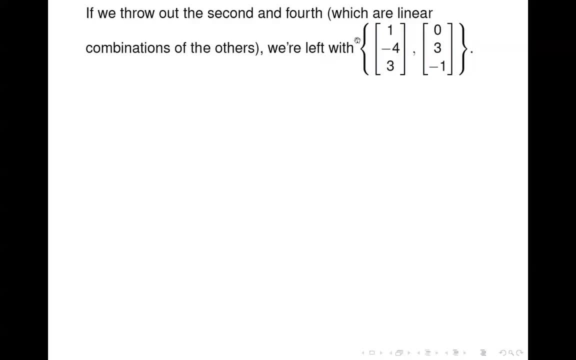 We don't need them, OK, And if we do, then we're left with these two vectors And we can look at it and see that it's linearly independent because we've got two vectors that are not multiples of each other. It's still a little iffy on whether this set spans the original set W right. 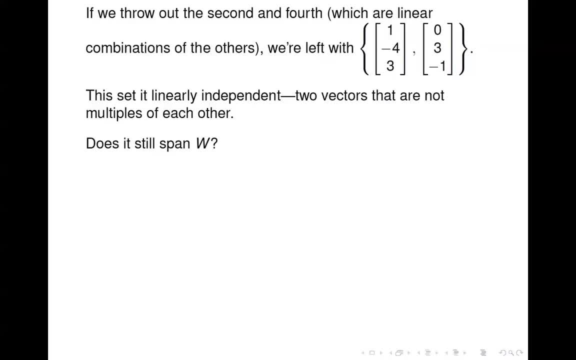 So, because we threw out some, how do we know that these two still span the subspace? Well, let's introduce a little shortcut notation here. Let's say we're going to call the four original vectors V1 through V4.. All right, 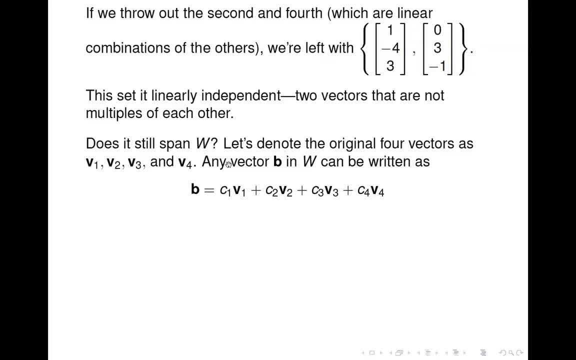 OK, And so any vector in the span of those vectors, or any vector in W, can be written in this form: Linear combination of those four vectors. all right Now we know, though, that V2, the second vector, was 2 times the first one. 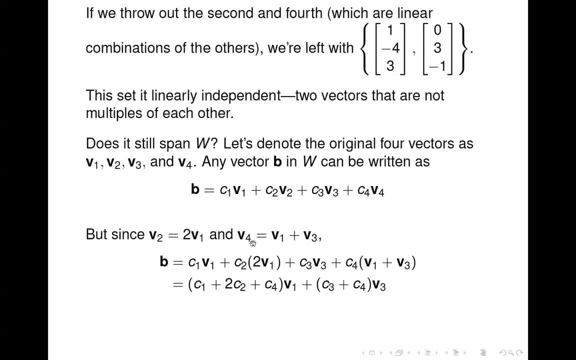 So we have this relationship here And we know that V4 was the sum of the first and the third. So we have this relationship, So we can plug that in back up in this equation. So, substituting for V2, we can plug in 2V1. 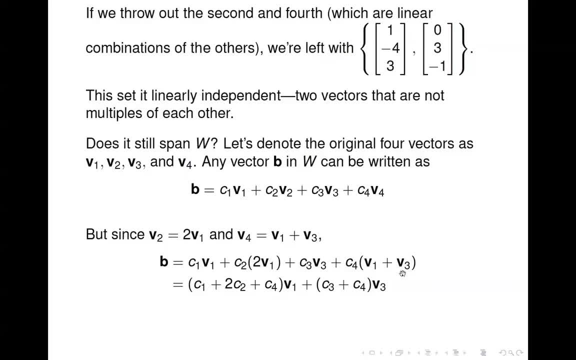 And for V4, we can plug in V1 plus V3.. And then, if we do a little rearranging, we can write V as just a linear combination of V1 and V3.. OK, We've got different coefficients, but that's OK. 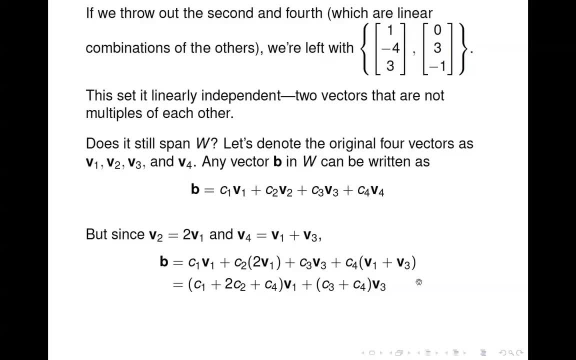 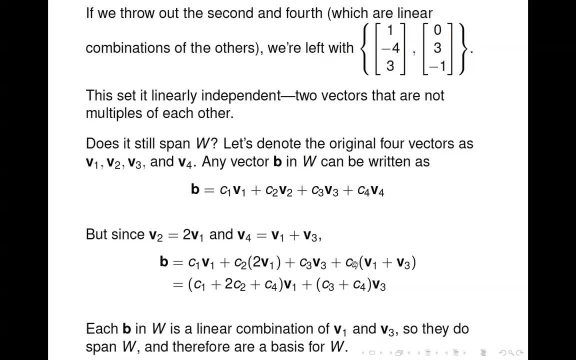 V1 and V3. Therefore, just V1 and V3, just those two vectors will span W, And we've already said that they're linearly independent. So therefore, they are a basis for W. All right, So we start off with our big set. threw out the ones that were dependent on the other. 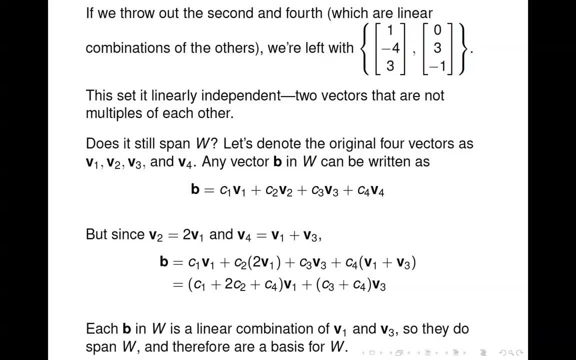 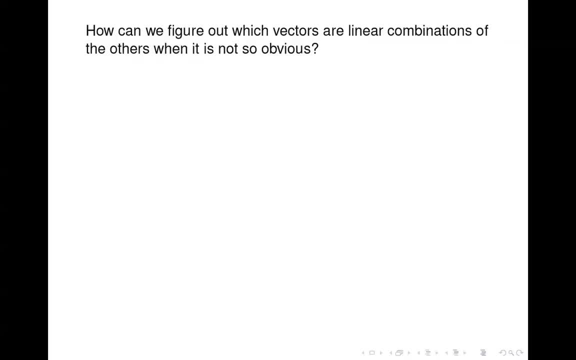 others, and what we were left with still spans and it's linearly independent. so it's a basis. now, in that problem, i told you which vectors were dependent on the others, so what can you do when that's not so obvious, right? how can you figure out which ones are? 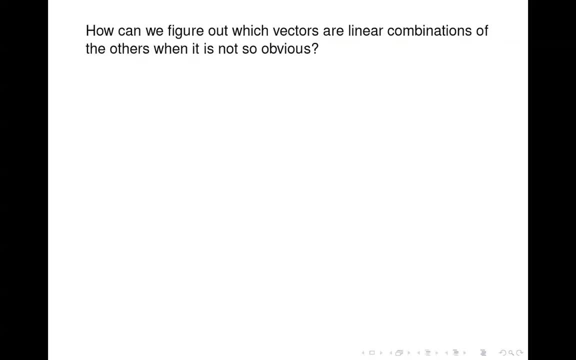 are dependent, when you can't just look at it and and tell, um well, there's an amazing thing, and that is that when you do elementary row operations um the, the dependence relations among the columns are not changed. okay, so these are the four vectors we had, uh, before. 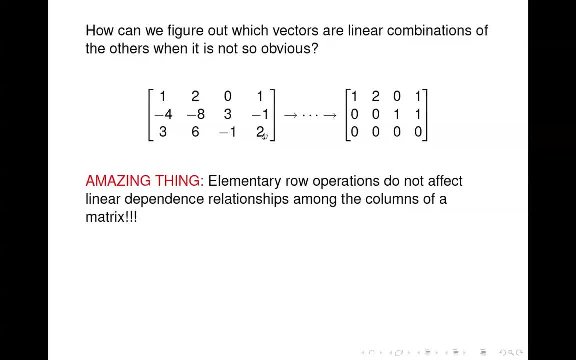 you remember, the second one is two times the first. the last one is the sum of the first and the third. all right, so i put it in echelon form and i get this matrix and look, the second column here is two times the second. so the second one is two times the third and the next one is two times the. 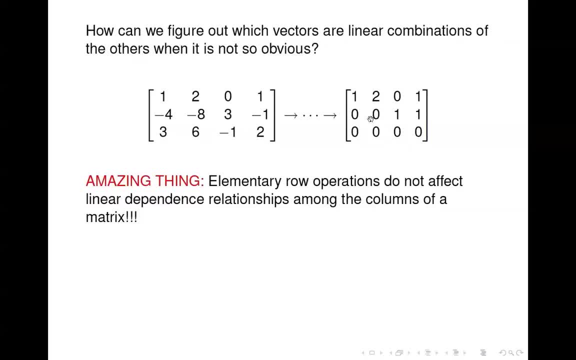 times the first right: 2 times 1 is 2,. 2 times 0 is 0,. 2 times 0 is 0,. and the last column is still the sum of the first and the third. 1 plus 0 is 1, 0 plus 1 is 1, 0 plus 0 is. 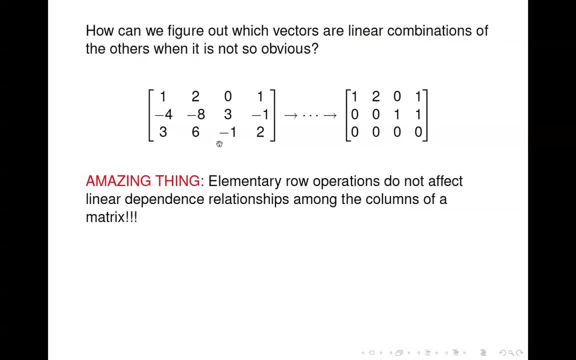 0, so you can take your original matrix or original vectors, throw them in a matrix, put the matrix in echelon form or reduced echelon form doesn't matter, and in that matrix the vectors will still exhibit the same relationships among each other. 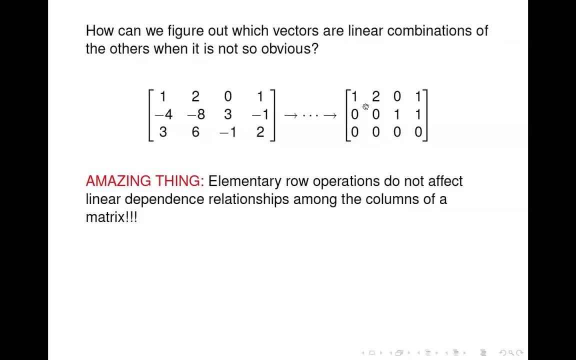 So what you see here is that the ones that we want to keep are the ones where we have pivot positions. okay, because if one, like the second one here, is dependent on the first one, there's no pivot position in column 2.. 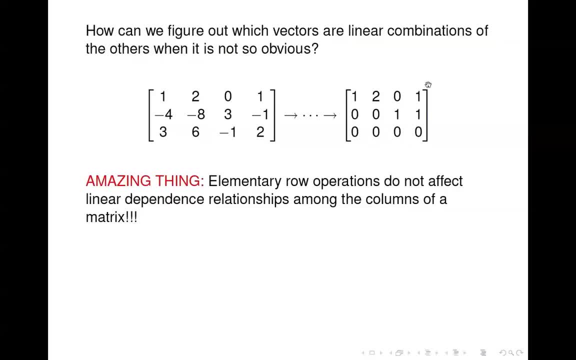 Column 4 is dependent on the first and the third. there's no pivot position in column 5. So the pivot columns indicate which columns are. indicate the columns that are linearly that should be independent. pivot columns indicate the columns that are linearly independent. 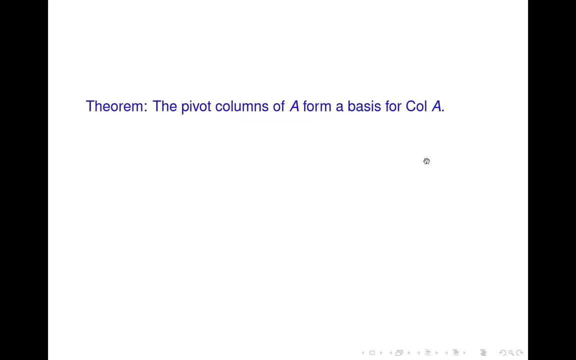 okay, so those are the ones we want to keep. We have a theorem that says that the pivot columns form a basis for the column space of A. All right now. along with this comes a warning, which is to be careful to use the pivot columns. 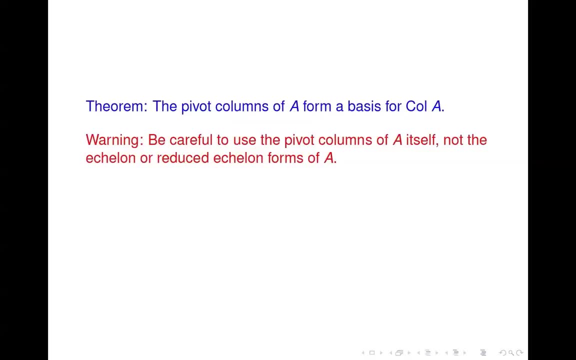 of A. that is the original matrix, not some echelon or reduced echelon form of A, and that's because elementary row operations can change the column space of a matrix. okay, So we go back and look at that example one more time. 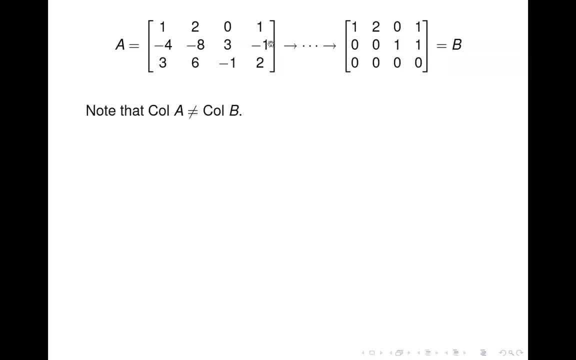 The column space of A, that is, all linear combinations of the columns of A, is not the same as the set of all linear combinations of the columns of B. okay, those are not the same, And so the column spaces are not the same. 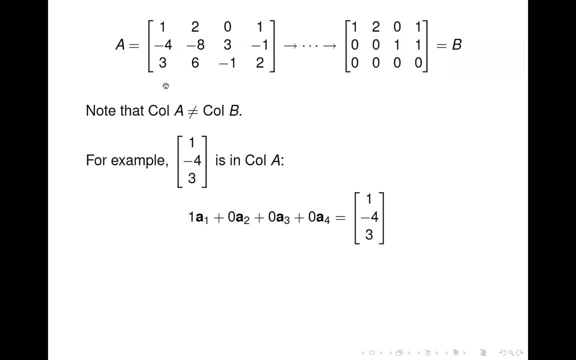 For example, the first column of A is clearly in the column space of A. we take one times first column, zero times the others, and that's what you get. but that column is not in the column space of B. Why? Well, when we set up the system, we've got this right-hand side notice system's inconsistent. 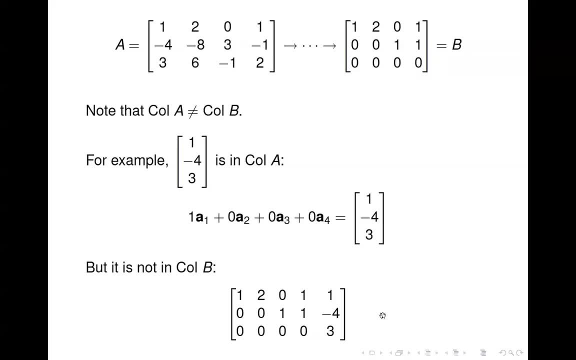 because we've got all zeros and then something not zero. okay, it's not in the column space. So the column spaces are different. therefore, you can't take the pivot columns from B and say that that's a basis for the column space of A. 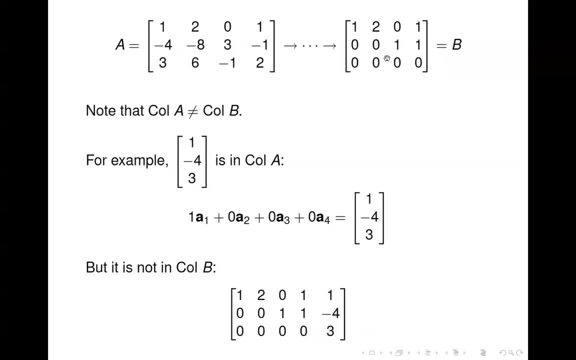 You need to look in your echelon form or your reduced echelon form, see which ones are the pivot columns and then go back and pull those from the original matrix. All right, here's another example. here's a matrix and you're asked to find a basis. 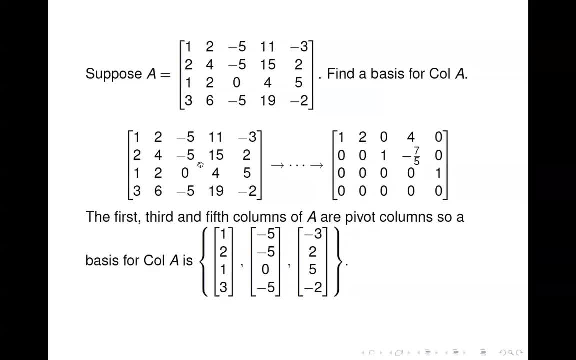 for the column space of this matrix. So we put it in echelon form: get this matrix and notice we've got pivot column, a pivot position in the first column, third column and the fifth column. So therefore we go back and take the first, third and fifth columns of A 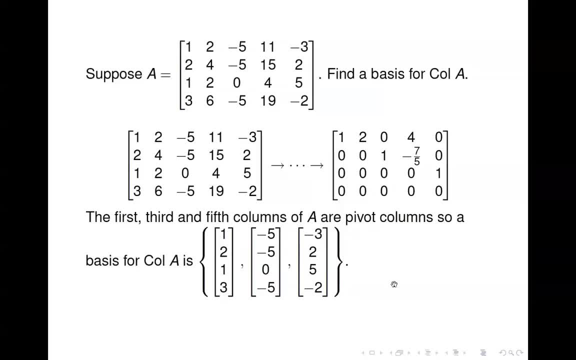 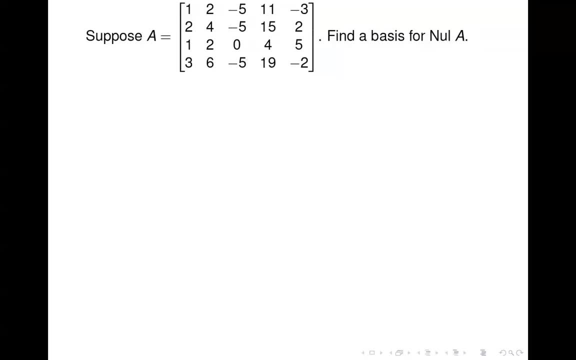 For a basis for the column space of A. Okay, now here's a little different question: Same matrix: you're asked to find the basis for the null space of A Right. remember the null space set of all solutions to AX equals zero. 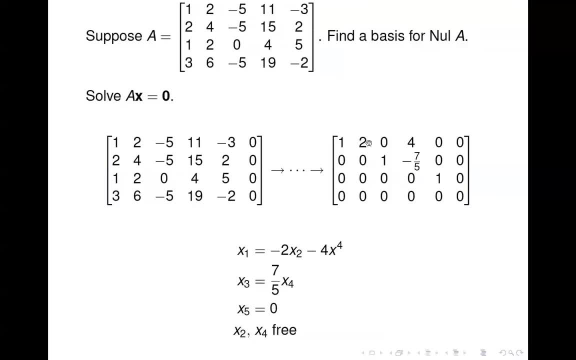 So let's solve: AX equals zero. Get the same matrix. here we look at the general form of the solution. from the first row we get X1. It's going to be negative, 2X2 minus 4X4, X3 is going to be 7 fifths X4, and from the 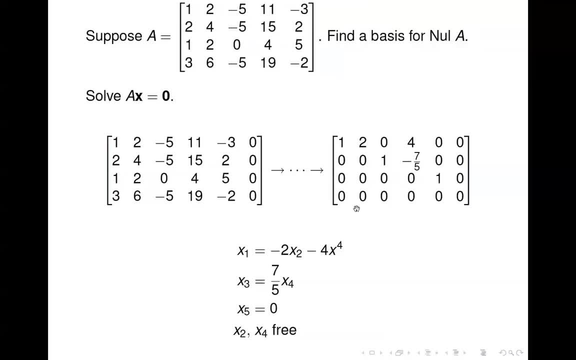 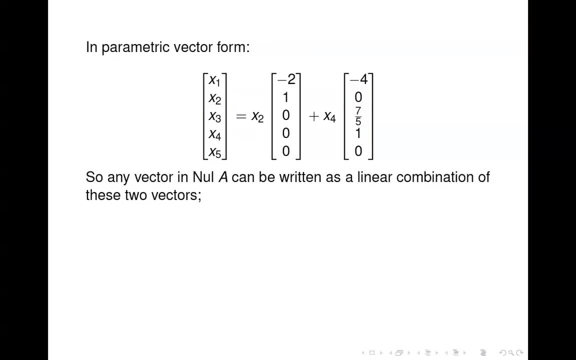 third row we get: X5 is just equal to zero, X2 and X4 are free variables, So we put that in parametric vector form. we get what's given here, and so any vector in the null space of A can be written as a linear combination of these two vectors. 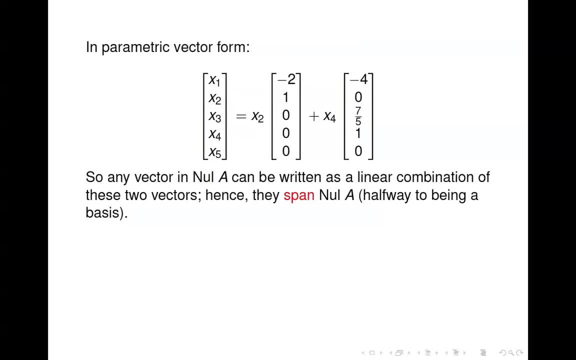 Right, So we know that they span the null space of A. so we've got half. we're halfway to being a basis. still need to show that they are linearly independent, or reduce the set so that we get a linearly independent set. 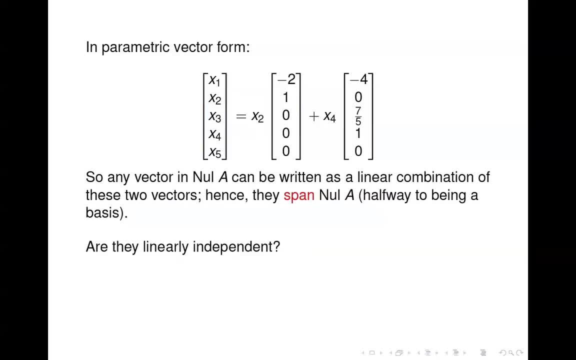 So the question is: we know that they span. are they linearly independent? And if you just look at them, it's clear that they are, because we've got two vectors that are not multiples of each other, So they must be linearly independent. 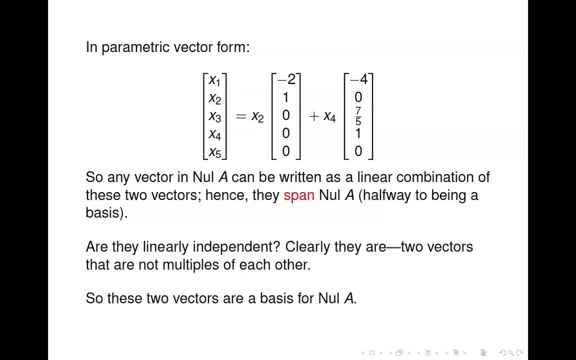 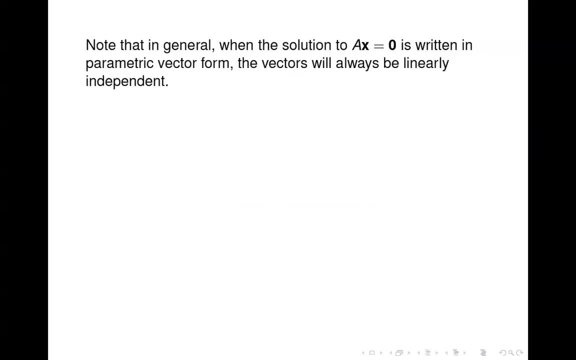 Okay, So these two vectors would be a basis for the null space of A. Now an important point is that, in general, when you solve AX equals zero and write your solution in parametric vector form, the vectors that you get will always be linearly independent. 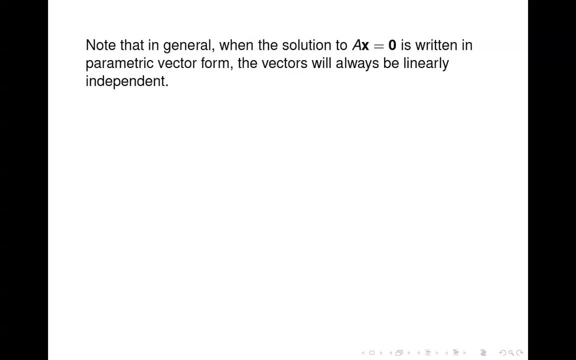 So, in fact, when you write that solution in parametric vector form, you've got a set of vectors that spans And they will be linearly independent. Now, why are they linearly independent? Because the only way to produce the zero vector is to set each of the three variables equal. 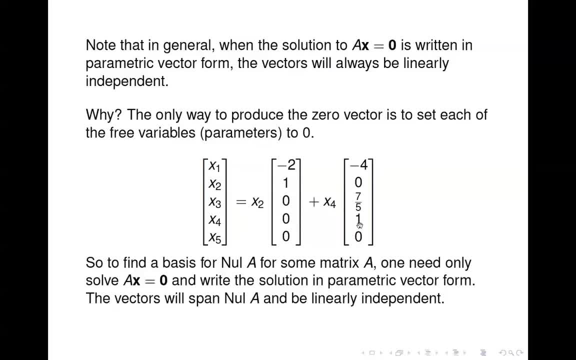 to zero. So if you go back and look at the one we were just looking at, right, if you didn't know, if you can just look at that and tell that they're not multiples of each other, so they're linearly independent, right? if you tried to solve the system, then notice that in the 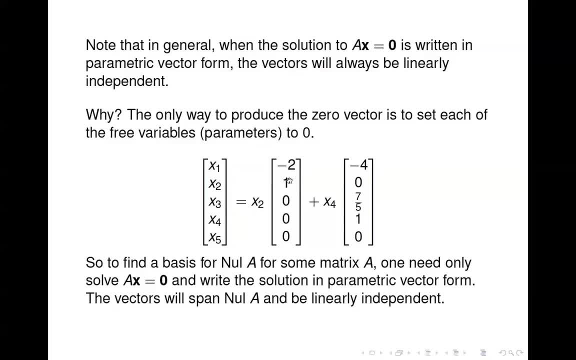 second component. you've got X2 plus zero would equal zero. So X2 has to be zero And X4 times one equals zero means X4 has to be zero. Because of the way these vectors are produced, you always end up with the element that corresponds. 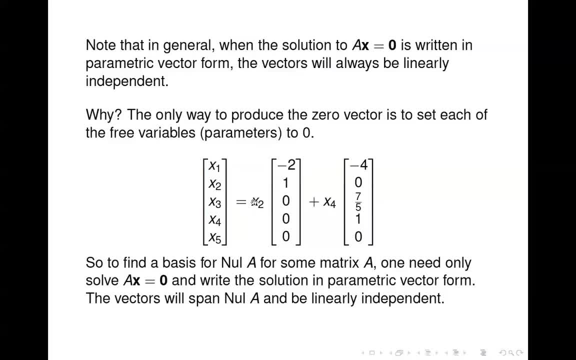 to the free variable. So in this case, the second component, since this is multiplied by X2, if you looked at that whole row Then the only solution would be set X2 equal to zero, And similarly for X4, X4 has to be zero. 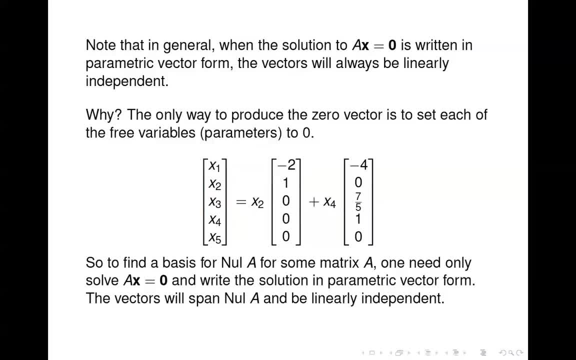 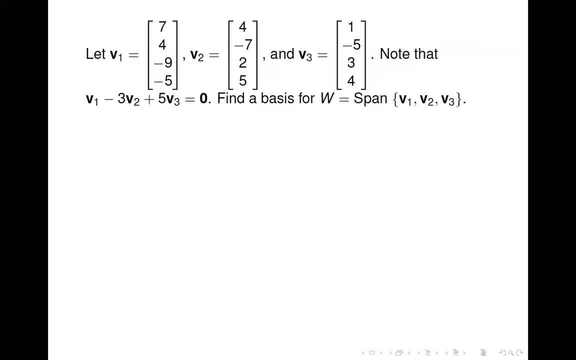 So when you write your solution in parametric vector form, automatically you have a basis because they span and they're linearly independent. All right, one more example. I've got three vectors here And We're given that V1 minus three, V2 plus five, V3 is equal to the zero vector. 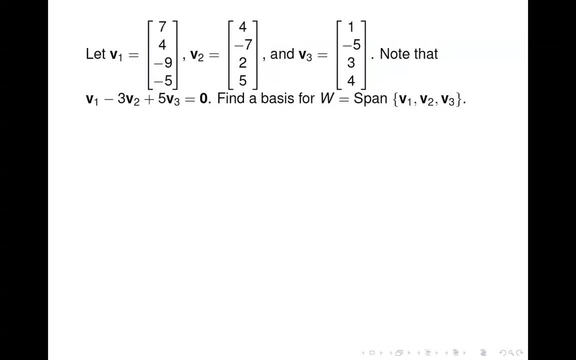 And you're asked to find a basis for the span of these vectors. So again, clearly you know that if you took all three you have a set that spans, But we know from what we're given that they're not linearly independent. 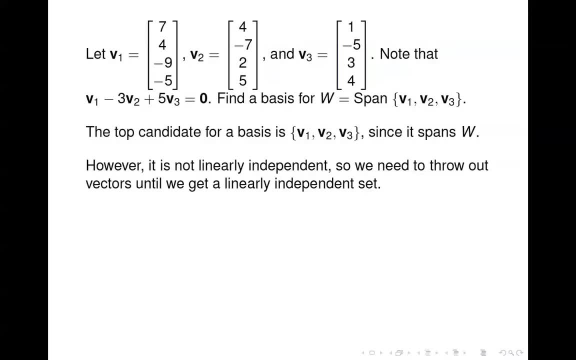 So we need to figure out which vectors to throw out until we get to a linearly independent set. And since we can write any of the three as a linear combination of the other two, right simply solve this equation for any of the three vectors. then we could throw any of. 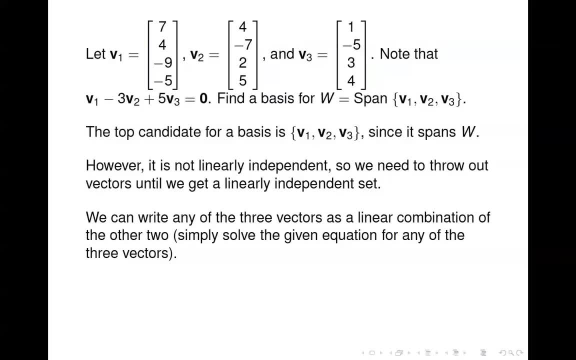 them out. But it's kind of convention to throw out the first one that's linearly dependent, which would be V3. And so we're left with V1 and V2. And if we just look at those we can see that they're not multiples of each other. So we're left with V1 and V2. And if we just look at those, we can see that they're not multiples of each other. So we're left with V1 and V2. And if we just look at those, we can see that they're not multiples of each other. 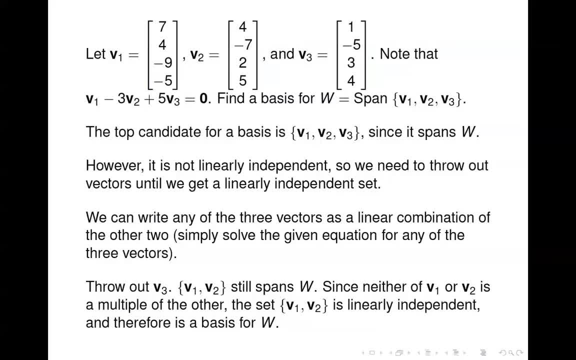 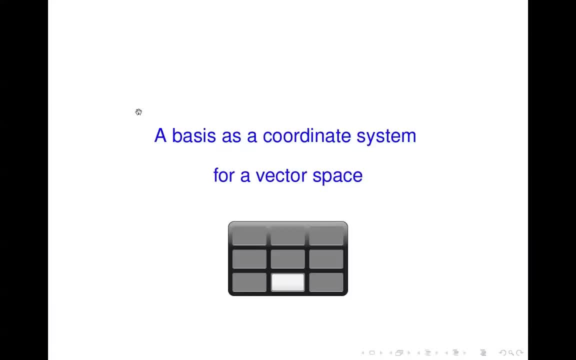 And so therefore, the set V1, V2 is linearly independent. It still spans And therefore it's a basis for W OK. today we're going to talk about using a basis as a coordinate system for a vector space. 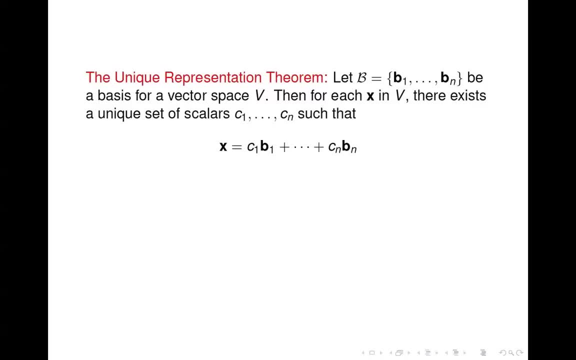 We start off with the unique representation theorem And it says: suppose you have a basis B Which consists of the vectors B1 through Bn And you choose some x from the vector space V, And the theorem says that no matter which x you pick from the vector space, there are 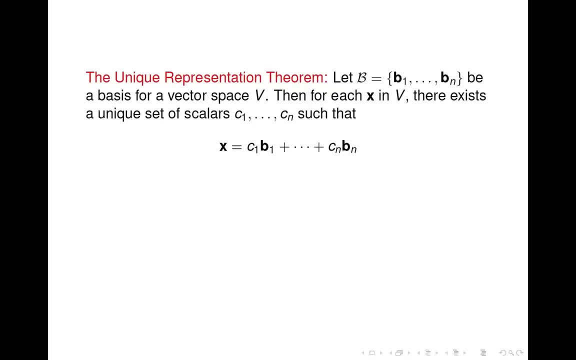 a unique set of scalars, C1 through Cn, that you can use to take a linear combination of the vectors in your basis to produce x. OK, So we're going to look at that, OK Now. so it's really saying two things. 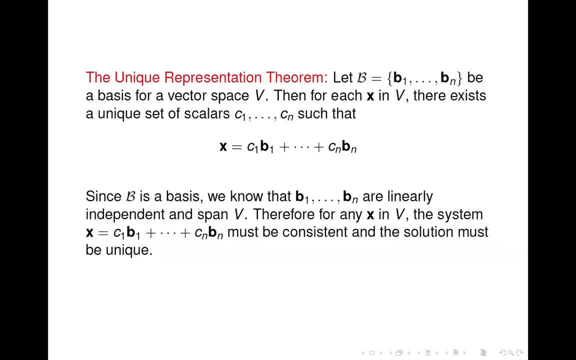 It's saying that that system's consistent. You can take a linear combination of the Bs and you can produce any vector in the vector space. And it's also saying that the solution to that system is unique. And both these things follow from the fact that B is a basis for V, The fact that it's 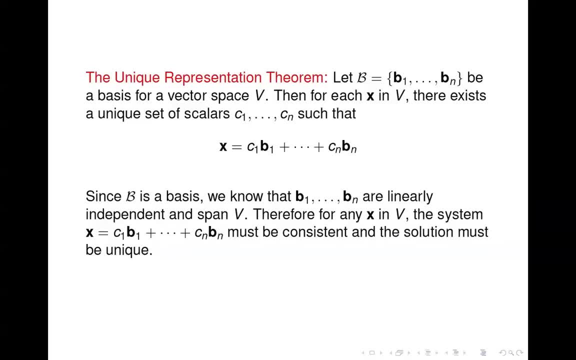 a basis tells you that these vectors span V, So therefore that system is going to have a solution, no matter what x is. And it also tells you that these vectors are linearly independent. And since they're linearly independent, the solution to that system will be unique, since 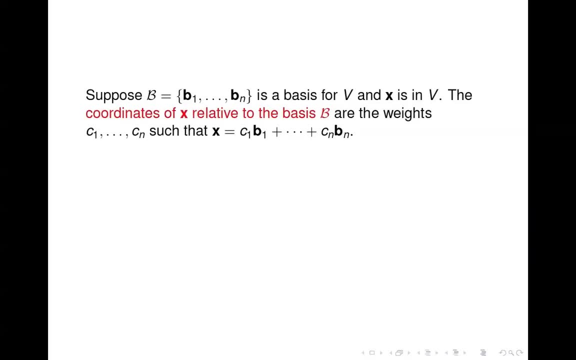 there's no free variables. OK, Now the weights that we use. these C values are called the coordinates of x relative to the basis B. OK, And we write that down. OK, And we write them using your book's notation as x, with the brackets around it, this notation. 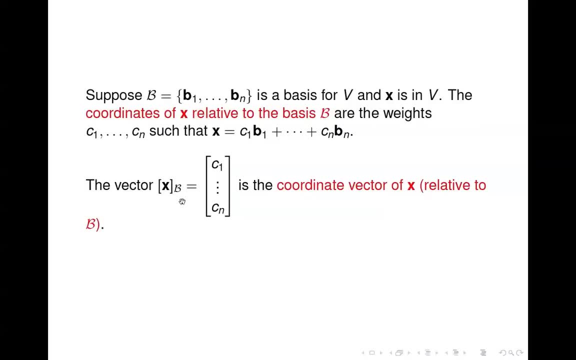 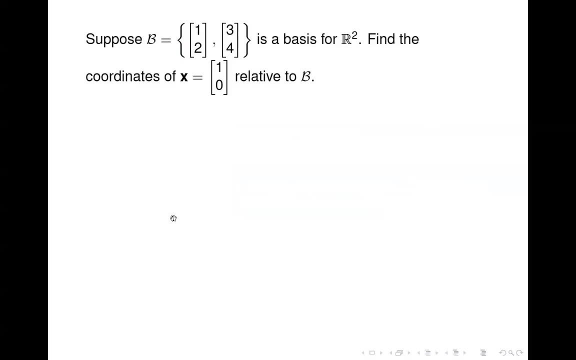 here with a subscript B And we call that the coordinate vector of x relative to the basis B. All right, So for example, we have a basis for R2 here, the vectors 1,, 2,, 3,, 4.. 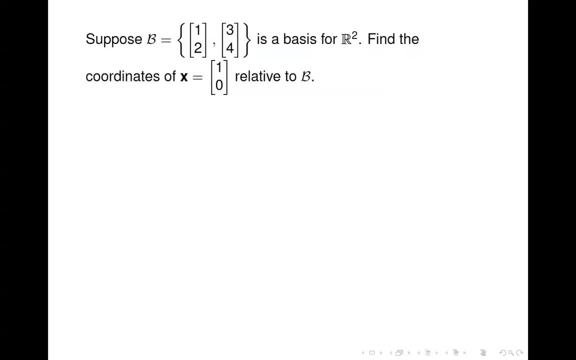 Just a quick aside. How do we know that that's a basis for R2?? Well, the simplest way is to say: well, we know, the dimension of R2 is 2.. And here we have a set with two vectors that are linearly independent. 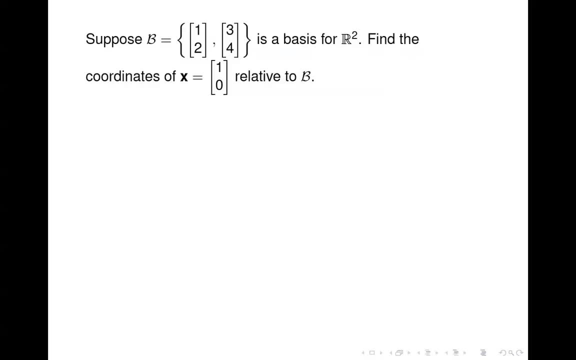 We know they're linearly independent because there's two vectors and neither's a multiple of the other. All right, So my question is based on this particular basis. can you find the coordinates of the vectors 0 or 1,? 0 relative to this vector? 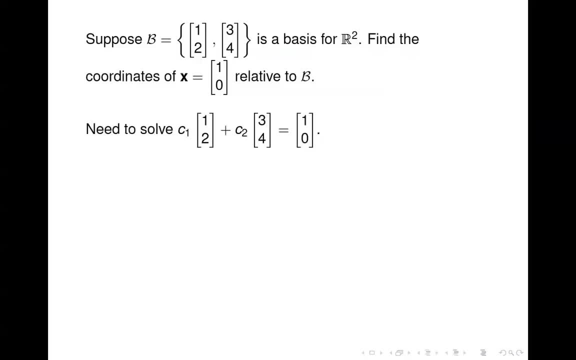 OK, So we can find the coordinates of this basis. So, just setting up the system that we talked about previously, we need to take a linear combination of the vectors and the basis to produce x, And so we can set up that system in an augmented matrix and solve the system. 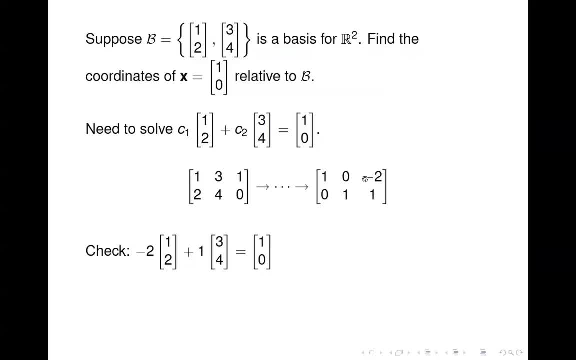 And this tells us that the numbers we're looking for are negative 2 and 1.. Just a quick check: We multiply negative 2 times the first vector Plus 1 times the second vector. That gives us 1, 0, which is what we were looking for. 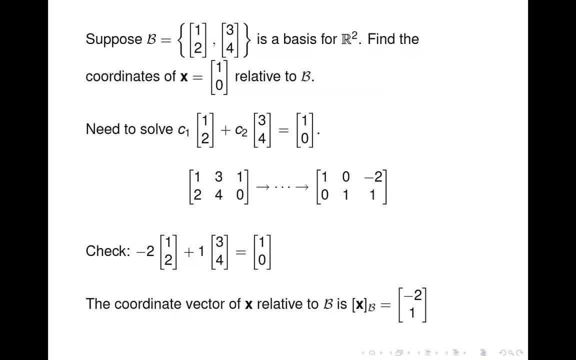 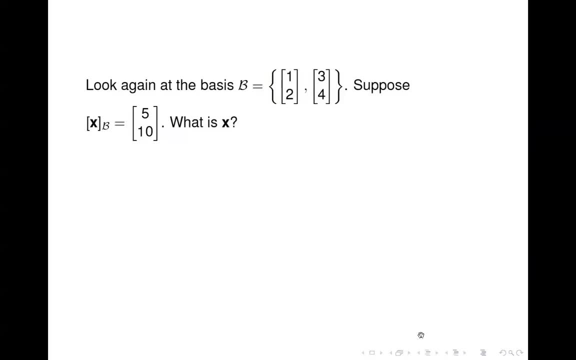 So that tells us that the coordinate vector of x relative to b, which we write in this notation, is negative: 2, 1.. All right, Suppose we go the other way. Suppose you're given the coordinate vector and you want to find the corresponding vector. 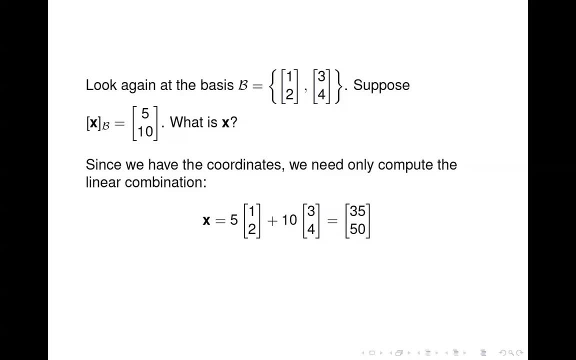 So in this case, all you need to do is compute that linear combination. You have the coordinates, So it's, in this case, be 5 times the first vector plus 10 times the second, And we compute that to be 35,, 50.. 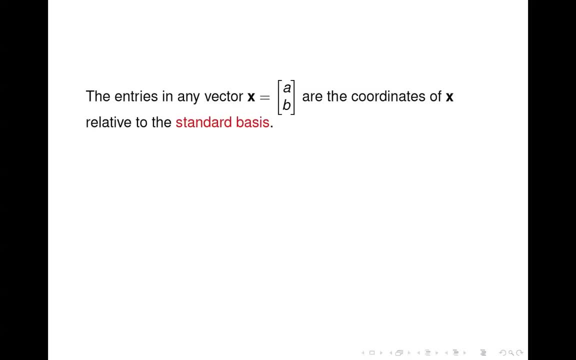 OK, This is a little bit of an aside, but kind of leads us into what we're going to talk about next. If you have any vector, say just ab, then the vector itself- OK- Is the coordinate vector relative to the standard basis. 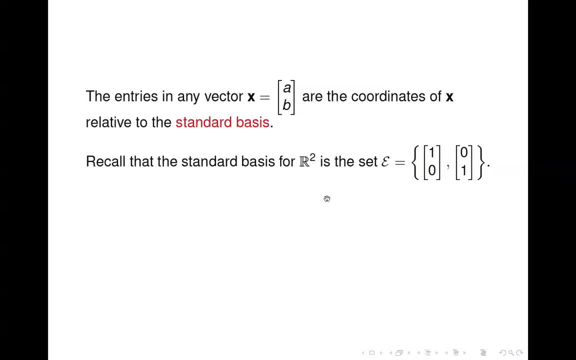 So let's refresh our memory about what the standard basis is. That's just the for R2, just the two columns of the identity matrix. Now your book refers to that as the labels that sit with a script E. All right. 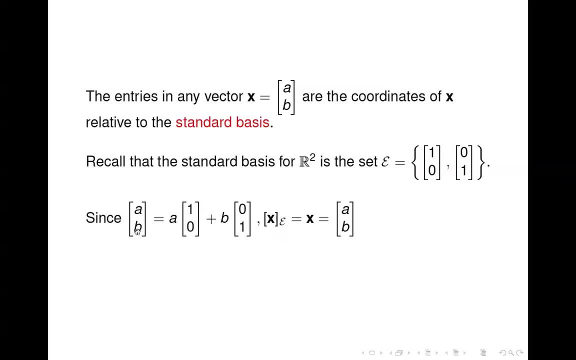 So notice that if you've got a vector ab, then that's just ab. OK, If you've got a vector ab, then that's just a times 1, 0 plus b times 0, 1.. So your coordinates are a and b. 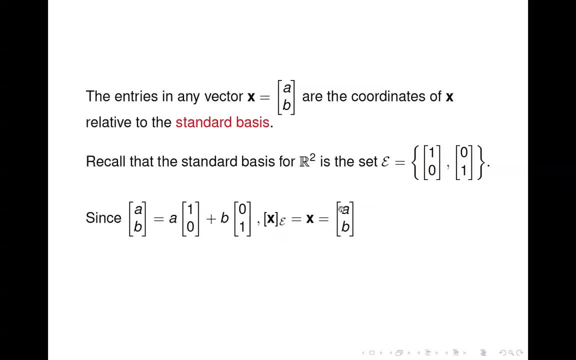 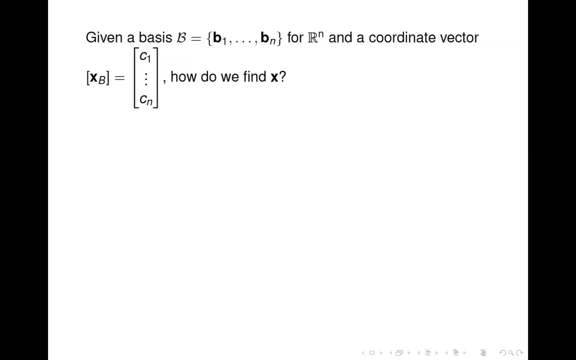 So therefore, the coordinate vector is just equal to the vector itself, which is just ab. So, relative to the standard basis, the entries in a vector are actually the entries in the coordinate vector. OK, So just a little review, If we have a basis, 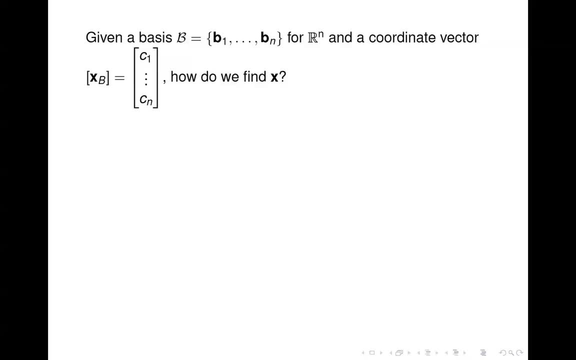 And a coordinate vector. How do we find the corresponding vector? Well, we just compute that linear combination, All right. So we know that this linear combination can be written in as a matrix times a vector. And so if we define this matrix, we'll call it p sub b, to be the matrix consisting of: 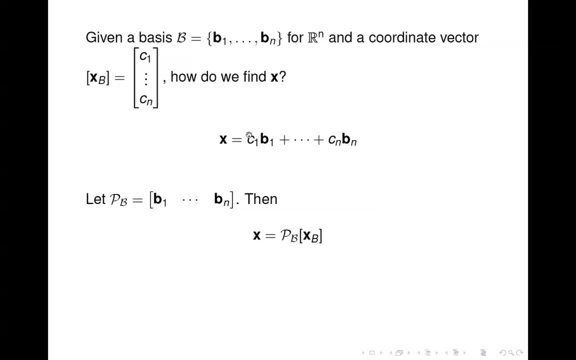 the vectors and the basis. Then This matrix combination can be written as p sub b times the coordinate vector And we say that p sub b is the change of coordinates matrix from b to the standard basis of our n. All right, So we're taking p sub b. 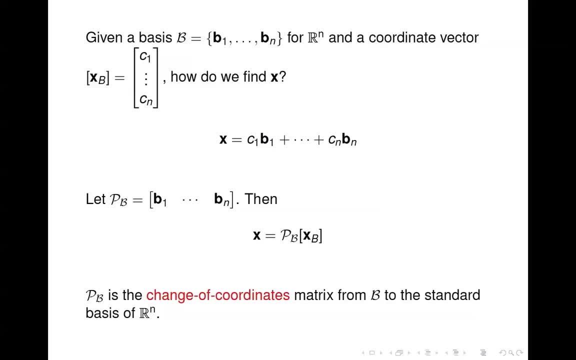 Multiplying it by the coordinate vector. All right, So we get the coordinate vector relative to b And we end up with the coordinate vector relative to the standard basis which, as we saw before, is just the vector itself. All right, 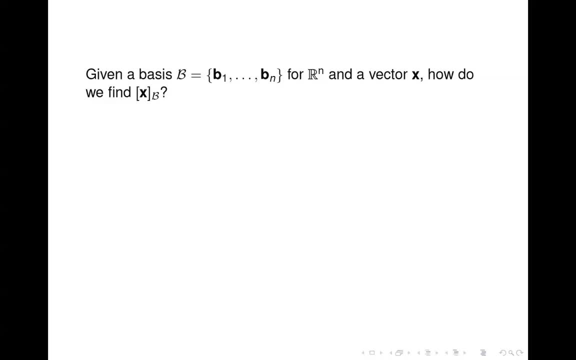 So talk about how we go back the other way. For given a basis and a vector, how do we find its coordinate vector? Well, we need to solve a system. Take the linear combination, set it equal to the vector and solve the system. 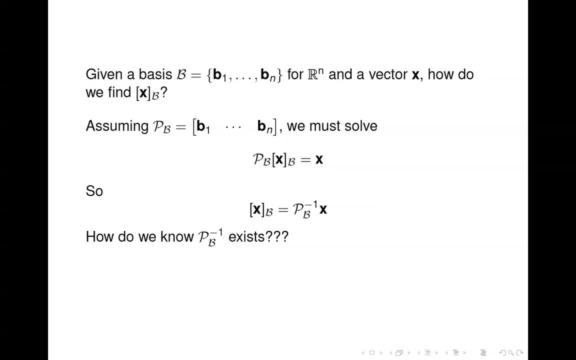 We need to figure out what those multipliers need to be. So, looking at it in matrix terms, we have this relationship, but we don't know what the coordinate vector is. So therefore, we need to solve the system for the coordinate vector. 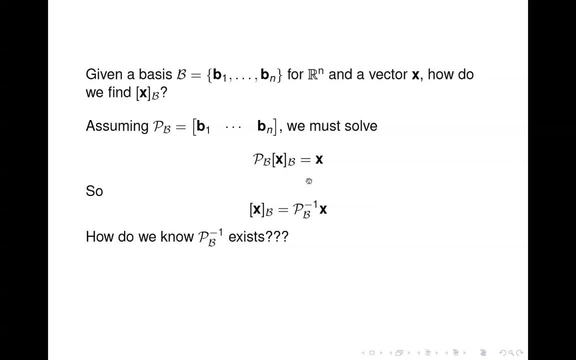 And one way to do that is to multiply both sides by the inverse of the matrix, and that'll give us the coordinate vector. Now, the danger there is. well, how do we know that matrix is invertible? Well, we actually do know that it's invertible because we know that its columns are basis. 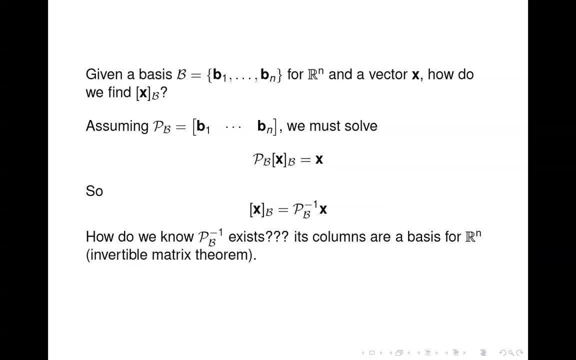 for Rn, And so that's actually straight out of the invertible matrix theorem. but you can get there in a couple of steps If you think well. columns are basis for Rn, so that means that the columns must be linearly independent, which means there's a pivot position in every column. therefore, 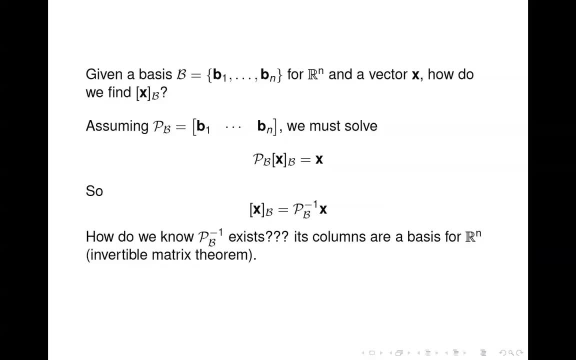 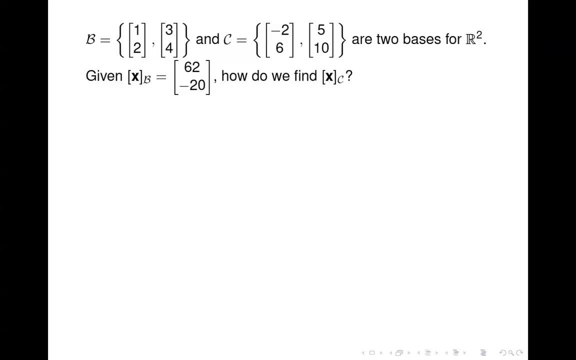 n pivot positions, So the matrix is invertible. OK, so we're going to put those two ideas together in this question. So here I've got two bases for R2.. Well, bases, that's the plural of basis, If you've seen that kind of confusing. but bases is just the plural of basis. 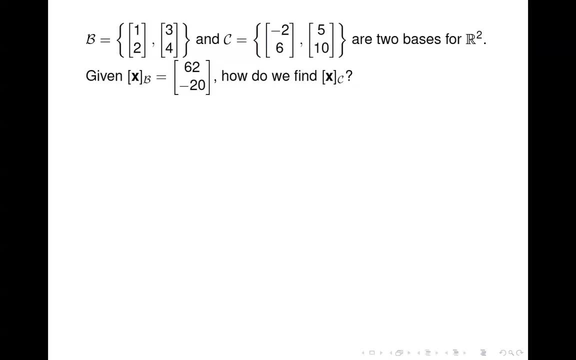 So we have two bases for R2 here, column B and C, And I have a coordinate vector for a, vector x relative to basis B. All right, so coordinate vector of x relative to B, which is this vector here? And I want to know how do we find the coordinate vector of x relative to C? 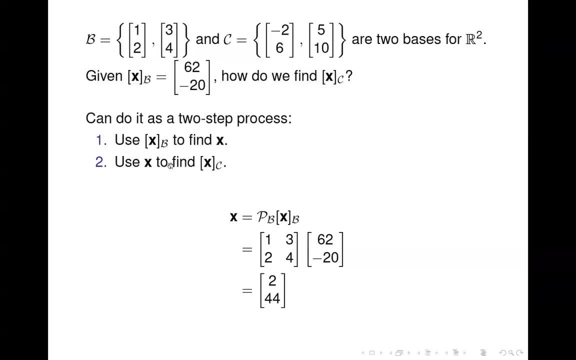 Well, you have to think about this. OK, So think of it probably easiest as a two-step process. So first use the coordinate vector relative to B to find actually what x is Right, and once you know what x is, then you can find the coordinate vector of x relative. 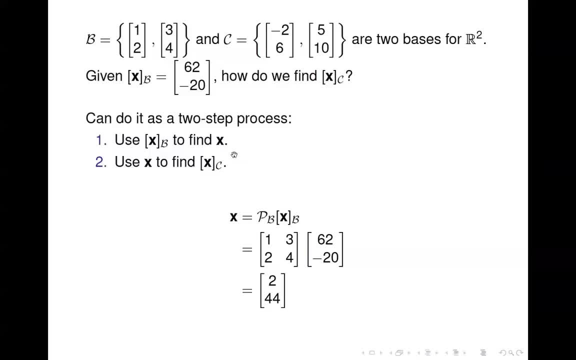 to C. All right, so we'll do those two steps. So the first one here to find x. we just multiply our P sub B matrix, the matrix consisting of the vectors in B Times, our coordinate vector, and we find that x is 244.. 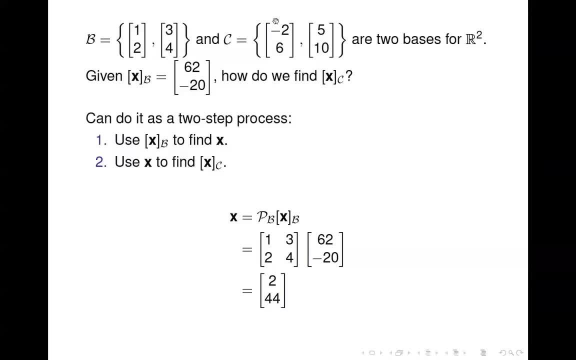 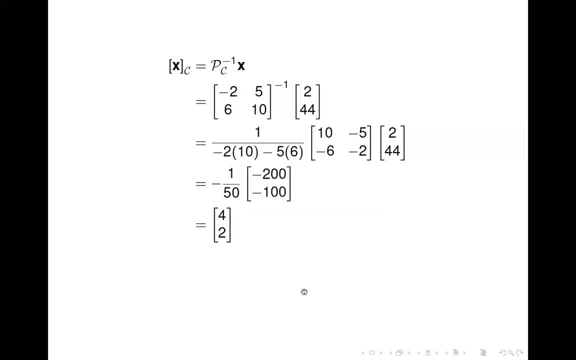 And once we know that, then we just need to take a linear combination of the vectors in C and set that equal to 244, and solve that system Right. or look at it like this, where we solve the system by taking the inverse of that matrix: 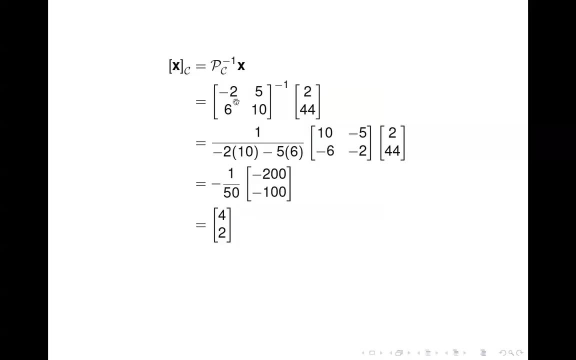 times x. So here's P sub C, And these are just the columns that are in the basis C. We invert that matrix, multiply by 244.. So what we have here- I'm taking 1 over the determinant times- this matrix times 244.. 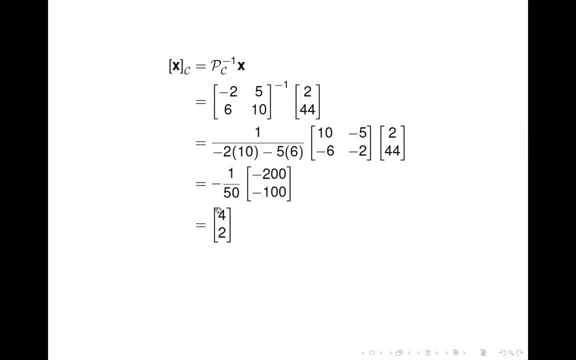 And I end up with a vector 4, 2.. So this is coordinate vector of x relative to C. Now, just to check, we can take that these coordinates times our vectors in C And see if we get x, Which we do. 244, all right. 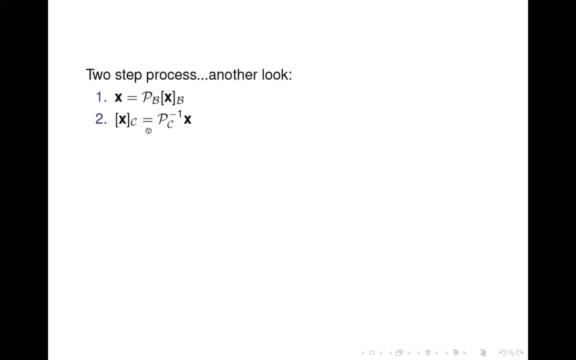 So let's take, let's go back and take a look at what we did, all right. First step was to compute x, which we did by P sub B times x sub B, And then compute the coordinate vector relative to C by P sub C inverse times x. 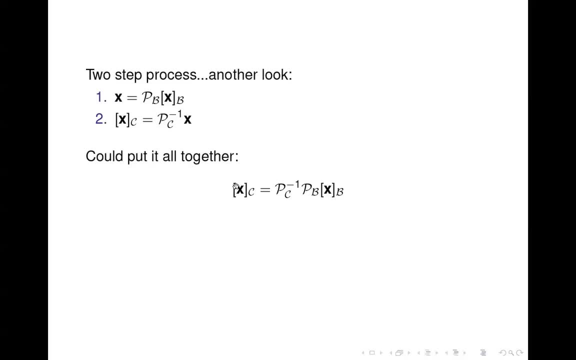 Now we can't put that all together. all right, just plug in for x and we have the coordinate vector of x relative to C. It's just P- C inverse times P sub B times the coordinate vector relative to B, And so what we have is a change of coordinates matrix from B to C. 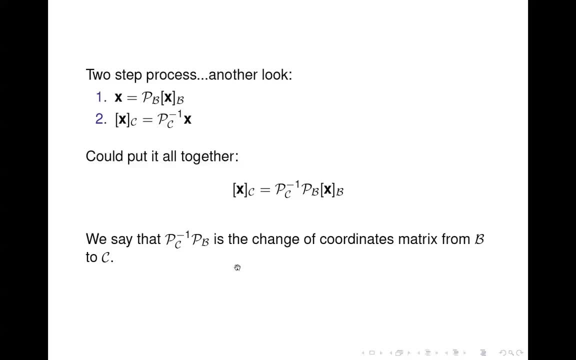 So this matrix takes us from coordinates in B to coordinates in C. all right, So P- C inverse times, P sub B is how we can change B coordinates to C coordinates. All right, we're going to switch gears just a little bit and talk about polynomials. 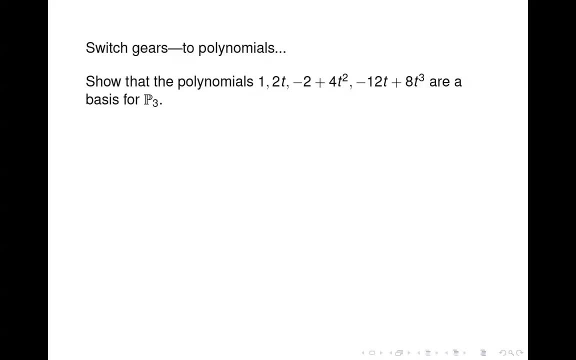 Let's examine this problem. I want to show that these polynomials are a basis for P sub 3.. Okay, this is actually a homework problem from section 4.5, I think. Okay. so to show that these are a basis for P sub 3, we need to show that they span P. 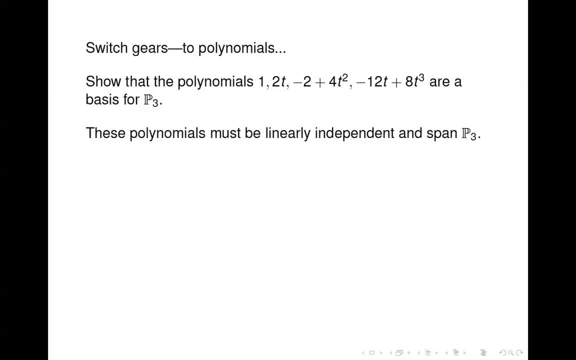 sub 3.. They're linearly independent. So let's start off and show that they're linearly independent. So to show any sets linearly independent, we have to take a linear combination and set it equal to the zero vector, or in this case, the zero element of P sub 3.. 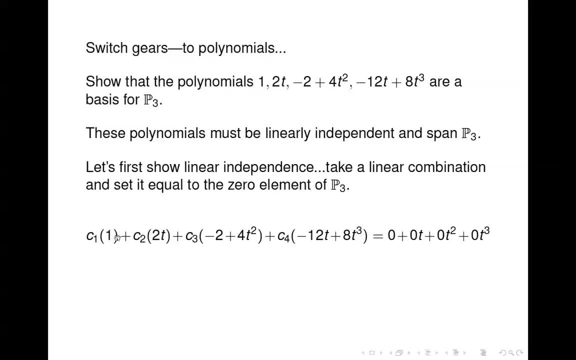 So here's a linear combination. all right: C sub 1 times the first element, C sub 2 times the second one. so forth equals here's the zero element of P sub 3.. Zero plus zero times T plus zero times T squared plus zero times T cubed. all right, and we: 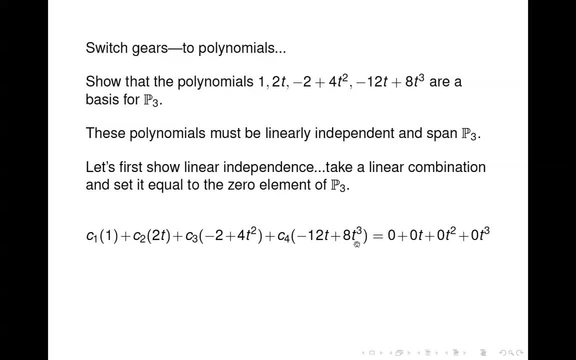 want to be able to show that the only solution to this system is that all the C's have to be zero. So the way to approach that is to collect like terms, all right, collect all the constant terms, collect all the coefficients of T and so forth, and then equate those coefficients. 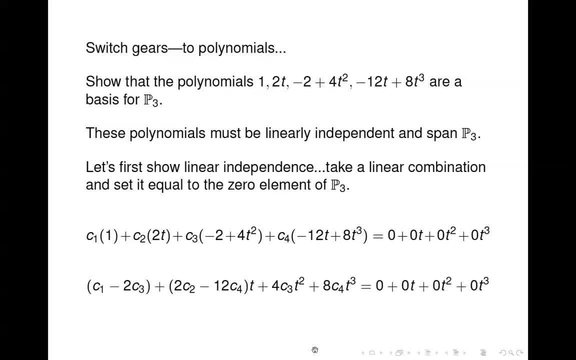 too. So that's what we have on the right-hand side. So we do that. we end up with this. so this comes from: we've got C1 here and then from this term, we get a 2 times C3, so that's our constant term. 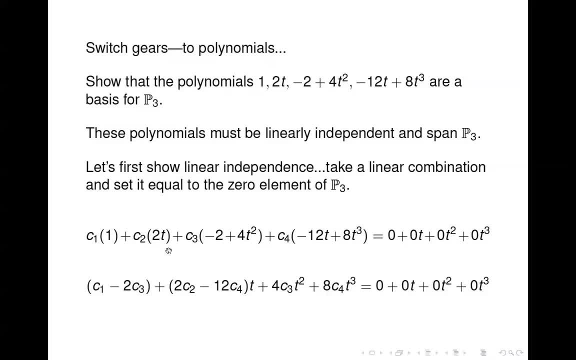 Coefficients of T. here we've got a 2 times C2 from here and over here a negative 12 times C4, so that's where that comes from. For T squared, I've got 4 times C sub 3.. 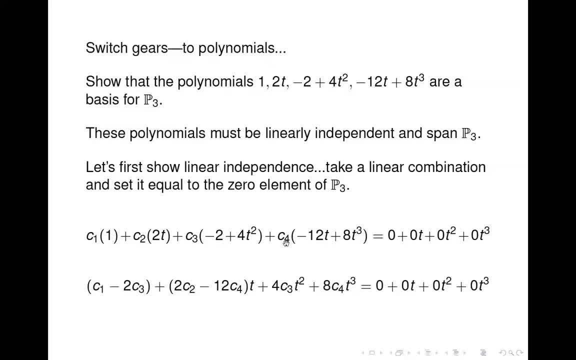 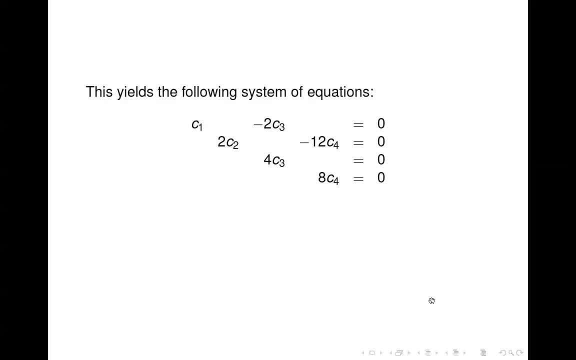 And for T cubed, I've got 4 times C sub 3.. So I've got an 8 times C sub 4, all right, So those are equal to this zero vector. again Now, if you write out that system of equations, right, we're going to get C sub 1 minus 2. 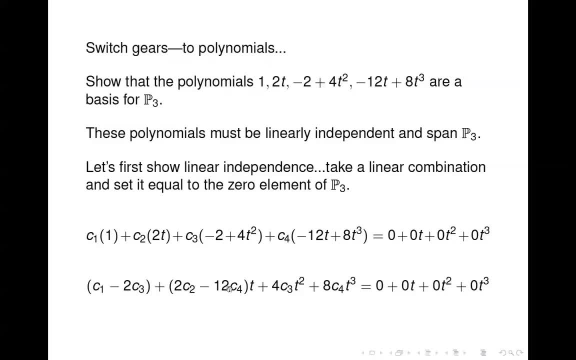 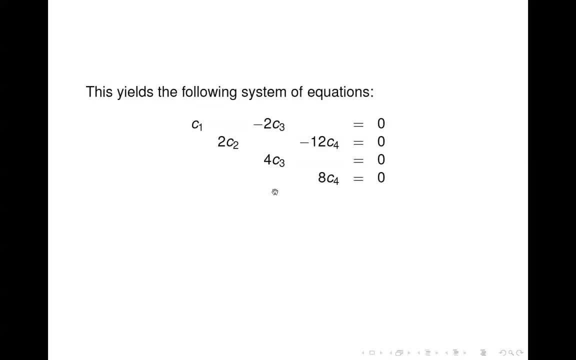 C3 equals zero, 2 C2 minus 12 C4 has to be zero and 4 C3 has to be zero and 8 C4 has to be zero. So if you write that out, it looks like this, and when you look at it like that, it's obvious. 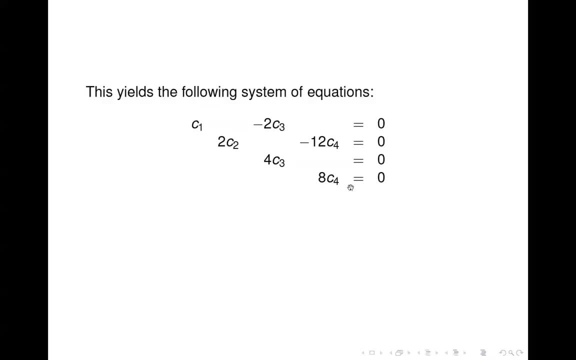 That all the C's have to be zero. right From the last equation you get: C4 has to be zero. From this one we get: C sub 3 has to be zero. and since both C3 and C4 are zero, then that. 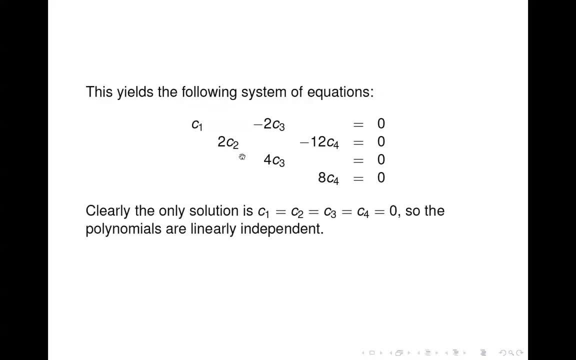 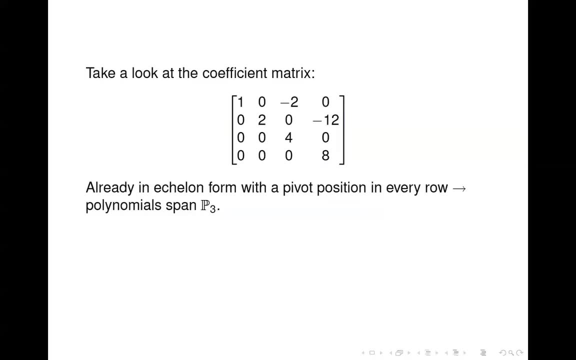 means that C1 and C2 have to be zero. all right, So we've shown here that the polynomials are linearly independent. Let's just look at it in matrix form. if we just look at the coefficients, it's already in echelon form, and we have a pivot position in every row. 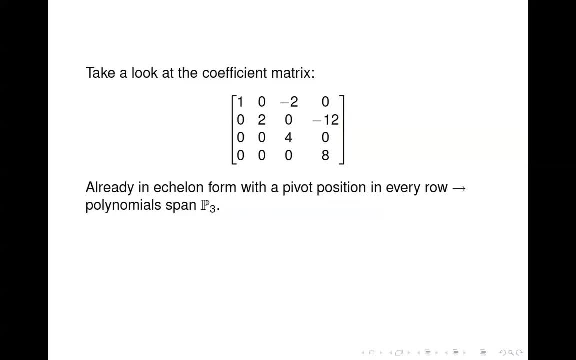 So from that we know that these polynomials must span P sub 3, so no matter what the right hand side is, there'll be a solution all right. So we have that they're linearly independent and they span P sub 3, so they have to be. 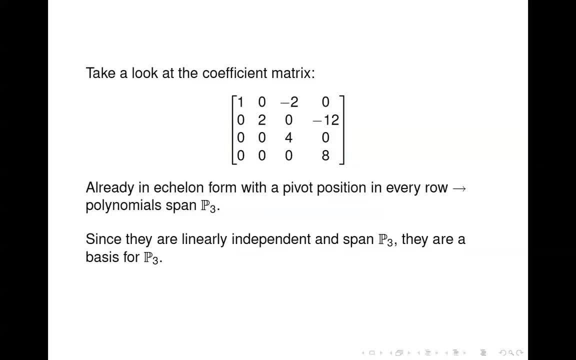 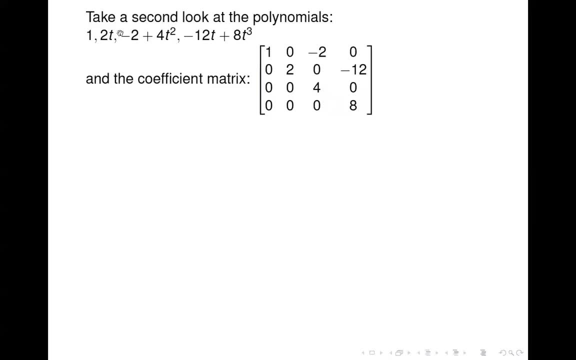 a basis for P sub 3.. Now, there's actually a somewhat easier way to look at this, and that is to look at the polynomials and what we ended up with And the columns of this matrix. Now, actually the way it works, is a polynomial of this form. here's a degree 3 polynomial. 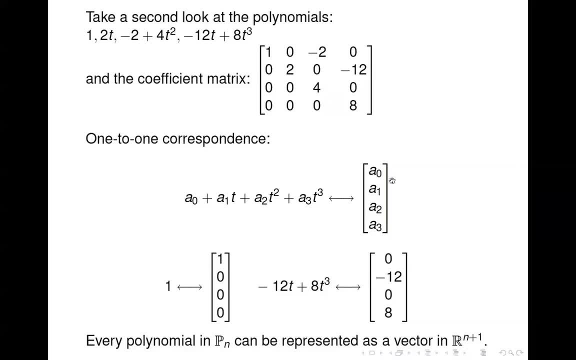 actually has a one-to-one correspondence with the vector in R4 that looks like this: First comes the constant term, then the coefficient of T, coefficient of T squared and the coefficient of T cubed. So, for example, our polynomial. one of them was just 1.. 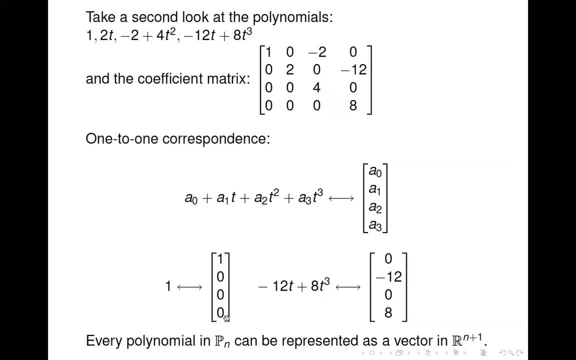 So that corresponds to 2. The vector 1, 0,, 0, 0, and R4.. And if you look, that's what the first column of this matrix, our coefficient matrix, was. And then just to pick another one, how about the last one? negative, 12T plus 8T cubed. 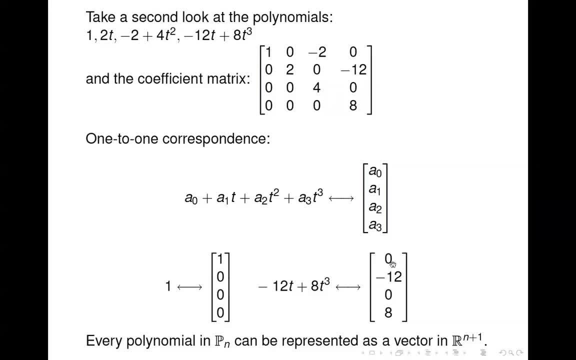 all right, Then that's going to have. that's 0 for the constant term negative, 12 for the coefficient of T, 0 coefficient of T squared and 8 for the coefficient of T cubed. And that's what the last column in our coefficient matrix looks like. 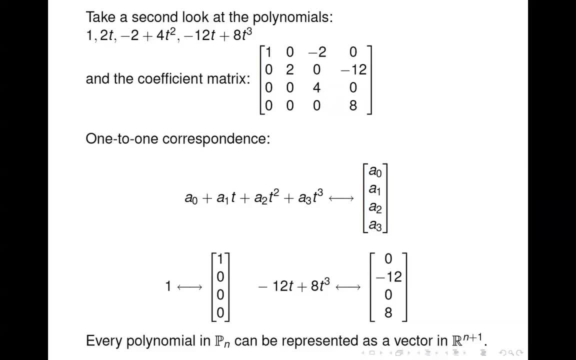 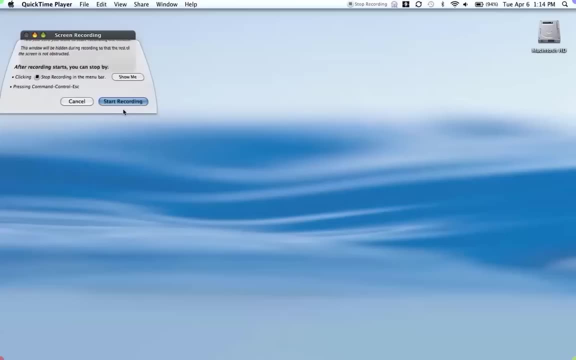 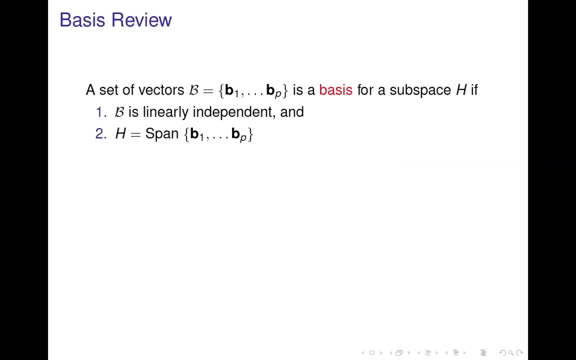 Bottom line is that every polynomial in P sub n can be represented as a vector in Rn plus 1. So there's a one-to-one correspondence between polynomials in P sub n and vectors in Rn plus 1.. All right, let's talk about the dimension of a vector space. 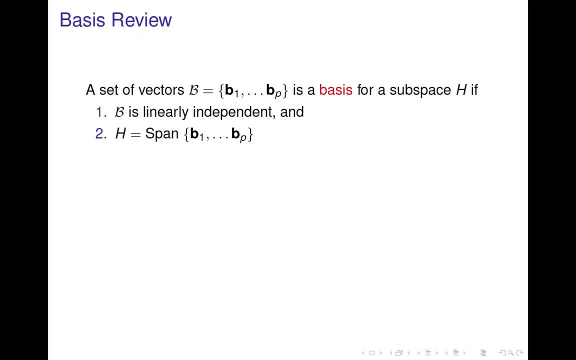 To do this, we need to go back and review what a basis is. So let's do that. Okay, Recall that a basis is a set of vectors that is linearly independent and spans the subspace that it's a basis for. So let's think about R3.. 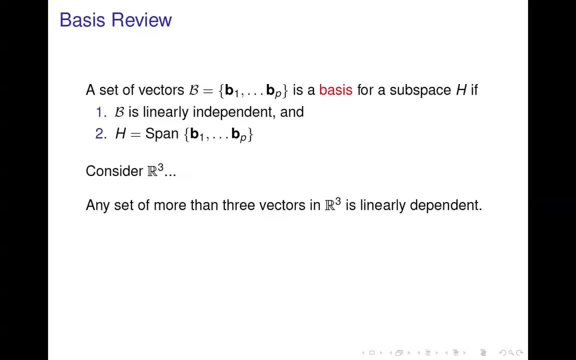 If you have more than three vectors in R3, then they must be linearly dependent. All right, If you put them in a matrix, put it in echelon form, then you would have free variables. If you have less than three vectors, then they don't span R3.. 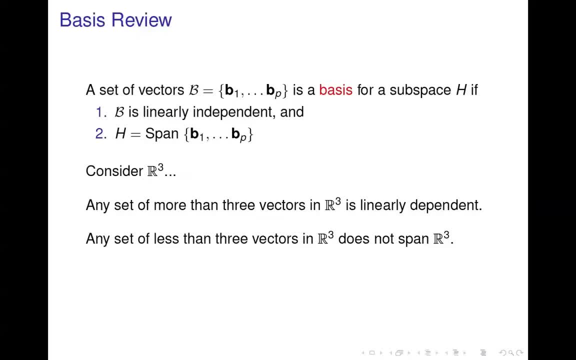 All right, If you had only two, you wouldn't be able to have a pivot position in every column if you stuck them in a matrix. So or wouldn't have a pivot position in every row. excuse me, So they would not be. they would not span R3.. 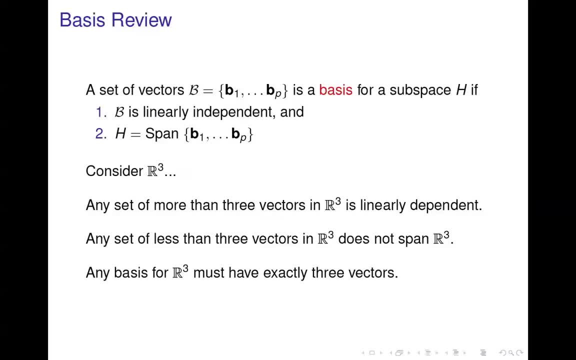 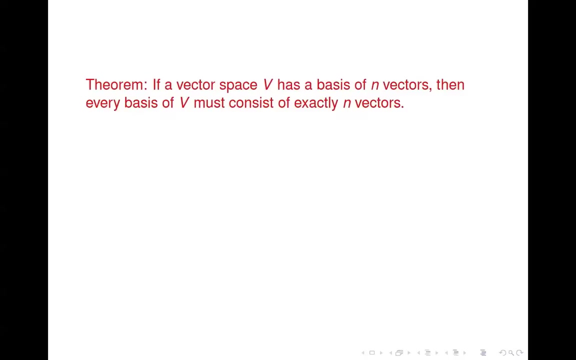 So put those two together. You need at least three to span. Okay. Uh, if you have more than three, they're linearly dependent. So that means that any basis for R3 has to have exactly three vectors. All right, Our theorem says that if a vector space has a basis of n vectors, then every basis for 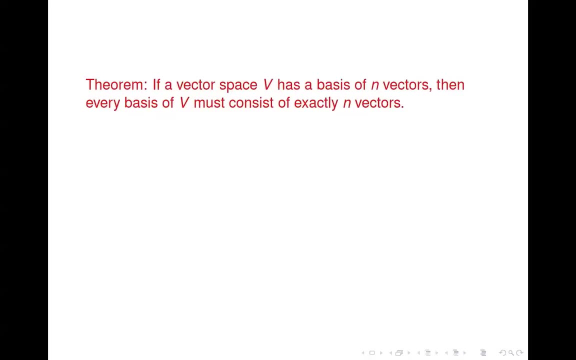 that space must have exactly n vectors, Um. this number of vectors in a uh basis, Uh basis for a vector space is called the dimension of that vector space. And we have a? uh, a special case where um uh, the vector space has only the zero element. 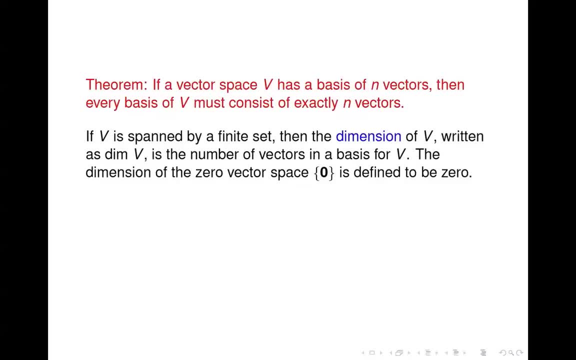 Okay, We call that the zero vector space, And since there's no basis for that set, then we define its dimension to be zero. Okay, So, to find the dimension of a vector space or subspace, Then one approach is simply to find a basis for that space and count the number of vectors. 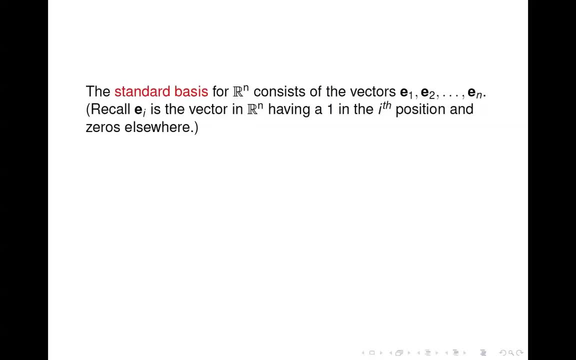 in that basis. Uh, the standard basis for Rn consists of the vectors e1 through en. So you might recall that uh e sub i is the uh vector in Rn that has a 1 in the ith position and zeroes out everywhere else. 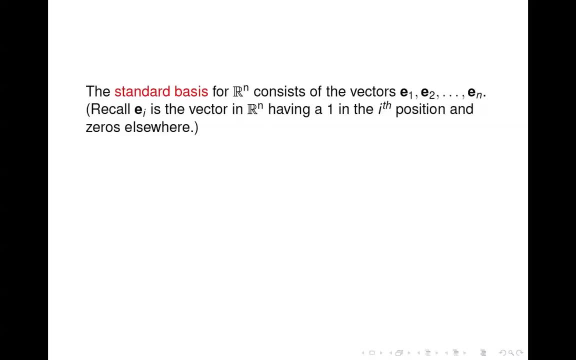 Or you can think of e, sub i as just the ith column of the eigenvalue. Okay, That's the 3 by 3 identity matrix. Uh, so the standard basis for R3 is, uh, uh, consists of these three vectors which you'll. 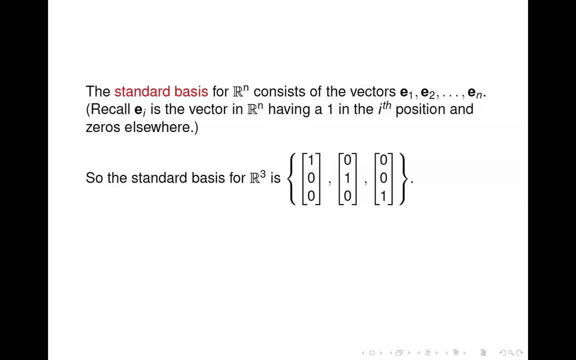 recognize as the columns of the 3 by 3 identity matrix. So, in general, the dimension of Rn is n. Now let's talk about polynomials. Uh, p, sub n, if you recall, is the set of polynomials of degree n or less. 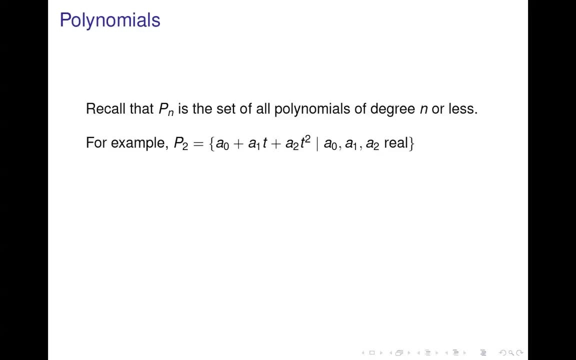 So, for example, p sub 2.. Uh Consists of all polynomials um that are quadratic or less, Okay, All polynomials that look like a naught plus a1 times t, plus a2 times t squared, where the uh a values are just real numbers. 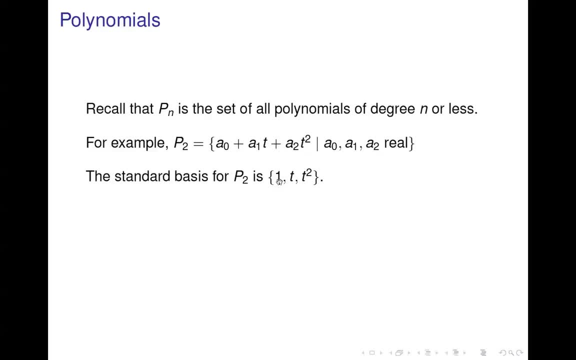 The standard basis for p sub 2 is uh. this set 1, t and t squared, So any vector in p sub 2, any polynomial in p sub 2, can be written as a linear combination of these three uh objects. 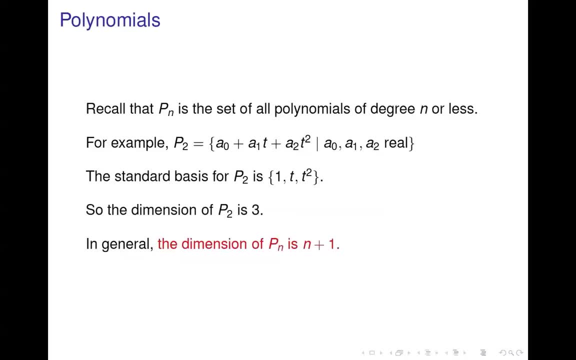 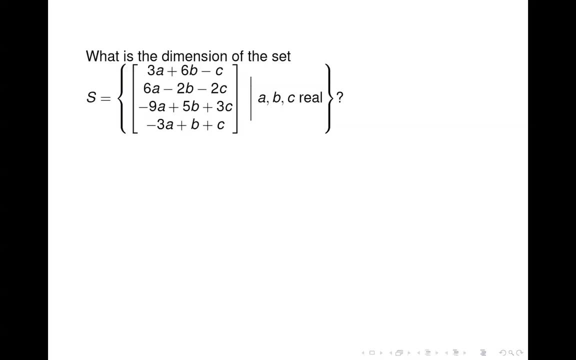 So the dimension of p sub 2 is 3.. And, in general, the dimension of p sub n is n plus 1.. Okay, what if we have a set like this: uh, defined, uh in terms of these parameters? 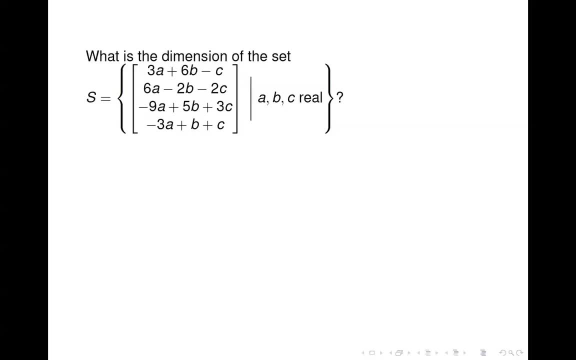 Um, how do we find the dimension of uh, such a set? Uh well, First let's find a basis, And to do that we can write uh, this generic vector, in parametric vector form, And uh. so at this point we know that these three vectors span our set s. 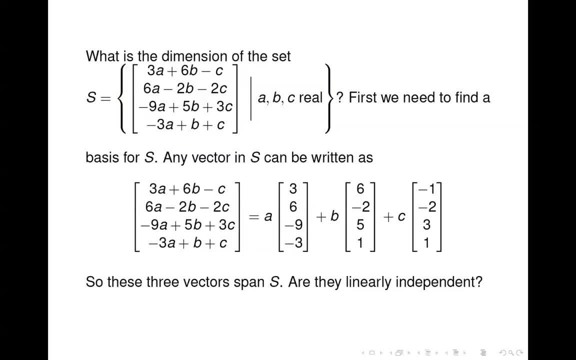 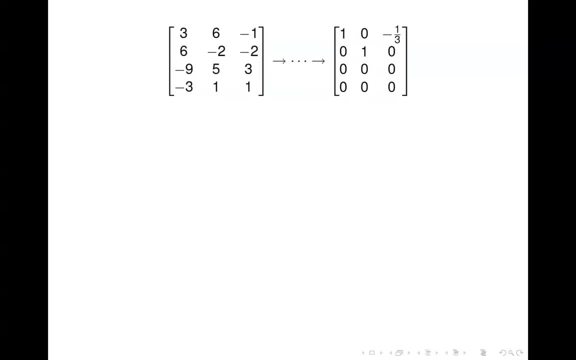 And so, excuse me. so we want to know, are they linearly independent? And to check to see if they're linearly independent, we throw them in a matrix. do some row operations? uh, get that in? uh, echelon or reduced echelon form. 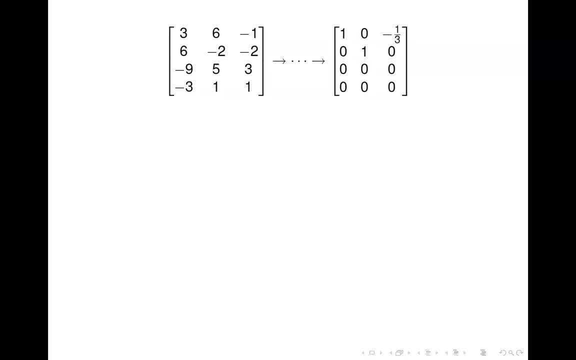 Uh, I, I got it in reduced echelon form, Okay, And uh, we can see here there's not a pivot position in every column. therefore, uh, they're not linearly independent. We can see that there's a pivot position in the first two columns, so that means that. 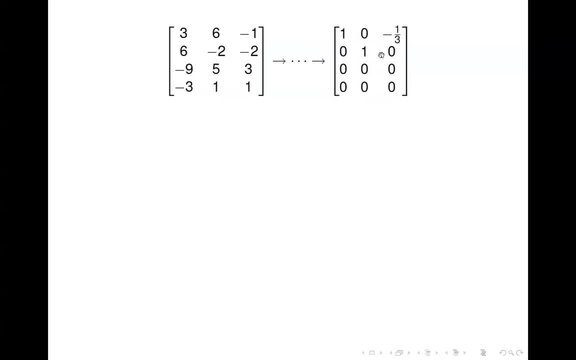 the first two vectors are linearly independent And notice that the negative one-third here means that the third column is minus one-third of the first column And if you look back, uh, that is, Uh, that is true. Minus one-third of three is negative one. 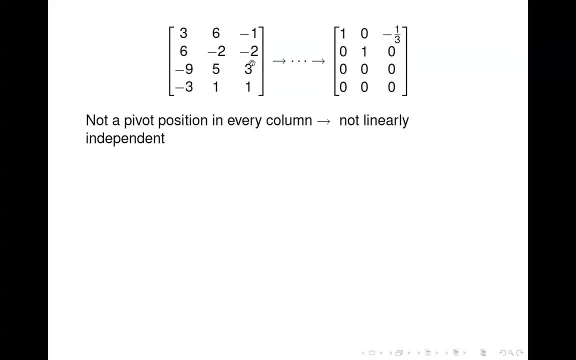 Minus one-third of six is negative two and so forth. All right, uh, so that means that that we can throw out that third column and a basis for s would just consist of the first two vectors. And once we have a basis, then we need to only count the vectors in the basis to get. 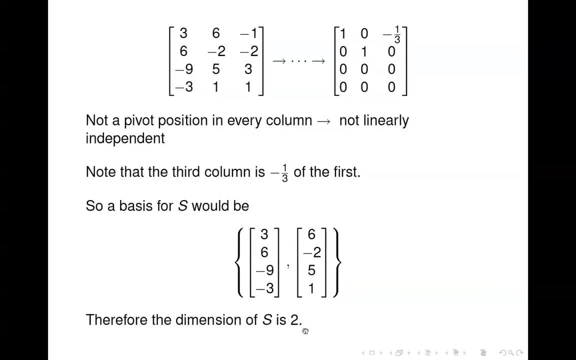 the dimension. So there's two vectors in the basis. That means the dimension of s is two. And uh, we don't say that s is r2, okay, because it's not, because these vectors are in r4. But what we do say is that s is a two-dimensional subspace of r4, right? 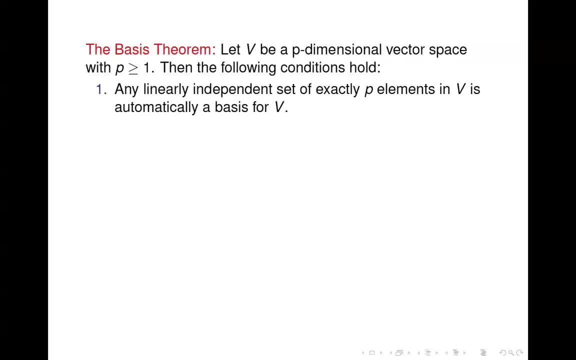 The basis theorem. this is an important theorem. It says that if you have a vector space with dimension p, where p is greater than or equal to one, Then the following conditions hold. Number one: any linearly independent set of p elements in v is a basis for v automatically. 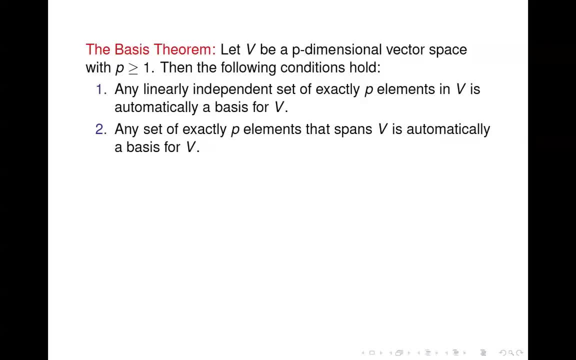 Don't have to check to see if it spans. Similarly, any set of p elements that spans v is automatically a basis. okay, Don't have to check to see if it linearly independent. All right, so, since we know, the dimension of r3 is three. 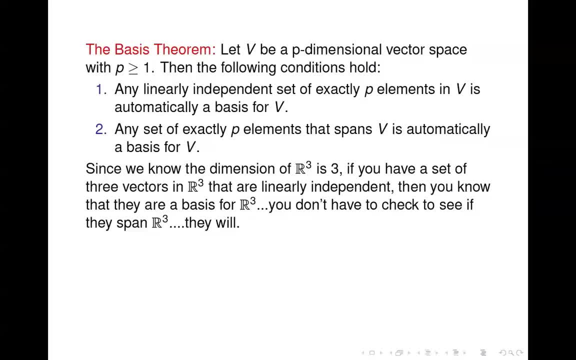 If you have a set of three vectors In r3 that are linearly independent, then you know they're a basis. You don't have to check to see if they span, because they will. Similarly, if you have a set of three vectors that span r3, then you know they're a basis. 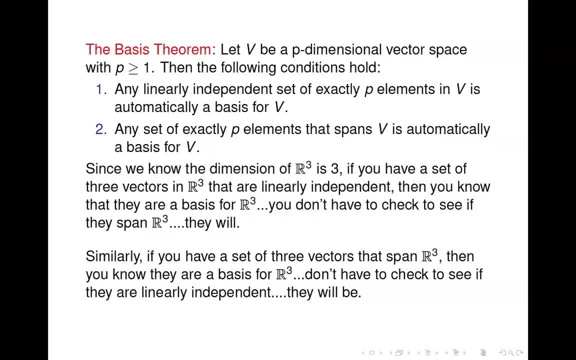 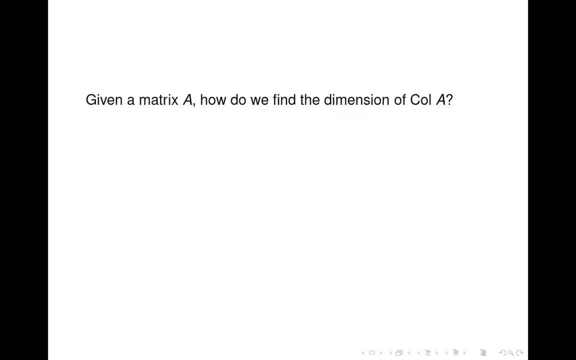 for r3.. You don't have to check to see if they're linearly independent, because they will be okay. So we basically end up with three pieces of the puzzle. Um, let's go back to that. Three pieces of the puzzle. 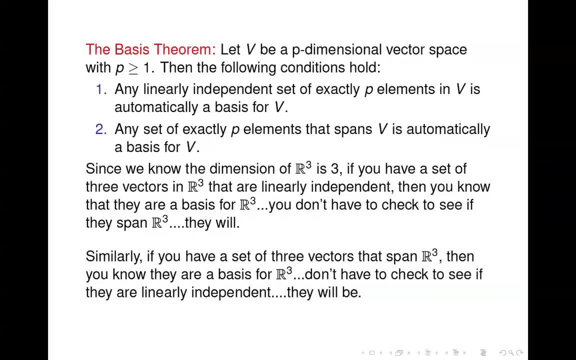 Knowing the dimension, Having a set uh of that many vectors that spans, or having a set of that many vectors that's linearly independent. If you have any uh two of those three pieces, then you can conclude that you have a basis. 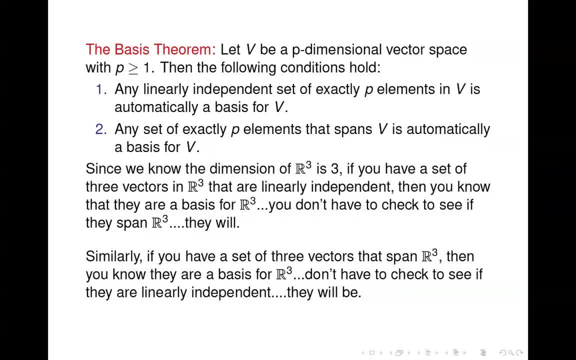 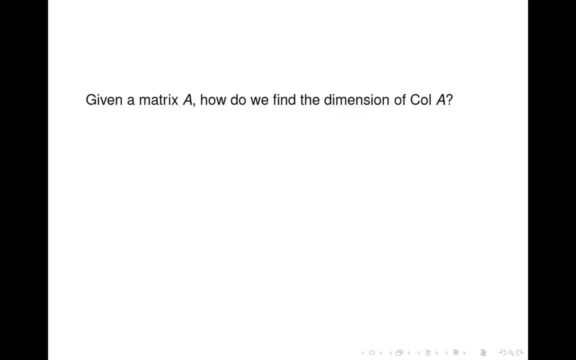 for the vector space you're dealing with. Okay, um, for, given a matrix A, how do we find the dimension of the column space of A? Well, we go back to our method: Find a basis and count the number of vectors in the basis. 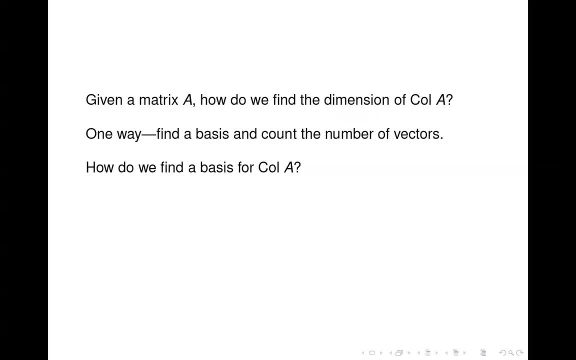 Now let's think back. how do we find the basis for the column space of a matrix? We will put A in echelon form, uh, so that we can find the pivot columns. We pull those columns from A. alright, not from the echelon form, but from the original. 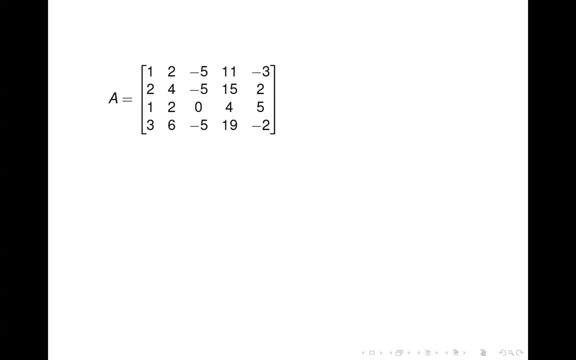 matrix A and that's our basis. So here's uh one. I think we looked at this one last time. Um, We take the matrix A, put it in echelon form. uh, we can see that the first third and 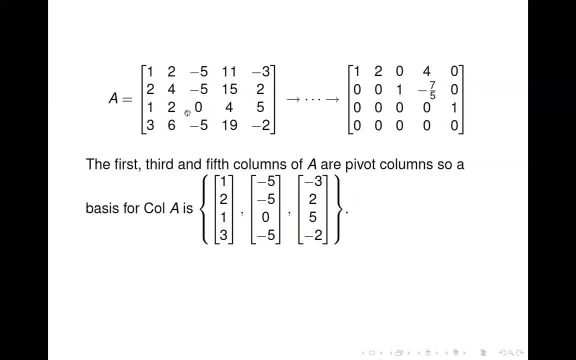 fifth columns are pivot columns. so we pull the first, third and fifth columns from A and that's a basis for the column space of A. And once you have a basis then, uh, getting the dimensions trivial, there's three vectors in the basis. so the dimension of the column, 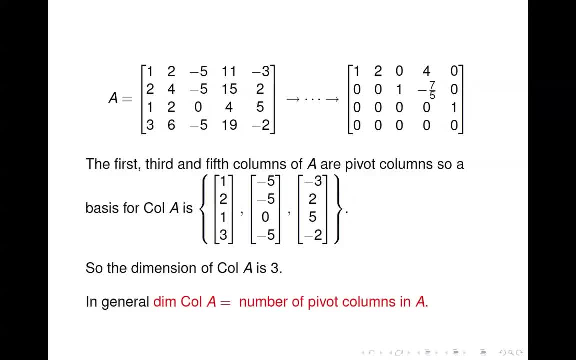 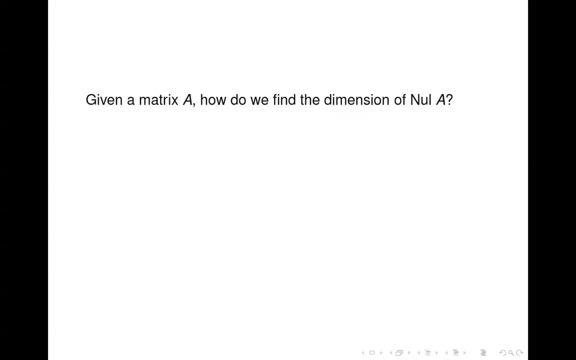 space of A is three. In general, the dimension of the column space of a matrix is simply equal to the number of pivot columns in the matrix. Alright, how about the null space? We have a matrix A. how do we find a basis, or how do we find the dimension of the null? 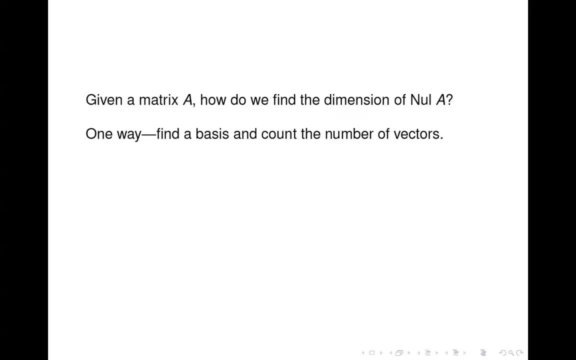 space of A. Well, once again find a basis and then count the number of vectors. So let's uh think back. how do we find a basis for the null space of a matrix? Uh well, we have to solve: AX equals zero and write the solution in parametric vector. 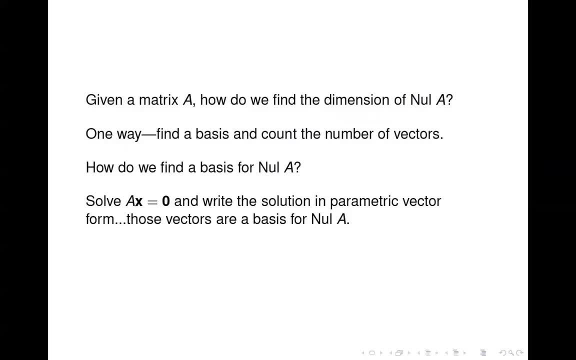 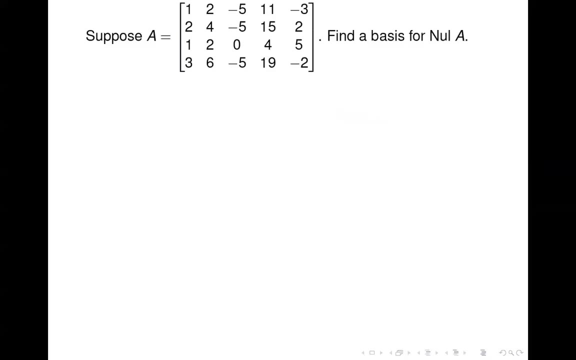 form And the vectors that we get there. Uh, both span the null space of A and they're linearly independent. We made that argument last time that when you write those in parametric vector form they will be linearly independent and therefore they'll be a basis for the null space of A. 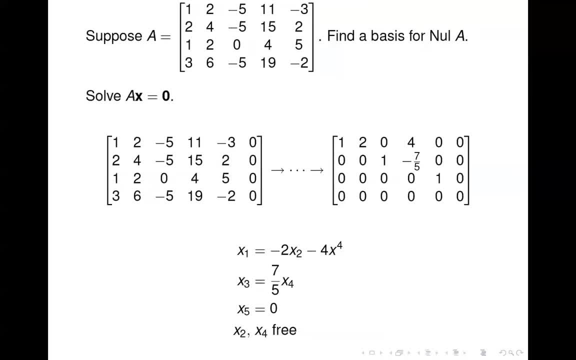 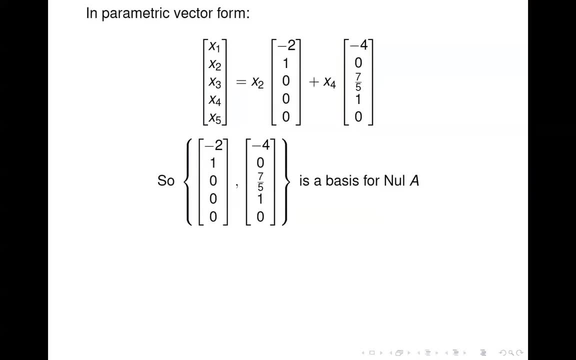 So if we start with this matrix A, we solve: AX equals zero, um, and uh, write the solution in parametric vector form. Uh, we get these two, We get these two vectors and uh, they are, oops, that should. yeah, X five is zero, right. 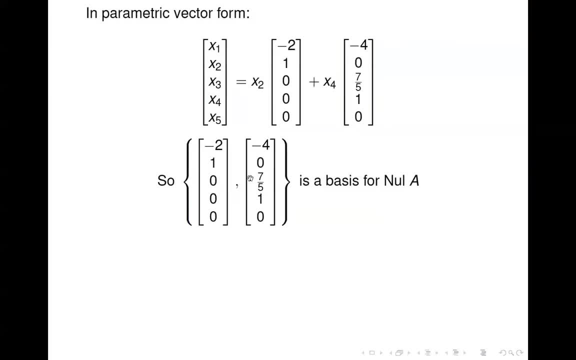 Yep, X, five is zero, so that that's right. Um, so these two vectors are linearly independent. they span the null space, so they're a basis for the null space. Therefore, the dimension of the null space for this particular matrix is two. 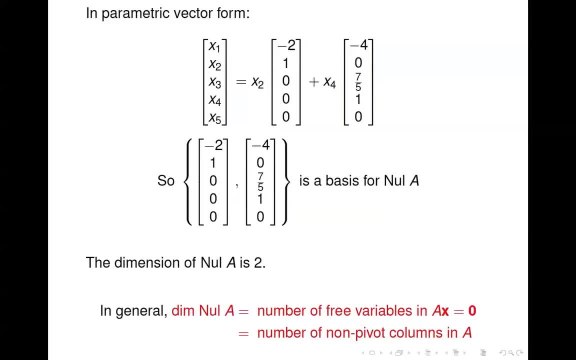 Now, in general, the dimension of the null space is equal to the number of free variables In AX. equals zero, right, because that's you have a vector here corresponding to each free variable. and where do free variables come from? They come from columns that don't have a pivot position. so the dimension of the null space 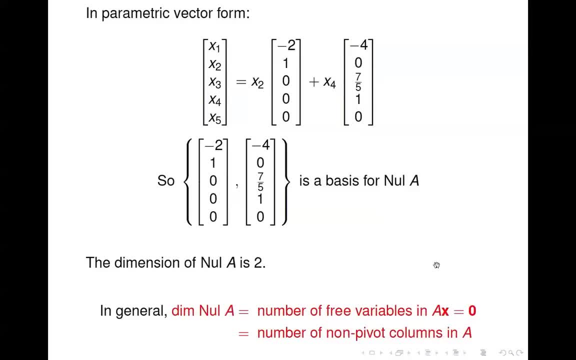 is equal to the number of non-pivot columns. in A Recall, dimension of the column space is: the number is equal to the number of pivot columns. Null space dimension is equal to the number of non-pivot columns. So if we add those two quantities together, the dimension of the null space plus the dimension 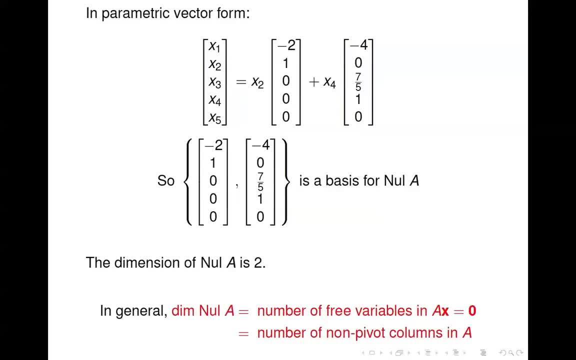 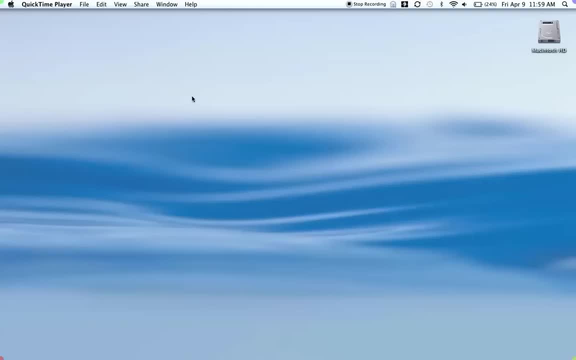 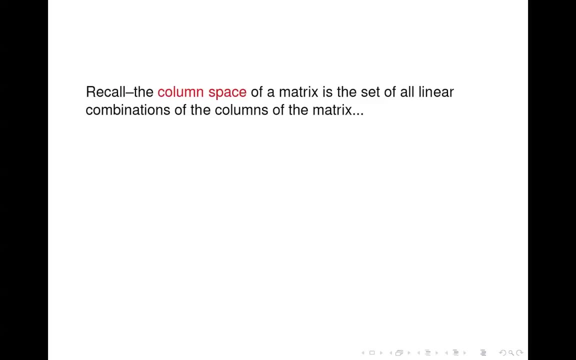 of the column space, we get the number of pivot columns plus the number of non-pivot columns, which is equal to the number of columns, and we'll hit on that some more next time. All right, let's uh move on to talk about the rank of a matrix today. 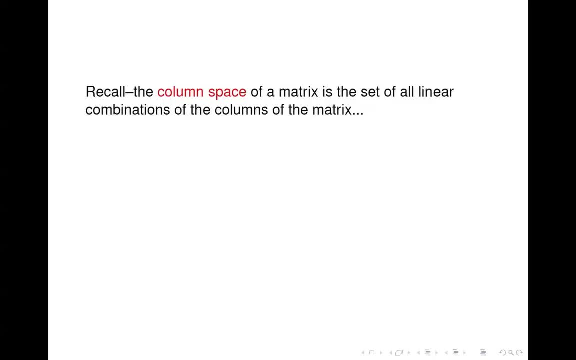 Now, first a little bit of review. Um, remember, the uh- columns Column space of a matrix is the set of all linear combinations of the columns, which is also the span of the set of columns of the matrix. So we're gonna talk about, uh, another subspace, um, this time the row space of a matrix. 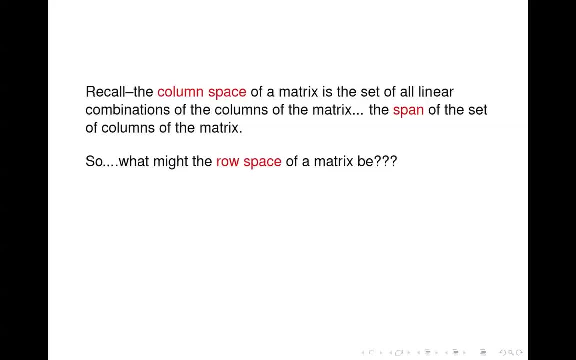 So we know what the column space is. so what do you think? the row space of a matrix, uh, is Mm. well, Take the analogous uh route, then we get uh. the row space of a matrix is the set of. 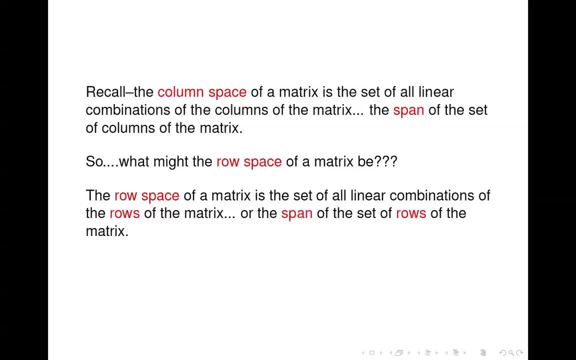 all linear combinations of the rows or the span of the set of rows of the matrix. So it is truly just the analogous uh term to the column space. Okay, we have the column space, all linear combinations of the columns. row space, all. 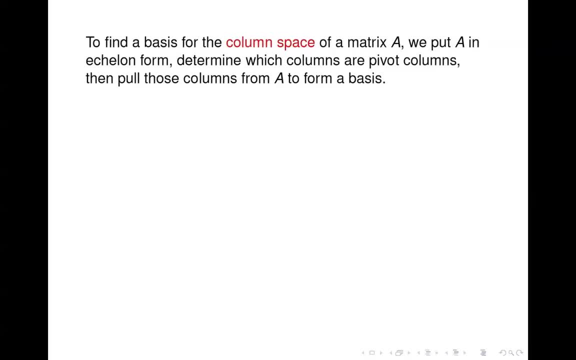 linear combinations of the rows. Okay, So think back. Okay, So we have a basis for the column space of a matrix. uh, we put the matrix in echelon form so that we can determine which columns are the pivot columns. Then we go back to the original matrix and pull out those columns and that's a basis. 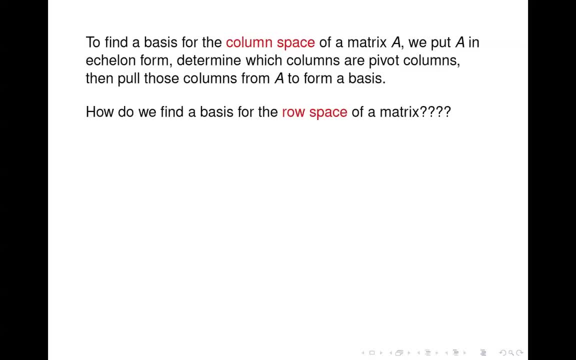 for the column space of the original matrix. So the question is: how do we find a basis for the row space of a matrix? And here, uh, the similarities end somewhat, although there still are some similarities, Um, But this theorem tells us how we can find a basis for the row space of a matrix. 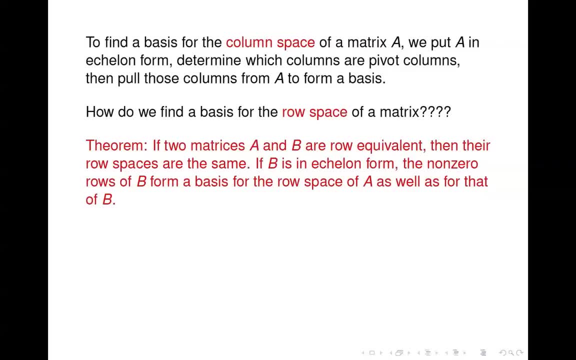 Okay. So it says if two matrices, A and B, are row equivalent, all right, so you can get from one to the other doing elementary row operations. then their row spaces are the same. Now you'll recall that that is not true for the column spaces. 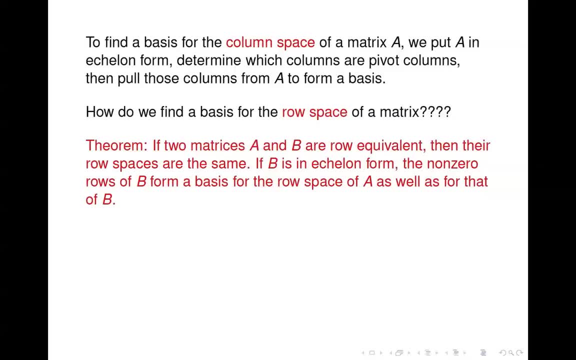 When you do elementary row operations you may be changing the column space of the matrix, But this theorem tells us that that for row space That stays the same when you do row operations. Okay, If B is in echelon form, the non-zero rows of B form a basis for the row space of A, as 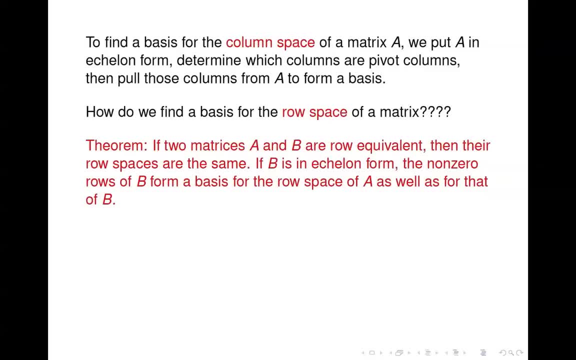 well as for that of B. Okay, So this tells us to find a basis for the row space of A. We put it in echelon form and pull the non-zero rows from that echelon form matrix and we have, uh, a basis for the row. 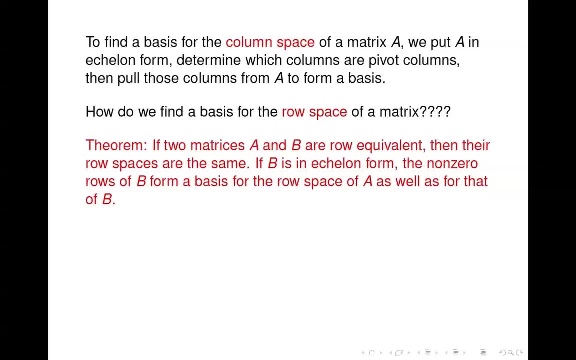 space of the original matrix Plus, uh, the echelon form matrix and any uh intermediate matrices that we encountered. All right, So again, elementary row operations: um, do not change uh this back up here, uh this. 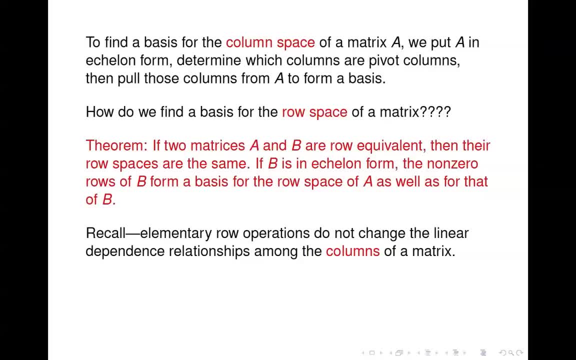 is talking about the linear dependence relationships among the columns. Okay, So that means like if the second column of A is, uh, 10 times the first column, then when you do elementary row operations that doesn't change. So elementary row operations do not change the linear dependence relationships among 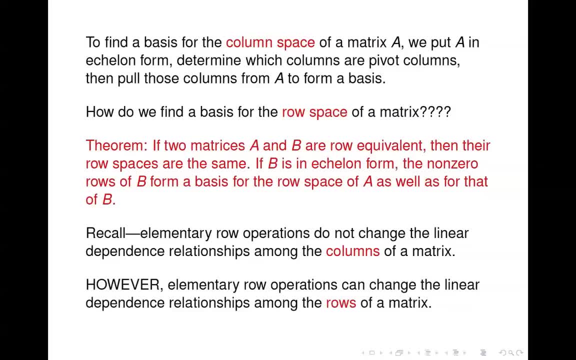 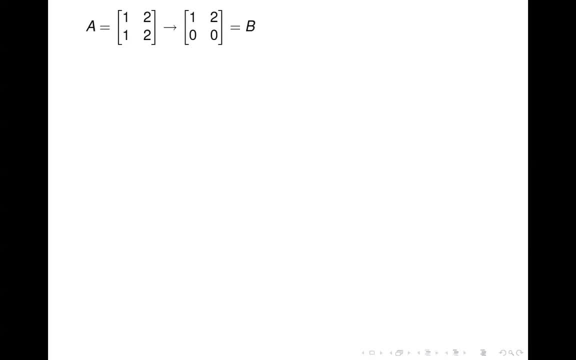 the columns of a matrix. However, they can change the linear dependence relationships among the rows of a matrix. Okay, So let's look at a little simple example. We start off with this matrix A. uh, we do uh. one row operation end up with this one. 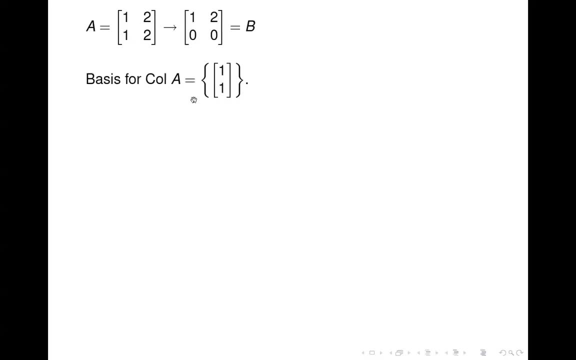 which I'll call B, Now a basis for the column space of A. all right, we, um, we could just look at A and say: well, I can see that the second column is a multiple of the first, so I throw it out and just keep the first column. 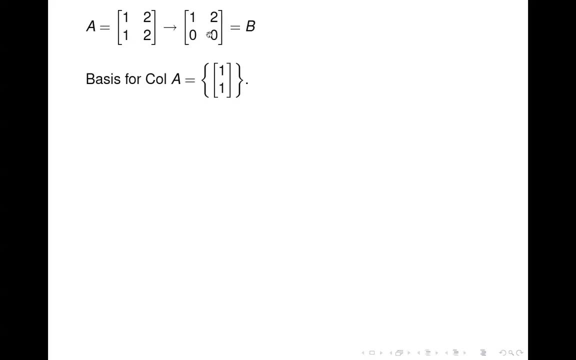 Or you could look at B and see where the pivot positions in B. well, there's only one in the first column. So that means we want to pull the first column for A from A, uh, to be a basis for the column. 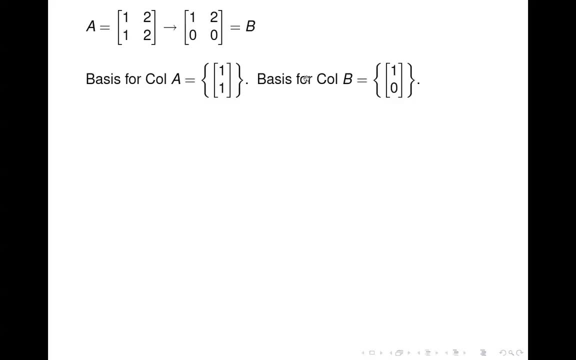 space of A. Um, if we want a basis for the column space of B, that's. that's straightforward, because B's already in echelon form, So we just pull. We know what the pivot column is. Okay, The pivot columns are: there's only one first column, so that's a basis for the column space. 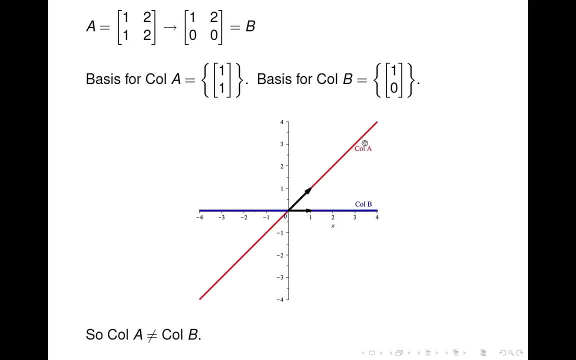 of B. Okay, So if we look graphically at the column space of each of these matrices, okay, the red line here, um, you can see this vector right here. this is one one, and so this red line is any multiple of the vector one one. 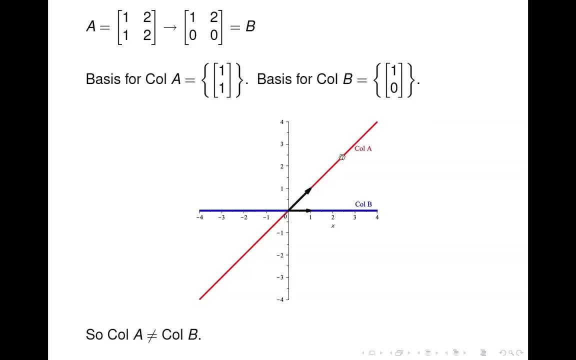 So that's the red line, is the column space of A. Uh, this vector here is one zero, And since that's a basis for the column space of B, the blue line, or the X axis, is the column space of B. right, 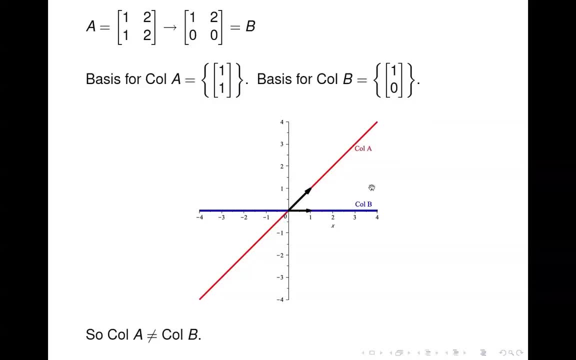 All multiples of one zero. So clearly here, these- uh column spaces are not the same, right? They, uh, these matrices are row equivalent, but their column spaces are not the same. All right, Let's look again. 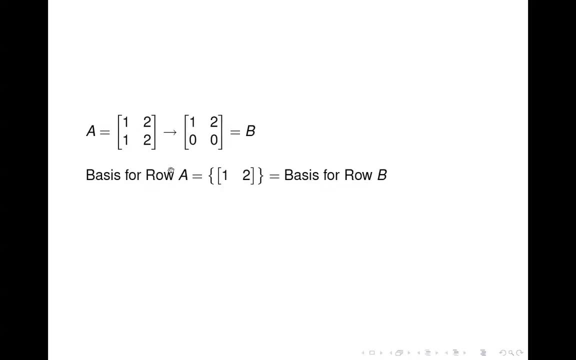 Same set of matrices. Now, the row spaces are the same, because if we want a basis for the row space of A, then right, we look at each row of A. well, they're the same row, right? Each row is the same and so we only need one of them. 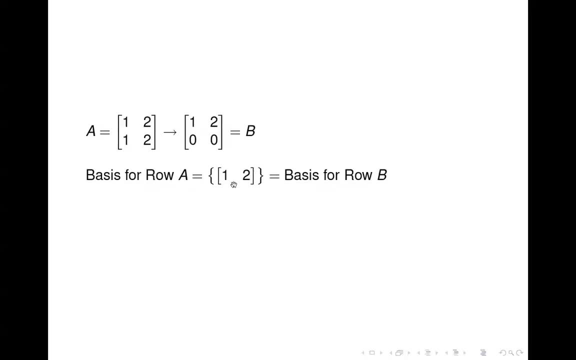 Throw out the second one and we keep the first row and that's a basis for the row space of A. All right, If we were using the theorem, we would get A in echelon form, which we have here, and take the non-zero rows of that matrix. 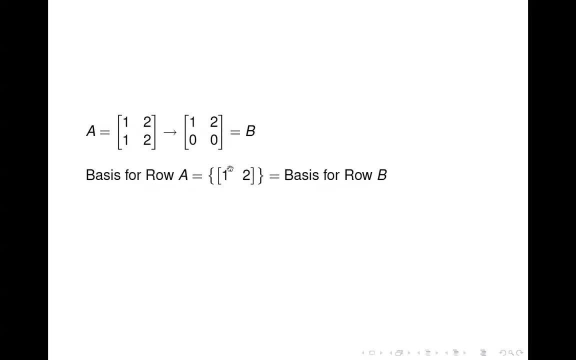 Well, the non-zero rows is just that row. Okay, It's a row one- two. So, either way you look at it, you end up with this basis for the row space of A And similarly for the row space of B. um, it's gonna be all multiples of the row one two, because 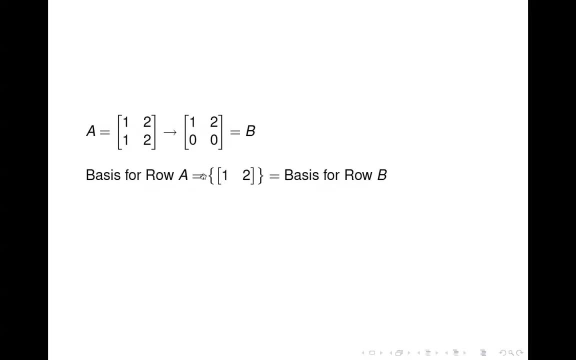 zero, zero didn't add anything to the picture. So this set, which consists of just that one row, is a basis for both the row space of A and the row space of B. Now let's look at a little, uh, a little more. 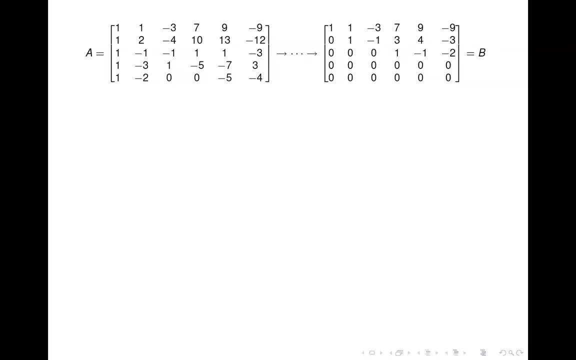 uh, interesting example. Um, there's a big matrix A and uh, after some row operations, we end up with this version of A. Okay, this is an echelon form and we'll call that matrix B. Okay, so to get a basis. 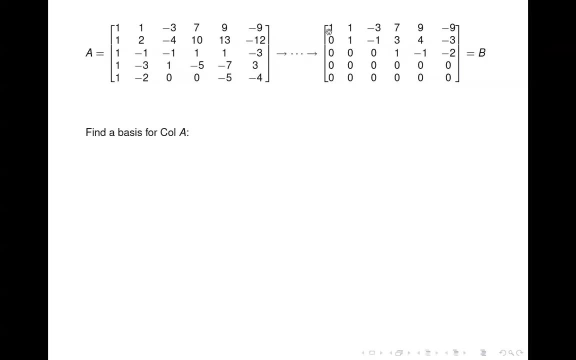 for the column space of A. we look at B. We can see that there's a pivot position in the first column, the second column and the fourth column. So we choose those columns out of A- First column, Second column And the fourth column. 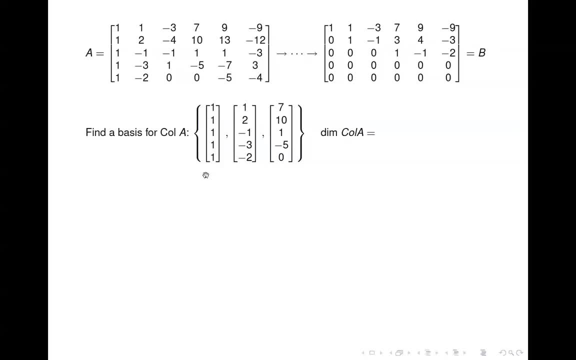 And that's a basis for the column space of A. So the dimension of the column space of A is the number of vectors in this basis, which is three. To get a basis for the column space of B, um, we look at B, It's already an echelon. 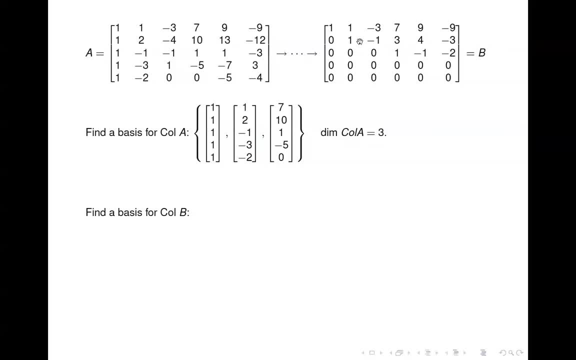 form. so we choose the non, uh, choose the pivot columns, And so we get the first, second and fourth columns, That's columns, the basis for the column space of B And the dimension of the column space of B, count the vectors in a basis that's three. 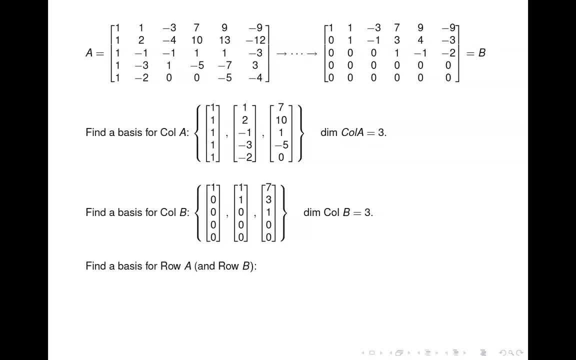 So the dimension of the column space of B is three. Um, alright, what about a basis for the row space of A, which, we know from the theorem, will also be a basis for the row space of B? Well, according to the theorem, put A in. 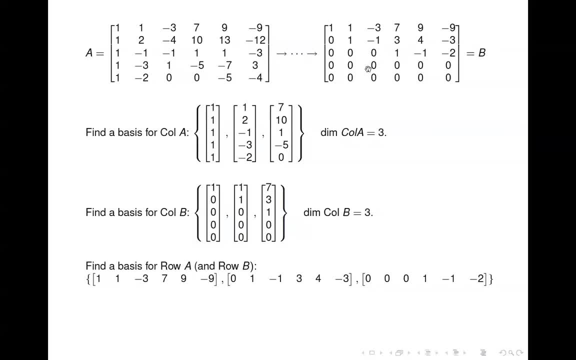 echelon form and choose the non-zero rows. So we do that. we get the first, second and third rows of B which are given here. Okay, So the dimension of the row space of A is equal to the dimension of the row space of 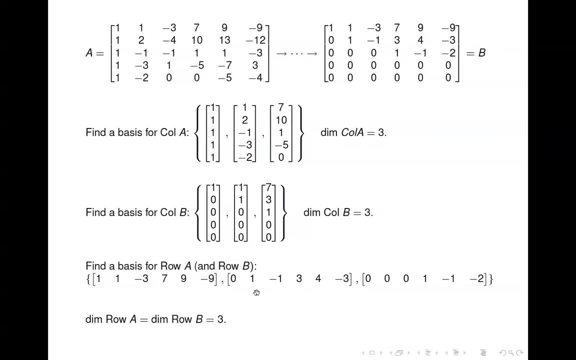 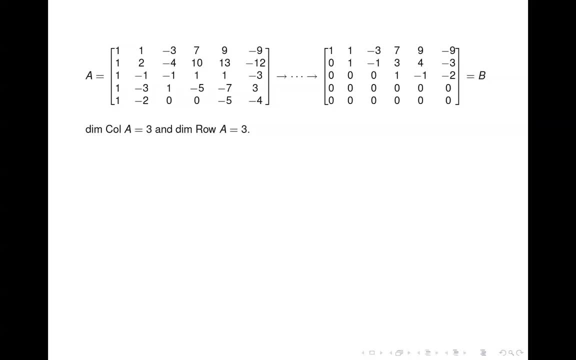 B and notice there's three vectors here, so that is three. Alright, so we got the dimension of the column: space of A is three. dimension of the row: space of A is three, and the question is: is this a coincidence that they're both the? 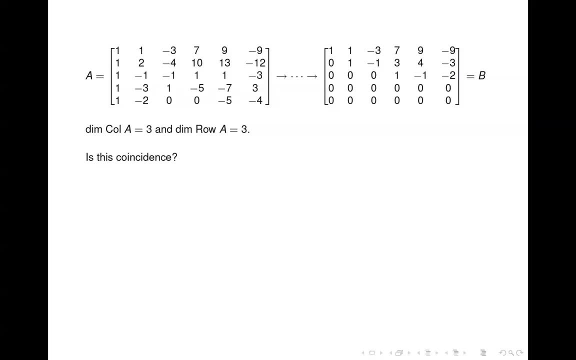 same value And, uh, if you think about that just a little bit, Uh, You can say no, um, I don't think so, because the dimension of the column space of A is the number of pivot columns or pivot positions in A, And that's uh, when we look at B to 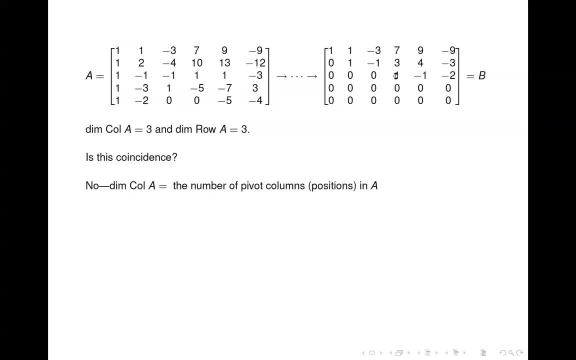 figure that out. but there's three pivot positions And, uh, the dimension of the row space of A is also equal to the number of pivot positions, because there's a pivot position in each non-zero row, in B, here, or in an echelon form of A. 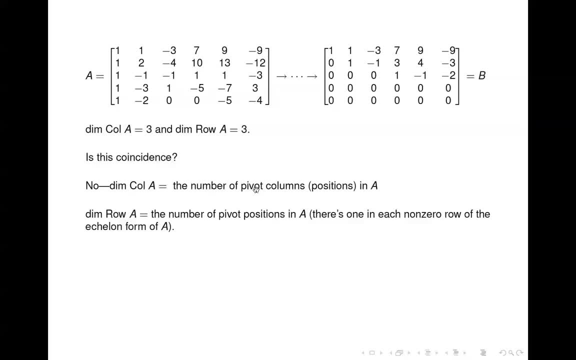 So So Each of these values is based off of the number of pivot positions. right, because a pivot position defines a pivot column, and a pivot position defines a non-zero row. So, uh, for any matrix, the dimension of the column space is equal to the dimension of 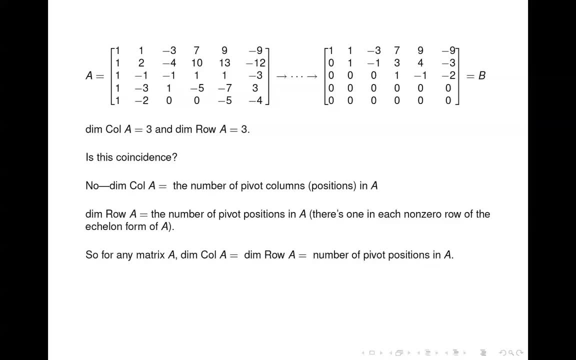 the row space, which is equal to the number of pivot positions in that matrix. Okay, and this quantity is what we call the rank of a matrix. Okay, the rank of a matrix is the dimension of the column space, which is also equal to. 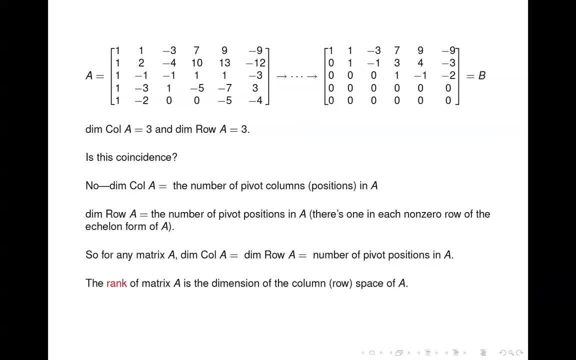 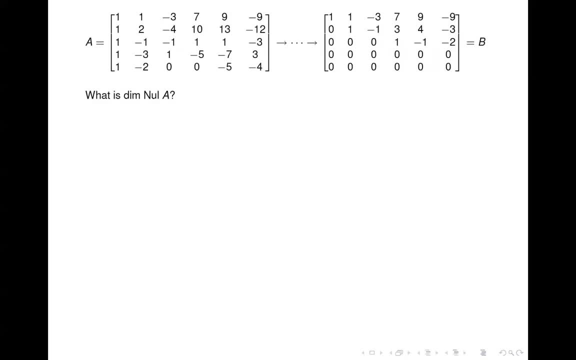 the dimension of the row space of that matrix. Okay, so we just call that the rank of the matrix. Alright, back to this one. let's talk about the null space. Uh, what is the dimension of the null space of A? 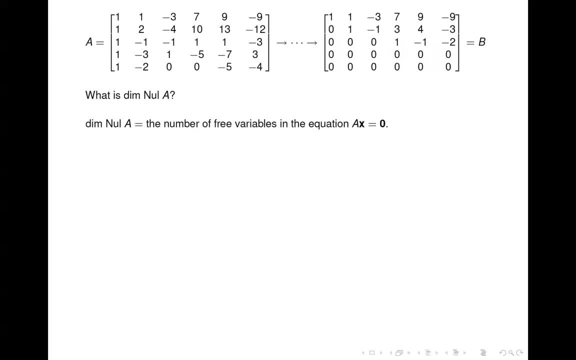 Well, we end up with a. uh, uh, uh. we want to find a basis for the null space. Okay, In this case, right, we um solve AX equals zero and write our solution in parametric vector form, and those vectors will be a basis for the null space of A. Now, um, how many? 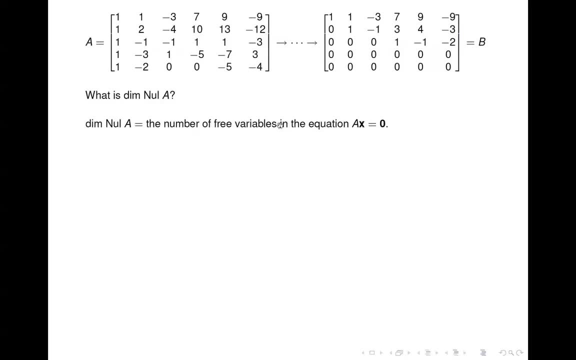 vectors do you end up with in that case? Well, you end up with one for each free variable. okay, Key is one for each free variable. And if you think about that a little more, you think: hmm, well, where do I get a free? 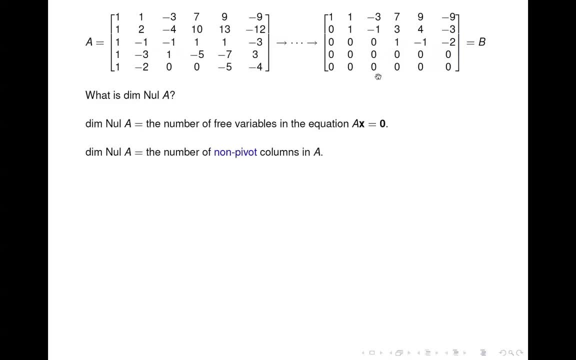 variable. Well, it's uh Uh. a free variable is one whose column does not contain a pivot position. So the dimension of the null space is the number of free variables. uh, in AX equals zero, also equal to the number of non-pivot columns in the matrix. okay, 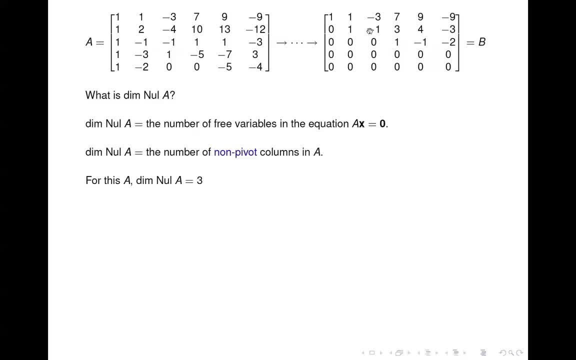 For this particular matrix, the dimension of the null space is three, because here's a non-pivot column. uh, the third one and the fourth, and oh, fifth and sixth. So the third column, fifth column, sixth column. 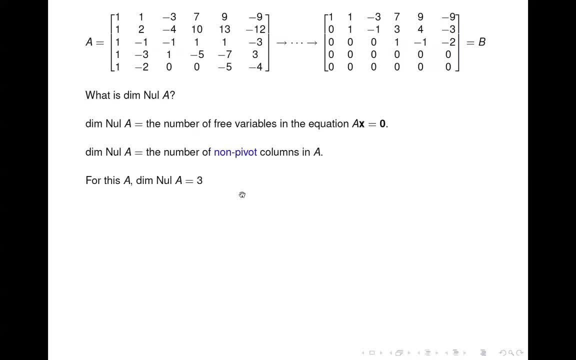 They're all non-pivot columns. So we have three non-pivot columns and therefore the dimension of the null space is three. Alright, so once again this number three pops up. We have: dimension of the column space is three. dimension of the null space is three. 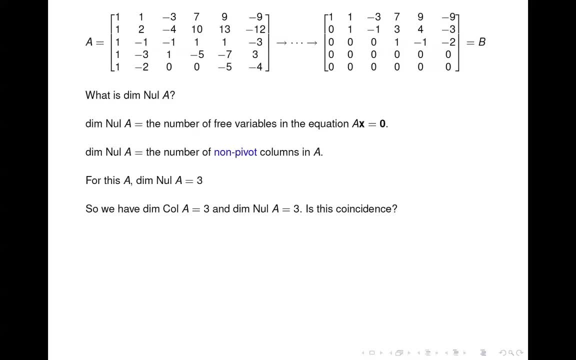 So I ask again: is this a coincidence? Hmm, and the answer is yes, it is a coincidence. It's coincidence because um dimension of the column space is the number of pivot columns. Dimension of the null space is the number of non-pivot columns. 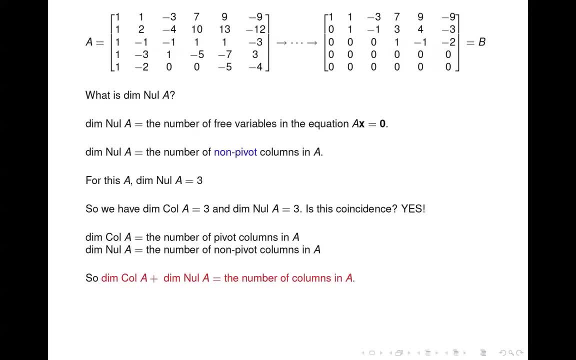 So when you add them together, you get what? The number of columns in the matrix? Um, so it just so happened that there were six columns in this matrix, and so if the dimension of the column space is three, then the dimension of the null space is gonna be. 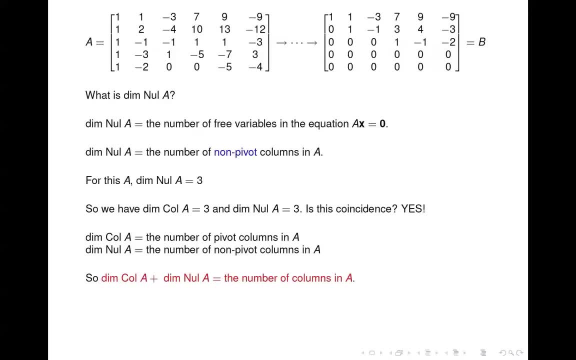 six minus three, which is also three. So that's totally coincidence. Had there been seven columns, The dimension of the null space would have been four. Alright, so we have the dimension of the column space plus the dimension of the null space is equal to the number of columns. 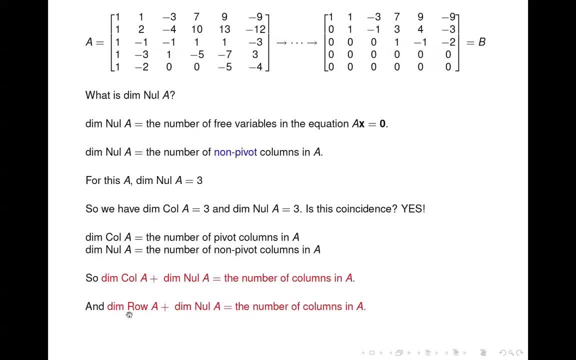 And since the dimension of the column space is equal to the dimension of the row space, we have the dimension of the row space plus the dimension of the null space is equal to the number of columns. And one more time: since the dimension of the column space and the dimension of the 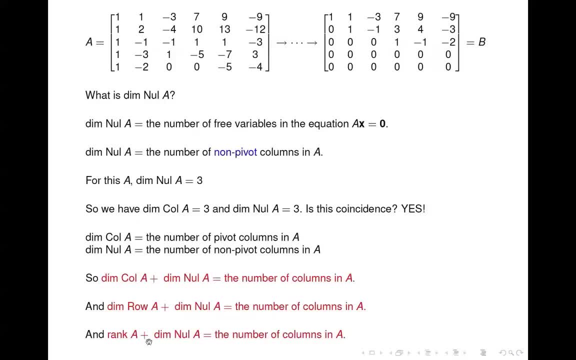 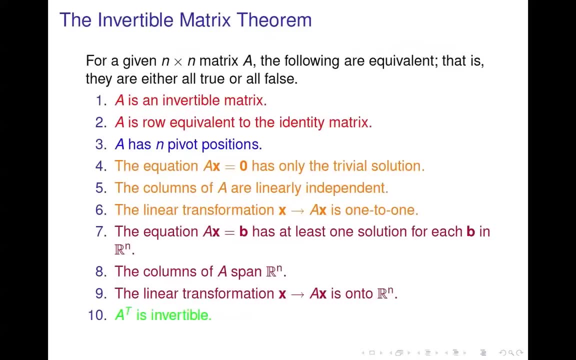 row space are equal to four, And since the dimension of the column space is equal to the rank of A, we have the rank plus. the dimension of the null space is equal to the number of columns. Okay, so in this section we have another installment of the Invertible Matrix Theorem. 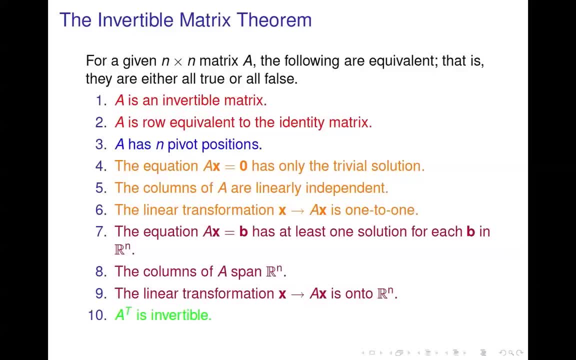 And, if you recall, we had this version of it or this installment of it back in section 2.3. Um and uh. so this should be Okay Seared into your memory at this point. If not, you can go back and review it. 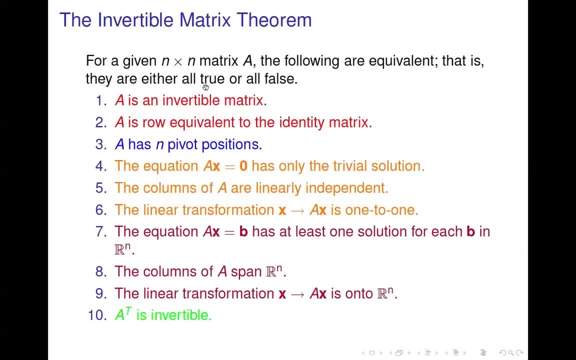 Um, but uh, one of the pertinent things is: uh, uh, recall that the whole idea here is that all these statements are equivalent, uh, which means that they're either all true or all false. Number one here says: A is an invertible matrix. 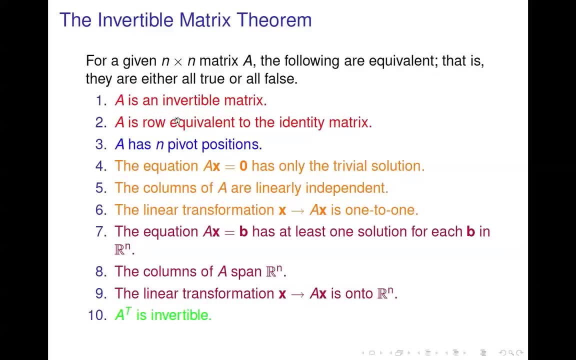 Now, one of the most important pieces of this is number three, that A has n pivot positions. Because if you recall- Okay, If you don't know how to uh remember all this- I told you the easiest way is to relate everything to pivot positions. 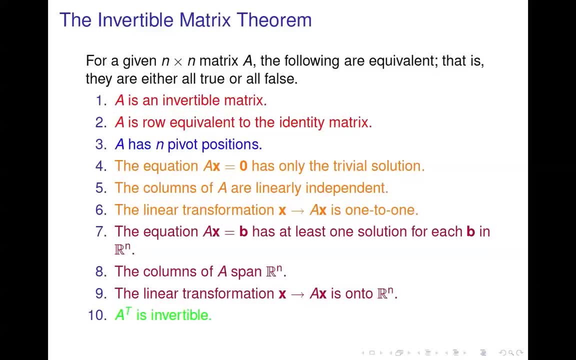 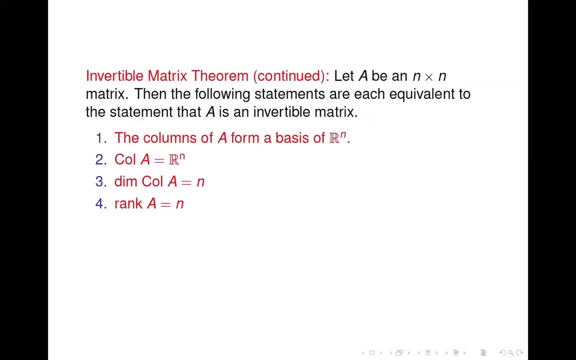 So if we can establish- uh for any part of this- that A has n pivot positions, then we're done All right. So what we have new here? uh, we have six new things. Four of them are given here, So let's take a look at these. 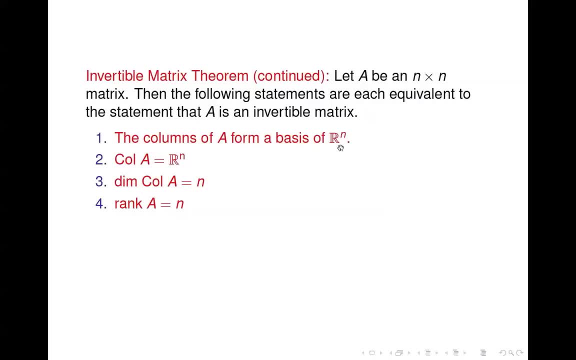 Uh, number one says the columns of A form a basis for R. Okay, Um, if that's true, if they're a basis for Rn, then that means, uh, that they must be linearly independent and they must span Rn. 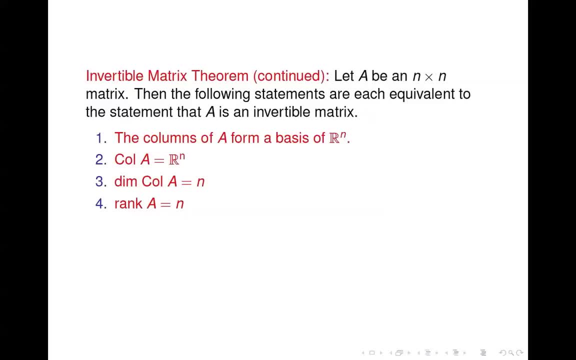 Either one of those says that there's a pivot position in every row and every column. Therefore they're n pivot positions. So A is invertible. Uh, the column space of A equals Rn. Uh, that means that, uh, the columns of A span, Rn. 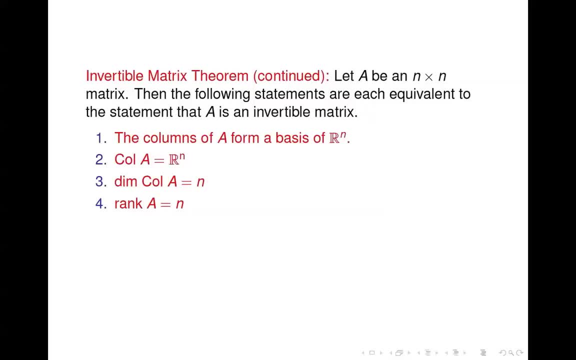 Uh, that means that, uh, the columns of A span Rn, Which, again, they can only do that if there's a pivot position in every row, meaning there's n pivot positions. The dimension of the column space is n. Um, that actually falls from number two here. 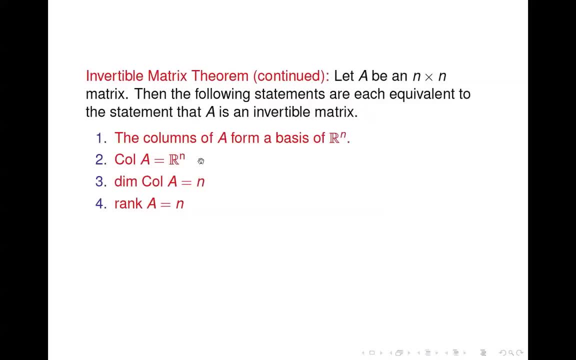 Um, if column space of A equals Rn, we know that they're n vectors and a basis for Rn. So therefore, the dimension of the column space is n And the rank of A equals n. That falls from number three, since the dimension of the column space 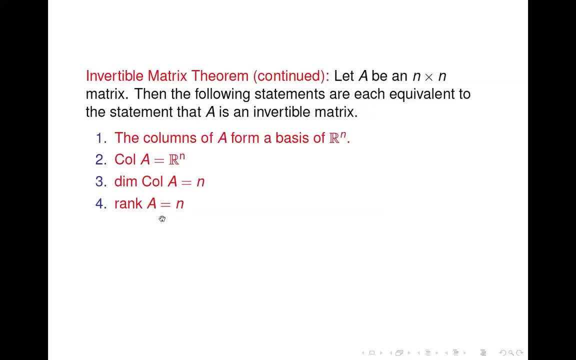 The column space is equal to the rank of a matrix. Okay. then we have two more that deal with a null space. Um, null space of A is just the zero vector. Okay. So if that's true, then that means that if we look at the system, Ax equals zero. it has. 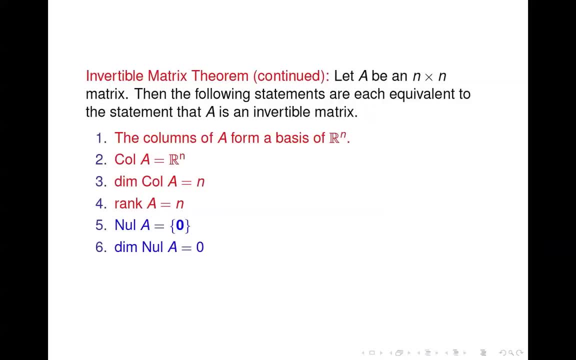 only the trivial solution. That happens when there are no free variables, which means there's a pivot position in every column, which means they're n pivot positions, And uh, from number five follows number six, because uh, the if you have only the zero. 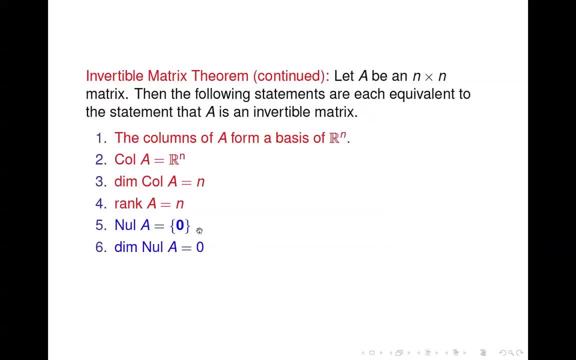 vector, uh, then that's a special case, and we define the dimension of that vector space to be zero. All right, so all these are equivalent to the statement that A is an invertible matrix. So, just like with those, uh, the first 10, I believe it was, let's see, yep- first 10,. 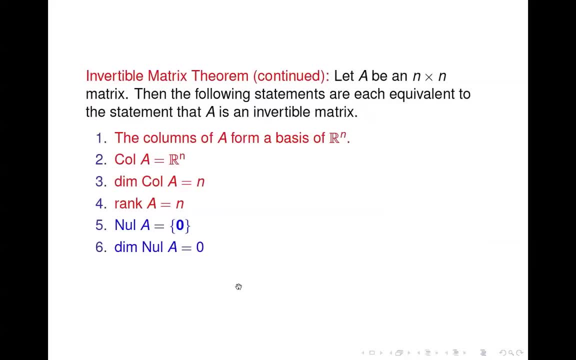 uh, these, these, So these extra six, you need to commit them to memory, relating them to to each other or to pivot positions. All right, uh, I want to go through some of the some of the problems at the end of this. 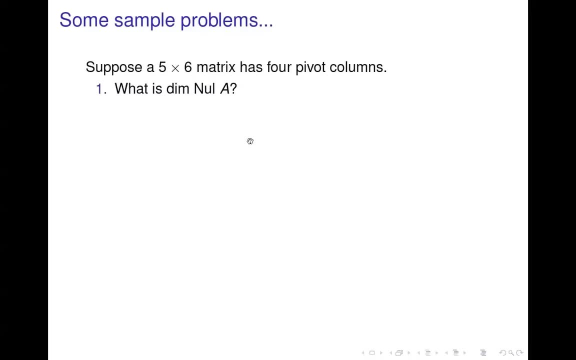 section, because there's some excellent problems here. Uh, in fact, this section, I think, is the most important section in the course, So make sure that you um really work on these problems and understand what you're doing. So I'm going to do several of them at the end of the section. 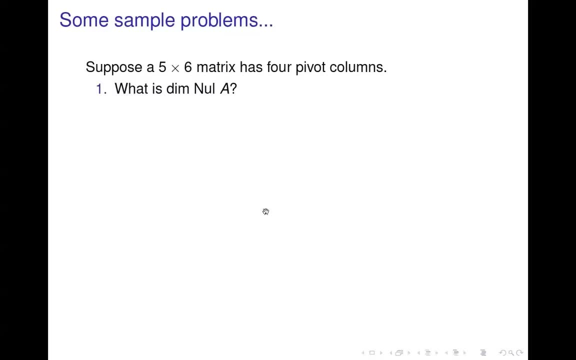 Okay. So the first one says: suppose, uh, a five by six matrix, let's call it a- has four pivot columns. Okay, So it's a five by six matrix with four pivot columns. Okay, If it has four pivot columns, um, then that means it has two non pivot columns. 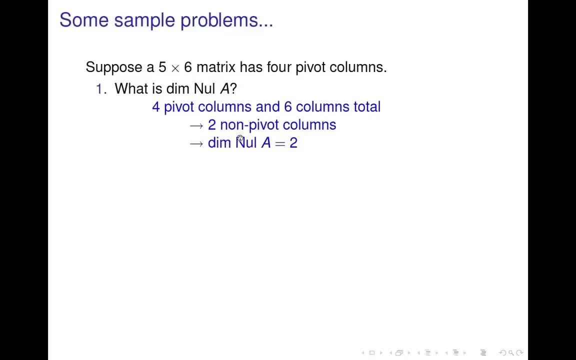 So what's the dimension of the null space of a must be two, right, Cause you got two non pivot columns. Um is the column space of a equal to our four? Well, um, the dimension of the column space is four because we have four pivot columns. 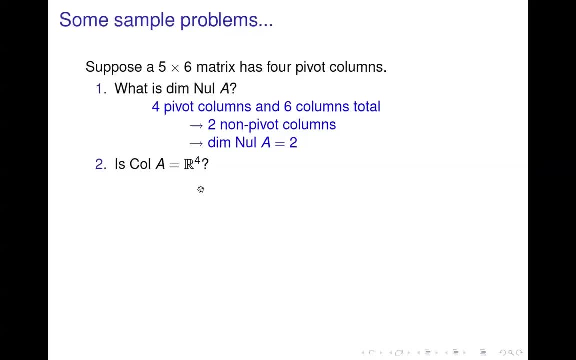 Okay, So the dimension of the column space is four, but the columns are in our five and therefore, um, they, uh, uh are. the span of the columns is not equal to our four. Uh, it's just a subset of our five. 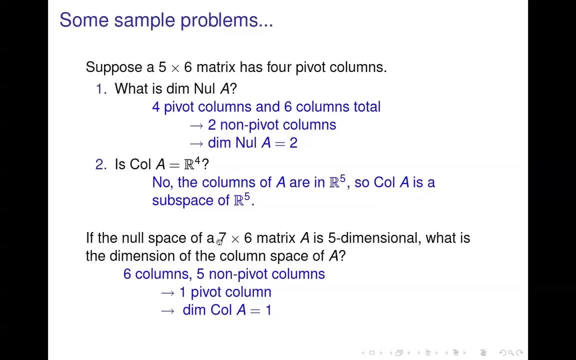 All right. Next one: If the null space of a seven by six matrix is five dimensional, okay, so that means you have five non pivot columns, which means out of six columns one is a pivot column. Then therefore the dimension of the column space has to be one. 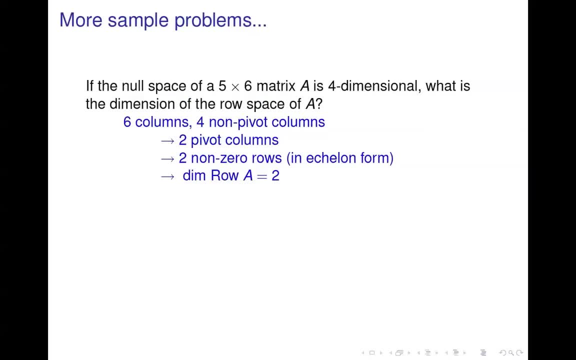 All right, Suppose the null space of a five by six matrix is four dimensional, Then that means you have four non pivot columns. So that leaves two pivot columns And, uh, we want to know the row dimension of the row space. We have two pivot columns. 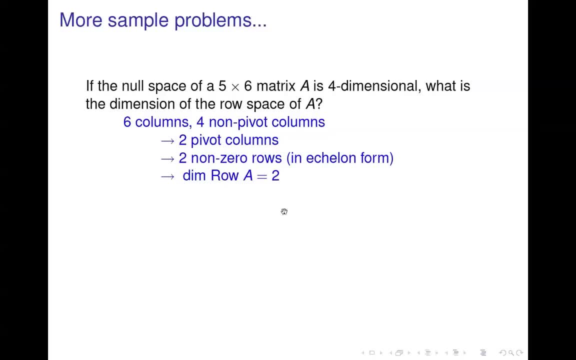 So that means we have two non zero rows when we put the matrix in echelon form. So the dimension of the row space is two. All right, How about if a is four by three? what is the largest possible dimension of the row space? 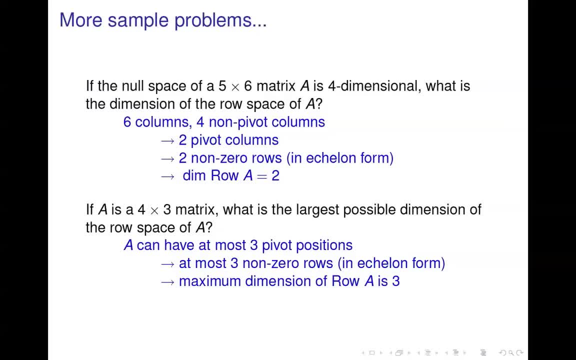 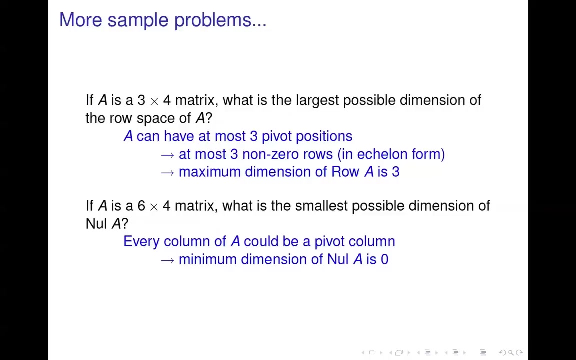 Okay, All right. Well, if a is four by three, then, uh, we could have, uh, at most three pivot positions, So at most three non zero rows when we put it in echelon form, So the maximum dimension of the row space is three. all right, uh, if a is three by 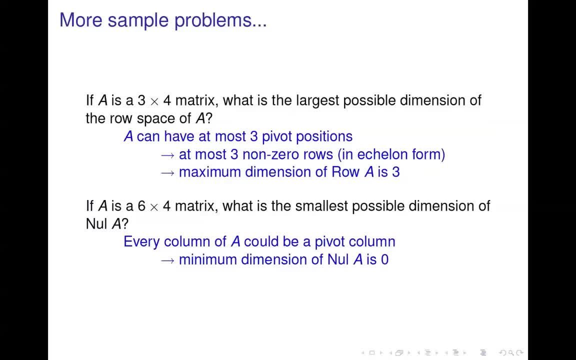 four. what's the largest possible dimension of the row space? Three. If a is three by four, then the again, the maximum number of pivot positions we can have is three. So we have at most three non zero rows. So the maximum dimension of the row space is three. 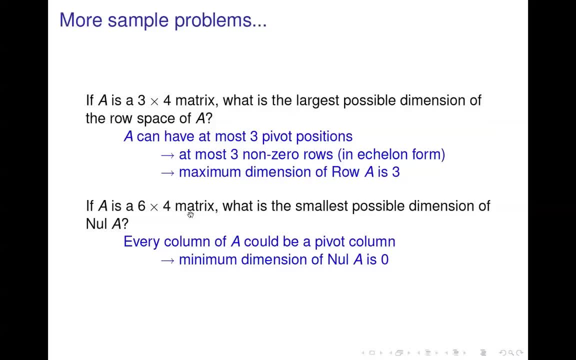 Uh, how about if a is six by four? What is the smallest possible dimension of the null space? That's asking what's the smallest number of free variables you can have and are what's the smallest number of non pivot columns you could have. 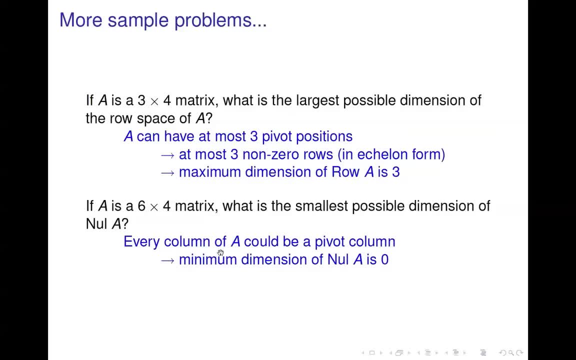 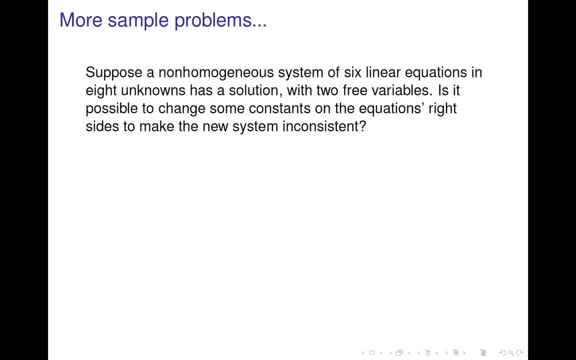 Well, since we have more rows than columns, every column could be a pivot column, in which case there's no free variables, And so the minimum dimension of the null space of a would be zero. all right, a little more complicated one here. 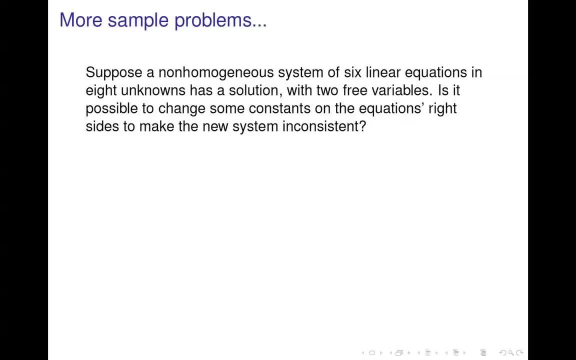 Um, suppose a non homogeneous system of six equations and eight unknowns has a solution with two free variables, Is it possible to change some constants on the equation's right sides to make the new system inconsistent? All right, So we got a non homogeneous system- six equations and eight unknowns, and it's consistent with. 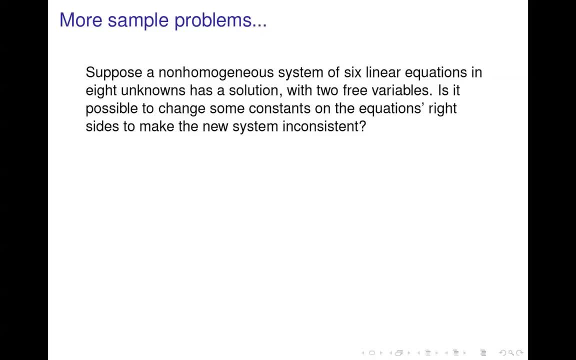 two free variables. And what that tells you are the two free variables is that, uh, you have, since there's eight unknowns, we got eight columns. two are free, So that means there are six, But our pivot columns okay. so that would look like this: 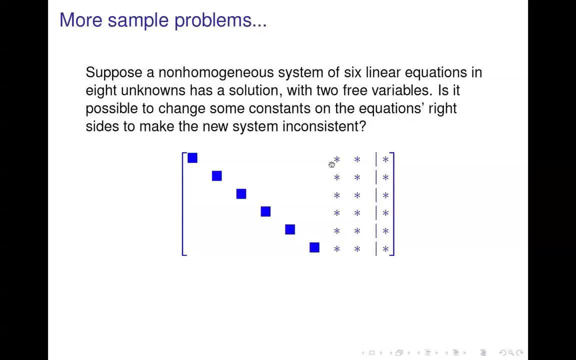 Got six rows here, eight columns um, two free variables, which leaves six pivot columns. All right, And it's saying, if we change the right hand side, will the system still be consistent? And the answer is yes, Um, I'll plug my computer in um. is it possible to change some constants to make the new system? 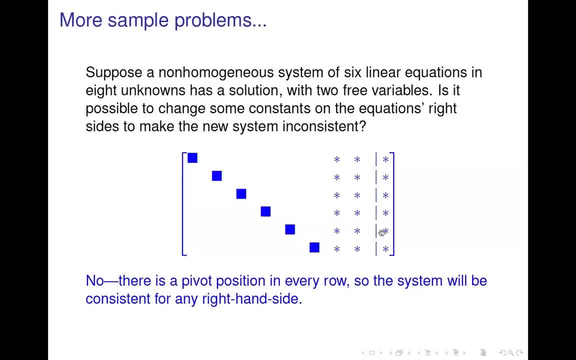 inconsistent? No, The answer is no to that. Um, because, uh, no matter what's over here, since you have a pivot position in each row, uh, the system's always going to be consistent. Now I was thinking. the question was is: is the system always consistent? 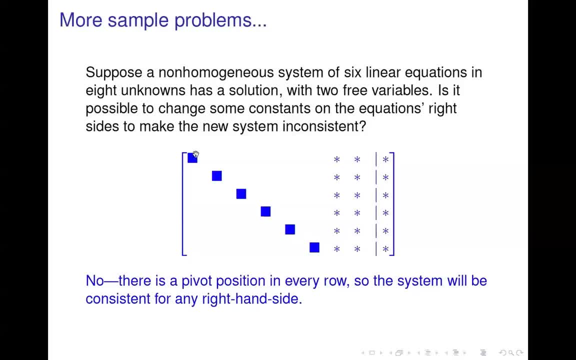 And the answer to that is yes, Right, And that is because you have a pivot position in every row, So you're never going to end up with a row of all zeros and then something not zero over here. All right, Another one. 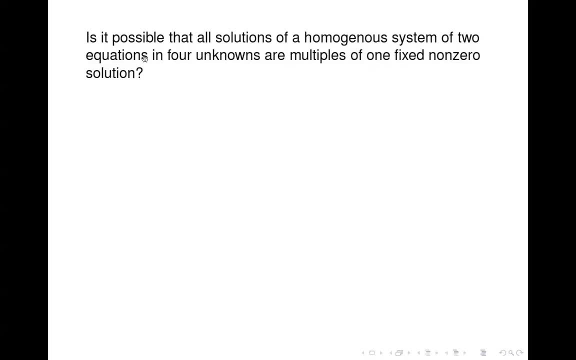 Is it possible that all solutions of a homogeneous system of two equations and four unknowns are multiples of one fixed, non-zero solution? Hmm, Okay, Homogeneous system, two equations and four unknowns- Okay. So if you think about that, we've got two rows and four columns. 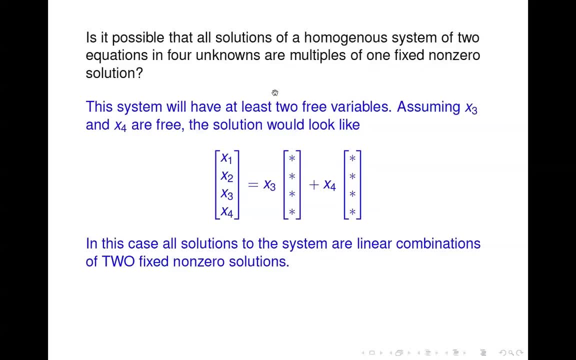 So we have at least two free variables, right? So if we wrote our solution in parametric vector form, so we had two free variables and it would look like this: you know what this says is that each solution is a linear combination of two fixed, non-zero solutions, right? 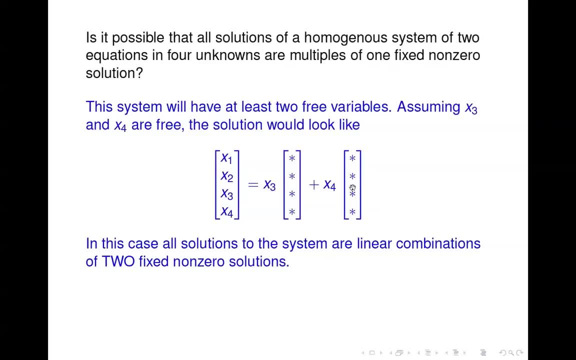 Each one of these vectors is what they're calling a fixed, non-zero solution. Okay, So we're going to have at least two of these vectors, So that means that it can't be the case that all the solutions are just multiples of one non-zero solution. 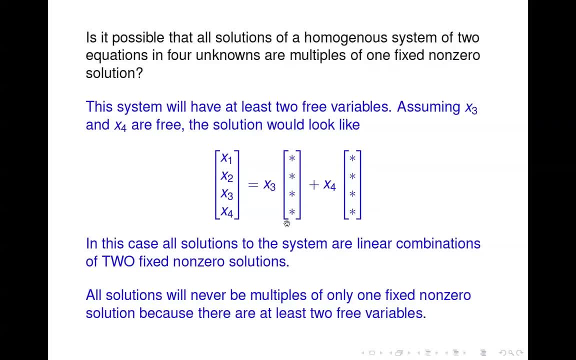 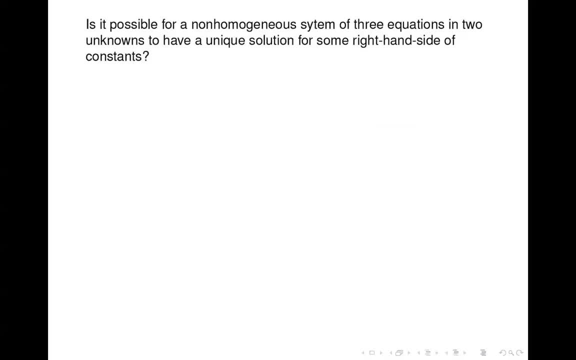 If that was the case, we would only have one vector here, and we can't have that because we have at least two free variables. All right, Another one, Hmm, Is it possible? Okay, So you could have a system of three equations and two unknowns to have a unique solution? 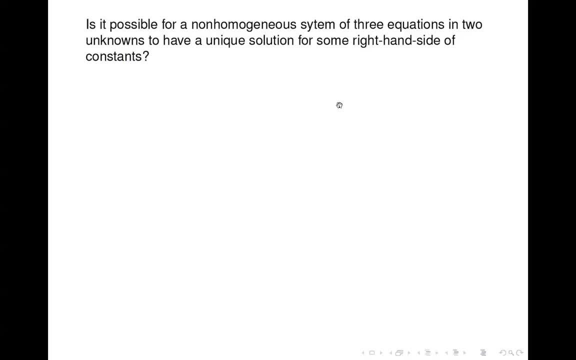 for some right-hand side of constants. So three equations, two variables, right? So that might look like this: three equations, two variables, So you could have a pivot position in each column and you could have a row of all zeros. In that case, yes, the system would be consistent. 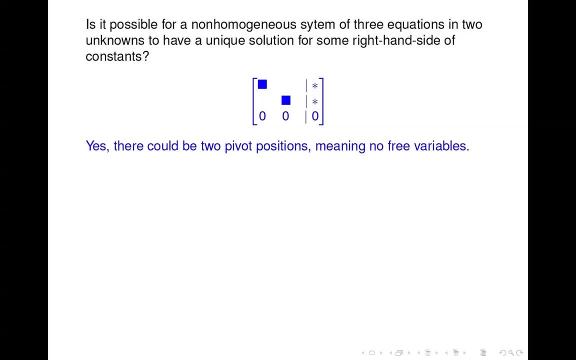 There would be, uh, a unique solution. All right, How about this one? Is it possible for such a system to have a unique solution for every right-hand side? And okay, look at that. you could have this situation: still have pivot position in each. 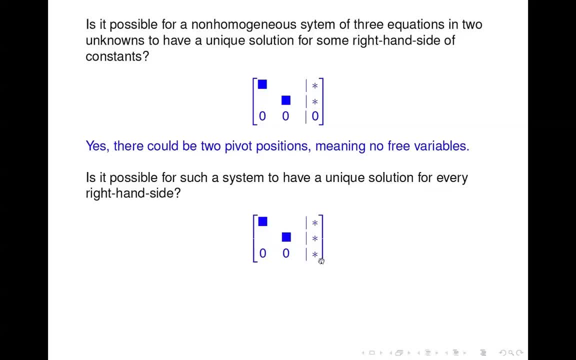 column but have zero, zero, something not zero, in which case there's no solution, right? So in this case it's not possible. It's not possible for such a system to have any sort of solution for every right-hand side, right? 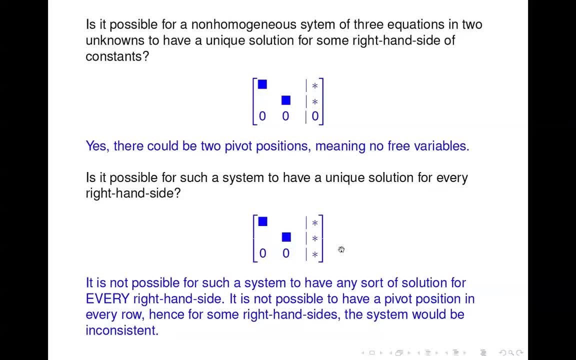 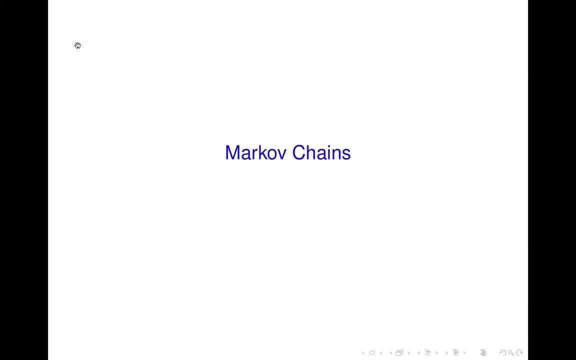 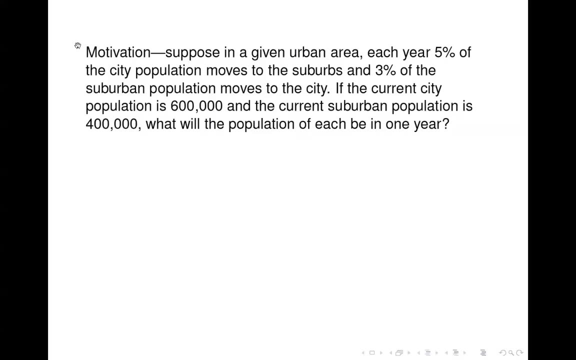 In some cases, it's simply going to be inconsistent. All right, That's it for this one. Okay, Our topic for today is Markov chains And uh to uh get us going on that. uh, we'll look at a a small example. 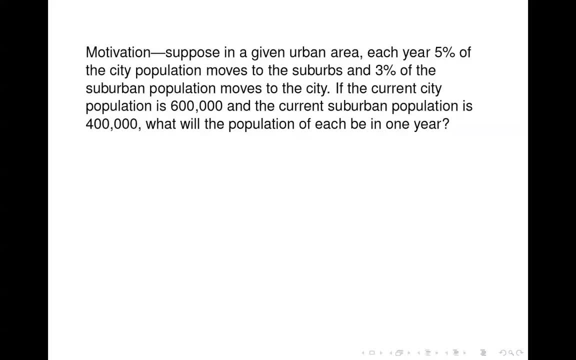 So let's suppose, Uh, in a uh given urban area, uh, each year 5% of the population that's in the city moves to the suburbs and 3% of the suburban population moves to the city, And we're going to assume that this is a closed uh um system here. 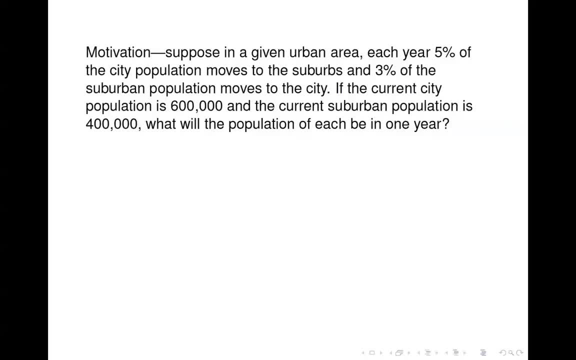 So, uh, any movement uh just goes from the city to the suburbs or suburbs to the city. So we're not considering moving elsewhere. Okay, There are people moving in from elsewhere. So just city to suburban, suburban to city. 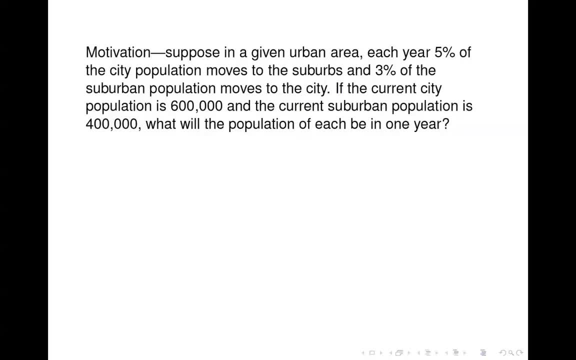 Okay, So let's assume that the current city population is 600,000 and the current suburban population is 400,000., Then what will the population of each be a year from now? Well, um, based on what we know, uh, next year, uh, the city population is going to. 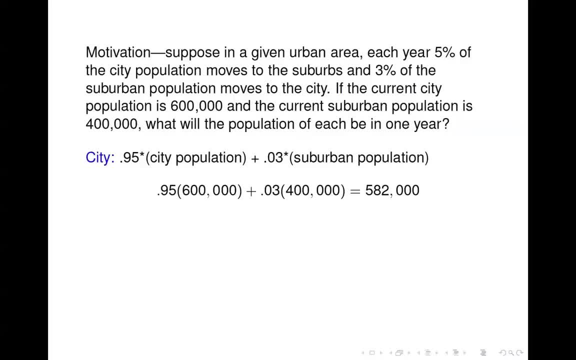 be, uh, 95% of what it is now. Okay, Right, Cause we each year 5% leave, So we're keeping 95%, and then 3% of the suburban population moves to the city, So we add on a 0.03 times the current suburban population. 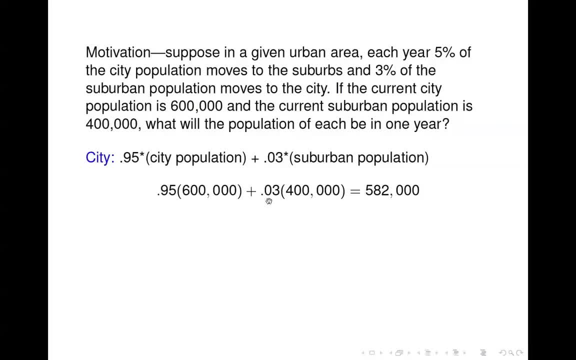 So that's a 0.95 times 600,000 plus 0.03 times 400,000, which gives us 582,000.. So you make sense that the city population is going down. We've got more moving to the suburbs than we have coming in. 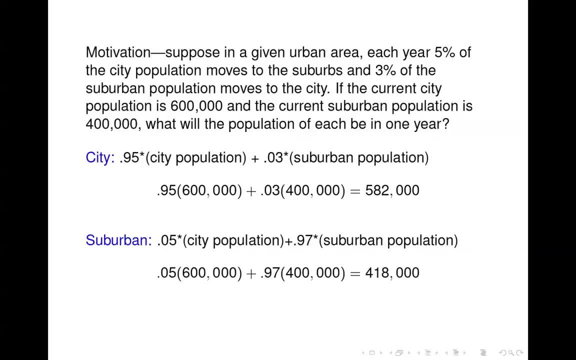 Uh, to find the suburban population in a year, uh, we could just say well, um, since the total is a million, then we can just say a million minus 582,000 and get it that way, which is correct. but we could also look at it the way we did with the city and say well. 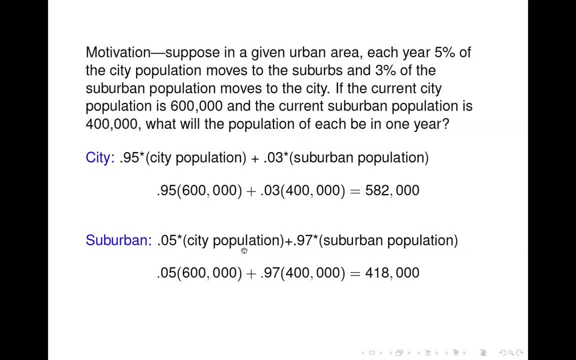 we're getting 5% of the city population moving to the suburbs and a 97% of the current suburban population is staying there. Okay, So we get 0.05 times 600,000 plus 0.97 times 400,000, which gives us 418,000. 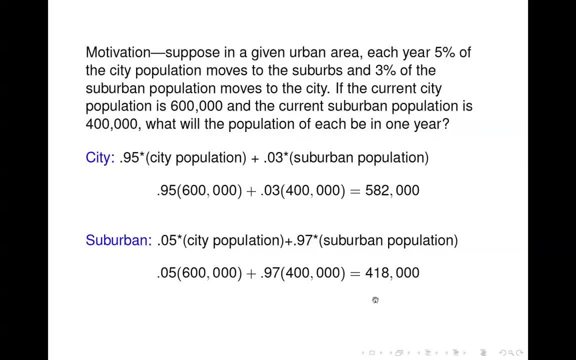 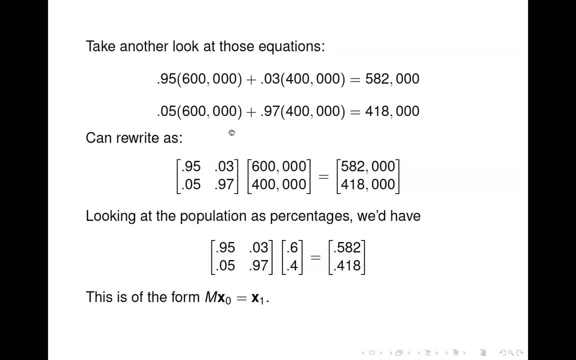 And a 418 plus 582, uh gives a million total Um. another way to look at it is: let's take a closer look at those equations, um and notice that we've got um 600,000 times the 0.95, 0.05 here. 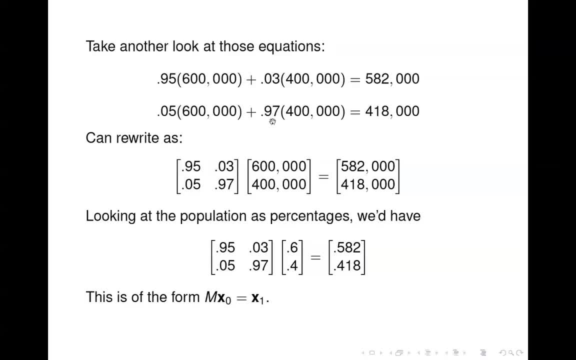 We've got the 400,000 times the 0.03 and the 0.97, and that looks like: hmm, we're taking a linear combination of a couple of vectors: the 0.95, the 0.05 and the 0.03, 0.97.. 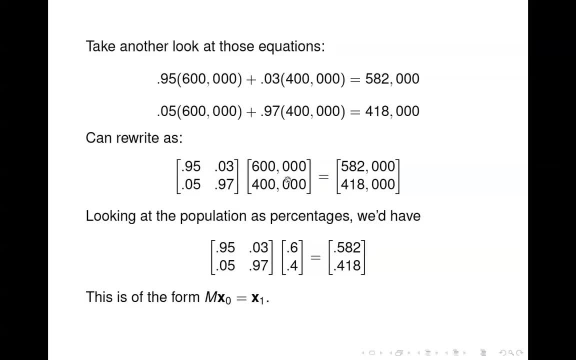 So we're going to rewrite it in this form as a matrix times a vector right, And so the linear combination is just 600,000 times the first column plus 400,000 times the second column, And that gives us our uh population figures for one year from now. 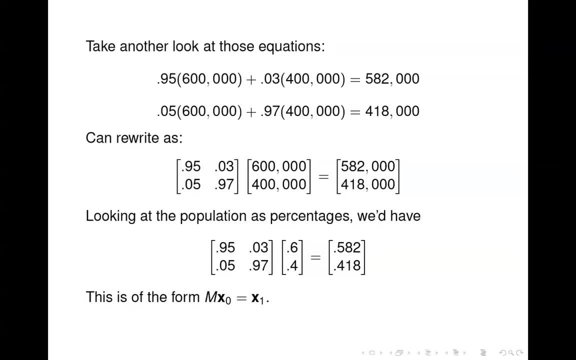 Okay, We can add it as percentages, which is typical um, instead of actual raw uh numbers, uh. so if we look at the population vectors 0.6, 0.4, um, we do the same sort of uh computation. 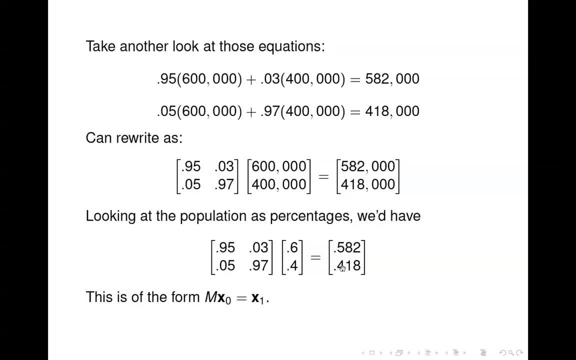 and end up with this, uh, population vector for a year from now. And, uh, if you notice that each one of these vectors, the columns of the matrix plus our two vectors here, each one of them sums to one. So they're, they're a special vectors, uh, because they represent probabilities. um, 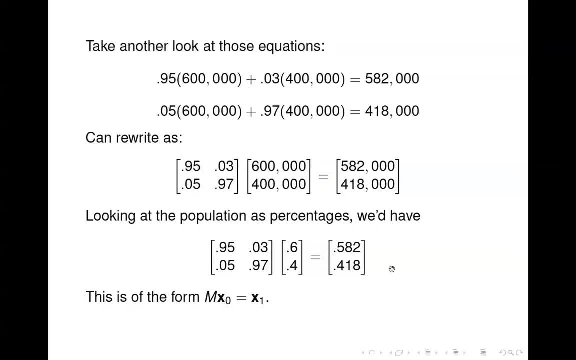 or percentages, And, uh, we'll talk about that a little more in just a minute. But before we get to that, notice that, uh, what we have here, this is of the form, some matrix, which I'm calling M, times a vector, I'll call X naught, which is like the original. 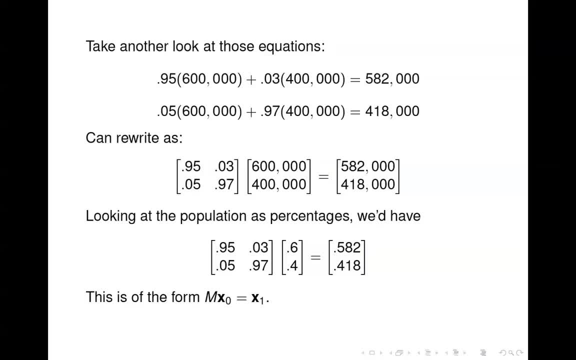 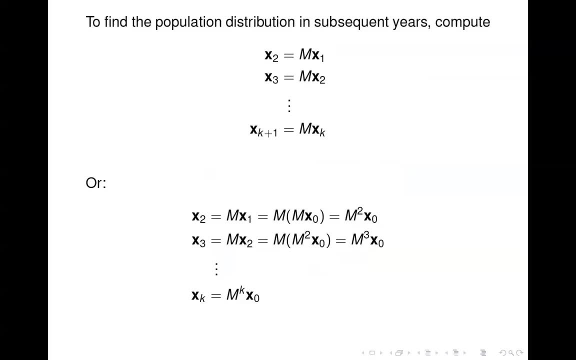 state of the system: original population. We multiply those together to get X1.. Okay, X1, which is the state in year one. We can continue that process to figure out what the population in year two would be, year three and so forth, year K plus one uh for any year. it's just uh M times the. 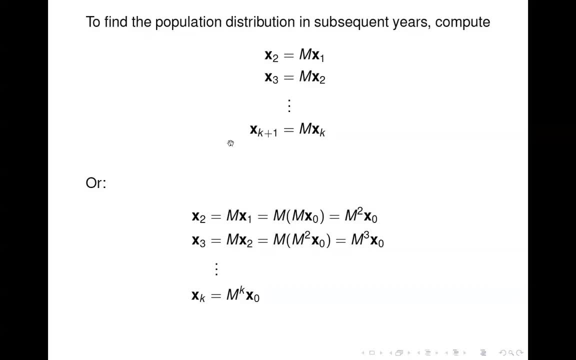 population from the previous year. So, for instance, if I wanted to figure out 10 years from now what's uh the population, then I could compute X2, which is well. to compute X10,, I need X1.. 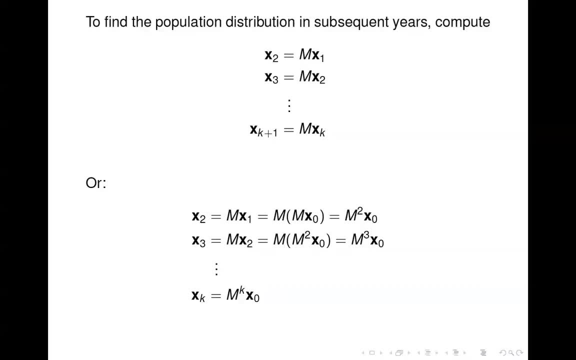 I need X9,. right, because X10 is M times X9.. To get X9, I need X8, to get X8, I need X7, and so forth. So I'd have to compute all those intermediate uh population vectors. 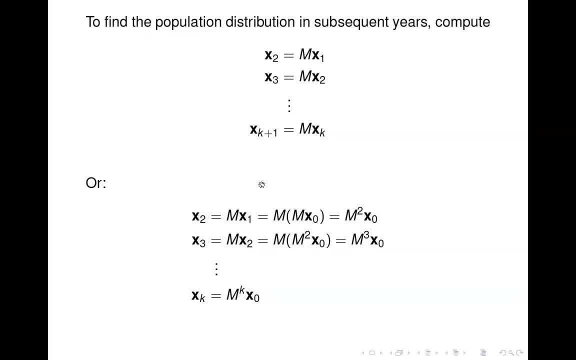 Uh, there is another way to do it which doesn't require, uh, that computation, um, and that is to look at it as I have here at the bottom. Uh, if we look at X2, for example, that's M times X1, but we know that X1 is M times. 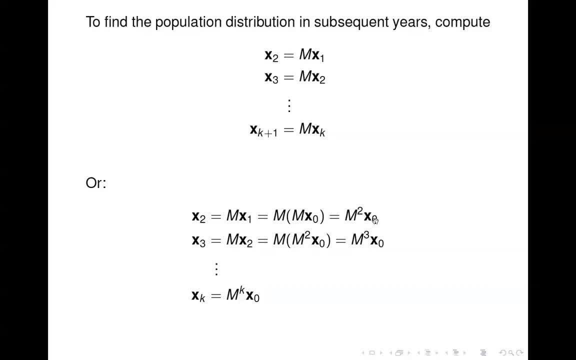 X0, so X2 turns out to be M squared times X0.. Similarly, X3 is M times X2, but we know X2 is M squared X0, so X3 is just M cubed times X0.. And in general we have XK, year K, uh population would be M to the K times the original population. 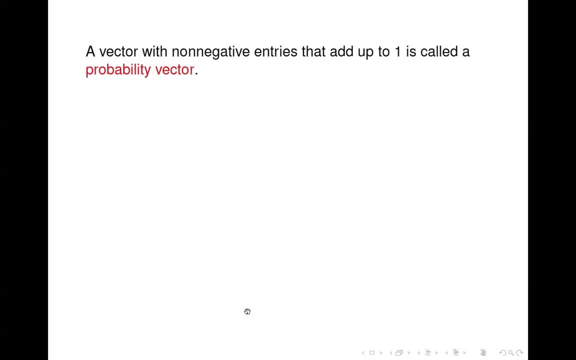 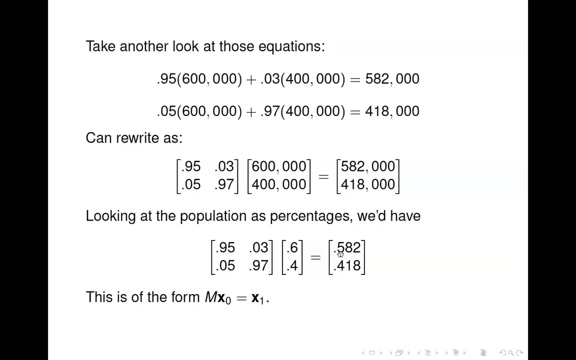 vector. Okay, So a vector with non-negative entries That add up to one is called a probability vector. So back uh to these. um, all these are probability vectors because they all add up to one. Each column adds up to one. 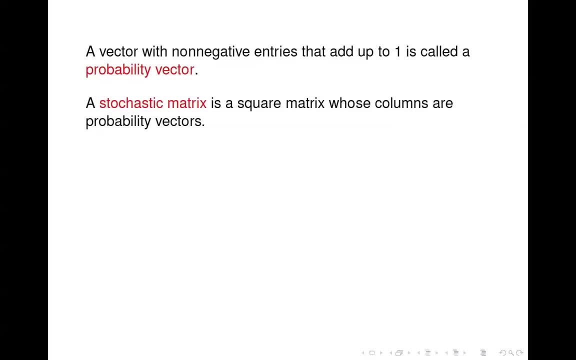 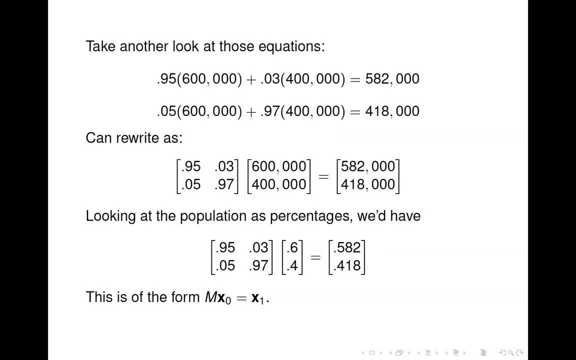 Okay, A stochastic matrix is a square matrix whose columns are probability vectors. So the matrix that we had here, that is a stochastic matrix because each of its columns is a probability vector. Okay, A vector where their entries are non-negative and they sum to one. 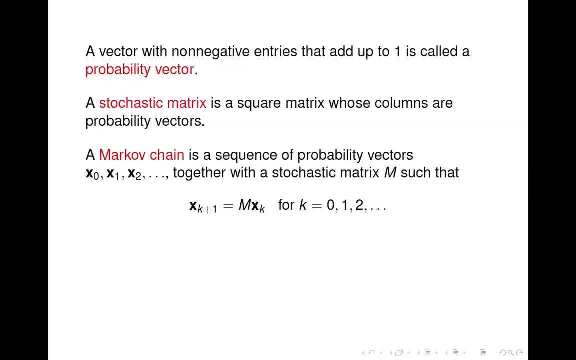 A Markov chain is a sequence of probability vectors- X0,, X1,, X2, and so forth, together with a stochastic matrix, M, such that X sub K plus 1 is just M times X sub K, which is the pattern that we had in our example. 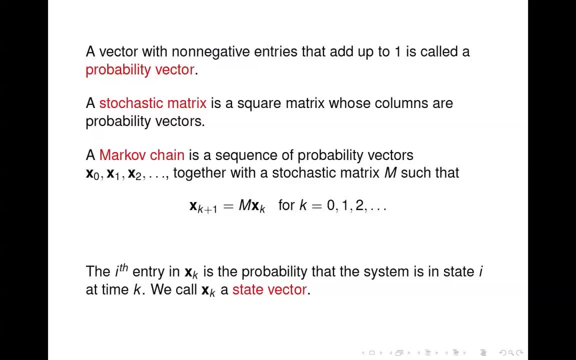 Um. the Ith entry in XK is the probability that the system is going to sum to one That the system is in state I at time, K, Okay, Um, and we call XK a state vector because it represents the state of the system at time. 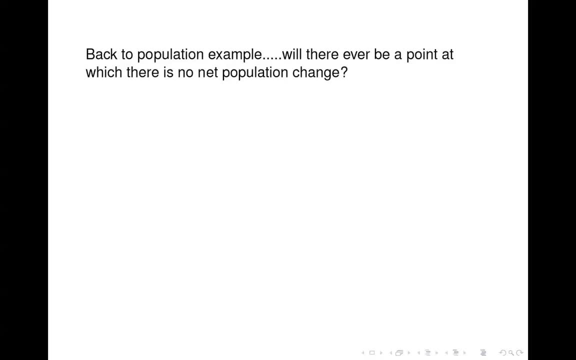 K. Okay, Now an interesting question, uh, related to our pop, our population example is: will there ever be a point at which there's no net population change, That is, the number of people moving to the suburbs is equal to the number of people moving. 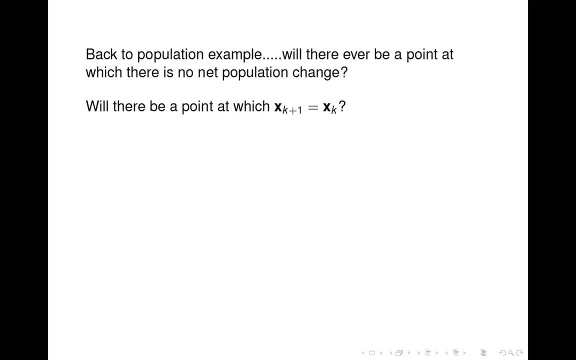 to the city. Okay, Another way to look at it is: will there ever be a point at which XK plus one is equal to XK? All right, So you compute XK plus one, um, and uh, it's the same as XK, or will there ever be a point? 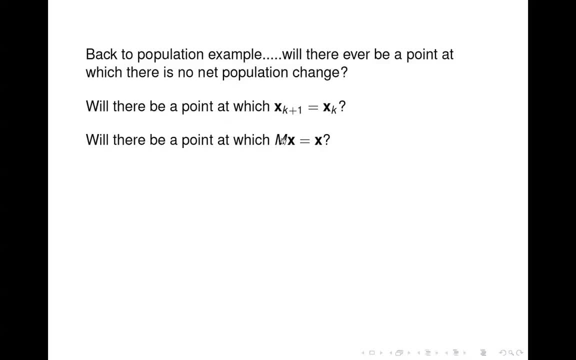 at which you have your current state is some vector X. you apply the transition matrix M to it and you end up back with the same vector X. Okay, And so this is the system. This is the system we want to look at. Um, it's similar to systems that we know how to solve, but it's a little bit different. 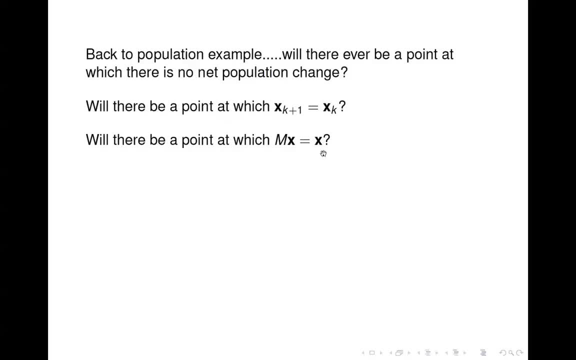 because on the right hand side here we've got a variable. It's not a constant um, so it's not like an AX equals B system Um, so we need to uh manipulate it a bit before we can uh use the things that we. 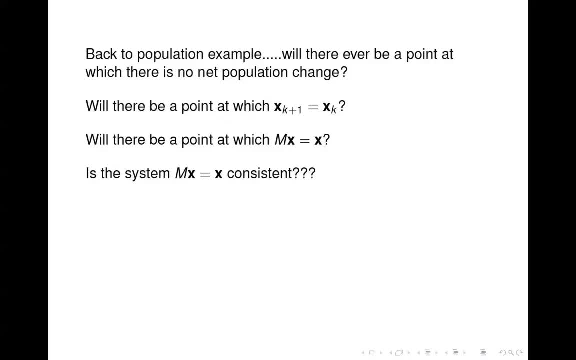 know about uh solving systems. Okay, So we want to know: is it consistent? And the way we determine that is: uh, we bring the X over to the left hand side, We get uh. MX minus X is a zero vector. 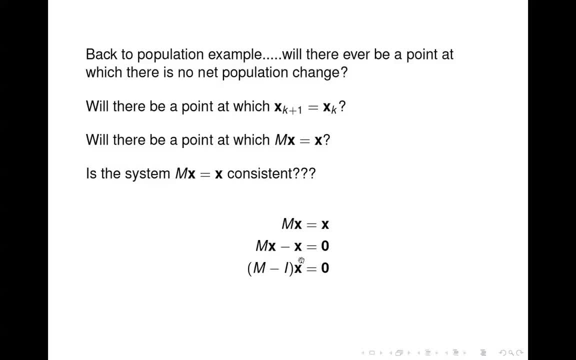 And then the key is to factor out that X. And if we factor out the X, then we're left with M minus the identity matrix. So I here is the identity matrix. So what we end up with is some matrix which is M minus the identity matrix which we can. 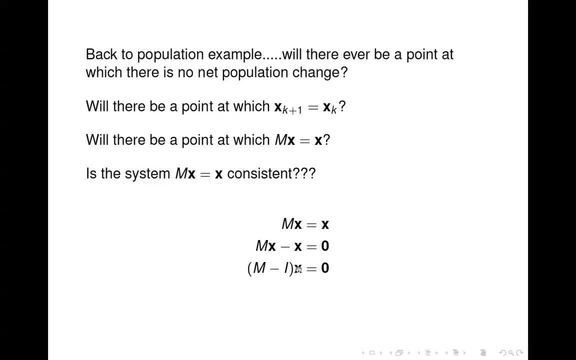 compute directly. We know both of those times, X, which we don't know, equals a zero vector. So when we write it in this form here, it's a simple, homogeneous system. Now, clearly it's consistent because uh X can be the zero vector and and uh that's. 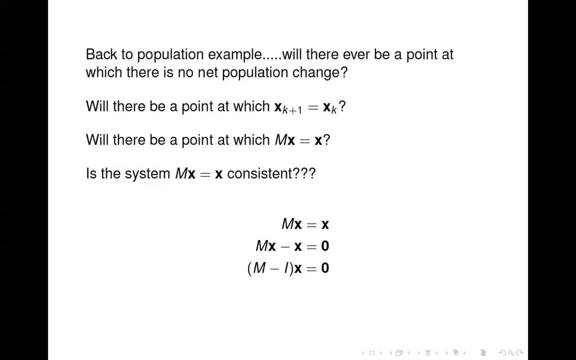 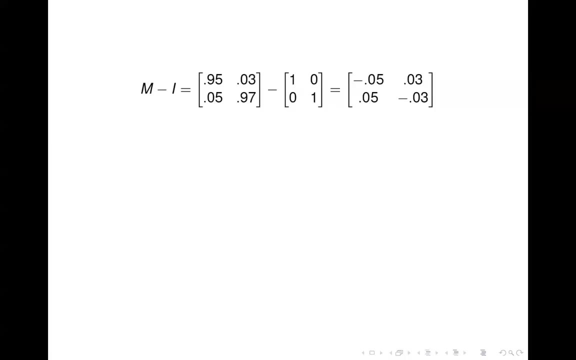 uh, obviously makes that consistent. However, that's not a very interesting case. So what we really want to know is: um, does this system have, uh, an infinite number of solution? Uh, are there any free variables? All right, well, if we look at this uh matrix, for our example: uh, all right, so we subtract. 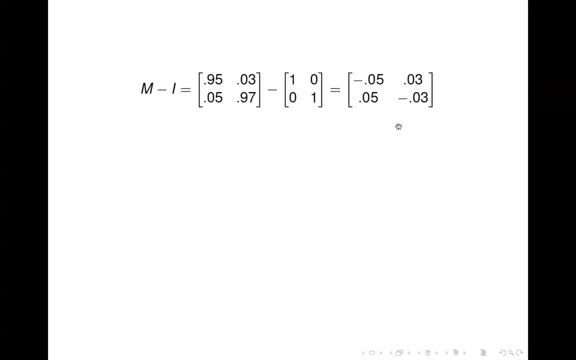 off the identity and we're left with this one, And it's clear when you look at that that the columns are not linearly independent and therefore you have a free variable. So if we solve this system, uh, it's pretty straightforward. 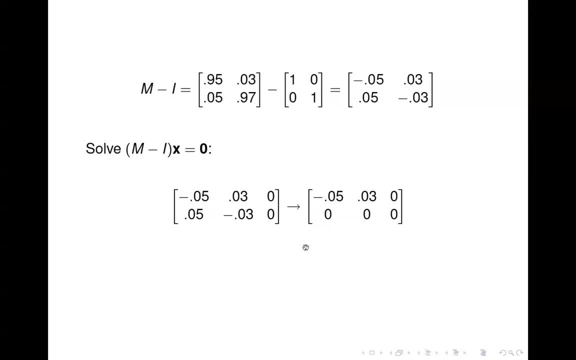 Um one row operation and we've zeroed out, uh, the bottom row, And um so Okay, Um first row tells us that five multiplied by 100 makes life simple. So we get: five X one equals three X two. 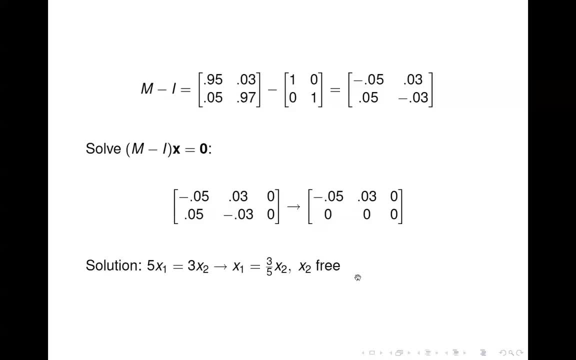 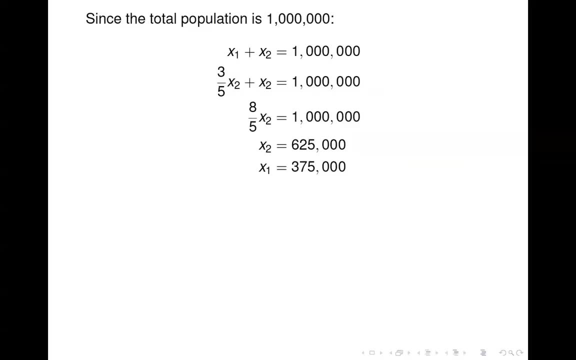 So that means X one is three fifths times X two, where X two is a free variable. And um, to get, uh the actual vector, that, uh, the probability vector that corresponds to, um, this, um relationship between X one and X two. 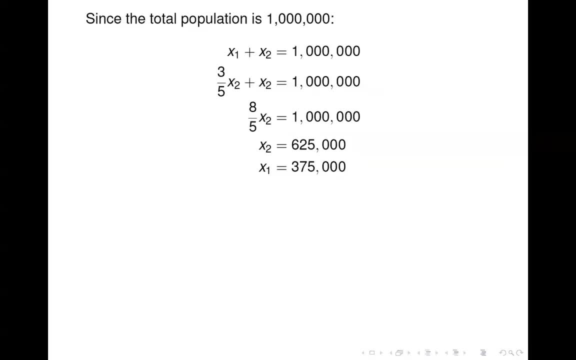 Okay, Uh, we want X one plus X two to equal a million. or we could say one um- I'm doing it just for raw population numbers- um and X one is three fifths X two. So we get this equation: putting these two together, eight fifths X two is a million. 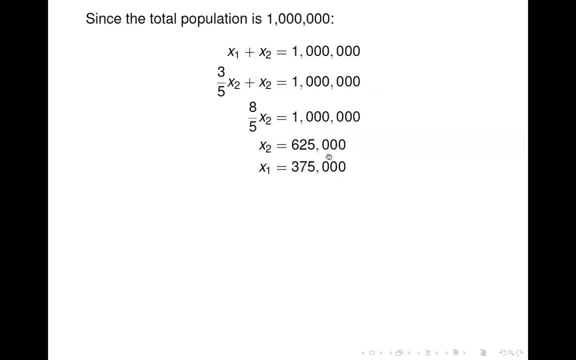 which is X two is uh 625,000, and therefore X one's 375,000.. All right, So, um, We've reached the point here at uh, that the number moving out of the city is a 0.05. 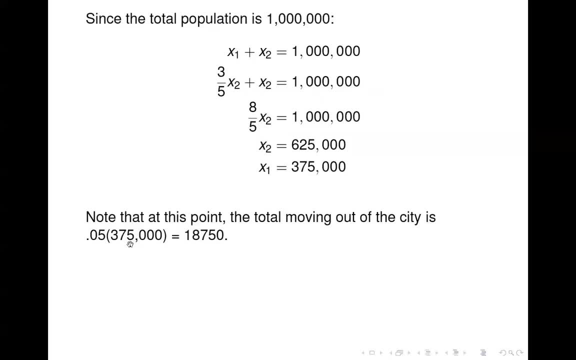 times 375,000.. All right, So that's five. every year, 5% leave the city. So the population of the city at this point is 375,000.. So 5% of that's 18,750.. 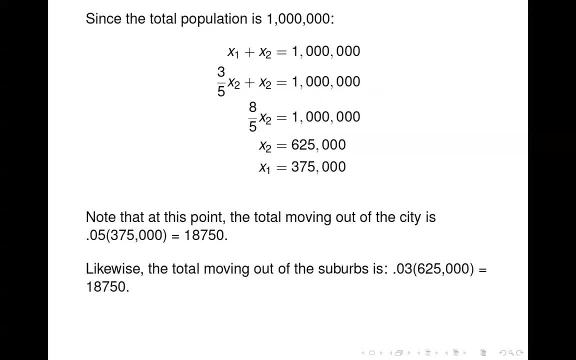 Likewise, the total moving out of the suburbs, which is 3% of the suburb population, which at this point 625,000, is also equal to 18,750.. So we've reached the point here where the number moving out of the city is equal to. 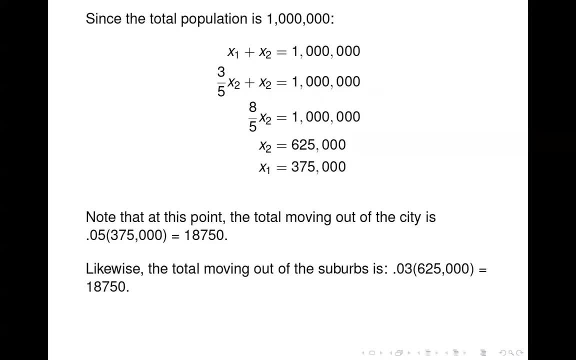 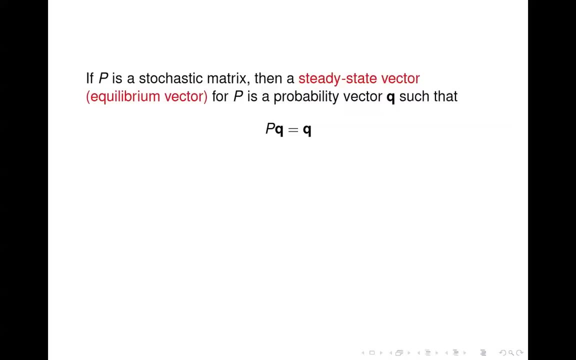 the number moving in, So there's no net population change. Once the system gets to this point, all right, um, a little more terminology for you. If P is a stochastic matrix, then a steady state vector, Also called equilibrium vector- for P is a probability vector, Q, such that P times Q is. 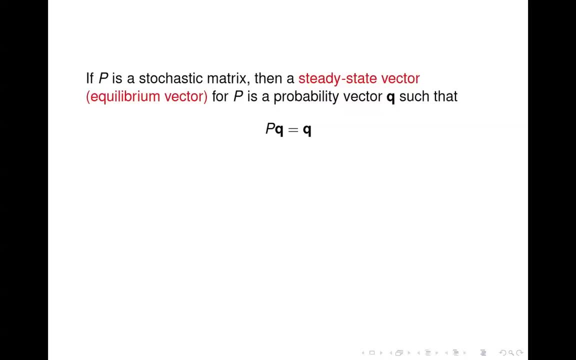 equal to Q. All right, Before we said M times X equals X, talking about the same thing here. all right, we have this theorem that says: if P is- uh, a stochastic matrix, then it has a unique steady state vector. 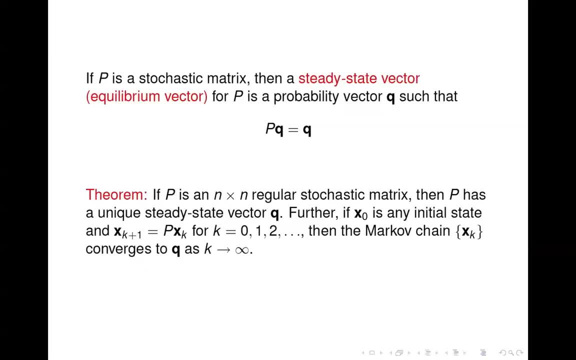 Okay, And it, it, even though the system has an infinite number of solutions, if we require that the uh elements sum to one, then that makes it a unique uh vector. Okay, Furthermore, um, if X naught is any initial state and we have X to the K plus X sub K. 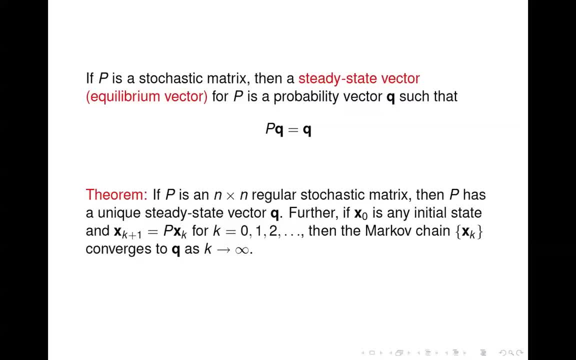 plus one equals P times X sub K, then, uh, the Markov chain converges to Q as K goes to infinity. So what's interesting about this is that, uh, the initial state is unimportant. It says: if X naught is any initial state, um, then the Markov chain will converge to. 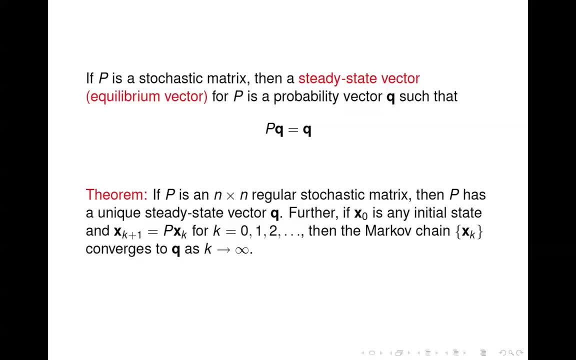 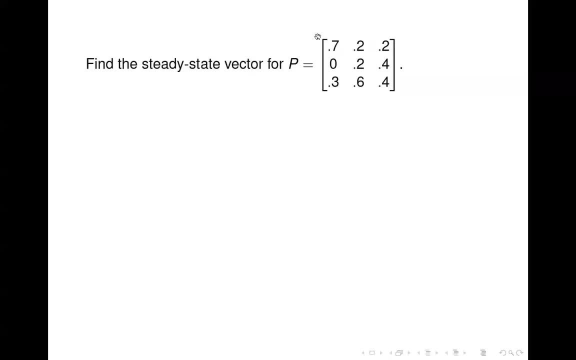 this steady state vector as, uh, if you go, go to a big enough K, Okay. So let's look at another example. Here's a matrix. Let's get a three by three, um, and find the steady state vector for this matrix. 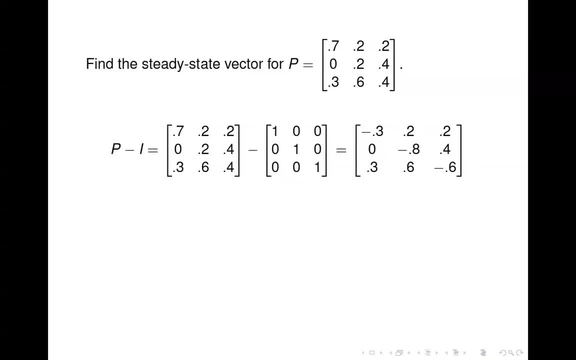 So we need to compute P minus the identity. So there's that. And then we need to solve P minus I times X equals zero. So do a few row operations end up with this matrix? And uh, so the solution is X one, X three, X two is a half of X three, where X three is. 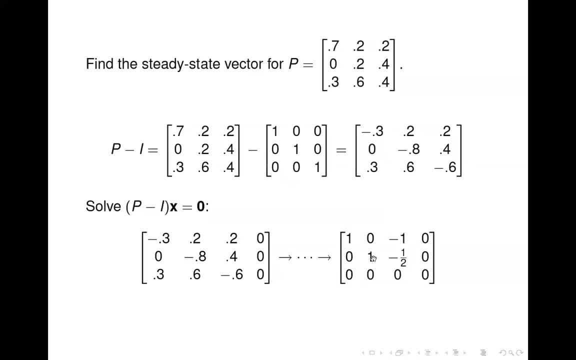 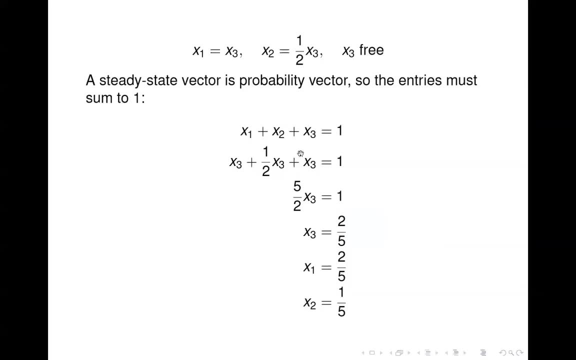 free. So back you can see: X one equals X three, X two is a half of X three and X three is free. And again, uh, the elements need to sum to one. So uh, we get uh, X one equals X three, X two is a half of X three and X three is free. 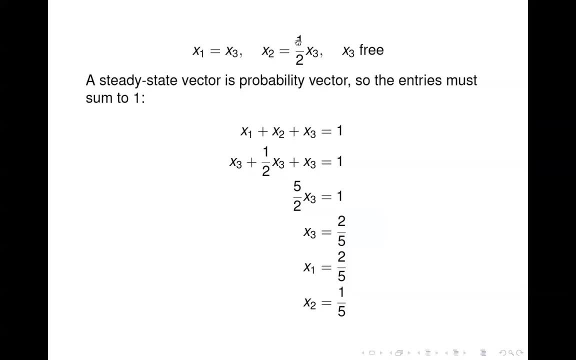 And again, uh, the elements need to sum to one. So, uh, since X one is X three, X two is a half of X three. that's where this second equation comes from. And, uh, it turns out that X three has to be two fifths. 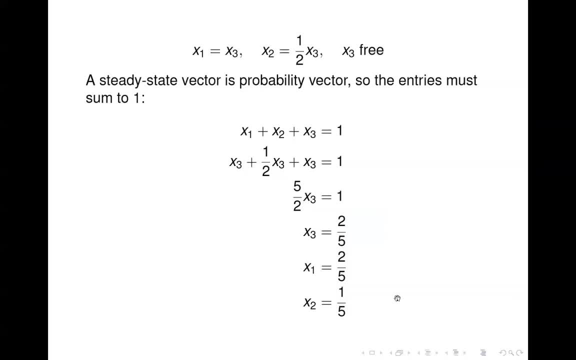 So that means X one is two fifths and X two is one fifth. So the steady state vector is this one here. And if you check out, uh, what P times X is multiply P times the steady state vector Turns out, you get, uh, that steady state vector back. 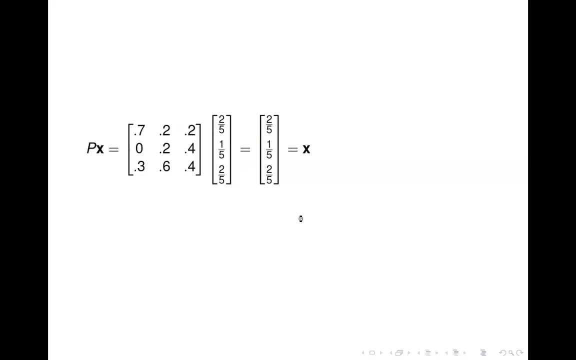 So It checks out. All right, I want to show you one more uh application problem, and this one I've taken from another book, uh book by Andrilli and Hecker. It's kind of an interesting one, I thought, and it's based on banks. 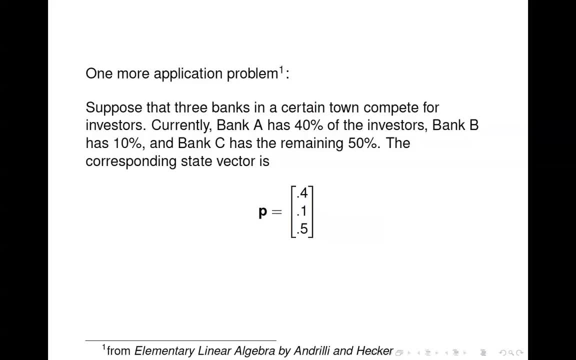 Uh, I say, suppose you're. you've got three banks in a certain town that compete for uh business and uh bank A right now has 40% of the customers, B has 10% and C has 50%. 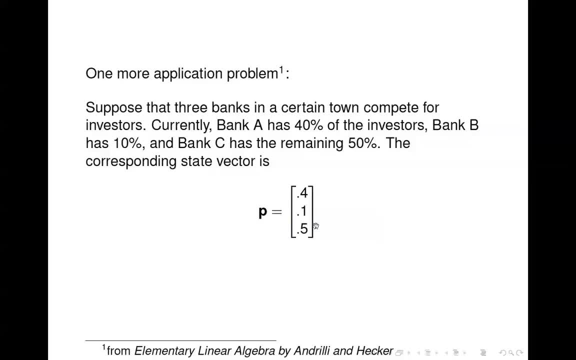 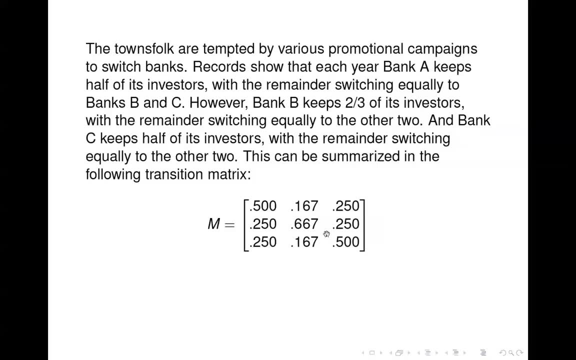 So we write that Uh Vector as uh given here, 0.4 corresponds to bank A, 0.1 for bank B and C with a 0.5.. Okay, So the banks are obviously trying to um woo customers from the other banks. 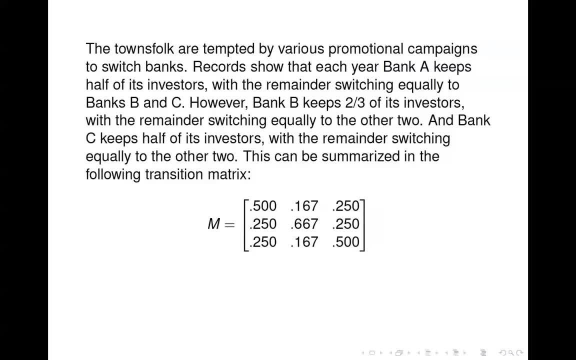 And, um, what we have here is, uh, um, information about how successful they are at that. So we see that records show that each year, bank A keeps half of its uh investors, with a remainder switching equally to B and C. So if you look at the first column of this, 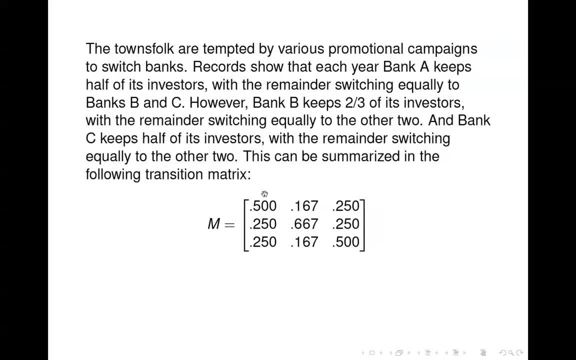 matrix that uh is. you can think of this column as being related to bank A. Um, in each row, uh uh, the row first row corresponds to bank A, the second row to B and the third row to C. So we've got an A column, a B column, a C column and an A row, a B row and a C. 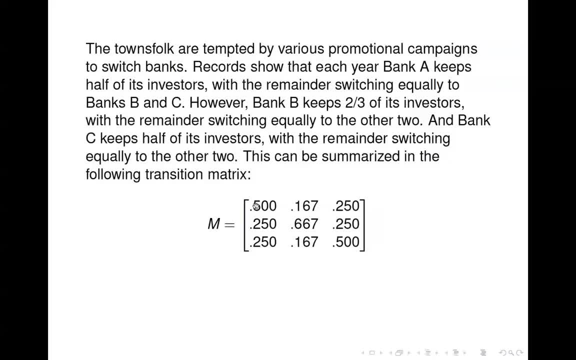 row. So the the 0.5 here, uh- represents the probability That a person at bank A is going to stay at bank A. Then the 0.2, uh. 0.25 here represents the probability that a person in bank A is going to switch to bank B And the 0.25 at. 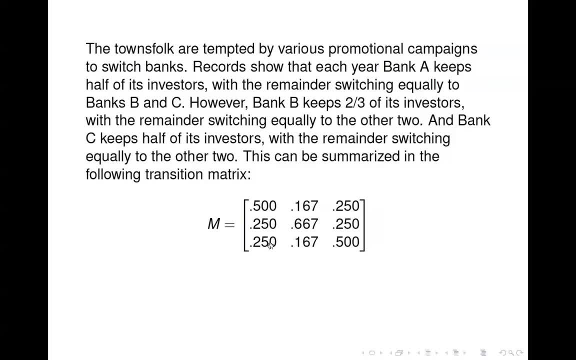 the bottom represents the probability that a person currently at bank A is going to switch to bank C. All right. and it says bank B keeps two thirds of its investors, with a remainder switching equally to the other two. So the 0.667. 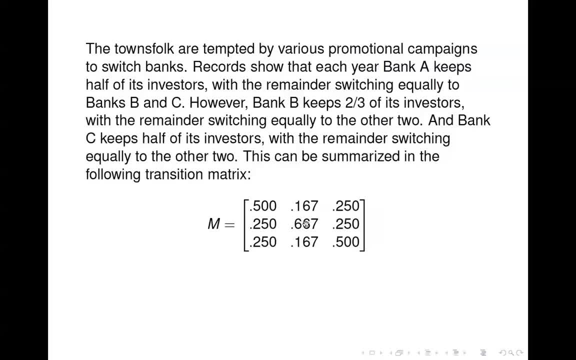 That's the probability that someone who who starts at bank B or who's currently at bank B is going to stay there, um, for the next year, And then, uh, the 0.167 here that's probability- someone who currently is at bank B switches. 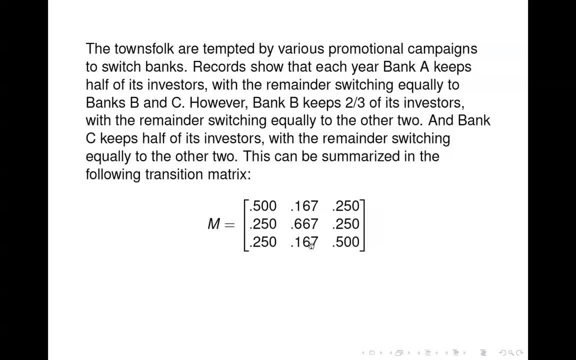 to bank A. Okay, and same thing down here, Somebody at bank a probability that a bank B customer will switch to bank C. Uh, then we say: uh, bank C keeps half of its investors and the remainder switching equally to the. 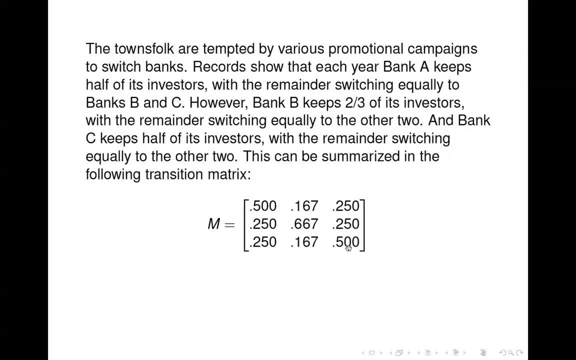 other two. So the 0.5 here is probability that customer at bank C stays at bank C, And these 0.25s here probability that somebody at bank C switches to A here and switches to B here. Okay, so this is what we call our transition matrix. 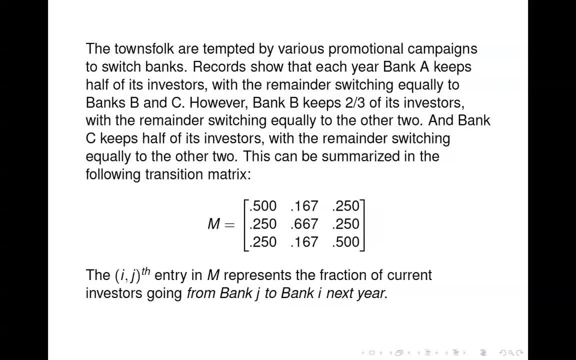 Um, and, as I said, the IJth entry represents the fraction of current investors going from bank J to bank I. Okay, So, Um, we think of again, if you think of this as uh labeled uh. columns A, B, C rows. 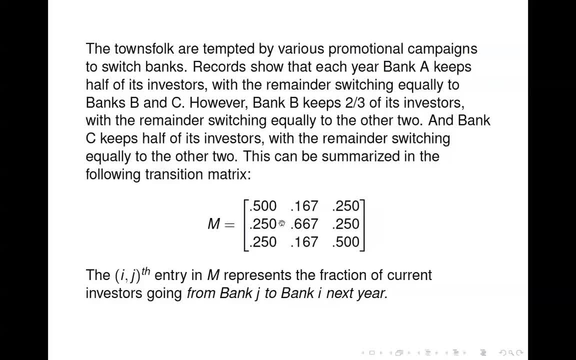 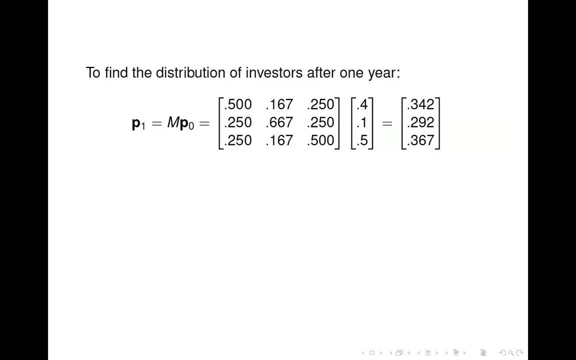 A, B, C, um the entry. a particular entry represents person switching from whatever column they're in to whatever row. uh that value is I like to find? uh the uh distribution of investors after one year. 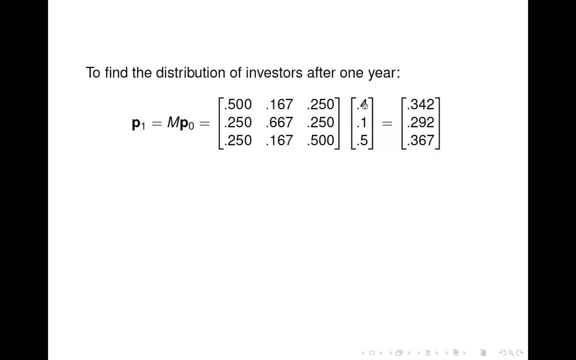 We take our transition matrix, multiply it by the current state value. Uh, which is this one, and uh, that gives us this vector here After two years. uh, multiply the transition matrix times the distribution after one year. Alright, so just take that one, slide it in here, do that multiplication and here's. 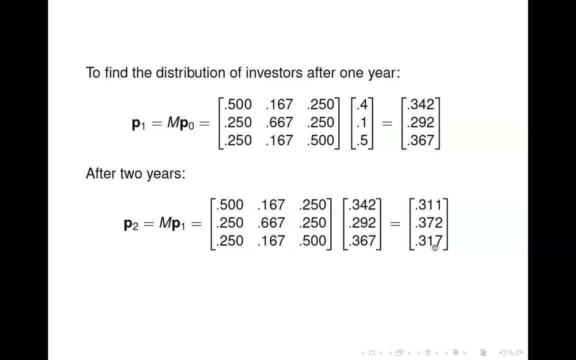 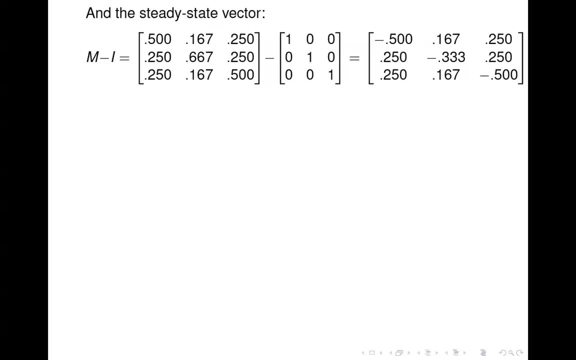 um, what we have after two years, And so you can keep doing that for as many years as you're interested in. Um, if you would like to find the steady state. Okay, So you take this vector, Then you compute M minus the identity, which gives you this matrix, and then you solve. 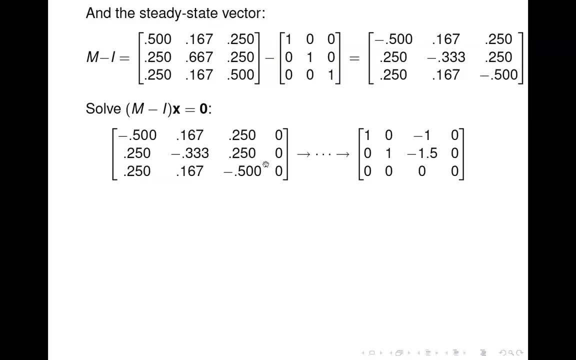 the system M minus I times X equals zero, Um which uh do some row operations. That takes you to this point And uh. so we have uh. X1 equals X3.. X2 is equal to uh 1.5 times X3.. 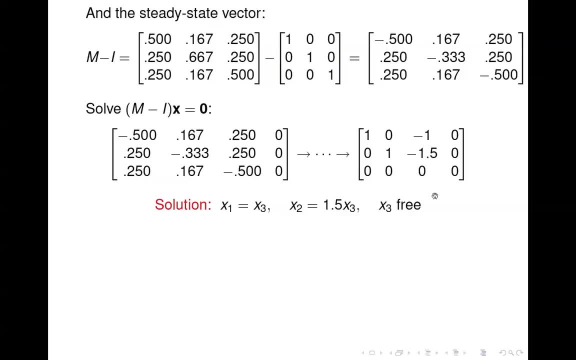 X3 is free. You should always end up with a free variable here, because otherwise, uh, you have the unique solution, Which is the zero vector, and that's, uh, that's an error, Right, Because it should always be a free variable. 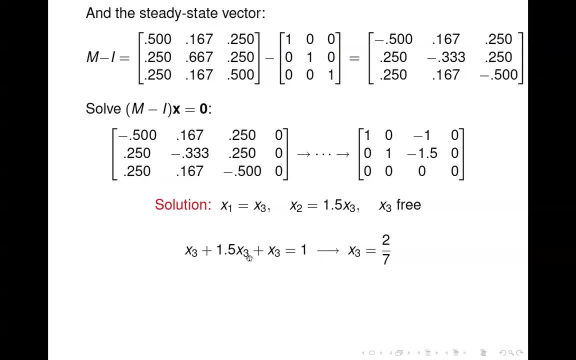 Alright, uh have the uh uh elements. sum to one Tells us that X3 is two-sevenths, And so our steady state vector looks like this: Two-sevenths, three-sevenths, two-sevenths. 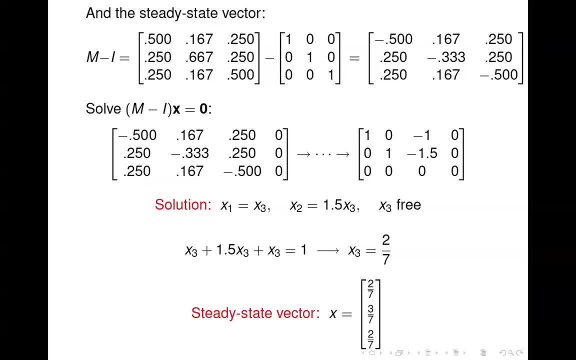 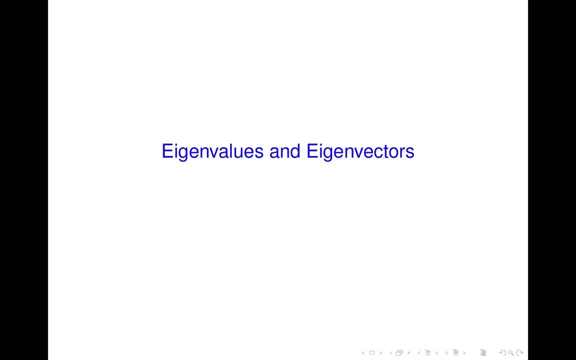 Um, and I didn't actually compute those uh probabilities, um, but um, this is the method that you would use. Okay, today our topic is eigenvalues and eigenvectors, The equation that we're interested in when uh trying to find eigenvalues and eigenvectors. 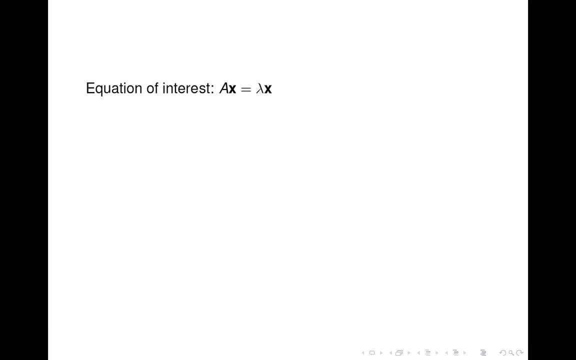 is this one: AX equals lambda times X. Here A is an n by n matrix. X is a vector in Rn, Okay, And lambda is a scalar. So we're essentially asking um: can you find X and lambda? We know, we don't know either of those, but can you find X and lambda such that when you 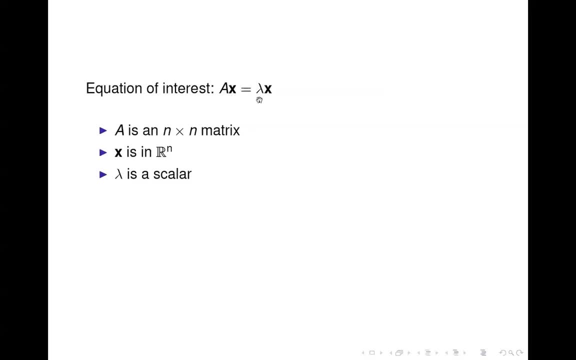 multiply A times X, you get the same result as simply scaling X by lambda. So if X is not equal to zero and satisfies AX equals lambda X, Then it's said to be an eigenvector of A with associated eigenvalue lambda. 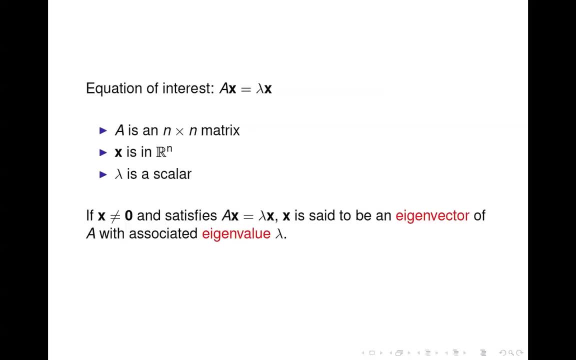 Okay. So we require that eigenvectors not be zero um cause. clearly the zero vector satisfies this equation. So we're looking for um non-zero solutions. So X would be an eigenvector, lambda an eigenvalue. Now we've seen a similar system uh to this when we were uh finding the steady state. 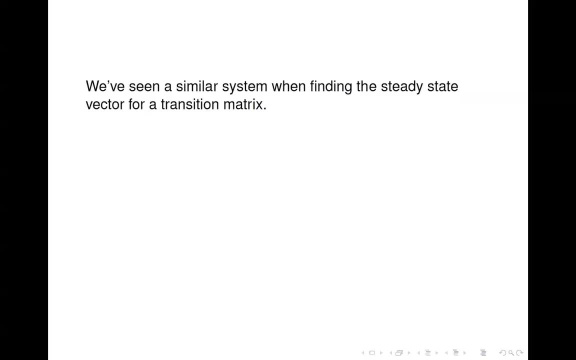 vector for uh a transition matrix, back when we were looking at Markov chains And that, if you remember, uh looked like this: we had MX equals X. So we wanted uh to know uh if there was a vector X such that you apply the transition. 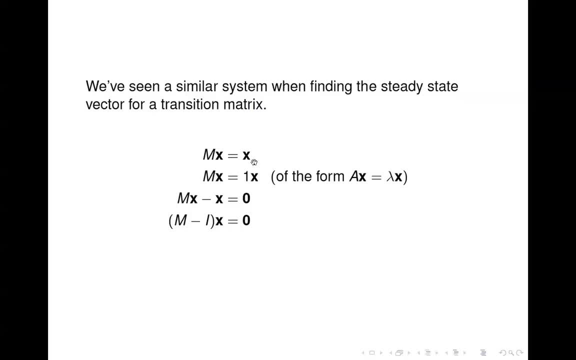 matrix to it and you get the same vector back. Alright, Um, if you just uh look at the X here as having a coefficient of one, uh, so we have: MX equals one, So that's one times X. Then it's of the same form as our eigenvector and eigenvalue equation. AX equals lambda X. 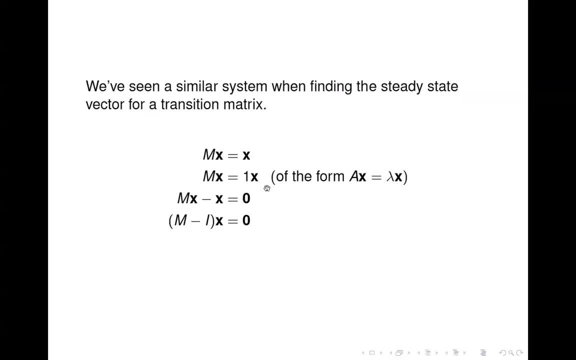 So we have seen systems like this before and we're going to solve them in a similar way as we, as we did when we found the steady state vector. So if you remember what we did then, we took the X over to the other side and factored. 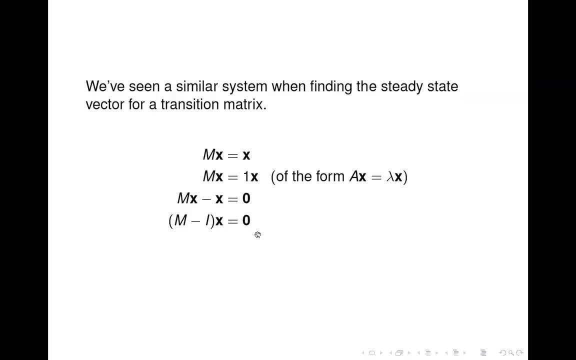 it out and we ended up with M minus I times X equals zero um, and that was the equation to solve. Again, steady state vector. We're going to do a similar thing, uh, with our eigenvector system. uh, bringing the lambda. 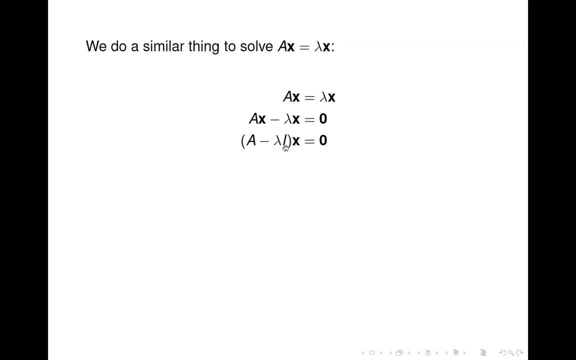 X to the other side. factor out X and we end up with A minus lambda times the identity matrix. uh times X equals zero. So this is a system that we need to solve Now. it's complicated here, more so than with the Markov chains, because we don't know what. 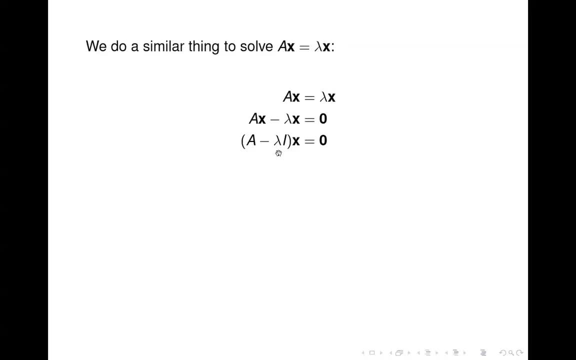 lambda is. We don't know X and we don't know lambda. Okay, All right now, uh, let's think about this a bit. We know that, um X to be an eigenvector, can't be the zero vector. 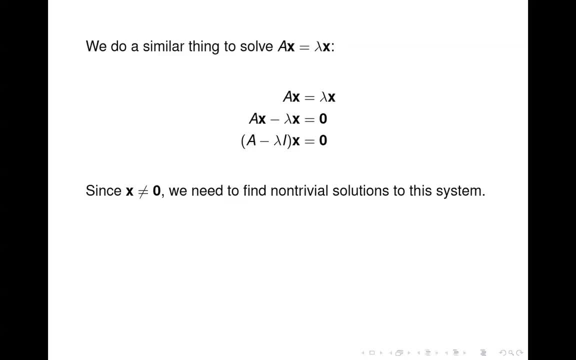 So we have a homogeneous system here and we want to find non-trivial solutions to it. All right, so some uh things that we know: uh, this system is going to have non-trivial solutions if, uh, it has free variables. 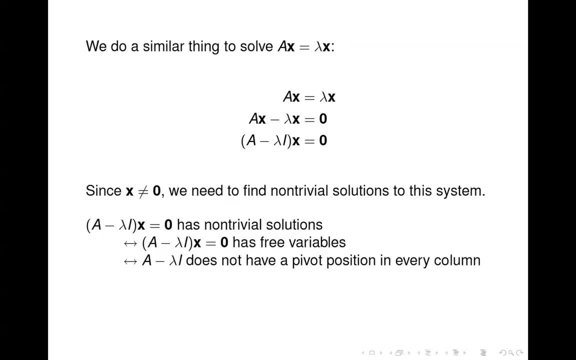 Okay, And it has free variables. if the matrix A minus lambda I does not have a pivot position in every column- And that happens when A minus lambda I is not invertible, right, because if it doesn't have a pivot position in every column, has fewer than N pivot positions, it's not invertible. 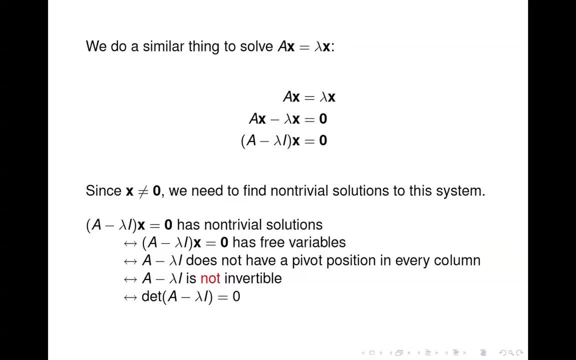 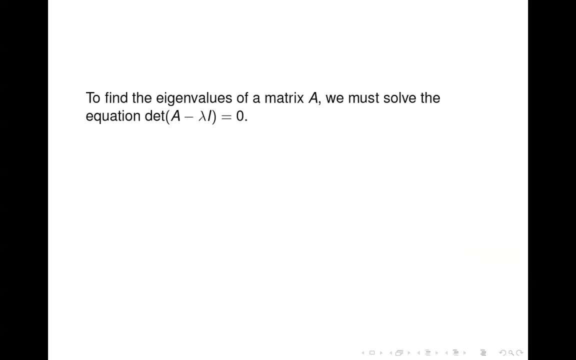 And, uh, that happens when the determinant of that matrix, A minus lambda I, is equal to zero. And this last uh item here is the key to how we are going to find eigenvalues. Okay, so we're going to compute the determinant of A minus lambda I and that actually turns. 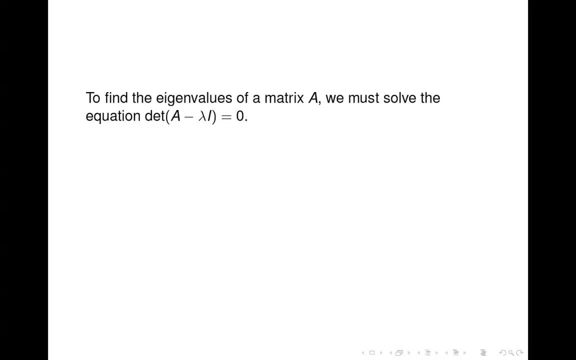 out to give us a polynomial And we're going to set it equal to zero and uh, solve for lambda. Once we have the eigenvalues, then we can proceed to finding the eigenvectors. Okay, Uh, by plugging in, uh, what we know for lambda, for the eigenvalues, and then we just 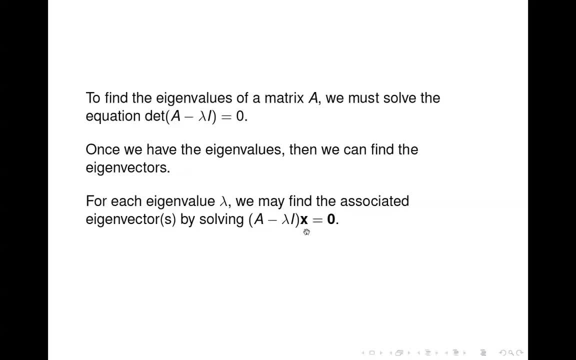 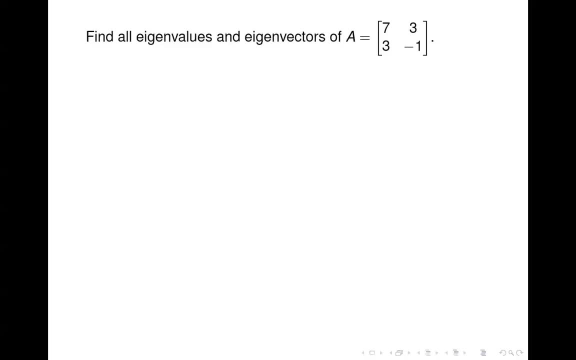 have a simple, uh homogeneous system to solve to find X. Okay, so let's look at an example. Here's a matrix A, It's a two by two. We first find the eigenvalues of A by solving the determinant A minus lambda I equals zero. 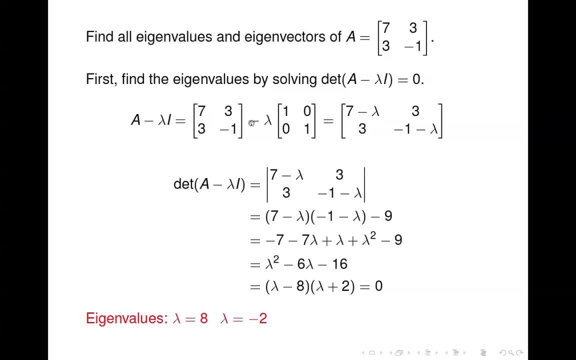 So here's A minus lambda I. Here's A minus lambda I. Here's A minus lambda times the identity matrix. Okay, So we end up, basically, we're- uh, what you end up with is just subtracting lambda off the diagonal elements. 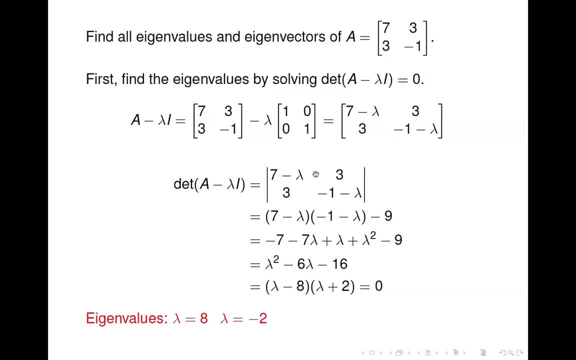 And then we want to take the determinant of that matrix. So we take the determinant, do the crisscross, uh and uh, we get this stuff And we, uh, expand, put it all together and uh, then factor it. 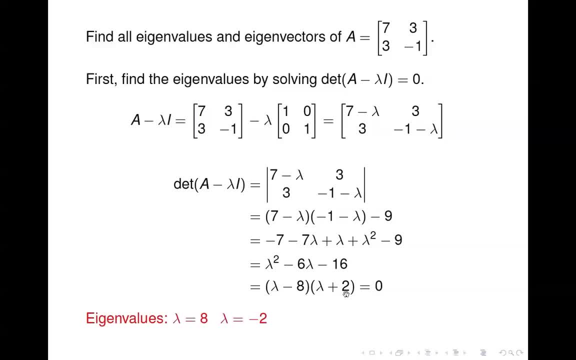 And when we factor it we get lambda minus eight times lambda plus two And we set that equal to zero. right, because that's what we want. the determinant of this matrix: to equal zero. And clearly the solutions are: lambda equals eight and lambda equals negative two. 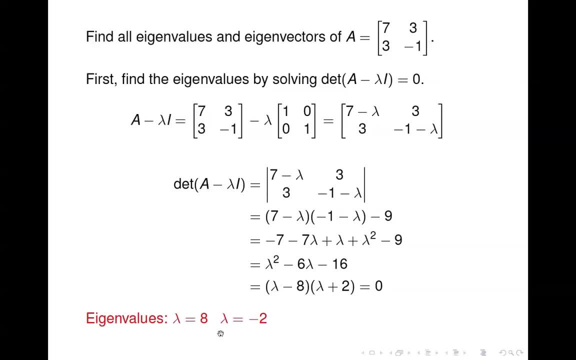 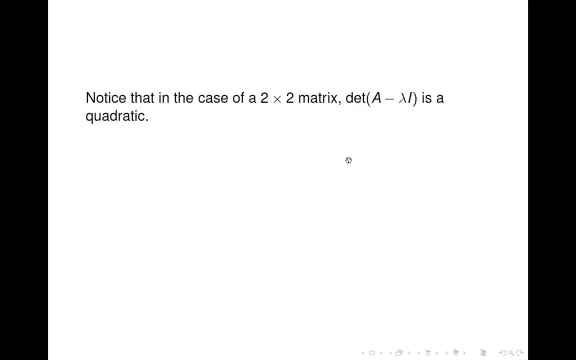 So those are our eigenvalues, Okay, um, here we ended up. go back, uh, we ended up with a lambda squared minus six, lambda minus 16.. So we ended up with a quadratic, uh function, So a two by two matrix. we ended up with a quadratic. 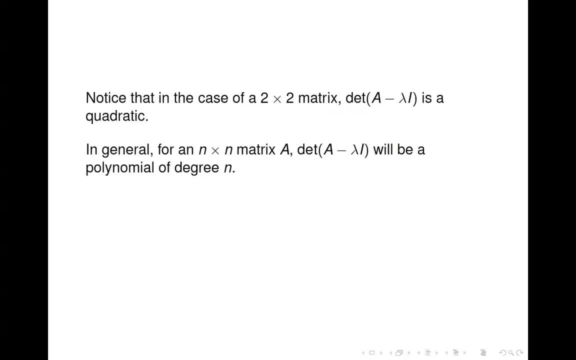 In general, if you have an n by n matrix, then the determinant of A minus lambda I will be a polynomial of degree n. So for a three by three, you get a cubic function. Four by four you get a degree four, and so forth. 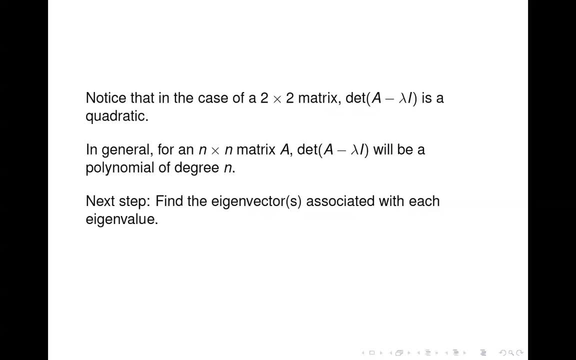 Okay, so at this point we have two eigenvalues for A And uh. we want to find the eigenvectors assoc or eigenvector or eigenvectors associated with each of these eigenvalues. So let's start off with: lambda equals eight. 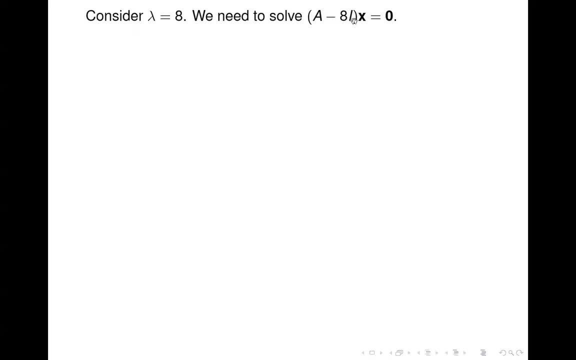 Um, so we want to solve A minus A minus lambda I. lambda in this case is eight. So A minus eight I times X equals a zero vector. So first we need to compute A minus eight I, and there it is, And then we set up that homogeneous system. 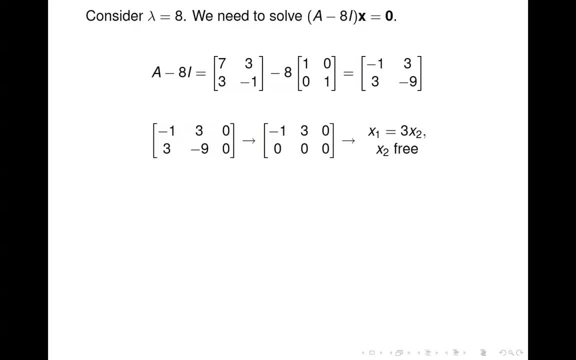 And remember that. Remember that the whole point of finding the eigenvalues was so that we would have a free variable. And so if you end up working on problems and you're trying to find an eigenvector and you don't end up with a free variable, then you've made a mistake somewhere. 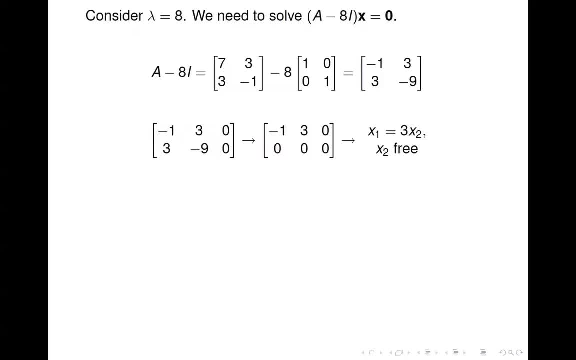 Either you don't have a correct eigenvalue or you you made a mistake in solving this system, Um. so you should always end up with um at least one free variable, so that the system has non-trivial solutions. So in this case, uh, we end up with X. one equals uh, three by two. 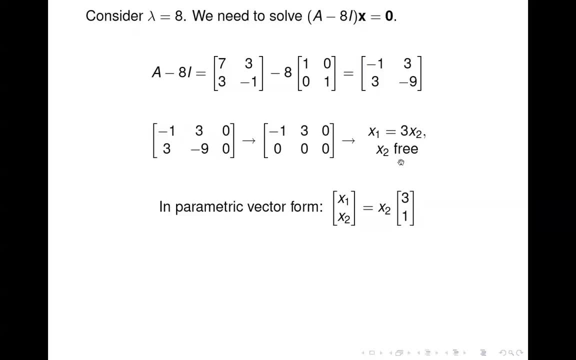 X, two is free. So if we write it in parametric vector form, it looks like this: And uh, so that tells us that any multiple right, any vector of this form multiple of three, one is an eigenvector of a corresponding to lambda equals eight. 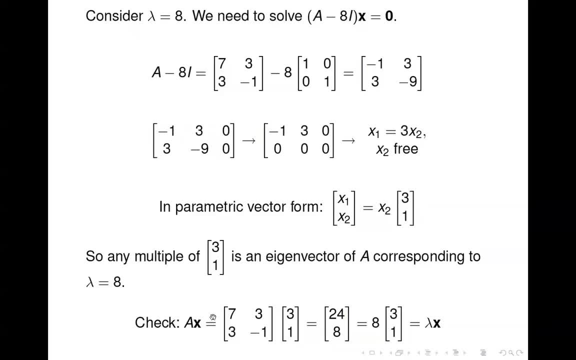 You can check that, uh, to make sure it works: AX should equal lambda X. So if we multiply A times X, Here's A, here's X, We end up with a vector 24, eight, and we can factor out lambda, which is eight. 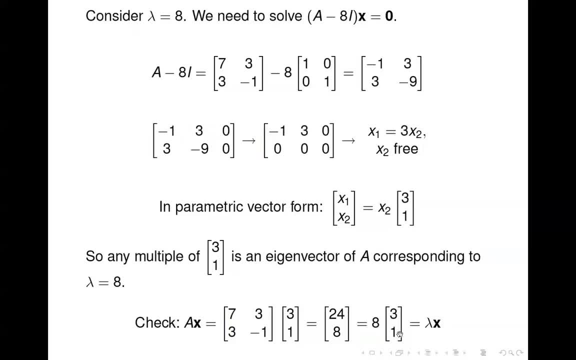 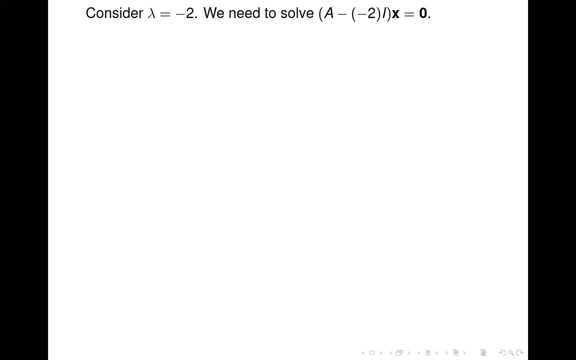 And, uh, that we get eight times three. eight times one and three one is our vector X, So that's equal to lambda X. So it works out. This is an eigenvector corresponding to lambda equals eight. All right, We got another eigenvalue to look at. uh, lambda equals negative two. 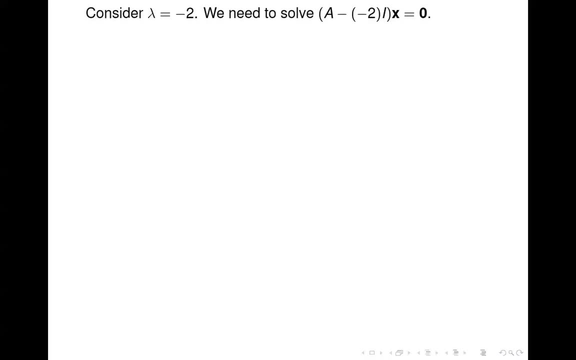 So we need to solve A minus lambda I. X equals zero. again for uh, lambda equals negative two. So we got A minus minus uh, two times. I is just eight plus two times the identity, which is this matrix, And we set up the homogeneous system. 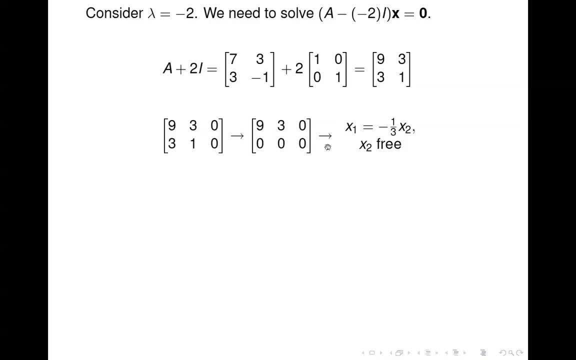 And again do one row operation, The second row goes away. We got a free variable And here's our solution. So if we write it in parametric vector form, we get this And uh, so that tells us that any multiple of the vector negative one third one is an. 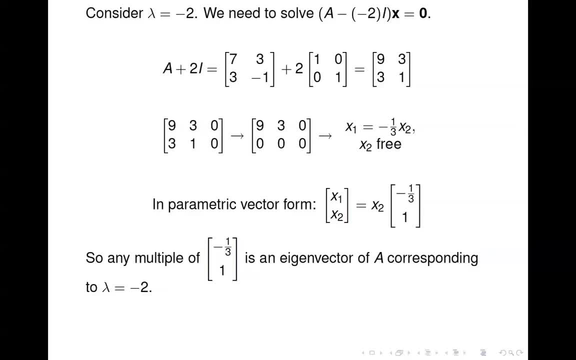 eigenvector of A, corresponding to the eigenvalue negative two. So um, and you can check again like we did last time- Multiply A times X, You get two negative six, And that is equal to negative two times negative one, three, which was the eigenvector that. 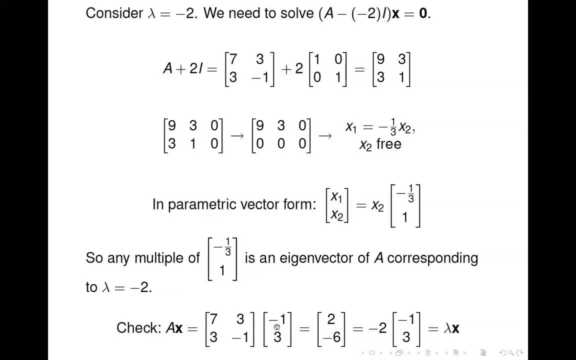 I picked Um, You, you. you might be saying, hey, that didn't look like, uh, this one that we got here And it doesn't because, uh, I just multiplied it, scaled it because, remember any multiple. 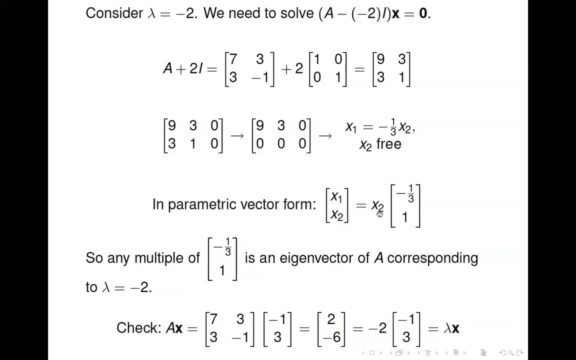 of this vector is an eigenvector, So I just uh chose X two to be three, and uh scaled it, And so uh, three times negative. one third gave me the negative one, and then three times one gave me three. 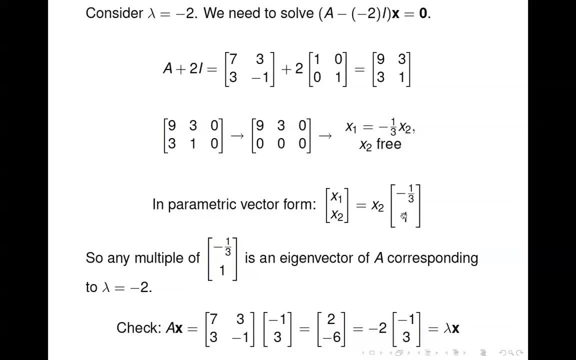 And I did that just to get rid of the fraction there. But any multiple, Any non-zero, Any non-zero multiple, I should say Any non-zero multiple of this vector would be an eigenvector. uh, corresponding to lambda equals negative two. 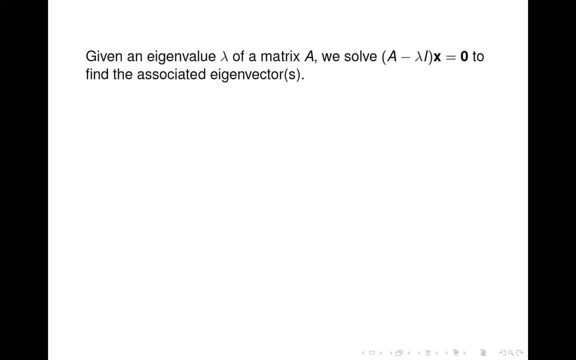 Alright, Um, So given an eigenvalue lambda of a matrix A, we solve this homogeneous system: A minus lambda. I times X equals zero to find the associated eigenvector or eigenvectors. Alright, Now So a little bit of terminology here. 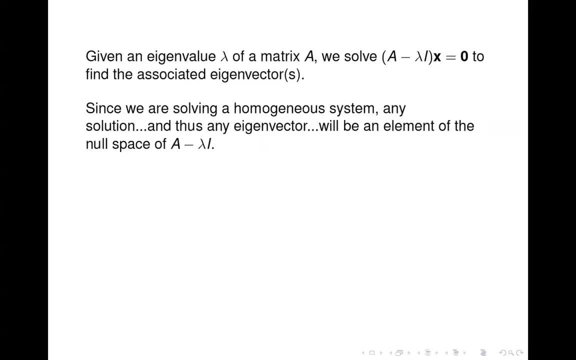 Think back um to uh, the previous chapter. We talked about the null space of a matrix And, uh, remember, the null space of a matrix is just the set of solutions, uh, to the homogeneous system involving that matrix. And so, if you look at this uh system we were solving to find the eigenvectors you. 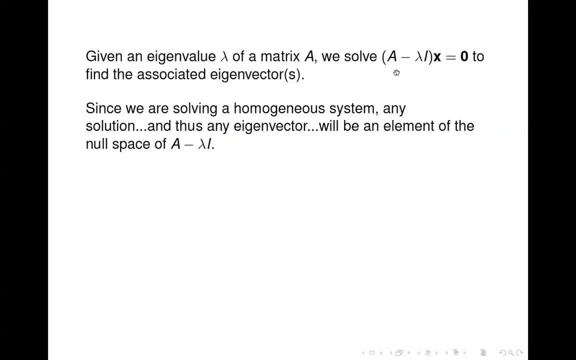 can see, it's a homogeneous system. So the set of solutions, uh to this will, Uh, Will be um elements of the null space, or actually will comprise the null space of A minus lambda I And uh. we give that space, since it's associated with finding eigenvectors, we give it a special 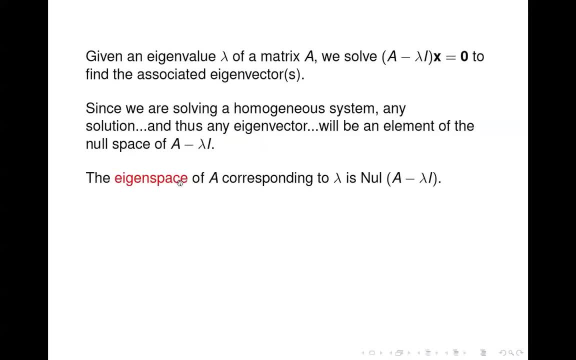 name and call it the eigenspace of A. So the eigenspace of A, corresponding to the eigenvalue lambda, is just the null space of A minus lambda. I Okay Set of all solutions to this system. A minus lambda I times X equals zero. 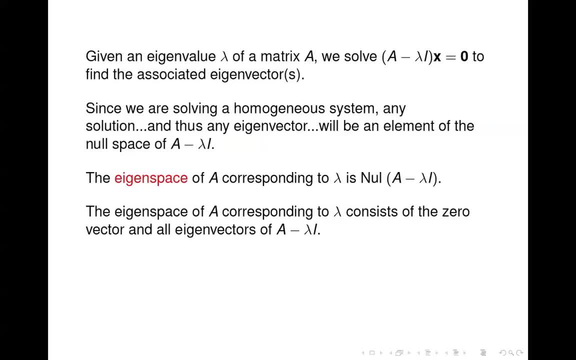 So the eigenspace of A corresponding to lambda consists of the zero vector right, because that's in every null space- and, uh, all eigenvectors of A minus lambda. I Therefore a basis for the eigenspace of A corresponding to lambda. 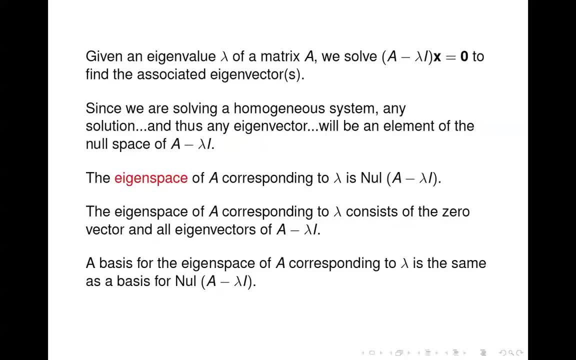 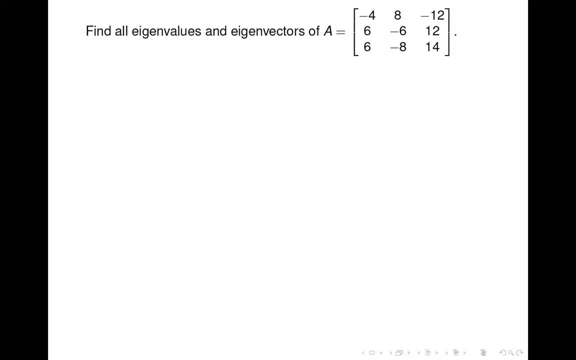 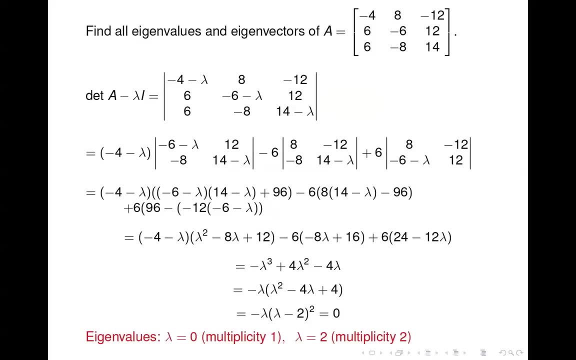 So the eigenspace of A corresponding to lambda is the same as a basis for the null space of A minus lambda. I, Okay, Let's look at another example. Uh, let's find all the eigenvalues and eigenvectors of this matrix A. So if we start off, uh, 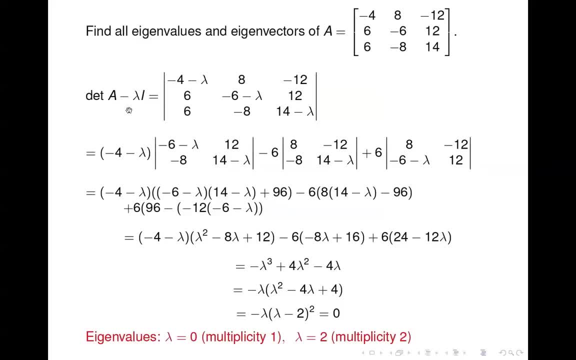 to find the eigenvalues. um, take the determinant of A minus lambda I and uh. here it gets a little complicated because we've got a three by three, So we have to expand about, uh, one of the rows or columns. 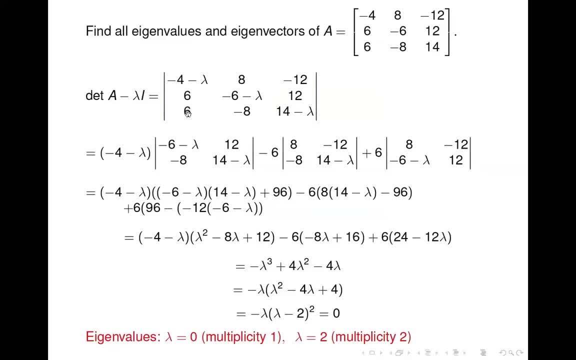 I expanded about the first column, And so we get negative four minus lambda times the determinant of this two by two matrix here. So that's what you see right here. Then it's: uh, since this is a plus position, next be minus. 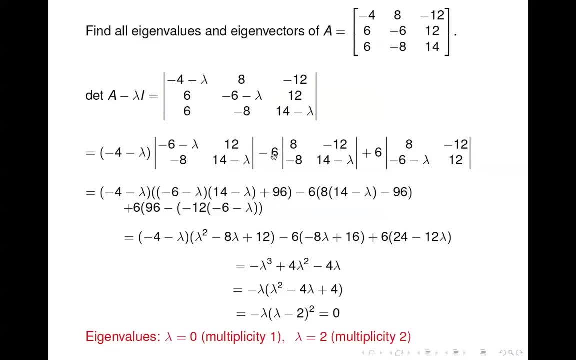 So that's where the minus six comes from, And then it's the matrix that you get when you delete that second row in the first column. So we'll get this. And then, uh, it's a minus term, So the next one's plus. 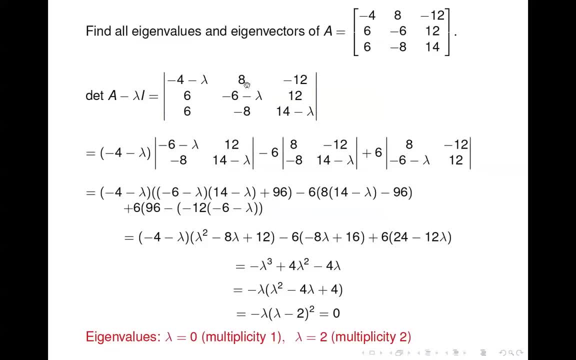 So I get plus six times, uh, this little two by two sitting up here in the uh upper right corner And uh, then it's just algebra. you know, take these two by two, determinants, do some algebra, Oops. 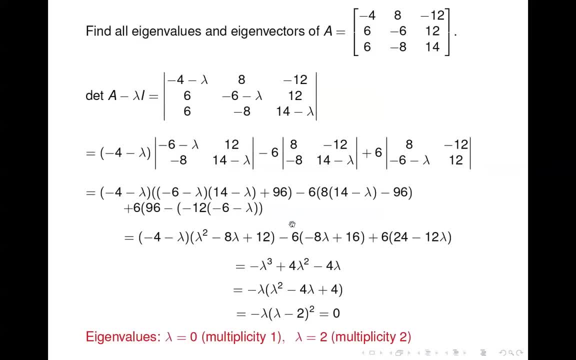 Uh, there we go, Um, and we end up, uh, with this cubic function, which makes sense because three by three matrix, uh is a minus. So we get three matrix and, uh, we end up being able to, um, rewrite it like this: negative. 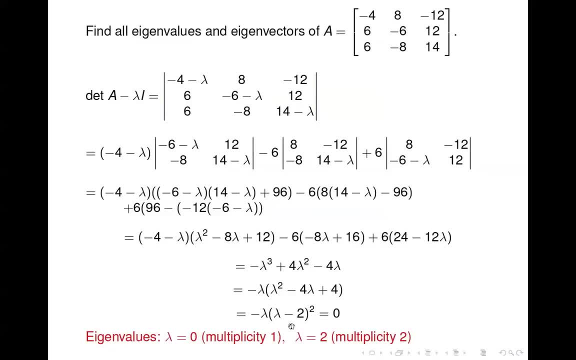 lambda times lambda minus two squared equals zero. And so clearly, uh, lambda equals zero is a solution and lambda equals two is a solution. Now, in this case, since it's uh, lambda minus two squared, uh, the eigenvalue two, actually. 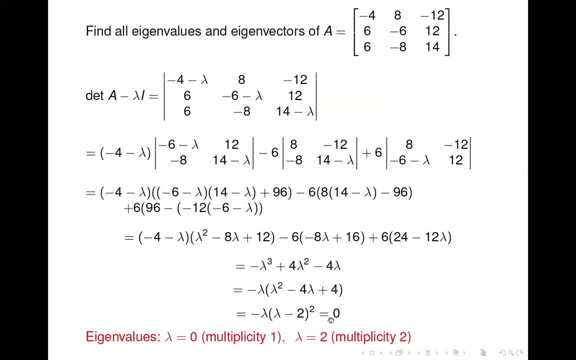 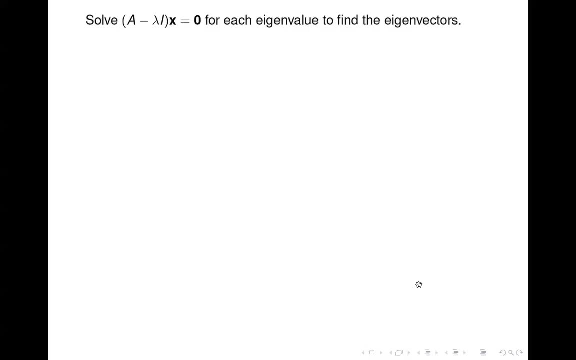 occurs twice because it's a solution twice here. So we say that lambda equals two has multiplicity two. That means it occurs two times. Lambda equals zero. It only occurs once, So it has multiplicity one. All right, Then we need to do the same process as before to find the eigenvectors. 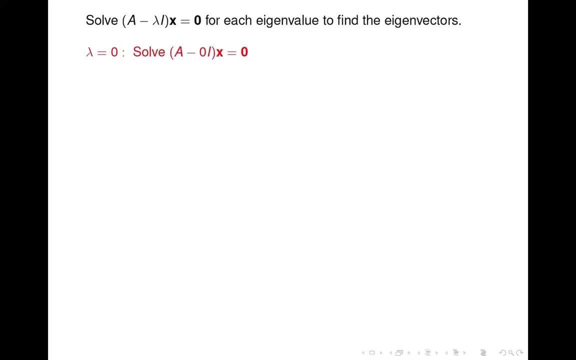 Um, so for lambda equals zero, we need to solve a minus zero times the identity times: X equals zero. So in this case, uh a minus lambda. Okay, I is just a. so we uh set up the homogeneous system and uh get that matrix into reduced. 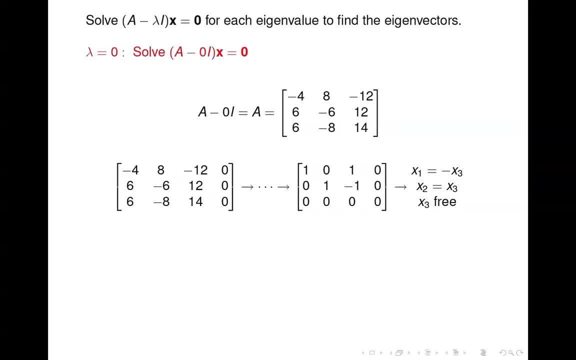 echelon form Um, and here's the solution. So we write that in parametric vector form And uh. so any multiple of negative one, one, one uh, would be an eigenvector associated with lambda equals zero. Okay. 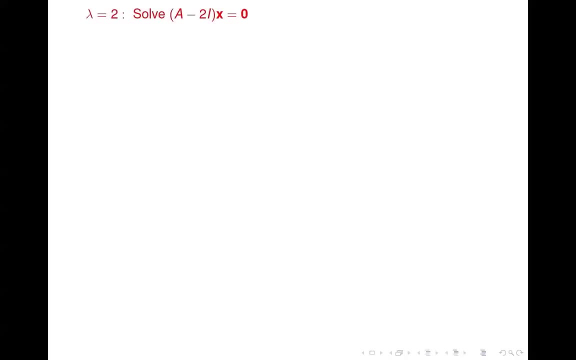 Then we move on to the next eigen value, which is two. So we solve a minus two. I times X equals zero And uh, to compute a minus two. I then set up the homogeneous system and get it in reduced echelon form. 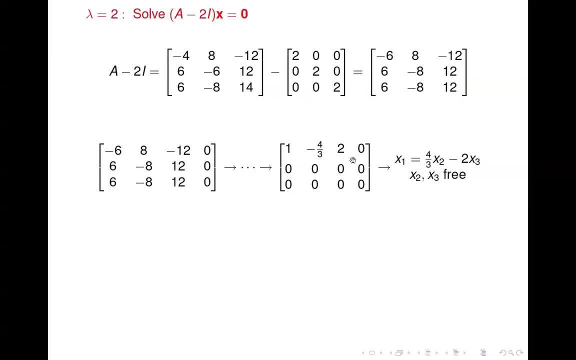 And notice here that we've got two free variables And so we're going to end up with two, uh, linearly independent eigenvectors. uh, here. And sometimes that happens because, remember, lambda equals two. Lambda equals two was um, an eigenvalue that occurred twice had multiplicity two. 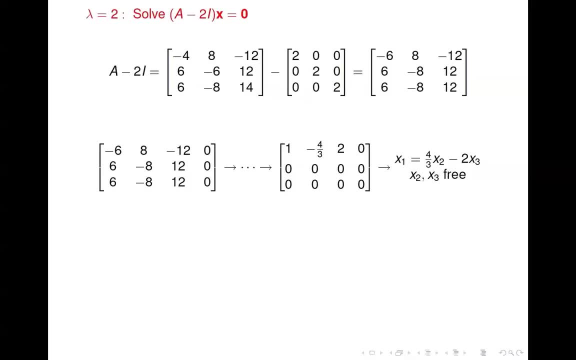 And so, sometimes, in that case, you end up with two linearly independent eigenvectors, sometimes only one. In this case, we're going to have two, because we have two free variables. So, uh, the solution looks like this: uh, every eigenvector of a associated with a lambda. 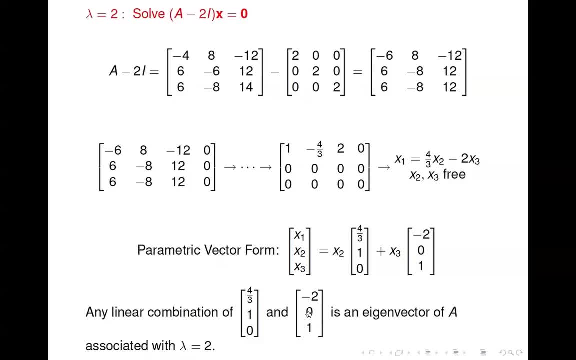 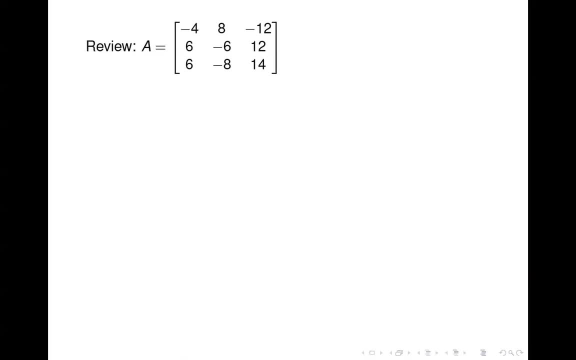 equals two. This is a linear combination of these two vectors And clearly they are linearly independent. So to review this problem we've just looked at, here's our matrix: A um eigenvalues were zero and two For lambda equals zero. we ended up with one eigenvector. uh, lambda equals two. 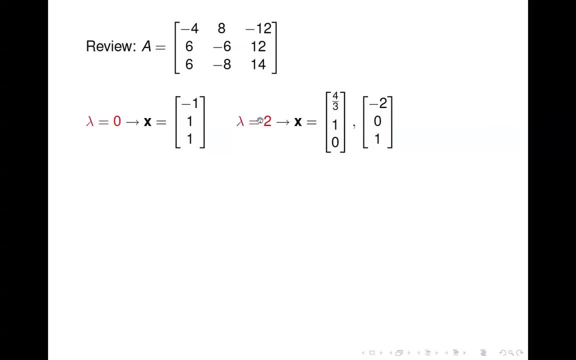 We've got two linearly independent eigenvectors. Now, clearly, any multiple of this one is an eigenvector, This one is an eigenvector associated with lambda equals zero, And any linear combination of these two is an eigenvector associated with lambda equals. 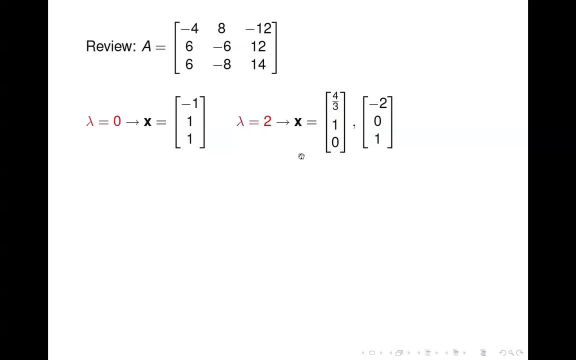 two. But we're really concerned about how many linearly independent eigenvectors we have, And so from lambda equals zero, we got one. From lambda equals two, we got two. Alright, so we can say that the vector negative one, one one, is a basis for the eigenspace. 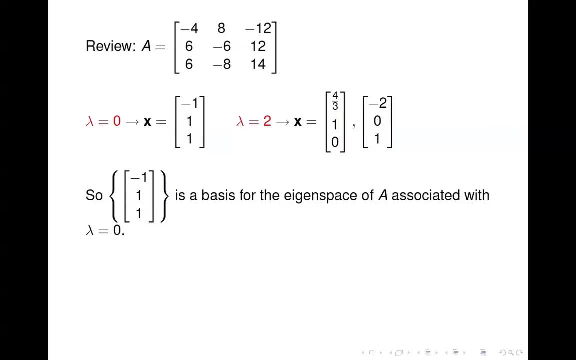 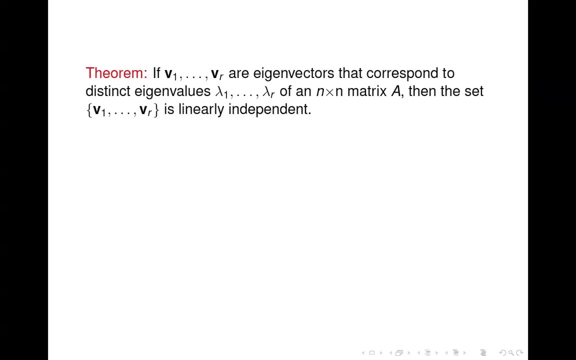 of A associated with lambda equals zero. Similarly, these other two vectors will form a basis for the eigenspace of A associated with lambda equals two. Alright, this brings us to a theorem which says: if uh, V1 through Vr are eigenvectors, 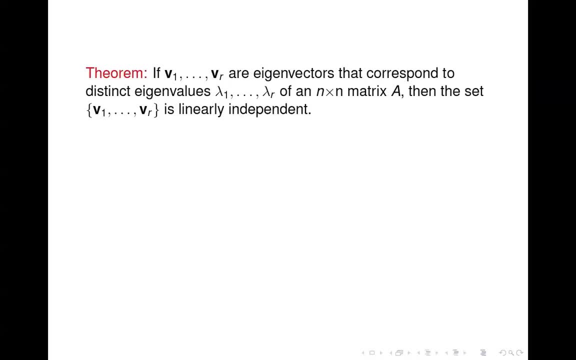 that correspond to distinct eigenvalues, lambda one through lambda r, of an n by n matrix A. So uh, lambda equals two. Then the set V1 through Vr is linearly independent. Now put in uh a little simpler terms. 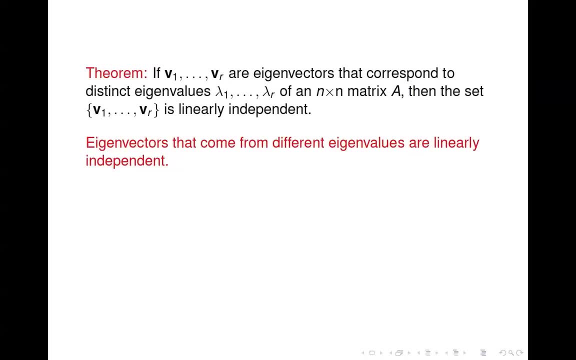 This just says eigenvectors that come from different eigenvalues are linearly independent. Eigenvectors that come from different eigenvalues are linearly independent. So from our previous example, right, this first one, uh, came from a different eigenvalue. 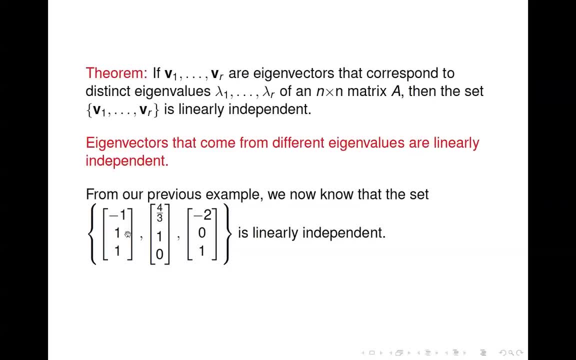 from the second two. So we know that, um, this set is linearly independent, right? because the the latter two came from the same eigenvalue, but they were linearly independent. We knew that from uh before, And then when you throw in this other one that came from the other eigenvalue, we know. 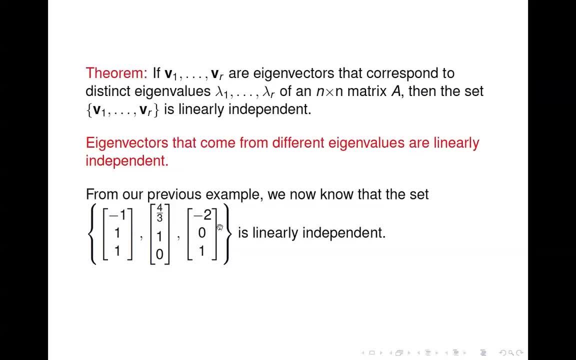 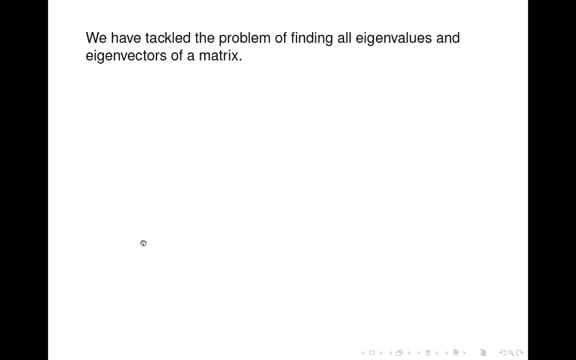 that this set is linearly independent because of the theorem. Because they came from different. uh, the first one and the second two came from different eigenvalues. Alright, um, we're gonna hit that a little bit more in the next section. um, but uh, 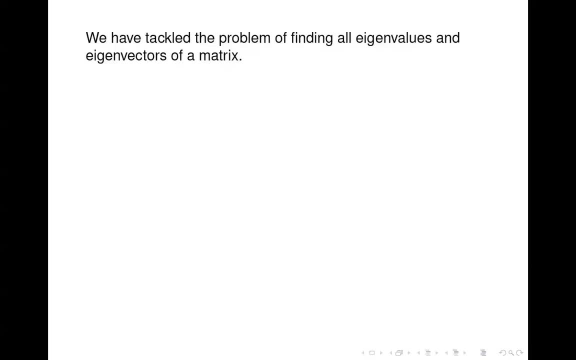 we'll leave it at that for right now And, um, I always want to talk about, um, uh, a little easier problem. okay, What we've done so far is just taken, basically done the hard problem. Here's a matrix: find all the eigenvalues and eigenvectors. 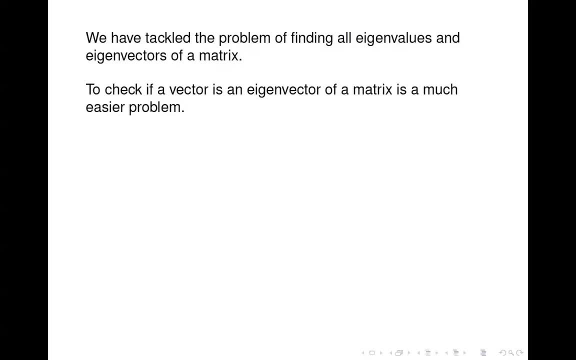 But sometimes, uh, you just want to know if a given vector um is an eigenvector of a matrix, And that is a much easier problem, okay? So suppose we just want to know if this vector x given here is an eigenvector of the matrix. 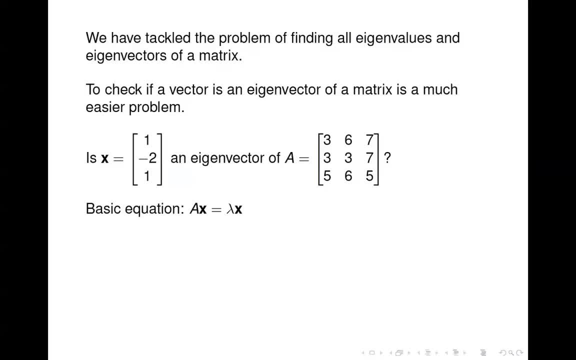 a For this. go back to the original equation and think: um, does ax equal lambda x? Well, we can multiply a times x. That's trivial right. And then how would we know if it's an eigenvector? Well, the result of a times x should be some scalar times a. 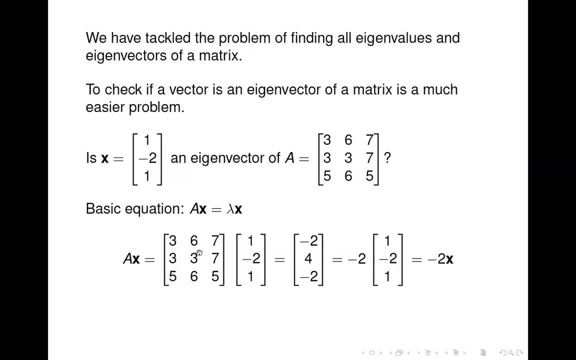 Okay, So we multiply a times x and in this case we get this vector here and notice that I can factor out a negative 2 and I end up with negative 2 times this vector, which is the original x. So in this case we have: ax equals negative 2 times x. 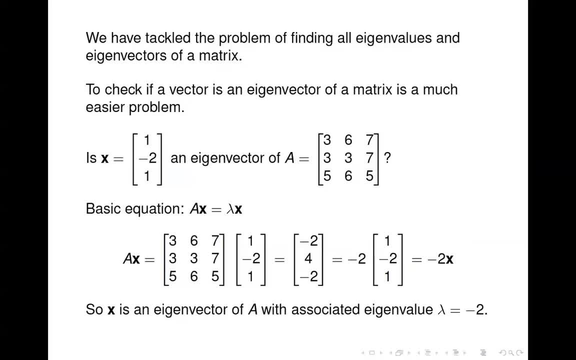 So that means that x is indeed an eigenvector of a and the associated eigenvalue is negative 2.. Okay, So we didn't have to solve any systems of equations or take determinants or anything like that. It was just a simple plug it in to the basic equation and see if it satisfies it. 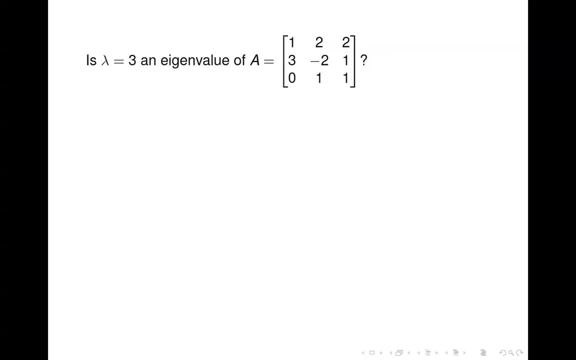 Alright. another similar question is: given a scalar value check to see if it's an eigenvalue of a matrix, And again, you don't have to go through the process That we were doing to find the eigenvalues. okay, just to check to see if a number is. 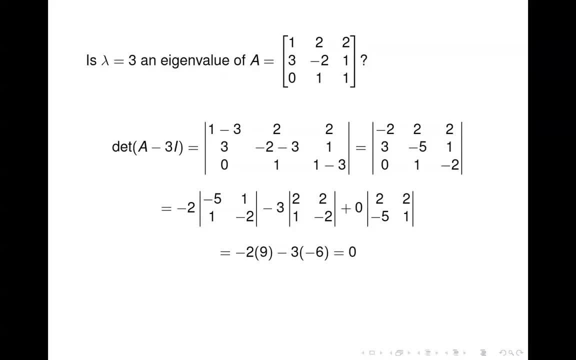 an eigenvalue. You need only look at the determinant of a minus lambda i, where lambda is the value that you're given. So in this case we look at the determinant of a minus 3 times the identity. So we set up that matrix, take its determinant and in this case we end up with 0.. 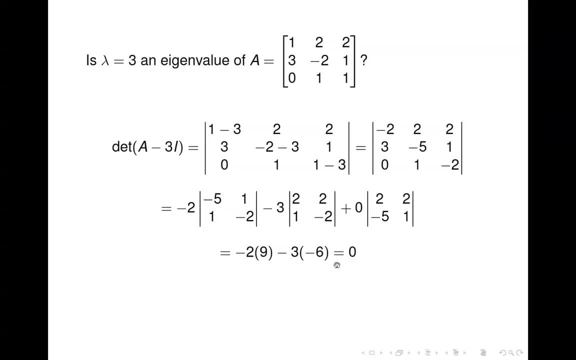 And so the determinant of a minus 3i is equal to 0. That tells us that 3 is indeed an eigenvalue of a. If we didn't get 0, then it wouldn't be an eigenvalue. Okay, a little more terminology. 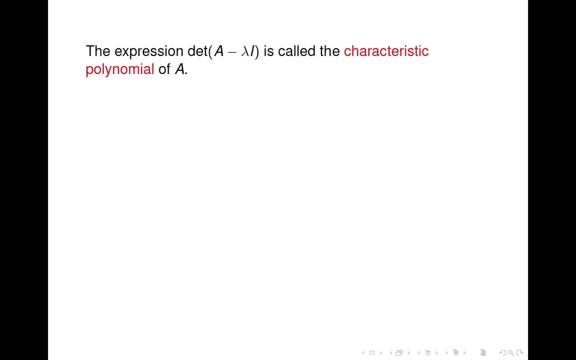 This expression, the determinant of a minus lambda. i okay, that's what you end up with when you are trying to figure out the eigenvalues of a matrix, And we said that you end up with a polynomial there. It's called the calculus. 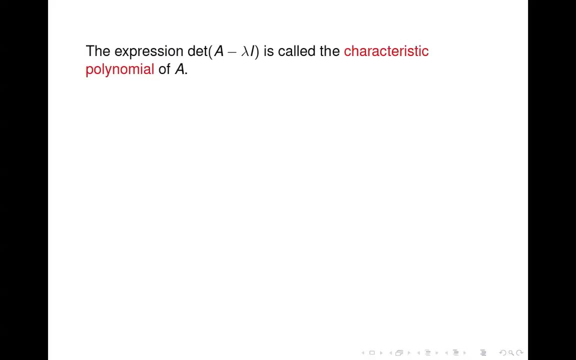 Okay, It's called the characteristic polynomial of a, And when you set it equal to 0, then we call it the characteristic equation of a. So the characteristic polynomial is just what you get when you take the determinant and then you set that equal to 0 and we call that the characteristic equation. 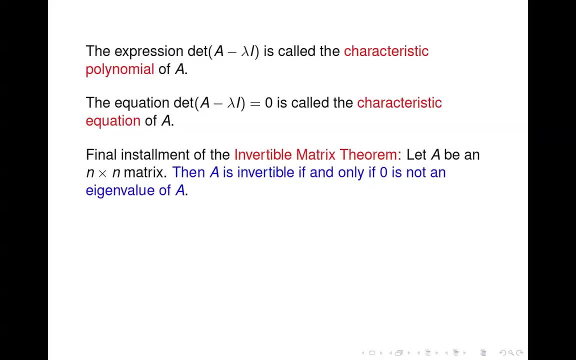 Okay, we have now the final installment of the invertible matrix theorem. So a is an n-theta, A is an n-by-n matrix. A is invertible if, and only if, 0 is not an eigenvalue of a. Okay, 0 is not an eigenvalue of a. 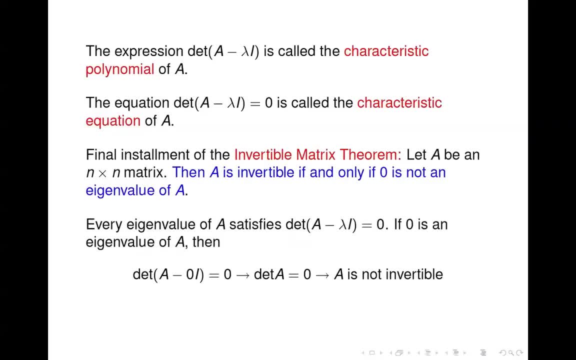 And actually it's pretty easy to see that, if you think about it a little bit, Every eigenvalue of a satisfies the characteristic equation which is the determinant of a minus lambda equals 0.. Okay, Okay, So if it's an eigenvalue of a, then we'd have the determinant of a minus 0 times i would. 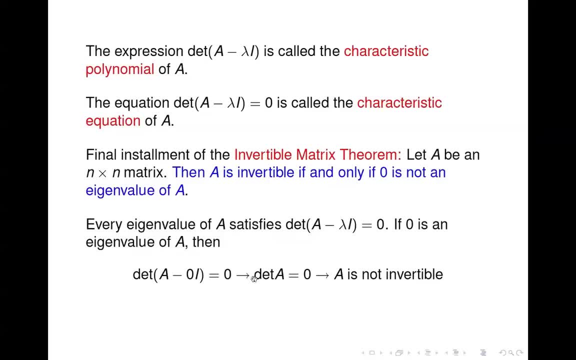 be 0. But a minus 0 times i is just a. So we would have: the determinant of a is equal to 0. And that means that a is not invertible. Okay, So therefore 0 can't be an eigenvalue of a if a is invertible. 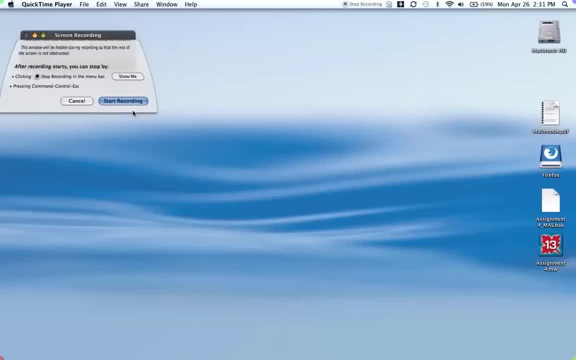 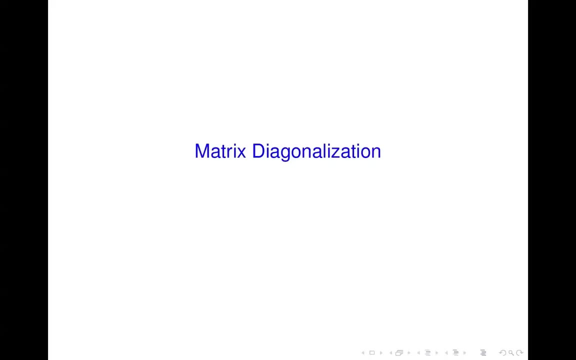 All right, Let's talk to you later. Bye, Today, about matrix diagonalization First, we're going to introduce the concept of a similar matrix. So if a and b are n-by-n matrices, then we say a is similar to b and also b is similar. 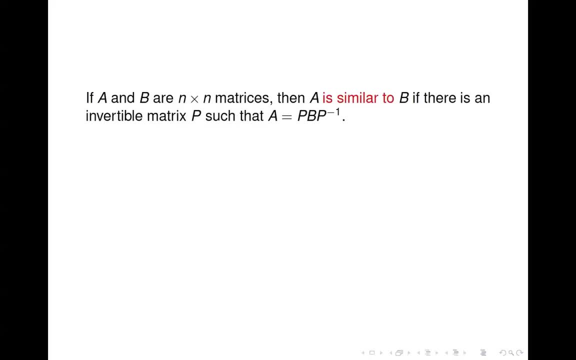 to a if there's an invertible matrix, P, such that a is equal to P, B, P, inverse. Okay, And we have this theorem which says: if you have two matrices which are similar, then they have the same characteristic polynomial and hence the same eigenvalues with the same. 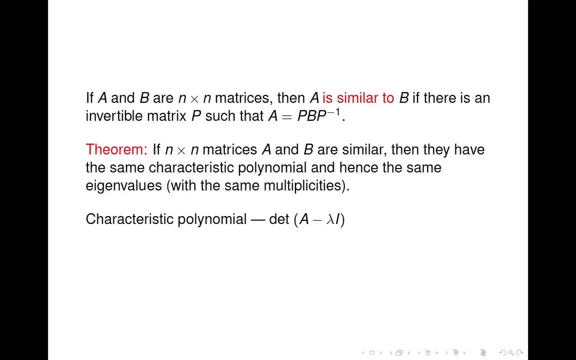 multiplicities. So remember, the characteristic polynomial is just the determinant of a minus lambda i. That's the polynomial that you get when you're trying to find the eigenvalues of a matrix. So this theorem tells us, If you have two matrices that are similar, then they have the same characteristic polynomial. 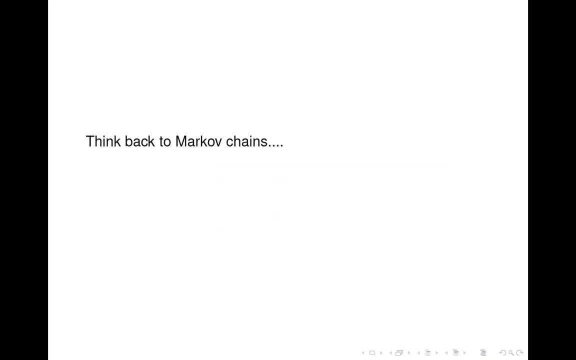 and therefore they're going to have the same eigenvalues. Okay, Now, why is this of interest? Well, think back to our section on Markov chains. We had this sort of equation that to get x1, we multiplied our transition matrix, which 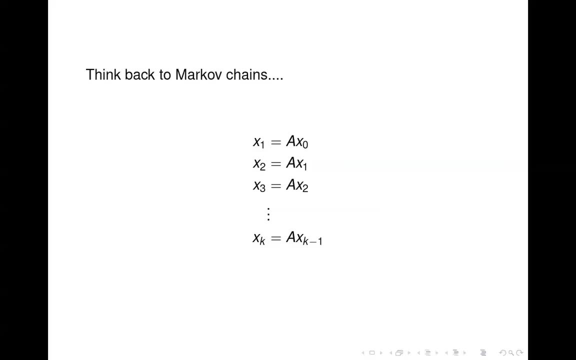 I'm calling a here. So we have x1 times the previous state vector. So for x1, a times x naught a2 is a times x1, and so forth. x sub k is a times x sub k minus 1.. 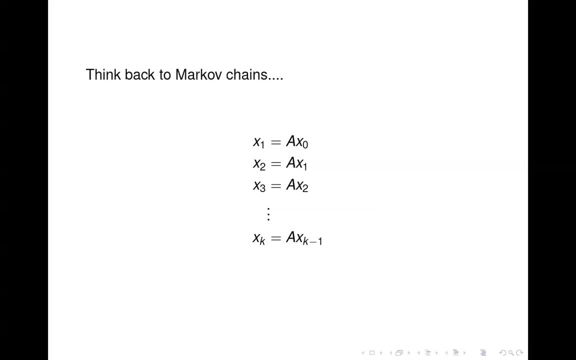 Now we can, if we look at it like this, then to find, say, our state vector at time 10,, then you need to find the state vector at time 9.. And to find the one at time 9,, you need the one at time 8.. 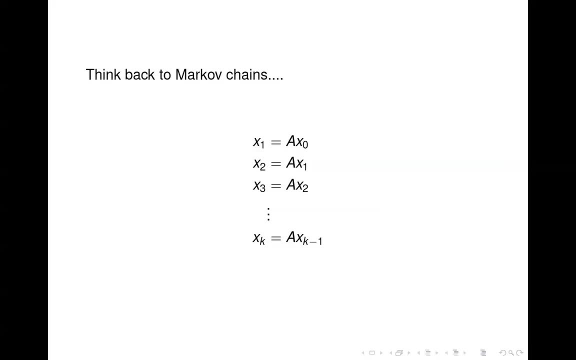 Okay And so forth, And so to compute x sub 10, you need x1,, x2,, x3, up through x sub 9.. Another way to look at it is like this: that we know, for instance, for x2, that's a times. 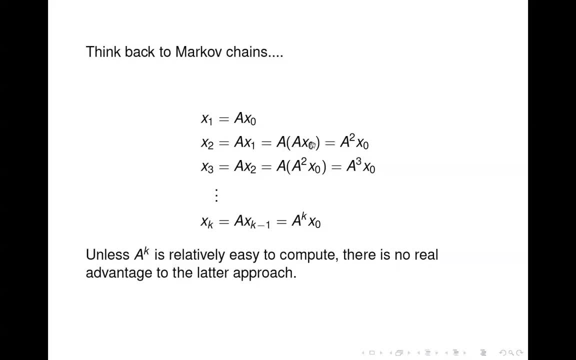 x1.. But we know x1 is a times x naught, So we make that substitution and so we end up with: x2 is a squared times x naught And similarly x3 is a cubed times x naught. 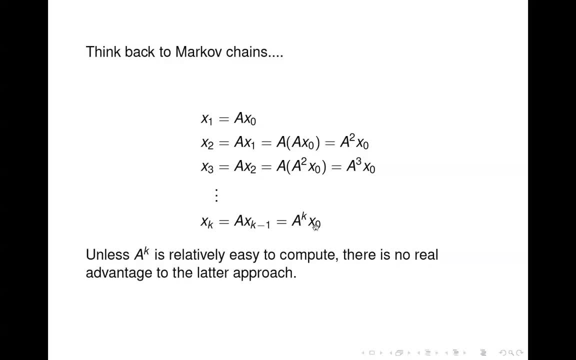 So in general, xk is a to the k times x naught. Now, unless a to the k is relatively easy to compute, this really doesn't help us. However, if a to the k is easy to compute, then we can compute x sub k much more quicker. 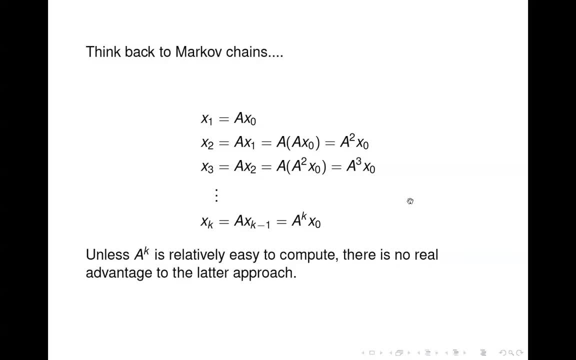 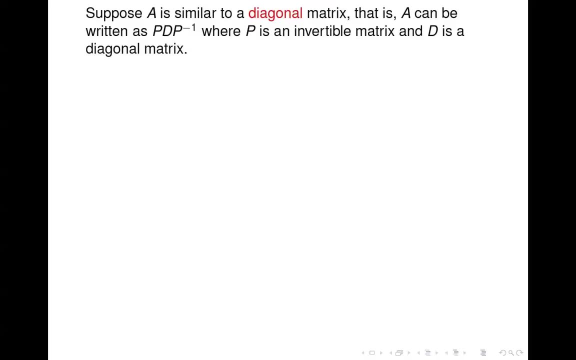 than going through and computing all these subsequent state vectors. All right, So let's suppose that a is similar to a diagonal matrix, That is, a can be written as pdp inverse, where p is invertible and d is a diagonal matrix. 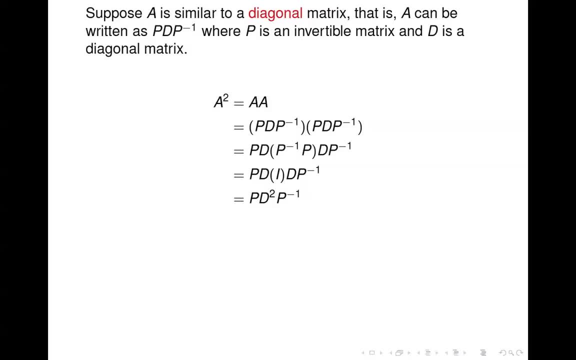 Now what does that get for you? Well, just look at what happens when you compute a squared. A squared is a times a, And when we substitute pdp inverse in for a, we have this. Now, the trick here is to group the p inverse times p together, so we've got p inverse p. 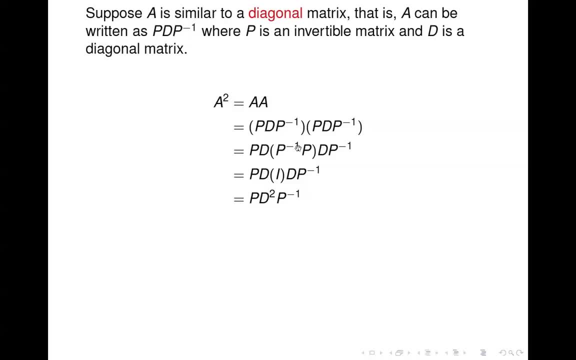 right here in the middle. If we group that together, that's the identity matrix, And so then we get pd times, the identity times, dp inverse, And of course, anything times the identity is just that, anything. And we've got d times d, which gives us d squared. 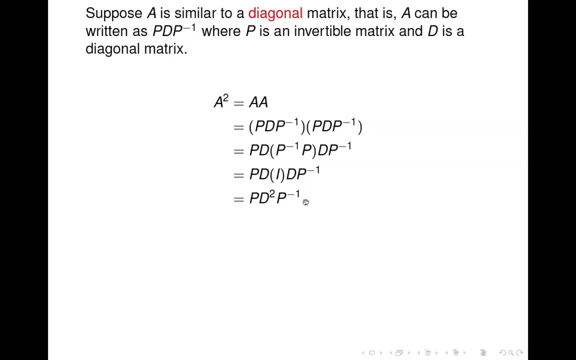 So a squared is pd squared, p inverse. How about a cubed? A cubed is a squared times a. And so we take the a squared, we compute it up here, plug it in times a and do our trick again: re-associate to get the p inverse, p together and we end up with pd cubed, p inverse. 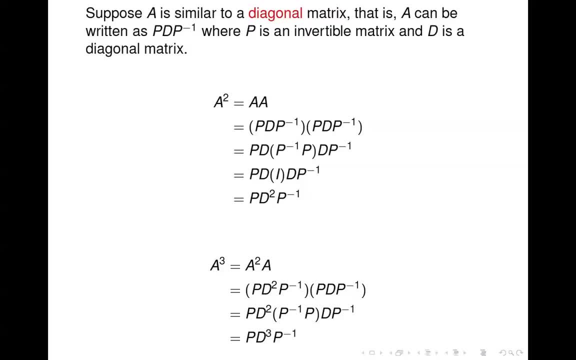 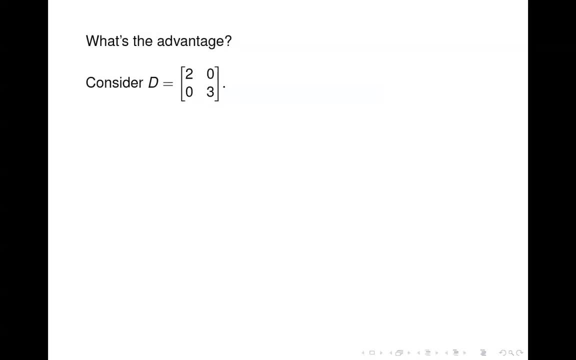 So it looks like in general, a to the k is p times d to the k, p inverse. Now what good is that? Well, let's look at a diagonal matrix. Here's a simple two by two diagonal matrix. If we compute d squared, then notice that we end up with another diagonal matrix and 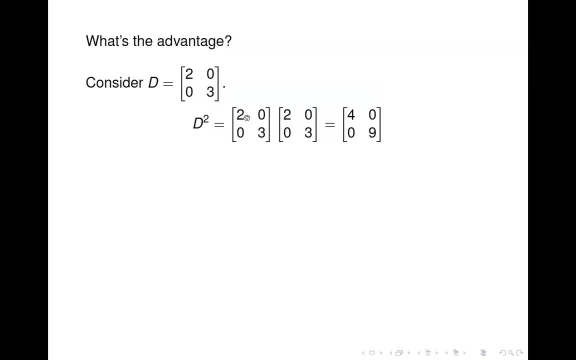 the entries on the diagonal are just the original diagonal entries raised to the second power. So in this case we were computing d squared. So these are the original diagonal entries squared D cubed. We get another diagonal matrix And the entries are the original diagonal entries, cubed. 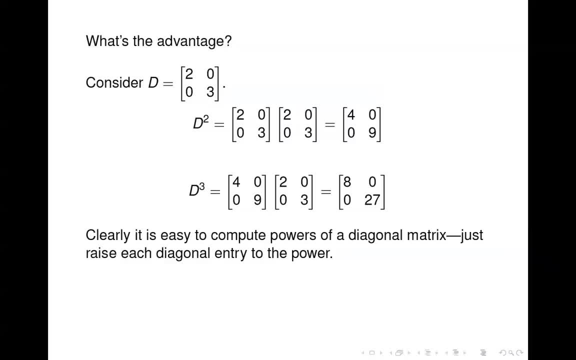 So just looking at this example, it appears that it's easy to compute powers of a diagonal matrix. We just raise each diagonal entry to whatever power we're trying to compute. So if a is similar to a diagonal matrix, computing powers of a is also easy. 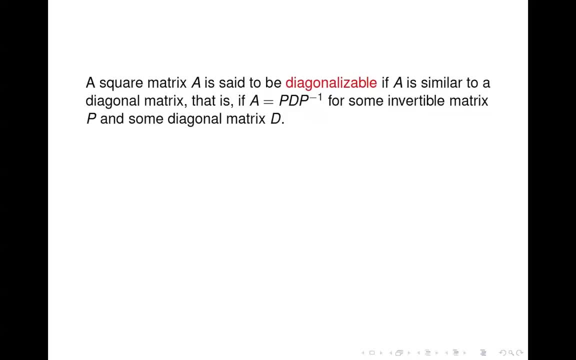 So we say that a square matrix A is said to be diagonalizable if a is similar to a diagonal matrix, That is, if a is equal to pd- p. inverse for some invertible matrix p and some diagonal matrix d. Now here is a very important theorem. 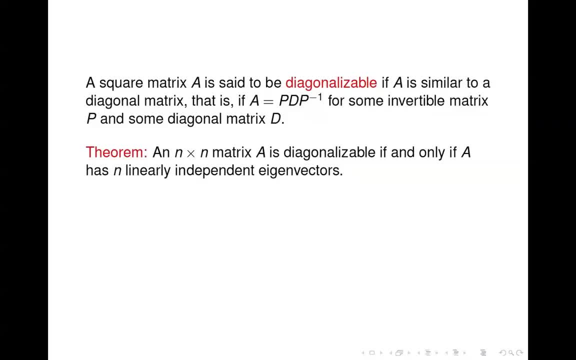 It says an n by n. matrix a is diagonalizable if, and only if, a has n linear limits, So if a is equal to pd p, inverse for some invertible matrix p and some diagonal matrix d, That is, if a has n linearly independent eigenvectors. 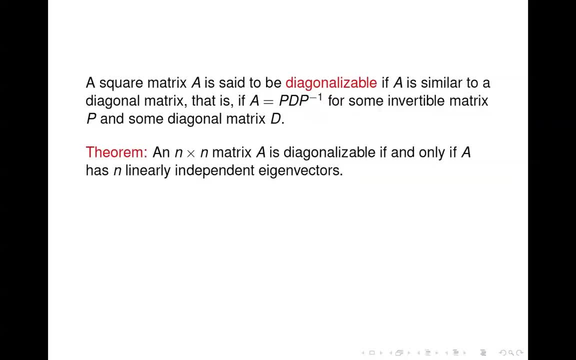 So a is diagonalizable if it has n linearly independent eigenvectors And furthermore, a equals pd, p inverse with d, a diagonal matrix if, and only if, the columns of p are n linearly independent eigenvectors of a. So this theorem not only tells us the condition, 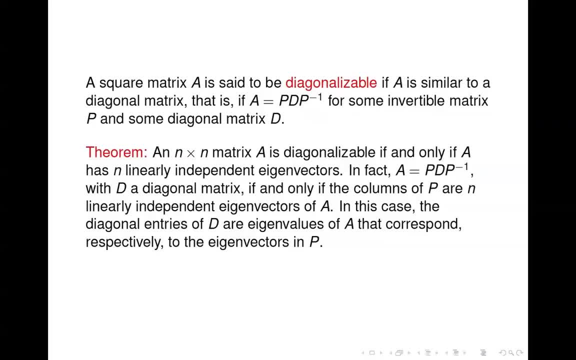 A condition Of which a is diagonalizable. It also tells us how to compute p and d. P is a matrix that consists of n linearly independent eigenvectors of a And continuing on, it says: the diagonal entries of d are eigenvalues of a that correspond. 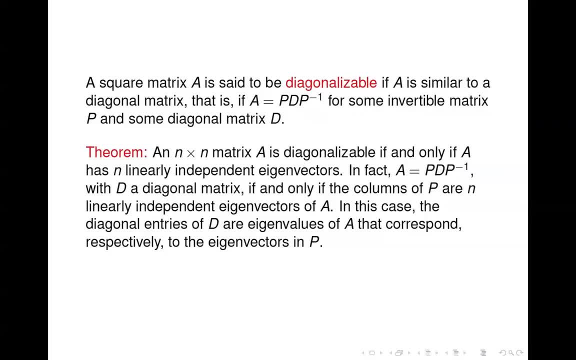 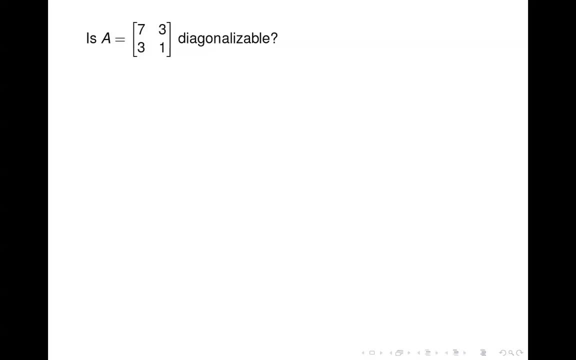 respectively to the eigenvectors in p. So p consists of the eigenvectors And d consists of the eigenvalues on the diagonal. So let's look at an example. Here's a matrix a. You can recognize this matrix. We looked at it in the video on the intro to eigenvalues and eigenvectors. 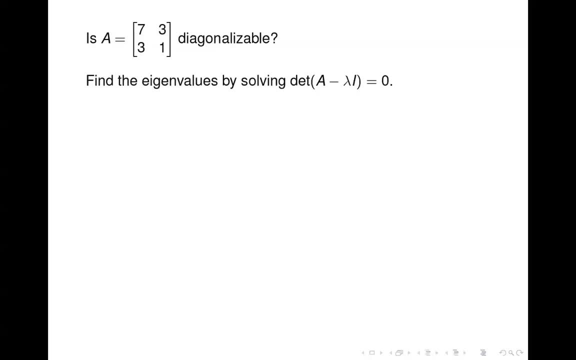 So is it diagonalizable? Well, let's find the eigenvalues. So we take the diagonal, We take the diagonal, We take the diagonal, We take the determinant of a minus lambda i, And we end up with lambda minus 8 times lambda plus 2 as our characteristic polynomial. 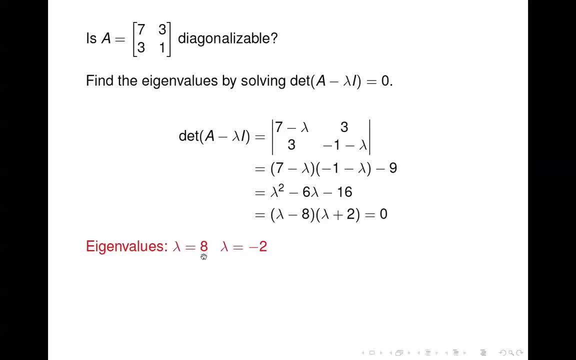 We set that equal to 0.. And so our eigenvalues are: lambda equals 8 and lambda equals negative 2.. Now at this point we know that a is diagonalizable because a has two distinct eigenvalues, So it's a 2 by 2 matrix. 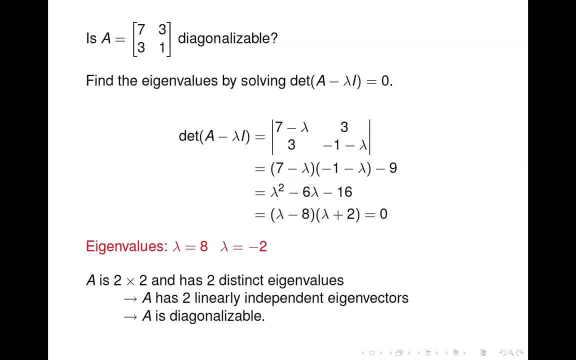 A matrix has two distinct eigenvalues. That means, since we know that distinct eigenvalues give us linearly independent eigenvectors, Eigenvectors that come from distinct eigenvalues are guaranteed to be linearly independent And therefore a is diagonalizable. Now to find p, we have to compute the eigenvectors. 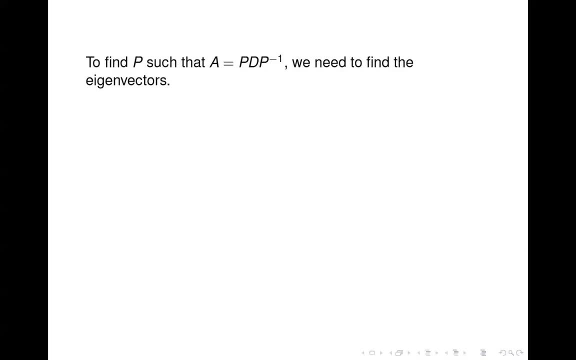 We already know what d is. d is a matrix, a diagonal matrix with the eigenvalues on the diagonal. So take lambda equals 8 and we need to solve a minus 8 times i times x equals a 0 vector. And so we solve that system and we end up with this vector in parametric vector form. 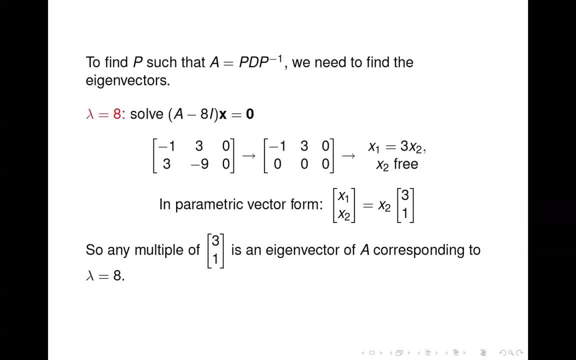 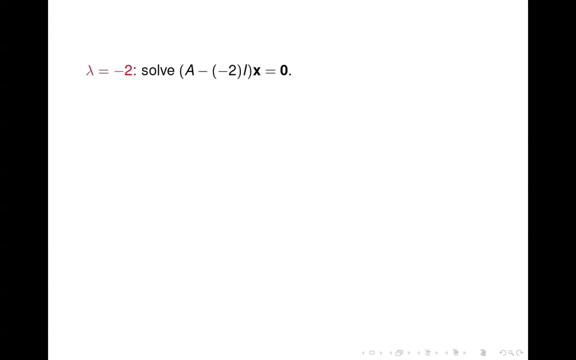 So any multiple of 3, 1 is an eigenvector of a corresponding to lambda. So at this point we have one column of p. To get the other column we look at the eigenvalue negative 2 and solve a minus negative 2i times. 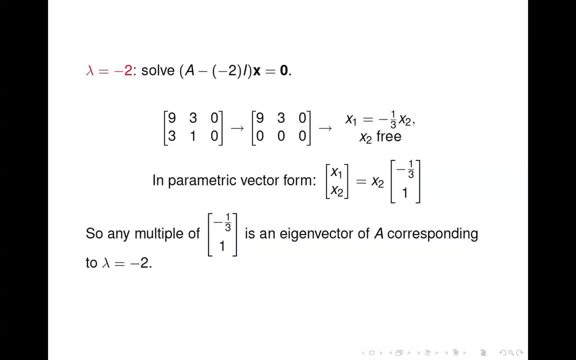 x equals 0. And here's that We end up with negative 1, third 1 as our eigenvector. So any multiple of that, Any non-zero multiple of that, would be an eigenvector, And so I multiplied by 3.. 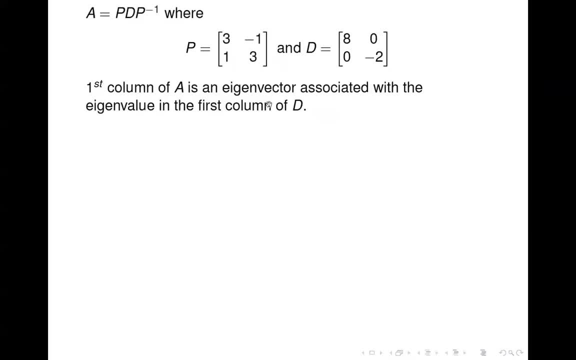 Go back to that. I multiplied it by 3.. And so we end up with negative 1: 3 for our second eigenvector. So the 3: 1 came from lambda, equals 8.. Negative 1: 3 came from lambda, equals negative 2.. 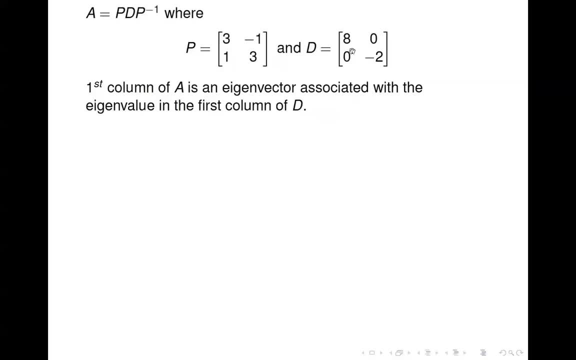 And so d consists of the eigenvalues, And the order To put the eigenvectors into p is not important. However, once you establish an order you have to hold that true for both p and d. So the eigenvector here- 3, 1 came from lambda- equals 8.. 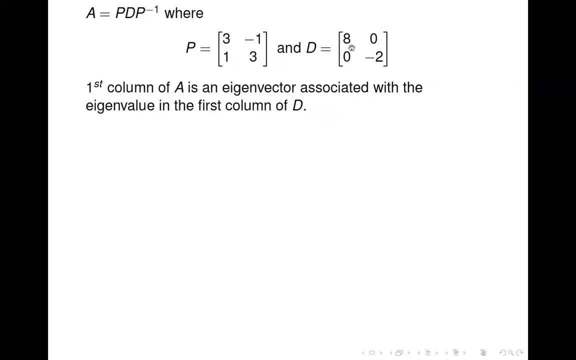 So we need the eigenvalue 8 in the first column of d, And then the eigenvector in the second column of p should correspond to the eigenvalue in the second column of d. All right, That's it, Thank you, Bye. 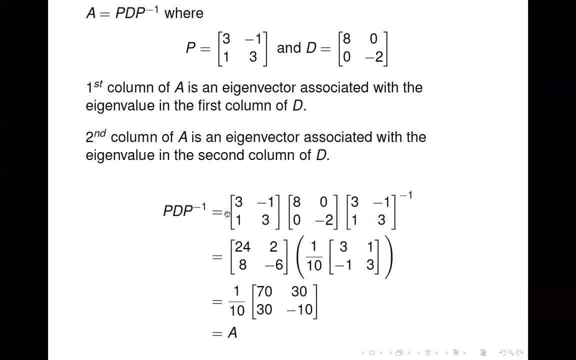 All right. And then, if we want to just check our work, we multiply pdp inverse And we end up with a. Go through that computation And you end up with a. So pdp inverse is equal to a. Let's look at another example. 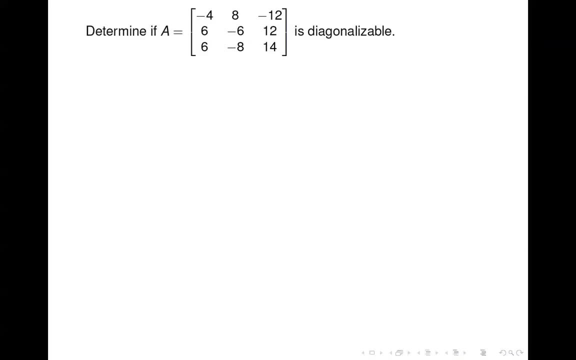 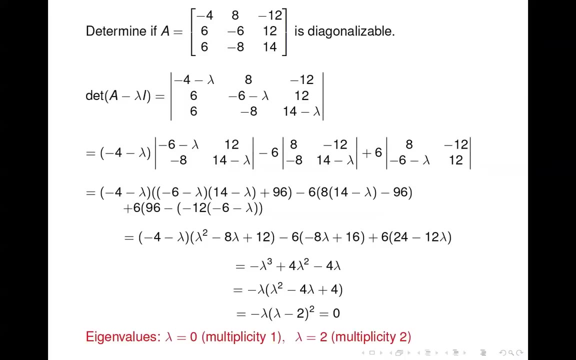 Here's another matrix, 3 by 3 in this case, And we want to know if it is diagonalizable. So, as before, we find its eigenvalues by looking at the determinant of a minus lambda i. We end up with this polynomial negative lambda times lambda minus 2, squared equals 0.. 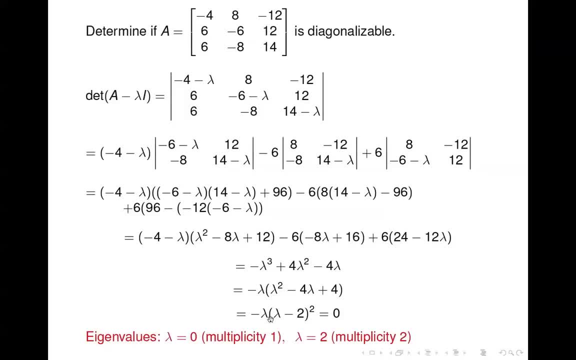 And the solutions will be lambda equals 0 and lambda equals 2.. Now lambda equals 0.. 0.. 2 occurs once. Lambda equals 2 occurs twice, since it's a squared term. So lambda equals 2 has multiplicity 2.. 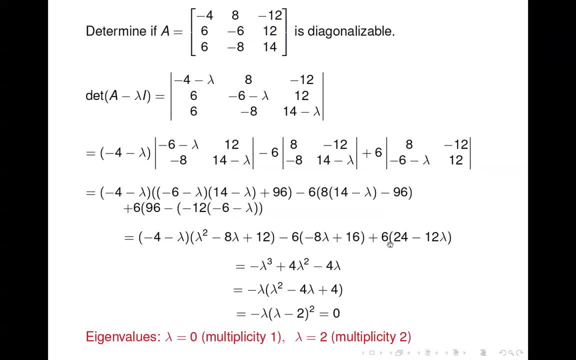 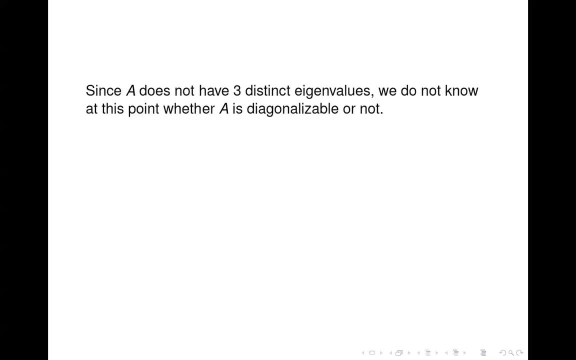 It appears twice as an eigenvalue. Now, at this point we know that a has only two distinct eigenvalues, So therefore we don't know if it has three linearly independent eigenvectors or not. So we don't know if a is diagonalizable or not. 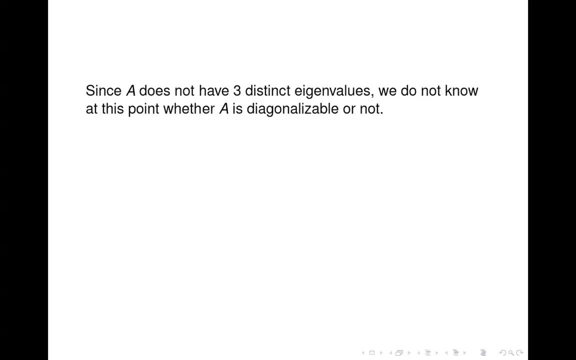 Just because it doesn't have three distinct eigenvalues doesn't mean that it's not diagonalizable. That theorem only goes one way: If it has n distinct eigenvalues, then it will be diagonalizable. If it doesn't have n distinct eigenvalues, you don't know whether it's diagonalizable. 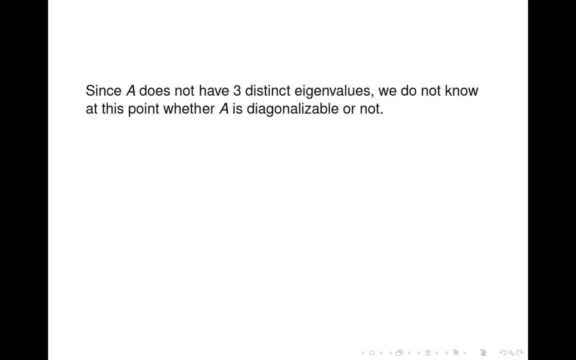 or not. You have to actually see if you can compute n linearly independent eigenvectors. So in this case that's what we've got to try And actually for this particular problem, the real question is whether lambda equals 2, which occurred with multiplicity 2, will have one or two linearly independent eigenvectors. 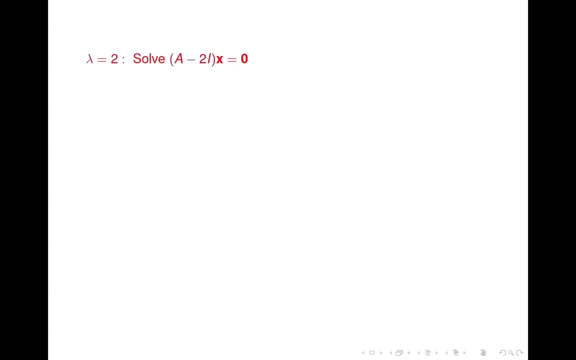 So let's look at lambda equals 2.. We solve a minus 2i times x equals 0. And we end up with notice in the matrix. here you can see that we've got two free variables. So therefore we're going to get two linearly independent eigenvectors from this eigenvalue. 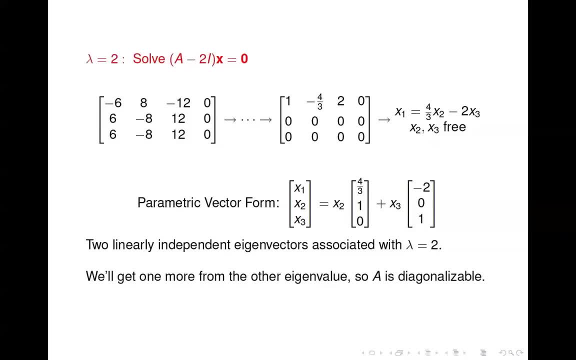 And so at this point we've got two linearly independent eigenvectors from lambda equals 2.. We know we'll get one more from the other eigenvalue. So at this point we know that a is diagonalizable And actually we're 2 thirds of the way towards producing the p. 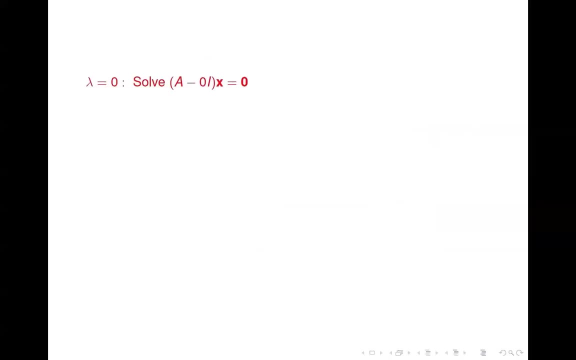 Such that a equals pdp inverse. So we look at the other eigenvalue of 0 and solve: a minus 0i times x equals 0. Then notice we've got one free variable. So we end up with one linearly independent eigenvector. 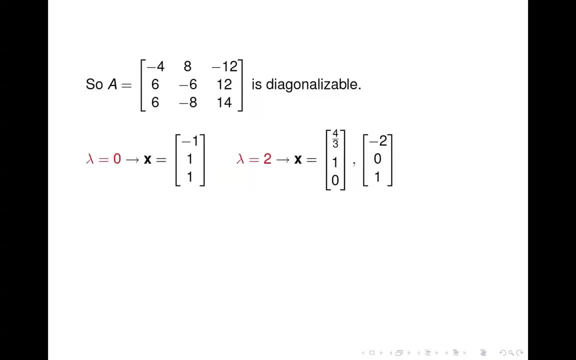 And so we know that a is diagonalizable. Here's our eigenvectors that we found. So we know that a is equal to pdp inverse. Where p is this matrix? Now notice that the negative 1, 1, 1 came from lambda equals 0. 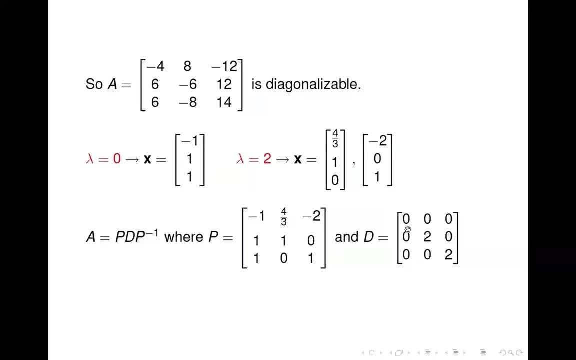 So that means in the first column of D I've got 0. here in the diagonal entry These last two eigenvectors came from lambda equals 2.. And so in the second column and the third column of D I've got 2 on the diagonal. 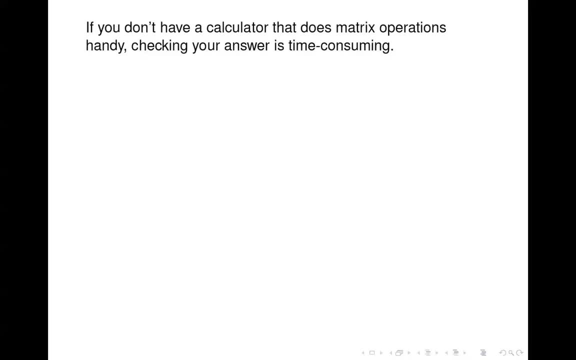 Now Before, In the 2 by 2 example we actually checked our answer by computing pdp inverse. But for 3 by 3, it's not so simple to compute an inverse And if you've got a calculator that's not that bad. 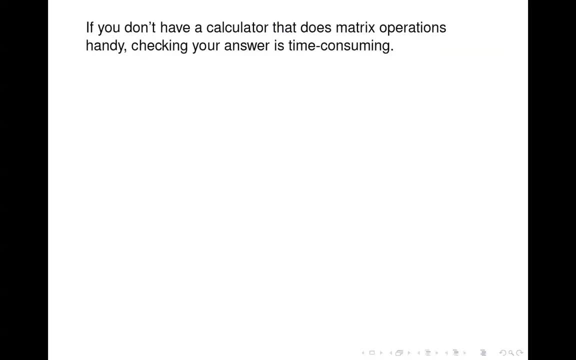 But if you don't, then there's an easier way to check your answer And that is to note that if a is equal to pdp inverse, if we multiply both sides of that equation by p On the right, Then we end up with P inverse times P, which goes away. 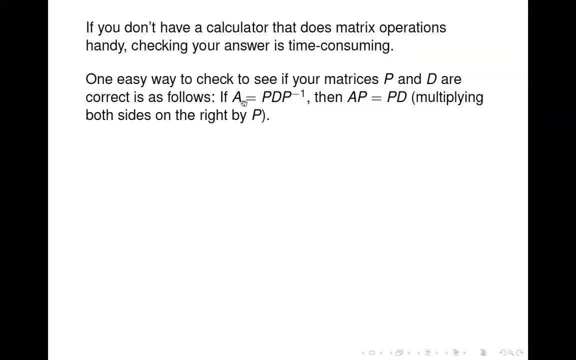 And then we end up on the left-hand side with A times P. So AP would equal PD, And so we can compute both those matrices. since it only involves multiplication of matrices, You don't have to find any inverses, So you can check to see if AP is equal to PD. 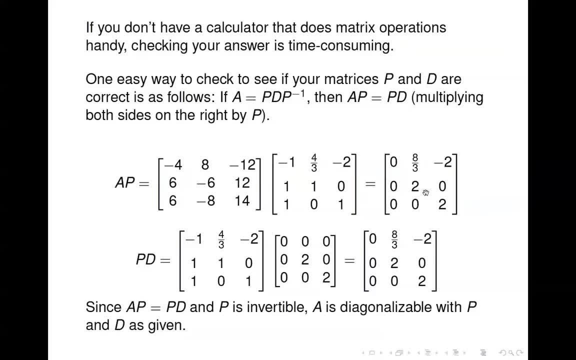 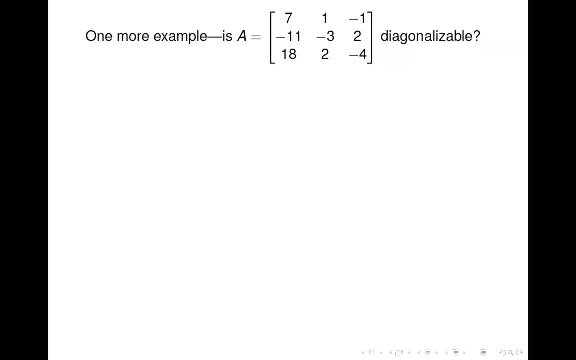 So if we compute both of those, you can see that in this case they are indeed the same, And so we can conclude that our P and D are correct. All right, let's look at one more example. Here's another 3 by 3.. 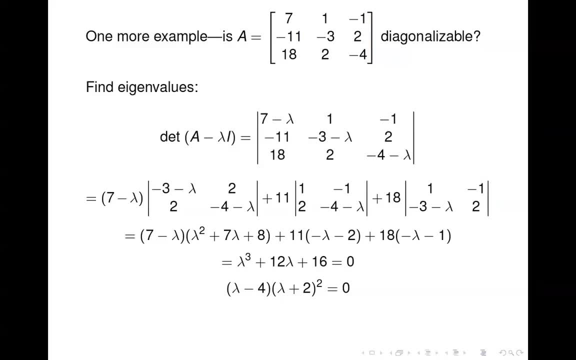 We want to know if it is diagonalizable. So we find the eigenvalues- I'm expanding about the first column here- when I take the determinant and end up with lambda minus 4 times lambda plus 2 squared, So again I don't have 3.. 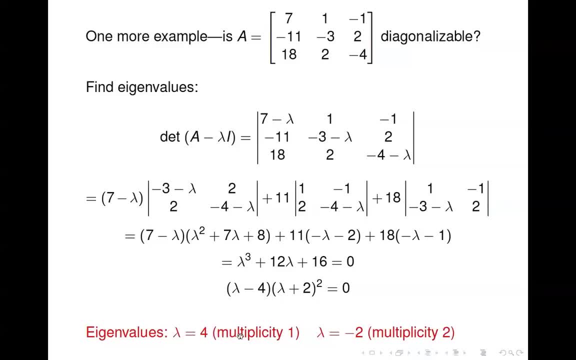 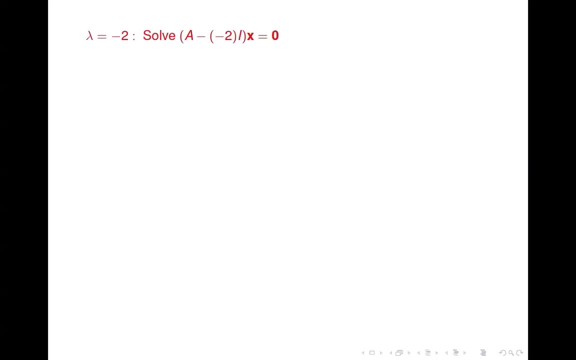 I only have 3 distinct eigenvalues. I only have 2.. Lambda equals 4 occurs with multiplicity 1.. Lambda equals negative 2 occurs with multiplicity 2.. So we want to know: does lambda equal negative 2 have, or we're going to get 2 linearly independent eigenvectors out of it? 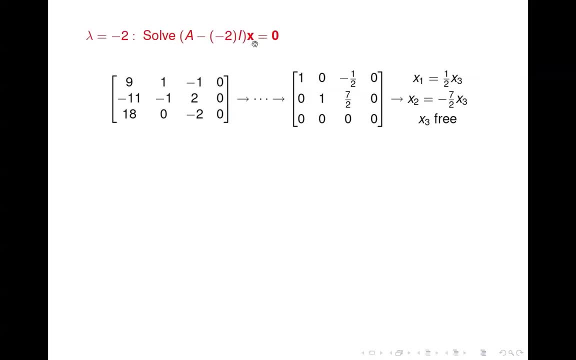 And when we solve A minus minus 2I times 2, which is x equals 0,, notice that we end up with this matrix in echelon form, And so we only have one free variable right. x3 is free, And so we don't get 2 linearly independent eigenvectors out of this eigenvalue. 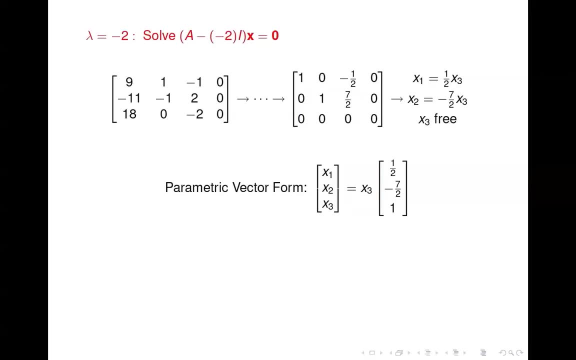 And so we only get 1.. We're only going to get 1 linearly independent eigenvector from the other eigenvalue lambda equals 4.. So that means we're only going to end up with 2 linearly independent eigenvectors. 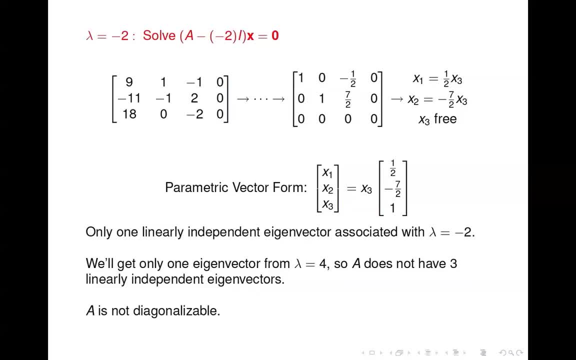 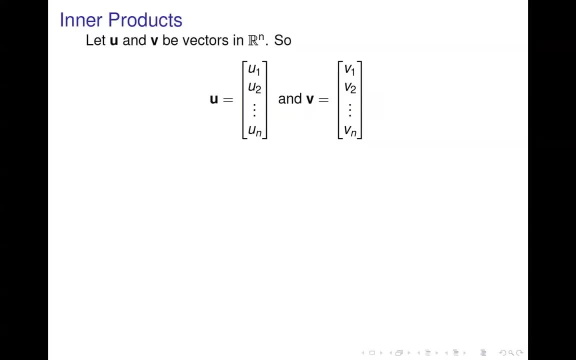 And that means that A is not diagonalizable in this case. Okay, so we're into chapter 6 now and section 6.1. And let's start off with inner products. We've discussed this before, I believe, when we were talking about how to multiply a matrix by a vector. 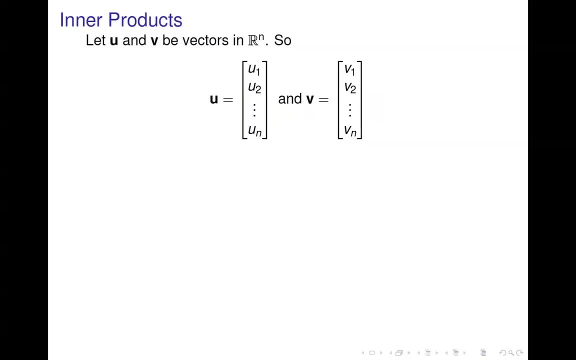 But Let's hit that again here. So the inner product is defined on two vectors that have to be the same length. So let's suppose that u and v are vectors in Rn. The inner product, also called the dot product of u and v, is given by u1 times v1 plus u2 times v2 plus dot, dot, dot, un times vn. 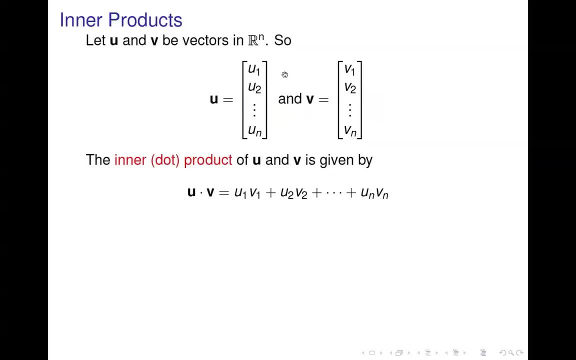 So we simply match up The elements, corresponding elements, multiply and then add them all up. The notation is, as indicated here, where there's a dot u, dot v, And that's where the term dot product came from, just because you normally see it written like that. 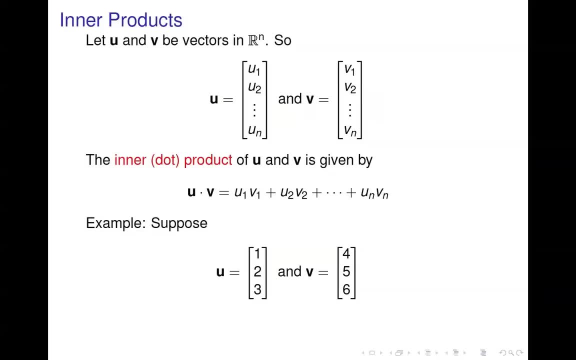 So for an example, suppose we have these two vectors, u and v, to compute their inner product. We just match up elements again, So 1 times 4 plus 2 times 5 plus 3 times 6. And so we end up with 32.. 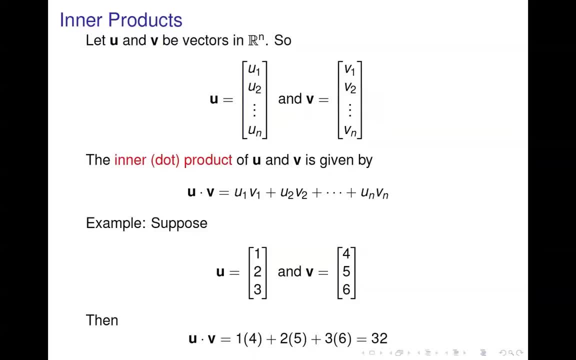 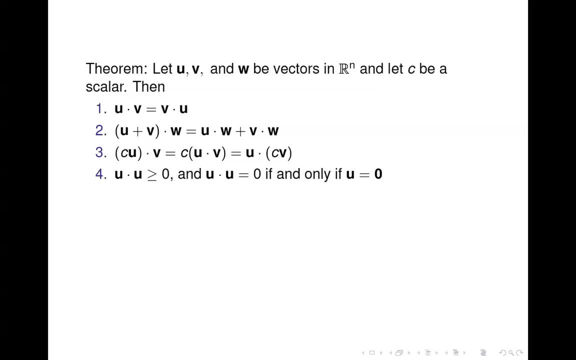 So the inner product of two vectors yields a scalar value. Okay, here's some properties of inner products. The fourth one, I think, is the most interesting because it discusses the inner product of a vector with itself And if we examine that, you see that u dot u. 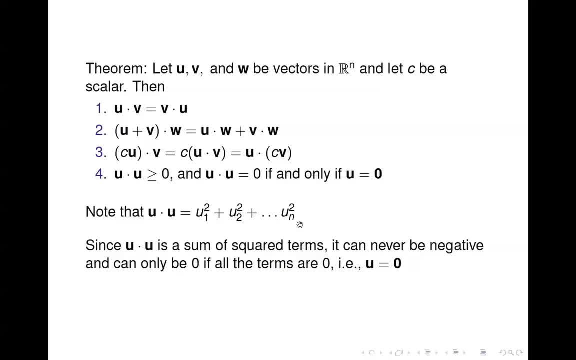 It's just u1 squared plus u2 squared plus dot dot dot plus un squared. So since we're adding up a bunch of squared terms, then it has to be non-negative. And notice that the only way that it can be zero, notice it's always going to be greater than or equal to zero. 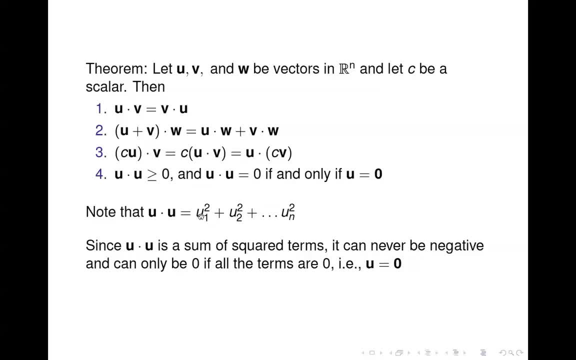 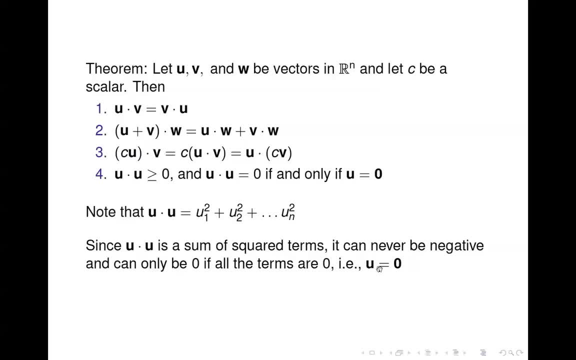 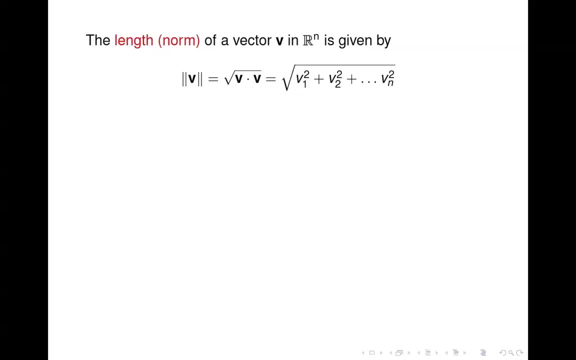 they all have to be zero for the sum to be zero. Okay, so u dot. u is always greater than or equal to zero, and it equals zero if, and only if, u is the zero vector. Okay, on to the length of a vector. 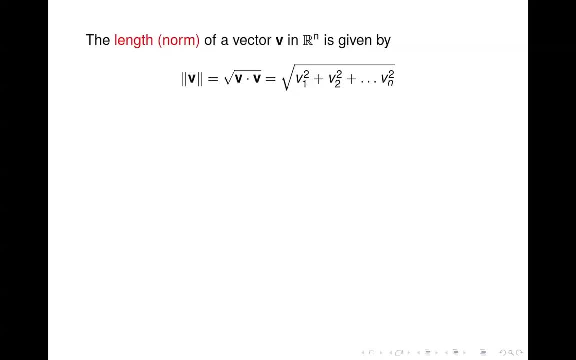 The length of a vector, also called the norm of a vector. If you go and take more math courses, you might encounter the idea of a norm later on, and there are different types of norms. This is just one of them. Actually, it's called the two norm. 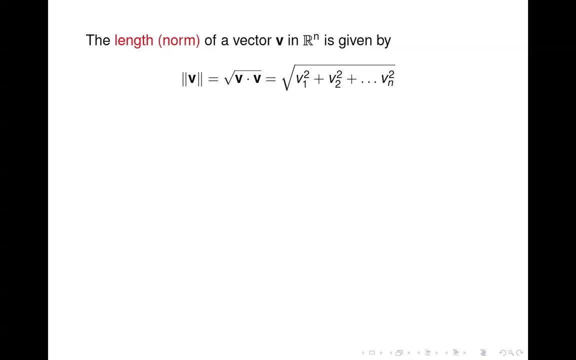 because we're squaring the entries and then taking a square root. Okay, but you see the notation: the double vertical bars indicates length or norm And it's just a square root of a vector with itself. Okay, So we know what v dot v is the sum of these squares. 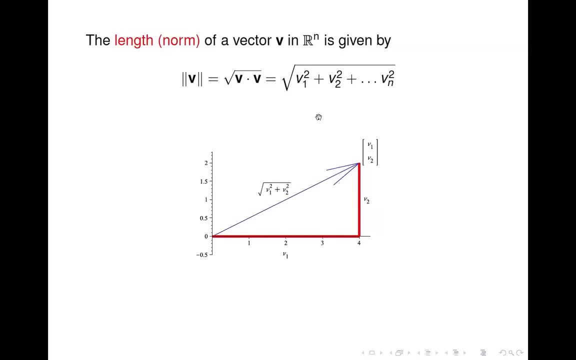 and so then we just take the square root of that In two dimensions it's easy to see how this works. So we have this vector, the blue one, here. Let's say it's v1, v2. Then we know that this distance here along the x-axis is v1,. 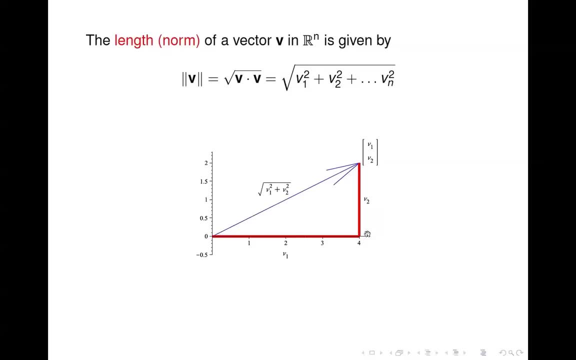 since that's the first component, And we know that the distance vertically is v2, since that's the second component And we have a right triangle here, And so by the Pythagorean theorem we know that the length of the hypotenuse here 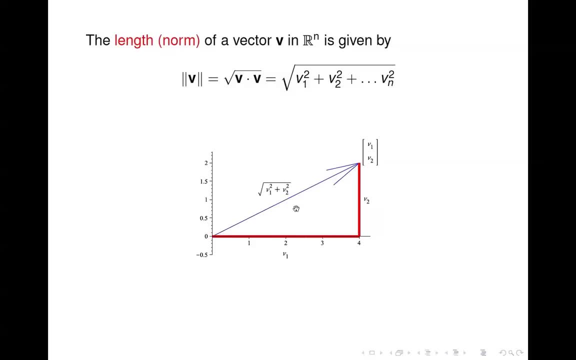 which is the length of v, is square root of v1 squared plus v2 squared. So this is clear in two dimensions And actually this scales. As you see it scales to n dimensions. Still use the same formula. At times we're interested in the number of times. 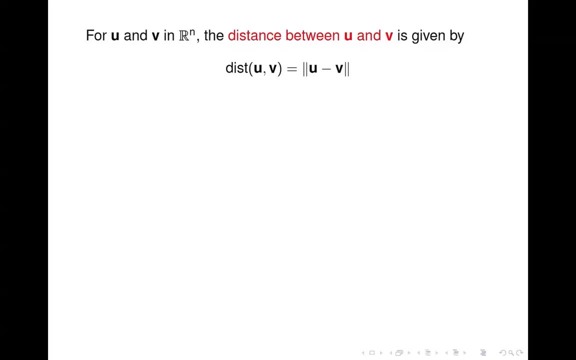 and we're interested in the number of times. At times we're interested in finding the distance between two vectors. okay, And so we denote that in this form: dist u of v, And that's equal to the length of the vector u minus v. 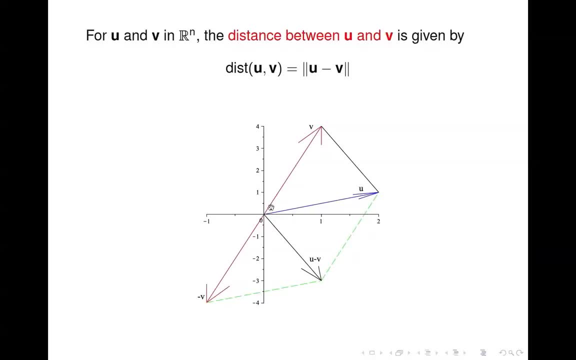 So let's see how that works. So here we have a vector u and here's a vector v, And what we'd like to determine is the distance between u and v. So that's the length of this line segment here. 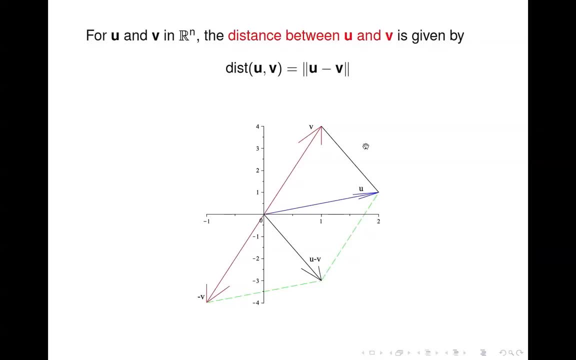 the black line segment. So let's examine what u minus v looks like. Well, that's u plus minus v, okay, So here's minus v down here. u's still here, And so if we do the parallelogram method, 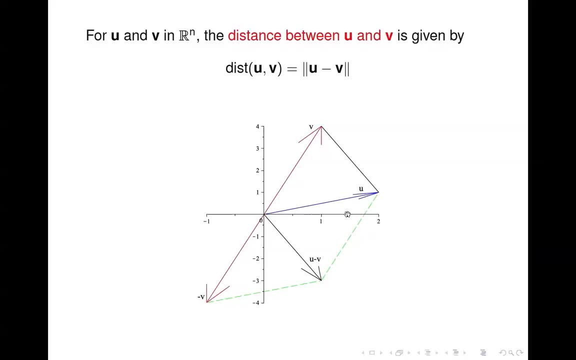 to compute u plus negative v, we end up with this vector. So here's u minus v right here, And you can see from the picture that it's the same length as this distance. It's the same distance between u and v. 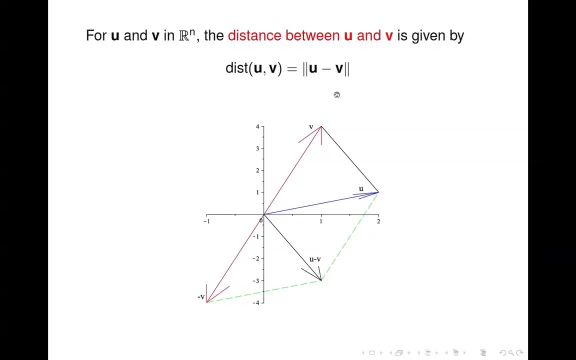 And so that's why we compute the distance between u and v as the length of u minus v. All right, we say two vectors are orthogonal to each other if their inner product is zero. Orthogonal is. looks like two vectors are orthogonal. 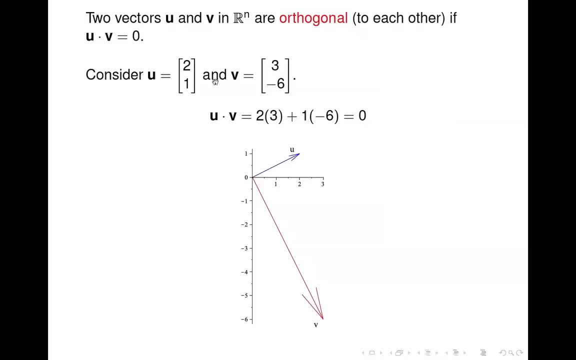 It means it looks like they're perpendicular, As you see here. here's a couple vectors: two, one and three negative six. If you take the inner product you end up with zero, And if you look at those plotted,